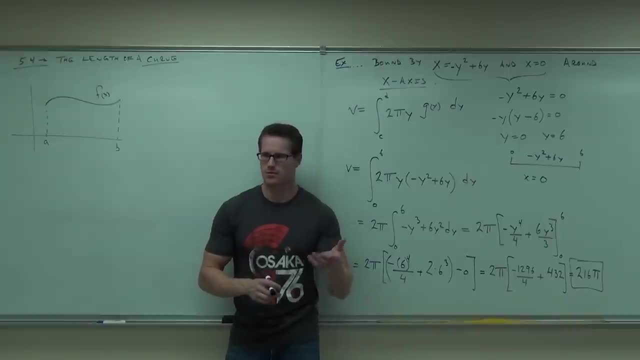 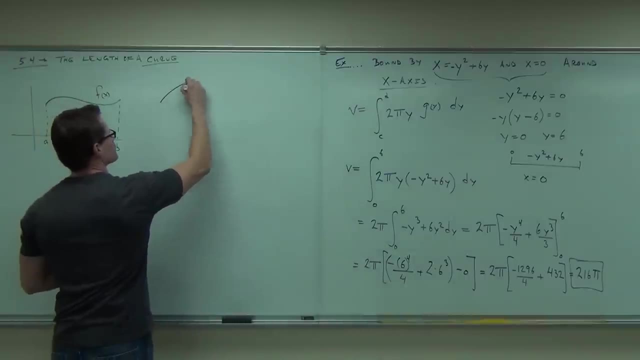 An area. Let me give you- maybe pause it- a different idea. Okay, What if we were to take part of this curve? Now, maybe that's this part right here. How would you find, using the idea of some calculus? 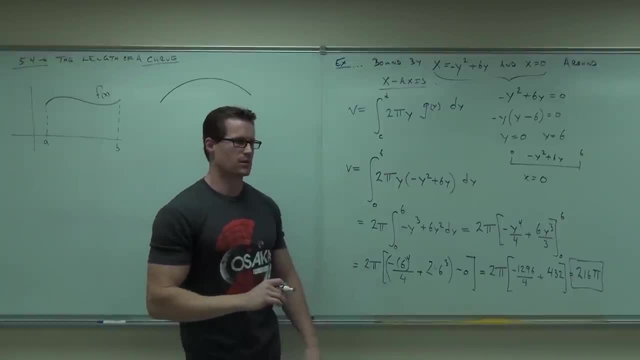 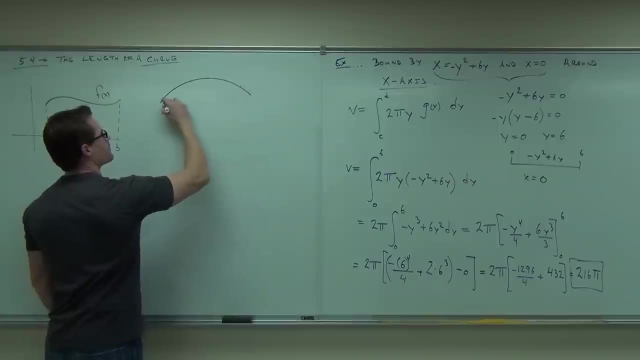 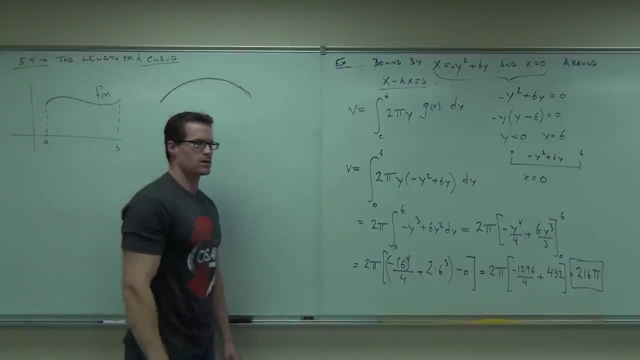 how would you find the length of something Change of that? We're going to be using some sort of limit, sure? Well, what if I were to divide this up and go and make straight lines? Can you find the length of a straight line? 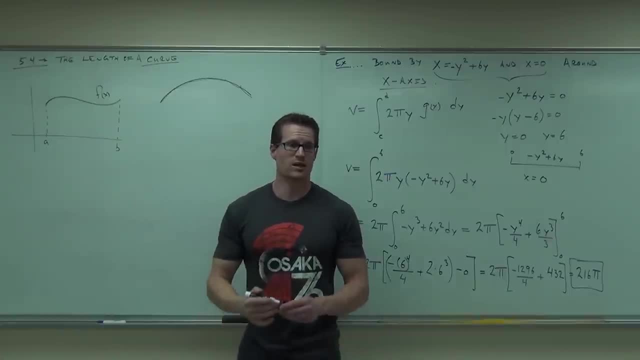 You can get sound effects on that Right. Can you find the length of a straight line? Geez, I hope so, And if you know the distance from here and the distance from here, you should be able to use Pythagorean theorem and find the distance of a straight line, right. 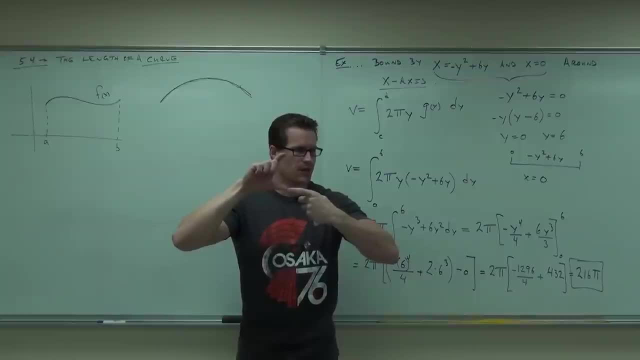 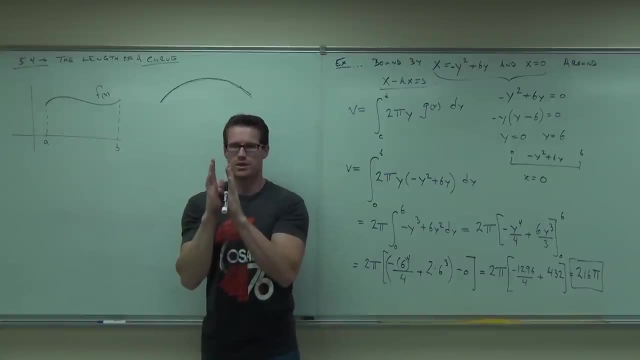 Now, of course, that's going to be approximation. However, if we move this distance to here, all these distances really really close, the length of the straight lines will be exactly the same as the length of those curves for those little teeny, itty-bitty pieces. 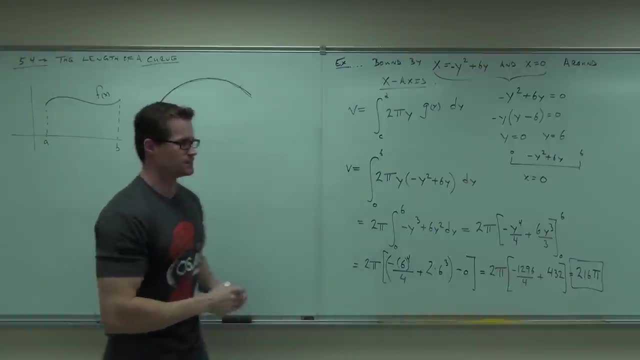 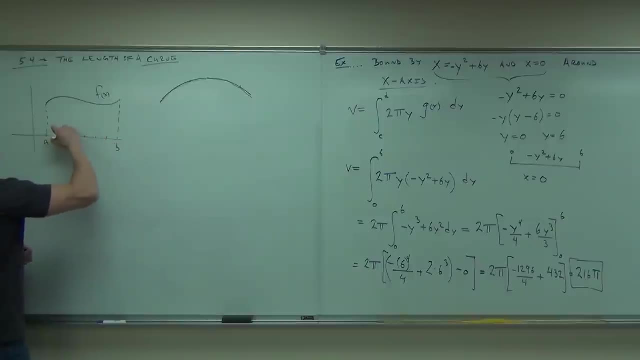 Have you seen the limit idea come back again? So here's our idea. Our idea is: let's go ahead and do the same exact thing we've been doing Now. we don't care so much about the height, We don't. 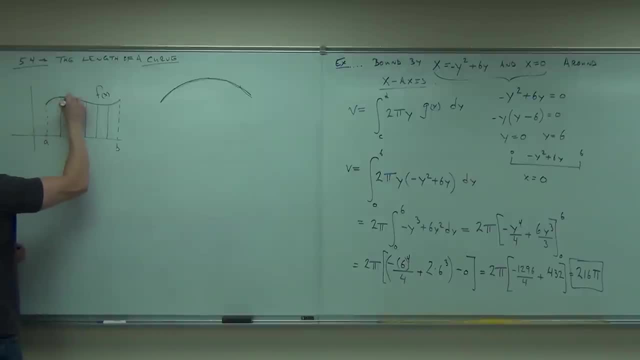 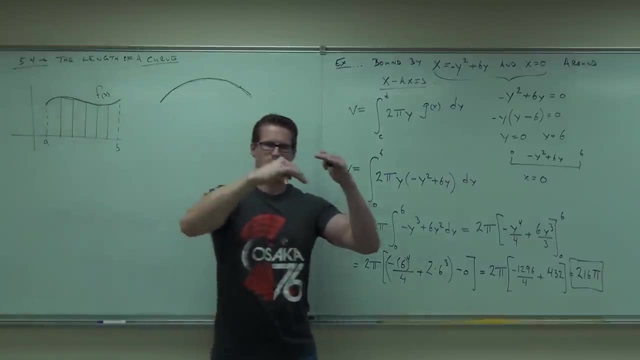 What we care about is this, this, that distance, that distance and that distance. We're going to truncate all the curves. We're going to truncate it. Just make a straight line from this point to that point where the vertical touches the function, to where the next vertical touches the function. 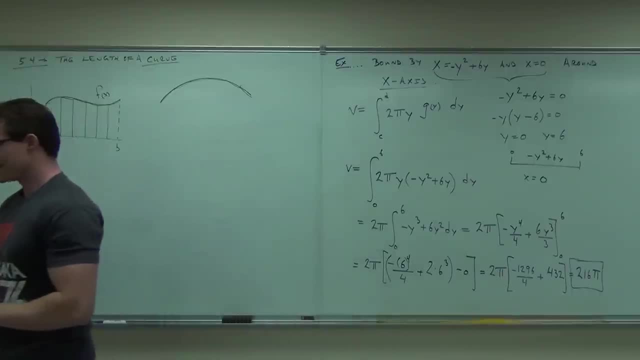 and try to find out where that is. So the idea is: let's cut these into small sections and let's add those lengths together. That's the idea. Very similar to areas, but we're not talking about areas, we're talking about lengths. now 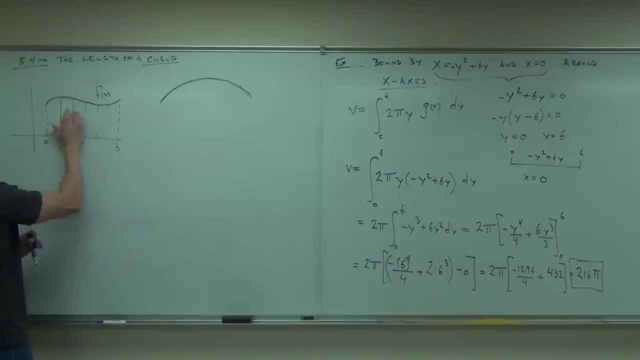 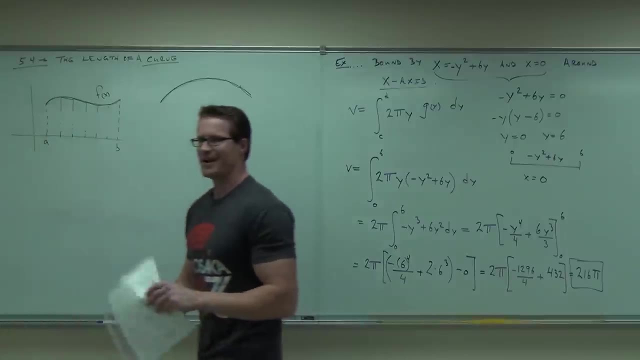 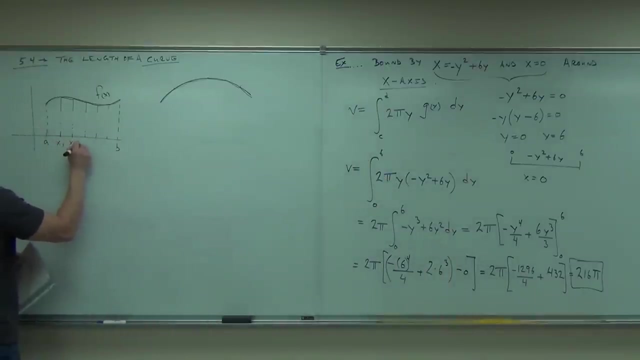 So this we don't care so much about. Just up here. Are you ready to go through and see how to do this? Ready? So if we call this x sub 1, the first cut and x sub 2, then we're going to get all the way up to the x sub nth cut. 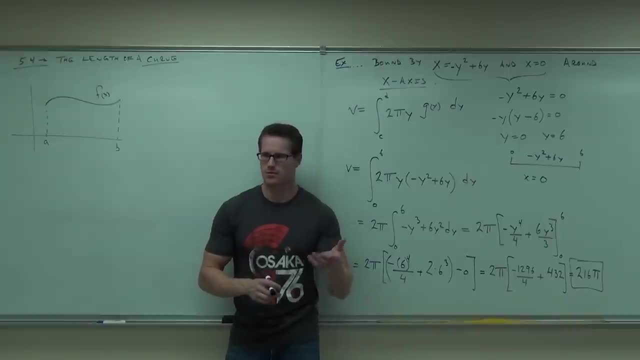 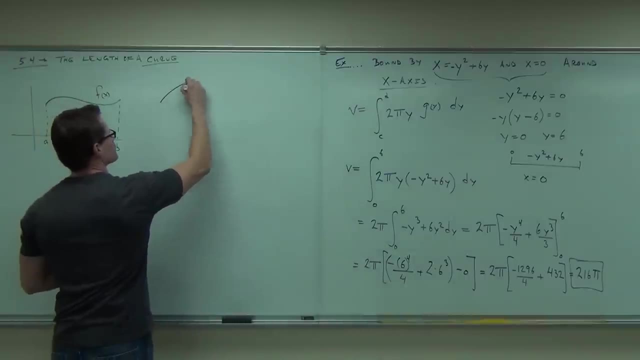 An area. Let me give you- maybe pause it- a different idea. Okay, What if we were to take part of this curve? Now, maybe that's this part right here. How would you find, using the idea of some calculus? 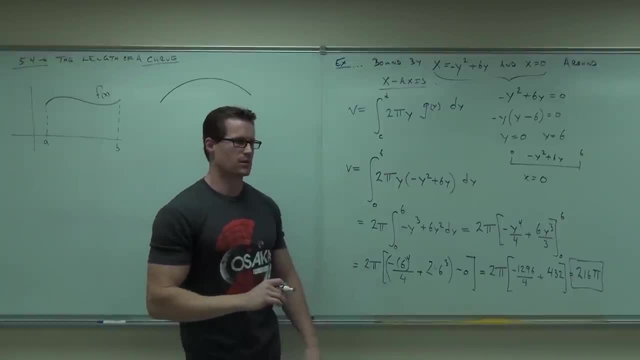 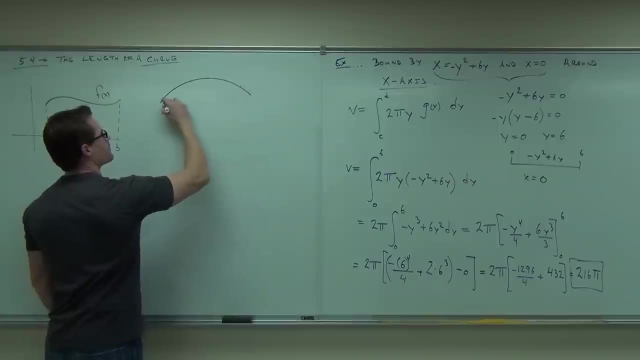 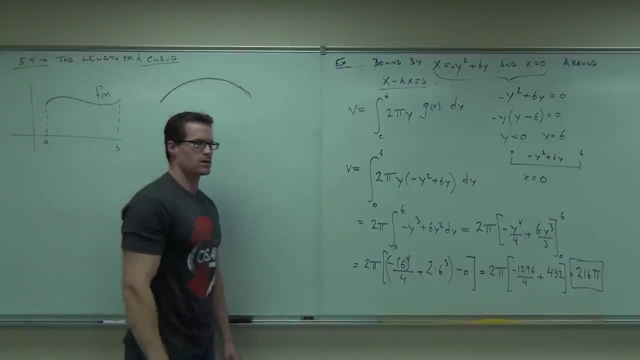 how would you find the length of something Change of that? We're going to be using some sort of limit, sure? Well, what if I were to divide this up and go and make straight lines? Can you find the length of a straight line? 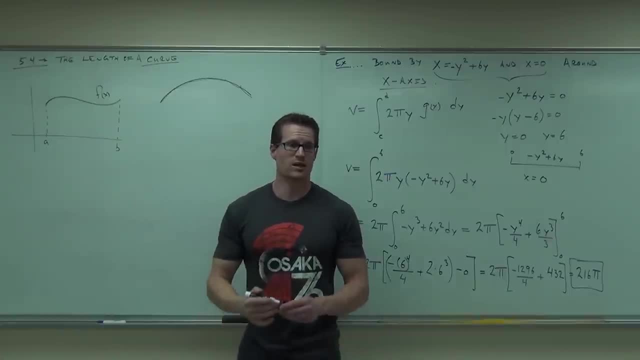 You can get sound effects on that Right. Can you find the length of a straight line? Geez, I hope so, And if you know the distance from here and the distance from here, you should be able to use Pythagorean theorem and find the distance of a straight line, right. 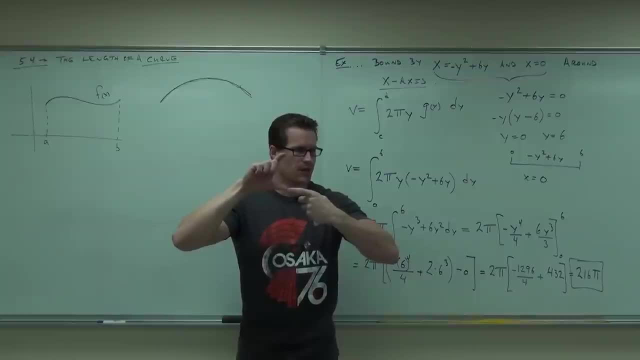 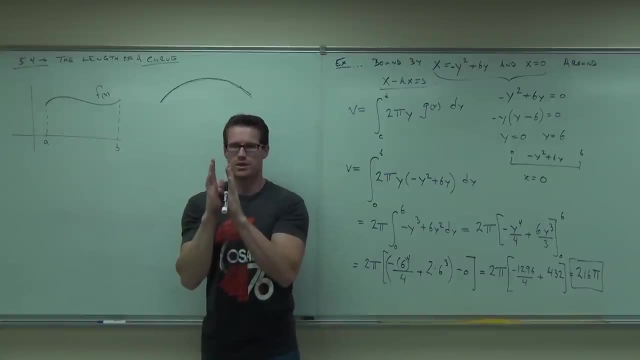 Now, of course, that's going to be approximation. However, if we move this distance to here, all these distances really really close, the length of the straight lines will be exactly the same as the length of those curves for those little teeny, itty-bitty pieces. 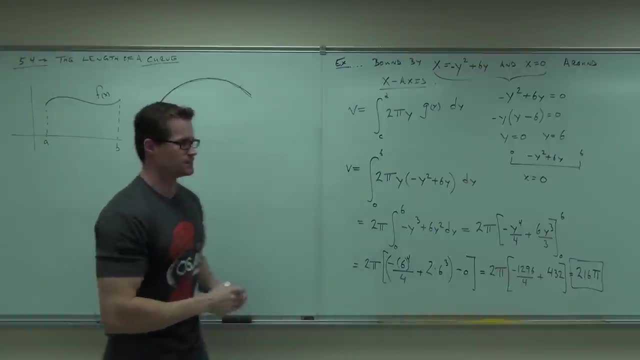 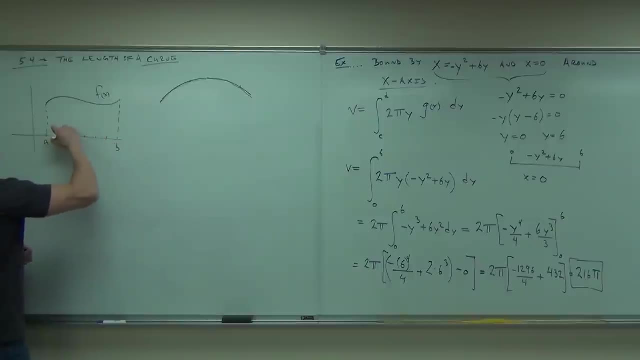 Have you seen the limit idea come back again? So here's our idea. Our idea is: let's go ahead and do the same exact thing we've been doing Now. we don't care so much about the height, We don't. 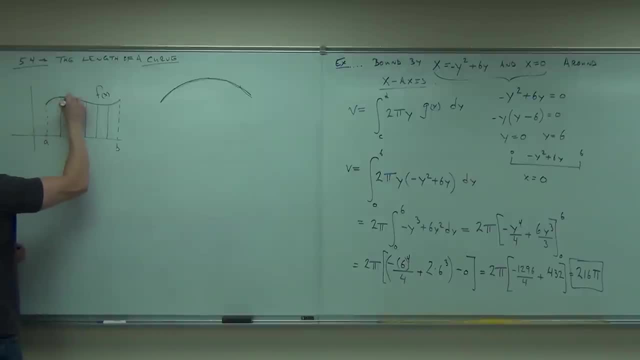 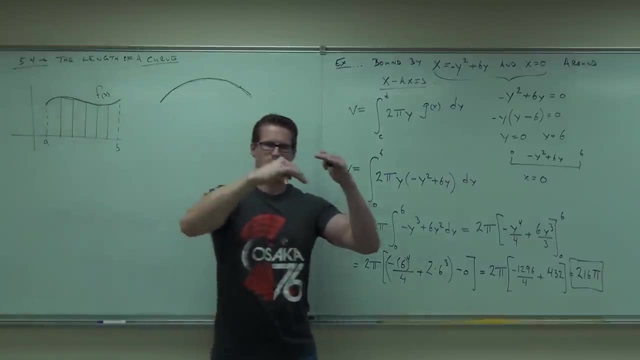 What we care about is this, this, that distance, that distance and that distance. We're going to truncate all the curves. We're going to truncate it. Just make a straight line from this point to that point where the vertical touches the function, to where the next vertical touches the function. 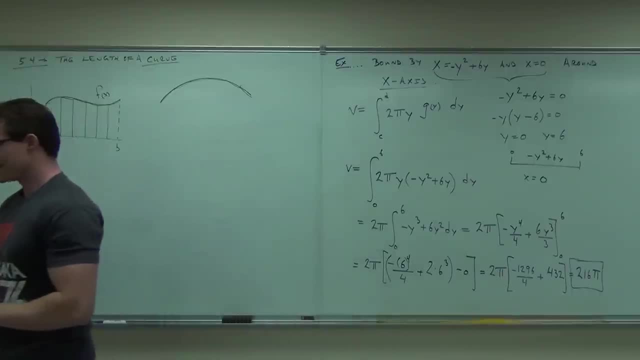 and try to find out where that is. So the idea is: let's cut these into small sections and let's add those lengths together. That's the idea. Very similar to areas, but we're not talking about areas, we're talking about lengths. now 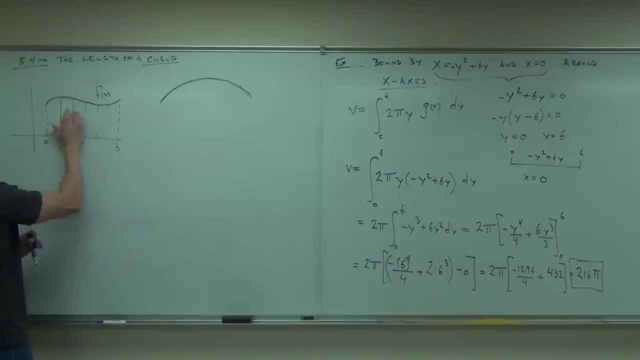 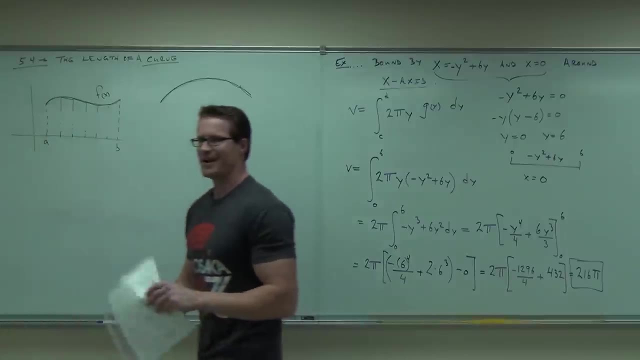 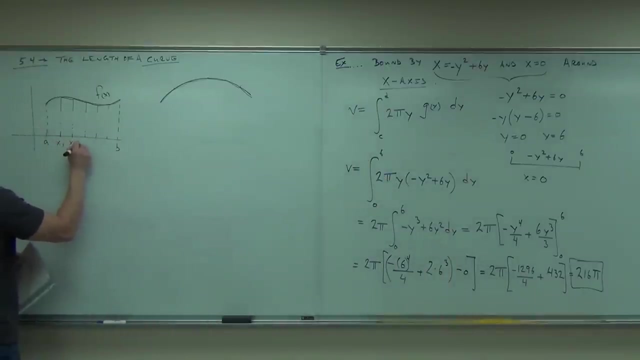 So this we don't care so much about. Just up here. Are you ready to go through and see how to do this? Ready? So if we call this x sub 1, the first cut and x sub 2, then we're going to get all the way up to the x sub nth cut. 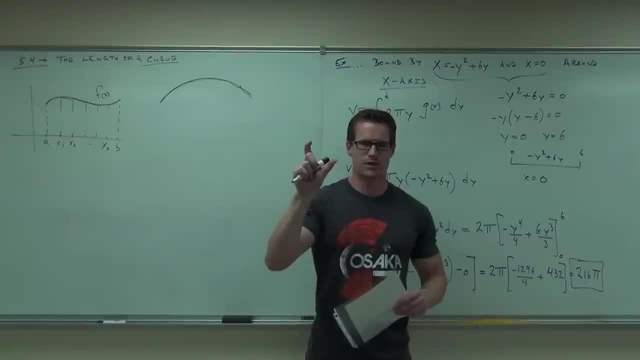 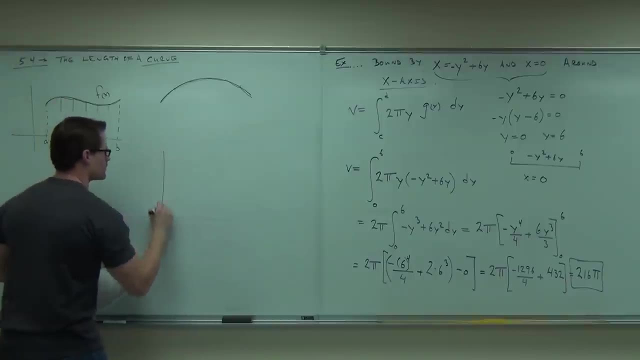 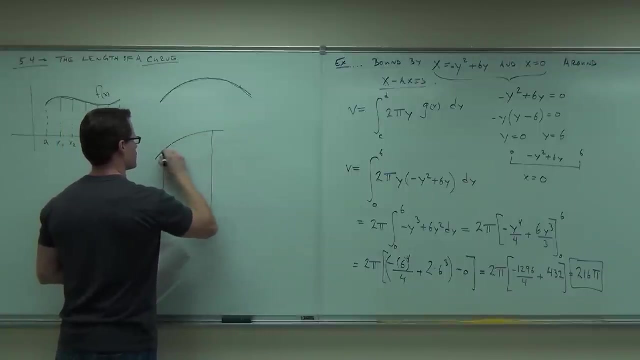 Can I take one of these pieces and blow it up for you so you see what's really going on here? Let's take something that looks like: how about this very first piece? Now, I'm going to be pretty general. I can't call this x sub 1, so I'm going to call it x sub k. 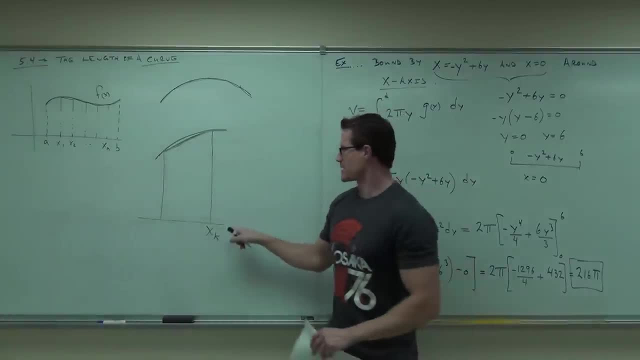 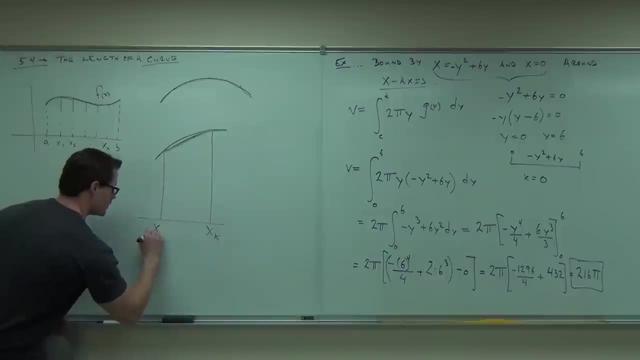 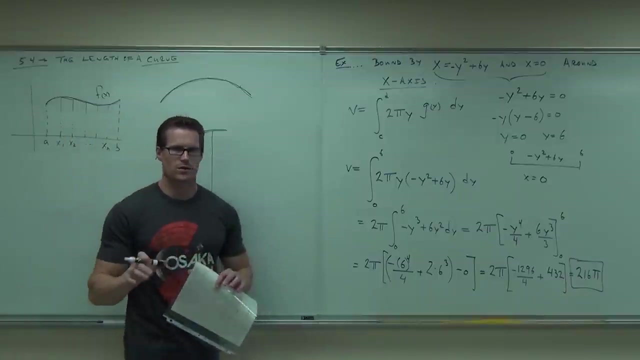 You guys are right with that one x sub k. If that's x sub k, tell me how much. that is Very good. the previous one: Brilliant. Okay, now you know our goal right. Our goal here is to do this. 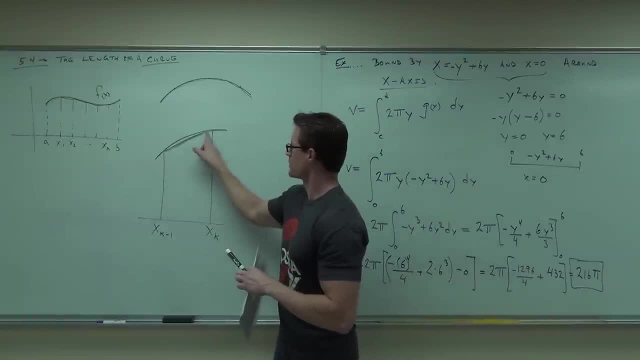 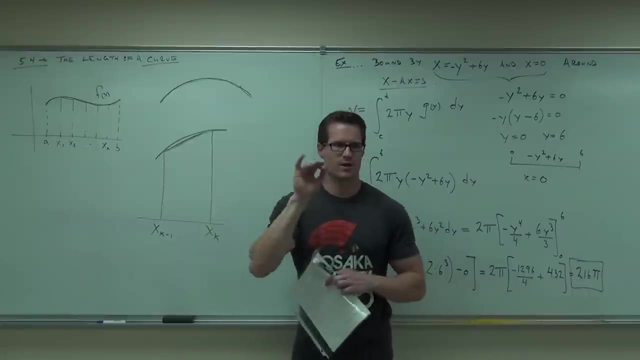 The goal is to find the length from here to here. That way, when I make this distance really, really, really, really, really small, it's going to very, very, very closely approximate that curve's length as well. Did you get the idea there? 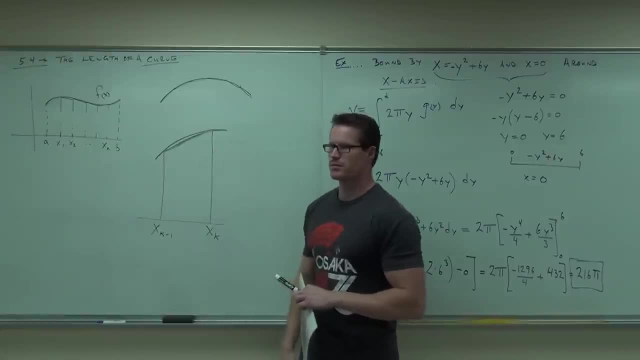 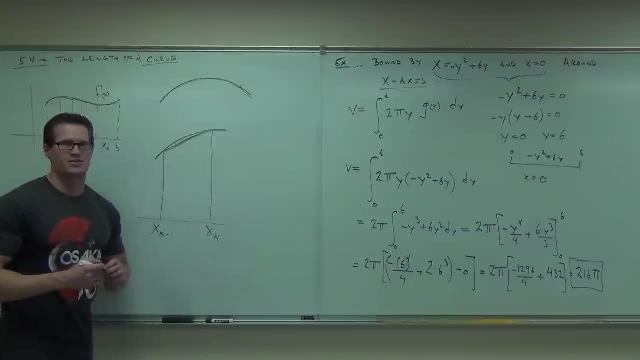 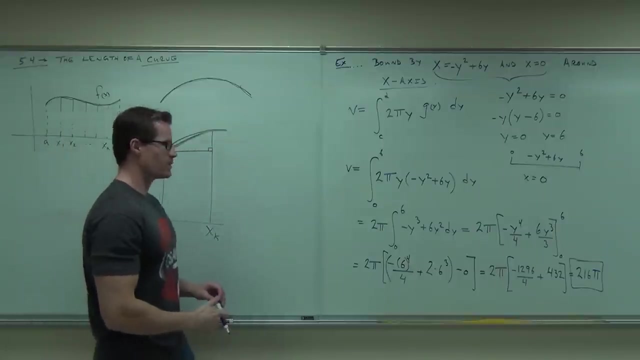 Okay Now how do you find the length Ideas? This is kind of a secret. mine Make a 90 degree triangle, Make a 90,. oh, that's a great idea. Why don't we make a 90 degree triangle? 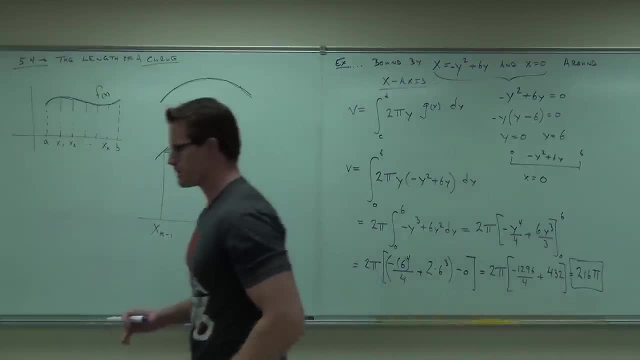 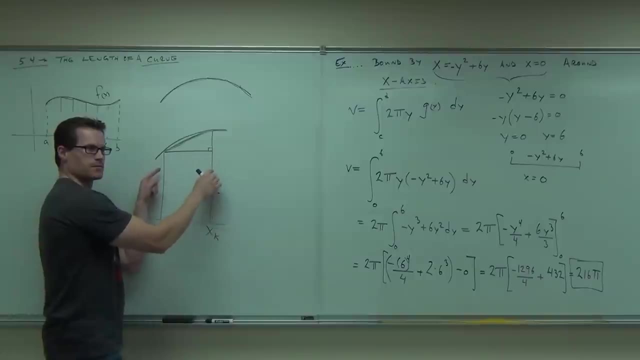 Why don't we make a 90 degree triangle? Let's talk about this for a bit, just for a second. What's this distance? You're overthinking it. What's the distance every time we go from one cut to another? L times. 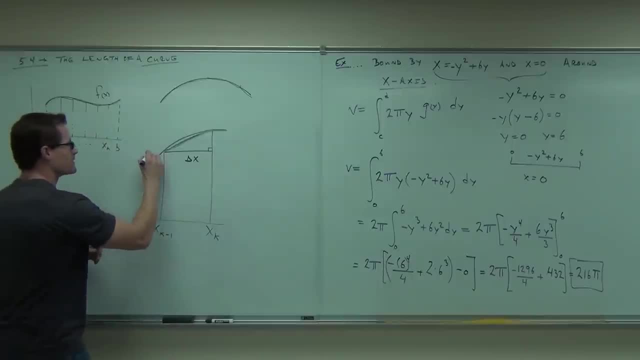 Yes, How high is this from here to here? F of X. No, No, not F of X. You're close, though You have the idea. F of X. F of K, Yeah, Not sub K, K minus 1.. 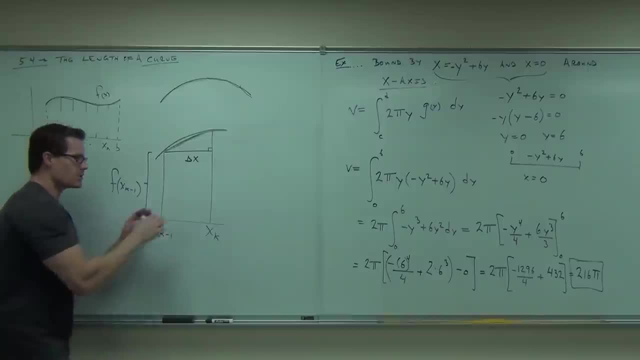 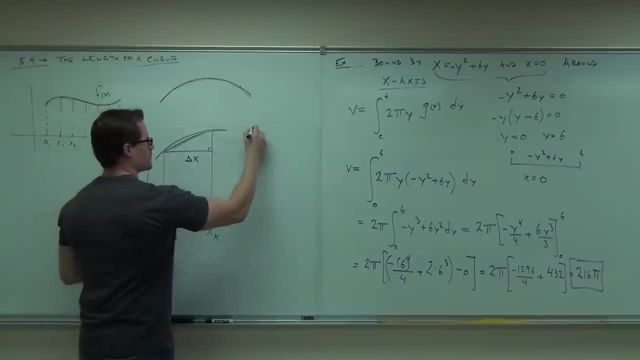 Oh Yes, Do you notice that? that's the height at that exact point. That's the function. That's going to be the height of that function there too. Now, Okay, Okay, Okay, Okay, Okay, Okay. What's the height here? 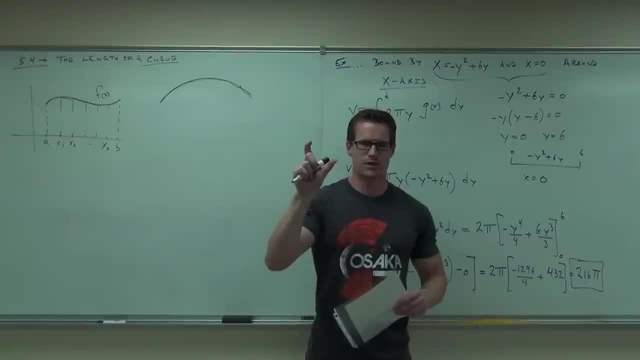 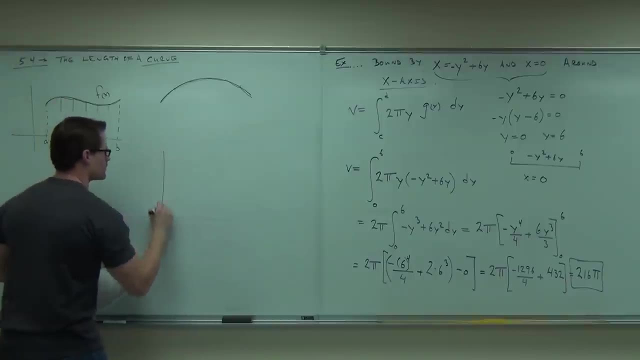 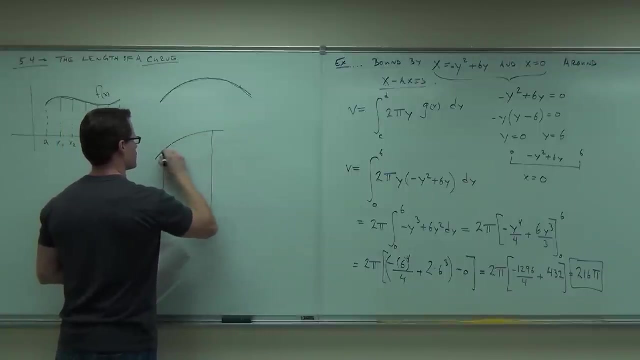 Can I take one of these pieces and blow it up for you so you see what's really going on here? Let's take something that looks like: how about this very first piece? Now, I'm going to be pretty general. I can't call this x sub 1, so I'm going to call it x sub k. 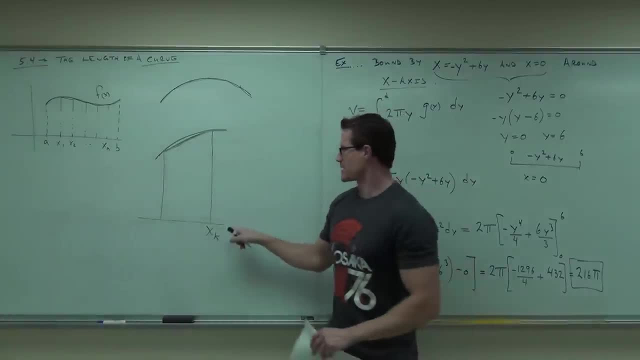 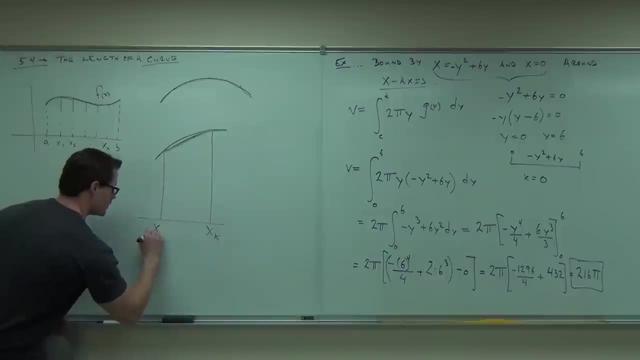 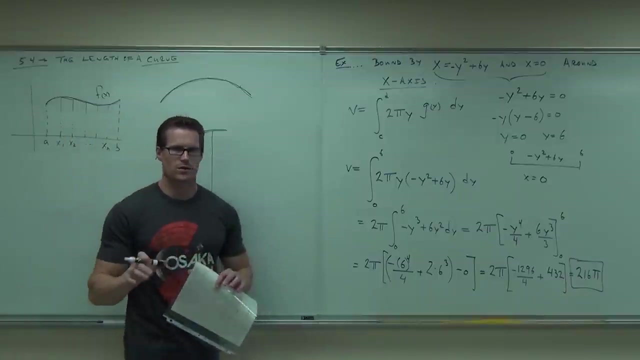 You guys are right with that one x sub k. If that's x sub k, tell me how much. that is Very good. the previous one: Brilliant. Okay, now you know our goal right. Our goal here is to do this. 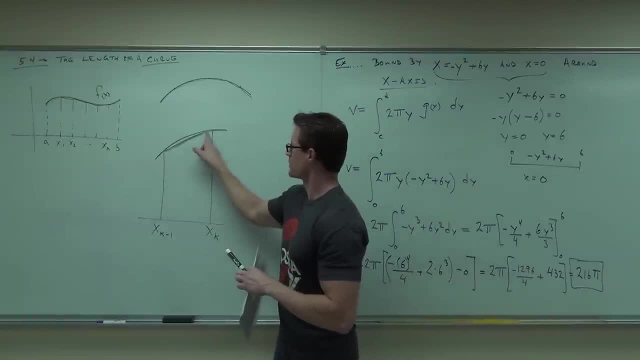 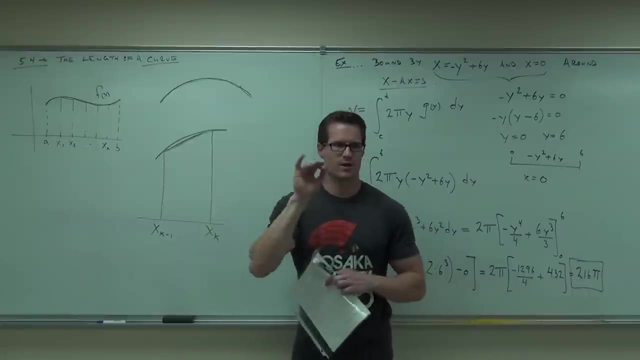 The goal is to find the length from here to here. That way, when I make this distance really, really, really, really, really small, it's going to very, very, very closely approximate that curve's length as well. Did you get the idea there? 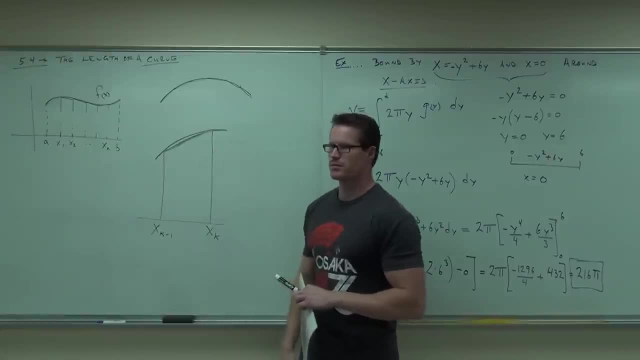 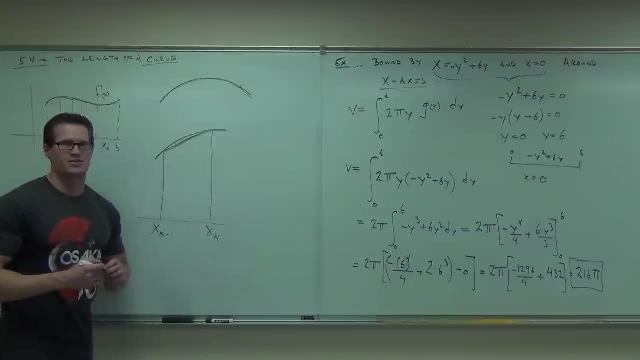 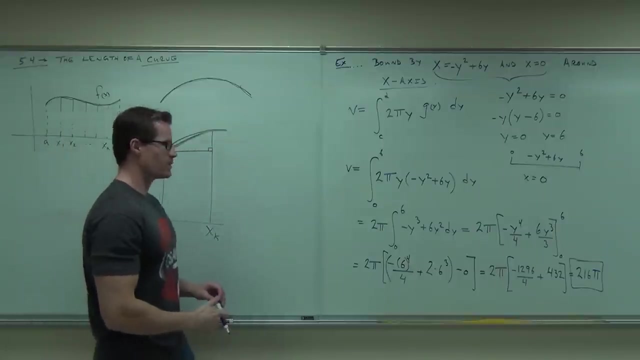 Okay Now how do you find the length Ideas? This is kind of a secret. mine Make a 90 degree triangle, Make a 90,. oh, that's a great idea. Why don't we make a 90 degree triangle? 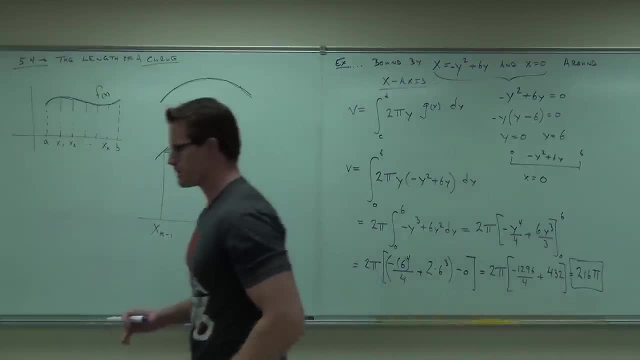 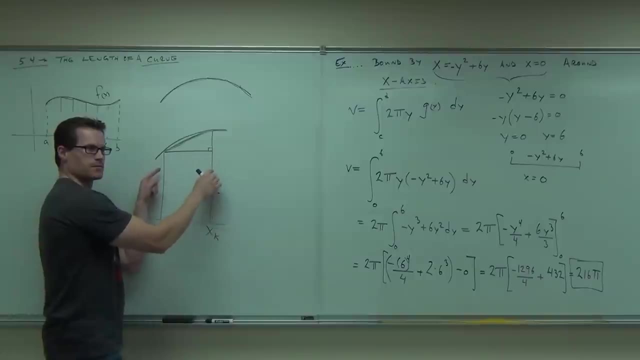 Why don't we make a 90 degree triangle? Let's talk about this for a bit, just for a second. What's this distance? You're overthinking it. What's the distance every time we go from one cut to another? L times. 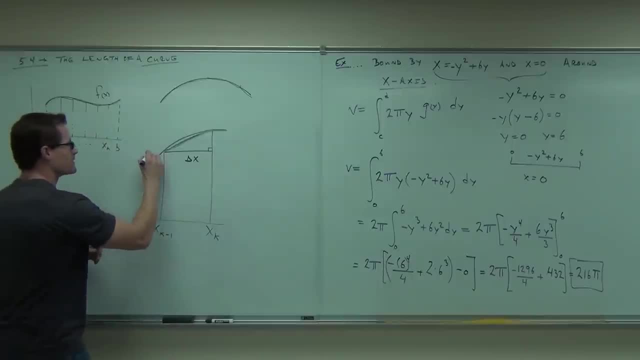 Yes, How high is this from here to here? F of X. No, No, not F of X. You're close, though You have the idea. F of X. F of K, Yeah, Not sub K, K minus 1.. 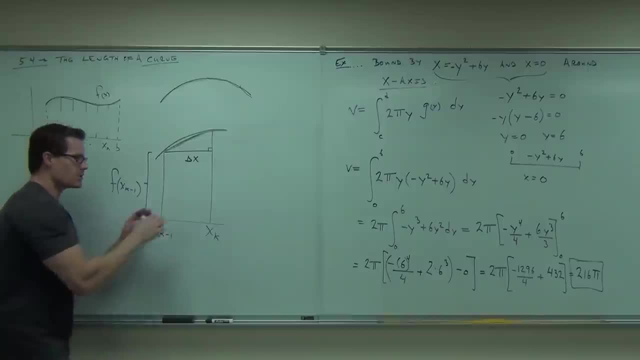 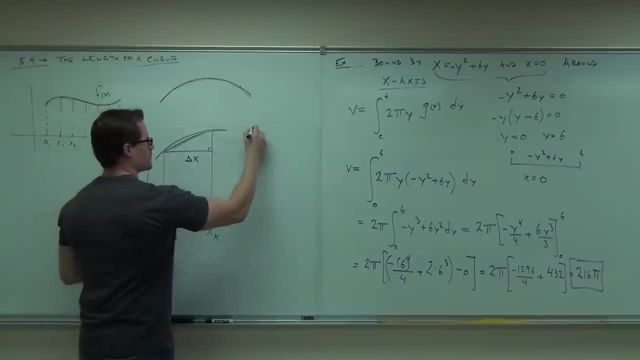 Oh Yes, Do you notice that? that's the height at that exact point? That's the function. That's going to be the height of that function there too. Now, Okay, Okay, Okay, Okay, Okay, Okay. So what's the height here? 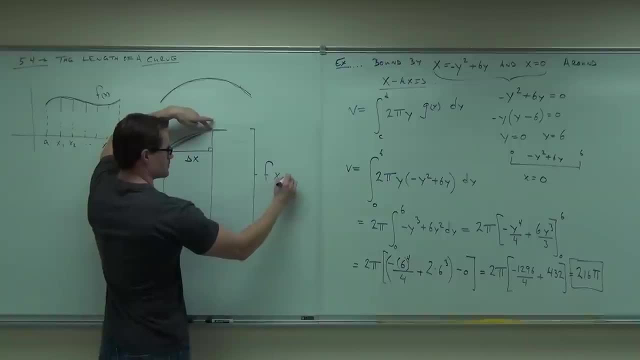 F of X sub K minus F of X K. That's the whole height. I'm talking about the whole height. Okay, We're going to get here in just a second. So this is F of X sub K and this is F of X sub K minus 1.. 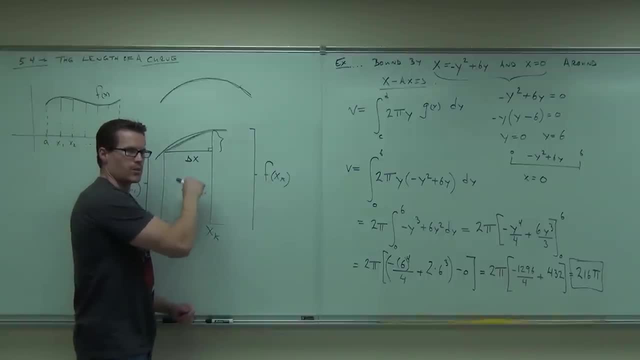 We already have the width of a triangle. We need to find the height of the triangle. That lets us use Pythagorean theorem to find the length of the hypotenuse. You follow me on this, So we're using Pythagorean Theorem. 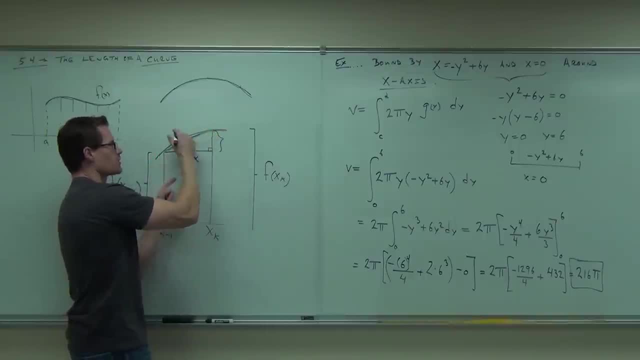 This squared plus this squared equals this squared. That's gonna be great. We'll call this L sub K for the length. What would this be? What's that distance? F of X sub K minus F of X sub K minus one? Yep. 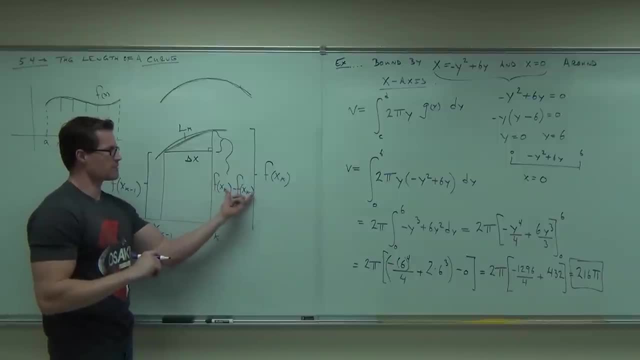 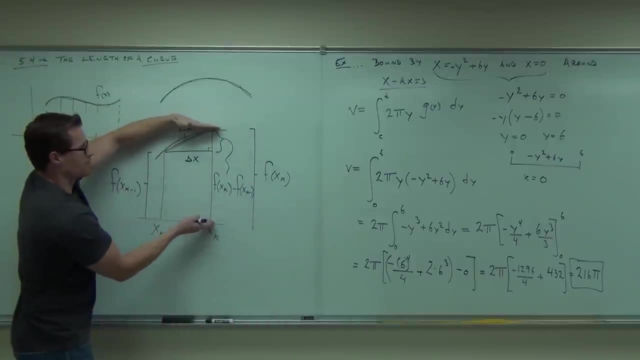 F of X sub K minus F of X sub K minus sure, If this is 10 and this is seven, that's three. You just take and subtract them. The big height, that's this height right there, Minus the little height, since that's a. 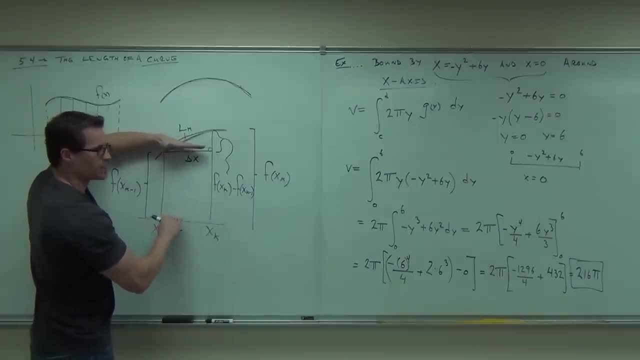 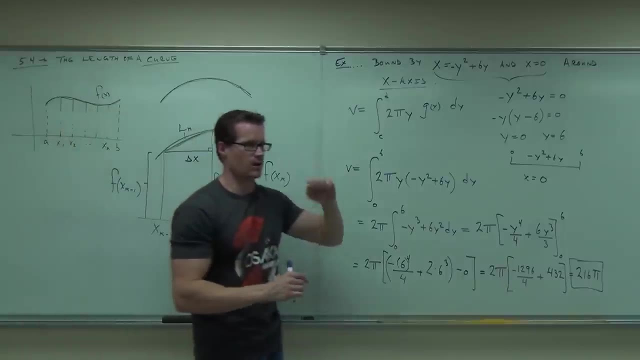 90 degree angle. 90 degree angle, that's gotta be the exact same parallel line. You know that this height, away from this height, gives you that distance, and that's what we're talking about. We just have to be okay with this so far. 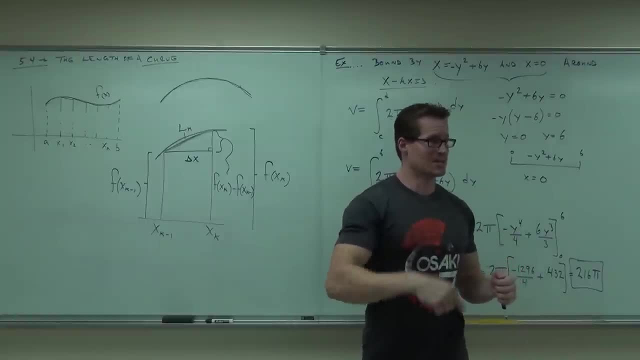 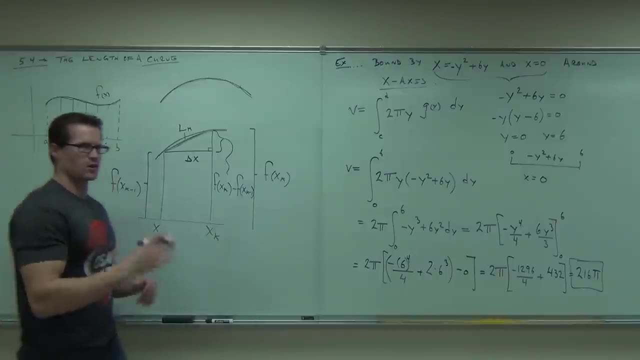 If you handle that, we're almost done. Well, not really Well. we have the idea. We have the idea. Now let's talk about Pythagorean Theorem and what it does. Pythagorean Theorem says: a leg squared. 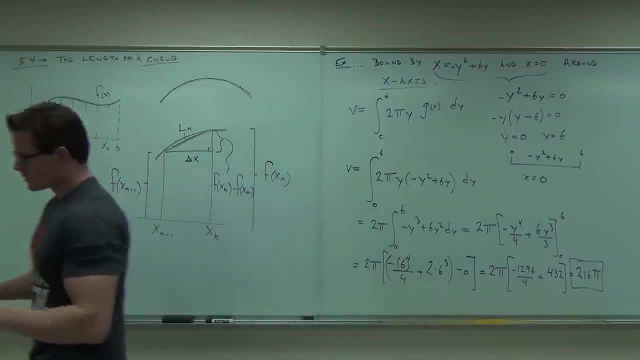 plus a leg squared equals a hypotenuse squared, and we have some symbols for all that stuff right now. Hypotenuse equals- let's see how I wanna do it: A leg squared plus a leg squared, Just like that. Okay, real quickly. 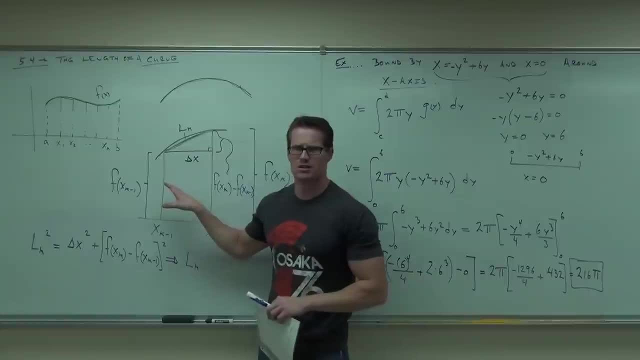 Are you guys? okay? Are you getting this from here? Are you sure? Do you see where it's coming from? Do you see how L sub k is our hypotenuse? Let's see. Is that a delta at the end of it or a narrow? 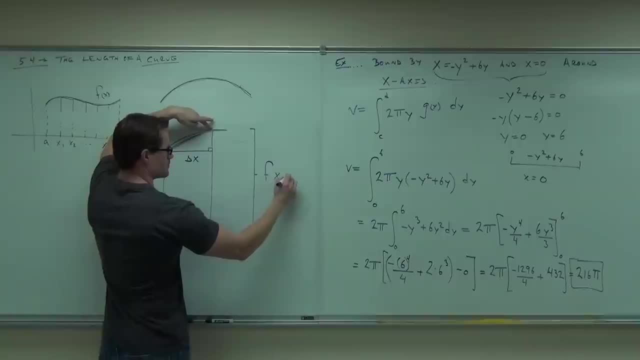 F of X sub K minus F of X- K minus 1.. I'm talking about the whole height. We're going to get here in just a second. So this is F of X sub K and this is F of X sub K minus 1.. 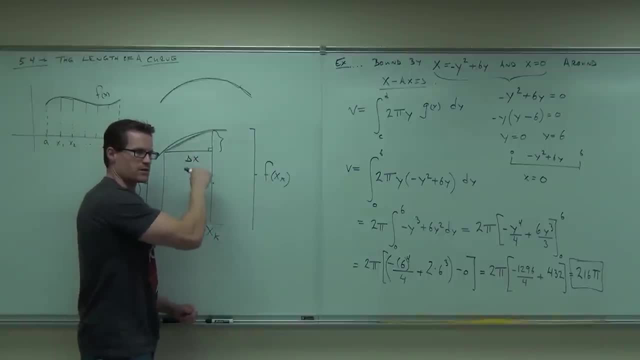 We already have the width of a triangle. We need to find the height of the triangle. That lets us use Pythagorean theorem and find the length of the hypotenuse. Do you follow me on this? So we're using Pythagorean Theorem. 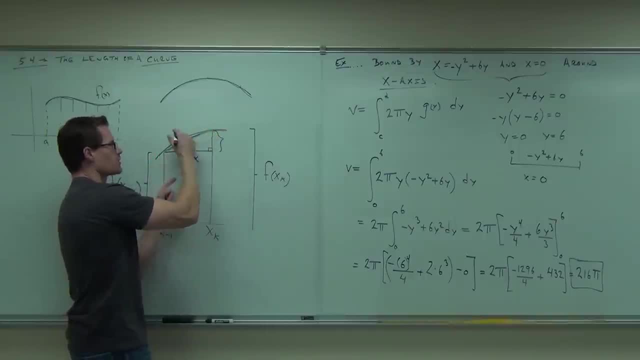 This squared plus this squared equals this squared. That's gonna be great. We'll call this L sub K for the length. What would this be? What's that distance? F of X sub K minus F of X sub K minus one? Yep. 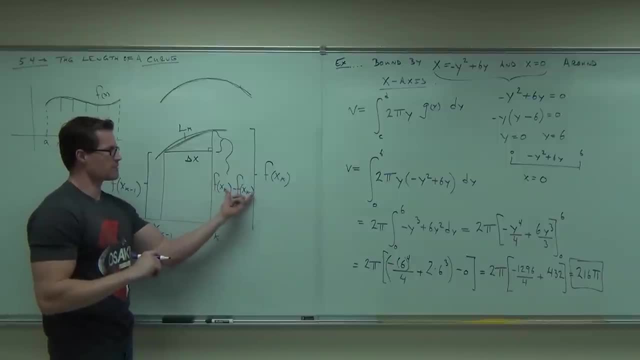 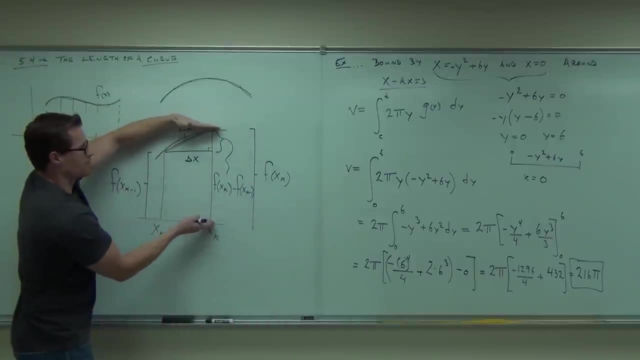 F of X sub K minus F of X sub K minus sure, If this is 10 and this is seven, that's three. You just take and subtract them. The big height, that's this height right there, Minus the little height, since that's a. 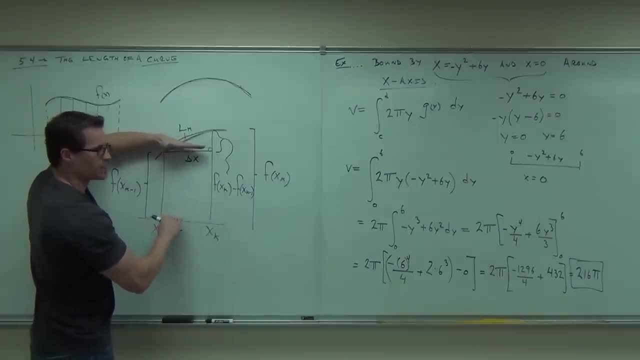 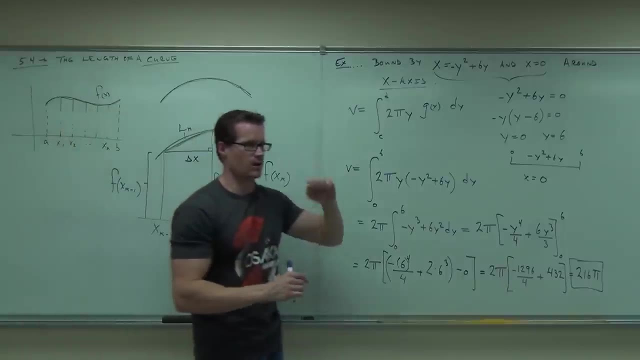 90 degree angle. 90 degree angle, that's gotta be the exact same parallel line. You know that this height, away from this height, gives you that distance, and that's what we're talking about. We just have to be okay with this so far. 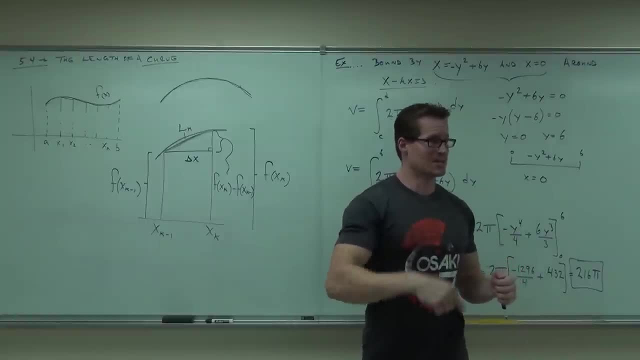 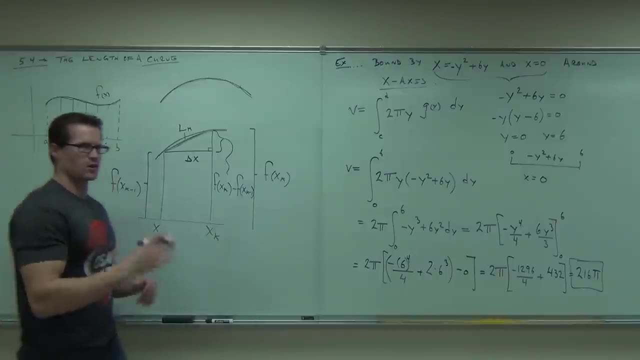 If you handle that, we're almost done. Well, not really, But we have the idea. We have the idea. Now let's talk about Pythagorean Theorem and what it does. Pythagorean Theorem says: a leg squared. 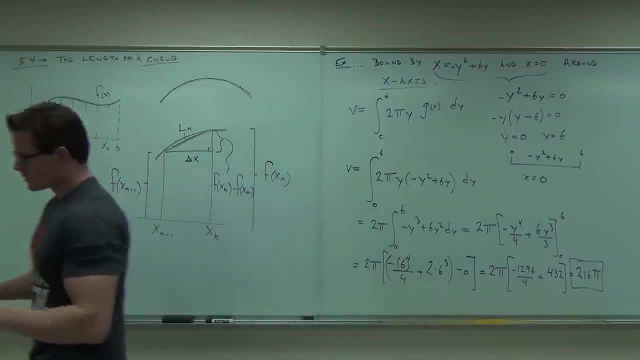 plus a leg squared equals a hypotenuse squared, and we have some symbols for all that stuff right now. Hypotenuse equals- let's see how I wanna do it: A leg squared plus a leg squared, Just like that. Okay, real quickly. 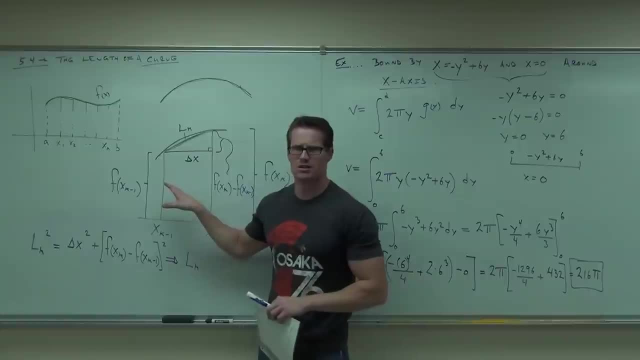 Are you guys okay getting this from here? are you sure? Do you see where it's coming from? Do you see how L sub k is our hypotenuse? Let's see, Is that a delta at the end of it or a narrow? 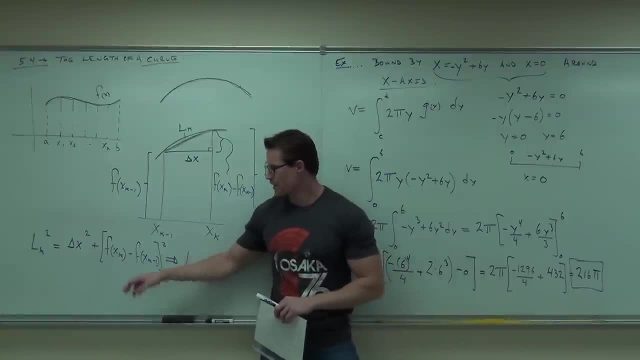 Okay, we're fine, Just a narrow. We're about to go further. Do you see how L sub k is our hypotenuse? Yes, no, Delta x is one of our legs. This is another one of our legs: F of x sub k minus. f of x sub k minus one. 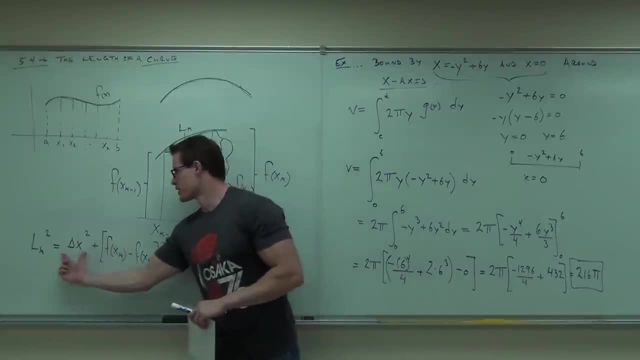 That's a leg, it's a distance. So this square plus this square equals hypotenuse squared. Quick head nod you. okay with it. Okay, cool. How do you get the square away from L sub k? Go to the square root of the first square root. 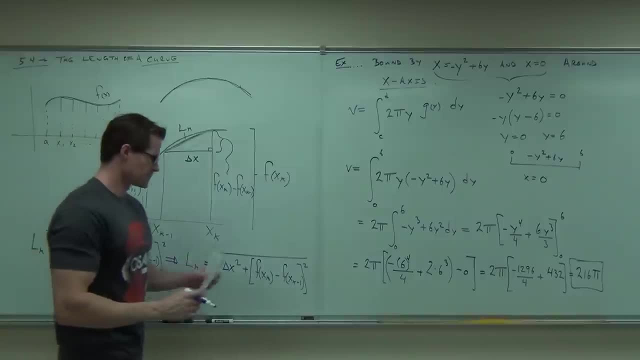 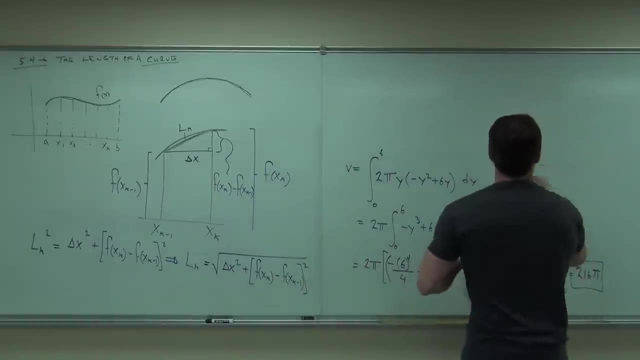 Are you so far, so good? do you guys have any questions on this? before I continue? Seriously, are there any questions on it before I continue? None of this. this is old stuff. You had your chance on that one. Now for the fun part. 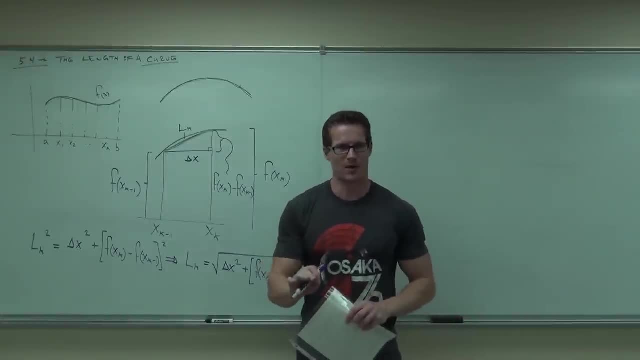 You ready for the fun part? You've got to follow me on this. This is bringing us some. this is like a recurrent development. This is a recurrent development. This is a recurrent development. Do you want to do something like this? That's also a number. oh, we're for the. we're regurgitating some stuff in there. 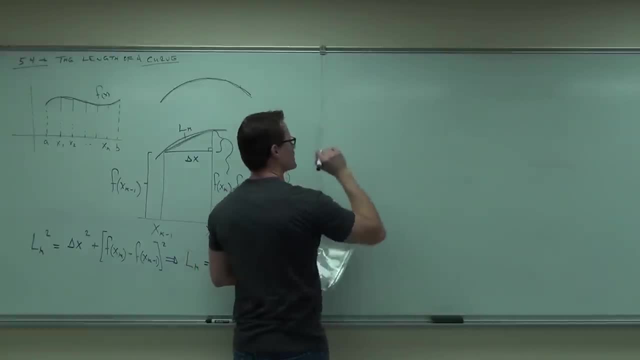 You're going to be like: oh no, throw it back, Just don't. don't bring that up, But just wait Now. do you recall what the mean value theorem says? Not a bit. That was like four weeks ago. 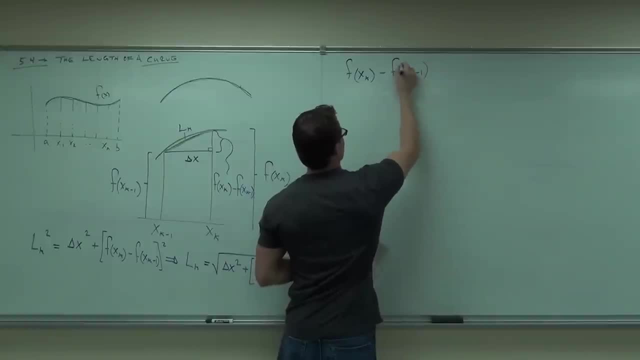 Oh, that was longer than that. That was like 10 weeks ago. Here's what the mean value theorem says. I think I have it. theorem says basically in layman's terms, we're layman. it says: if I take the slope between two points, ie the slope between two points, then on this segment, the 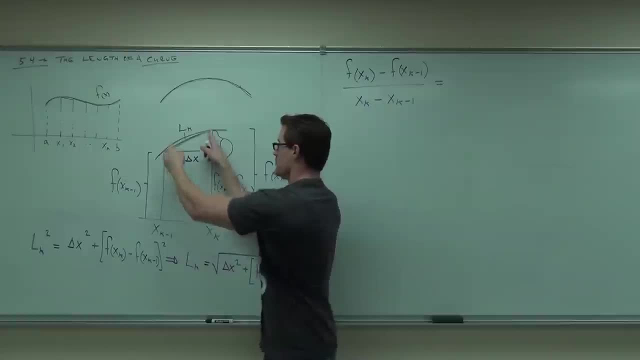 first derivative must equal that slug slope at some point between these two. follow me again. the slope of this line is something true. at some point between here and here, the slope of my function will equal the slope of that line, agree, and where that takes place will be between these two points, somewhere on. 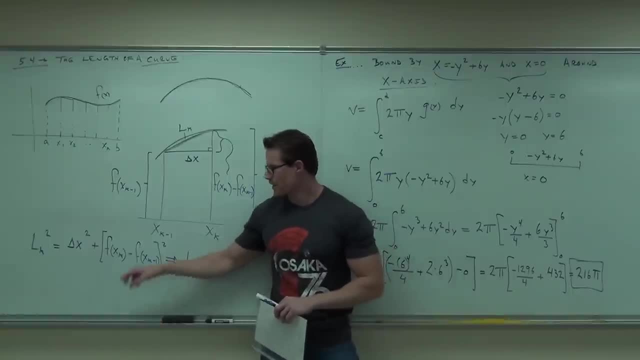 Okay, we're fine, Just a narrow. We're about to go further. Do you see how L sub k is our hypotenuse? Yes, no, Delta x is one of our legs. This is another one of our legs: F of x sub k minus. f of x sub k minus one. 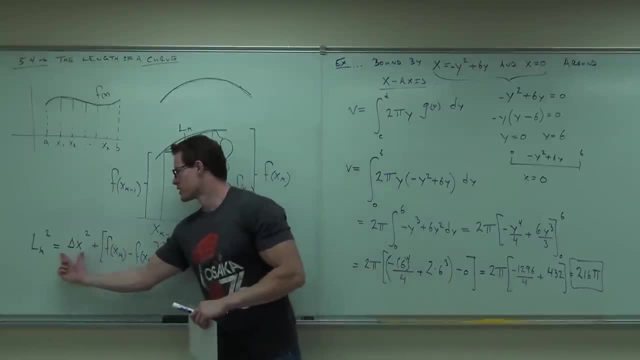 That's a leg, it's a distance. So this squared plus this squared equals hypotenuse squared. Quick head, nod you, okay with it. Okay, cool, How do you get the square away from L sub k? Go to the square root of the first square root. 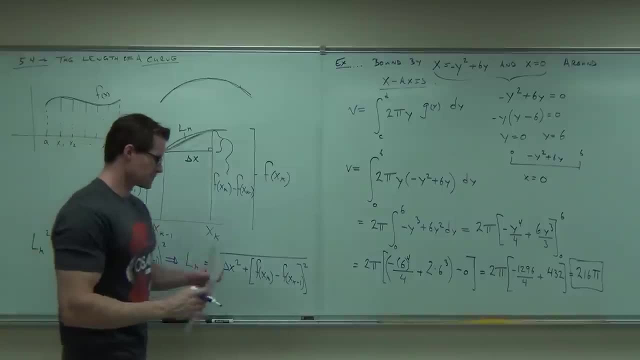 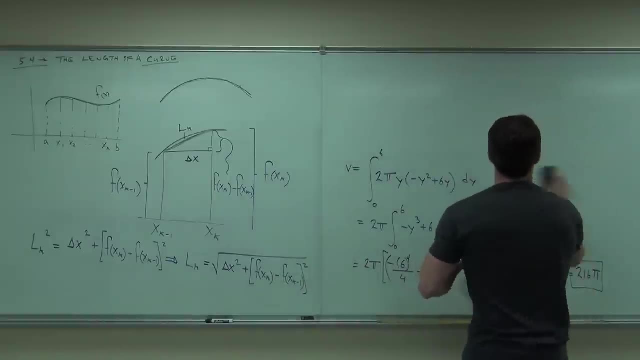 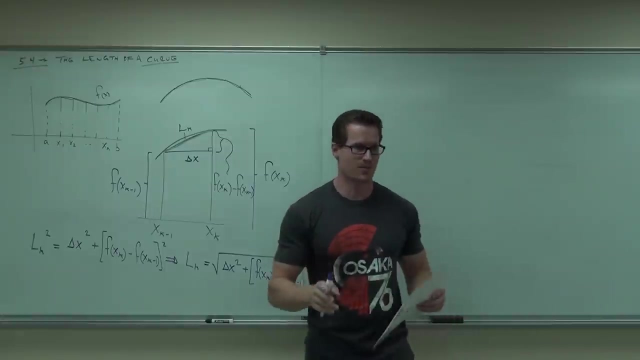 You get the square root of the first square root. You get the square root of the first square root. Okay, cool, Now let's do this. Are you so far, so good? You guys have any questions on this? before I continue, 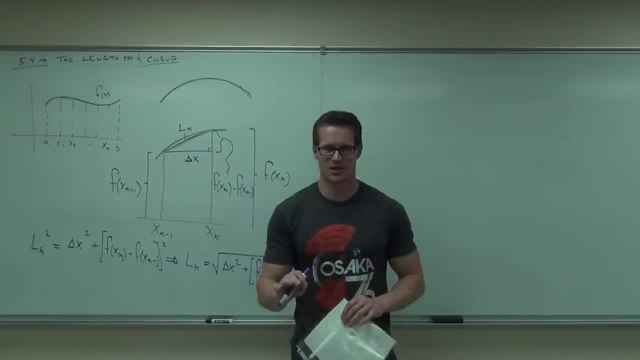 Seriously. are there any questions on it? before I continue? None of this. this is old stuff. You had your chance on that one. Now for the fun part. You ready for the fun part? All right, One minute, one minute. 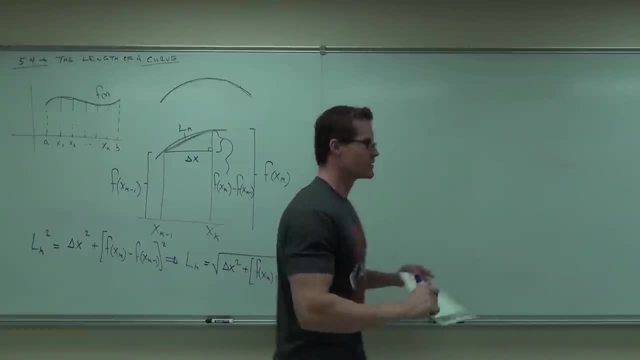 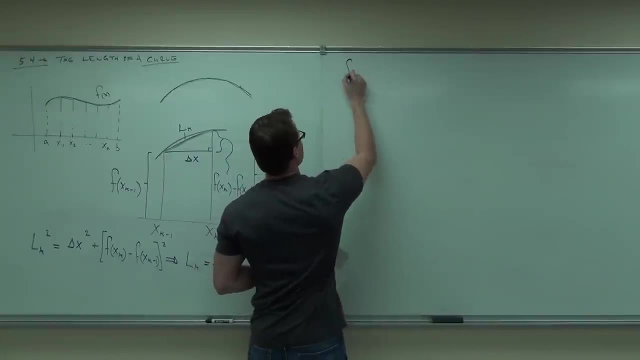 Okay, go ahead and say it one more time. You're going to be like: oh no, throw it back, Don't bring that up, But just wait Now. do you recall what the mean value theorem says? None of it. 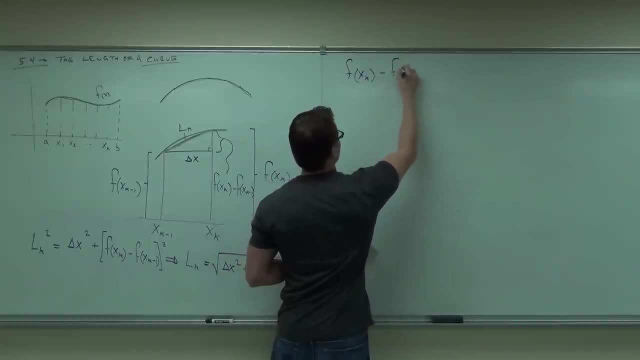 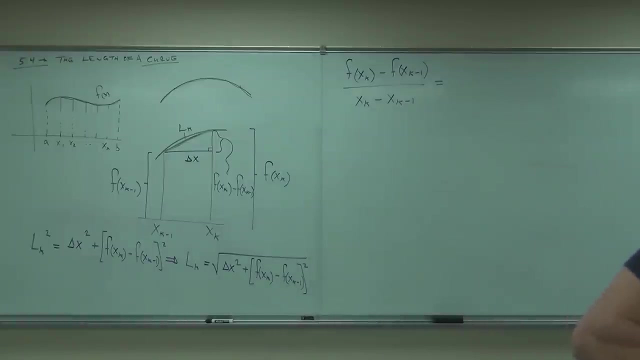 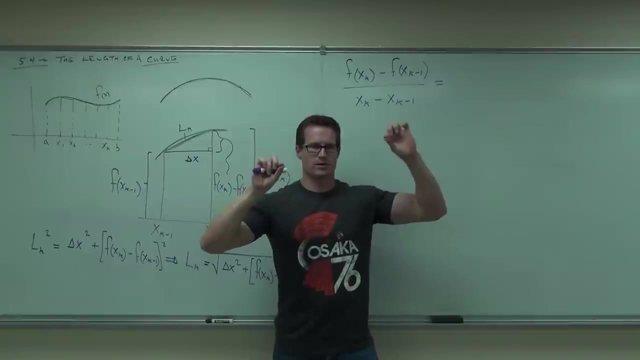 I remember a few days ago, That was like four weeks ago. Oh, that was longer than that, That was like ten weeks ago. Here's what the mean value theorem says. It's really cool, Basically, in layman's terms- we're laymen- it says: if I take the slope between two points, ie the slope between two points, then on this segment the first derivative must equal that slope at some point between these two. 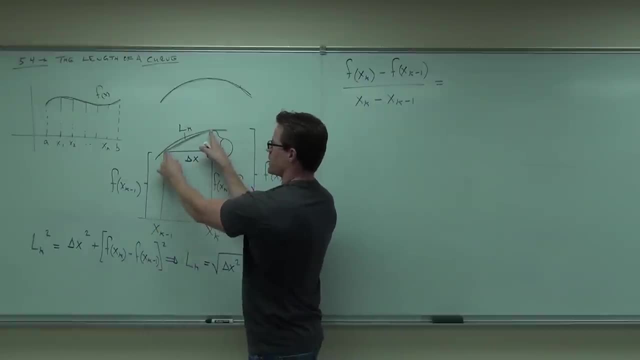 Follow me again. The slope of this line is something true. True. At some point between here and here, the slope of my function will equal the slope of that line, Agreed, And where that takes place will be between these two points, somewhere on that interval. 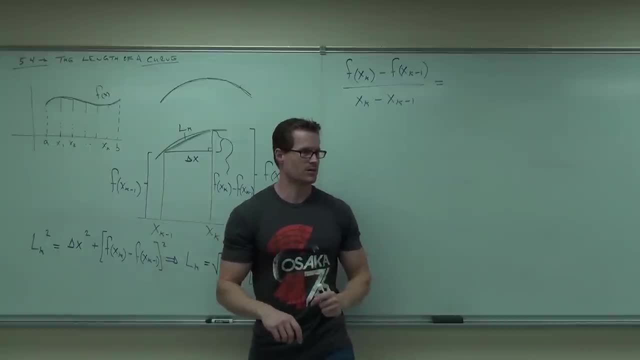 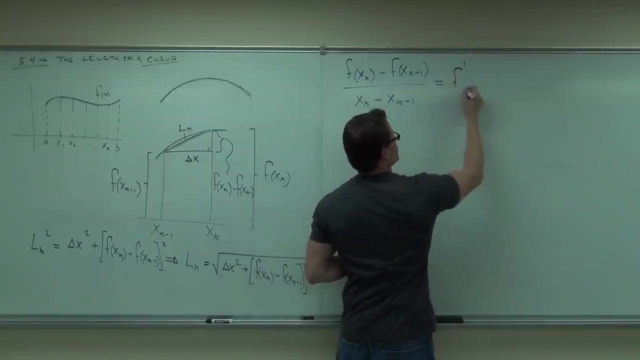 the interval. do you understand that? yeah, everybody. here's what it says, in that it says this will equal what's the slope of a function in terms of calculus, the what first derivative? first derivative at some point, oh, look, at some point between here and here. we don't know what. 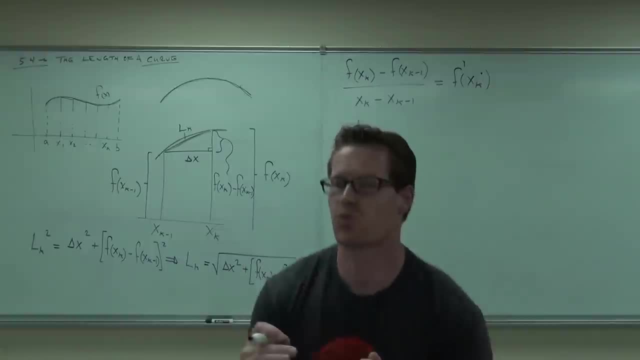 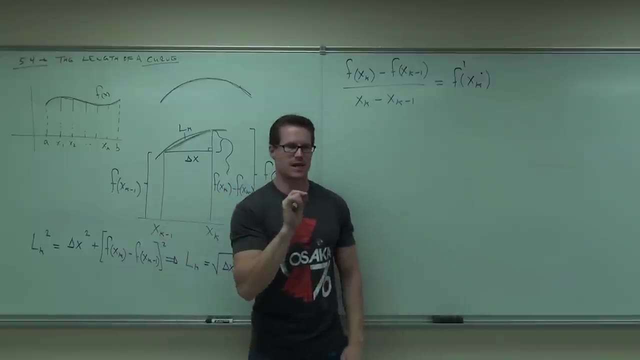 it is arbitrary point at some point between there and there. does it matter where it happens? I don't care why. why don't I care? what's gonna happen to these two numbers? BAM, smash them together, that X, K, dot the sub, the sum point where the slope of my function equals the slope of my secant line, where 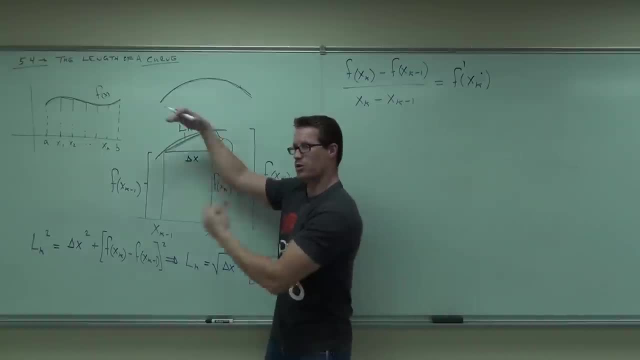 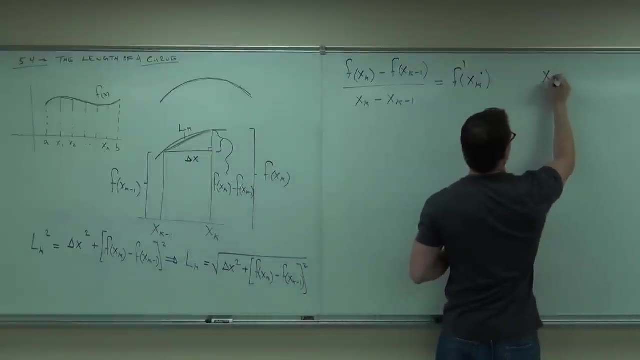 that happens by the mean value theorem. it has to happen for a continuous function and we're assuming the this is a continuous function. that has to happen. we call X, K dot. it's going to be somewhere on this interval. this is all by the mean value theorem. by the way, 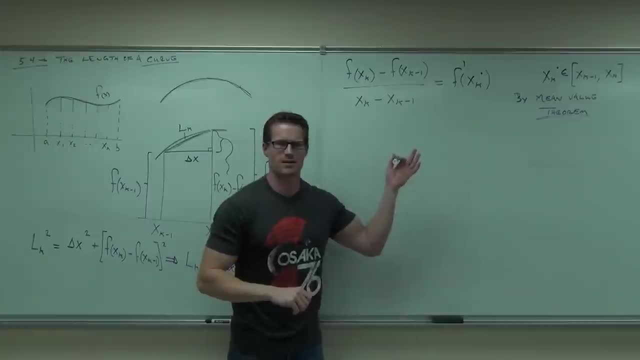 by the mean value theorem. by the way, did you believe me see what this stuff actually is? I hope you see what it is. this is the change in height. we will. we have this on the board. actually, this is the change in height over the change in width that by 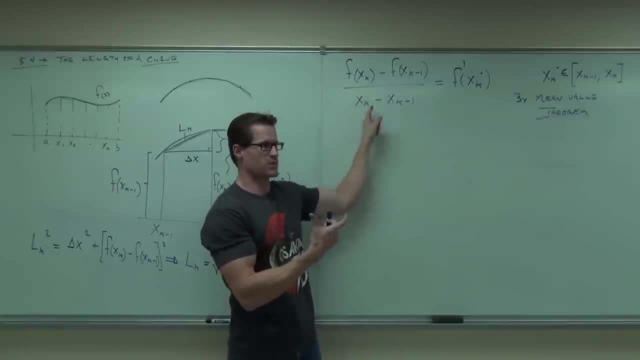 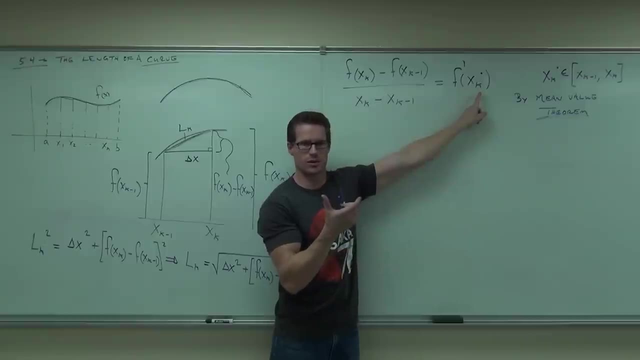 definition is a slope. you see it, the slope between two points must equal the slope of the function at some point, that's between those two points. that's what the mean value theorem says. believe it or not, that's true. you got it. now we're gonna do some fancy dancy math. we go wiggle, wiggle, wiggle, wiggle, wiggle. 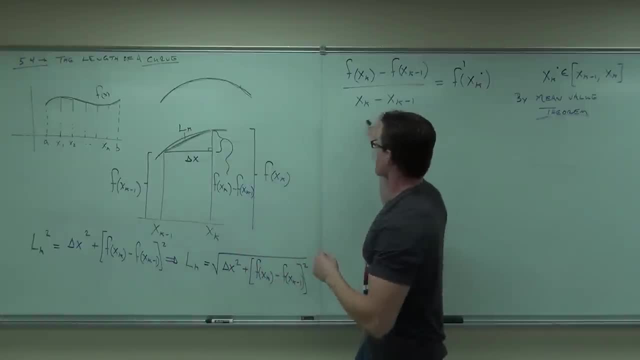 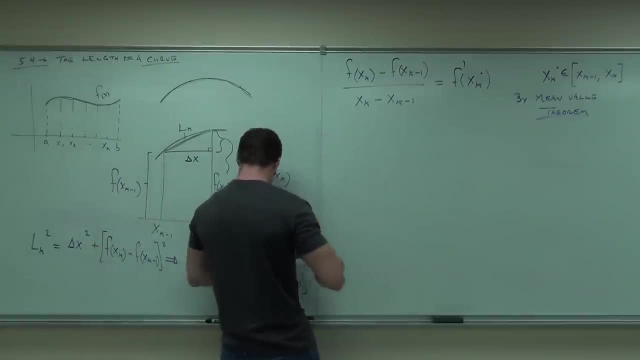 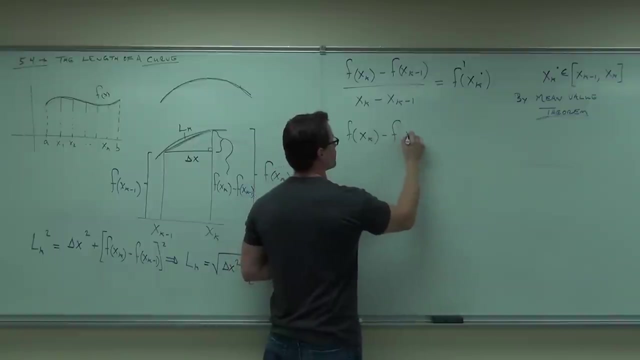 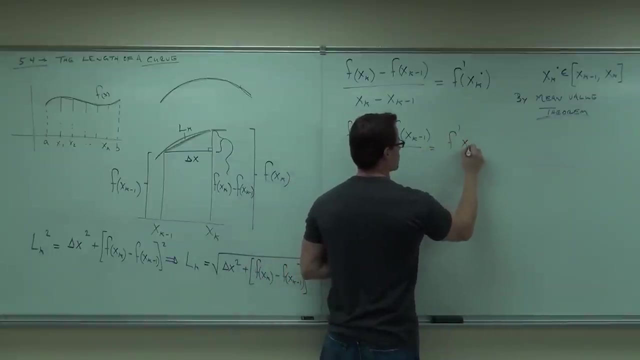 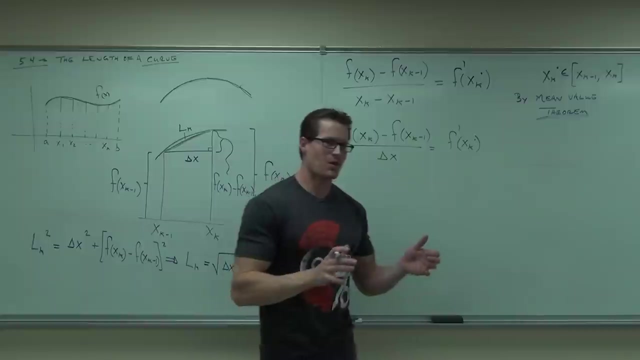 around. do you understand what? X, K, X of K minus X of K minus 1 is very good. so substituting we're gonna have: ah, that's dope X. are we having fun yet? are we having fun? this is not fun. it's awesome. here's my goal. by the way, you don't know the goal. the goal is: this thing sucks I. 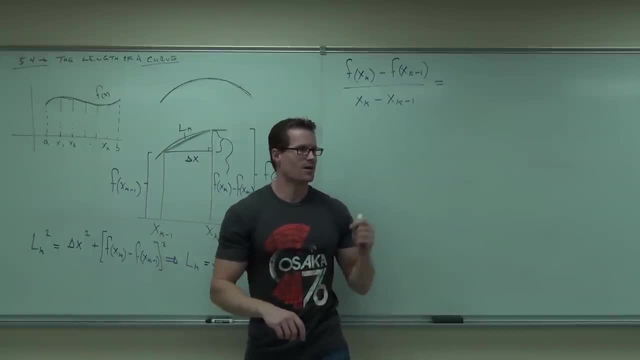 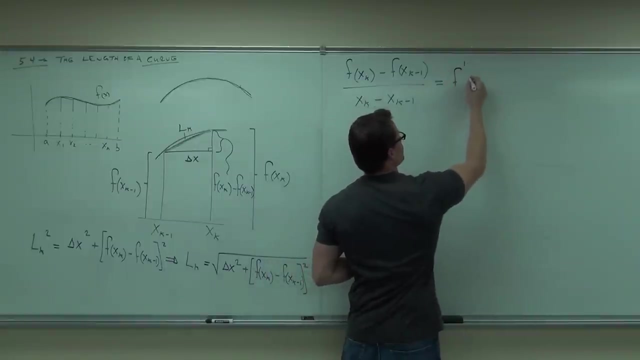 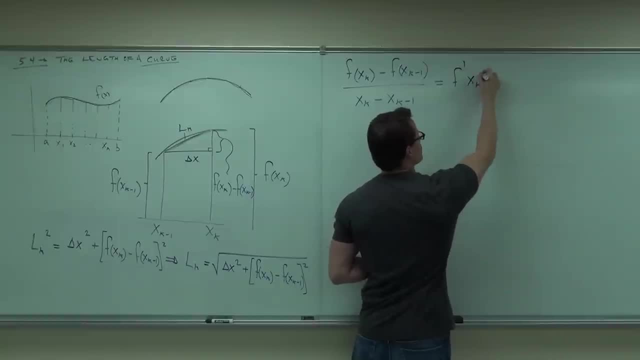 First derivative At some point. oh, oh, look at some point between here and here. we don't know what it is. arbitrary point at some point between there and there. does it matter? where it happens, I don't care. 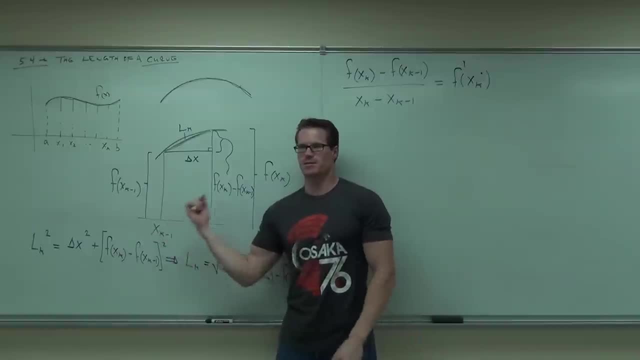 Why? Why don't I care What's going to happen to these two numbers? Bam, smash them together. That xk dot, the sum point where the slope of my function equals the slope of my secant line. where that happens by the mean-related theorem, it has to happen for a continuous 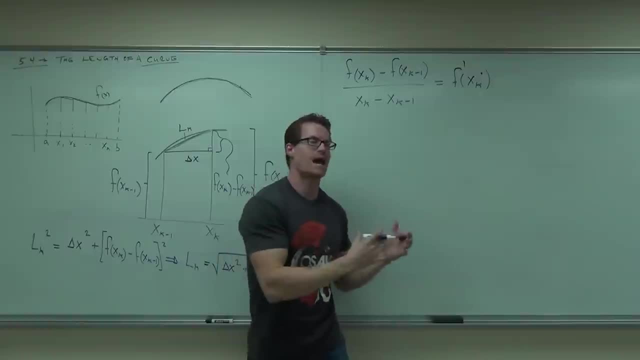 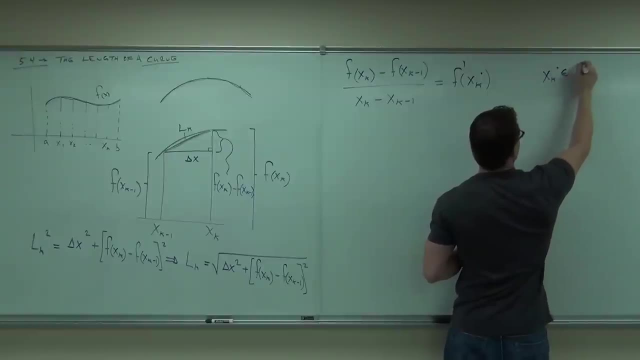 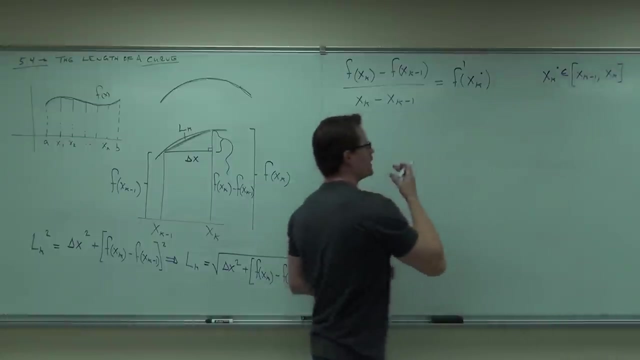 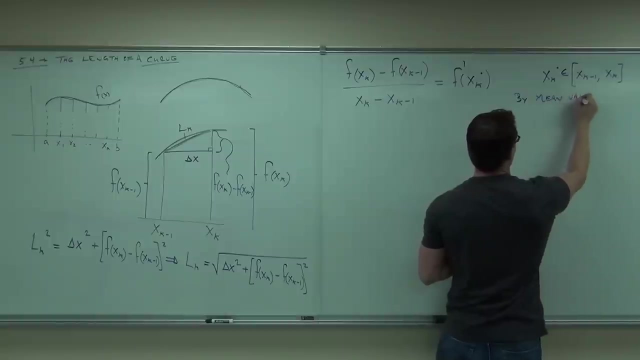 function, and we're assuming this is a continuous function. That has to happen. We call it xk dot. It's going to be somewhere on this interval. This is all by the mean-value theorem, by the way. By the way, did you believe me? 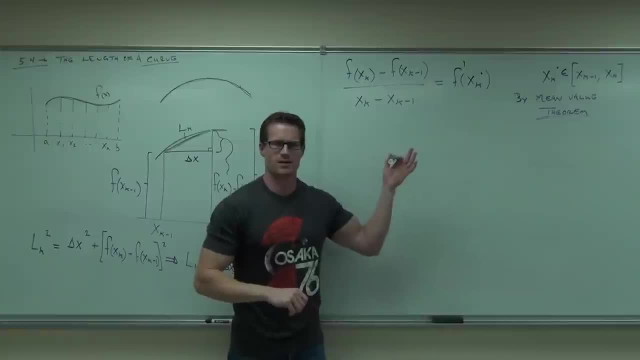 See what this stuff actually is. I hope you see what it is. This is the change in height. We already have this on the board. actually, This is the change in height over the change in width. That, by definition, is the slope. 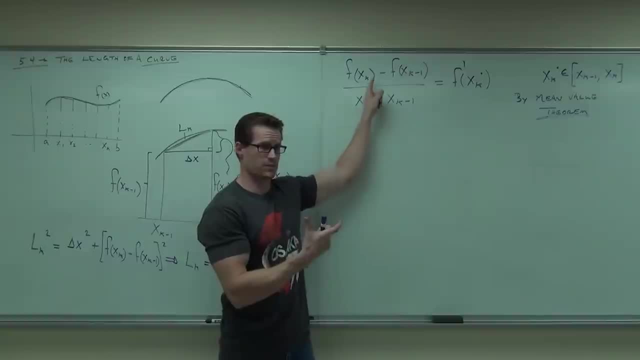 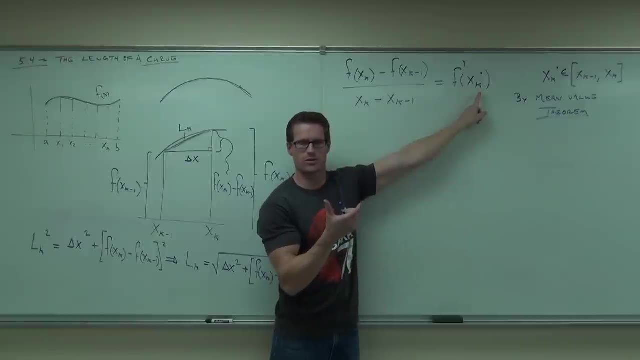 You see it, The slope between two points must equal the slope of the function at some point, that's between those two points. That's what the mean-value theorem says. Believe it or not, that's true. Do you got it? Now we're going to do some fancy-dancy math. 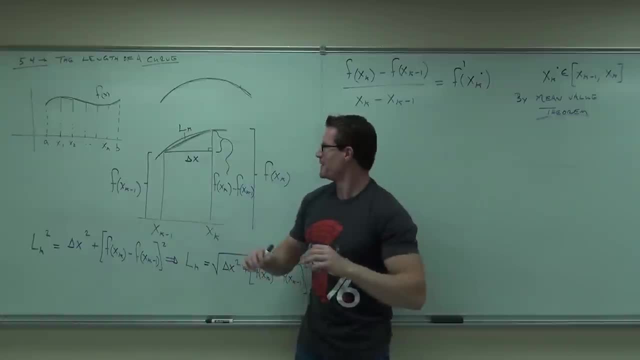 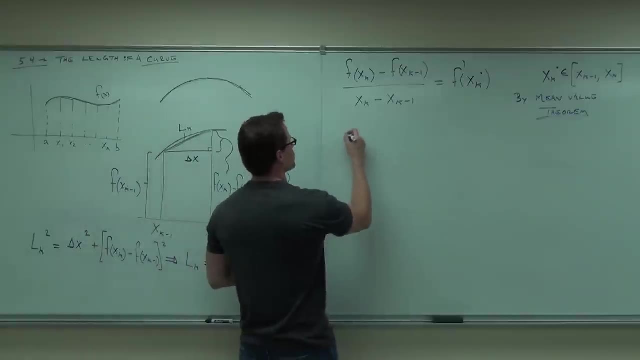 Wiggle, wiggle, wiggle, wiggle, wiggle, wiggle. We're going to wiggle this around. Do you understand what? x sub k minus 1 is Very good Substituting we're going to have. 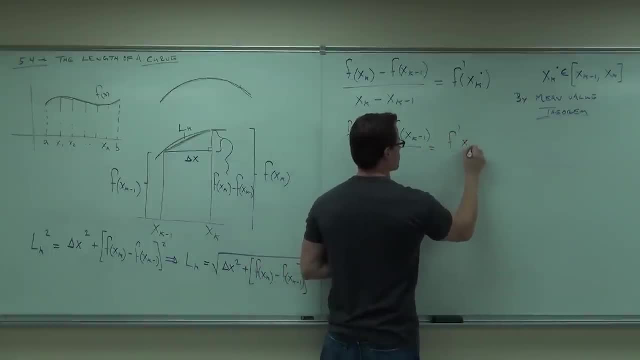 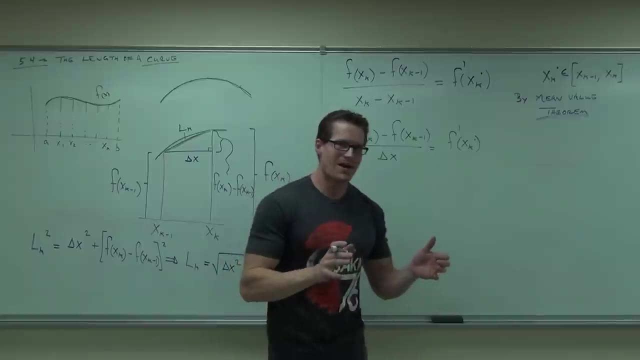 Ah, that's still x. I'm not even fun. yet I'm not even fun. This is not fun, It's awesome. Here's my goal. by the way, You don't know the goal. The goal is this thing sucks. 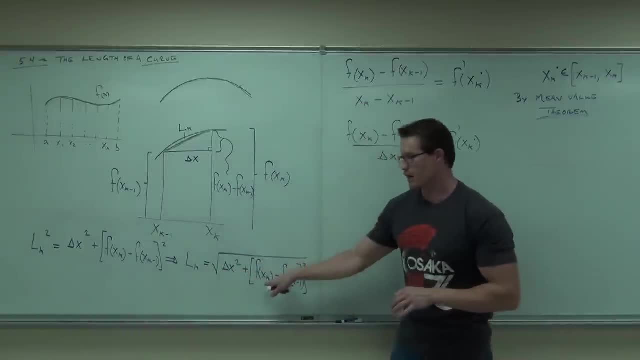 I want to get rid of it. That's the goal. That thing sucks. How do I get rid of it? Let's try to find this Here. Do you see it? Solve for it. If I solve for this piece, I just multiply both sides by delta x. 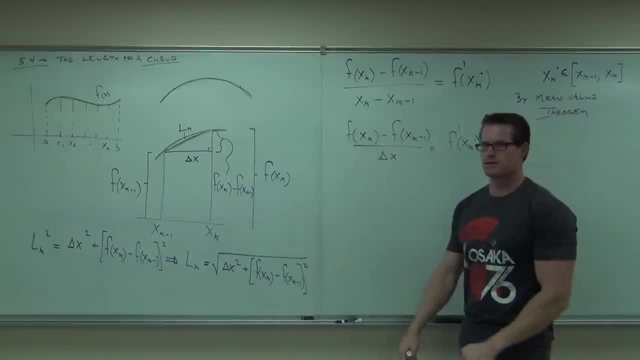 Let's see. I'm going to solve for this. I'm going to solve for this Here. I'm going to solve for this Here. I'm going to solve for this. I'm going to solve for this Here, Here. 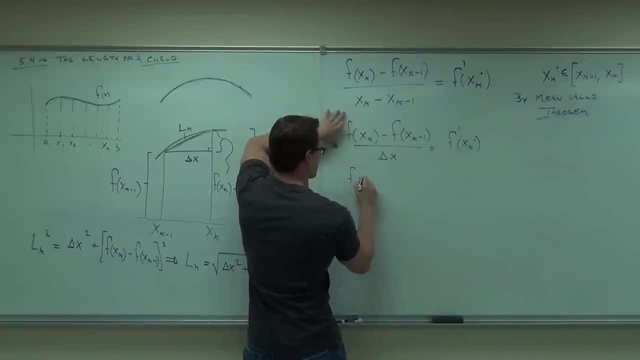 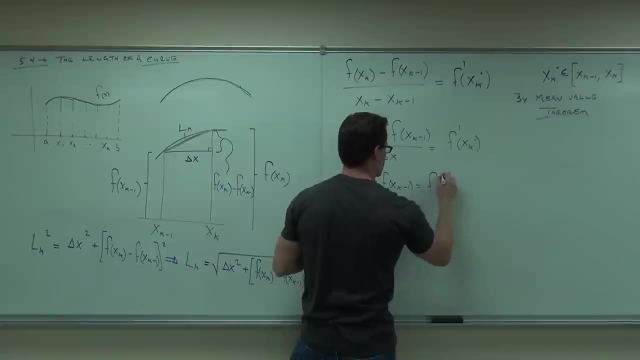 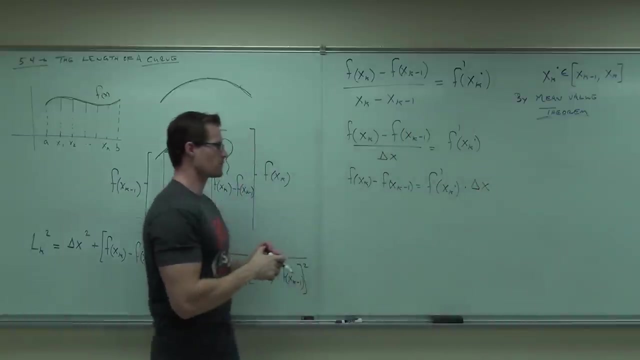 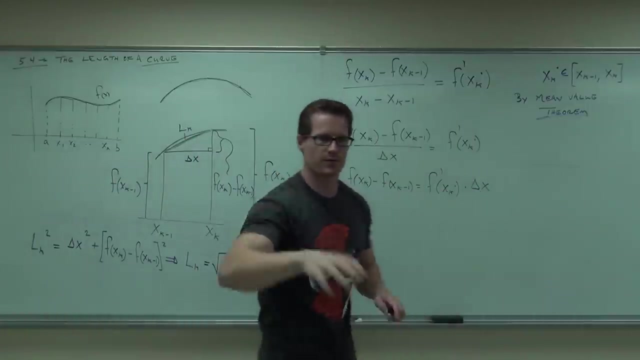 I'm going to solve for this. Okay, we've done a lot of math work. Do you feel okay with it so far? Raise your hand if you do feel okay with it. so far, A lot of theory. right, We haven't done anything actually. 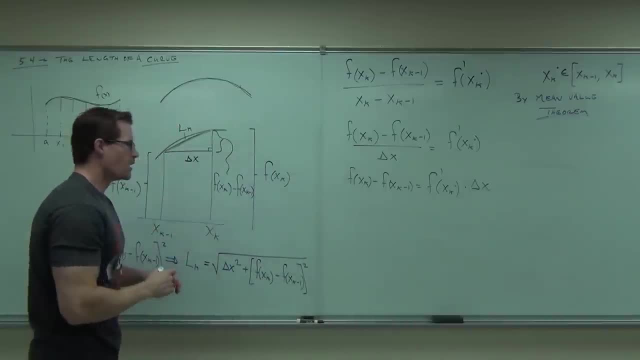 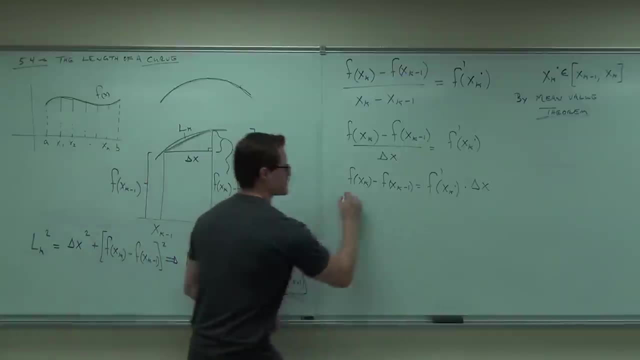 Well, we manipulated algebraically, but we haven't done an example yet. Here's what I'm going to do. I'm going to notice that this piece right here is the same as this piece right here. I'm going to put that thing in instead of it. 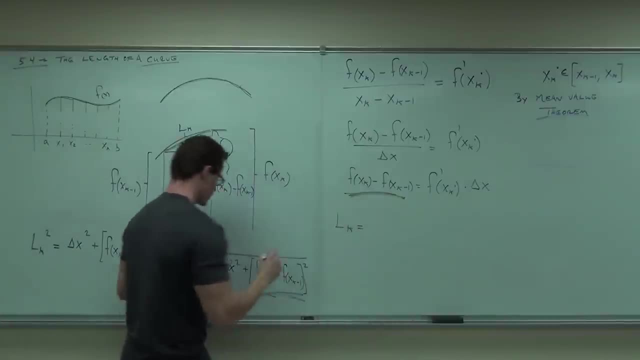 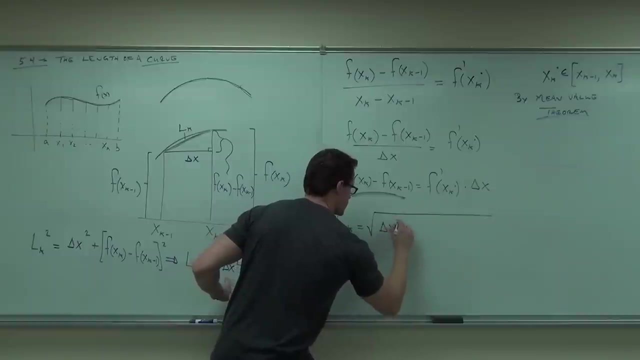 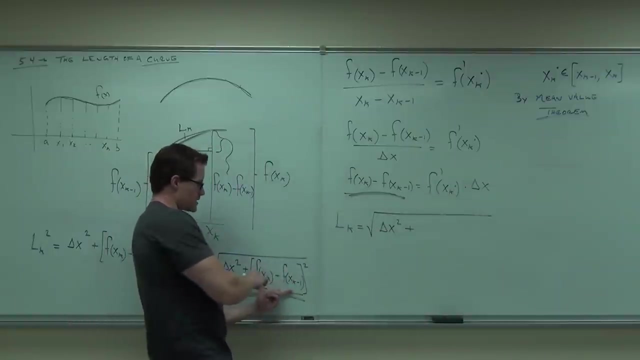 So L sub K equals: we got the square root. Inside the square root we have delta X squared, plus this big fat piece of junk. We're going to replace it with this big fat piece of junk. Instead of this, we have F of X sub K minus F of X sub K. 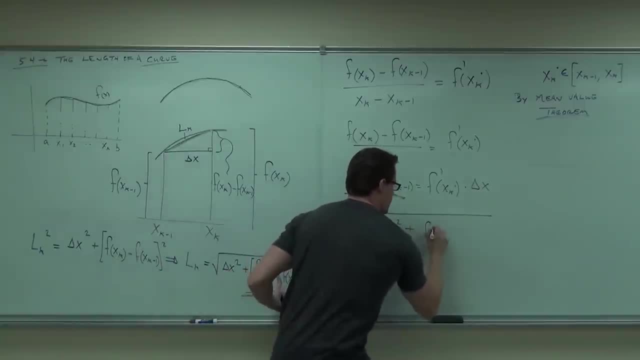 minus F of X sub K, minus F of X sub K, That's one. That's F of F. We're going to have F prime X sub K dot or XK dot times delta X. Don't forget it has to be squared. 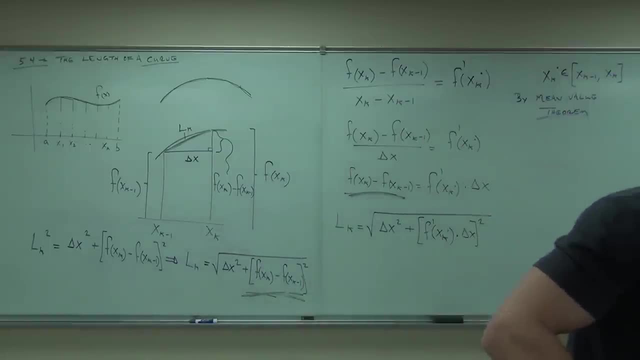 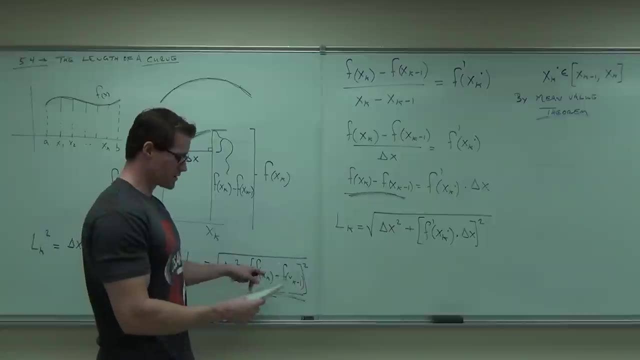 Are you still okay with it? Do you guys have any questions so far on it? Do you see where the sub is coming from? I don't see one sub coming from the other way around. Well, there's not much we can. There's not much we can do with this. 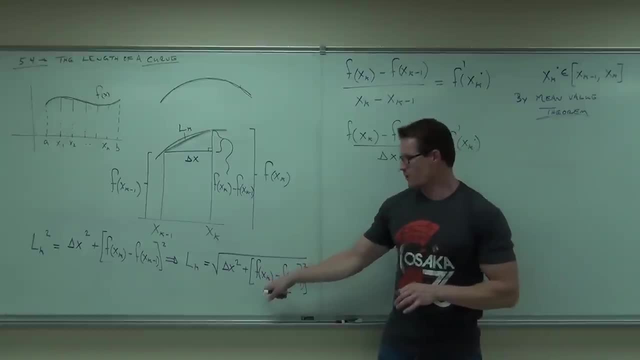 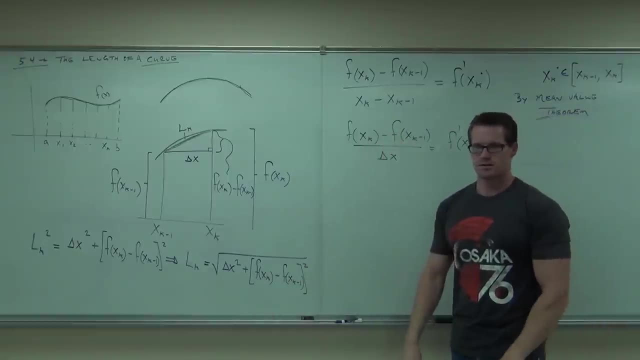 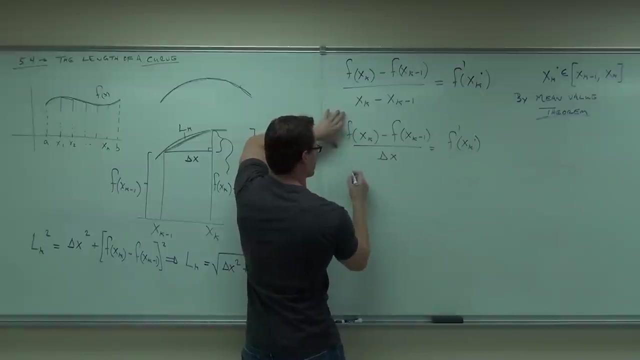 want to get rid of it. that's the goal I think sucks. so how do I get rid of it? let's try to find this here. do you see it? so for it, if I solve for this piece, I just multiply both sides by Delta X you. 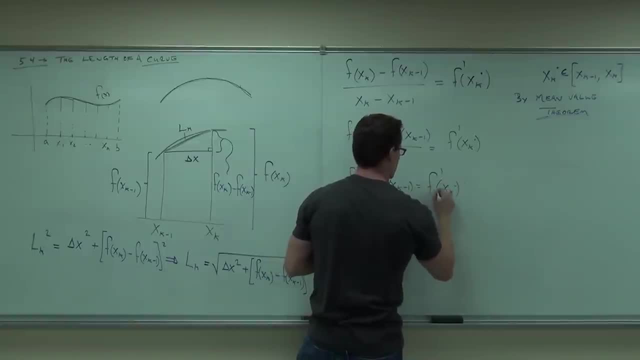 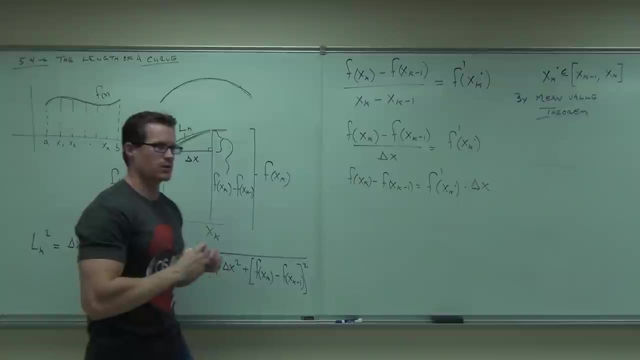 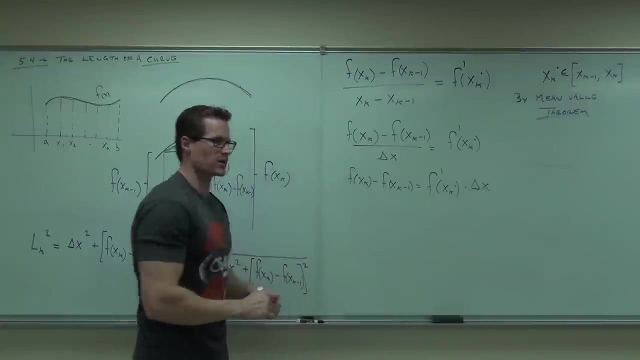 okay, we've done a lot of math work. do you feel okay with it? so far, we're just going to do is be located. so far, a lot of theory, right, we haven't done anything. actually, we manipulated algebraically, but we haven't done an example yet. here's: 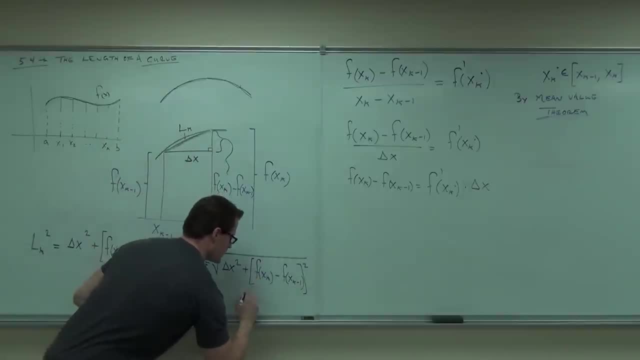 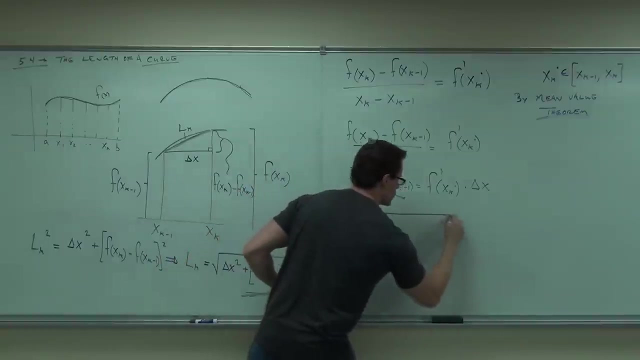 what I'm gonna do. I'm gonna notice that this piece right here is the same as this piece right here. I'm gonna put that here on top of that piece right here. I'm gonna put that thing in and said of it: so L sub K equals. we got this square root inside. 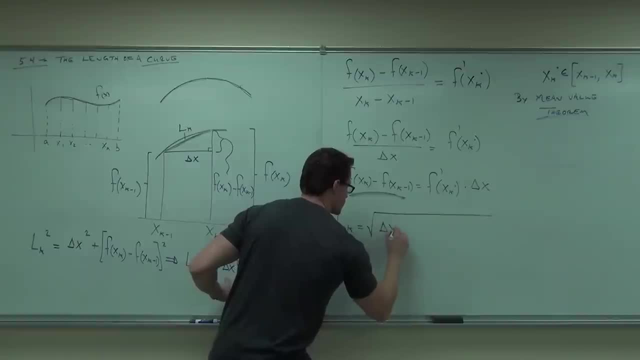 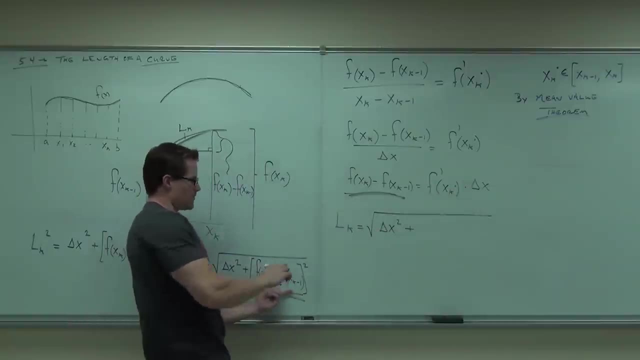 the square root with Delta X square rise. this big fat piece of junk we're going to replace with this big fat piece of junk. instead of this we have f of x sub k minus f of x of k minus x. we're gonna have M prime. 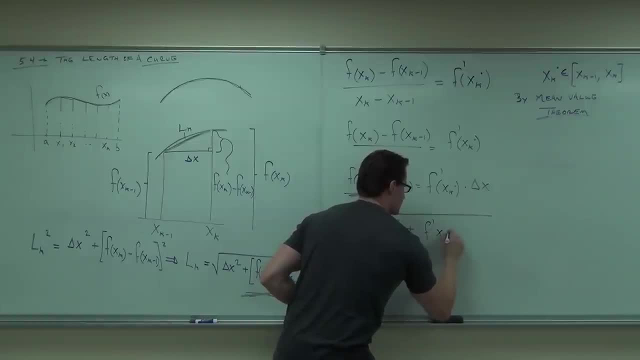 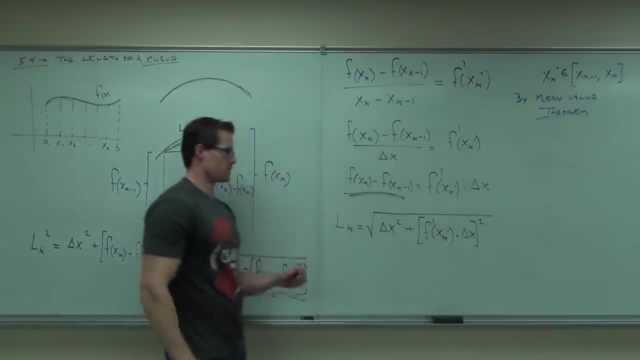 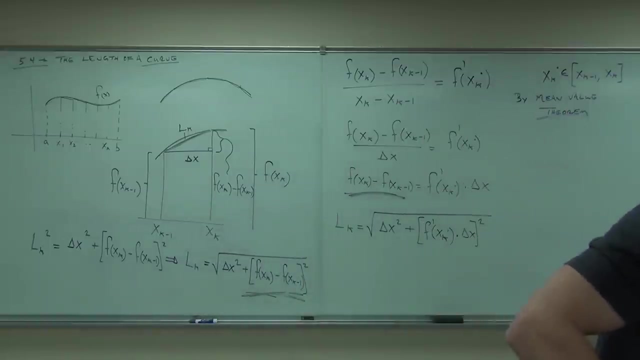 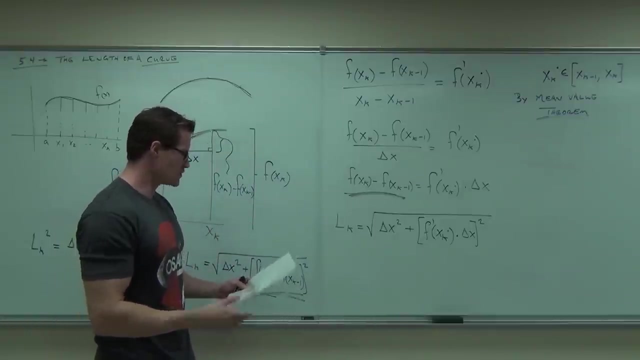 X sub K dot times: delta x. don't forget it has to be squared. Are you still okay with it? Do you guys have any questions so far on it? You see where the sun's coming from. Well, there's not much we can do with this. 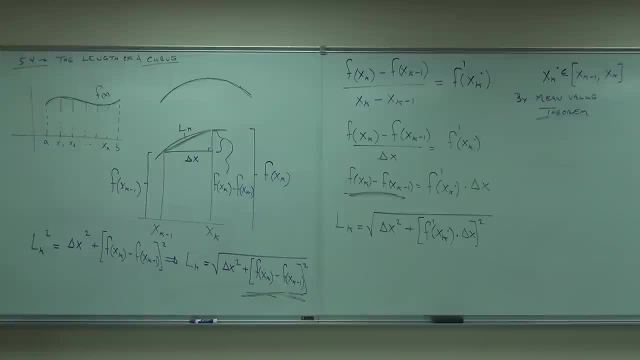 There's something that we can do with that. Do what we're gonna do right now. We're gonna do. oh, let's see, let's do one more thing here. Let's break this up a little bit, Let's just do. 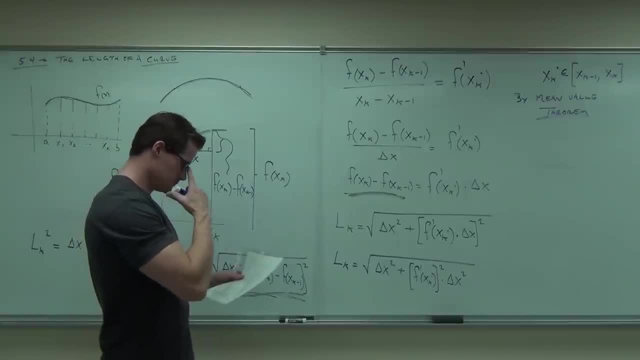 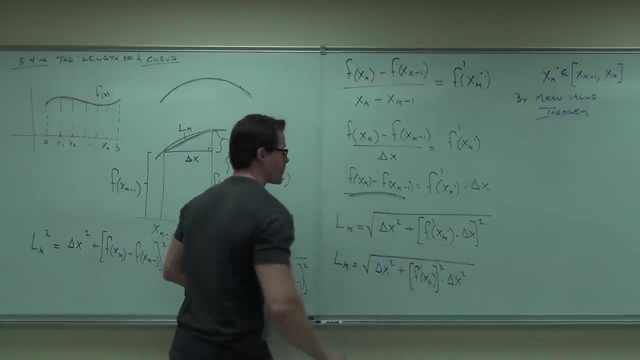 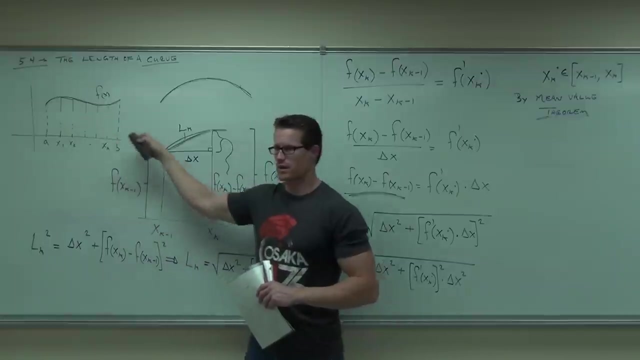 that So far, so good. By the way, did you guys have any questions over here? Because I'm gonna erase and continue. So you understood the idea of cutting it up right, Finding the length of each segment using the Pythagorean Theorem. 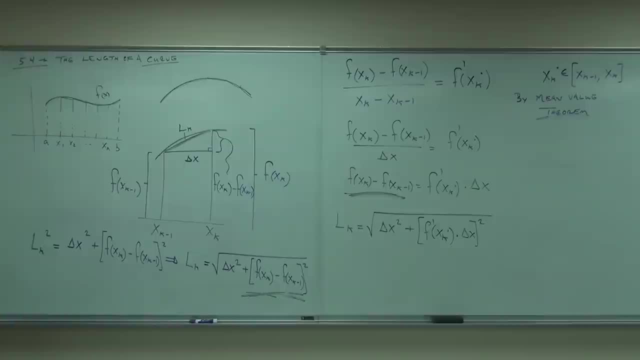 There's something that we can do with that. Here's what we're going to do right now. Oh, let's see, Let's do one more thing here. Let's break this up a little bit, Let's just do, Let's do that. 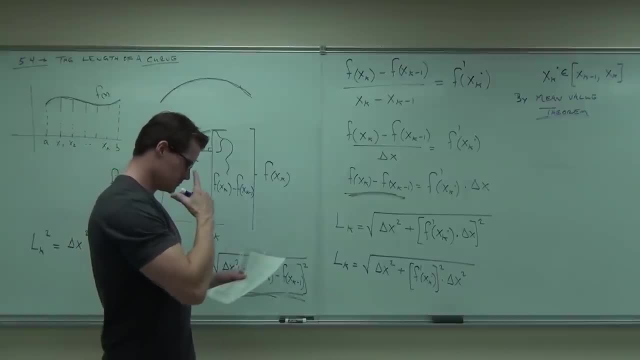 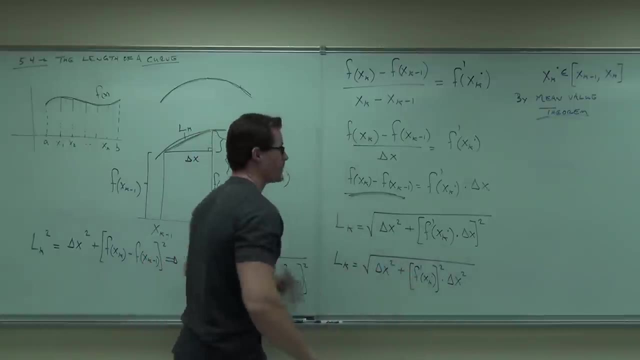 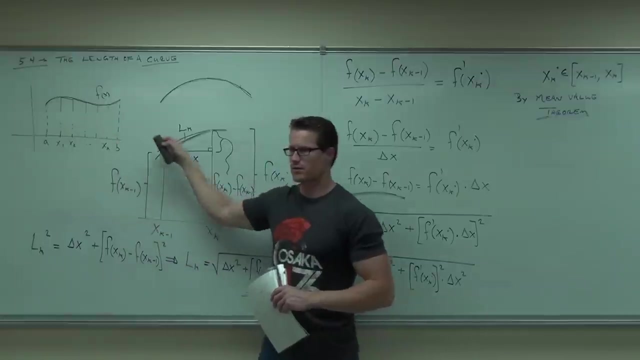 So far, so good. By the way, did you guys have any questions over here? Because I'm going to erase and continue. So you understood the idea of cutting it up right. Finding the length of each segment using my diagram theorem. 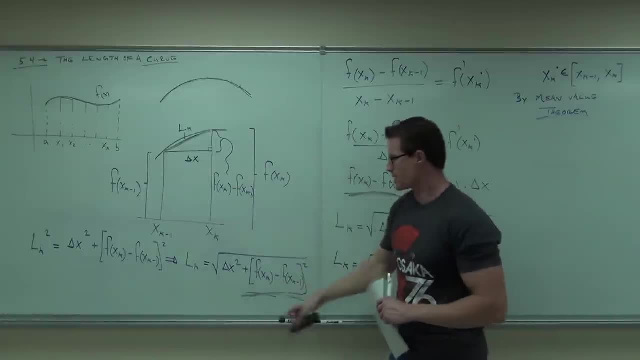 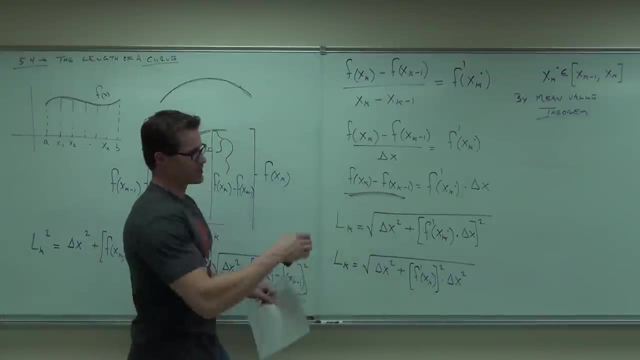 Now we're just working that down, So take note of that. Hopefully you have that. The important part was to get our substitution Done from here to here. That was the idea. I guess I do have some room over here I can work on. 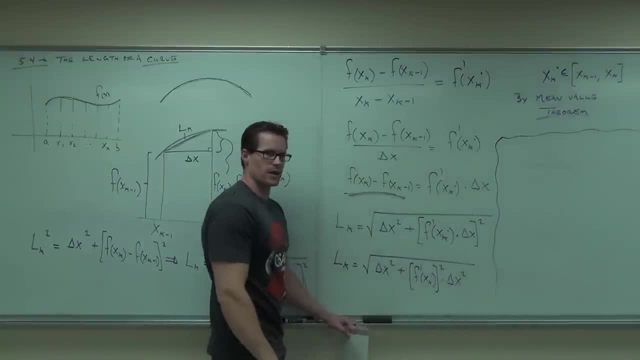 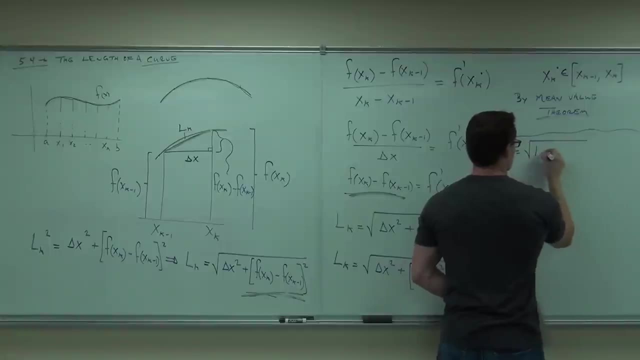 So from here Do you see that we can factor out a delta x squared. So we're going to have one f prime of xk dot squared Times, delta x squared. But that is going to be in a little bracket. I'm going to draw it in black so you can see it a little bit better. 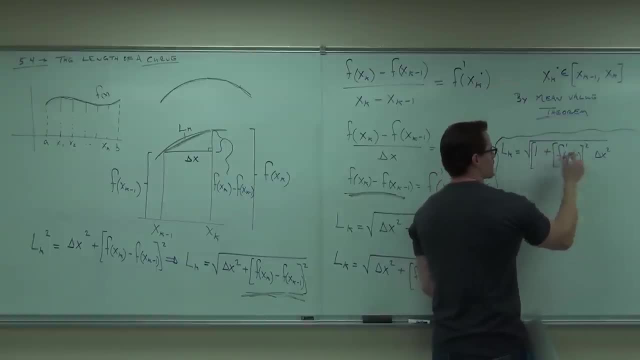 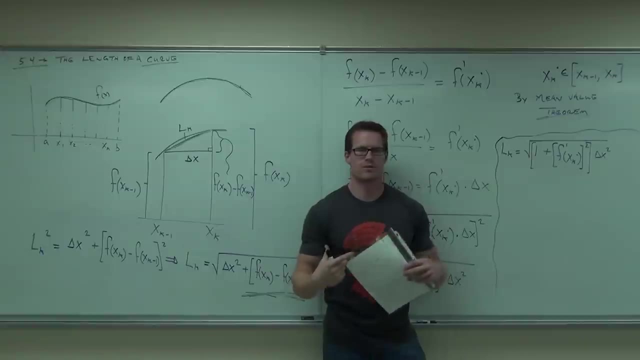 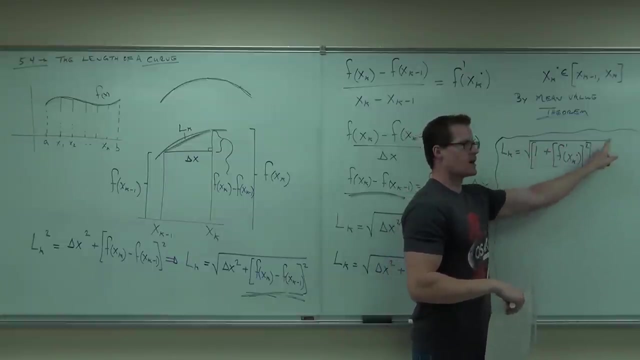 If you factor out the delta x squared, you need a bracket around this little thing, just like that. You okay with that? Now, roots are kind of awesome because you can split them up apart by multiplication. So do you see that I can have a square root of this? first thing times a square root. 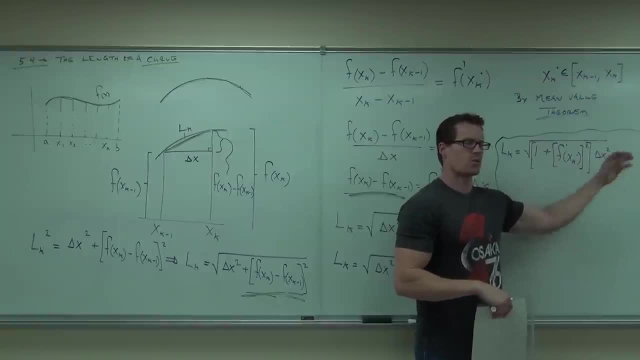 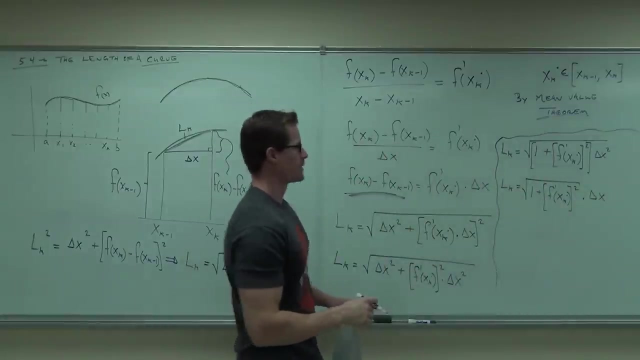 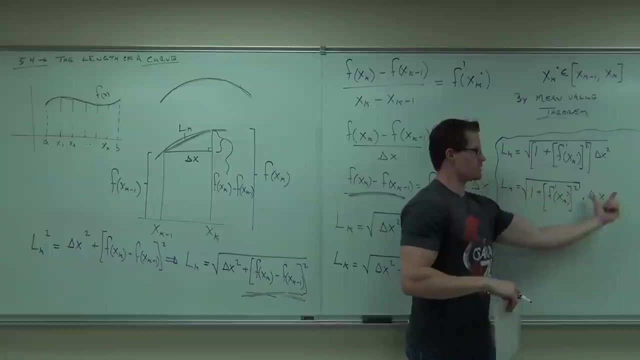 of this second thing. But a square root of delta x squared will give you just delta x. So next step is going to be l sub k. This times that Notice how I'm putting the stop after the square root. right there. We take the square root of delta x squared. it becomes delta x. 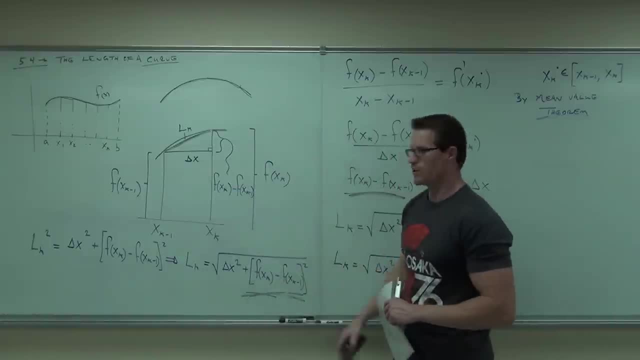 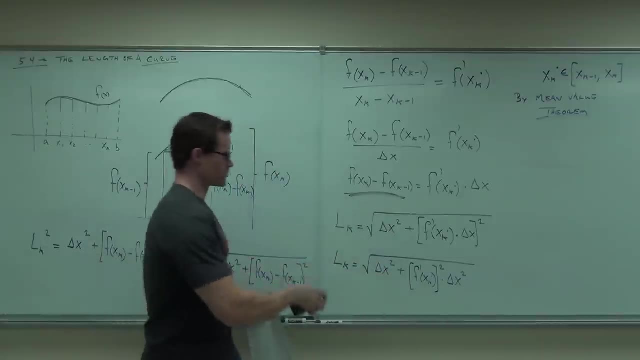 Now we're just working that down, so Take note of that. hopefully you have that. The important part was to get our substitution done from here to here. that was the idea. I guess I do have some room over here I can work on. 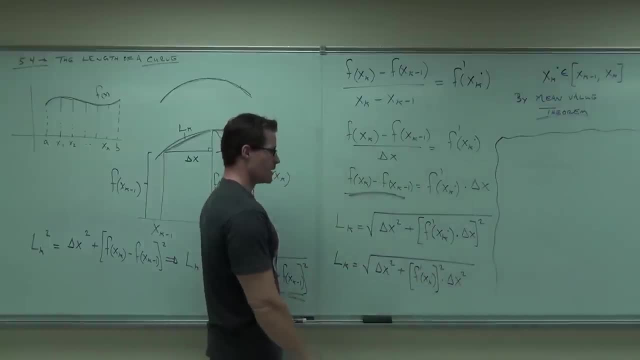 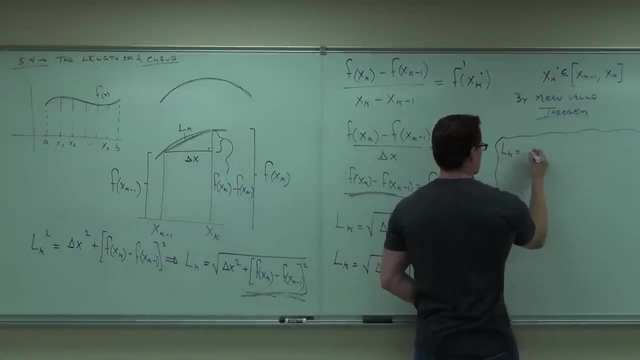 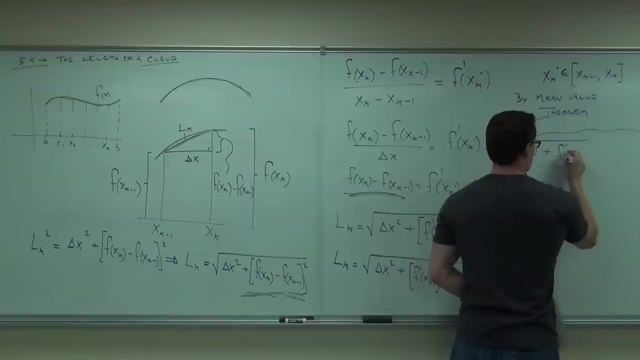 So from here do you see that we can factor out a delta x squared. So we're gonna have one f prime of xk dot squared times, delta x squared, but that is gonna be in a legal bracket. I'm withdrawing black so you can see. 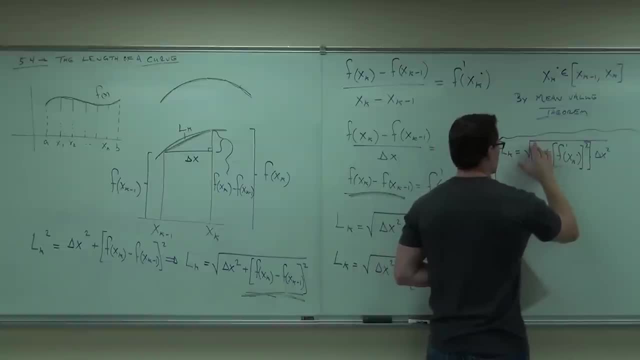 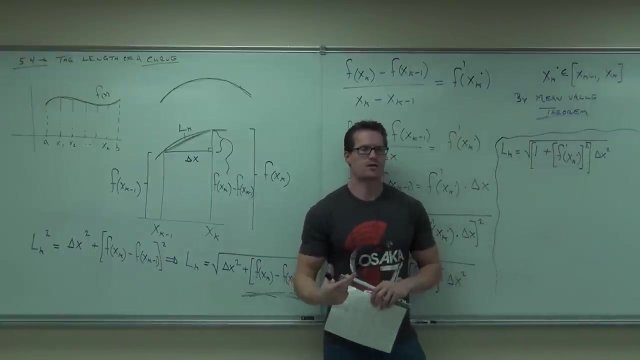 I'm gonna draw it in black so you can see a little bit better. If you factor out the delta x squared, you need a bracket around the square thing, just like that. You okay with that? Now, roots are kinda awesome because you can split them. 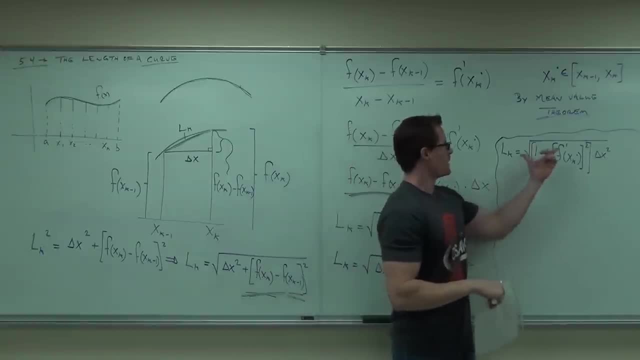 apart by multiplication. So do you see that I can have a square root of this first thing times a square root of the second thing. But a square root of delta x squared will do the same thing. But a square root of delta x squared will do the same thing. 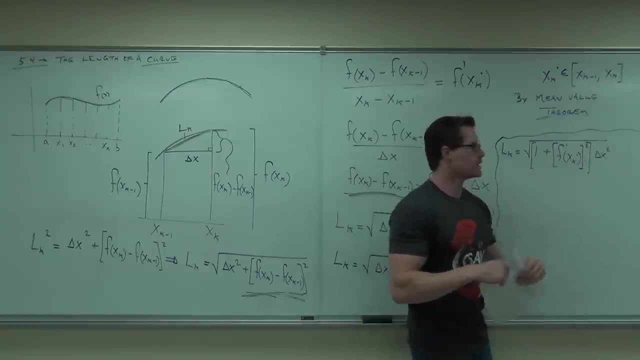 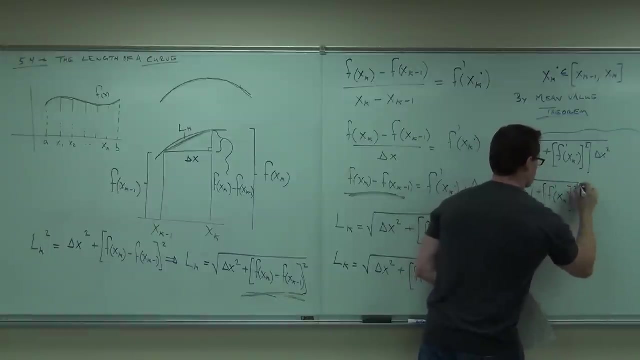 But a square root of delta x squared will do the same thing. give you just delta x. So next step is going to be L sub k. This times that Notice how I'm putting the stop after the square root. right there We take the square root of delta. 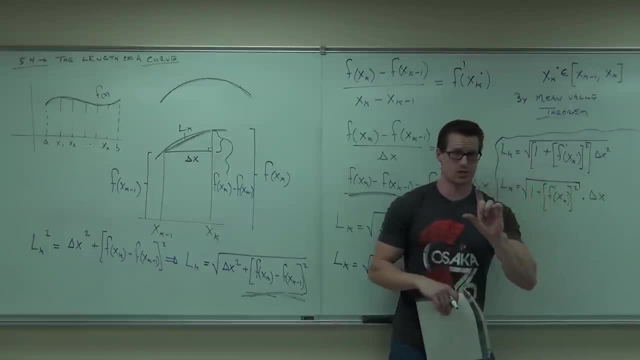 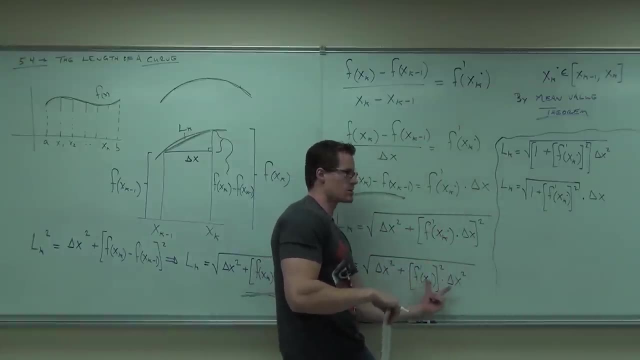 x squared, it becomes delta x. The only reason why we can do this, ladies and gentlemen- please notice this- is because we were able to factor out the delta x squared from right. here. We were able to factor it out, create a big bracket that's being multiplied and 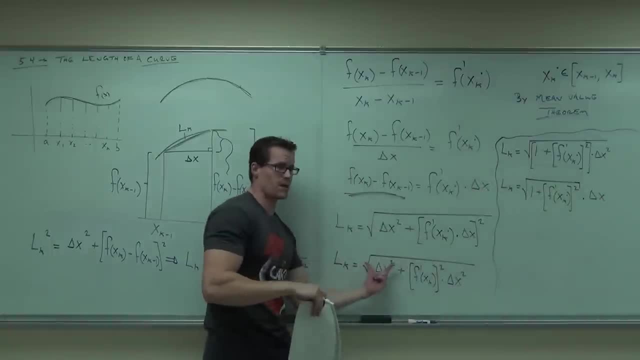 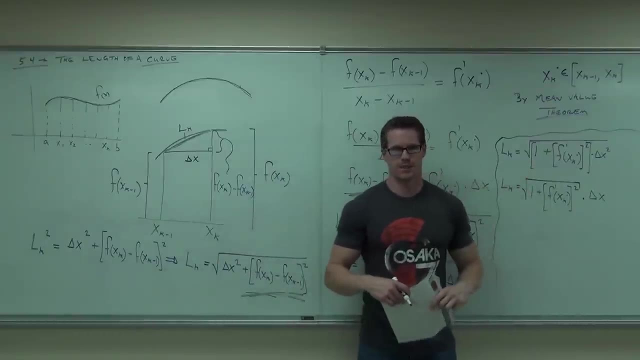 you can split up multiplication. You can't split up addition. We could not have done it here. You can't just take a square root and take a square root. It doesn't happen. You have to factor it, split it off, do all that nonsense, and then you can do it. How? 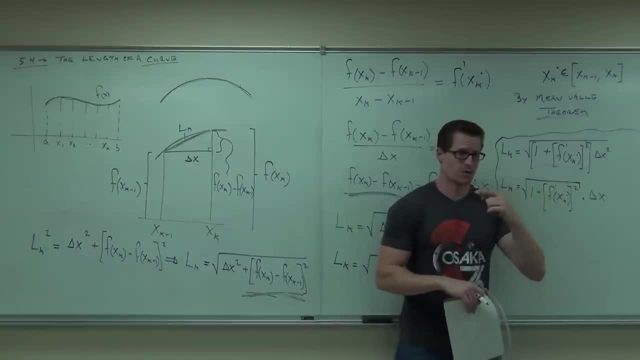 The only reason why we can do this- ladies and gentlemen, please notice this- is because we were able to factor out the delta x squared from right here. We were able to factor it out. Create a big bracket that's being multiplied And you can split up multiplication. 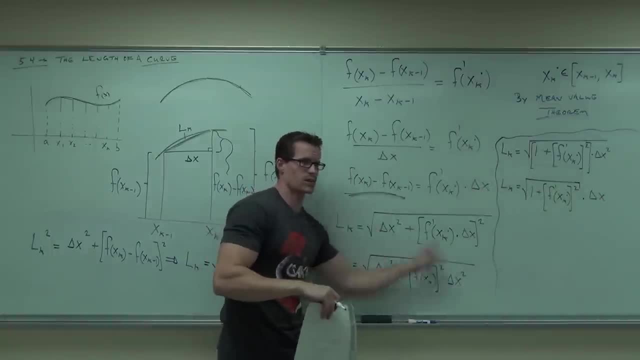 You can't split up addition. We could not have done it here. You can't just take a square root and take a square root. It doesn't happen. You have to factor it, Split it off, Do all that nonsense And then you can do it. 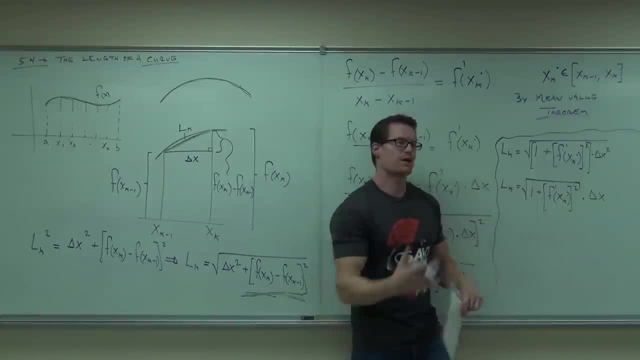 How many of you feel okay with all we've done so far? Hey, that's the length. That's the length for one single section. Tell me how I find multiple sections. A summation would help me find multiple sections Very good. 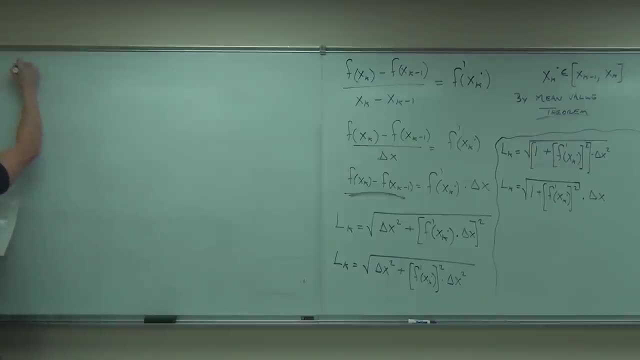 So that's for one, All right. So here's for all of them, but it's an approximation. So here's for all of them, but it's an approximation. So let me do this Here, And we're going to go down to our line. 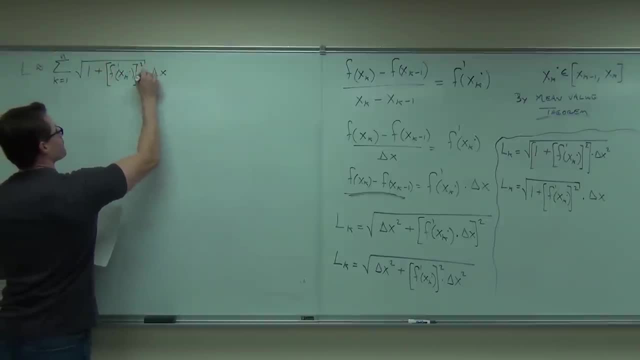 Here, Here, What's what? What's what? I can't do this, Okay, I can't do this. What I can't do this? What? Okay, Okay, I can't do this. Let's see, Okay. 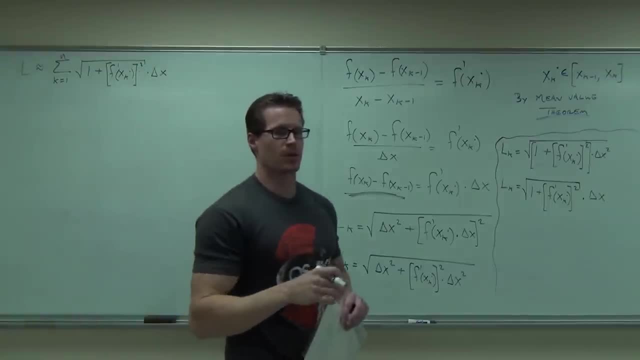 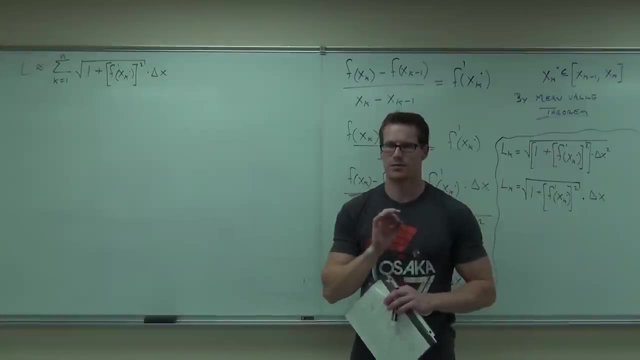 How do I make it a better approximation? Yeah, as n goes to infinity. that means, instead of just a few cuts within there, we're going to make an infinite number of cuts. That causes this distance. remember that was the distance between those points to go to zero. 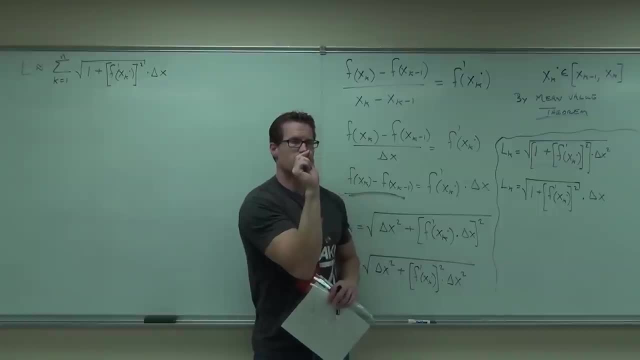 It causes the arbitrary point to be smashed in between there. So yeah, you have a little distance, because otherwise you can't find the length of that, right, You can't find the length of nothing. So it's a little distance, but it's so small it doesn't make any difference. 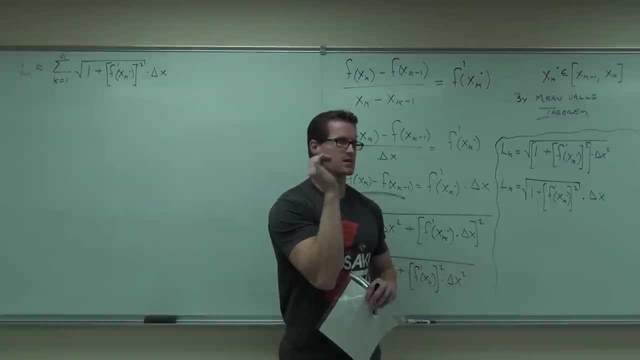 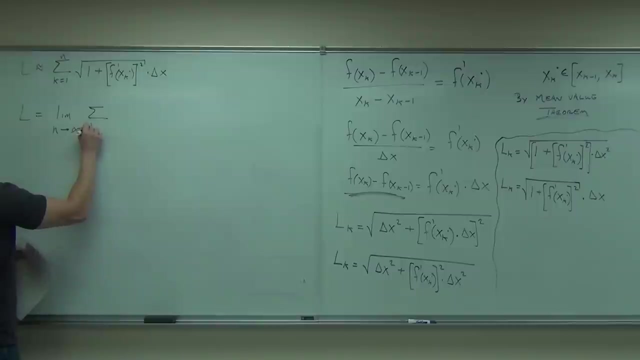 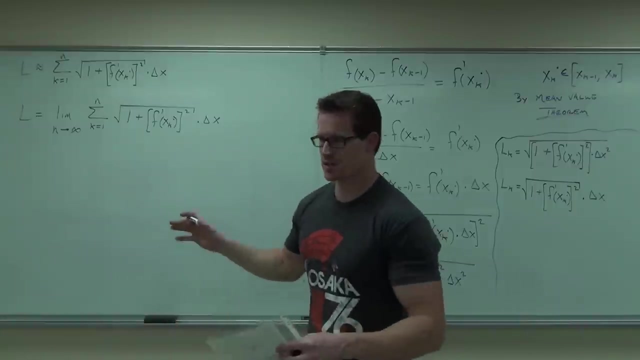 between the actual line, the secant line and the distance of our arc. So take a limit that l equals a limit of this thing. Now, when you take a limit, we've noticed just by practice what these pieces mean. Can you tell me what the limit of a sum becomes? 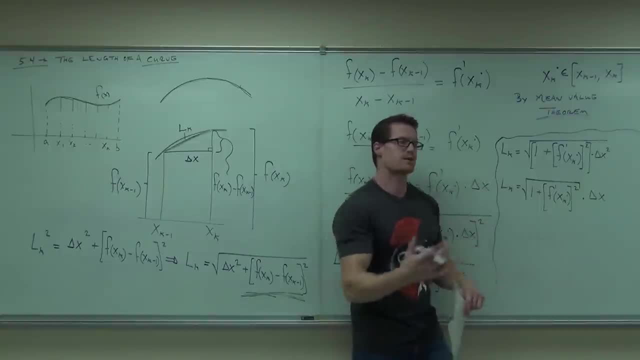 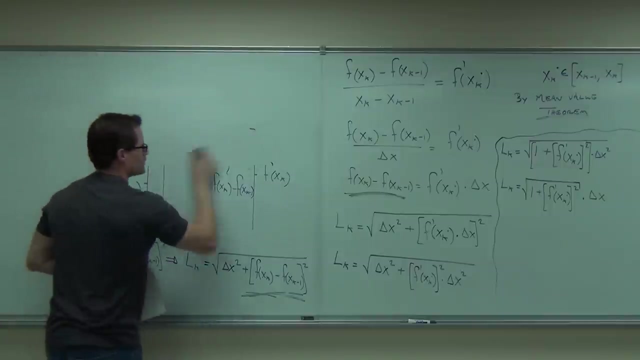 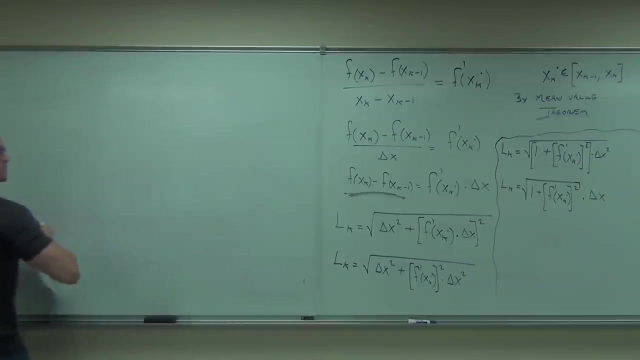 do people feel okay with all we've done so far? Hey, that's the length. That's the length for one single section. Tell me how I find multiple sections. Summation: A summation would help me find multiple sections Very good. 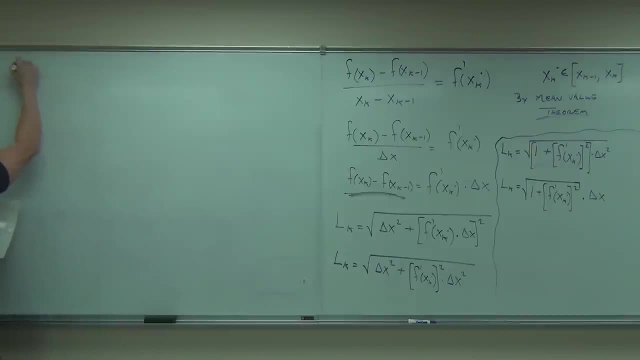 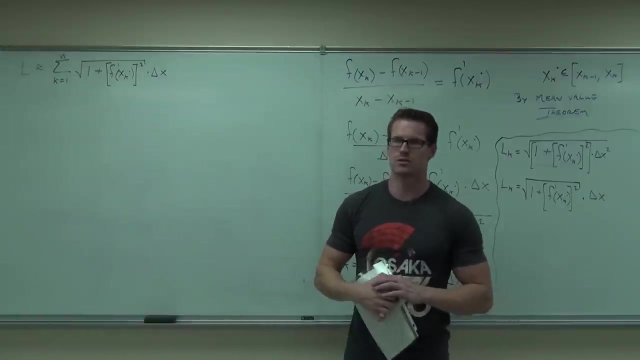 So that's for one. So here's for all of them. but it's an approximation. How do I make it a better approximation? Yeah, as n goes to infinity. that means infinity. Instead of just a few cuts within there, we're going to make an infinite number of. 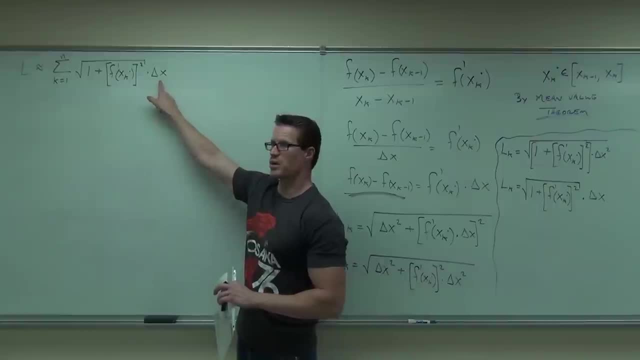 cuts. That causes this distance- remember that was the distance between those points- to go to zero. It causes the arbitrary point to be smashed in between there. So, yeah, you have a little distance, because otherwise you can't find the length of that right. 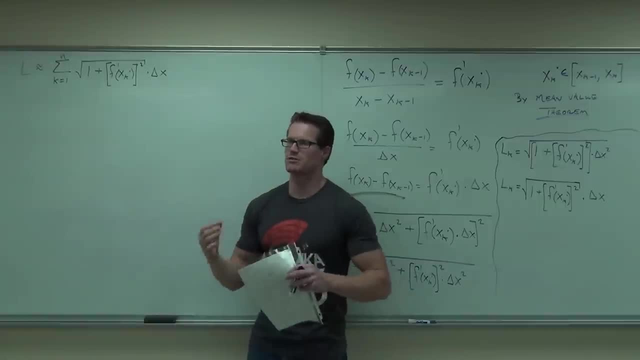 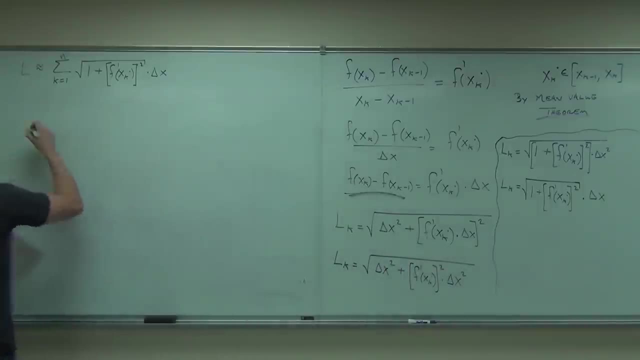 You can't find the length of nothing. So it's a little distance, but it's so small it doesn't make any difference between the actual line, the secant line and the distance of our arc. So take a limit that L equals a limit. 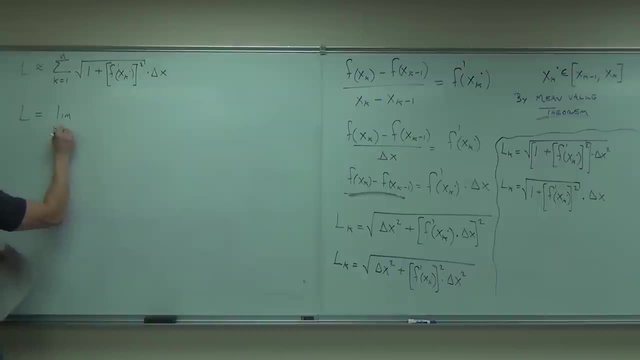 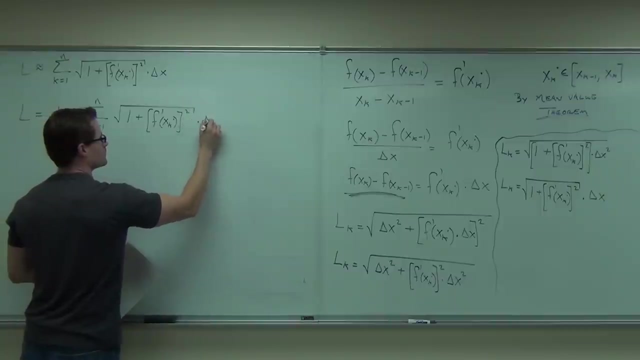 Okay, Okay, Okay Of this thing. Now, when you take a limit, we've noticed just by practice what these pieces mean. Can you tell me what the limit of a sum becomes? and it goes from where you start to where you stop. 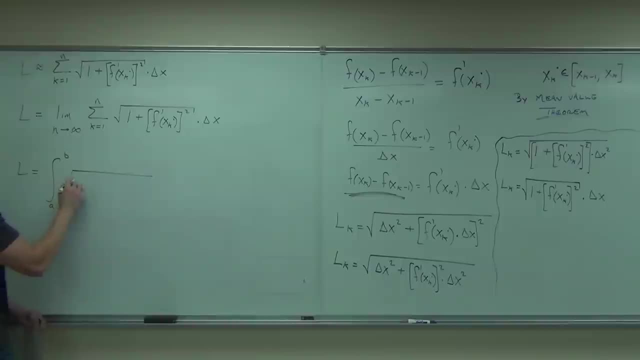 The square root. hey, that's a square root. The 1 is a 1.. Plus is a plus F prime. look at it. We're going to have a first derivative inside of our integral. Isn't that interesting? That's kind of weird. 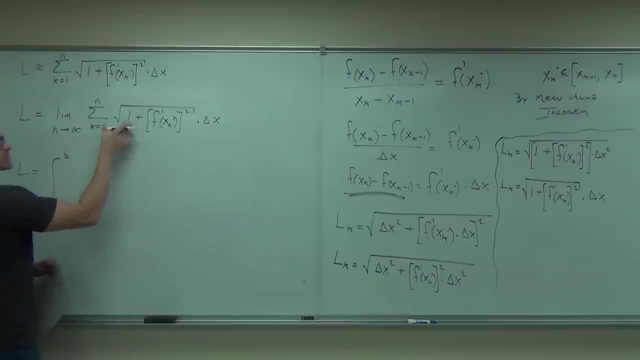 And it goes from where you start to where you stop. The square root- hey, that's a square root. The 1 is a 1.. Plus is a plus F prime. look at it, we're going to have a first derivative inside of our integral. 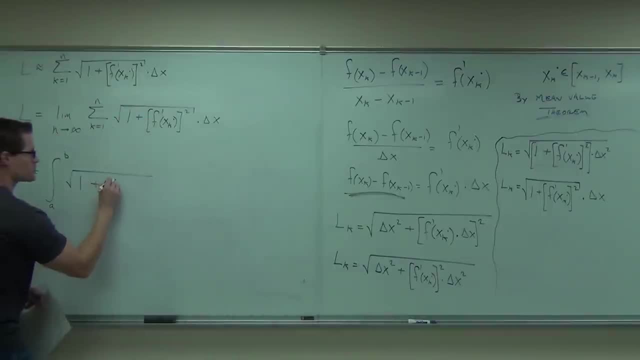 Isn't that interesting. That's kind of weird, But that's what that says. It says you have a first derivative of a function. What's xk dot become? Just s, Don't forget to square it. And what does the delta x become? 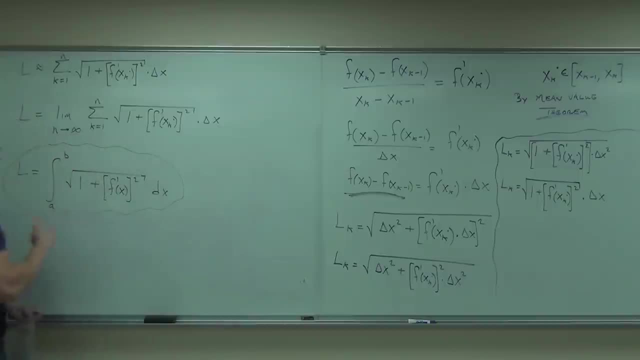 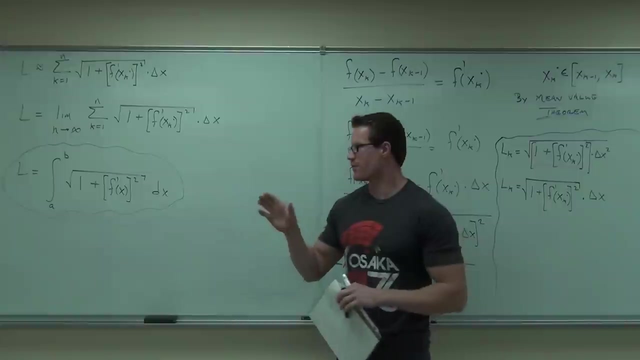 That's it. What we've just done is something that's freaking awesome. We just found the length of a curve between two points. Is that not cool? Very cool. We know how to find the length of a curve. You draw me a curve? 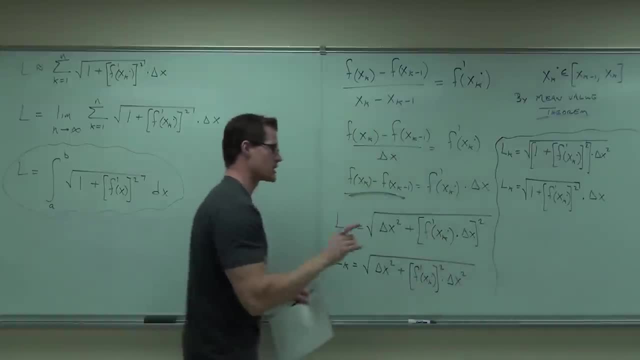 If you know the function to it, you find the length Now that clocks a little fast. We're going to do one example, because I don't want to leave you hanging on this. I'll explain something in a little while about why we are going to go over it a little bit. 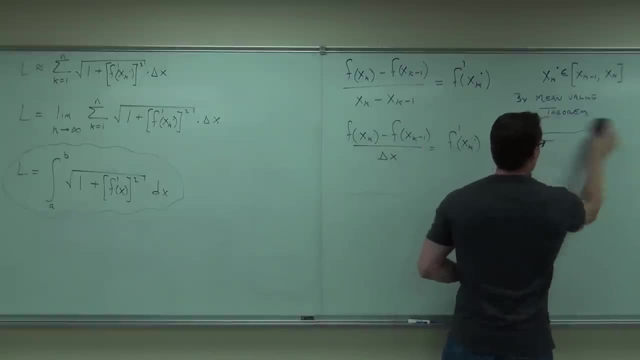 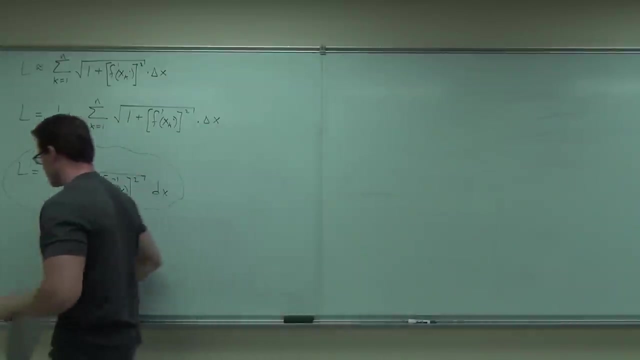 But stick with me. please Don't hate me. Trust me, I'm doing you a favor. So this is the length of a curve. Note that this is along which axis. And whatستheir swallowed. How do you feel? 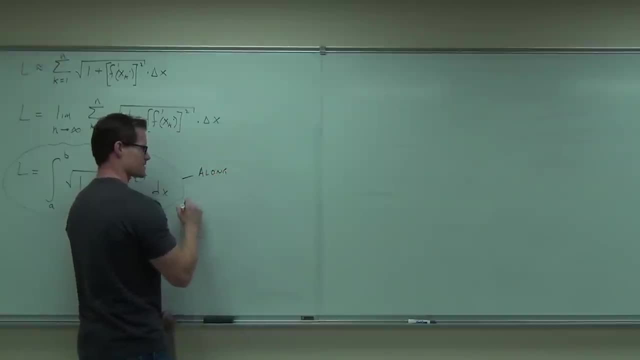 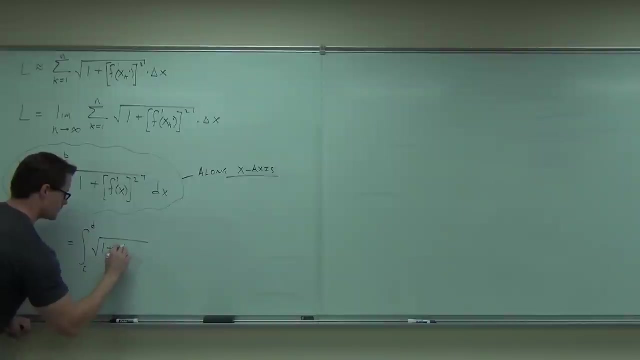 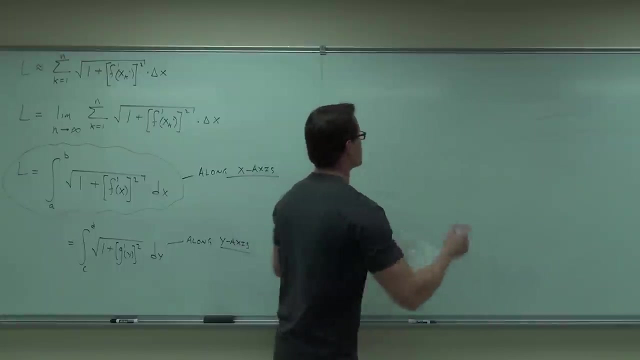 Shoot, I can't spell today, Yes, Yes, Why did you say that You should have? So these are going back to matching up along the x in terms of x, along the y in terms of y. It matches. I'll give you one example here. 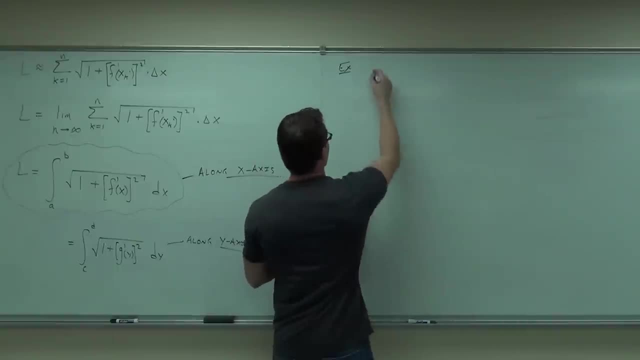 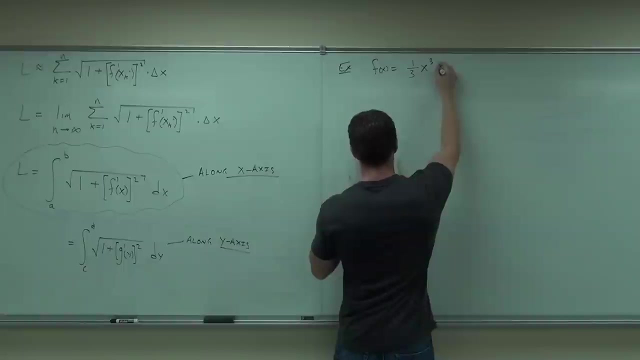 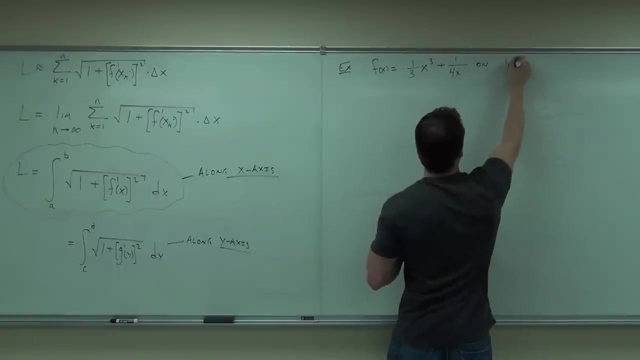 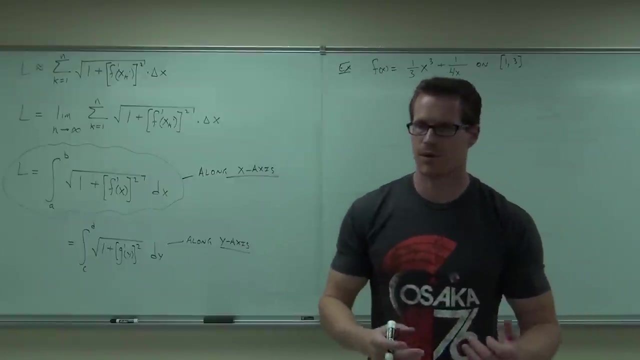 Let's say I would like you to find the length of the curve. this on that, I want to, right now, just practice setting this up, making sure we see where these pieces are coming from. That's important for us to do, So what's the first step? 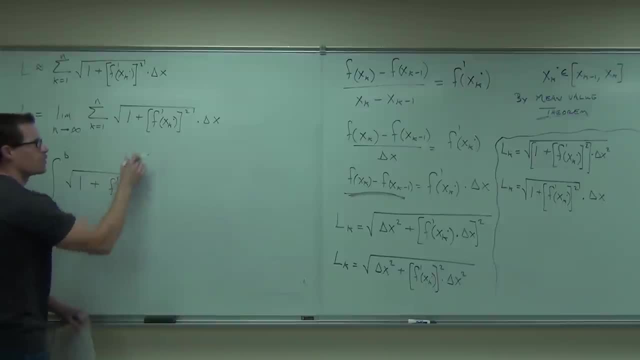 But that's what that says. It says you have a first derivative of a function. What's xk dot become? Just s? Don't forget to square it. And what does the delta x become Delta x? That's it. What we've just done is something that's freaking awesome. 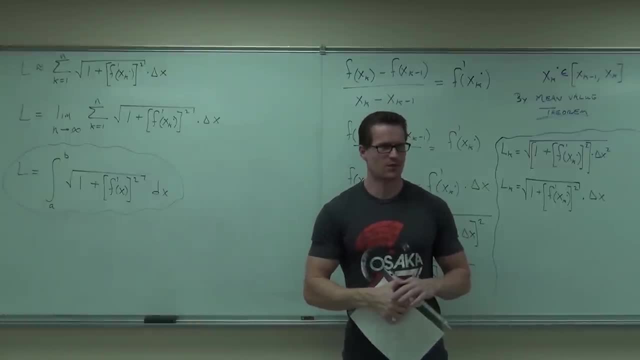 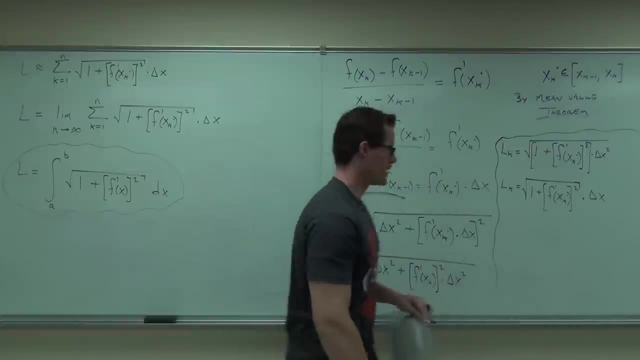 We just found the length of a curve between two points. Is that not cool? Very cool. We know how to find the length of a curve. You draw me a curve. if you know the function to it, you find the length. Now that clocks a little fast. 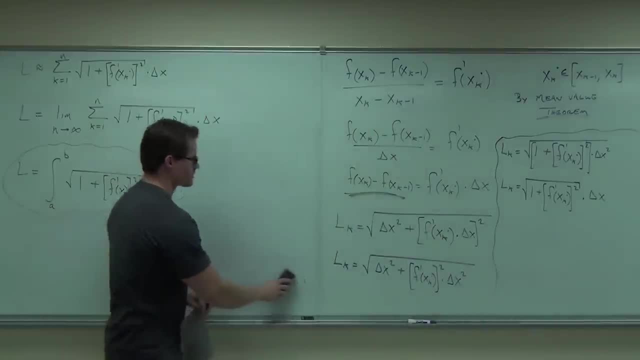 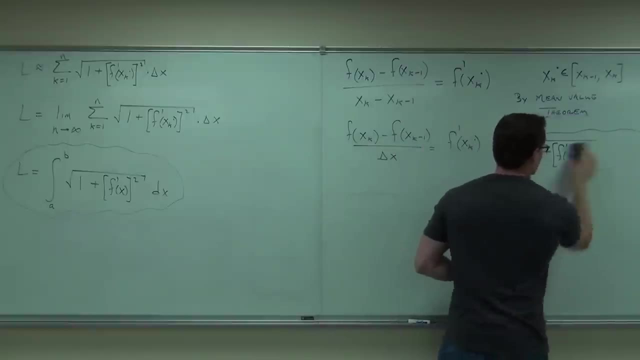 We're going to do one example, because I don't want to leave you hanging on this. I'll explain something in a little while about why it's important. We are going to go over it a little bit, But stick with me, please Don't. 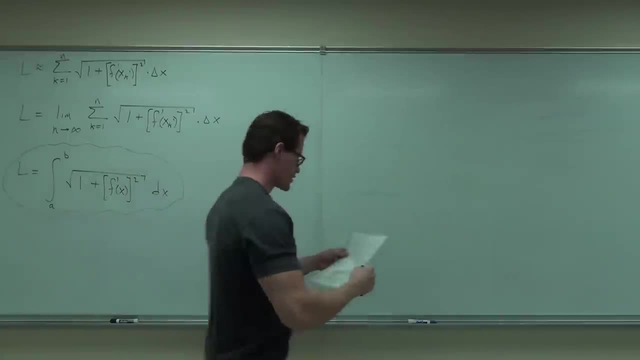 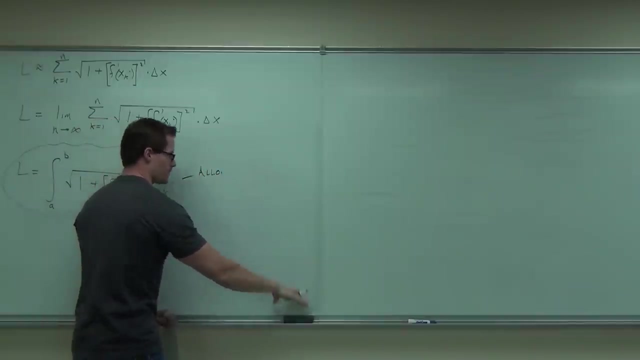 So this is the length of a curve. Note that this is along which axis X The value of. Okay, This is along the x axis. Okay, How do you spell long Shoot, I can't spell today. Yes. 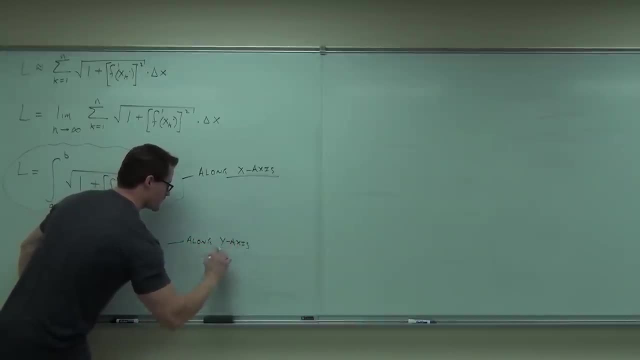 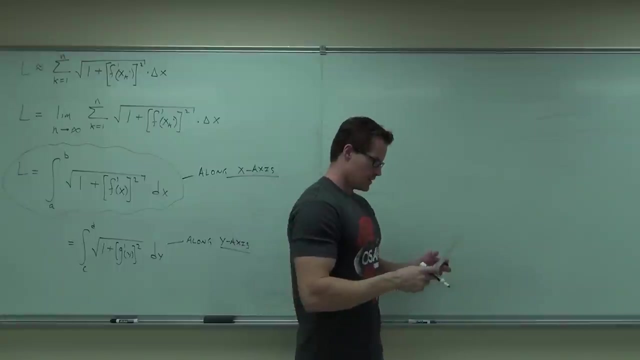 So these are back to matching up. Along the x in terms of x, along the y in terms of y, It matches. I'll give you one example here. Let's say I would like you to find the length of the curve This: 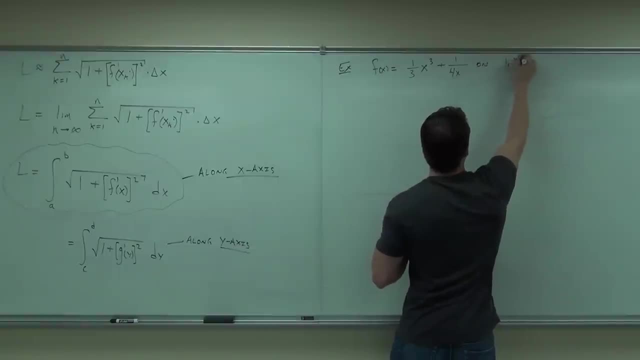 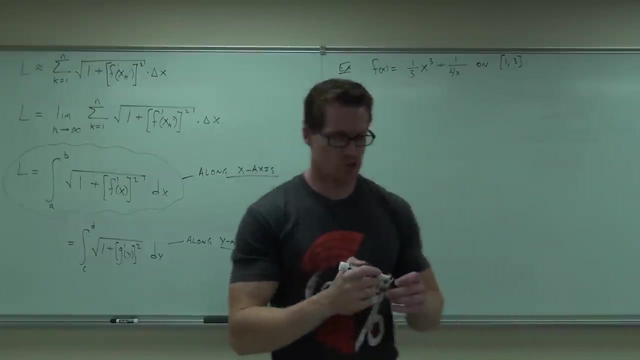 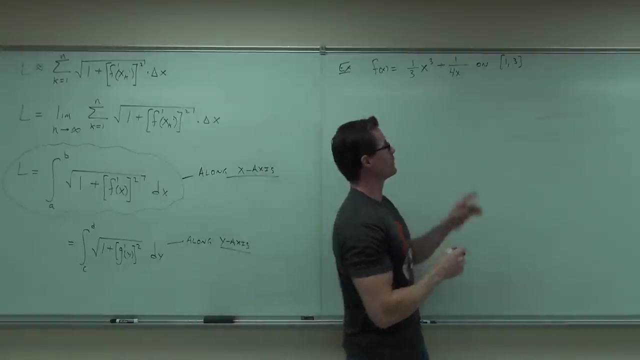 This. On that, I want to right now just practice setting this up, making sure we see where these pieces are coming from. That's important for us to do, So what's the first thing? If we're going along well, it doesn't really matter. 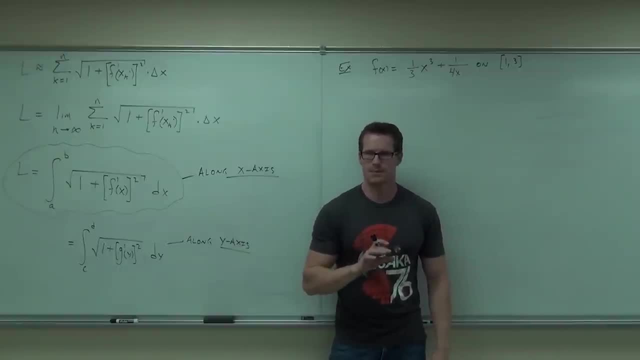 Let me put it another way. Whether you think of this in terms of x or y, the length of the curve doesn't change. Length of the curve is the length of the curve, So do what's easiest for you. Okay, The volume of a region is the volume of a region, right? 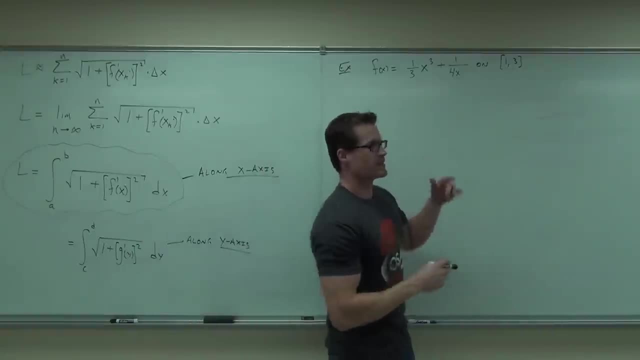 What's the first step, The first thing: if we're going along well, it doesn't really matter. let me put it another way: Whether you think of this in terms of x or y, the length of the curve doesn't change. 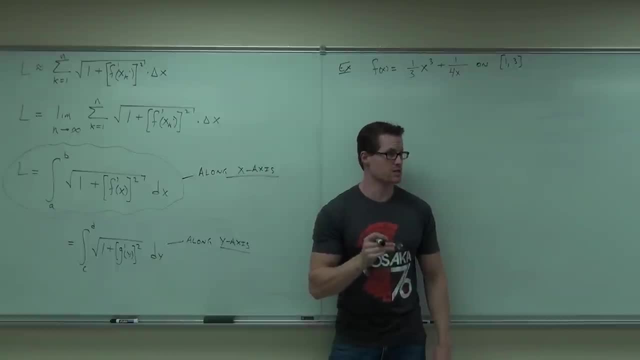 The length of the curve is the length of the curve, So do what's easiest for you. The volume of a region is the volume of a region, right? It doesn't matter what you do it in, as long as you do it correctly. 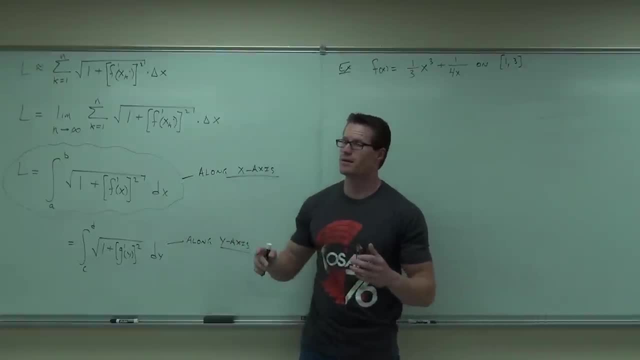 So whether you want to treat this along the x-axis or along the y-axis doesn't matter. Use what's given to you Now. this is in terms of x. We're going to do it along the x-axis Now. the process doesn't change at all, really. 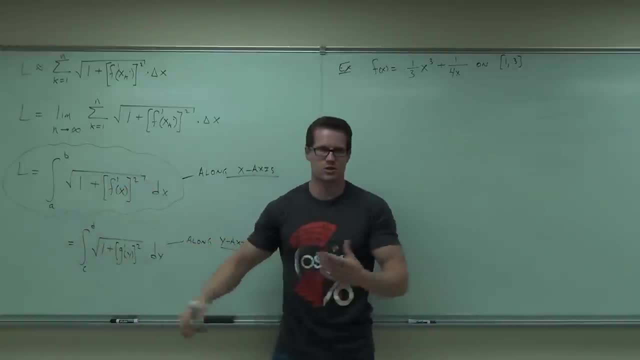 There's no x's or y's in here. Everything's coming from your function, so it's good to go Looking at our formula. what's the first thing you're going to do? Add a derivative. Say it again: Add a derivative. 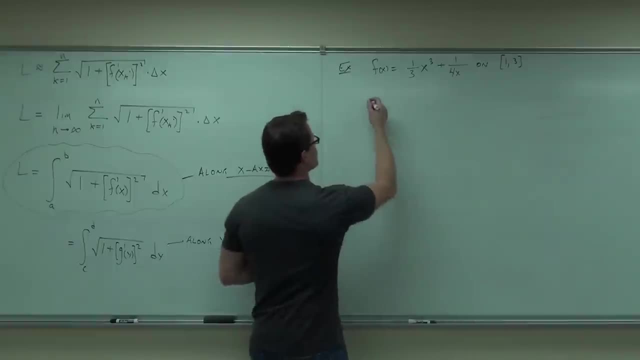 Yeah, you've got to have a derivative. That's nice. Find a derivative. If I do the derivative, don't forget how to do a darn derivative. all right, Some people just miss the little constants. The little constants are man. it's just a simple mistake. 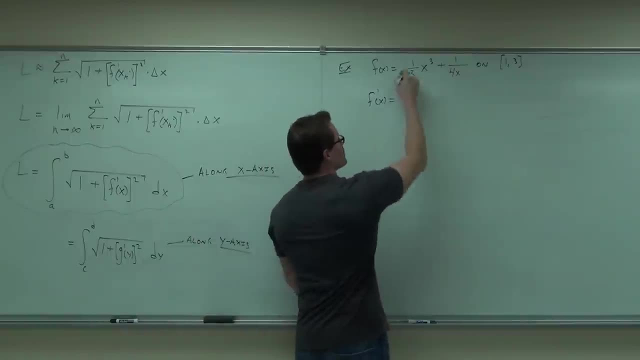 No, It's killing you. It's not simple anymore. Three comes down, No more one-third, You just get x squared. That is well negative one-fourth, Oh well, negative one over four: x squared. Can someone double check that for me please? 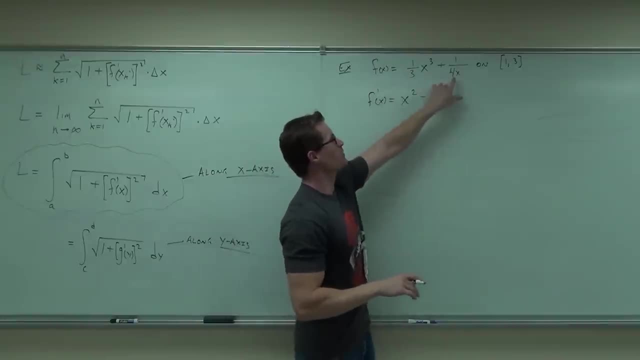 It's right, isn't it? So find your derivative. Notice. I moved my x up. I left the one-fourth alone. Moved my x up. Negative one comes down in front. It's negative one-fourth Subtract And the exponent becomes negative two. 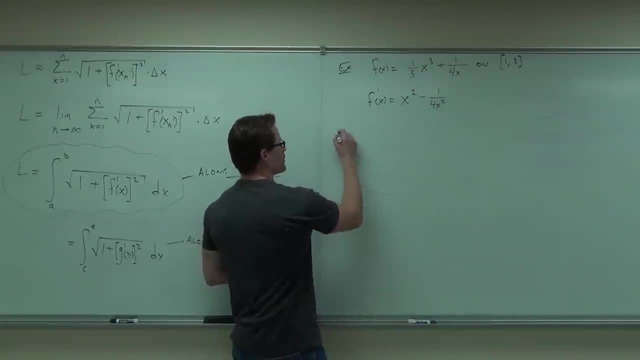 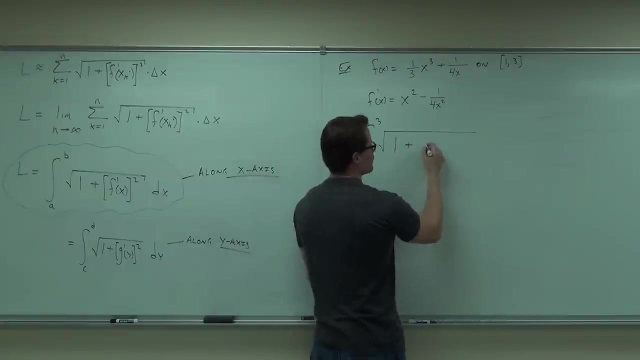 Move it back down, You get over x squared. If we set up our integral, where are we starting? On inside the integral, we're going to have a square root. We're going to have one plus. On the inside of that square root, you're going to have x squared minus one over four. 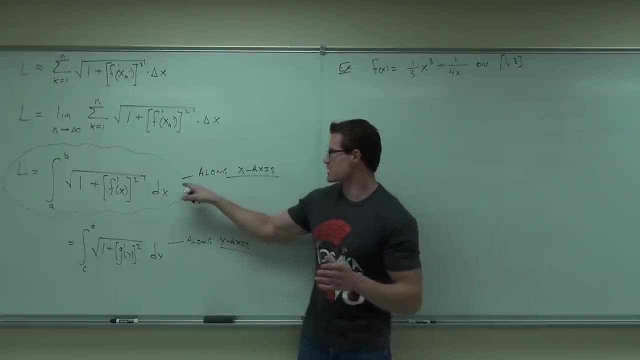 It doesn't matter what you do it in, as long as you do it correctly. So whether you want to treat this along the x-axis or along the y-axis doesn't matter. Use what's given to you Now. this is in terms of x. 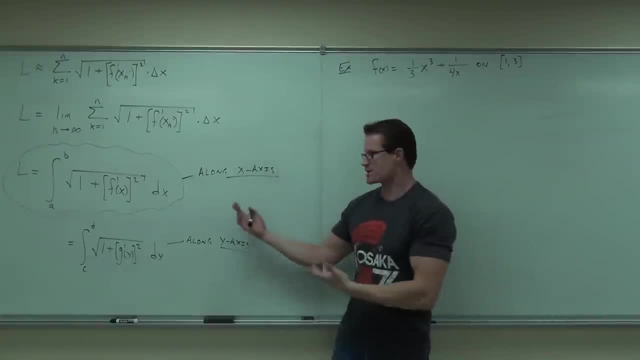 We're going to do it along the x-axis Now. the process doesn't change at all. really, There's no x's or y's in here. Everything's coming from your function, so it's good to go Looking at our formula. what's the first thing you're going to do? 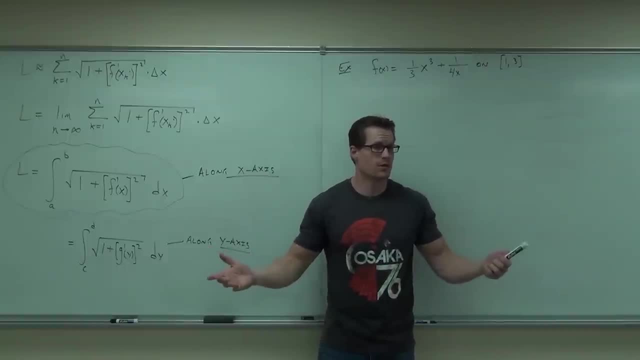 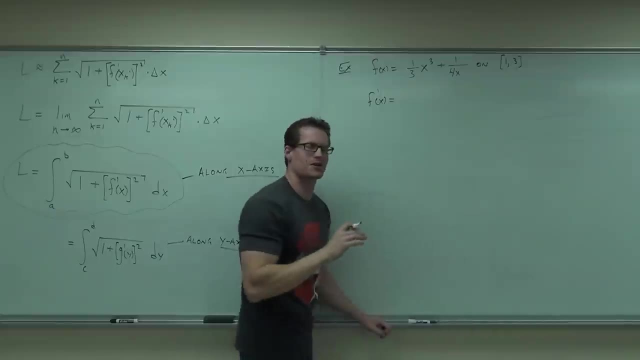 Say it again: Yeah, you've got to have a derivative. That's nice. Find a derivative. If I do the derivative, don't forget how to do a darn derivative. all right, Some people just miss the little constants. The little constants are man. it's a simple mistake. 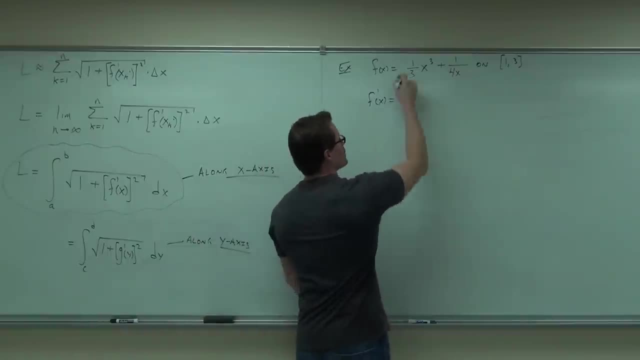 No, it's killing you. It's not simple anymore. Three comes down, no more one-third, You just get x squared. That is well negative one-fourth, Oh well, negative one-fourth. One over four: x squared. 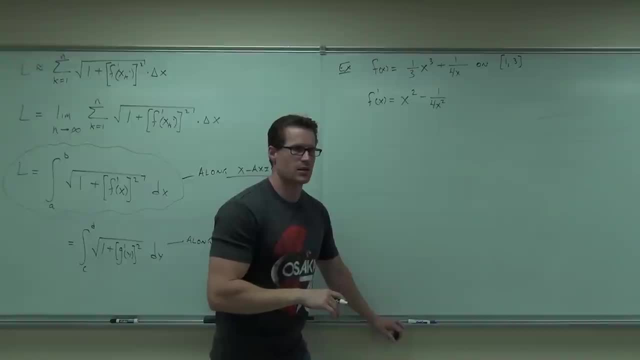 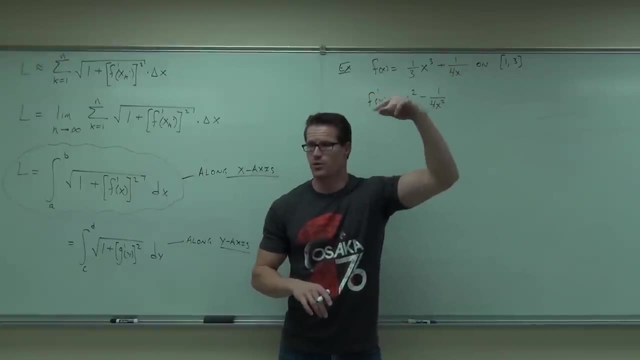 Can someone double-check that for me please? It's right, isn't it? So find your derivative. Notice, I moved my x up. I left the one-fourth alone. Moved my x up. Negative one comes down in front. It's negative one-fourth. 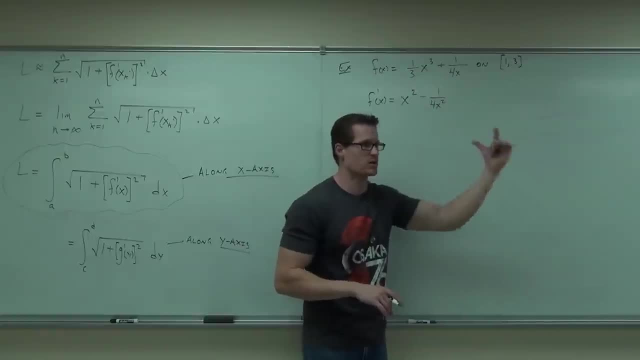 Subtract from the exponent, It becomes negative. two: Move it back down, You get over x squared. If we set up our integral, where are we starting One-third? Wait a minute. Inside the integral, we're going to have a square root. 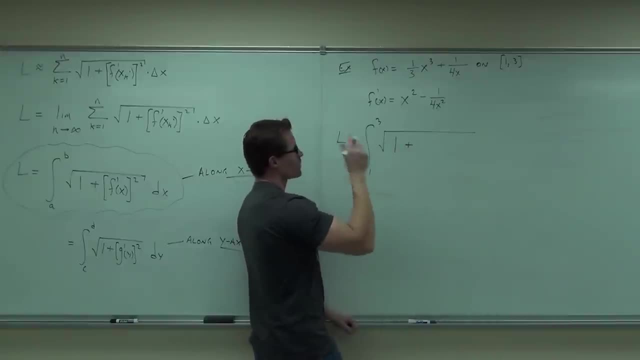 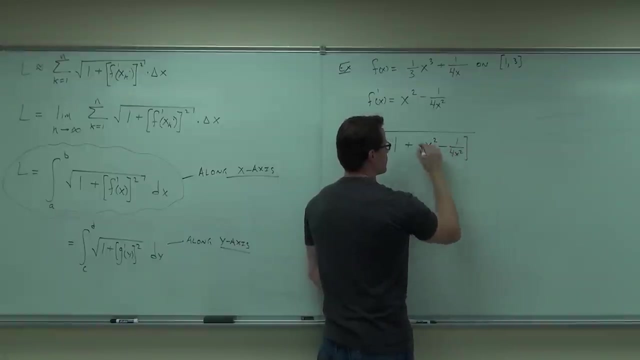 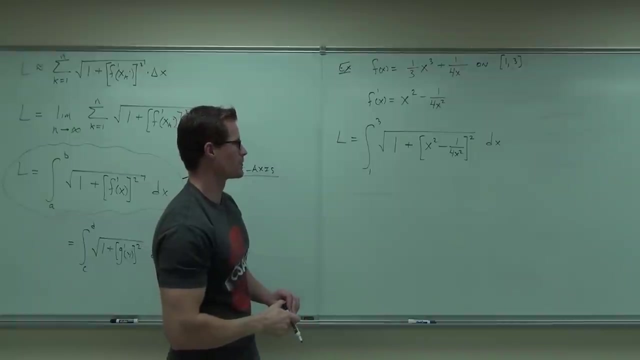 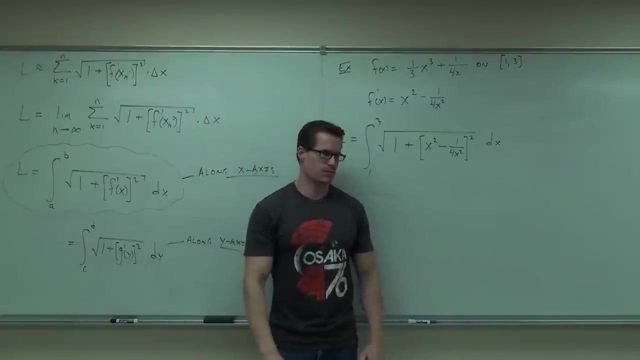 We're going to have one plus On the inside of that square root. you're going to have x squared minus one over four x squared squared dx. How many of you feel okay with a setup, at least a setup? What's your next step? 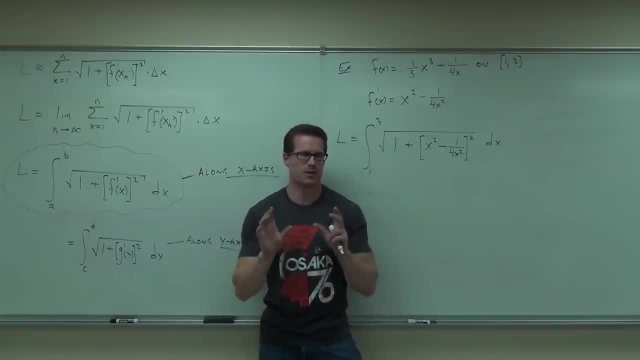 Remember, These have to work out. They have to be able to be manipulated or you can't do them. There's not going to be a substitution, There's nothing to substitute. They have to be algebraically manipulated for this class in order for you to even do them. 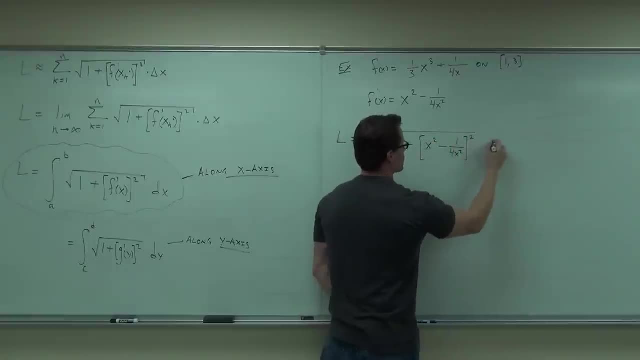 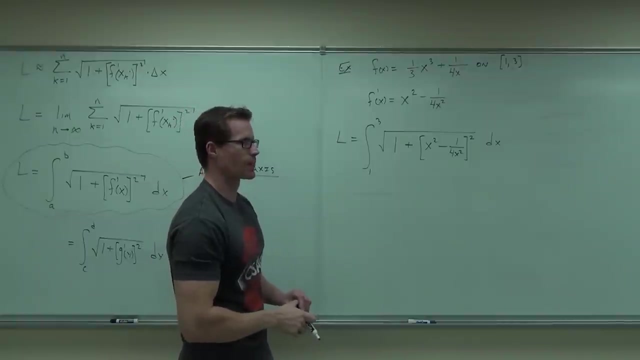 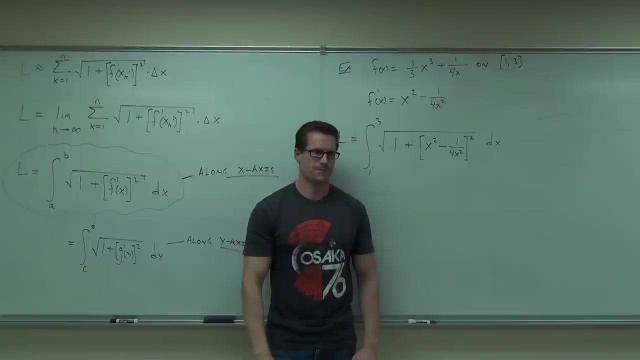 x. squared, Squared, Squared Dx. How many of you feel okay with the setup, at least the setup? What's your next step? Remember, these have to work out, have to be able to be manipulated, or you can't do. 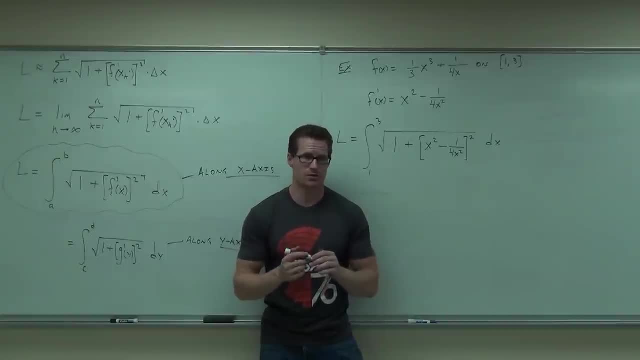 them. There's not going to be a substitution. There's nothing to substitute. Okay, They have to be algebraically manipulated for this class in order for you to even do them. What's the first Square? root Square. Yeah, You're going to square. 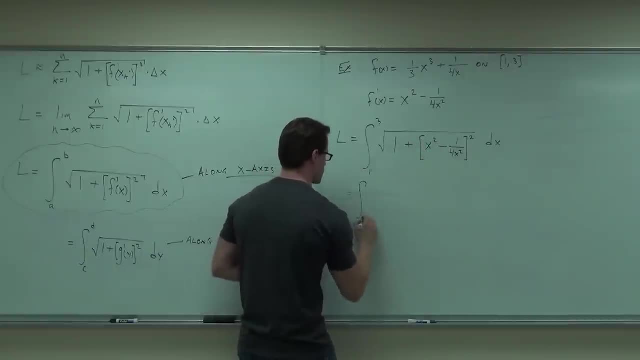 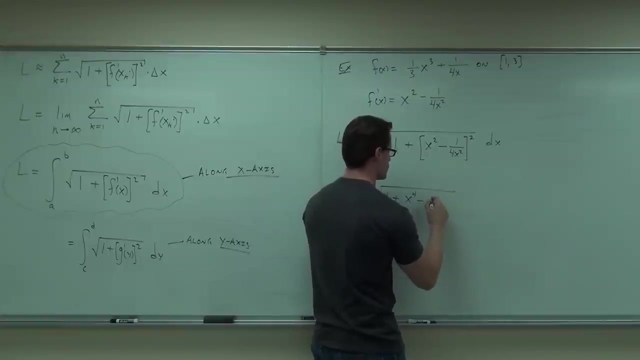 What you're going to get is x to the fourth minus one half x squared. No, I'm sorry, I need to work it out. I can't do that. one in my head. One-sixteen, One-sixteen Minus. 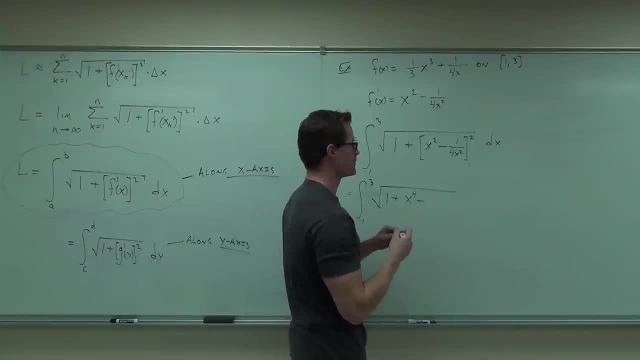 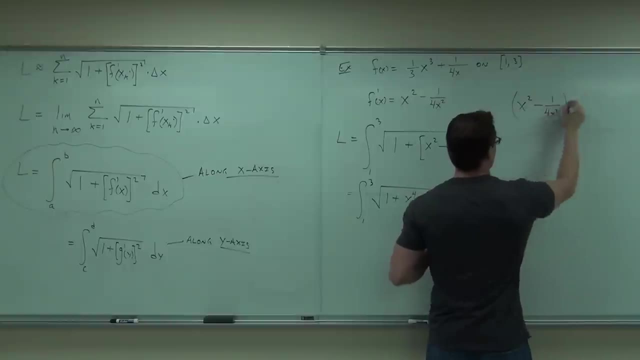 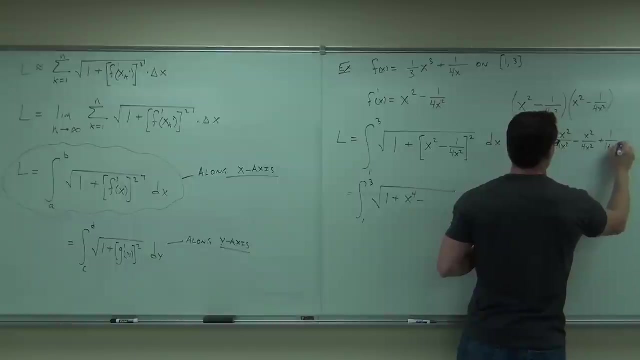 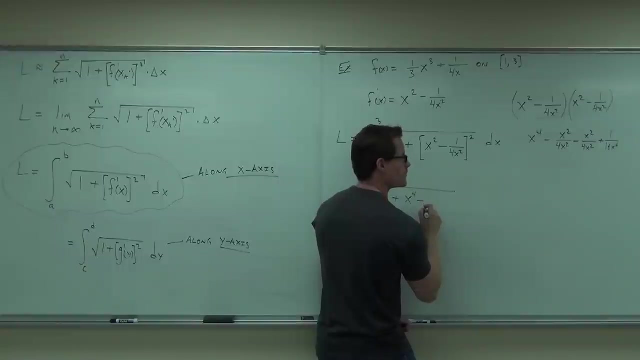 Minus One minus seven equals my fourth minus one-sixteen, where I have minus, Yeah. And then x to the fourth ити. One fourth minus one fourth is just minus one half. Okay, I think we'll leave it for there. 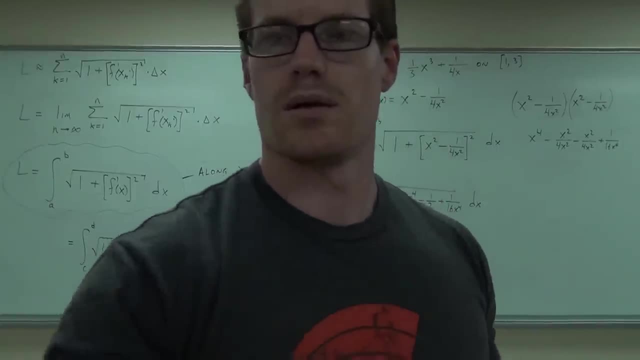 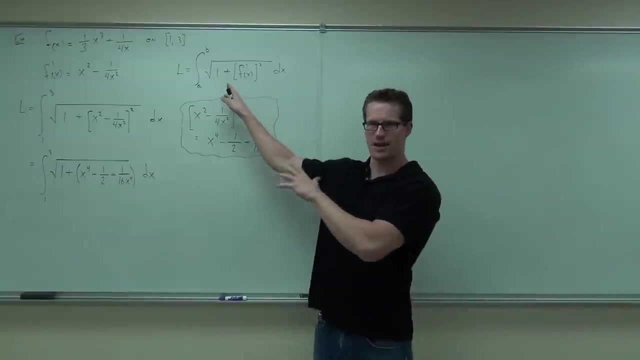 We'll talk about how to do the recess later on. I won't go into too long, Let's continue our problem. Find the length of a curve between two points. So we have. I think I derived that for you last time, didn't I? 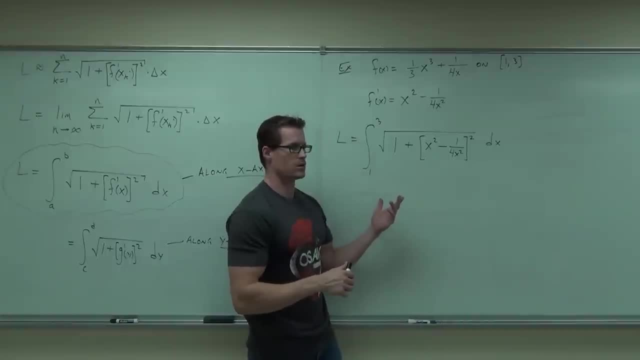 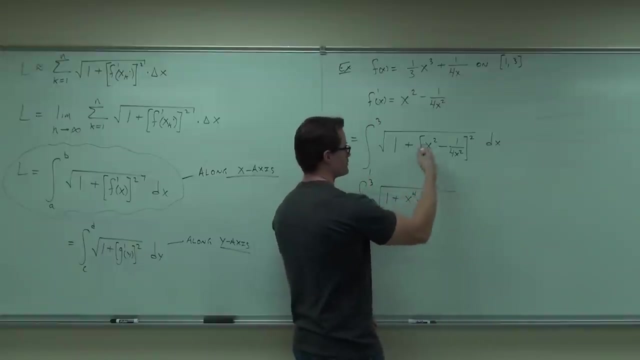 So what are you going to do? first, Square, Square. Yeah, you're going to square. You're going to get is x to the fourth minus One-half x squared. No, I'm sorry, I need to work it out. 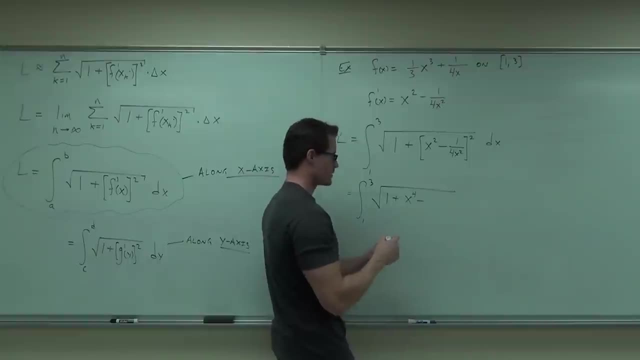 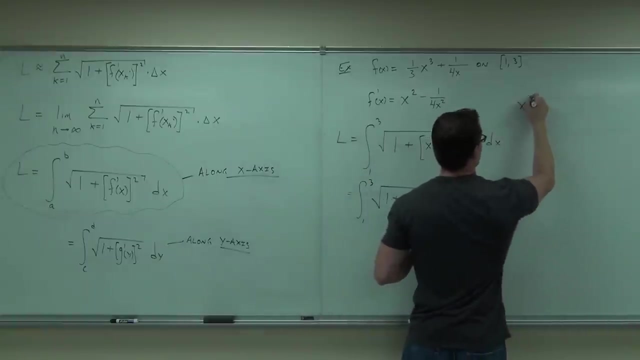 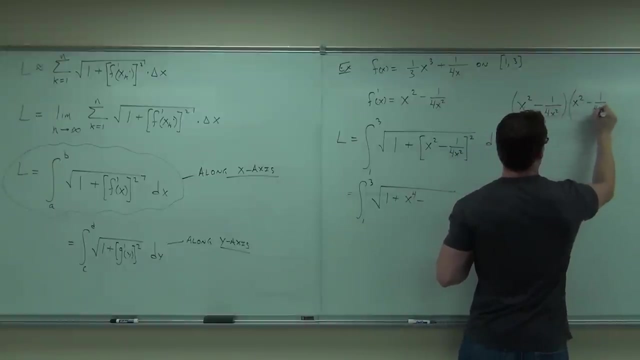 I can't do that. one in my head: One-sixteenth minus x to the fourth minus one-sixteenth And then x to the fourth. Oh, ok, I'm sorry. One-sixteenth minus x, squared. Ok, This is right, right. 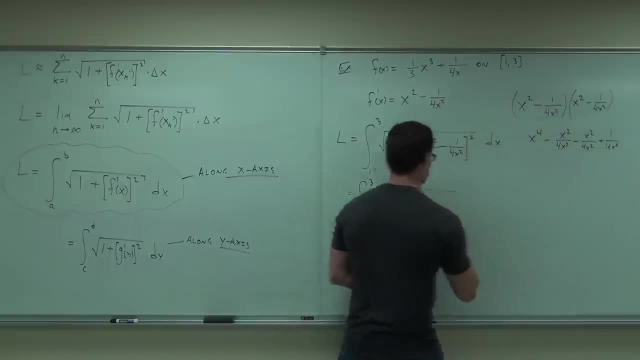 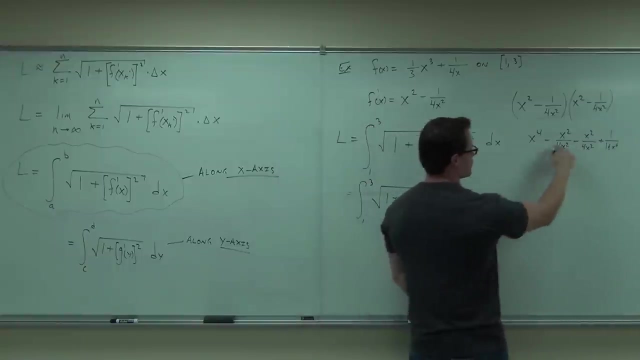 One-fourth minus one-fourth is just minus one-half. And then, doing that, is there a solution to this, To this? Let's try this again. This is right, right. One-fourth minus one-fourth is just minus one-half. 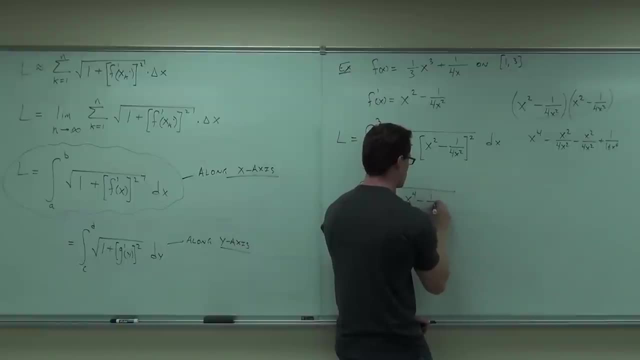 Ok, And this, This is right, right, One-fourth minus one-fourth is just minus one-half. Oh, ok, Ok, And this Look at me. Okay, I think we'll leave it for there. We'll talk about how to do the recess later on. 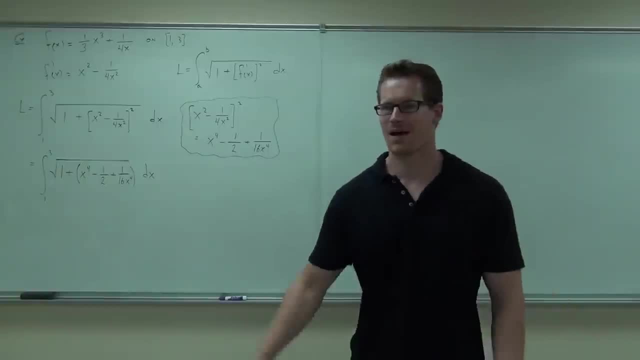 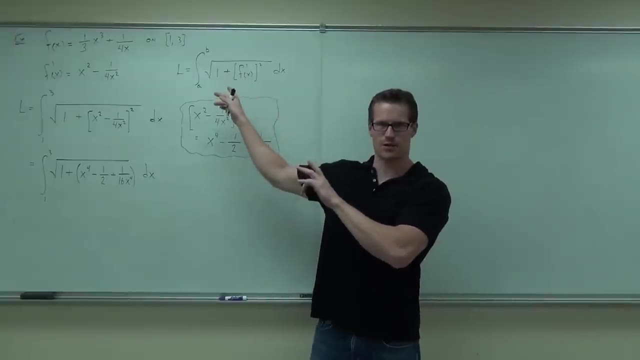 I don't want to put you in too long. Let's continue our problem. We'll find the length of a curve between two points. So we have. I think I derived that for you last time, didn't? I Made that up for you. 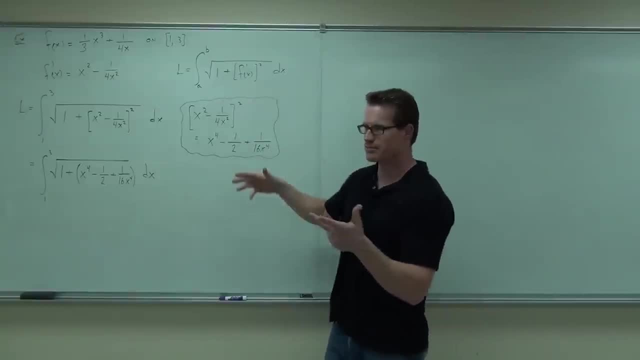 Cool. So we have. we're doing an integral from our two. you know bounds And we're going to go square root of 1 plus the derivative of the function, squared. Don't forget that's a derivative of the function. Don't forget to square it. 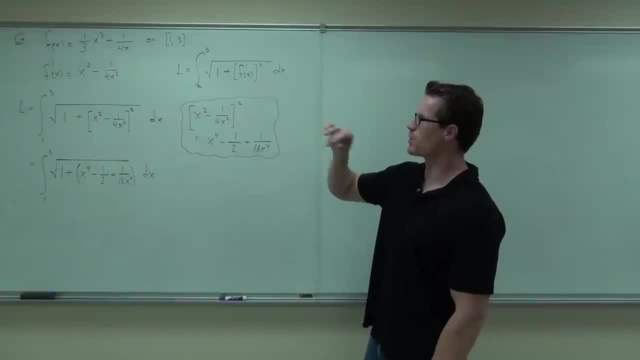 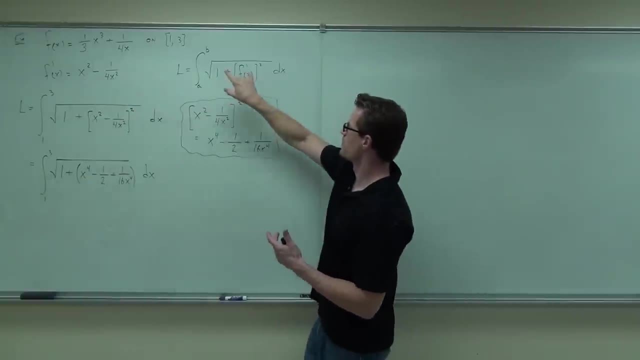 Dx. So our function is 1 third x cubed plus 1 over 4x. We've gone ahead and found the first derivative. So what we're doing here is we're just taking this first derivative, plugging it into this function or this formula and we have this integral is left. 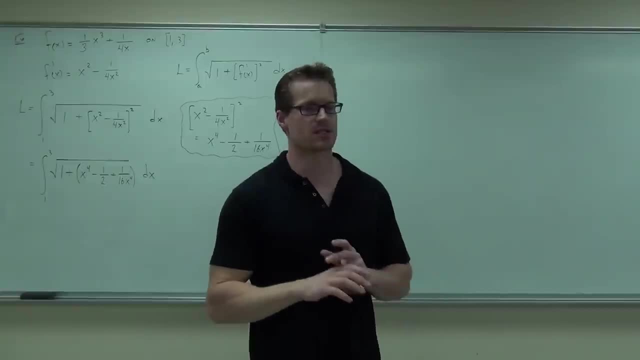 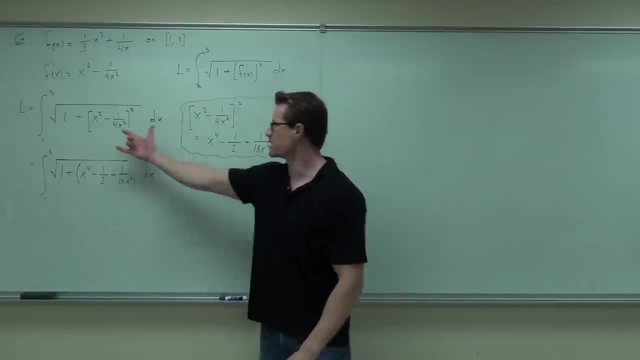 After that it's really just algebraic manipulation. The integral is not going to be hard. in general, It means you have to manipulate it, though algebraically, before you can even do the integral. See, right now you're stuck, I mean you can't do anything. 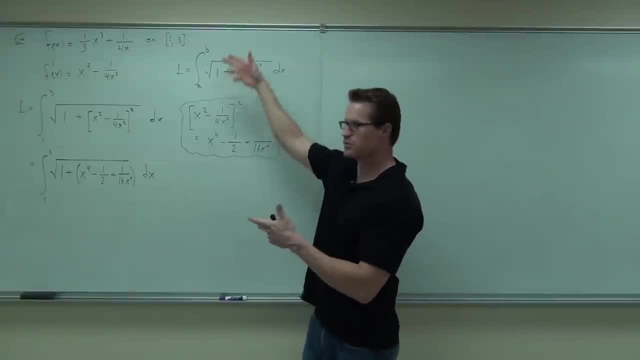 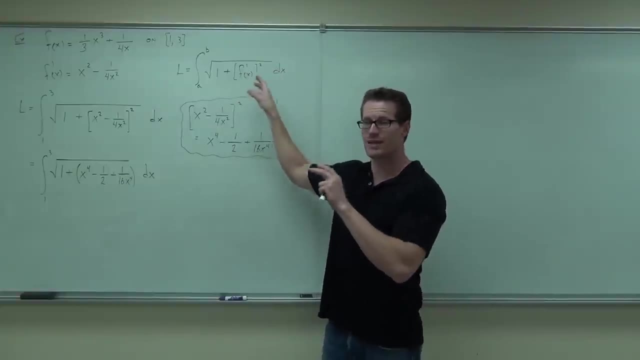 I made that up for you, Cool. So we're doing an integral from our two bounds and we're gonna go square root of one plus the derivative of the function squared. Don't forget that's a derivative of the function. Don't forget to square it, dx. 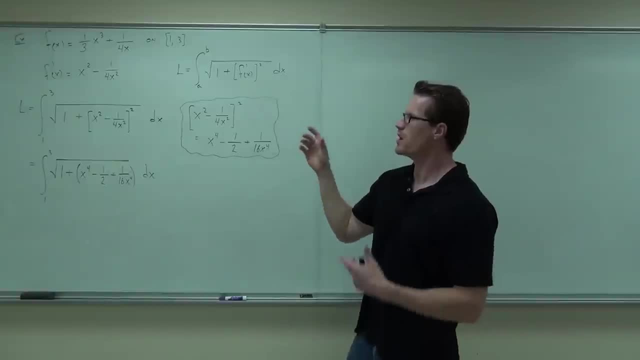 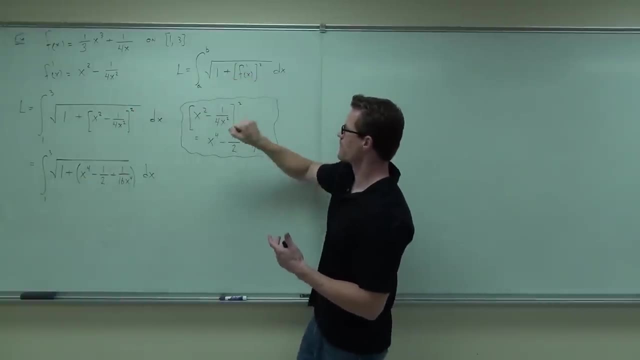 So our function is one third x cubed plus one over four x. We've gone ahead and found the first derivative. So what we're doing here is we're just taking this first derivative, plugging it into this function or this formula. 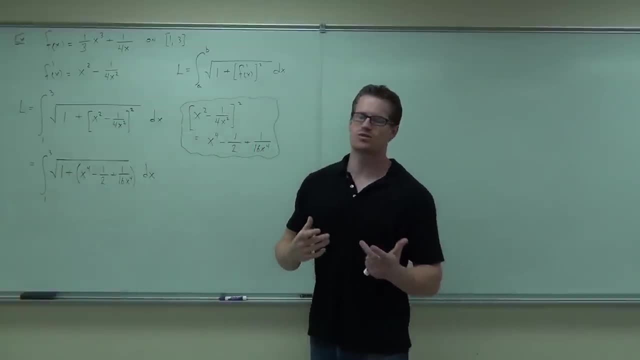 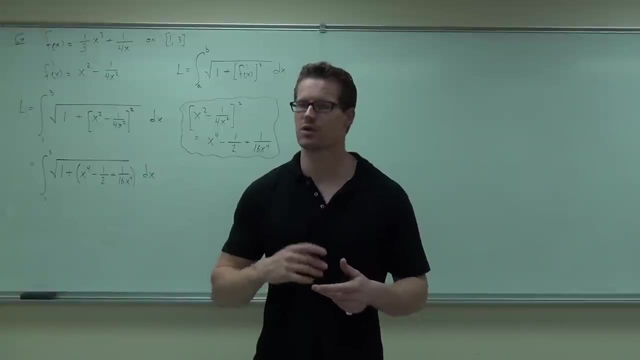 and we have this integral is left After that. it's really just algebraic manipulation. The integral is not going to be hard. in general, It means you have to manipulate it, though algebraically, before you can even do the integral. See, right now you're stuck. 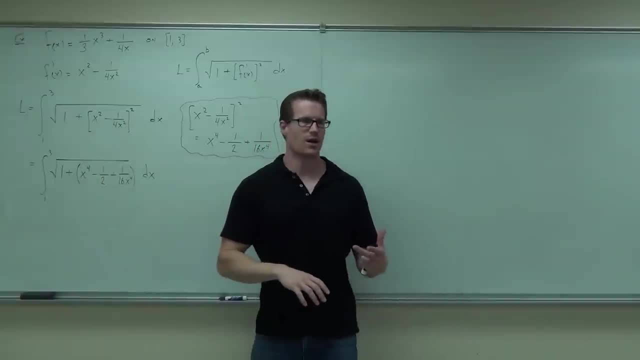 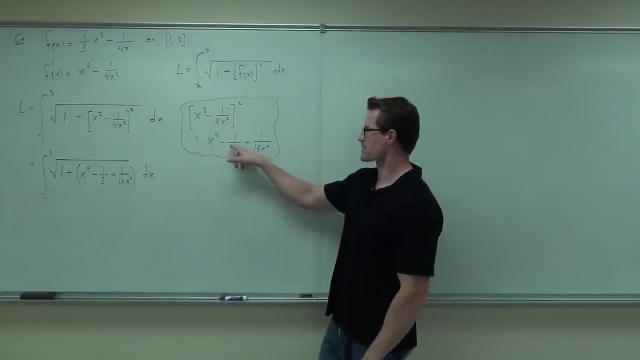 You can't do anything with that. You gotta completely break this thing down and see exactly what we can do. You follow me on that. So we square this. we get x to the fourth minus one, half plus one over 16: x to the fourth. 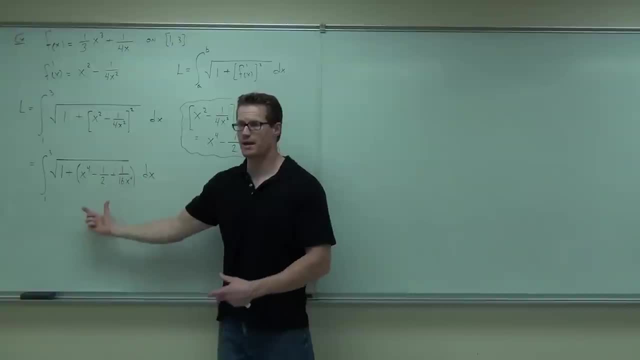 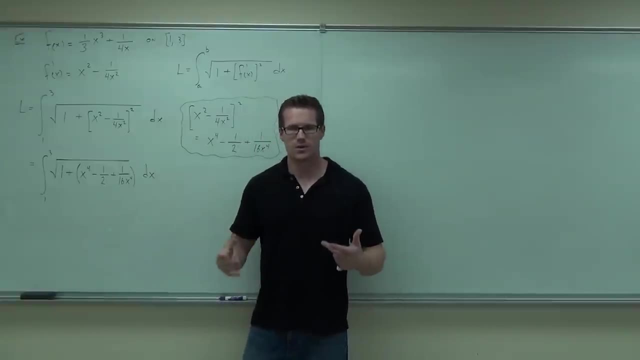 So that's Where that's coming from. We're just expanding that, Just squaring it, distributing, combining some like terms. You're gonna get this thing. Did you follow me on this so far? Now let's continue going. 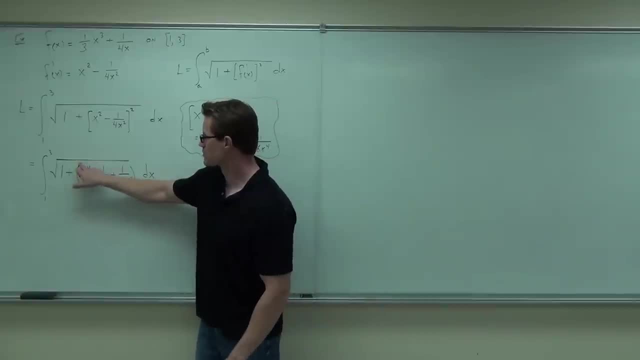 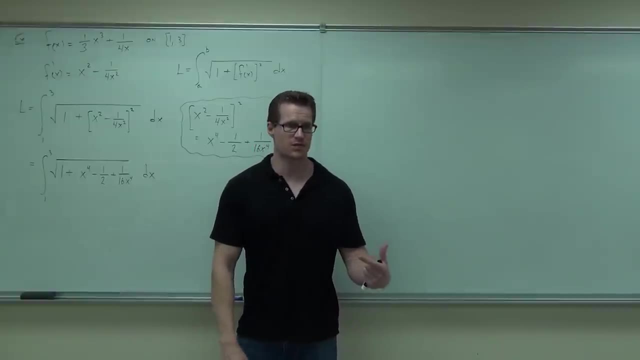 Let's get rid of some of those parentheses. We have one plus this. The parentheses really aren't doing much, Really aren't doing much there. If it was a minus, yes, it would change every sign, But with that plus, not so much. 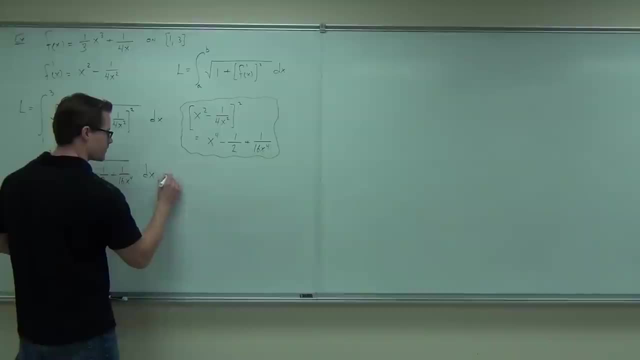 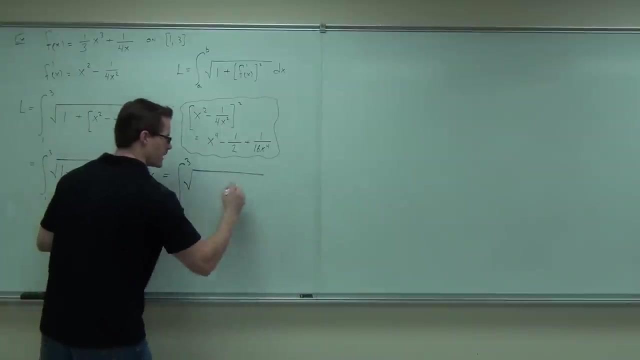 Let's continue rolling here. We'll still be going from one to three. We'll still have a square root and a dx Inside the square root. I'm gonna combine some like terms. I'm gonna have one minus one half is gonna give me one half. 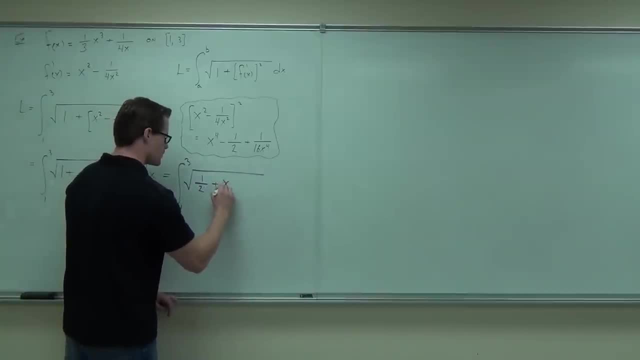 I'm gonna have x to the fourth And I'm gonna have one over 16. x to the fourth, dx Quick head nod, if you're okay, getting that far algebraically. Now, here's the deal. This thing right now, just kidding. 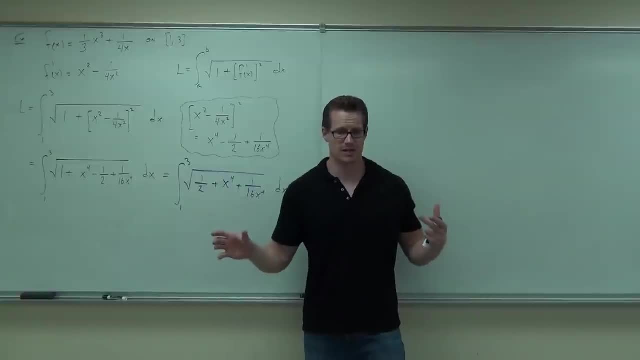 It's gonna probably hit these socks, But you can't split up square roots by addition, can you? So you can't just start taking square roots of things, can you? So, somehow, what you need to do any time you see these multiple terms in here. 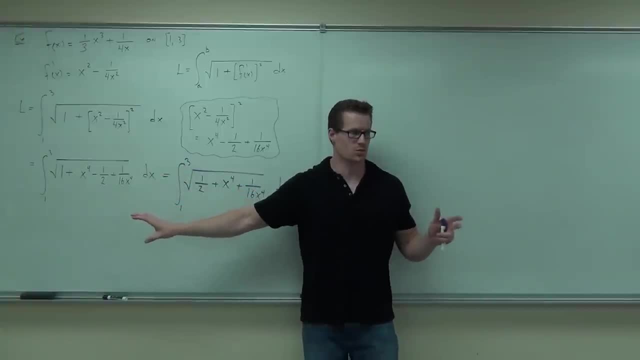 and there's no substitution. Notice there's no x's at all. No substitution's gonna work for you here. Combine everything, Combine it all And see if somehow you can manipulate the fact that a square root can be broken up across a quotient. to try to simplify this expression: 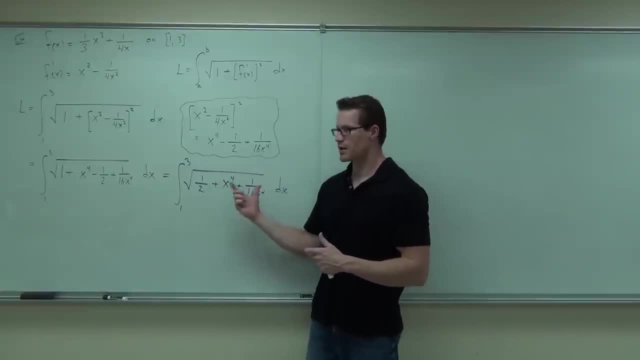 So, in other words, when we have these fractions and all these terms, you're gonna have to find a common denominator. You're gonna have to somehow put all of these things together and then see what you get. If it can be done, it will work out. 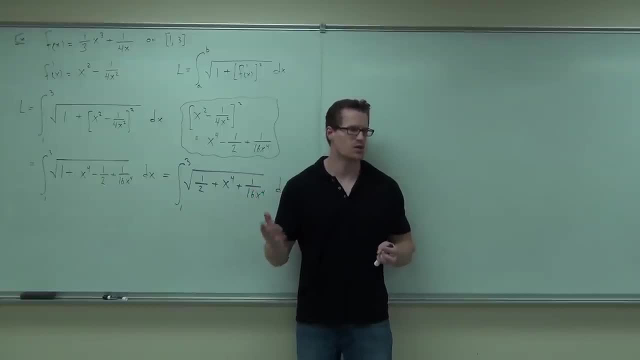 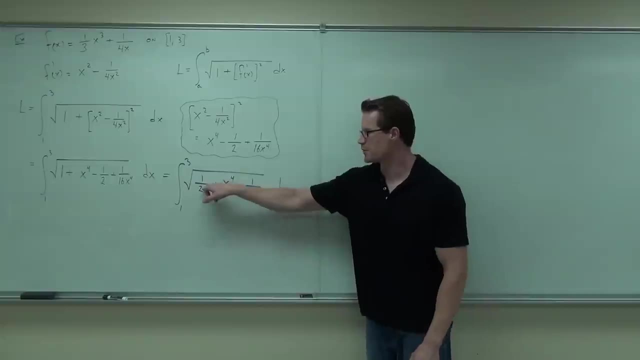 Okay, if it can be done, Some of them. I mean, if I had to give you just a random function, it's not gonna happen. These are very specific functions, So let's find a common denominator. What is your common denominator between? 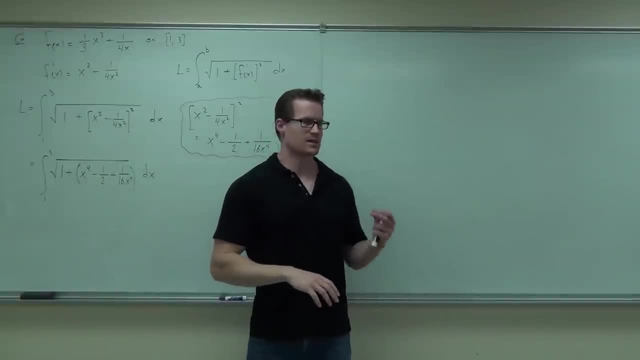 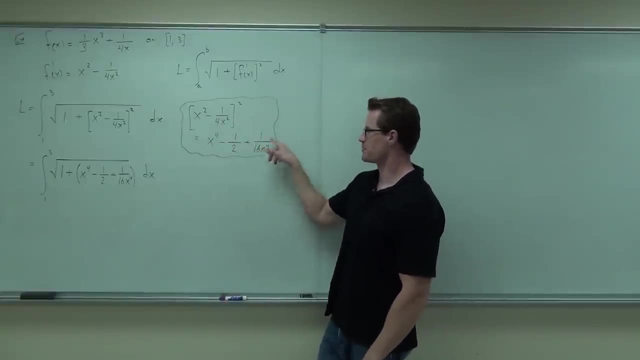 You can't do anything with that. You've got to completely break this thing down and see exactly what we can do. Can you follow me on that? So we square this. We get x to the 4th minus 1 half plus 1 over 16x to the 4th. 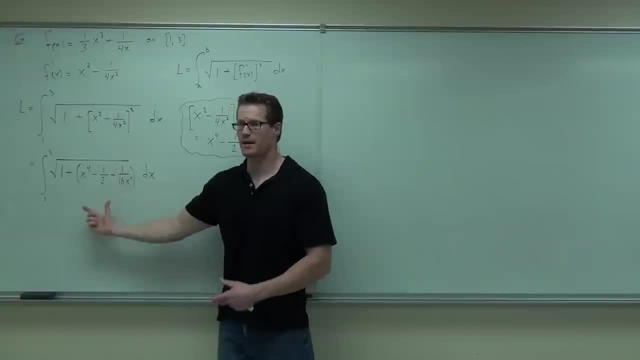 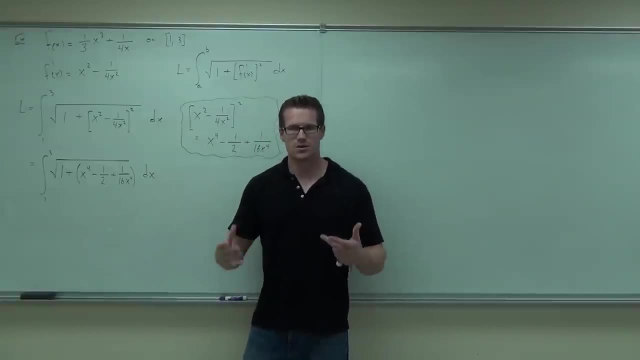 So that's where that's coming from. We're just expanding that, just squaring it, distributing, combining some like terms. You're going to get this thing. Can you follow me on this? so far, Now let's continue going. 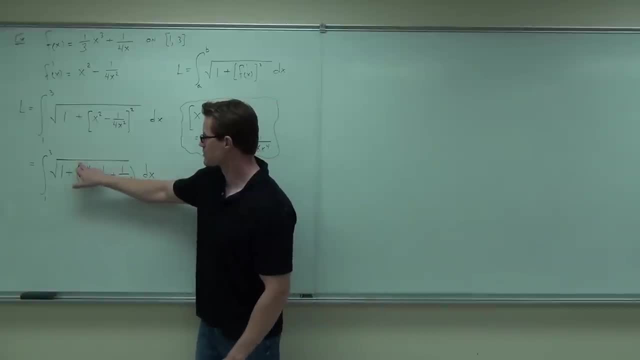 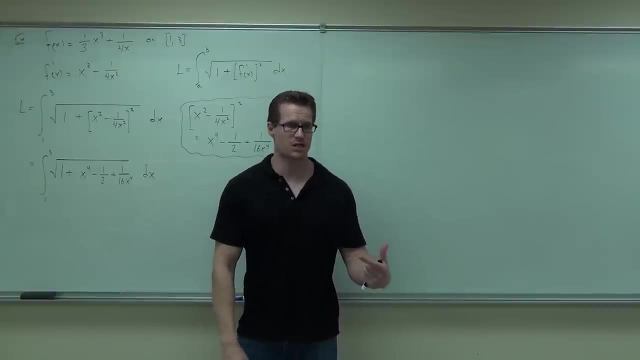 Let's get rid of some of those parentheses. We have 1 plus this. The parentheses really aren't doing much, Really aren't doing much there. If it was a minus, yes, it would change every sign, But with that plus, not so much. 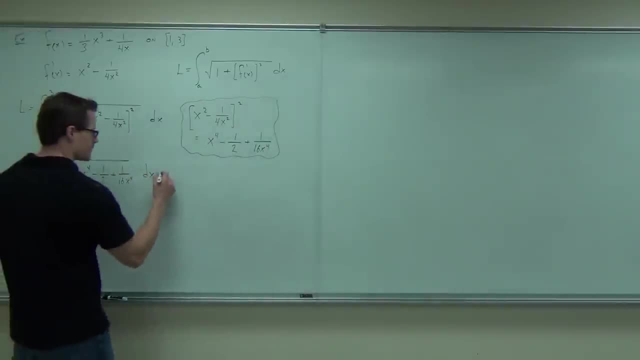 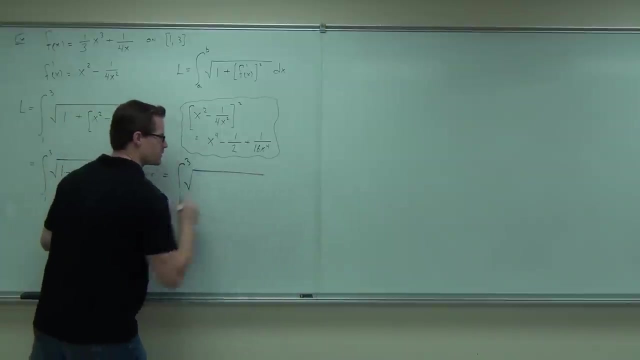 Let's continue rolling here. We'll still be going from 1 to 3.. We'll still have a square root and a dx Inside the square root. I'm going to combine some like terms. I'm going to have 1 minus 1 half is going to give me 1 half. 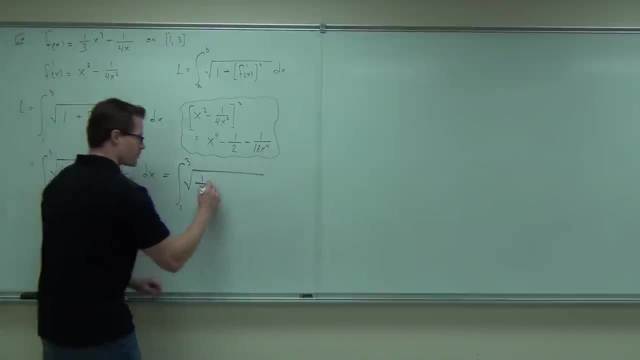 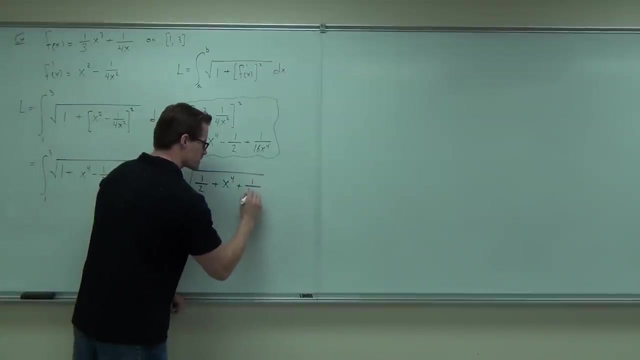 I'm going to have x to the 4th, I'm going to have x to the 4th, I'm going to have x to the 5th And I'm going to have 1 over 16. x to the 4th, dx. 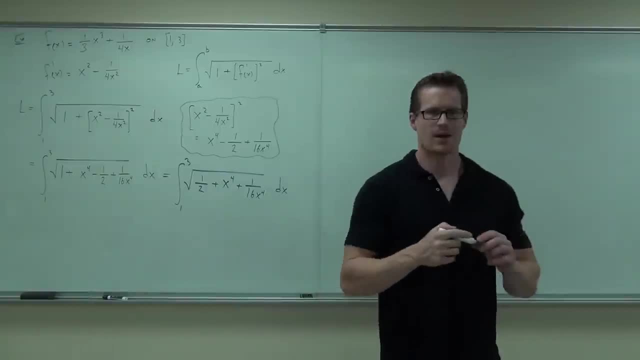 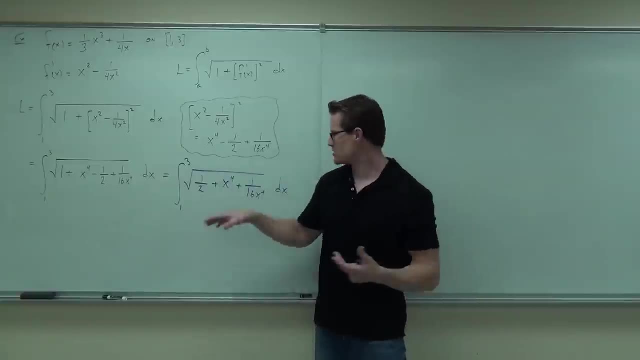 Quick head nod, if you're okay. getting that far algebraically. Now here's the deal. This thing right now just completely sucks. But you can't split up square roots by addition, can you? So you can't just start taking square roots of things, can you? 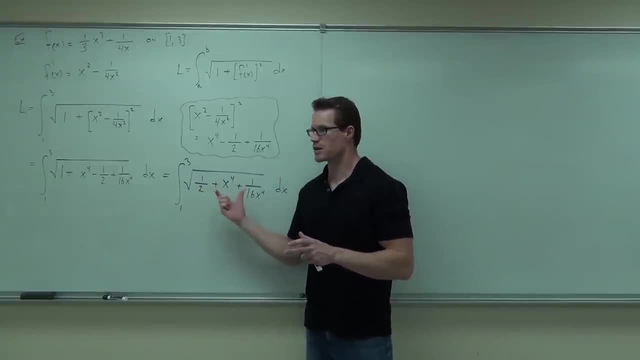 So somehow, what you need to do anytime you see these multiple terms in here- and there's no substitution notice, there's no x's at all. No substitution is going to work for you here- Combine them, Combine everything, Combine it all. 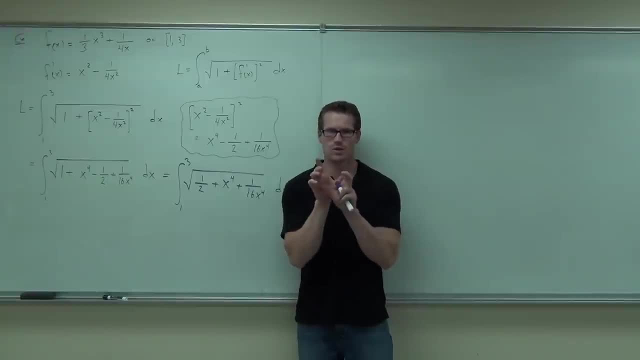 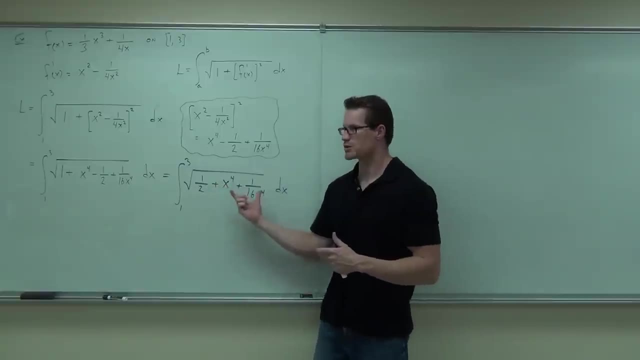 And see if somehow you can manipulate the fact that a square root can be broken up across a quotient to try to simplify this expression. So, in other words, when we have these fractions and all these terms, you're going to have to find a common denominator. 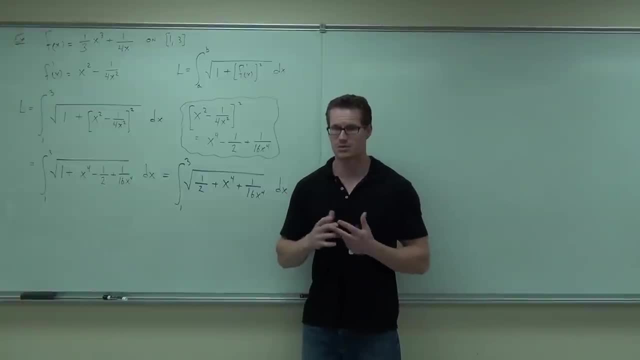 You're going to have to somehow put all of these things together and then see what you get. If it can be done, it will work out. Okay, If it can be done Some of them, I mean, if I had to give you just a random function, it's not going to happen. 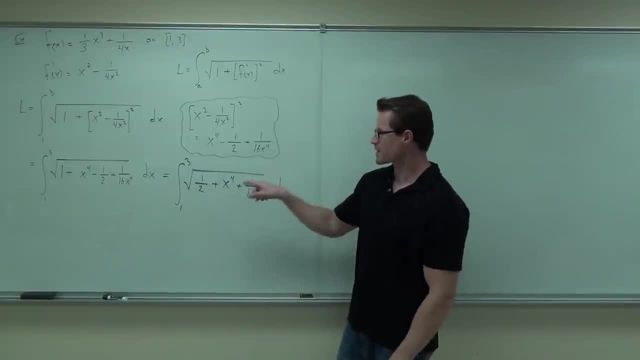 These are very specific functions, So let's find a common denominator. What is your common denominator between 1 half x to the 4th and 1 over 16x to the 4th, 16x to the 4th? 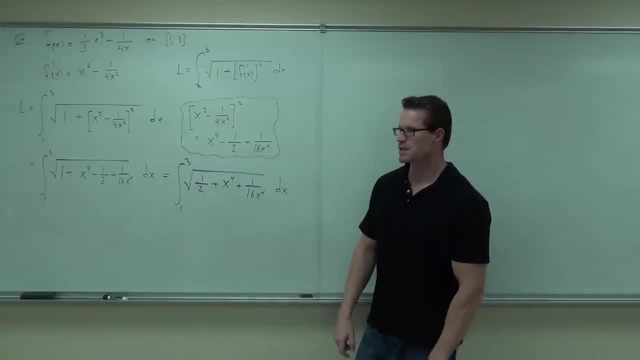 one half x to the fourth and one over 16 x to the fourth, 16 x to the fourth. Very good, So we're gonna go ahead and make all these fractions equivalent, but have the denominator of 16 x to the fourth. 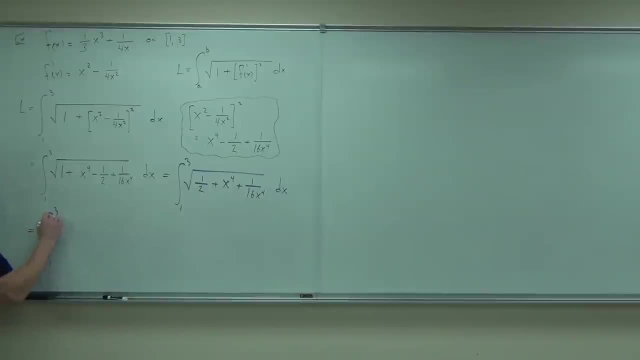 What that means is we're gonna get- let's go careful on this thing. One half is the same thing as eight x to the fourth, over 16 x to the fourth. One half is this? Do you believe me? I hope so. I'm the teacher. 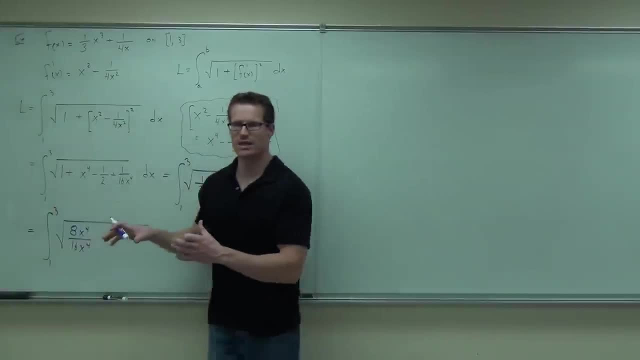 You shouldn't believe me, Although maybe I've lost your trust. Are you guys okay giving the one half to the eight, x to the fourth, over 16 x to the fourth? See, it is one half right. In other words, we're just multiplying. 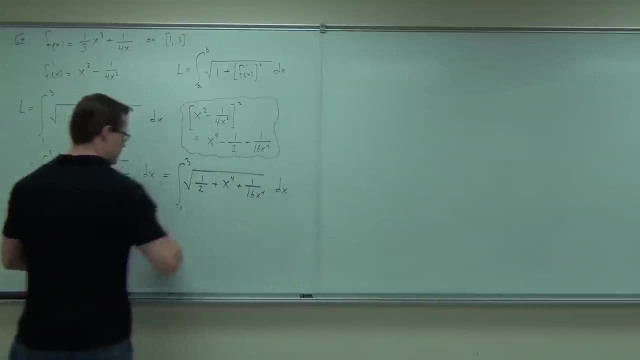 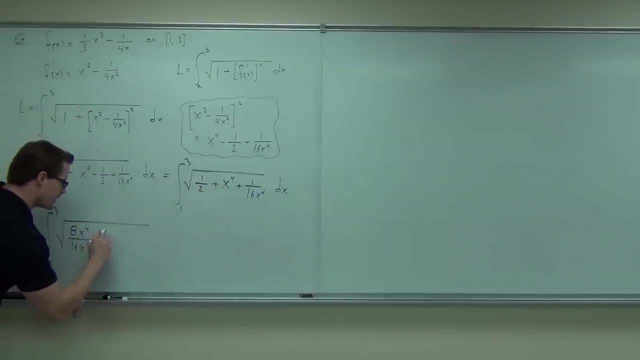 by eight x to the fourth over eight x to the fourth, That's it. Plus this thing, x to the fourth is the same thing as 16 x to the eighth. over 16 x to the fourth, That still equals x to the fourth. 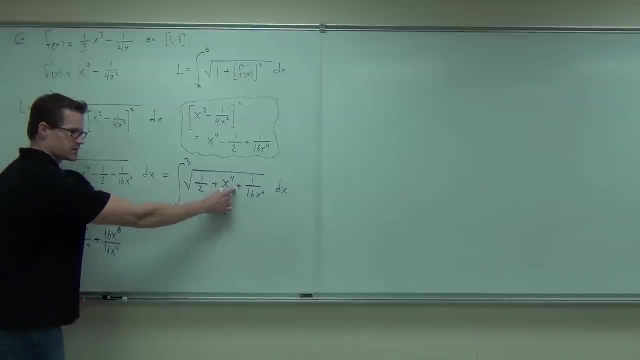 So that's an equivalent expression as well. This is this Plus nothing I need to do there. It's already the denominator that I want: One over 16 x to the fourth. Tie it all up with a bx And switch some pen, so we get a different step here. 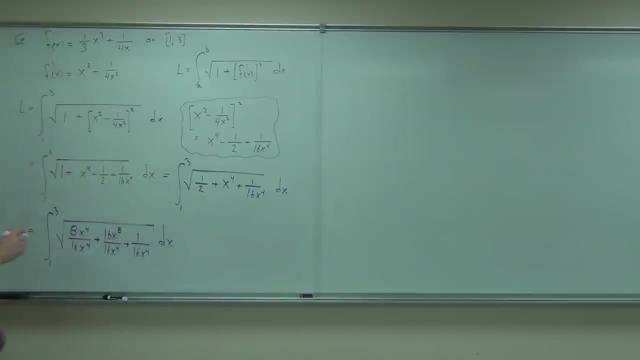 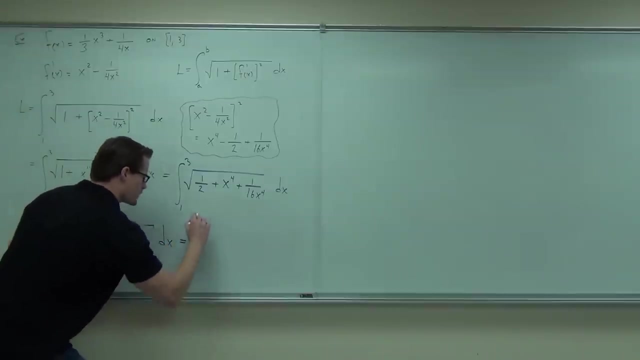 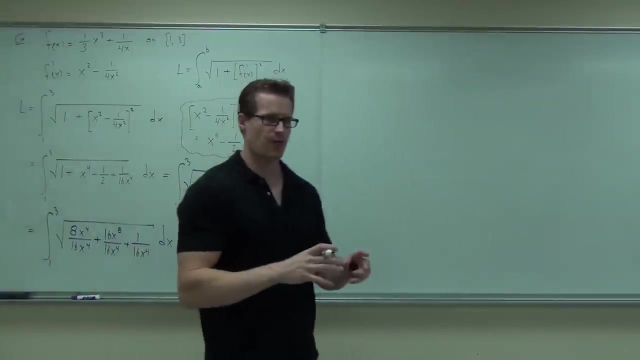 So that's the integral from one to three Big square root. Check out what happens Now that I have that common denominator. I can make everything as one fraction with the denominator of 16, x to the fourth on the bottom of a fraction. 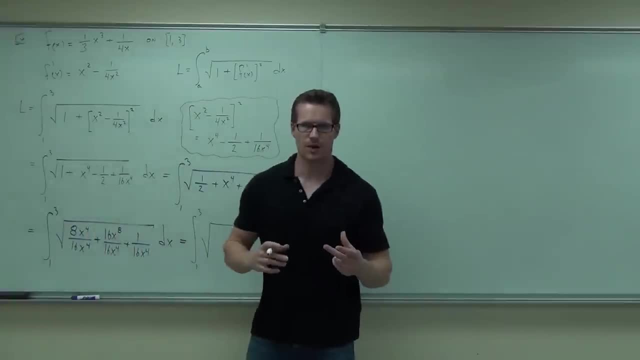 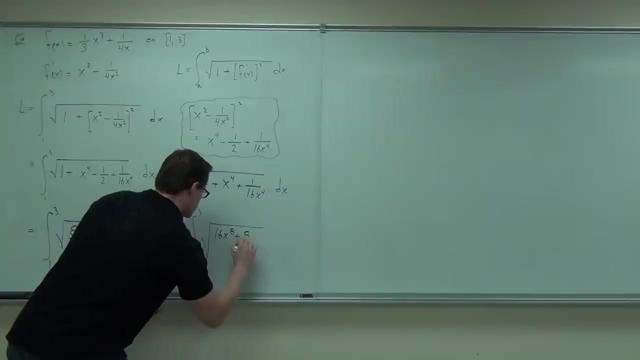 Also, I'm going to choose to write these in a different order. I'm going to write the 16 x to the eighth, then the eight x to the fourth and then the one. Are you guys okay with that? All algebra right now. 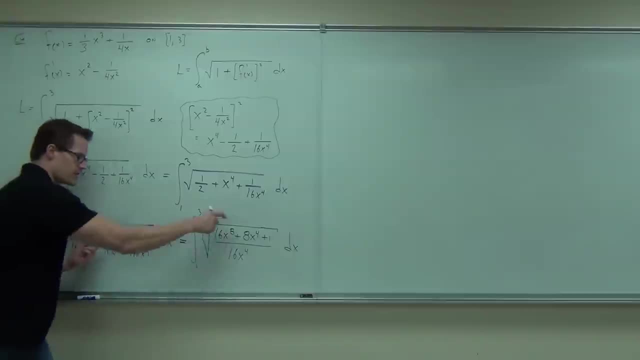 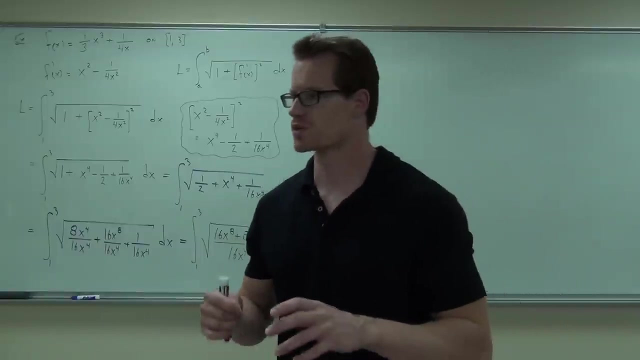 All algebra, 16 x to the eighth, Eight x to the fourth. yes Plus one yes. All over our common denominator, We're good to go, Do you feel okay with it? so far, Now, I told you this is kind of a special function because when you look at it, notice how. now 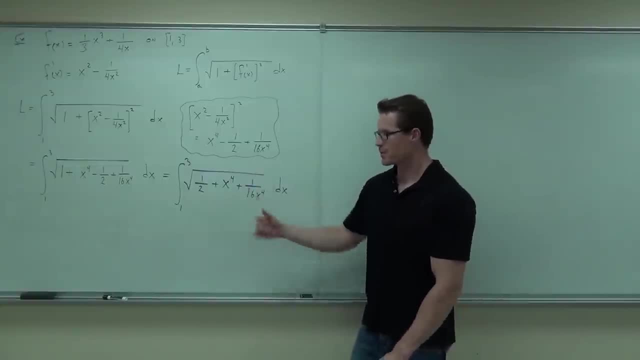 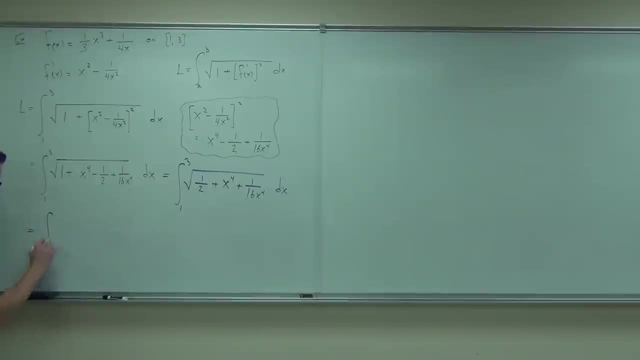 Very good. So we're going to go ahead and make all these fractions equivalent, but have the denominator of 16x to the 4th. What that means is we're going to get- let's go careful on this thing- One half is the same thing as 8x to the 4th over 16x to the 4th. 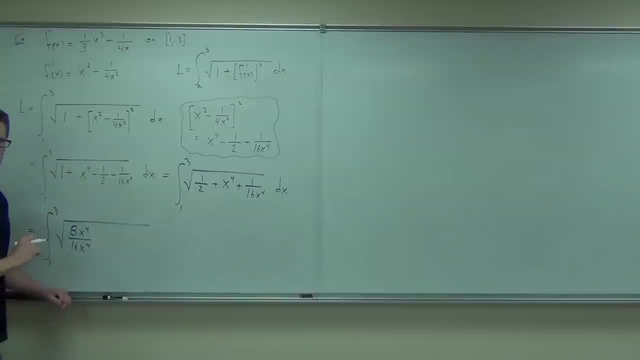 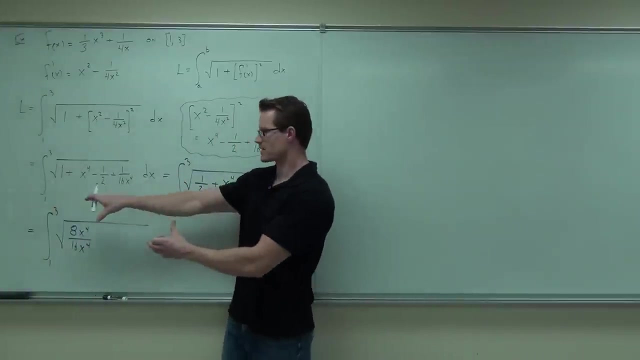 One half is this: Do you believe me? I hope so. I'm the teacher. You shouldn't believe me, Although maybe I've lost your trust. Are you guys okay giving the 1 half to the 8x to the 4th over 16x to the 4th? 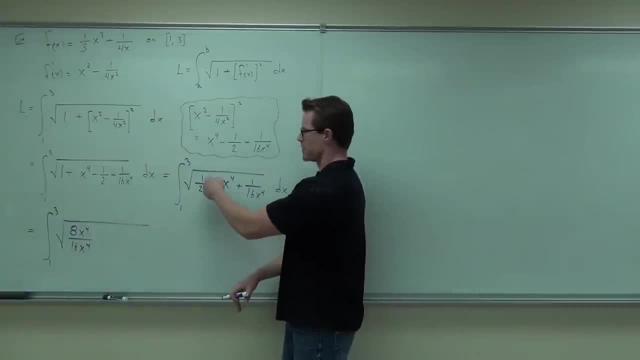 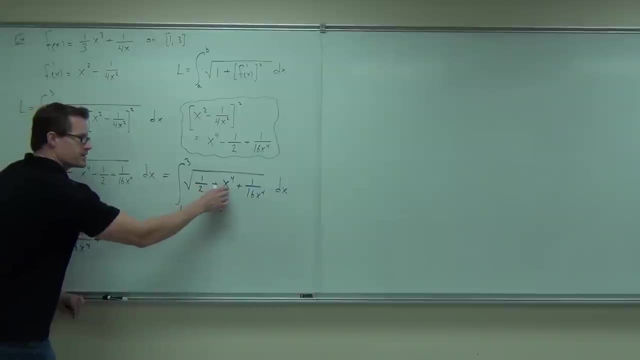 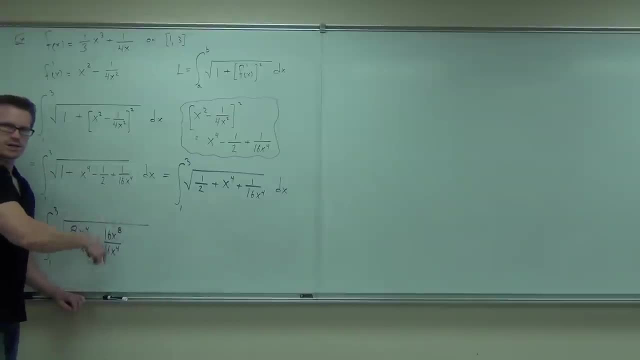 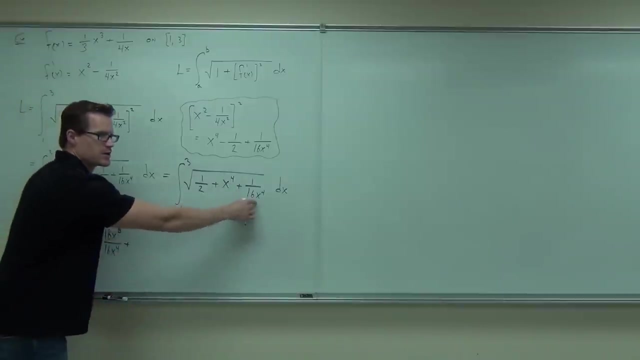 x to the 4th, That still equals x to the 4th, So that's an equivalent expression as well. This is this Plus nothing I need to do there. It's already the denominator that I want: 1 over 16x to the 4th. 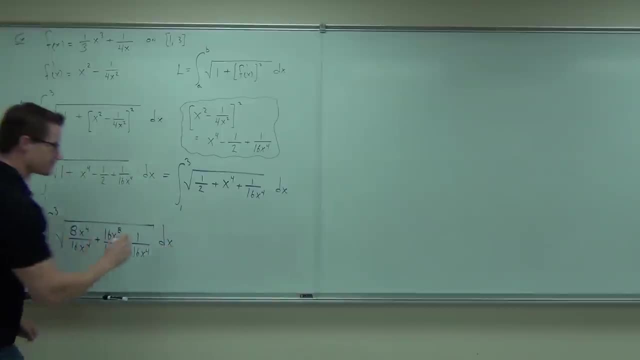 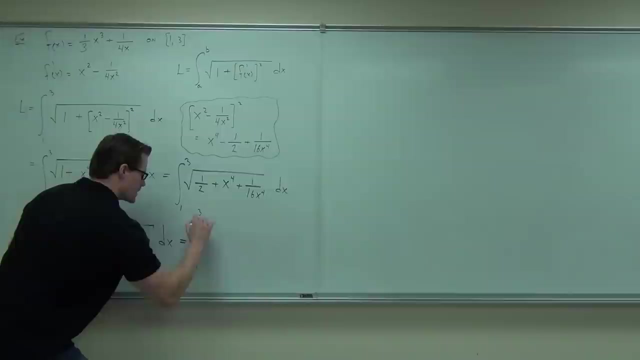 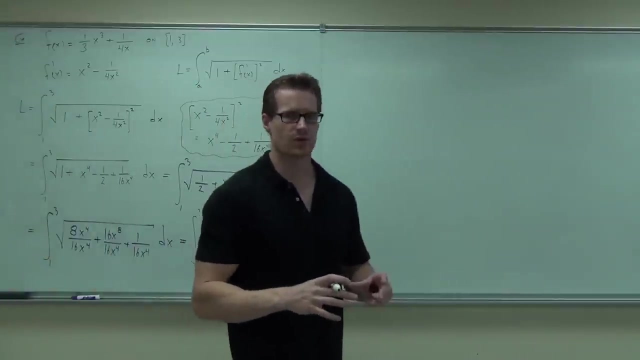 Tie it all up with a dx And switch some pens, so we get a different step here. So that's the integral from 1 to 3.. Big square root: Check out what happened. Now that I have that common denominator, I can make everything as one fraction with. 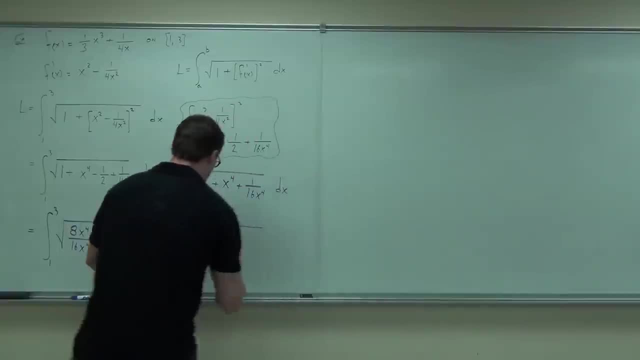 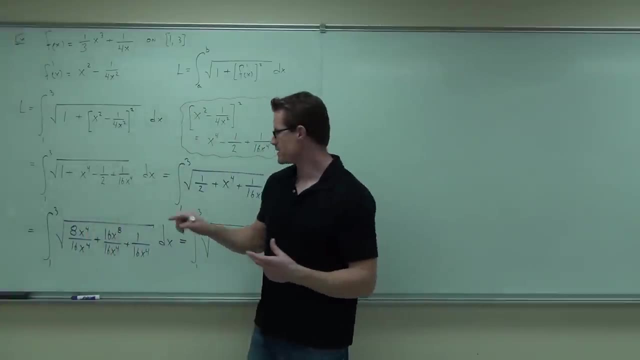 the denominator of 16x to the 4th on the bottom of our fraction. Also, I'm going to choose to write these in a different order. I'm going to write the 16x to the 8th, then the 8x to the 4th and then the 1.. 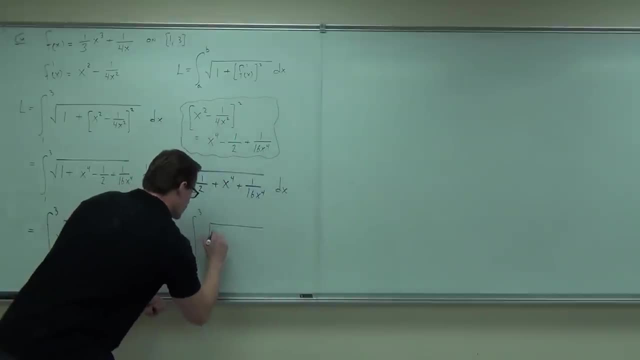 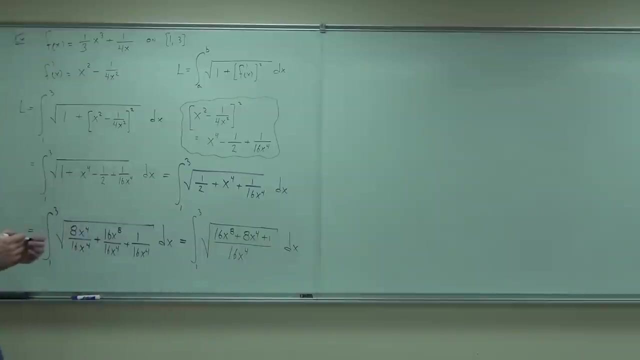 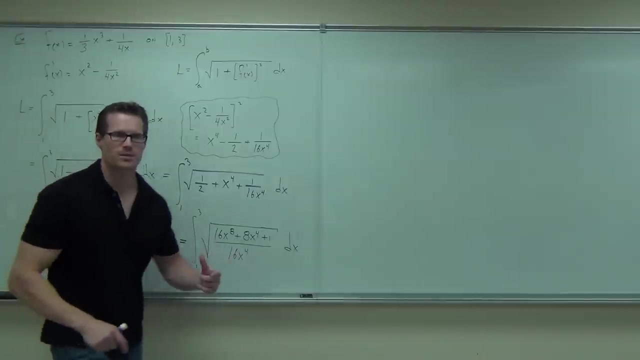 Are you guys okay with that? All algebra right now. All algebra, 16x to the 8th, 8x to the 4th. Yes Plus 1.. Yes, All over our common denominator, We're good to go. 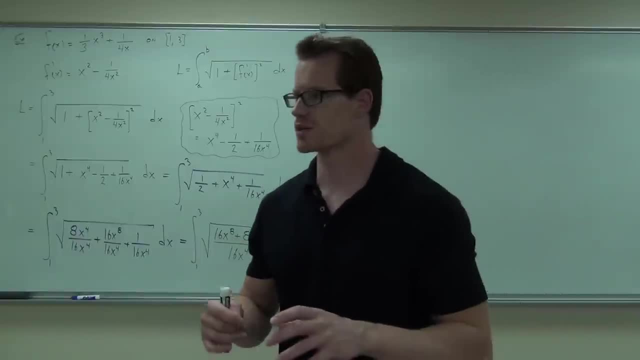 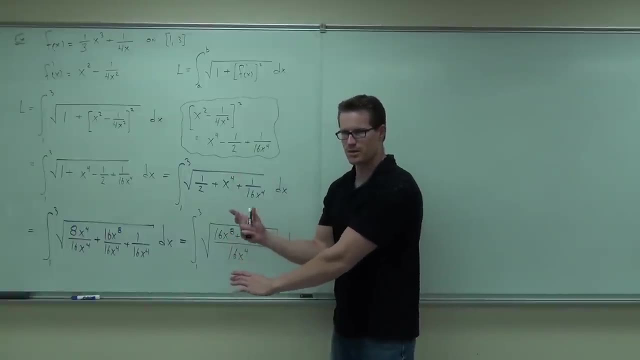 Do you feel okay with it so far? Now I told you this is kind of a special function because when you look at it, notice how now I can break up my square root by the numerator and the denominator. So I'm going to move up here. 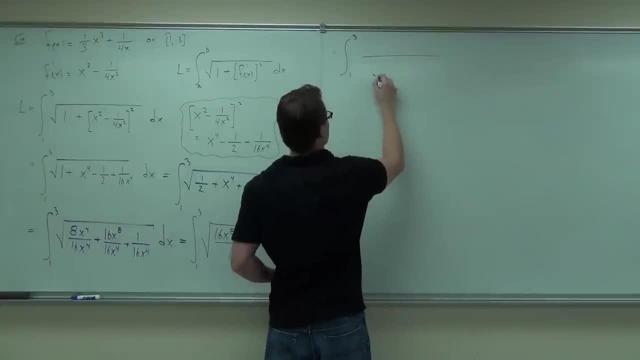 So that's 1 to 3. Square root of 16x to the 4th, that's a denominator, sure, And also the square root of 16x to the 8th plus 8x to the 4th plus 1.. 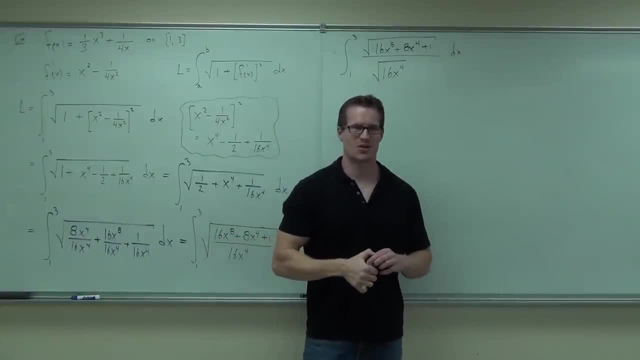 You didn't know there was going to be so much algebra in this stuff, did you? I expected hard integrals. They're not hard integrals, They're hard algebra. to get to an integral, You get to an integral. You get to an integral. 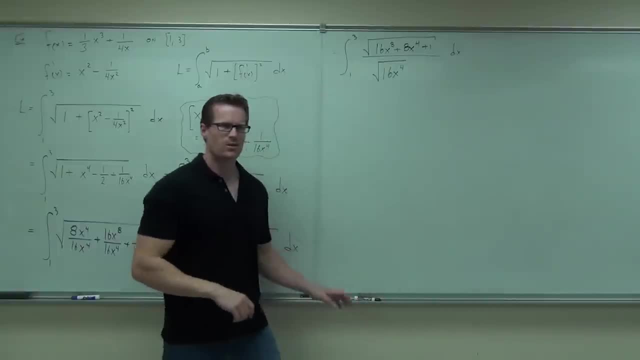 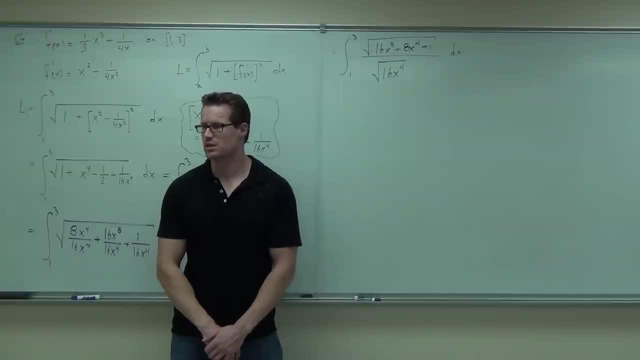 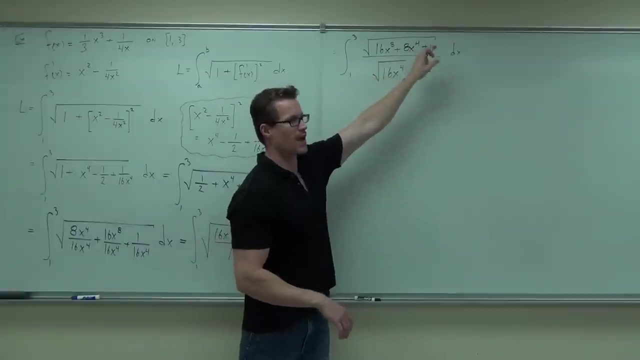 Denominator, It does. Yeah, what's the square root of 16?? Cool, x to the what? now, Good, because you have a power of 1 half Numbers to the- excuse me- x once you multiply. So you have a like to the 4th to the 1 half, or a square root of x to the 4th, either. 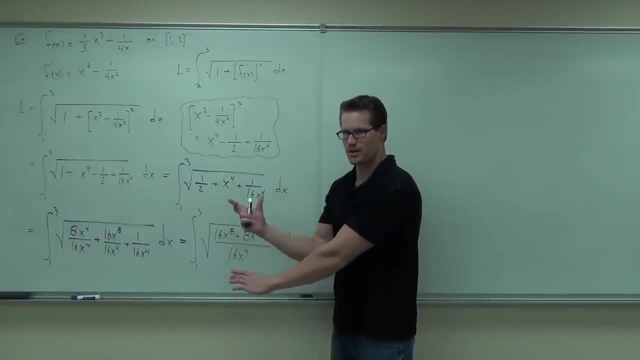 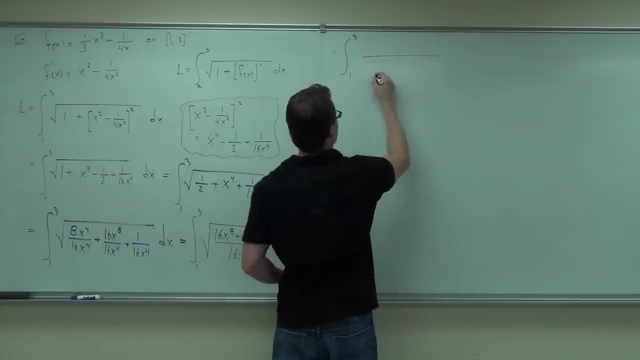 I can break up my square root by the numerator and the denominator, So I'm going to move up here. That's one to three, Square root of 16 x to the fourth. that's a denominator, sure, And also the square root of 16 x to the eighth. 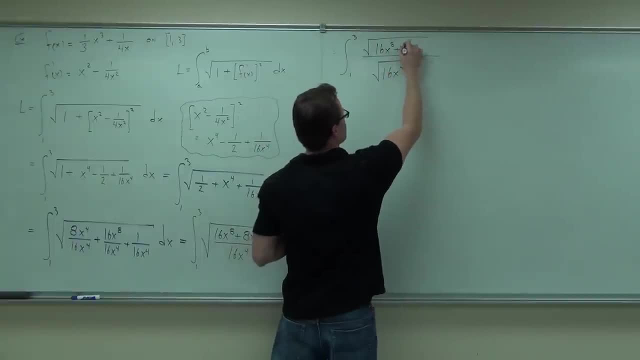 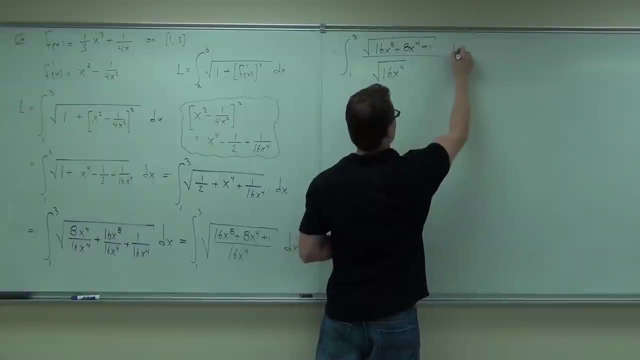 Okay, 16 x to the eighth Plus eight x to the fourth plus one. You didn't know there was going to be so much algebra in this stuff. did you Expected hard integrals? They're not hard integrals, They're hard algebra to get to an integral you can actually do. 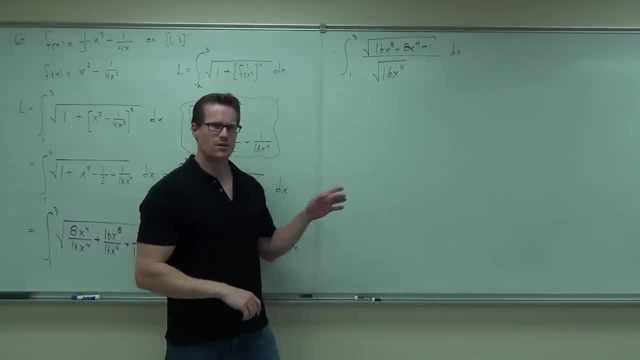 It's different, Weird. Do you feel still all right with getting that far? Tell me some cool things that happen specifically with the denominator, Denominator, Square root of what It does. Yeah, What's the square root of 16?? 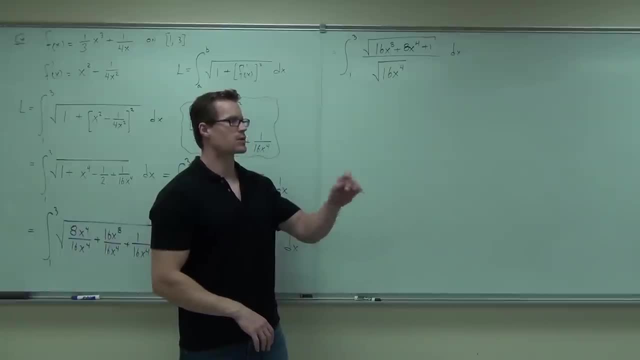 Four Square Cool. X to the what now Square? Good, Because you have a power of one half Numbers to the- Excuse me- X once you multiply. So you have to the fourth to the one half, or a square root of x to the fourth. 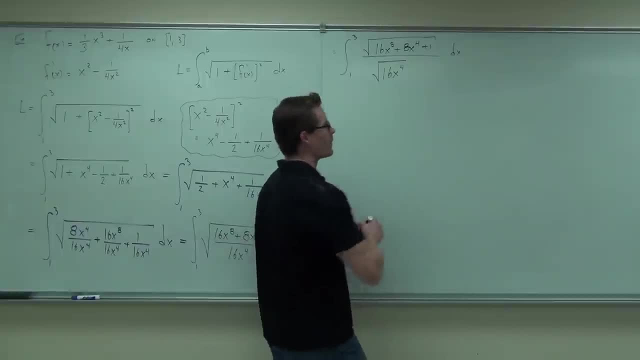 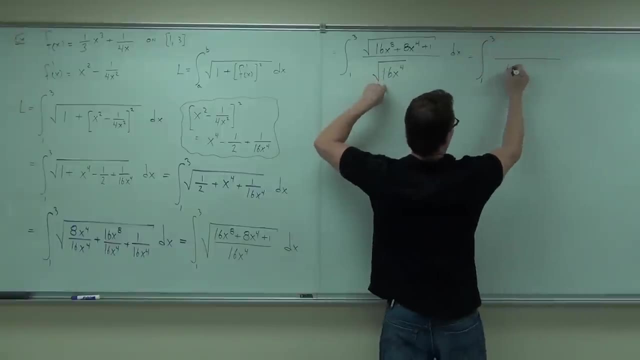 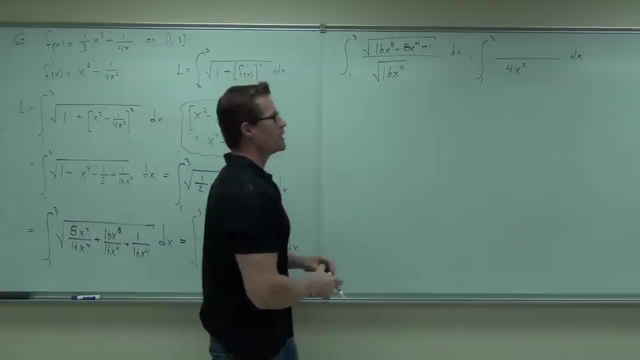 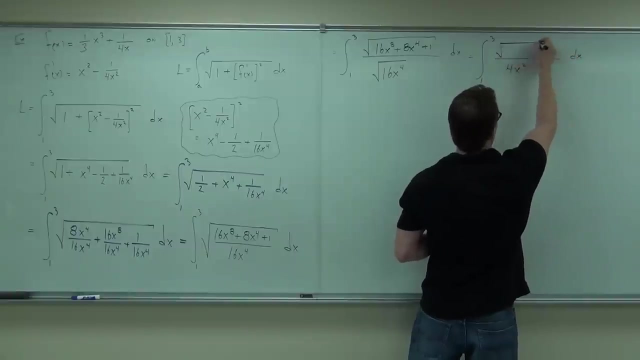 Either way, you're going to get x squared out of that. So, denominator, not bad at all. Four Square root of x squared dx. Very cool. Let's work a little bit more on the numerator In order for this to work out nicely for us. something has to happen. 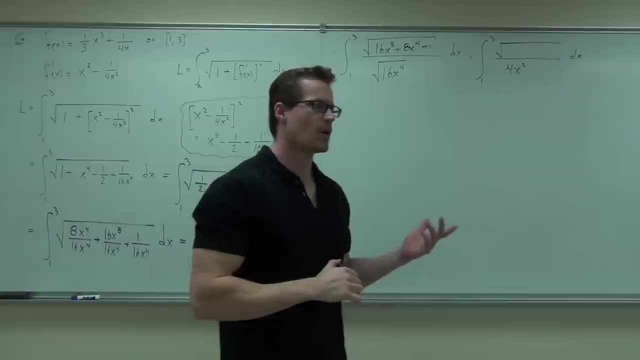 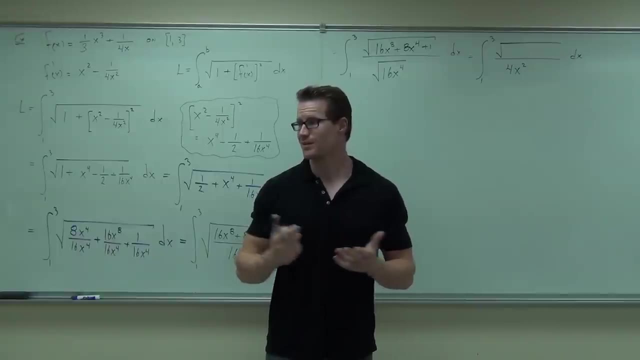 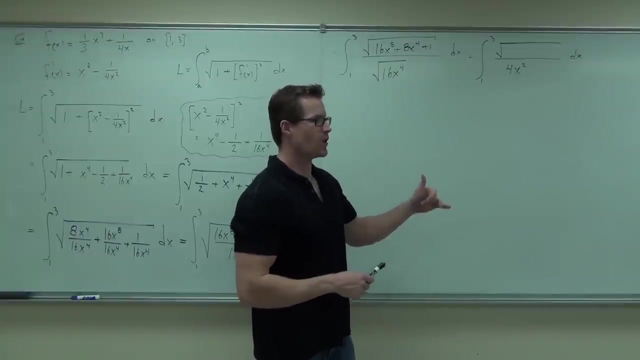 We either have to have a substitution that's present, have to- or we need to create some sort of a square. Why square? Yeah, So the square root will actually work here. Now, when you look at that- 16x to the eighth plus 8x to the fourth plus one- it might not. 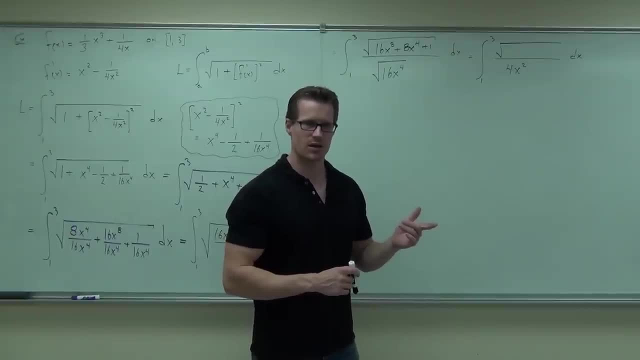 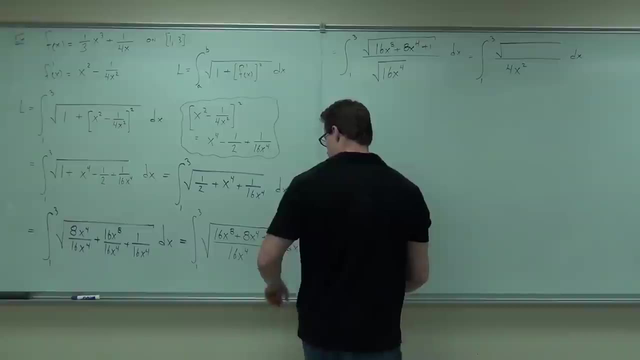 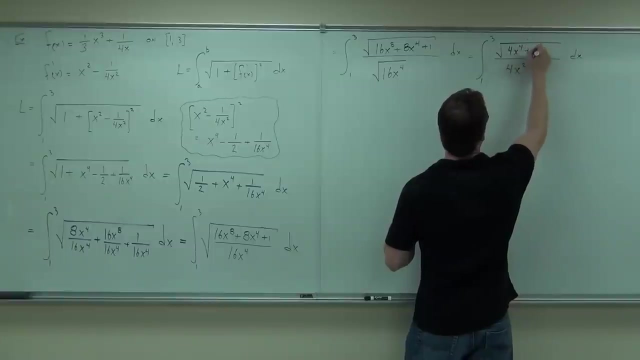 be easy to see, but that's a perfect square. Do you guys see the perfect square out of that? Yeah, That is a 4x to the fourth Plus one Plus one Square. 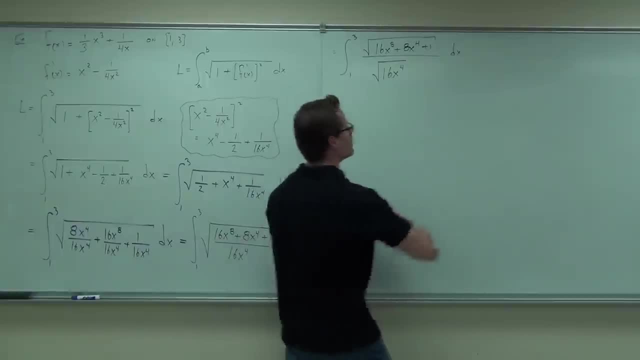 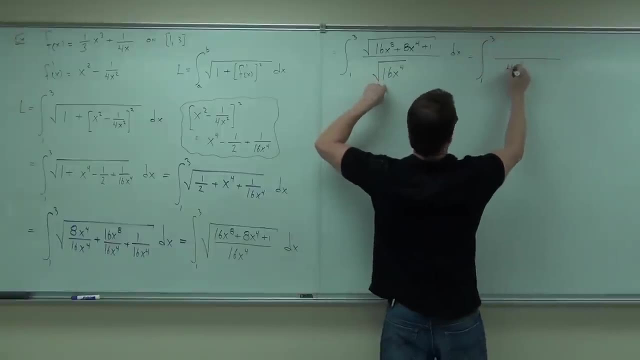 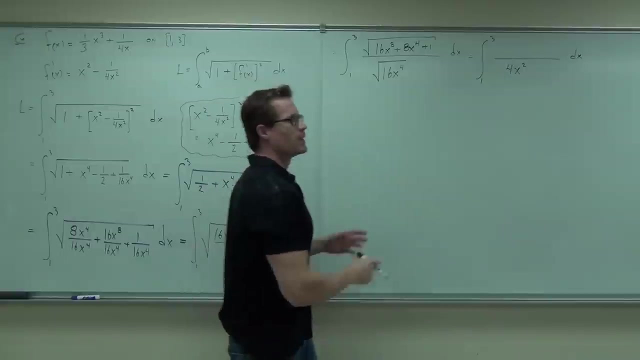 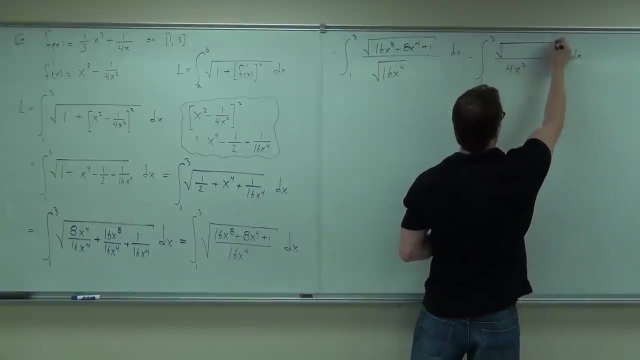 way you're going to get x squared out of that. So, denominator, not bad at all. 4x squared dx: very cool. Let's work a little bit more on the numerator In order for this to work out nicely for us. something has to happen. 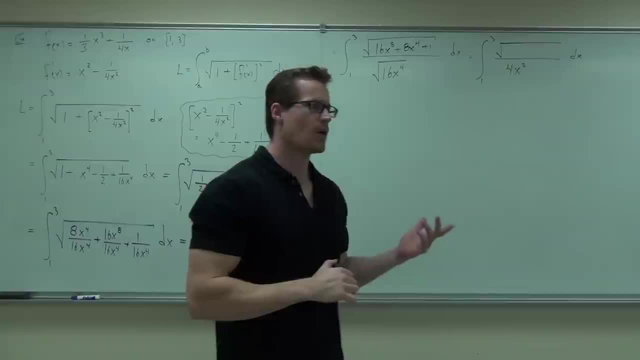 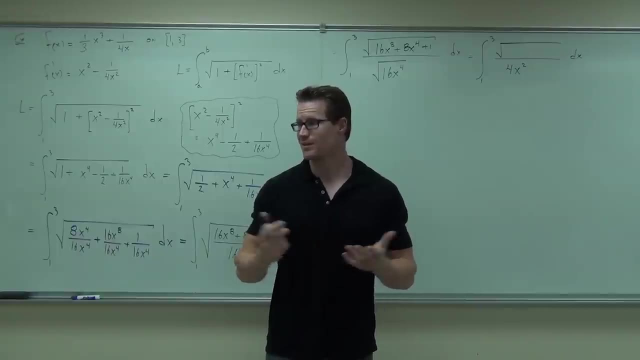 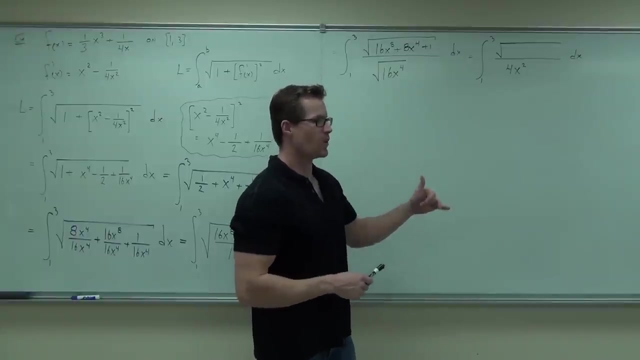 We either have to have a substitute- We have to have a substitution that's present, have to- or we need to create some sort of a square. Why square? Yeah, so the square root will actually work here. Now, when you look at that- 16x to the 8th plus 8x to the 4th plus 1, it might not be. 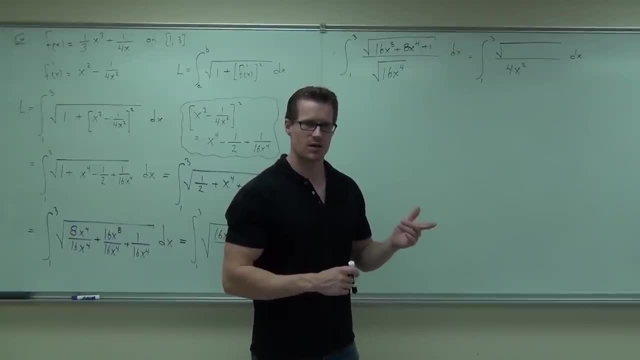 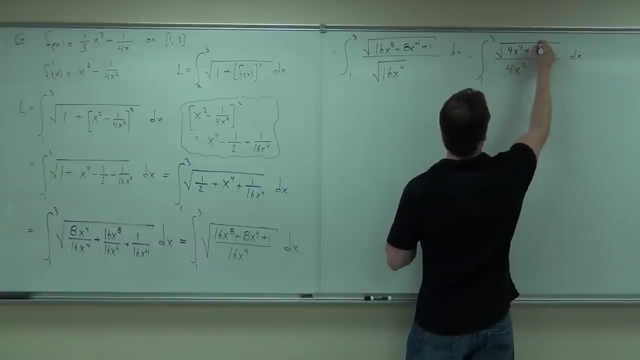 easy to see, but that's a perfect square. Do you guys see the perfect square out of that? That is a 4x to the 4th plus 1 squared. 4x to the 4th plus 1 squared. let's verify that just for a second. 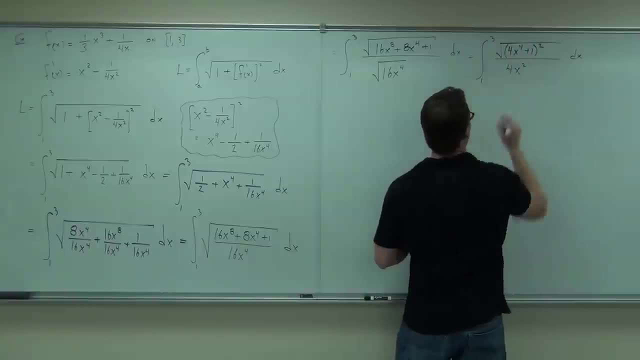 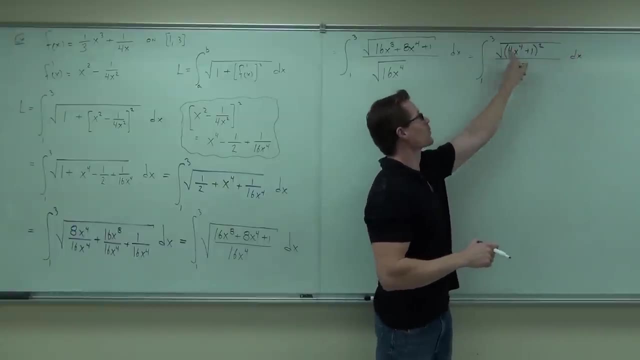 4x to the fourth Plus one Square. Let's verify that. just for a second. 4x to the fourth times 4x to the fourth is 16x to the eighth. Great, We're going to have two 4x to the fourths. 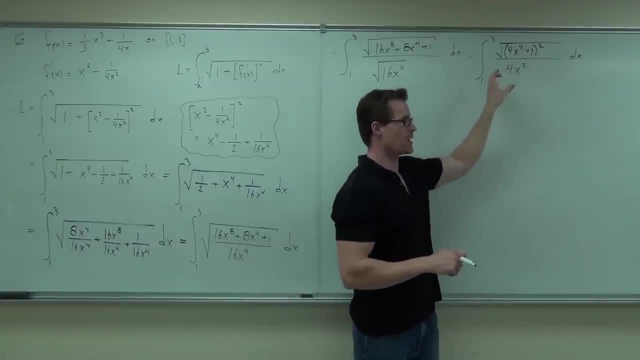 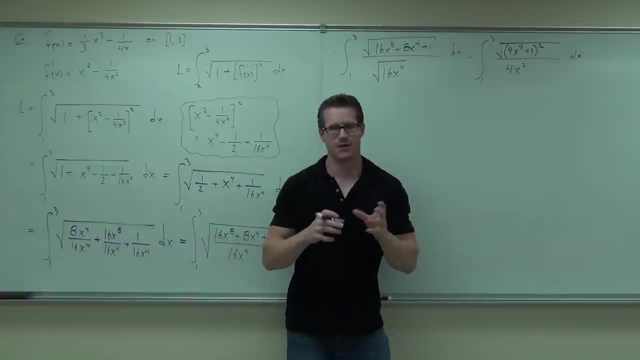 That's 8x to the fourth and then a plus one on the back end. So that's the appropriate factorization. If you wanted to, you could make a substitution for x to the fourth equals y and substitute it that way, And then the factorization becomes a little bit easier, since you don't have those eighth. 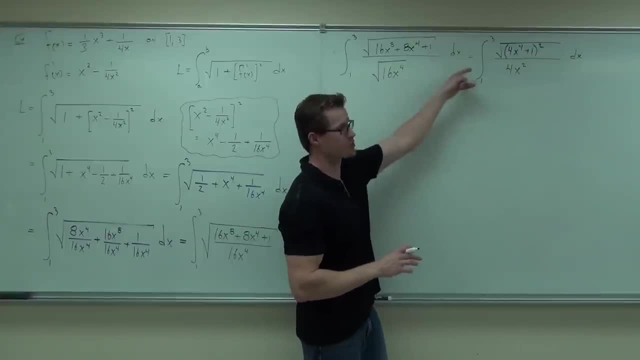 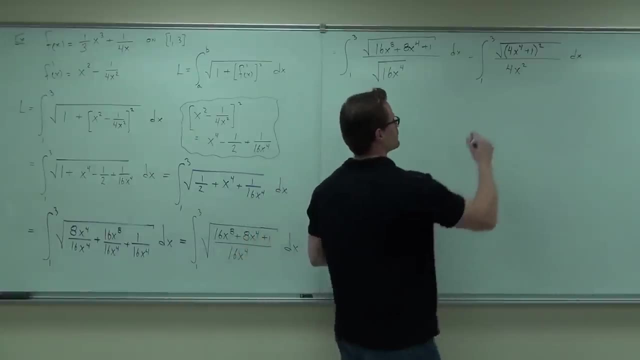 powers and fourth powers. It's a little bit hard to think of, But that's certainly the appropriate factorization. Why is that so important for us to do? It's not a square root. it's not a square root. Exactly That has to happen. has to happen. 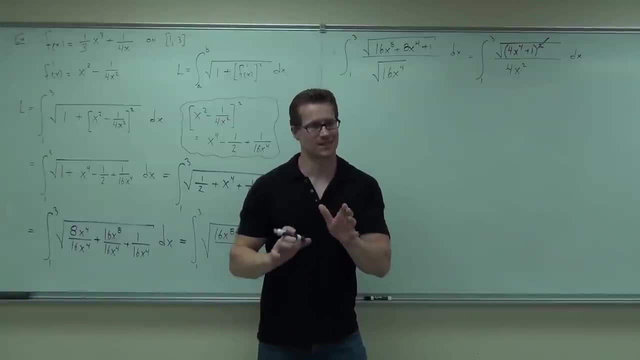 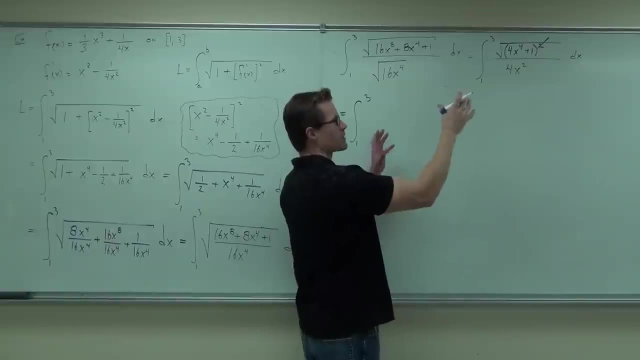 or you've got to be able to find a substitution for that to work, Otherwise you're going to be kind of stuck. So square and square root. those are inverse operations. Those things are gone. We have 4x to the fourth plus 1 over 4x squared. 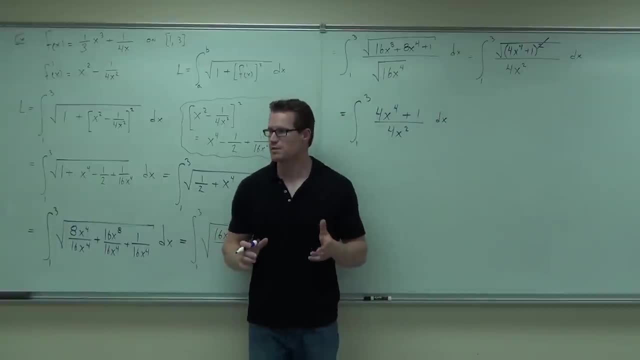 Yes, Hey, we're almost home free. We've got something that looks really nice. What now? You could, you could. I'm going to do it a little different way, but you could do that. What if you did that? though, notice you have parenthesis times 4x squared, sorry. 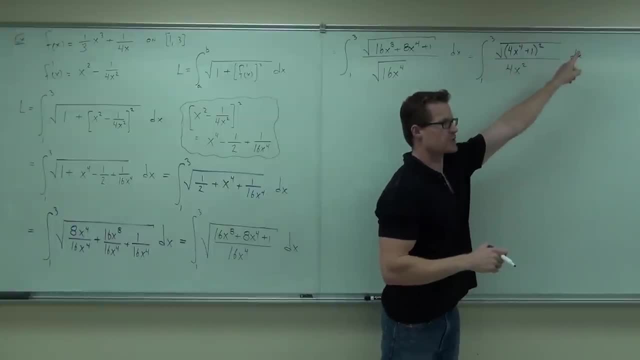 4x to the 4th times 4x to the 4th is 16x to the 8th. Great, We're going to have 2, 4x to the 4th, so that's 8x to the 4th, and then the plus 1 on the. 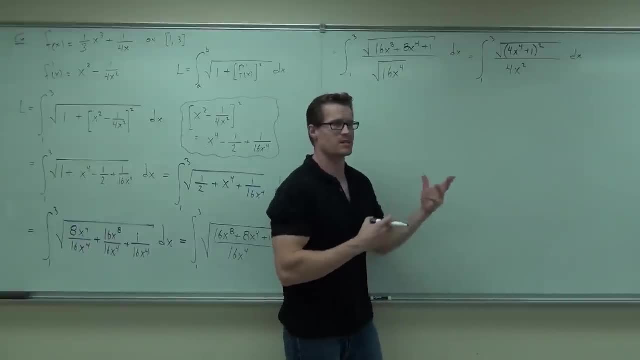 back end. So that's the appropriate factorization. If you wanted to, you could make a substitution for x to the 4th equals y and substitute it that way, And then the factorization becomes a little bit easier. Since you don't have those 8th powers and 4th powers, it's a little bit hard to think. 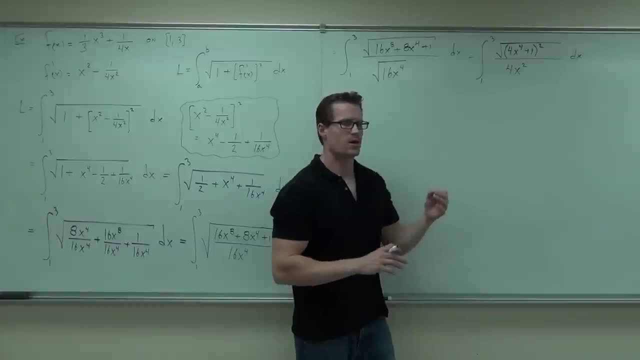 of, but that's certainly the appropriate factorization. Why is that so important for us to do? It's kind of square root. Exactly That has to happen. has to happen or you've got to be able to find a substitution for. 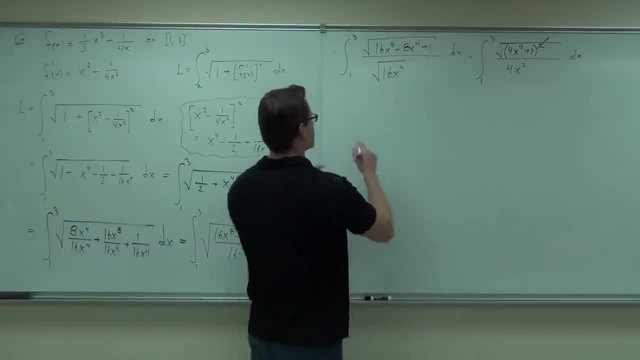 that to work, Otherwise you're going to be kind of stuck. So square and square root, those are inverse operations. Those things are gone. We have 4x to the 4th plus 1 over 4x squared dx. 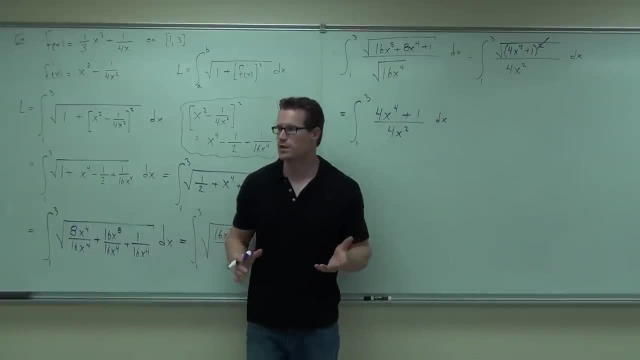 Hey, we're almost home free. We've got something that looks really nice. What now? You could, You could. I'm going to do it a little different way, but you could do that. If you did that, though, notice you have parentheses, times, 4x squared. sorry, you have 1, 4th and. 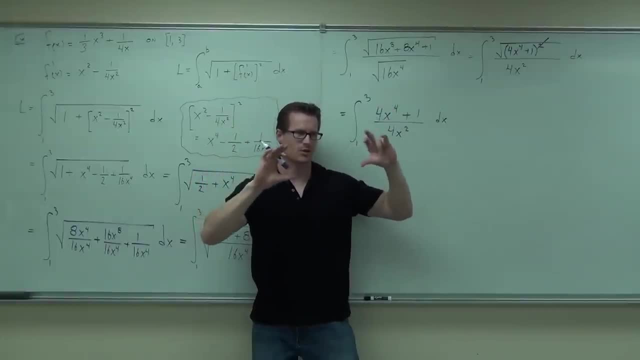 you have 1 fourth and then x to the negative 2. So you'd have something a little bit awkward to deal with. Other ideas: Split it up. Split it up, probably, Substitution. No, No, don't do substitution unless you absolutely need it. 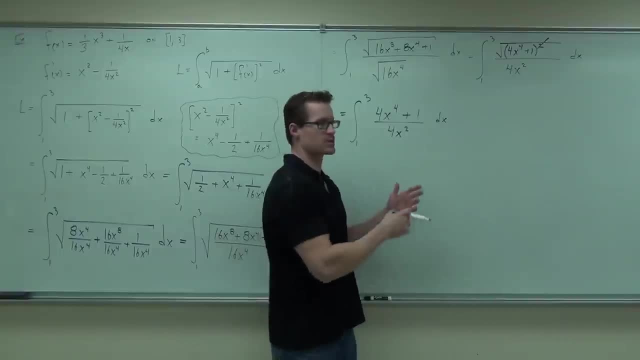 You don't have to Split things up if it's easy to do so. So here, yes, split it up. Remember these: when I gave them to you, Like the first first time we ever dealt with integrals, I gave you something that looked like that: 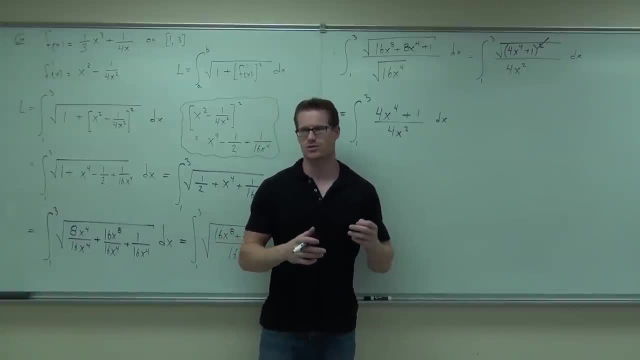 It had t, though It was like a t cubed plus 1 over t squared or something I said: think a little bit more about these things, Split them up when you can, because if you have like variables, you can combine those things. 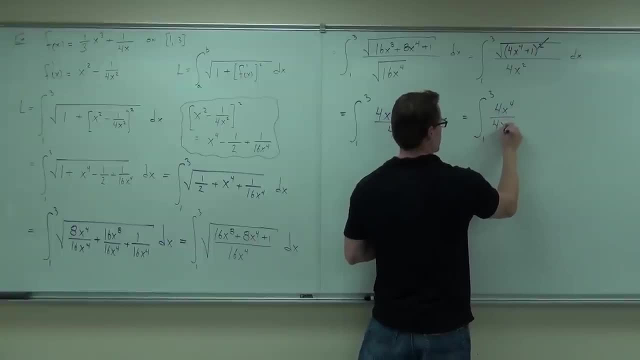 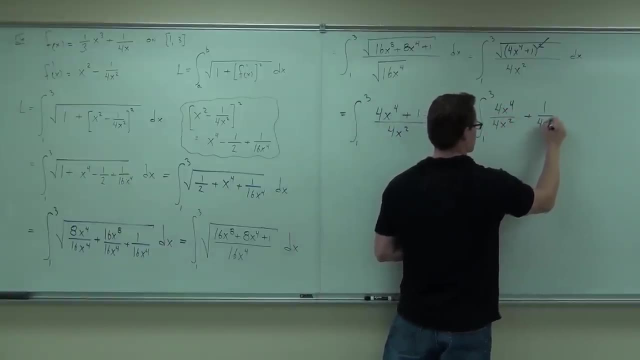 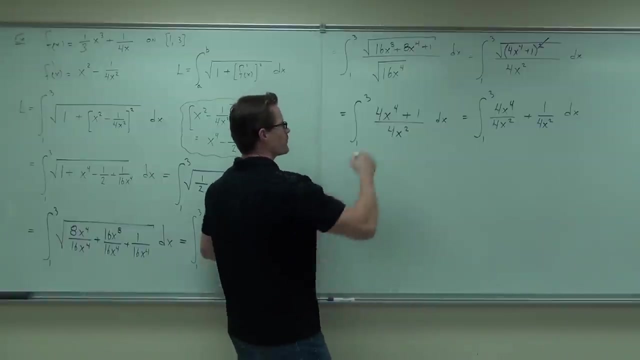 So 4x to the fourth over 4x squared. Yes, Plus that. So let's simplify them a little bit. We've got 4x to the fourth over 4x squared. That's going to give you x squared. 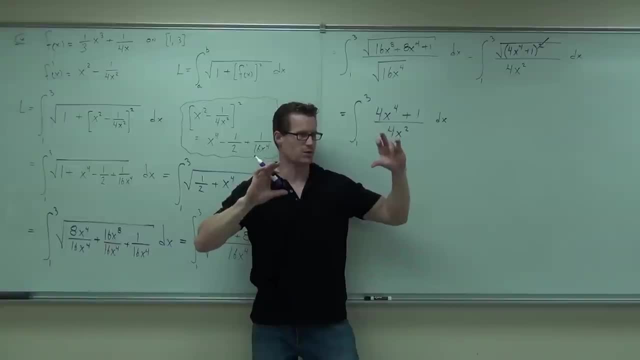 then x to the negative 2. So you'd have something a little bit awkward to deal with. I don't know Any other ideas. Split it up. Split it up, Probably. Substitution. No, No, don't do a substitution unless you absolutely have to. 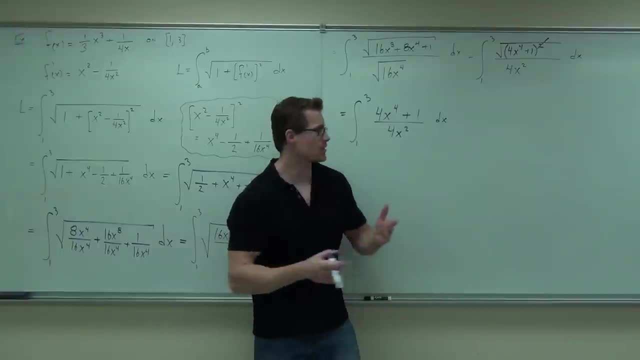 Split things up if it's easy to do so. So here, yes, split it up. Remember these: when I gave them to you The first time we ever dealt with integrals, I gave you something that looked like that. It had t, though. 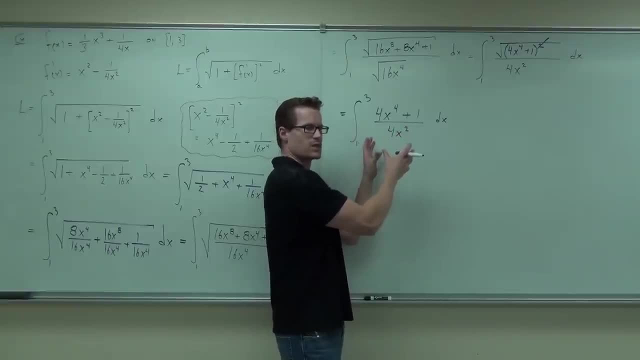 It was like t cubed plus 1 over t squared or something. I said: think a little bit more about these things, Split them up when you can, because if you have like variables, you can combine those things. So here, yes, split it up. 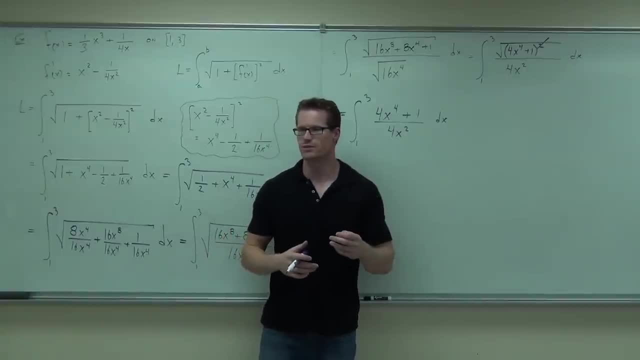 Remember these? when I gave them to you The first time we ever dealt with integrals, I gave you something that looked like that. It had t, though It was like t cubed plus 1 over t squared, or something I said. think a little bit more about these things. 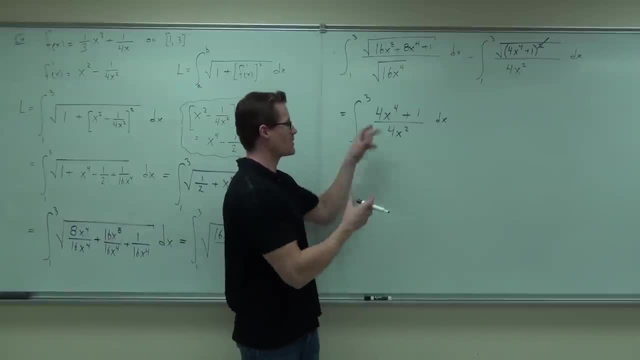 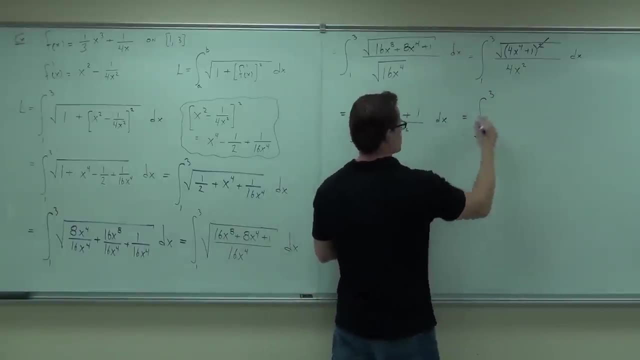 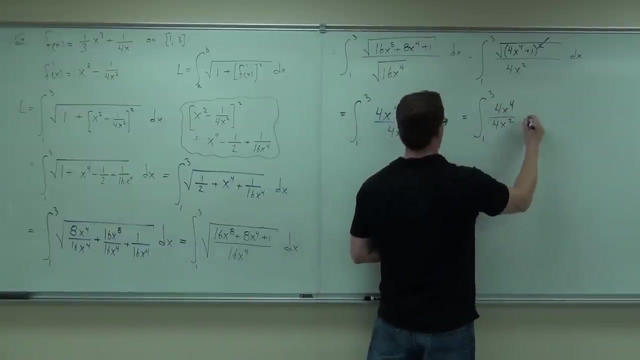 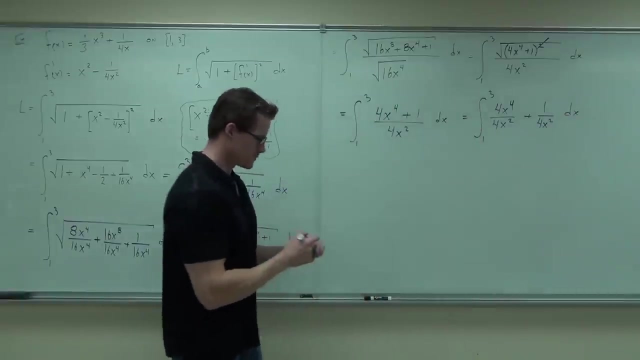 Split them up when you can, because if you have like variables, you can combine those things. So 4x to the fourth over 4x squared, yes, Plus that. So in a rule- let's simplify them a little bit- We got 4x to the fourth over 4x squared. 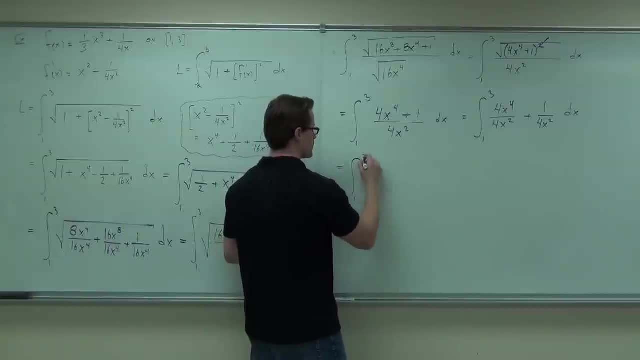 That's going to give you x squared. When you do the 1 over 4x squared, please don't make the mistake of taking the 4 with the x squared. That doesn't happen. The 4 stays on the denominator. Do you follow? 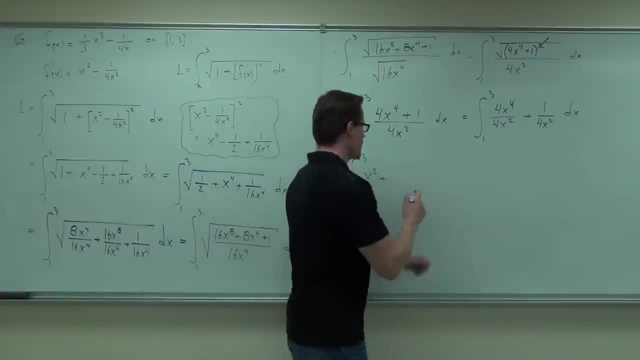 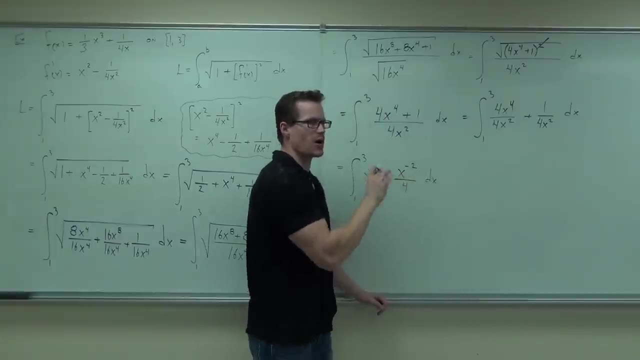 It stays. It doesn't have a negative exponent. It doesn't even have an exponent. It's going to be x to the negative, 2 over 4.. That's the appropriate way to do that integral. When you take the 4 up there, you're going to be off by a factor, by a large factor. 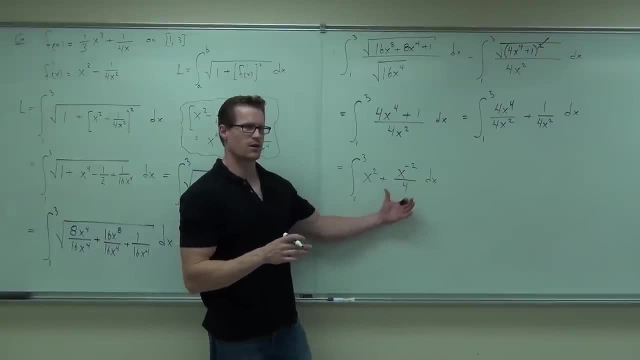 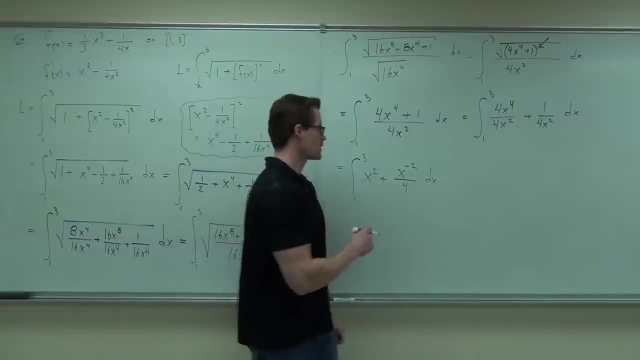 You don't want to do that. Do you see why the 4 stays down there? Can you do the integral? It's not too bad. Not too bad at all, really, When we think about it. we're going to have x to the third over 3.. 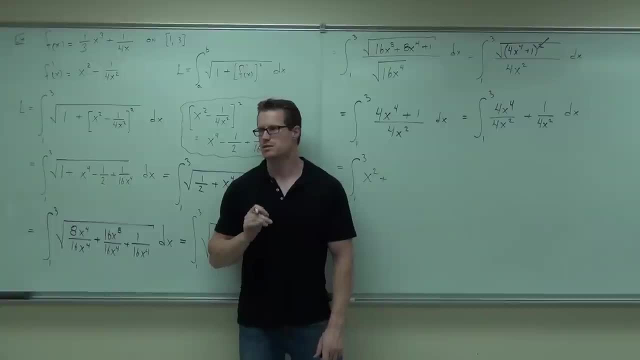 When you do the 1 over 4x squared, please don't make the mistake of taking the 4 with the x squared. That doesn't work. That doesn't happen. The 4 stays on the denominator. Do you follow? It doesn't have a negative exponent. 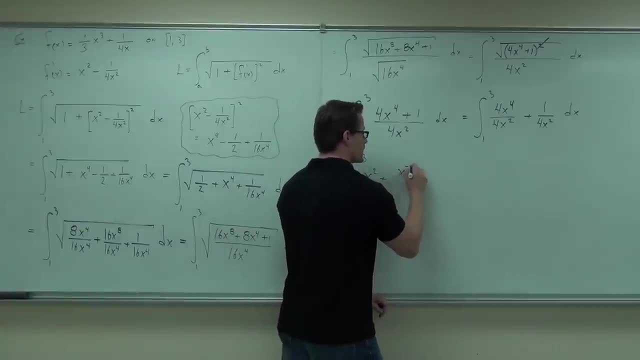 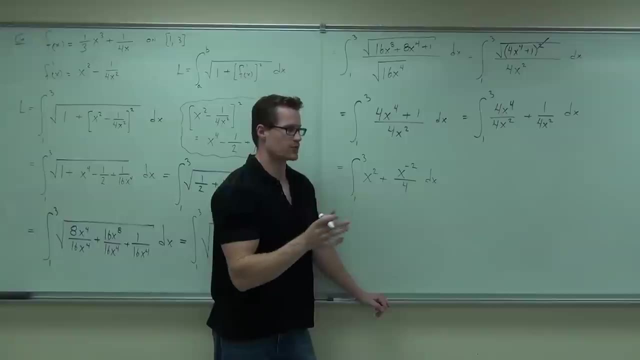 It doesn't even have an exponent. It's going to be x to the negative, 2 over 4.. That's the appropriate way to do that integral. You take the 4 up there you're going to be off by a factor, by a large factor. 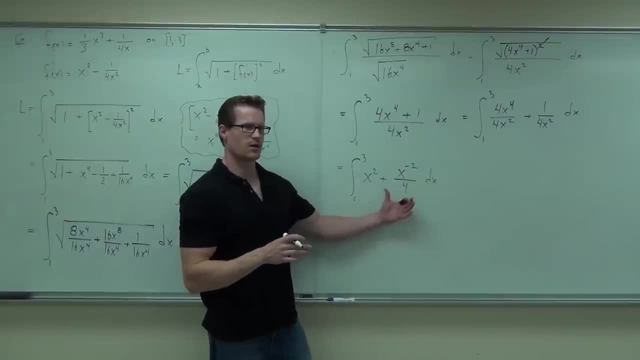 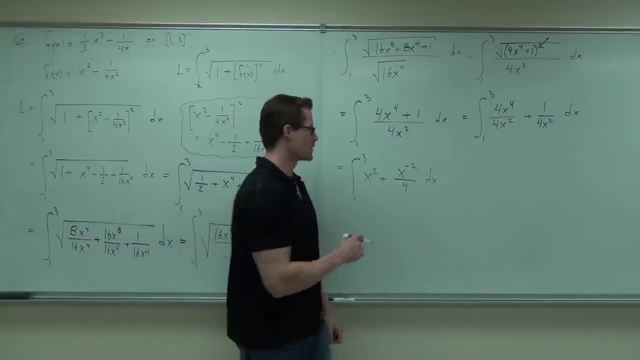 You don't want to do that. Do you see why the 4 stays down there? Okay, Can you do the integral? It's not too bad. Not too bad at all, really, When we think about it, we're going to have to do it. 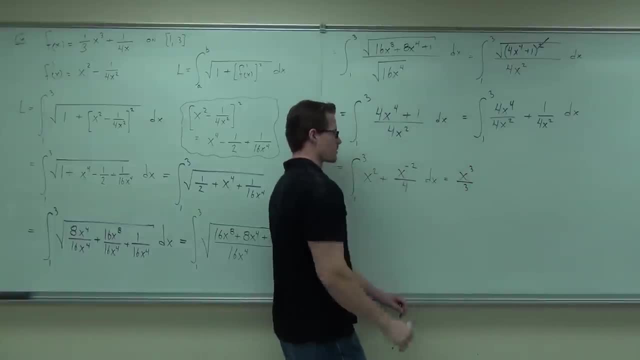 We're going to have x to the third over 3.. That's an easy one: x to the third over 3 plus. watch carefully, Remember that with integrals you are adding, you're not subtracting. So can you please tell me what does x to the negative 2 become? 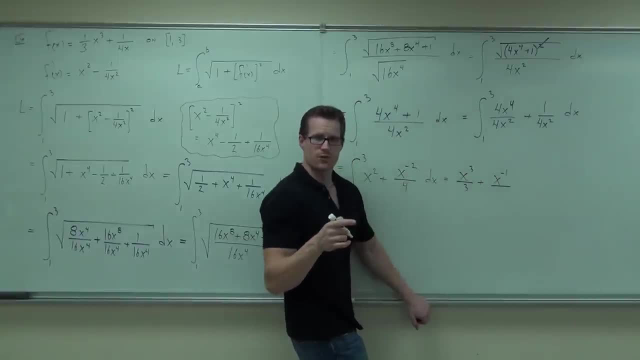 Perfect. Over what Negative 4.. Negative 4.. Do you see where the negative 4 is coming from? Yeah, Get the negative 1 times the 4.. That's negative 4.. Before you go and evaluate, take care of this mess. 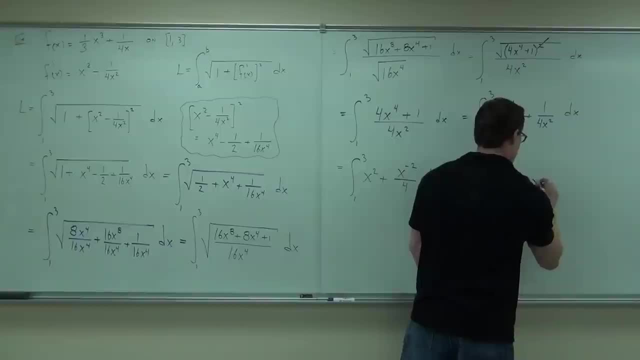 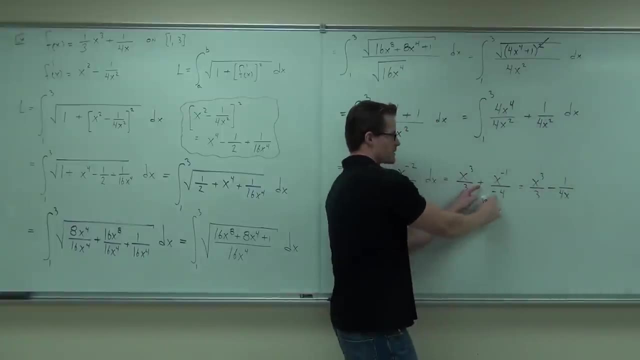 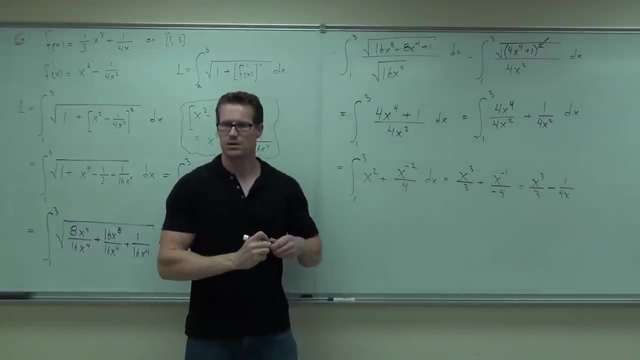 Make it look prettier right here. This is going to be x to the third over 3.. We're going to have a minus 1 over 4x. Minus 1 over 4x. Yes, no, I feel like I can all the way down that far. 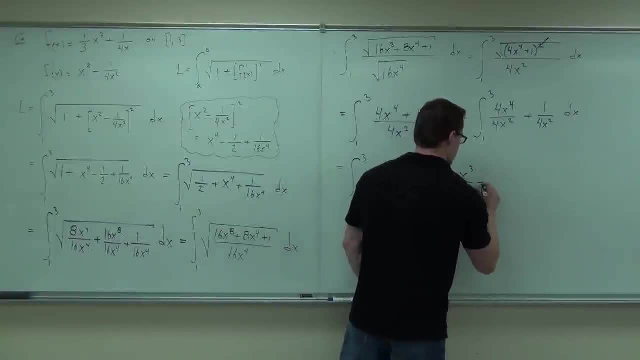 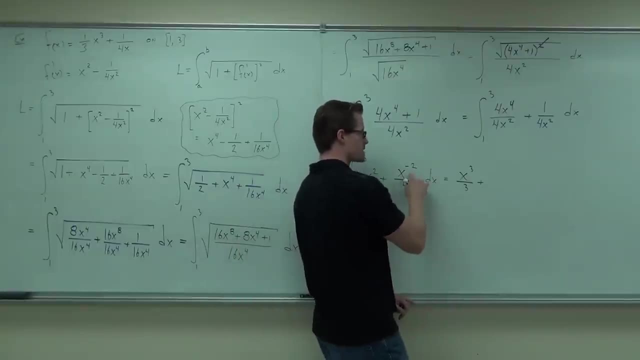 That's an easy one: x to the third over 3 plus. watch carefully, remember that with integrals you are adding, you're not subtracting. So can you please tell me what does x to the negative 2 become x to the third over 4.. 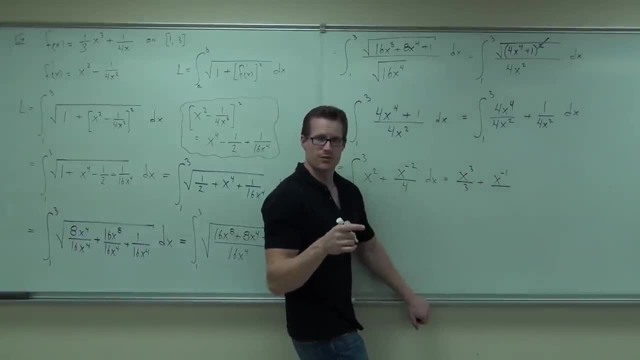 Perfect. Over what Negative 4.. Negative 4.. Do you see where the negative 4 is coming from? You get the negative 1 times the 4.. That's negative 4.. Before you go and evaluate, take care of this mess. make it look prettier, right here. 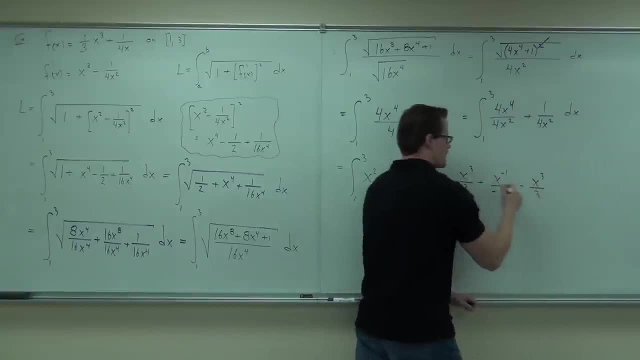 This is going to be x to the third over 3.. We're going to have a minus 1 over 4x, minus 1 over 4x, Okay, Okay. So we're going to have a minus 1 over 4x. 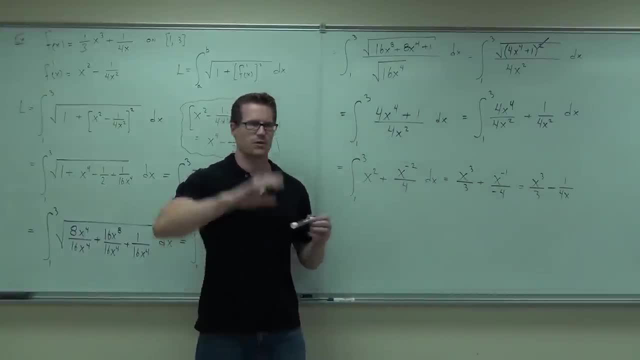 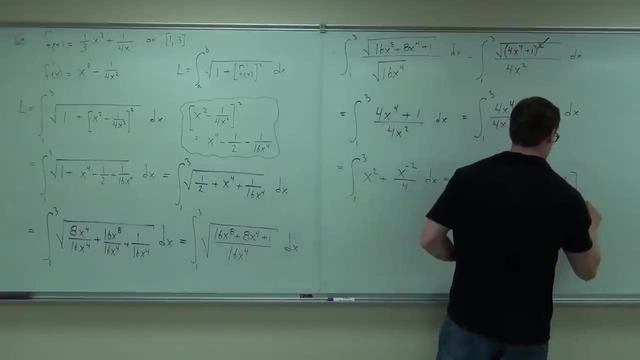 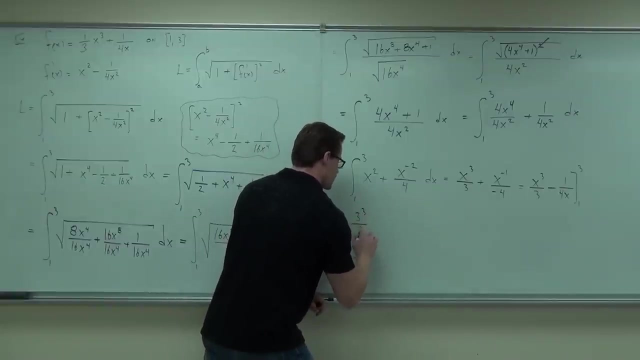 Yes, no, Rich, and I feel like we can all lay down that far. Cool. Hey, it's just a valuation for this. We've got to go from 1 to 3.. We'll plug in the 3 first. So that's going to be 3 cubed over 3 minus 1 over 4 times 3 minus. remember, we have a. 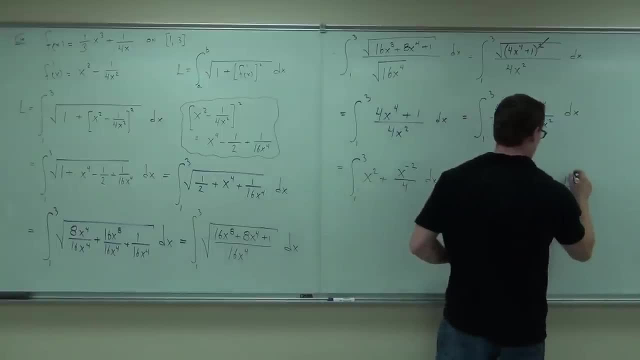 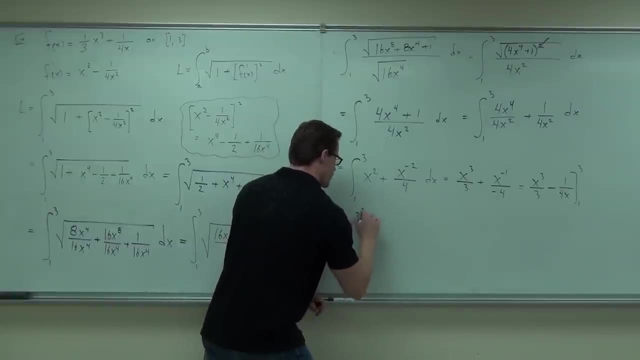 Cool. Hey, it's just a valuation. for this We've got to go from 1 to 3.. We'll plug in the 3 first. So that's going to be 3 cubed. That's going to be 3 cubed. 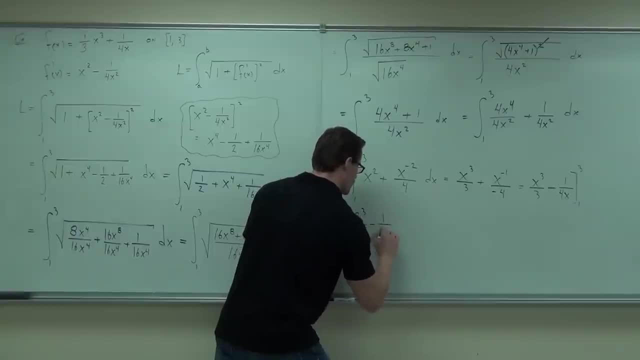 That's going to be 3 cubed, 3 cubed over 3 minus 1, over 4 times 3 minus. remember we have a 1 right now. You can't just put a 0 at the end, We have a 1.. 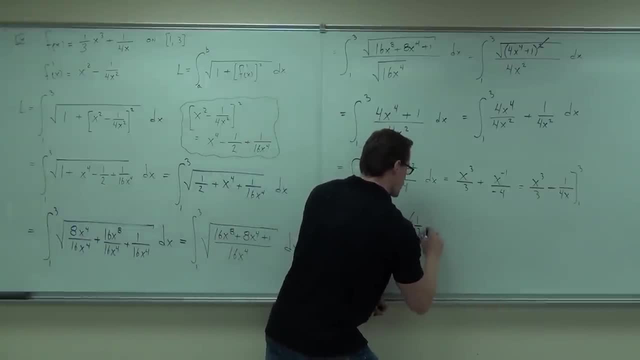 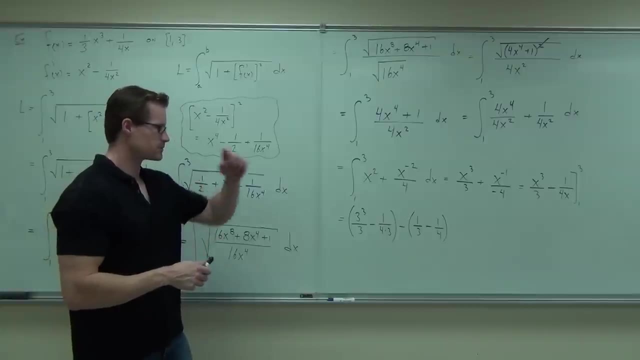 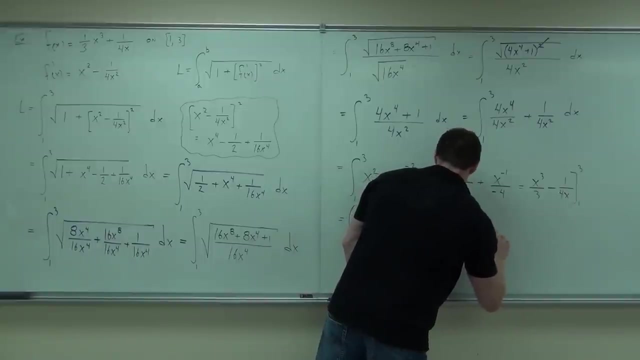 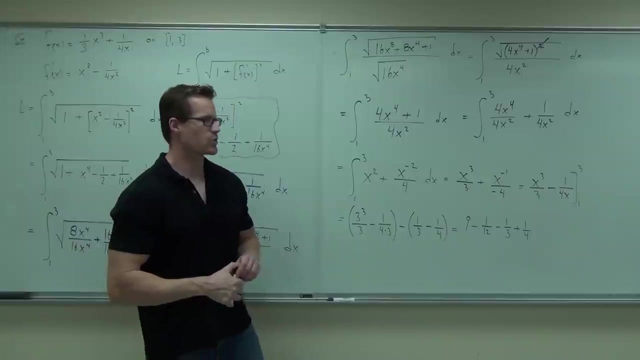 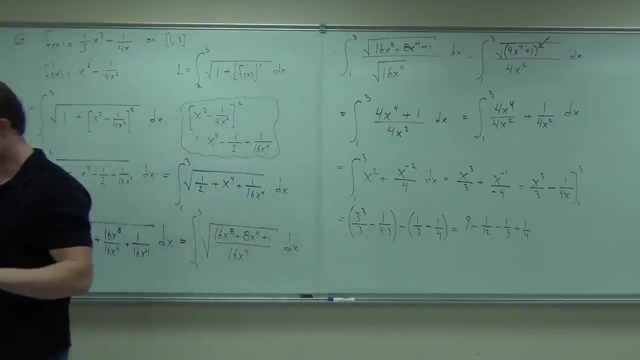 So you have 1 third minus 1 fourth. If you do 9 minus 1 twelfth minus 1 third plus 1 fourth, Do you know where the plus 1 fourth is coming from? first of all, Can someone do that on a calculator and see what you get? 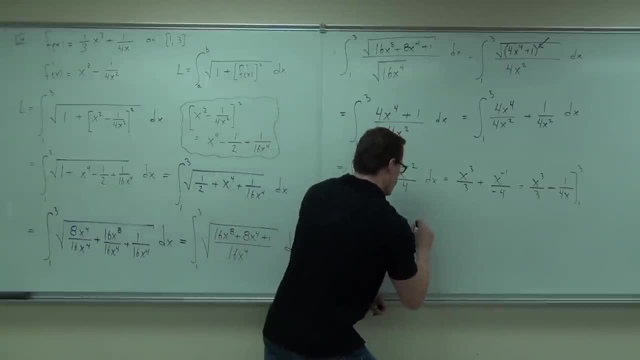 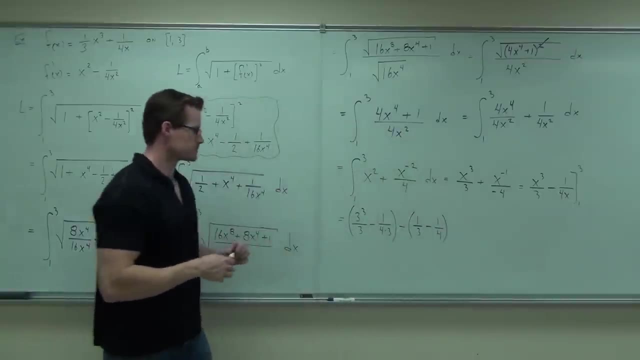 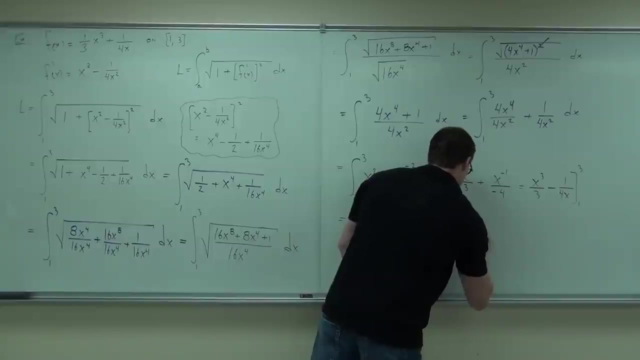 1. right now We have a 0, at the end We have a 1.. So you have 1 third minus 1 fourth. If you do, 9 minus 1 twelfth minus 1 third plus 1 fourth. Plus 1 fourth is coming from first of all. 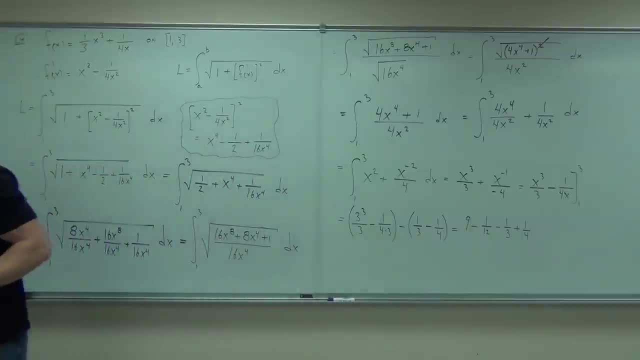 Can someone do that on a calculator and see what you get? Okay, Colony denominator is 12. if you want to do it that way, 108 over 12 minus 1 twelfth minus 4 twelfths plus 3 twelfths. 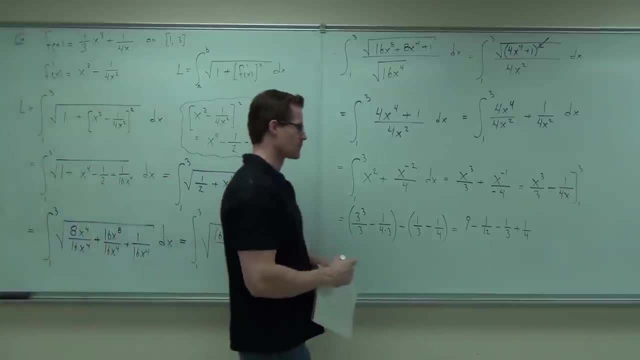 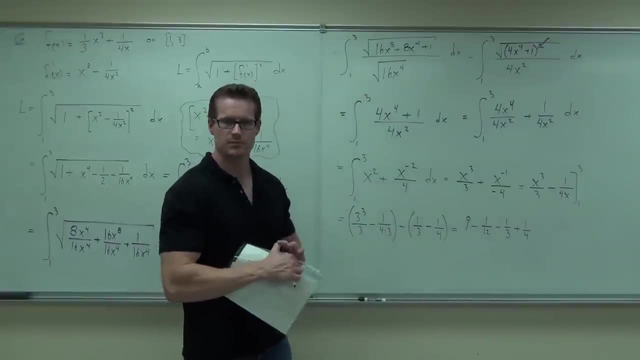 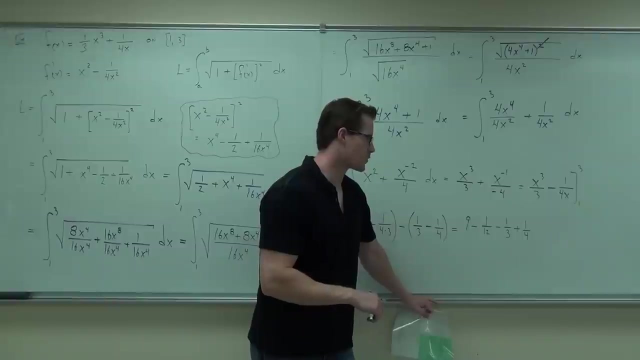 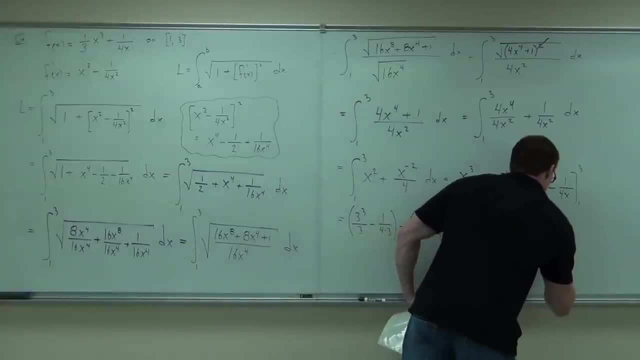 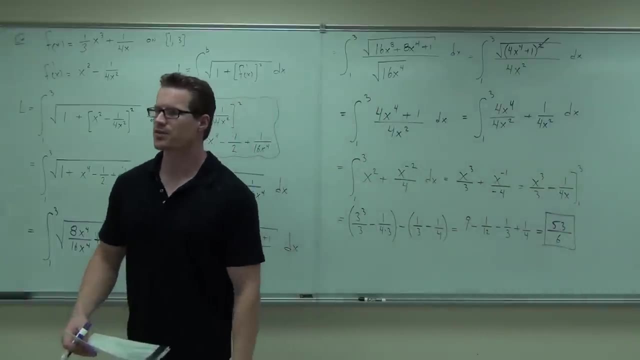 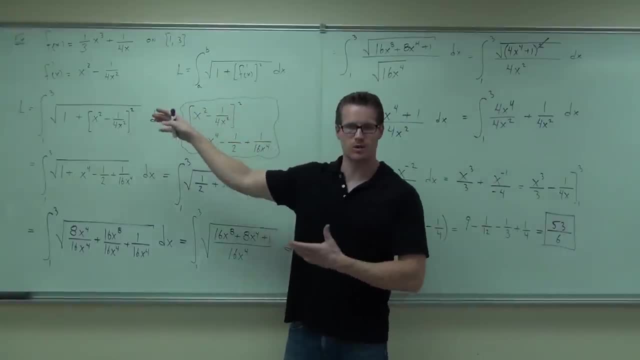 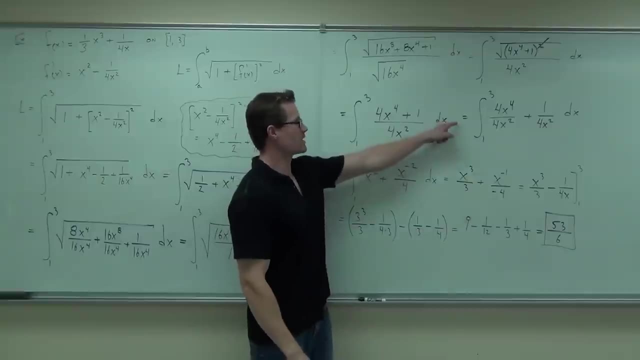 This took us a long way to do it, But most of it is algebra. The only calculus you actually get to do is plug in the formula in and from right here. Let's see: Right here and right here. That's it. After that, algebra, algebra, algebra. 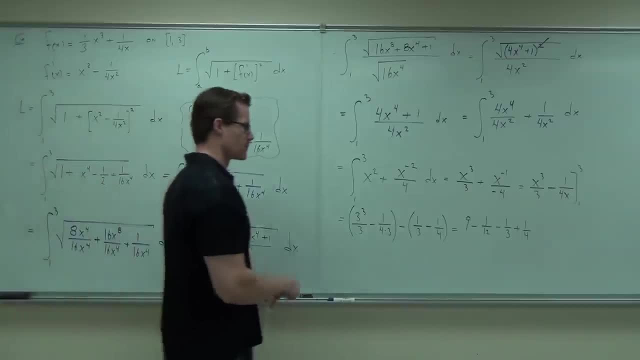 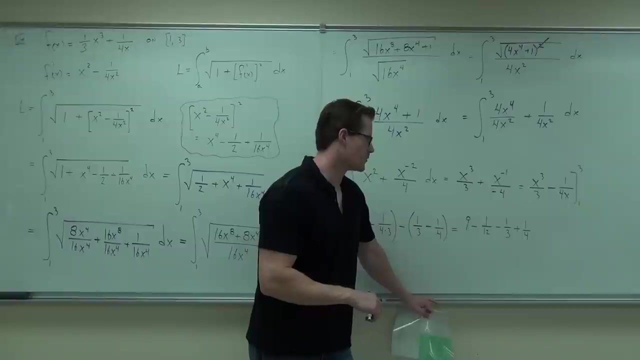 Okay, Okay, The common denominator is 12. if you want to do it that way, 108 over 12 minus 1, twelfth minus 4, twelfths plus 3 twelfths. Huh, 53 over 6?. 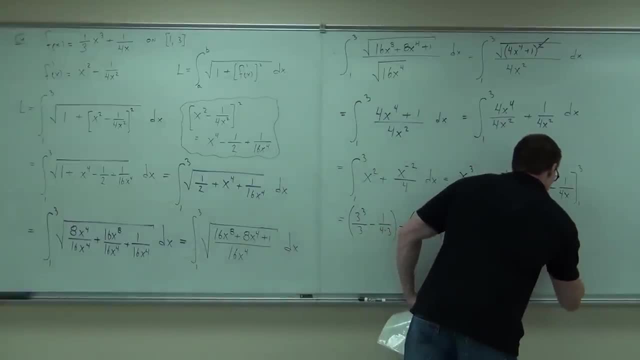 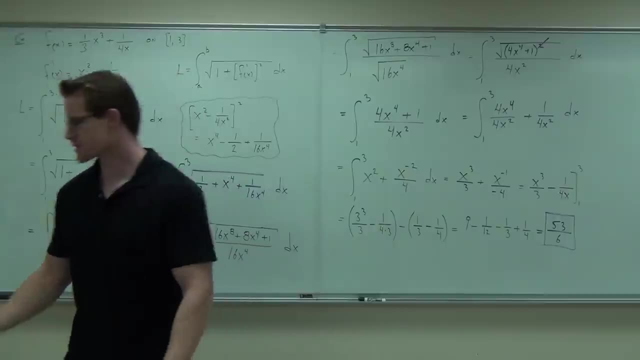 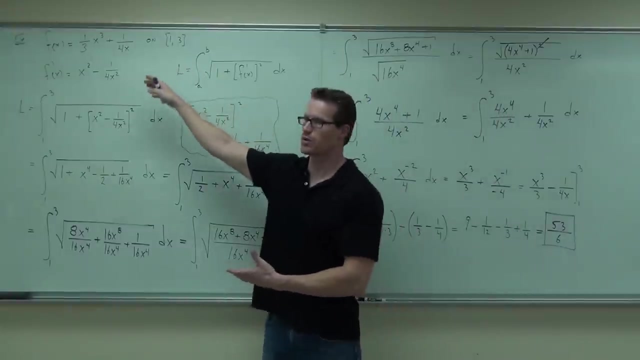 Yeah, 53 over 6.. 53 over what's that? 53 over 6? The length, The length. That's crazy, But we just found the length of this curve right. It took us a long way to do it. 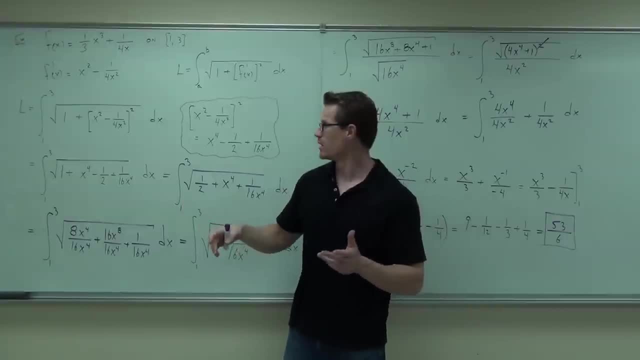 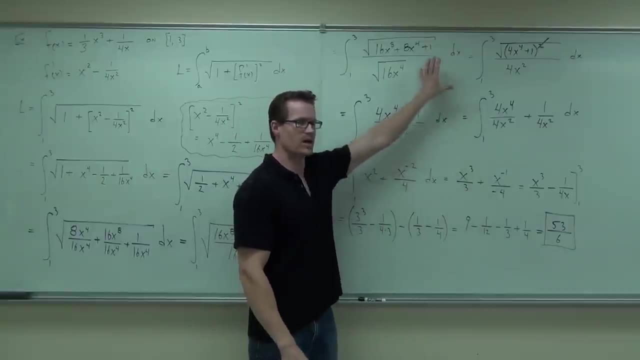 But most of it is algebra. The only calculus you actually get to do is plug in the formula in, And from right here, let's see, right here, to right here. that's it After that: algebra, algebra, algebra, evaluation, evaluation. 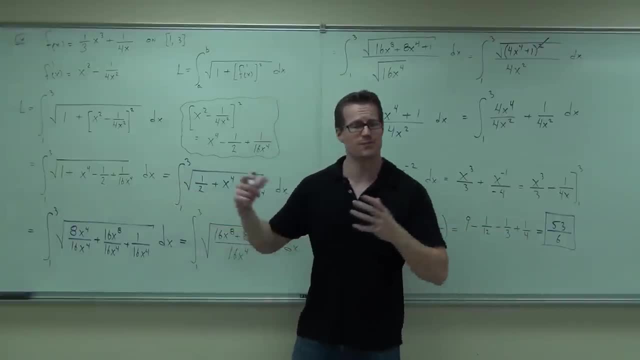 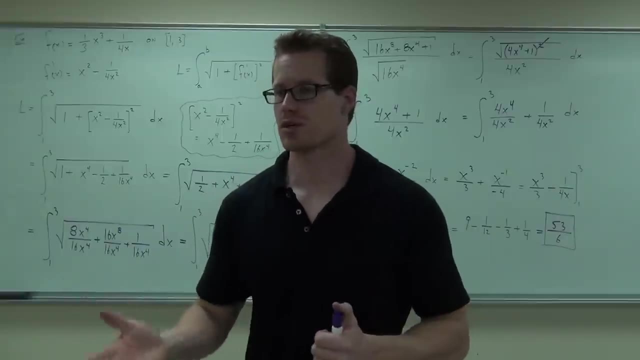 So that's really what this is all about: is being able to use that formula, identify what goes where and find the length out of that thing. So we found the length of 53 over 6.. If it's in inches, it's inches long. 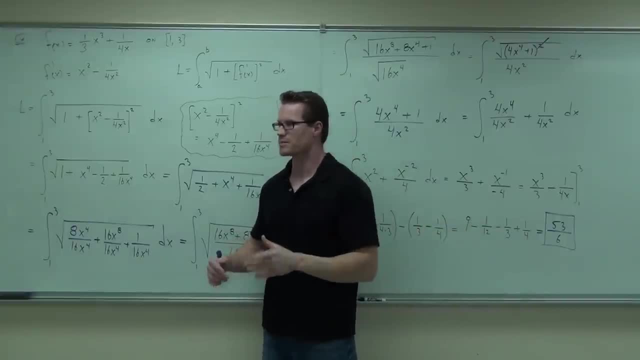 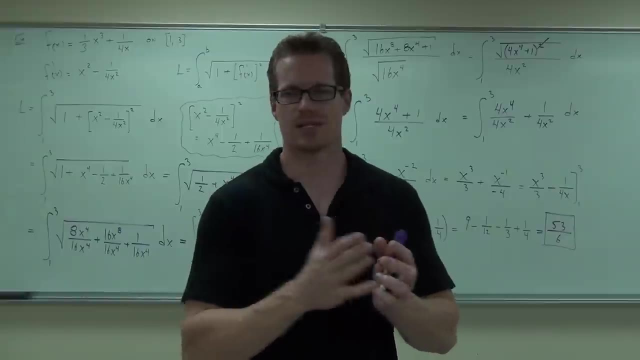 Evaluation, evaluation. So that's really what this is all about is being able to use that formula, identify what goes where and find the length out of that thing. So we found the length of 53 over six. If it's in inches, it's inches long. 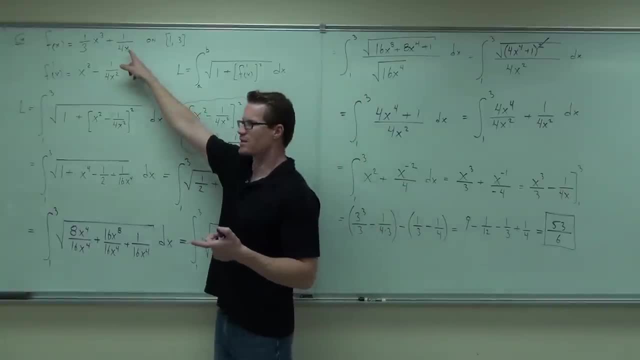 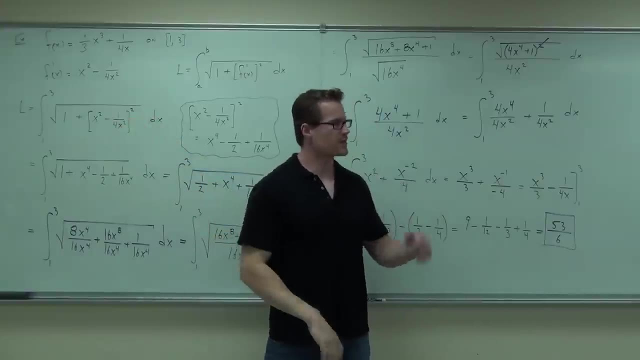 It's kinda cool. It's really unique that we're able to do that. To take some random function- actually it's not very random, it's a specific function, because some of these things don't work out and find the length of it, which is neat. 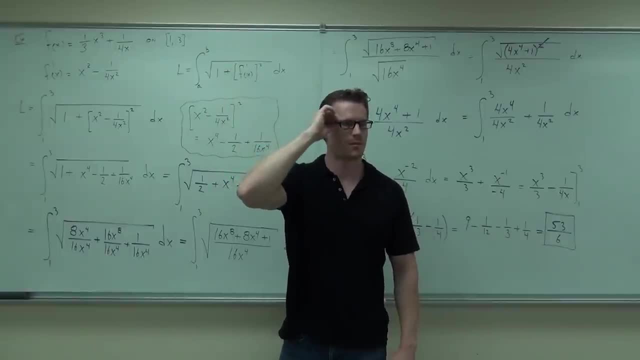 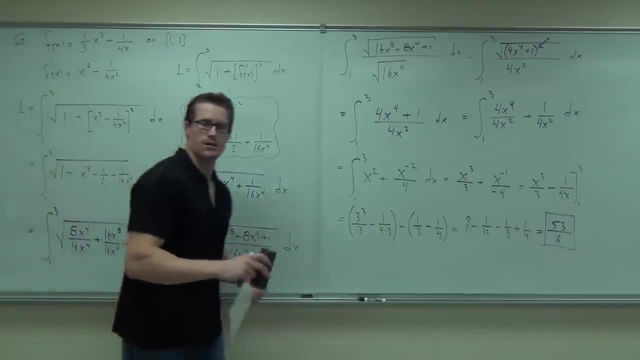 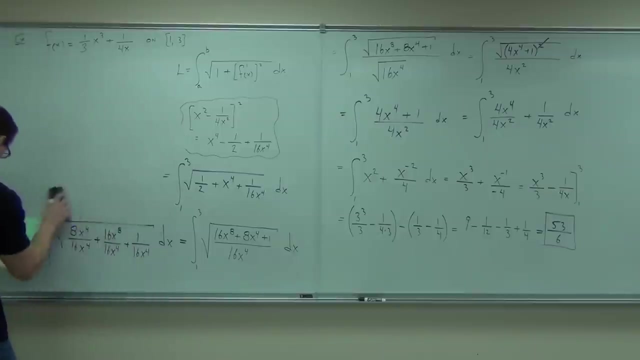 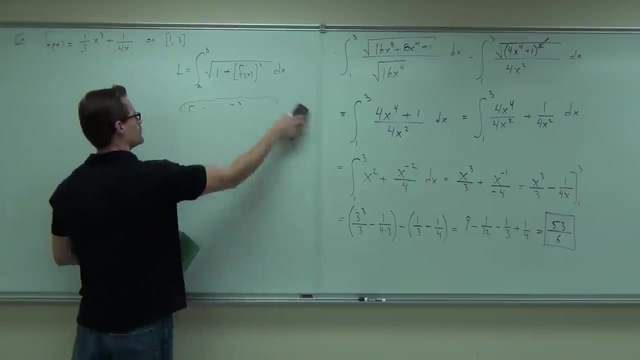 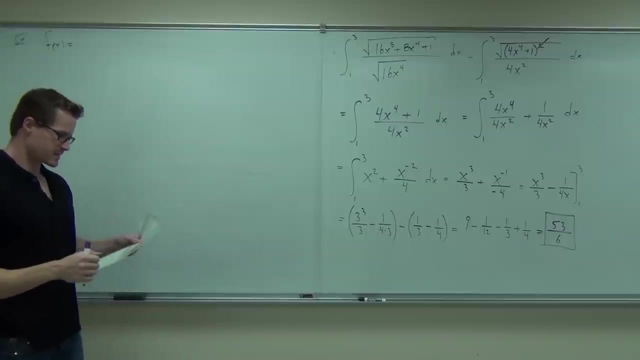 And we're able to understand the example. Would you like one more? Yes, Okay, any questions before I erase it all, All right, Okay, so let's do this one. F of x is now x to the power of x. 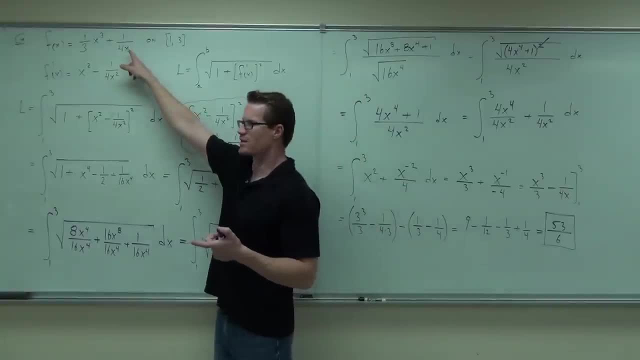 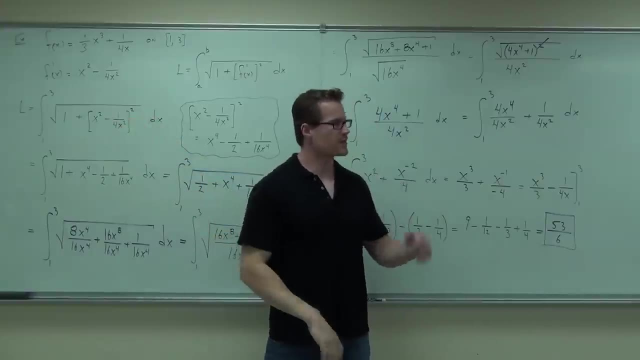 It's kind of cool. It's really unique that we're able to do that. To take some random function- actually it's not very random, It's a specific function, because some of these things don't work out And find the length of it which is neat. 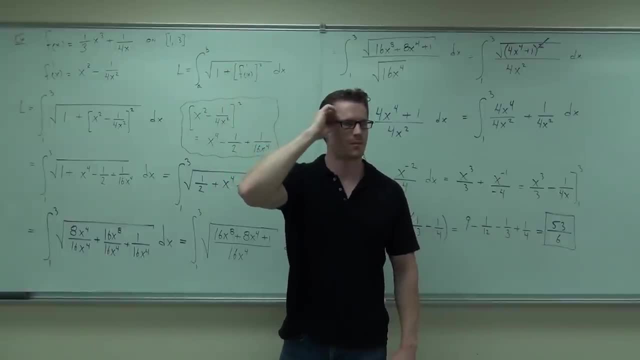 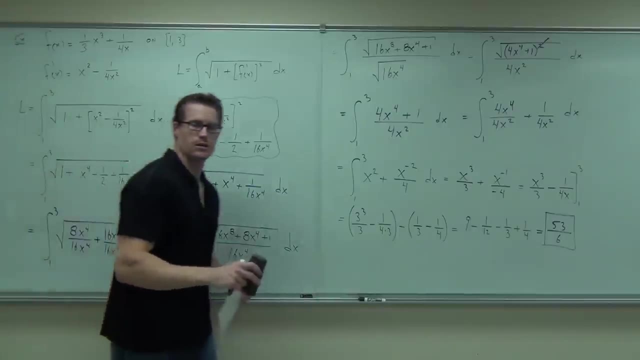 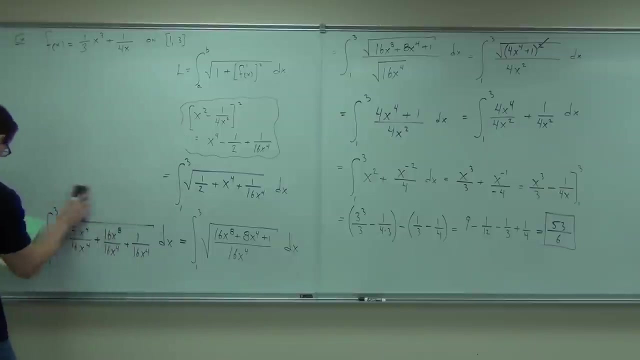 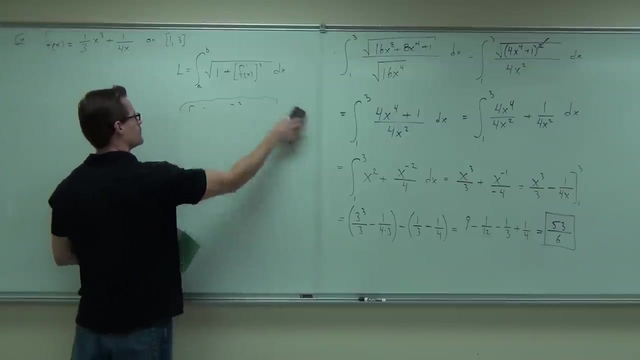 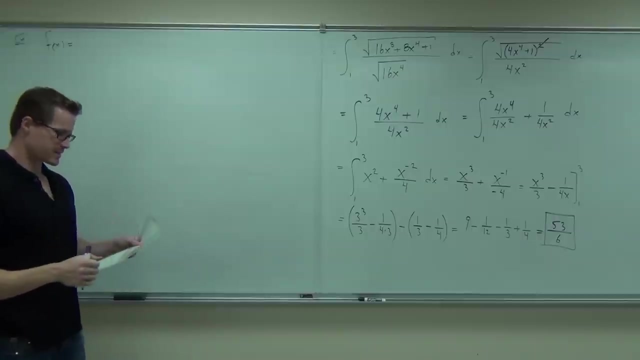 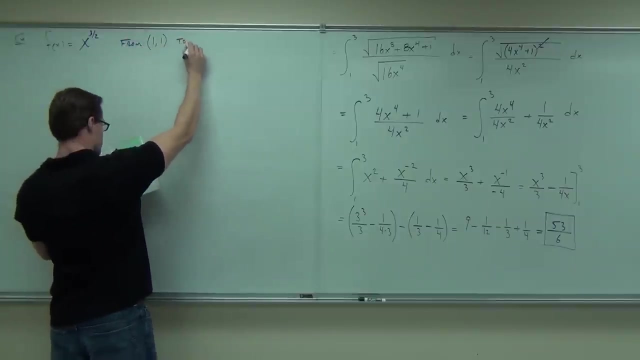 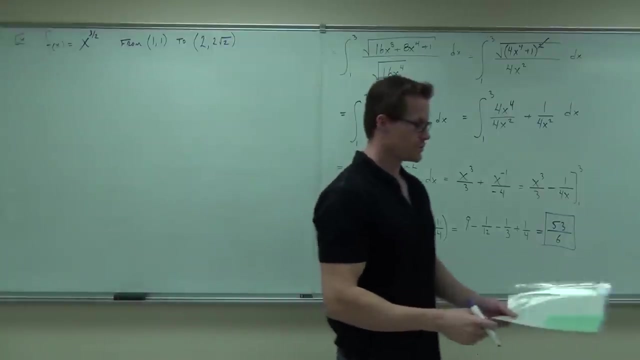 And we're able to understand the example. Would you like one more? Yes, Any questions before I erase it all, All right, Okay, So Let's do this. one. F of X is now X to the 3 halves From 1, 1 to 2, 2 root 2.. 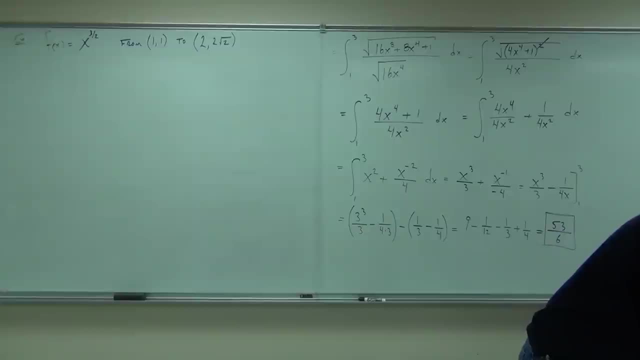 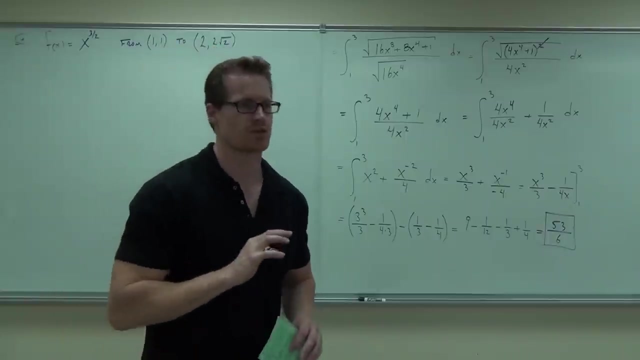 You ready for this one? I hope so. Well, I want you to help me. I want you to tell me what I should do first. If I'm trying to find the length, what should I do first? Take the derivative, Very good. 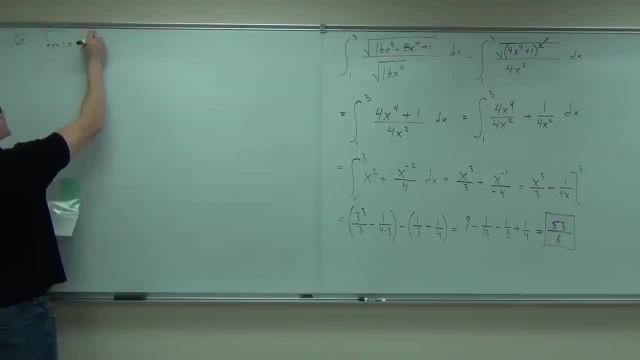 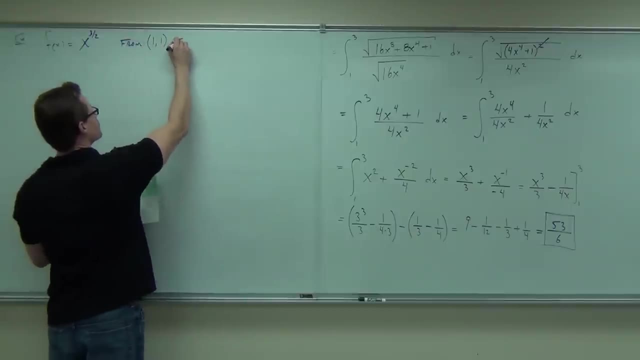 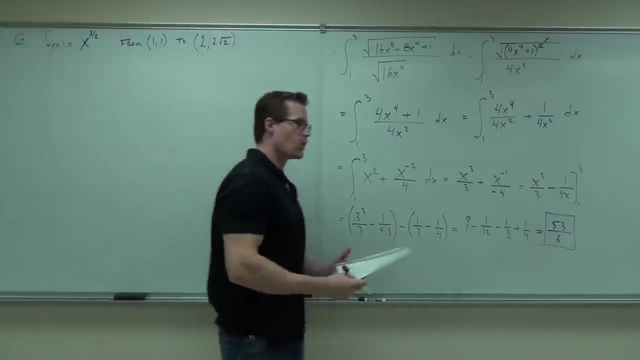 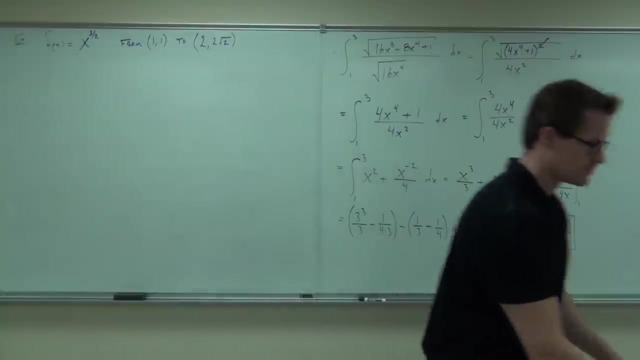 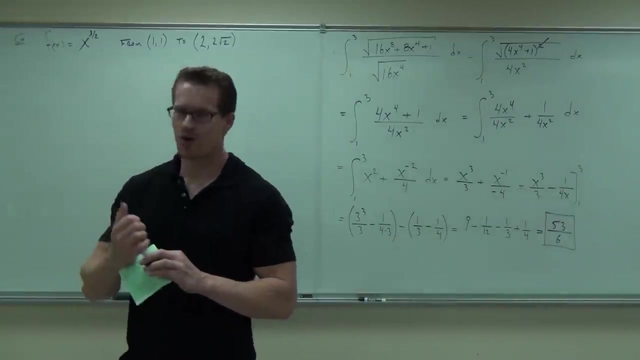 Question three has, From one one to two comma two, root two. You ready for this one? I hope so, I hope so. Well, I want you to help me, I want you to tell me what I should do first. 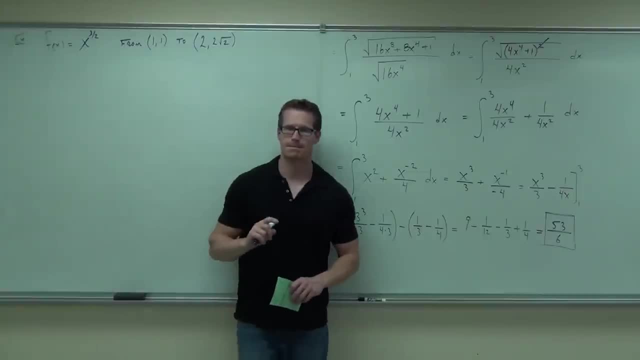 If I'm trying to find the length, what should I do? first, Take the derivative. Very good, take the derivative. Am I worried about changing this into certain terms, Like, do I wanna change it into terms of y or x, depending on length? 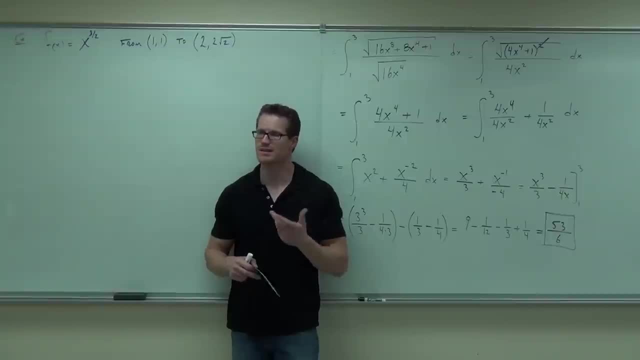 The length's gonna be the same, no matter whether you have this in terms of x or in terms of y. so it really doesn't matter. I'm gonna show you in a little bit that it's gonna come up with the exact same measurement. 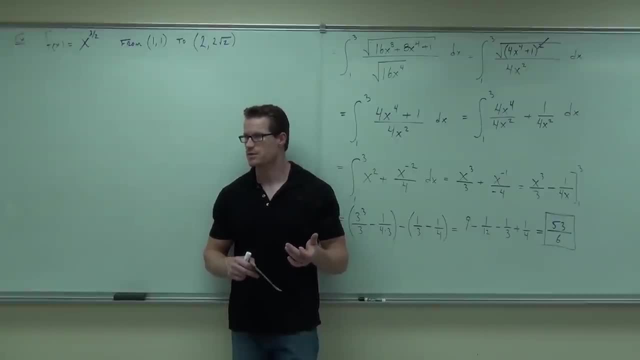 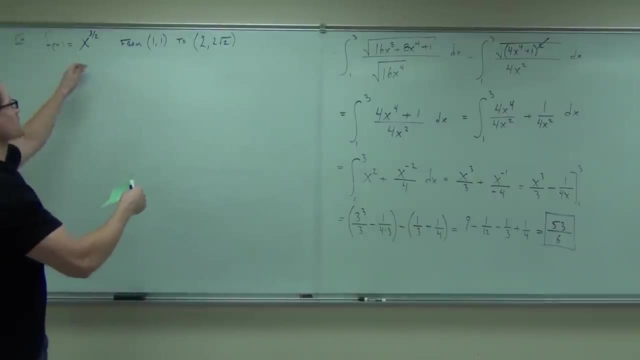 exact same measurement either way. either way that you do this, okay. So whatever it is, it is, it's fine. Just make sure that you have it in some terms. So y equals. this happens to be in terms of x. 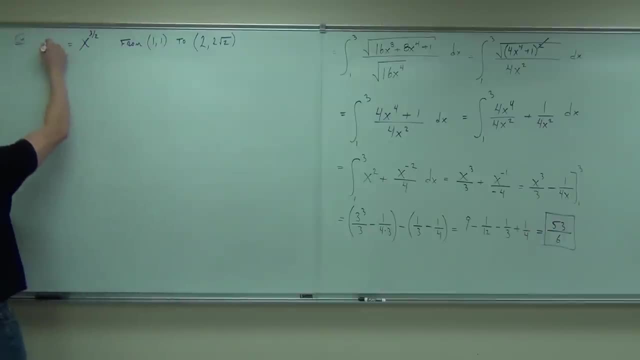 Maybe you can write a y if you want. Y equals x to the three halves. That's in terms of x. Leave it in terms of x. okay, Taking a derivative, great, First derivative: everybody, what's the first derivative of that thing, please? 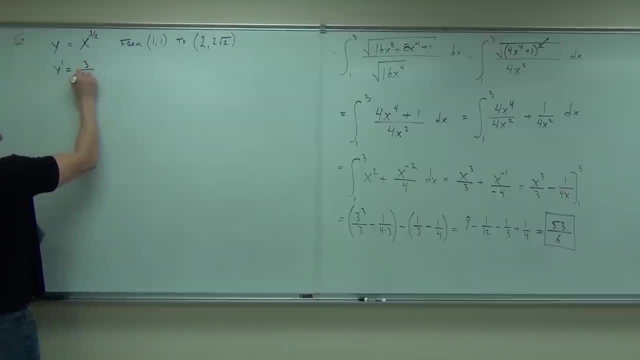 Three halves, Three halves. don't forget the three halves, That would blow your problem up. Three halves x to the what? One half, One half. very good, So our length is an integral. from now, this is the only place. 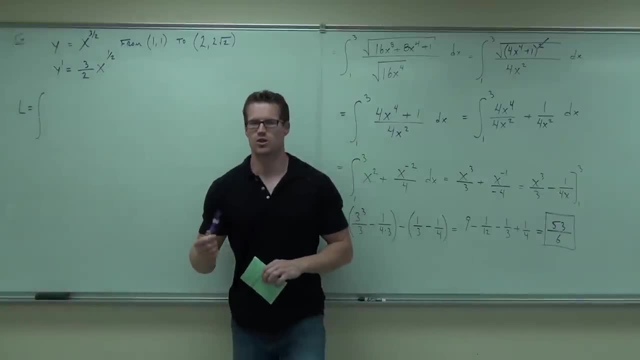 where you gotta be a little careful. What is your function in terms of? Is it in terms of y or in terms of x? In terms of x? Very good, it's in terms of x. So what are our bounds going to be? 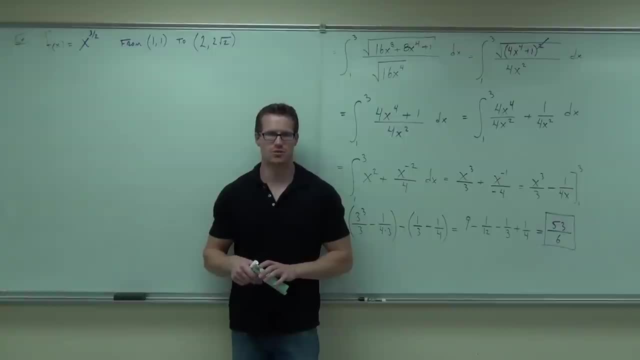 Take the derivative. Am I worried about changing this into certain terms, Like: do I want to change it into terms of Y or X, depending on length? The length seems the same, no matter whether you have this in terms of X or in terms of Y. 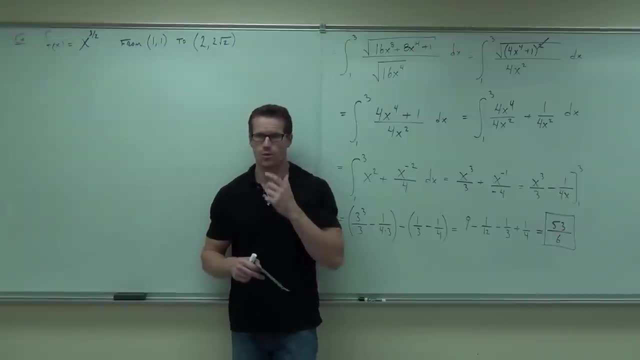 So it really doesn't matter. I'm going to show you in a little bit that it's going to come up with the exact same measurement- exact same measurement either way that you do this, Okay. So whatever it is, it is. 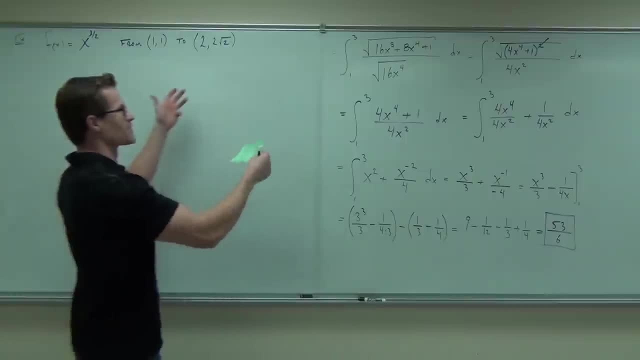 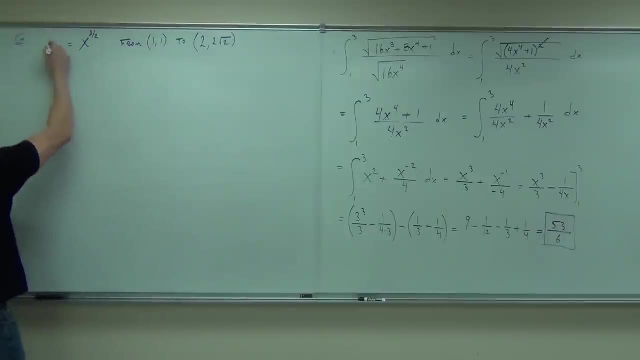 It's fine, Just make sure that you have it in some terms. So Y equals- this happens to be in terms of X. Maybe you can write a Y if you want. Y equals X to the 3 halves, That's in terms of X. 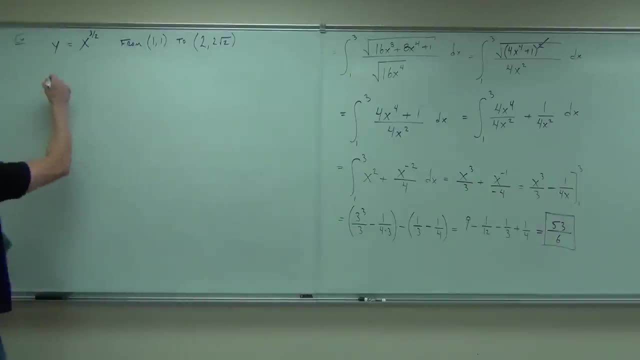 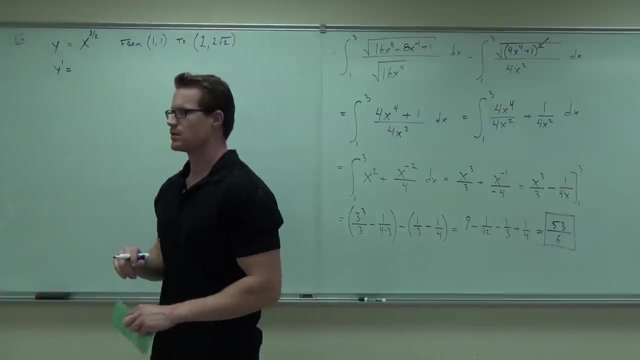 Leave it in terms of X. Okay, Taking a derivative, great First derivative: everybody. what's the first derivative of that thing, please? Three halves, Three halves. Don't forget the three halves, That would blow your problem up. 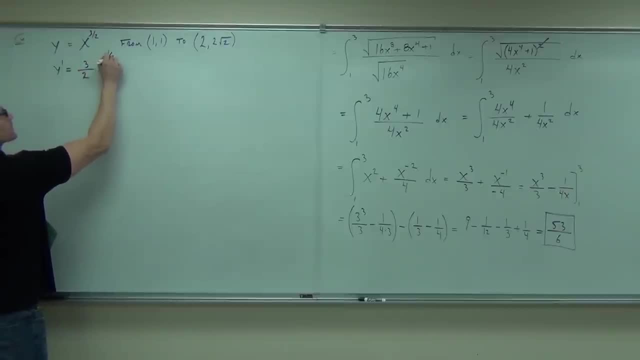 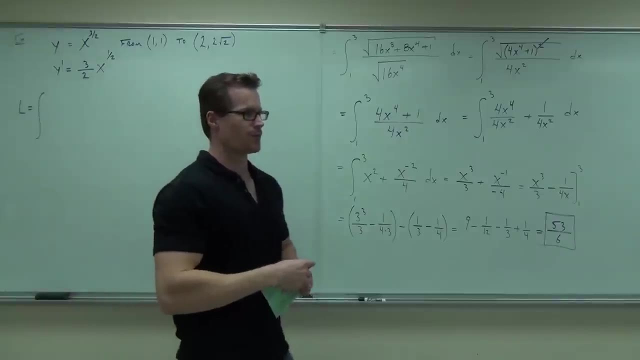 Three halves X to the. what? One half, One half. Very good, So our length is an integral. from now, this is the only place where you've got to be a little careful. What is your function in terms of? Is it in terms of Y or in terms of X? 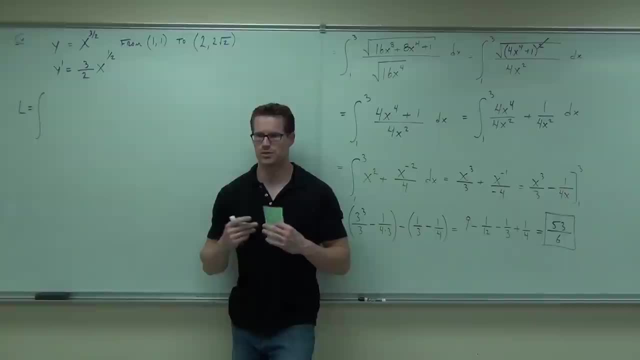 In terms of X. Very good, It's in terms of X. So what are our bounds going to be X's Or Y's, Y's? What's your function in terms of X's? Are you going to put Y's into X's? 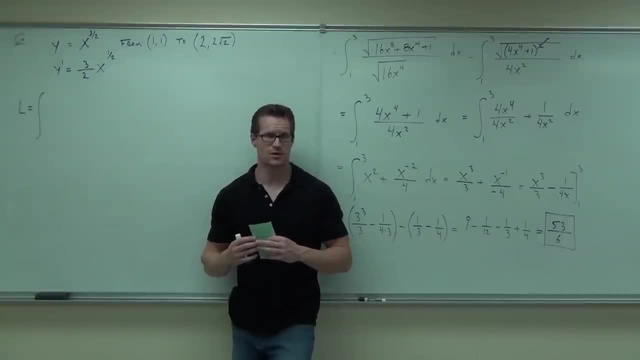 No, I hope not. So what are your bounds going to be in terms of X's, X's? You have, in terms of X, right, this has an X in it, So am I going to go from 1 to 2, or 1 to 2 root 2?? 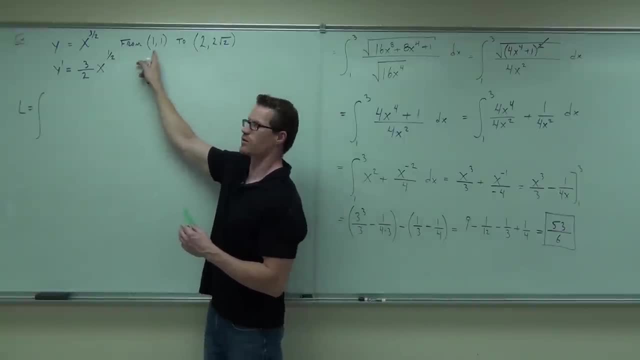 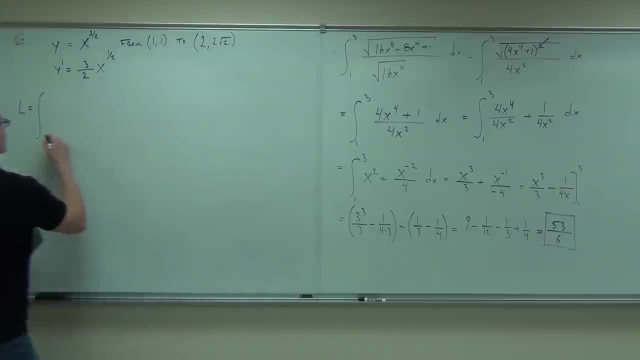 1 to 2.. 1 to 2 because those are my X's. It wouldn't matter here, right, X and Y is the same there, but here it definitely would make a difference. So because I'm in terms of X right now, I'm going to go from 1 to 2, square root, 1 plus. 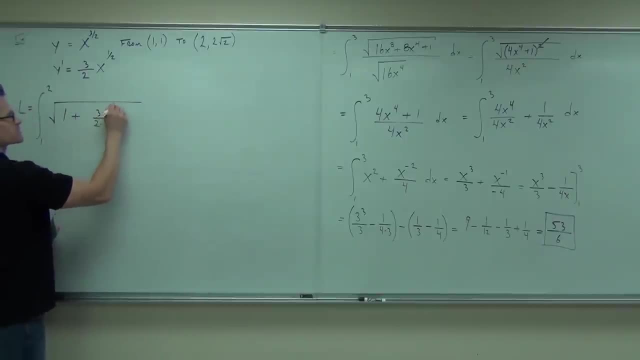 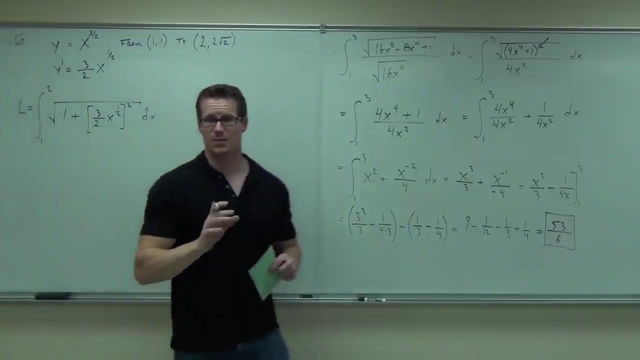 I've already taken the first derivative. we've got 3 halves X to the 1 half. don't forget to square it DX. Are you okay on the set up, ladies and gentlemen, Honestly, are you okay with it? 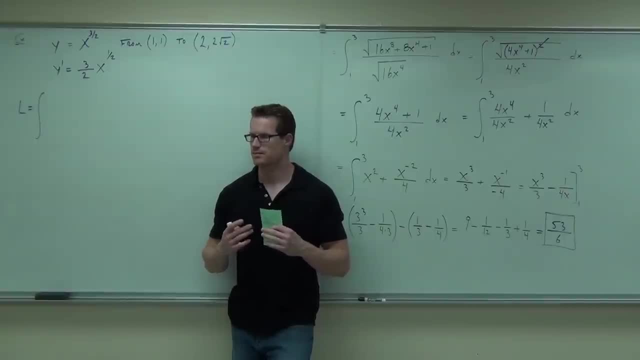 Xs or ys, Ys And ys. What's your function in terms of? are you gonna put ys into xs? I hope not, So what are your bounds gonna be in terms of Xs? You have in terms of x, right, this has an x in it. 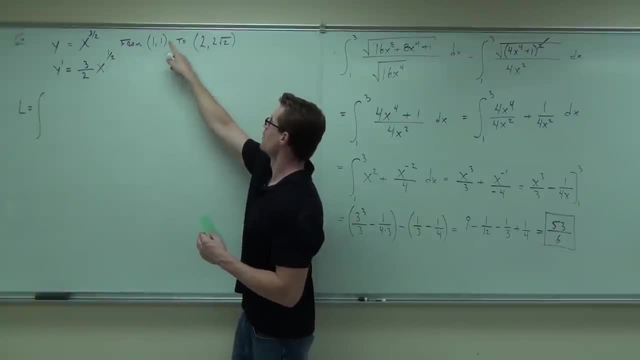 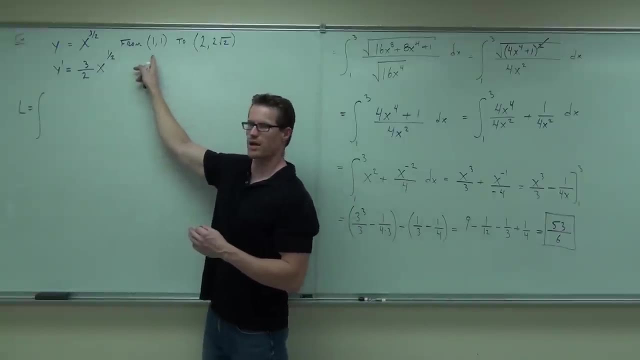 So am I gonna go from one to two or one to two, root two, One to two, One to two, because those are my xs. Wouldn't matter here, right, x and y is the same there, But here it definitely would make a difference. 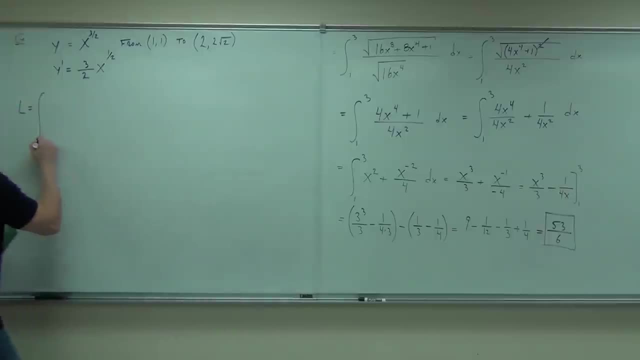 So, because I'm in terms of x right now, I'm gonna go from one to two Square root, one plus. I've already taken the first derivative. we've got three halves x to the one half. don't forget to square it dx. 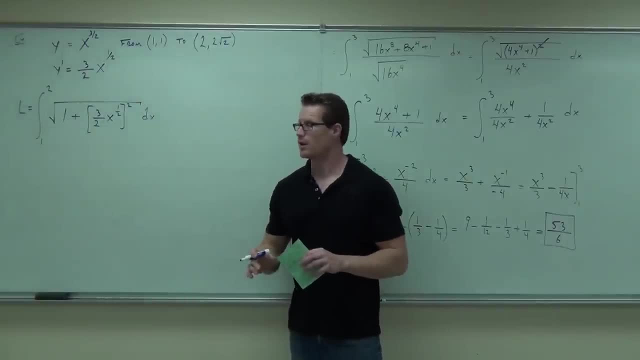 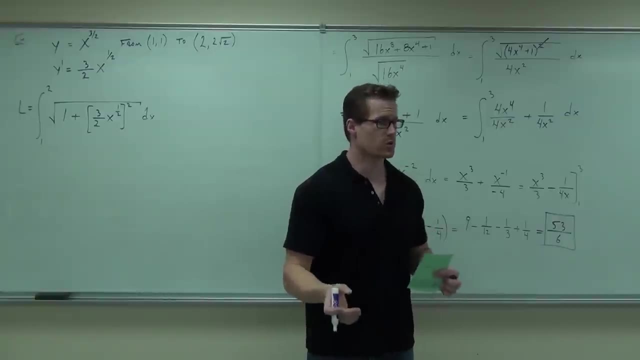 Are you okay on the set up, ladies and gentlemen? Honestly, are you okay with it? Okay, That's the calculus. We're gonna have a whole bunch of algebra and then a little bit more calculus. Let's see if we can work through this thing. 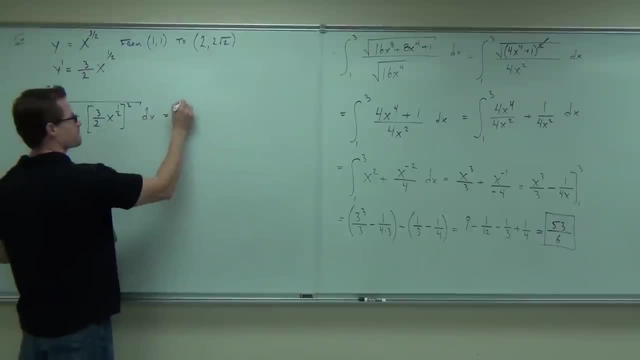 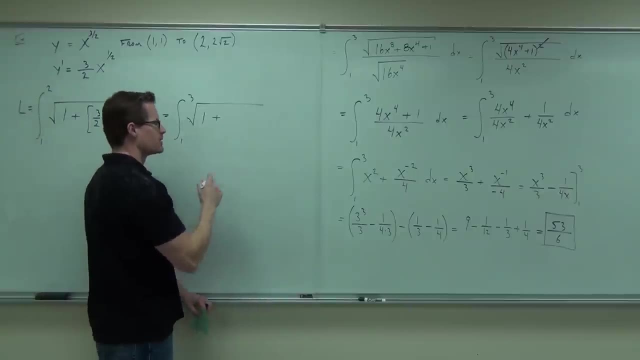 What's the first thing we're gonna do? Help me out. come on Square root of x. Mm-hmm, I'm pretty sure that's gonna do a sidebar. Pretty sure that's gonna be what. Nine fourths of x. 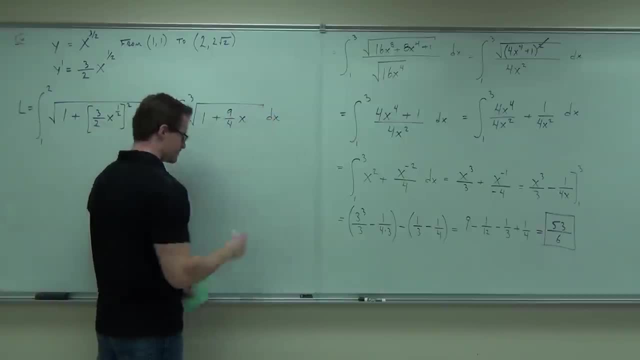 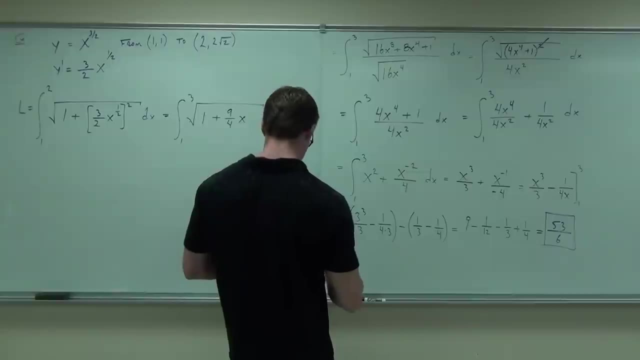 Nine fourths of x. I like it. One to two, one to three. Oh, what'd I do? What did you do? What did you do Your bounds Like that? We got excited, We got excited, we got excited. 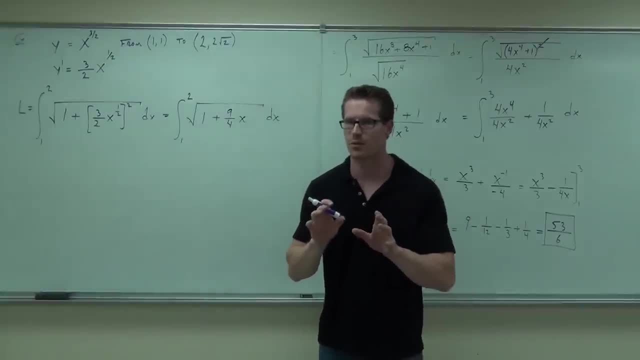 What now? What now? Think back to the previous problem. Think back to the previous problem. Find the common denominator. Say what. Find the common denominator, Find the common denominator. Do we have a denominator right now? Yes, we do. 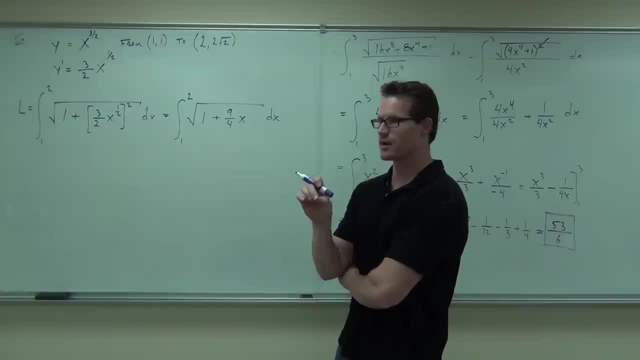 Actually, you know what? Can we make this a little easier Instead of doing all that? can we make it a little easier? Would you mind if I made it a little easier, Because we can do all that and you're still gonna have the same problem. 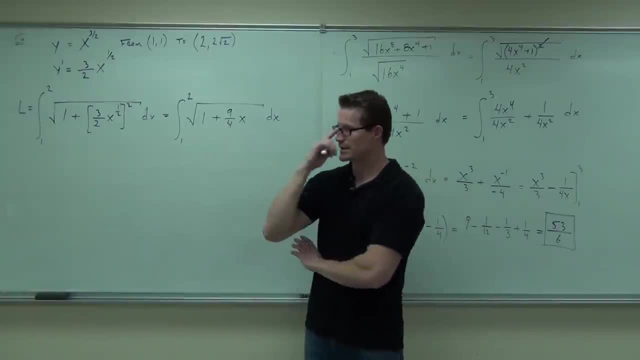 However, I want you to think about this for a second. What does substitution work? Tell me something. What's the derivative of this whole thing? right here? Nine fourths: Do we care about constants when we're doing substitution? So what does substitution work? 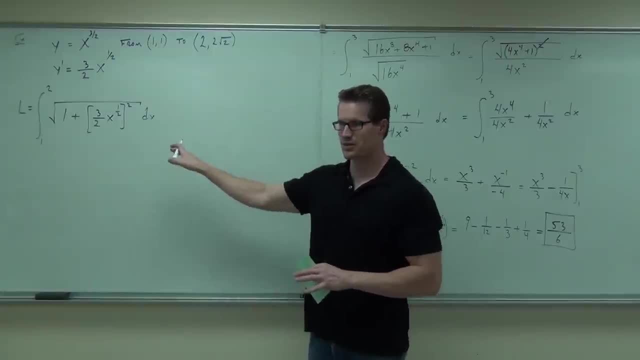 No problem. Okay, That's the calculus. We're going to have a whole bunch of algebra and then a little bit more calculus. Let's see if we can work through this thing. What's the first thing we're going to do? Help me out. 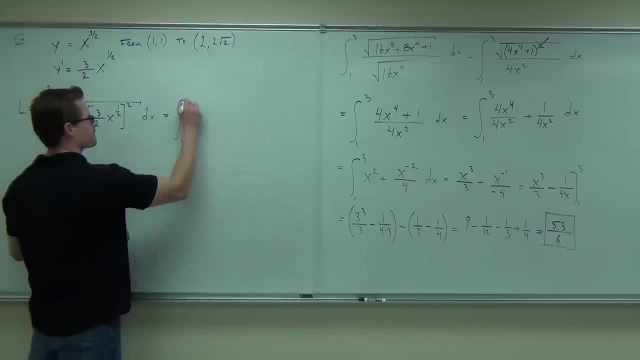 Come on, Square root of X. Pretty sure that's going to be what: 9 fourths X. 9 fourths X. I like it. 1 to 2.. 1 to 3.. Oh, what did I do? 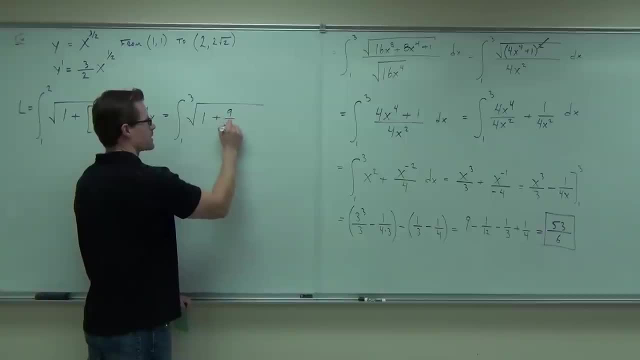 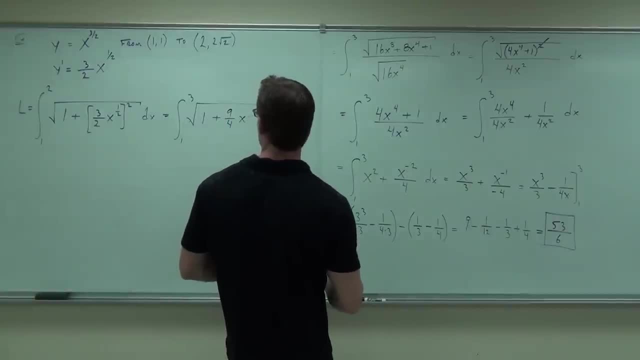 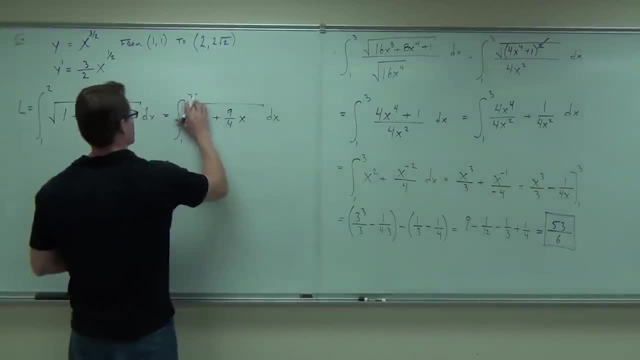 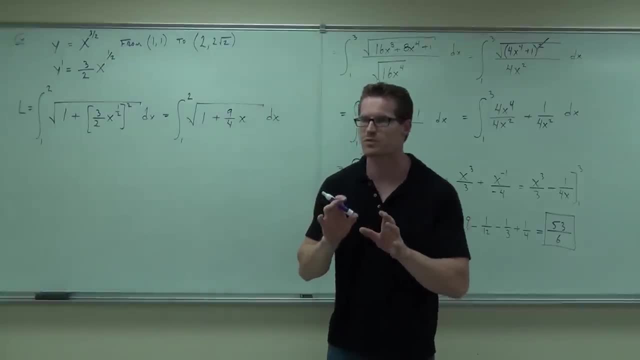 1 to 3.. 1 to 3.. 1 to 3.. 5 to 4.. 3 to 4.. 1 over 5. 0 to 8.. 2. 5 to 8.. 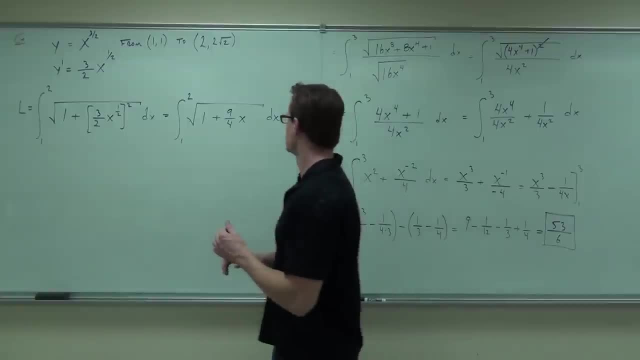 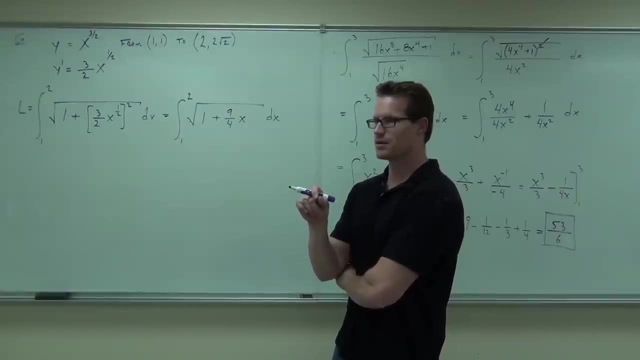 1 to 8.. 0 to 8.. Share a little bit for me. at school, We픇an слово. Say it with a ton, Sure, Sure For you. So you've got family and friends. Why did you go there that? sometimes we take too long like that. you can do a point mine. 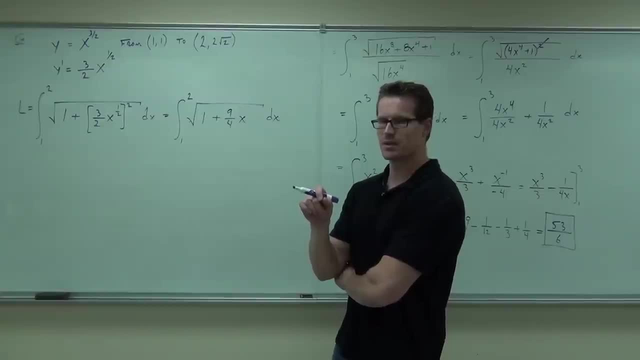 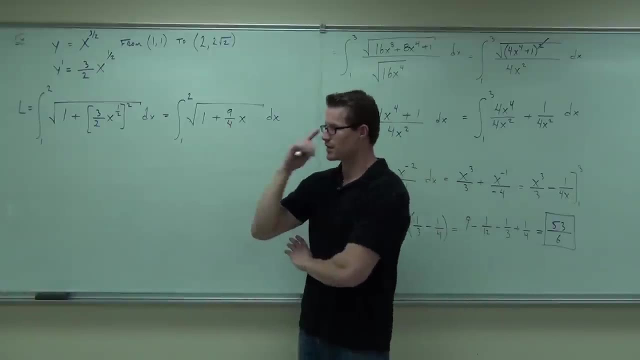 after this. Would you mind if I made it a little easier, Because we can do all that and you're still going to have the same problem. However, I want you to think about this for a second. What does substitution work? Tell me something. 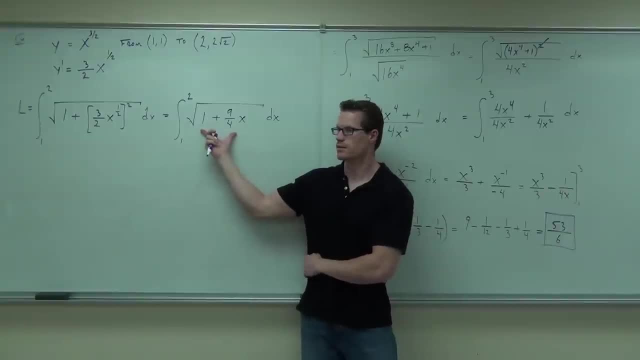 What's the derivative of this whole thing right here? Nine fourths: Do we care about constants when we're doing substitution? So what does substitution work? So don't forget about substitutions. That's going to work. If you found the common denominator, would work out. the common denominator is 4, which. 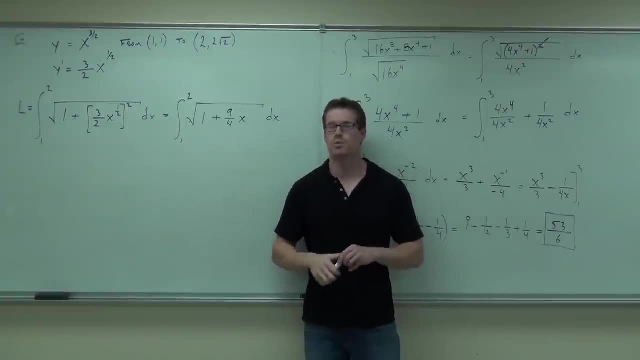 So don't forget about substitutions. that's gonna work If you found the common denominator would work out. The common denominator is 4, which you're going to get is 4 plus 9x over 4.. That would be the square root of 2, but you're left with 4 plus 9x. 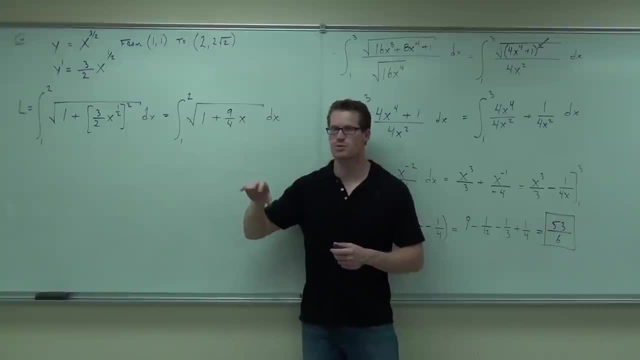 you're going to get is 4 plus 9x over 4, that would be the square root of 2, but you're left with 4 plus 9x. You're still going to have think about that for a second. 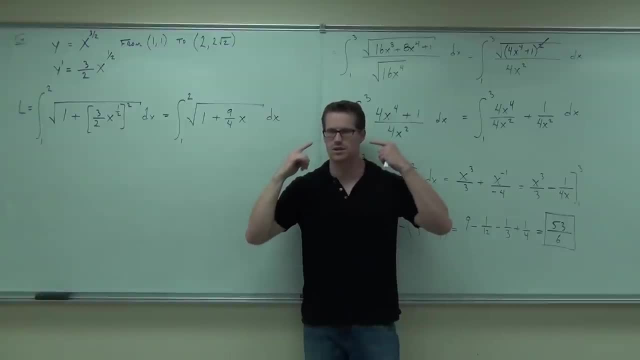 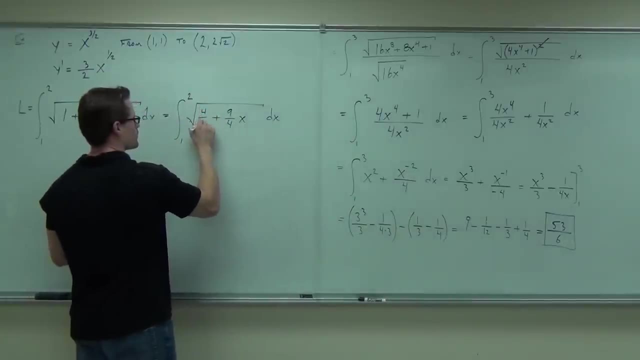 You're still going to have think about that for a second. Please just think of the equation in your head. If you find a common denominator, you have 4 over 4.. Write it if you want. You have 4 over 4 plus 9 fourths, right. 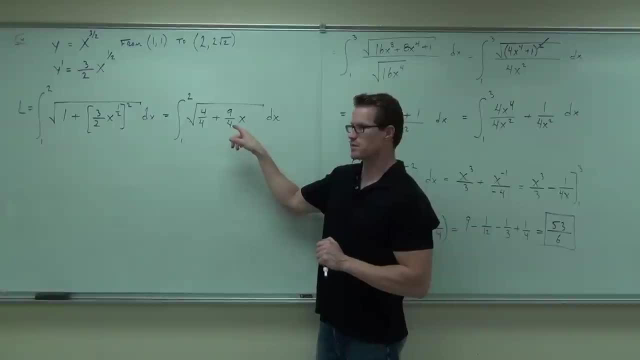 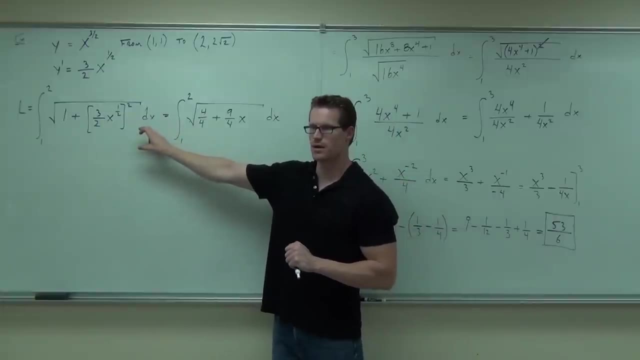 You have that. When you do this, when you do this, you're going to have 4 plus 9x over 4.. Remember, you're going to be pulling out a 2 right there. You clear on that one. You're still going to have the 4 plus 9x in there. 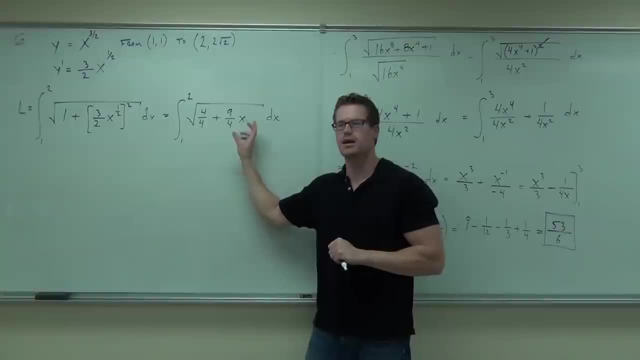 You're still going to need a substitution, where you have to have a constant of 9.. The 9 is going to be somewhere in this problem as well, So we can do a substitution now. It's going to work out exactly the same. exactly the same. 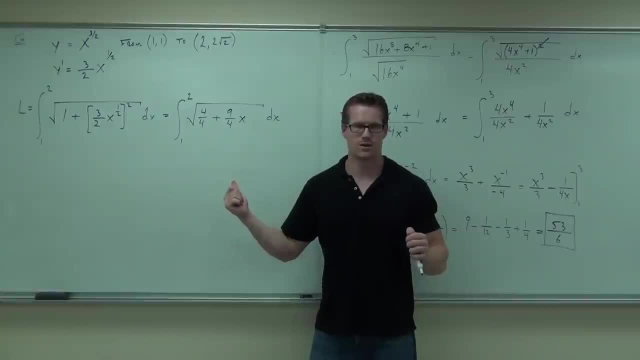 Do you want to see the substitution or do you want to do it the other way? You're going to have a substitution either way. Do you see why you're going to have a substitution either way? Yeah, Let's do it. I think so. 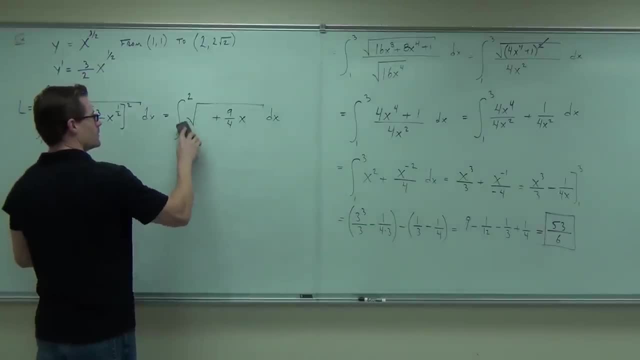 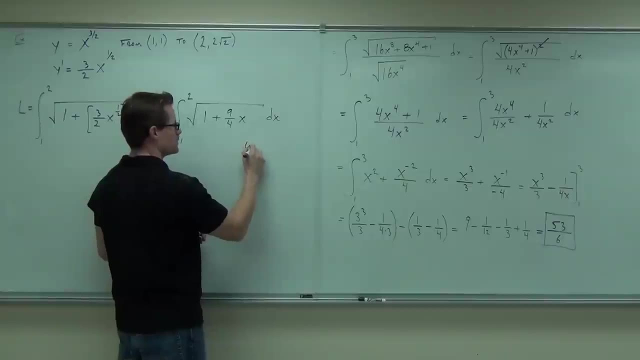 Shouldn't it be 2 root 2?? Well, explain to me why that's not the case. Someone else explain why I have a 2 and not a 2 root 2.. Because the 2 is the x and it's in terms of x. 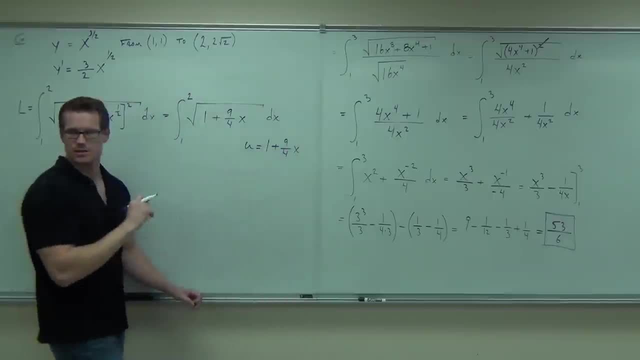 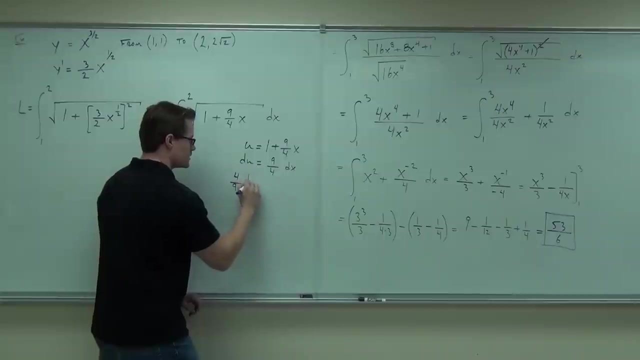 Very good, Did that make sense? If we have du equals 9 fourths dx, if we reciprocate it, we get 4 ninths du equals dx. du equals dx. Well, let's keep going with that, That's great. 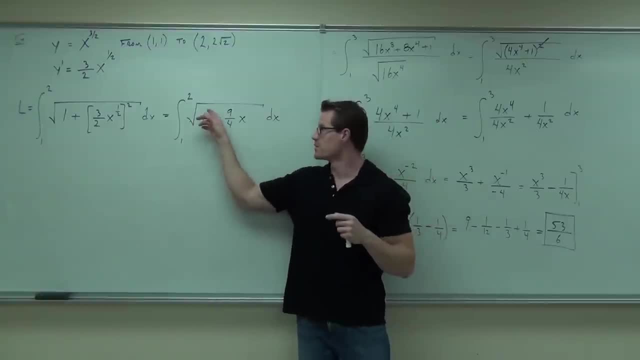 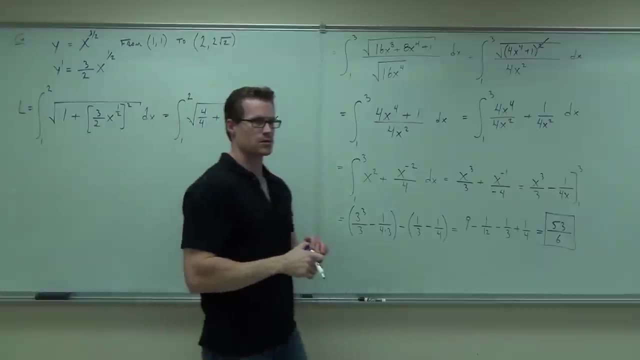 Please just think of the derivative in your head. If you find a common denominator, you have 4 over 4, write it if you want. you have 4 over 4 plus 9 fourths. right, You have that. When you do that, you're still going to have the same problem. 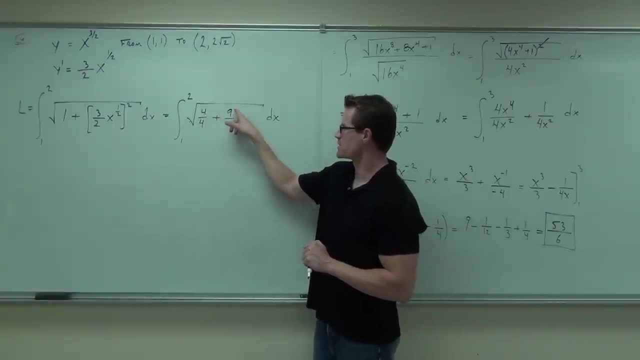 When you do this, when you do this, you're going to have 4 plus 9x over 4, you're going to be pulling out a 2 right there. you clear on that one. You're still going to have the 4 plus 9x in there. you're still going to need a substitution. 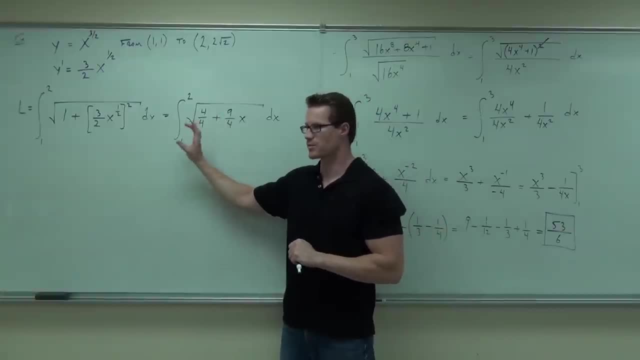 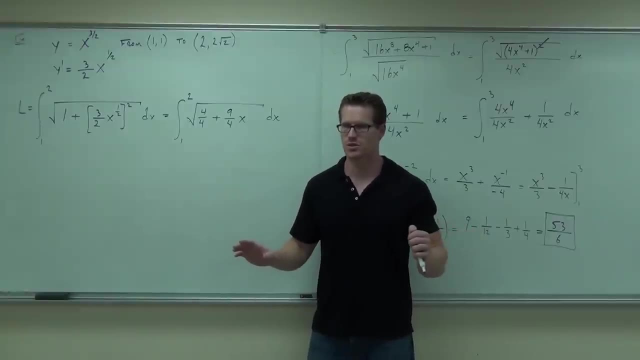 where you have to have a constant of 9, the 9 is going to be somewhere in this problem as well, So we can do a substitution now. it's going to work out exactly the same. exactly the same. You want to see the substitution or you want to do it the other way. 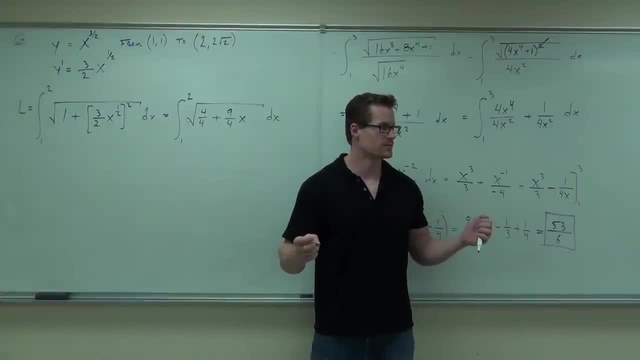 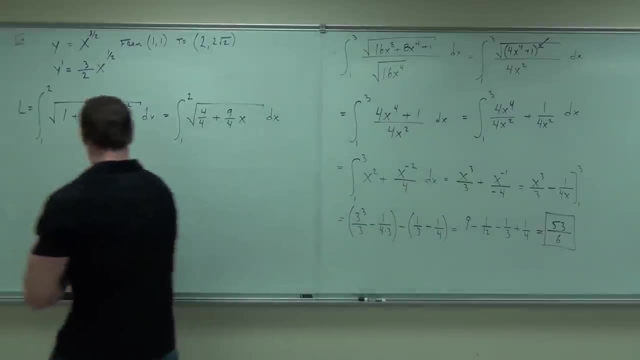 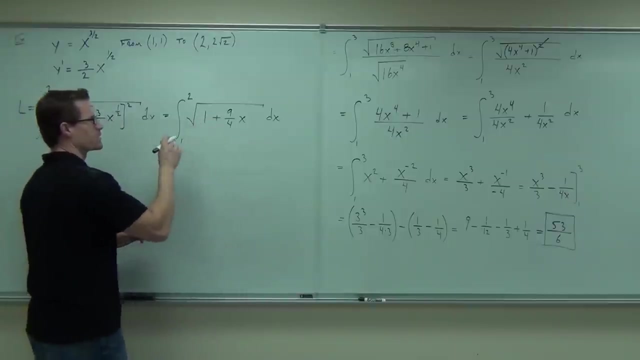 You're going to have a substitution either way. Do you see why you're going to have a substitution either way? Yeah, I think so. Well, explain to me why that's not the case. Someone else explain why I have a 2 and not a 2 root 2.. 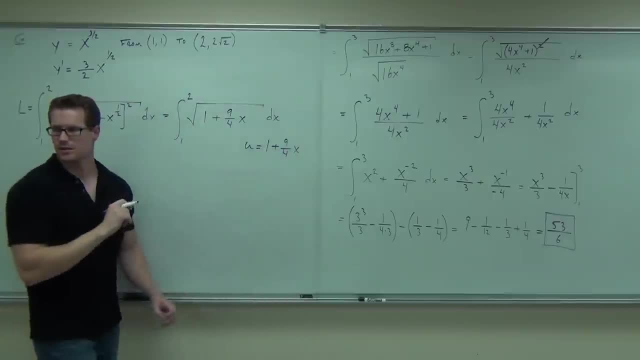 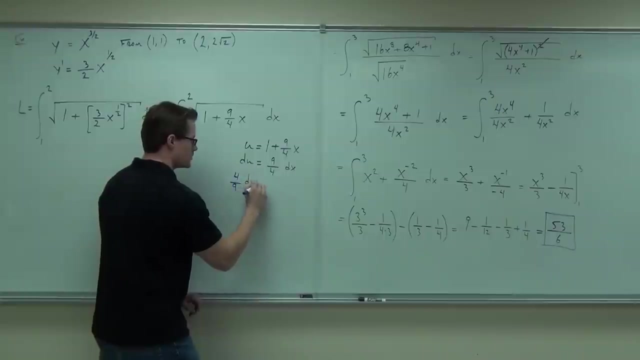 Very good, Did that make sense, Thisustingrn-dy? And then this is going to be- let's call it glial. I'm going to have out objective of non-negative, of non-negative, of non-negative. 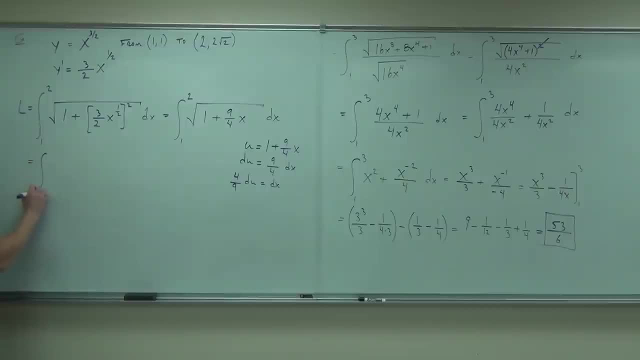 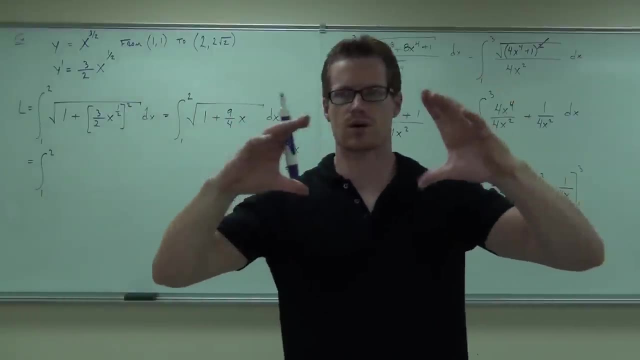 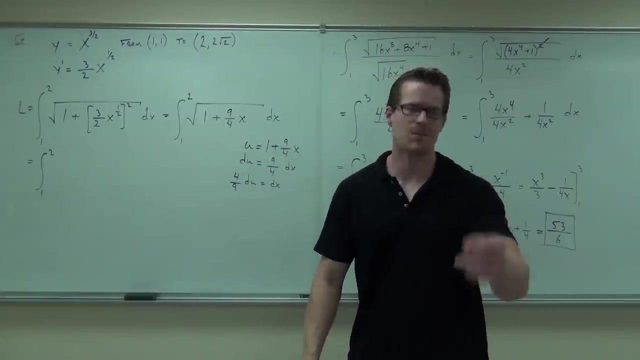 You see, there it got confused. It's going to be negative of non-negative Ratio of the inevitable, of Zurich's integral z to the value of a, 1 minus h plus one minus h minus. It's not going to be negative. Now what you want to estimate the excel equation for your employers statement, or what would? 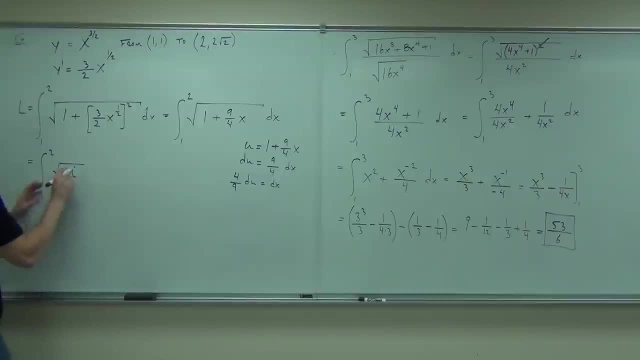 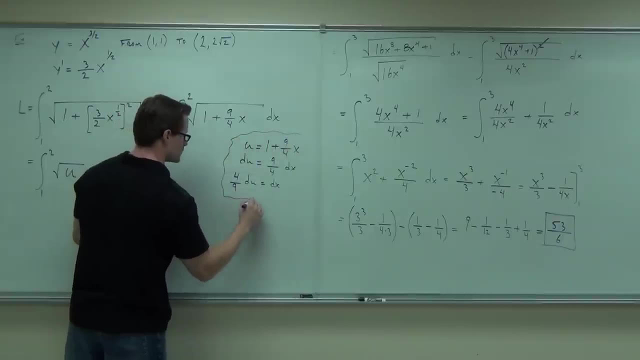 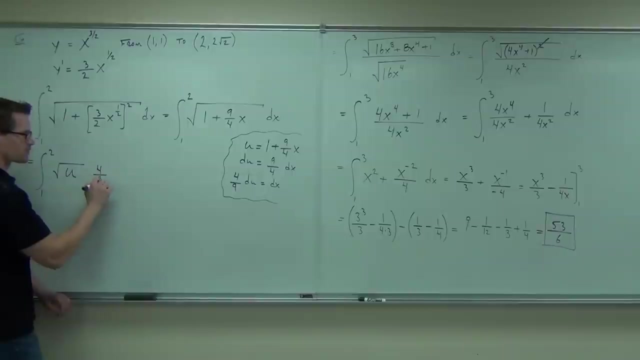 be it. Just so you see where it's coming from: The square root of u, that's our entire u, from right here. Also, we have instead of dx. what are we going to put? Don't forget the 4- 9ths. 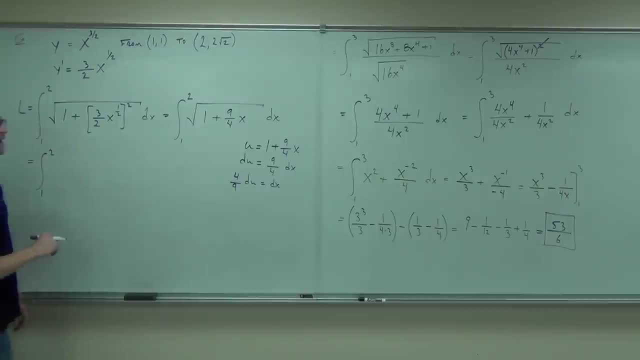 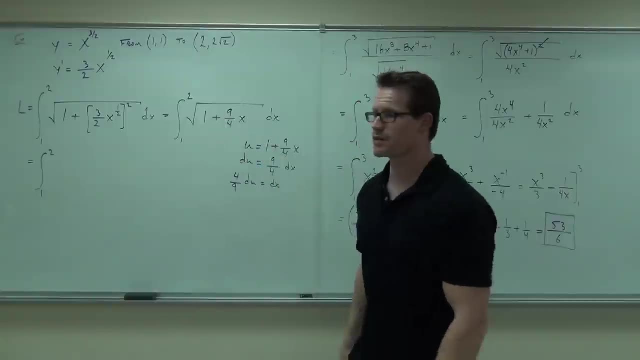 We've got 1 to 2.. We've got what was our. u Use the whole thing, So what's our integral become if I take u to be 1 plus 9, fourths x? Say what I'm going to leave it the square root of u for right now. 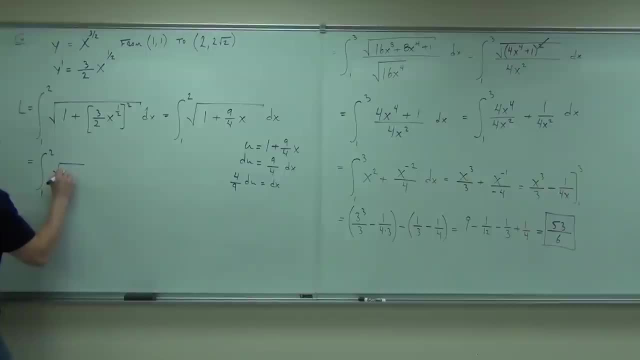 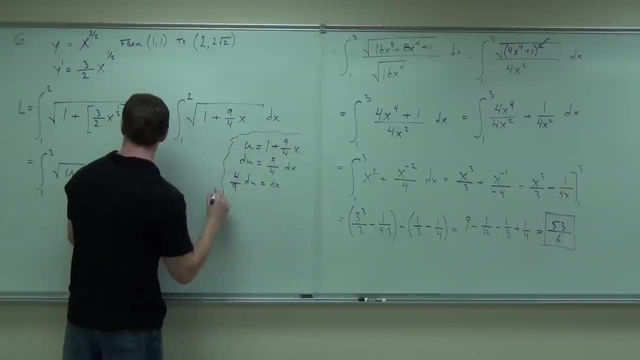 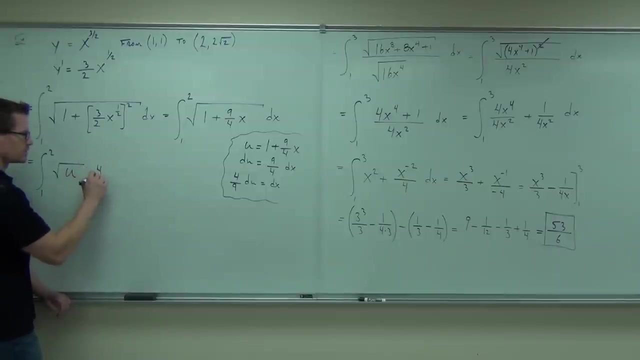 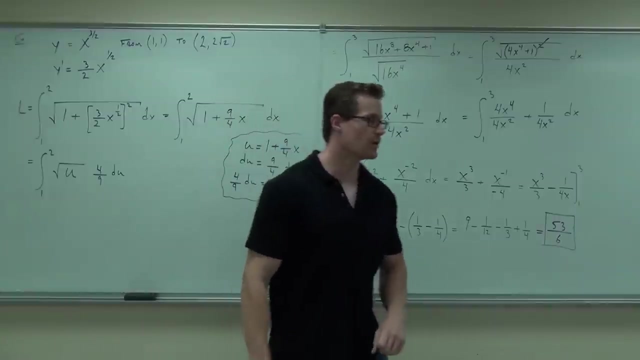 But we have the square root, just so you see where it's coming from. The square root of u, That's our entire u. right here. also, we have, instead of DX, we're gonna put: don't forget, the four nights. do you tell me one more thing? I could do right now if I wanted to say: 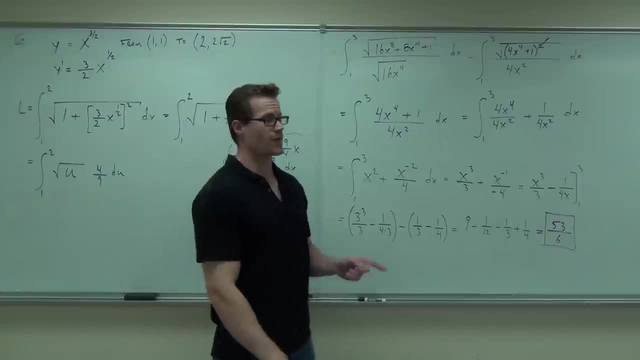 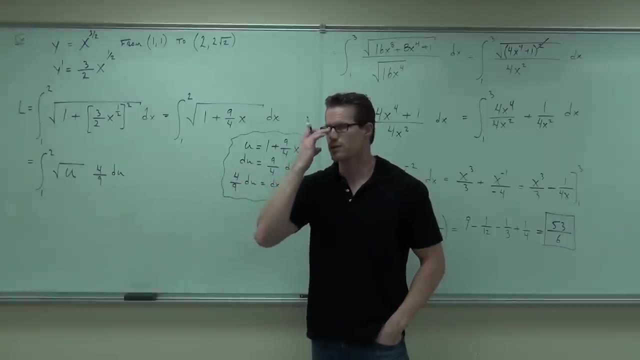 du, Tell me one more thing I could do right now if I wanted to Say what? Yes, I could pull the 4 9ths out. What else? Change the bounds? I could change the bounds. Remember, with substitution you can change the bounds. 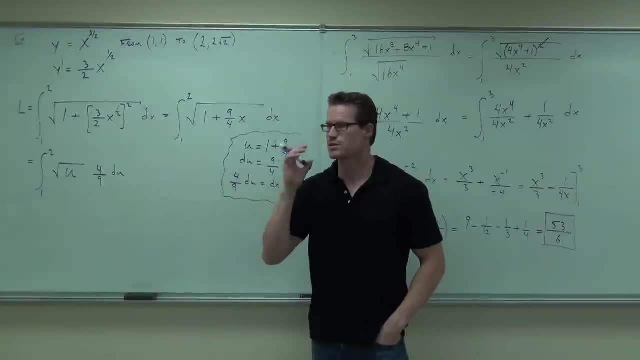 what? yes, I could pull the four nights out. what else I could change the balance. remember the with substitution you can change about. do you want to do that now? do you want to do it later? if I don't change the balance now, if I leave it one, 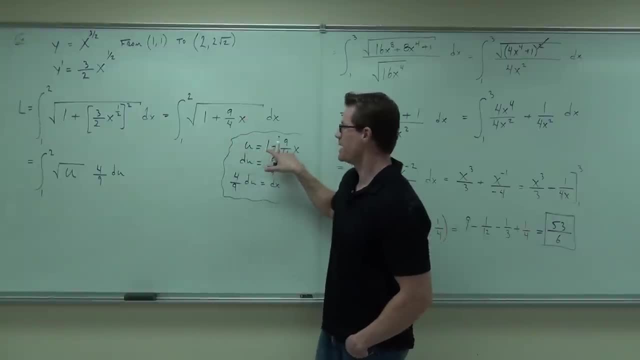 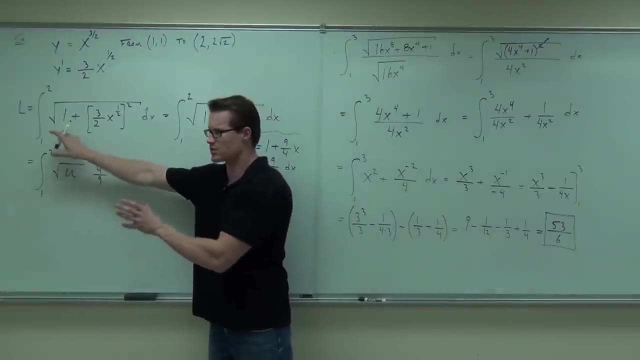 two notice. I will have to plug this back into you before I evaluate. do you remember doing that? so it's one of the other. you either leave it like it is. it's kind of not correct because you're saying X's and use, then do the whole. 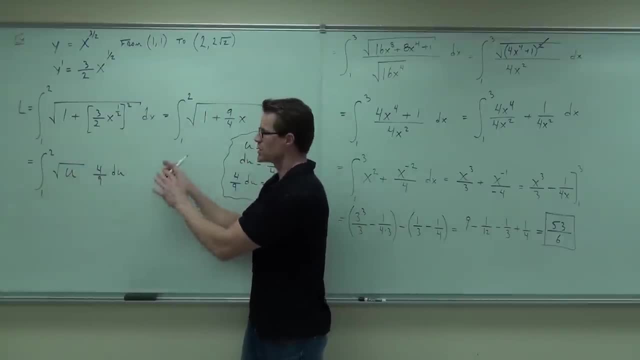 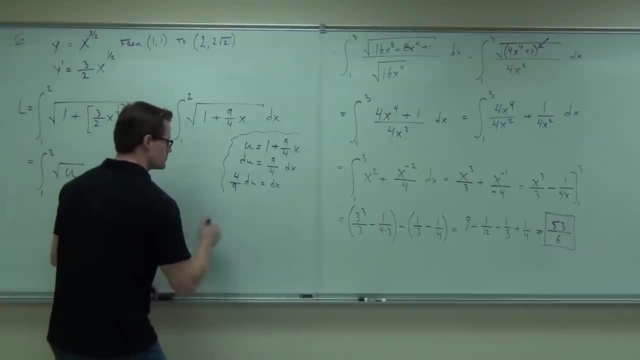 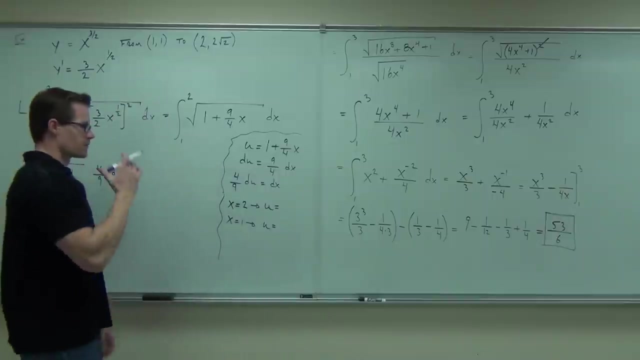 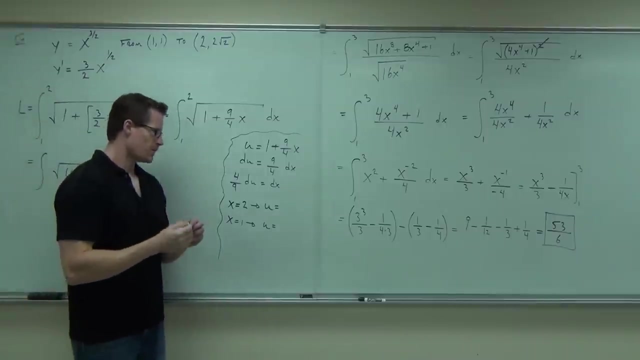 integral and then plug this back in. that's okay. or you can change the balance now and we're going to change two and one to something else. let's try that. so changing bounds. so I'm gonna race this real quick. when X is 2, how much do we get for you? 11 over. 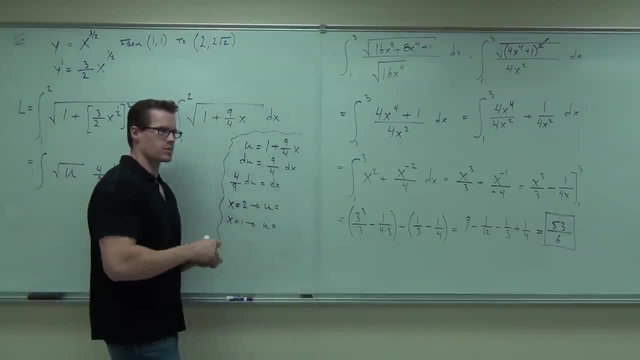 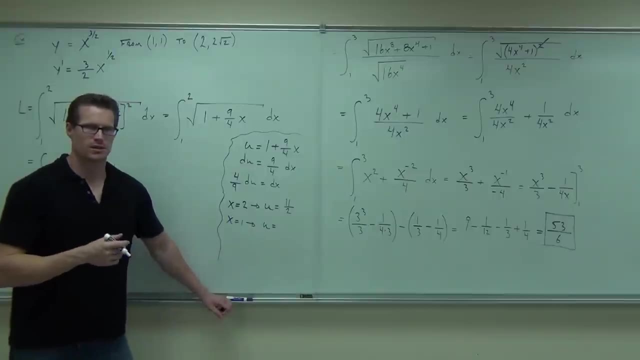 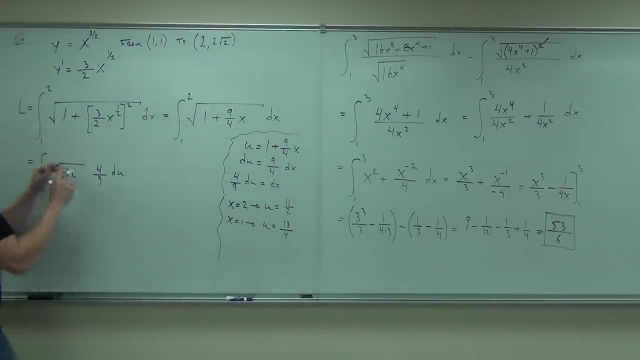 2. okay, let me get a double check on that as well. how about, when you go in, X is 1? how much do we get? perfect, make sure these go the right spot. so for the two instead of two. we've just changed our balance. basically, what you do is you take your two, you plug in for your X, it's going to give. 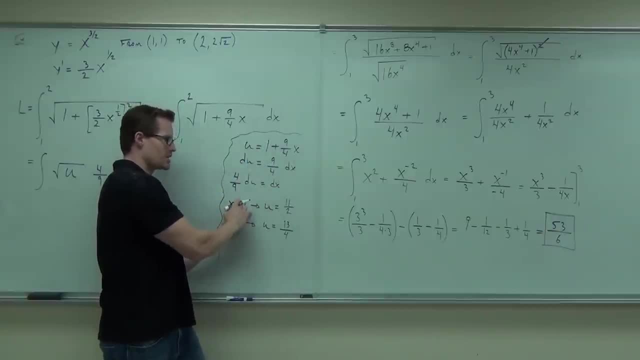 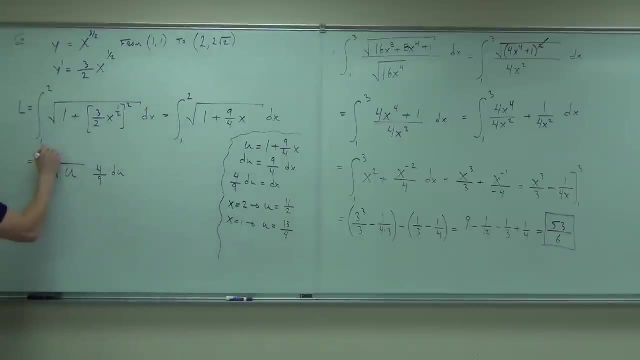 you out a you. so our two became 11 over 2. same thing here. we plug in our one gives you out. our one became 13 over 4. 1 and we're going to do it, Sarah says. she said let's pull the four nights out. I. 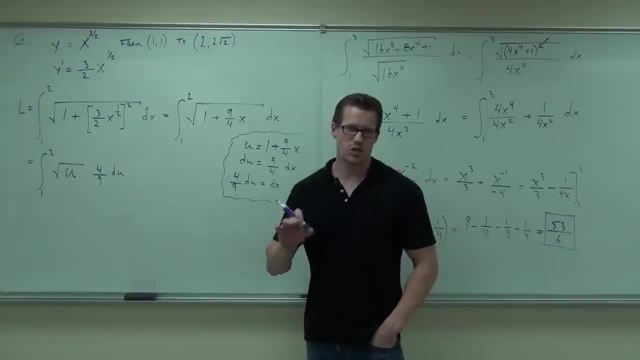 Do you want to do that now or do you want to do it later? If I don't change the bounds now, if I leave it 1,, 2, notice, I will have to plug this back into u before I evaluate. Do you remember doing that? 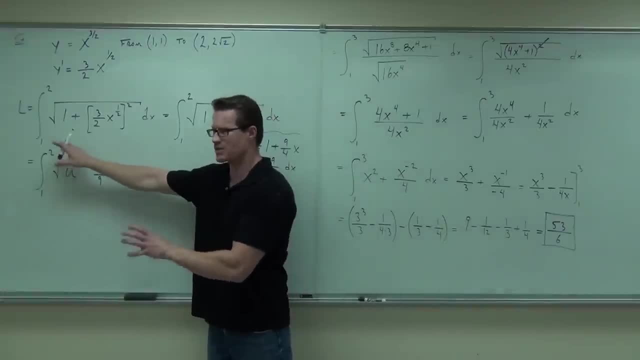 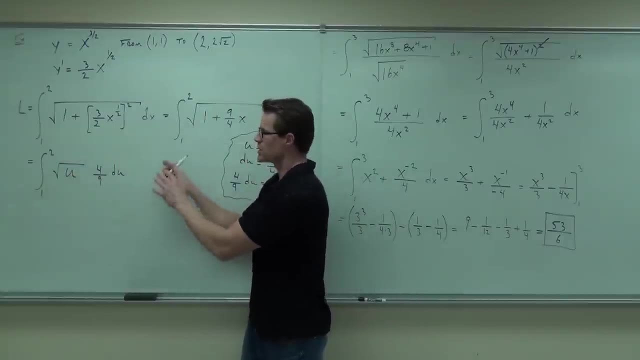 So it's one or the other. You either leave it like it is- it's kind of not correct because you're saying x's and u's, then do the whole integral and then plug this back in. that's okay- Or you can change the bounds now, and we're going to change 2. 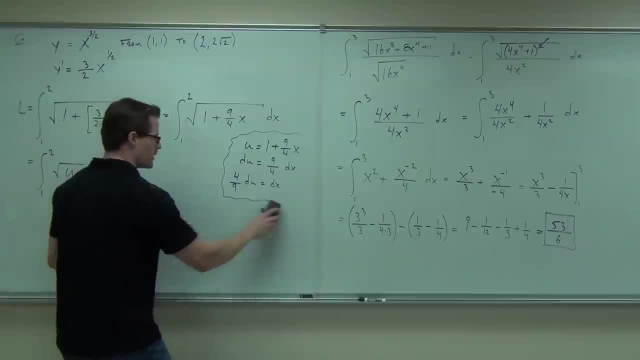 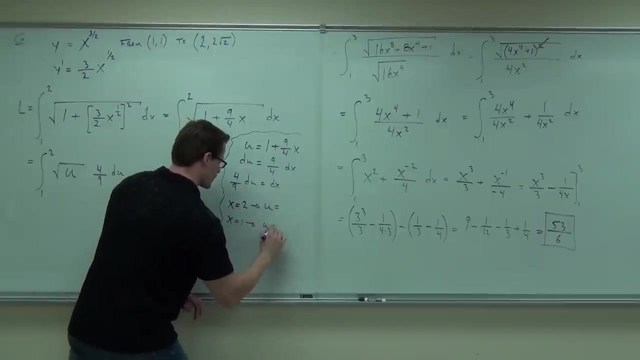 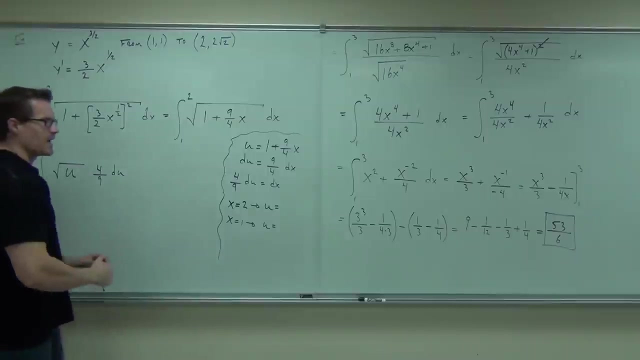 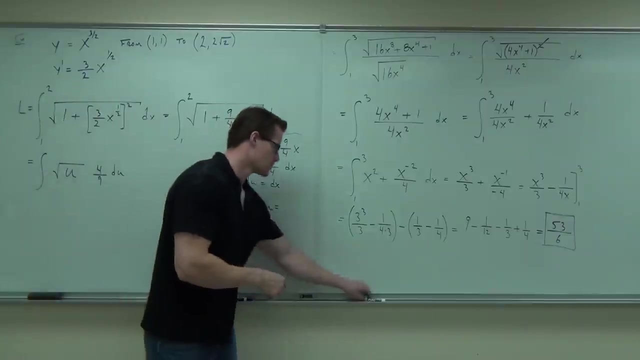 and 1 to something else. Let's try that. So changing bounds. So I'm going to erase this real quick. When x is 2, how much do we get for u? 11 over 2.. Okay, Let me get a double check on that as well: 11 over 2.. 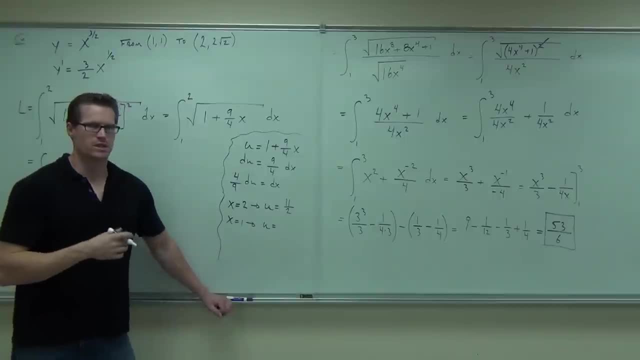 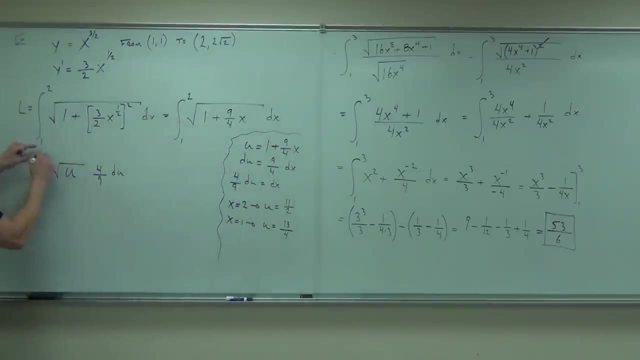 Yeah, How about when u, when x is 1, how much do we get 13.. Perfect, Make sure these go in the right spot. So for the 2, instead of 2,, we've just changed our bounds. 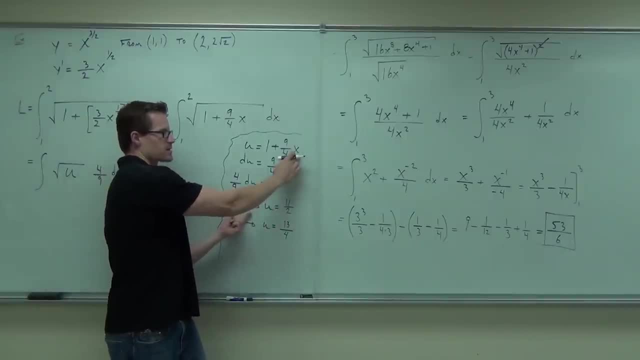 Basically what you do is you take your 2, you plug it in for your x. it's going to give you out a u. So our 2 became 11 over 2.. Same thing here: You plug in our 1, it gives you out a u. our 1 became 13 over 4.. 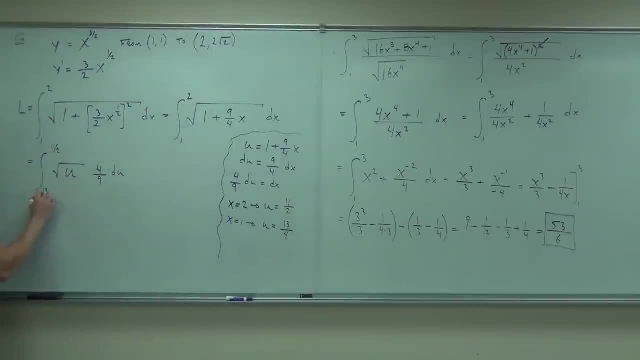 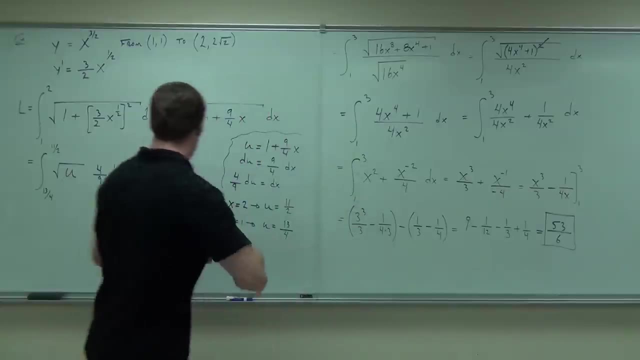 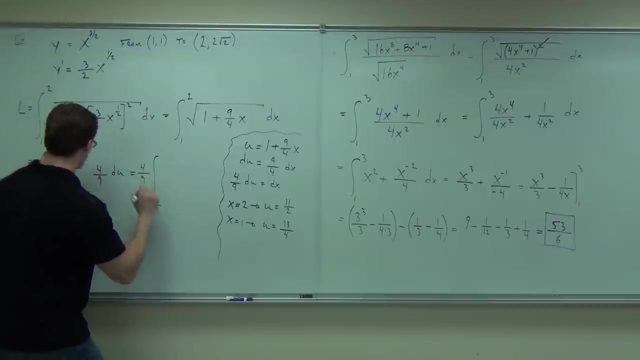 Now I'm going to do what Sarah said. She said: let's pull the 4 ninths out. I like that. So we're going to have 4 ninths, integral, from 13 over 4 to 11 over 2.. 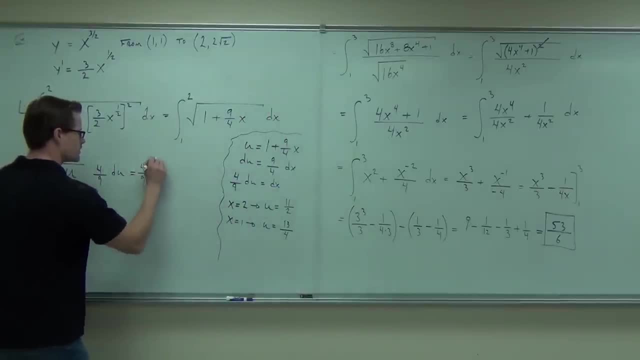 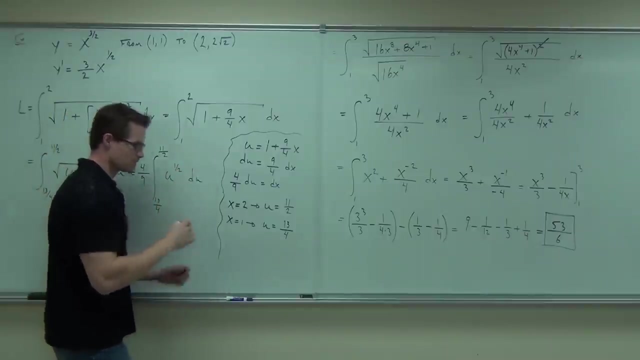 like that. so we're going to have four nights integral, from 13 over 4 to 11 over two, and I'm going to do with Joseph which said: change the square root of you to use one half for you. hey, hard integral, easy integral. what do you think? 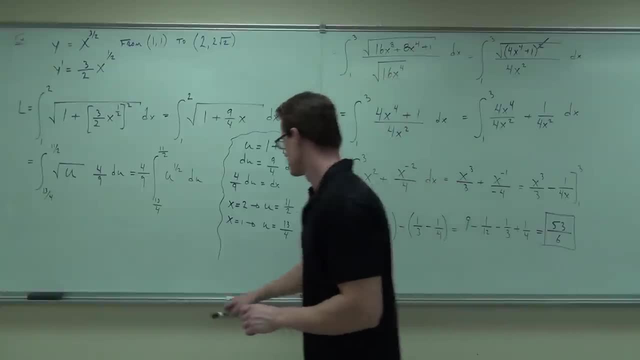 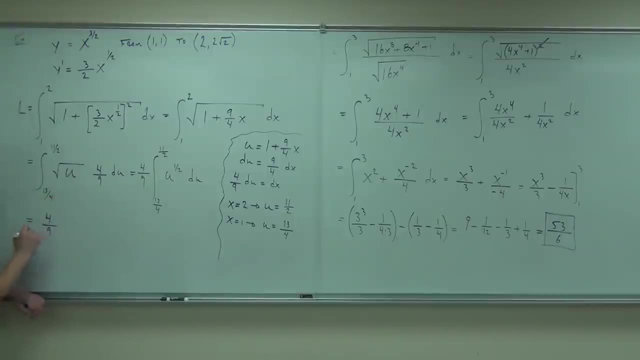 Pretty easy, Pretty easy, yeah, So we'll have the four-ninths. Don't lose that four-ninths. We have u to the three-halves over three-halves. I'll evaluate in just a minute. Notice that we add one to the one-half. 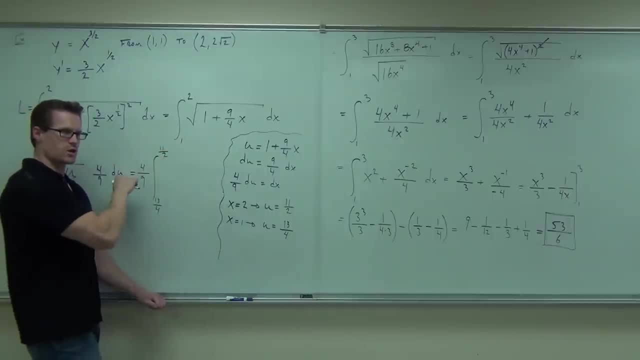 And I'm going to do what Joe said, which said: change the square root of u to u to the square root of x. Okay, So I'm going to do what Sarah said, which said: change the square root of u to u to the square root of x. 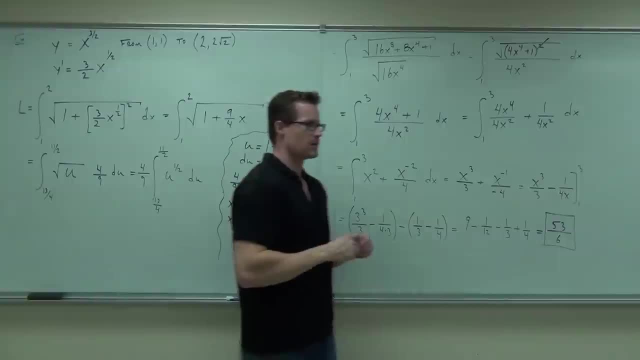 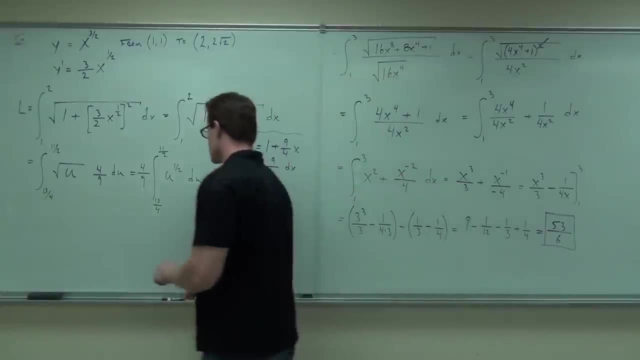 u to the 1 half, The? u Hey hard, integral, easy, integral. What do you think? Pretty easy, Pretty easy, yeah. So we'll have the 4 ninths. Don't lose that 4 ninths. 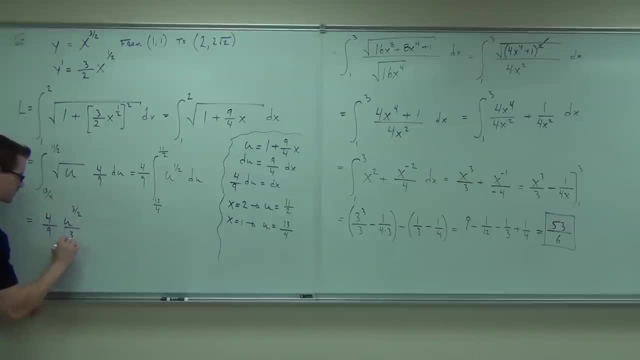 We have? u to the 3 halves over 3 halves. I'll evaluate in just a minute. Notice that we add 1 to the 1 half, you get 3 halves over 3 halves. Be careful on Making this a little bit prettier. you'll have four-ninths times two? u to the three-halves over three. 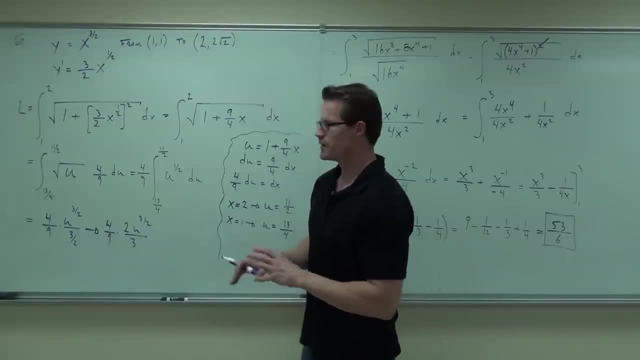 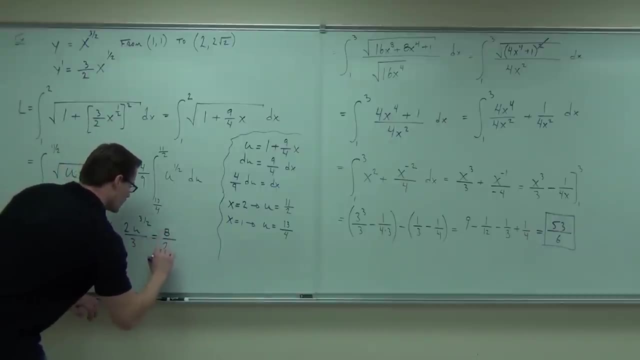 Still okay getting that far. Now we're going to have eight over twenty-seven? u to the three-halves. Do I need to put this back in to this? No, because I changed the balance. It's great. All I want to do is evaluate from some really nasty numbers actually. 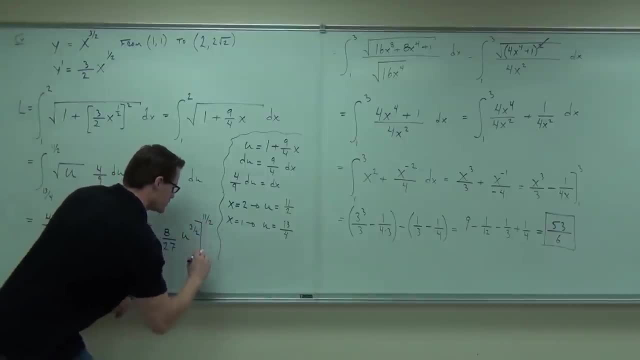 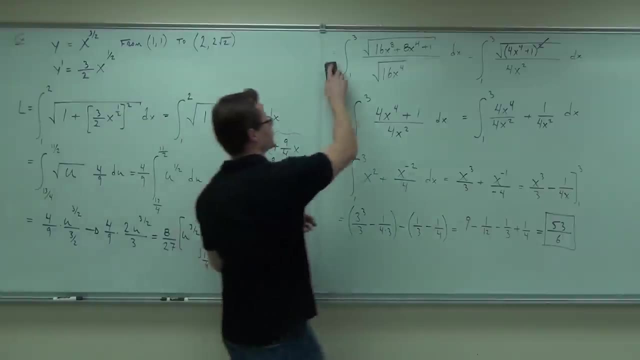 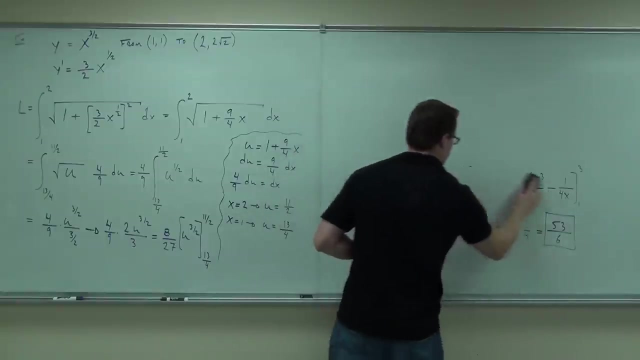 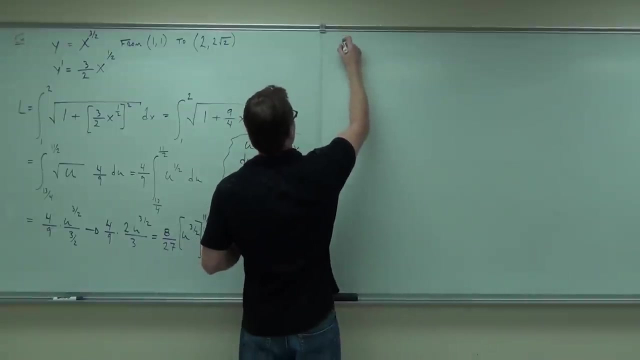 Really nasty numbers. You got eleven over two. you got thirteen over four. Let's see where that thing works out at. So eight over twenty-seven. What do you say? we leave that out in front and don't deal with it for right now. 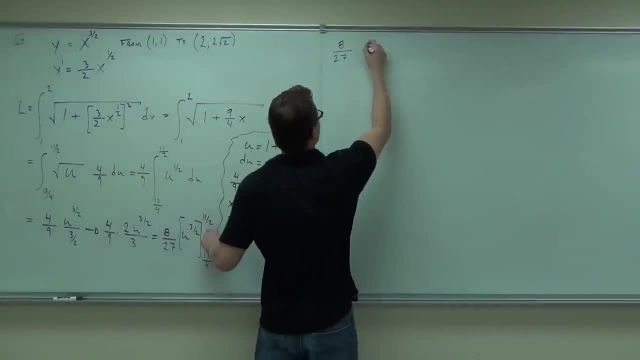 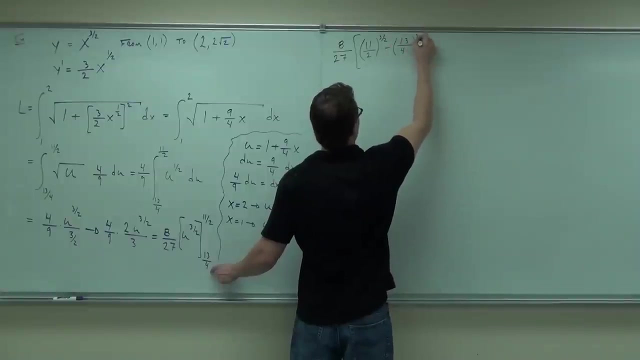 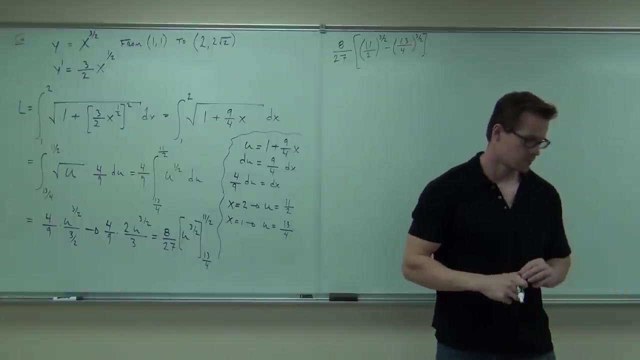 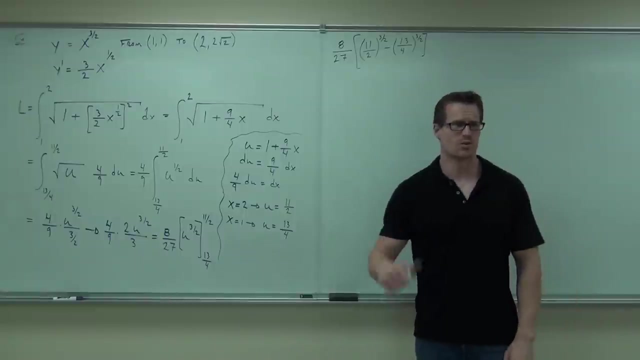 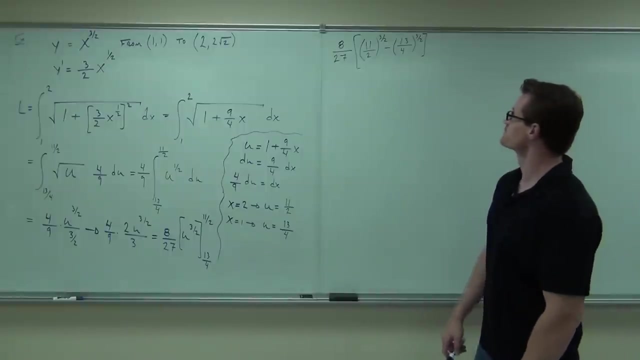 Let's just plug in eleven over two to the three-halves And thirteen over four, Two to the three-halves. Still okay with it? I'm not. It's horrible, It's ridiculous, Oh man. Well, now we get to do eleven to the three-halves over two to the three-halves. 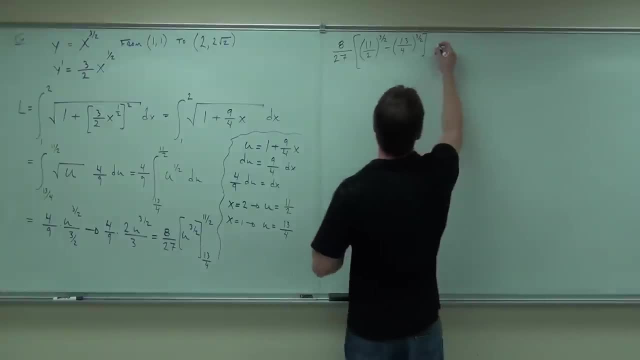 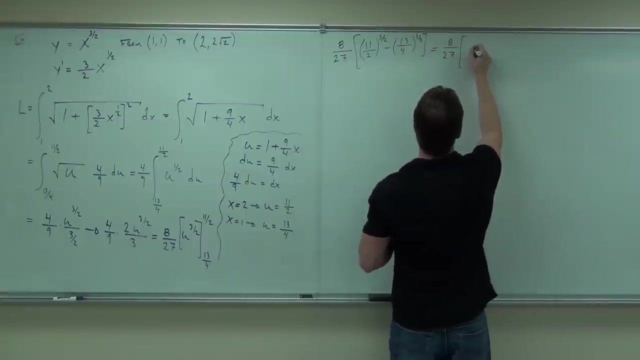 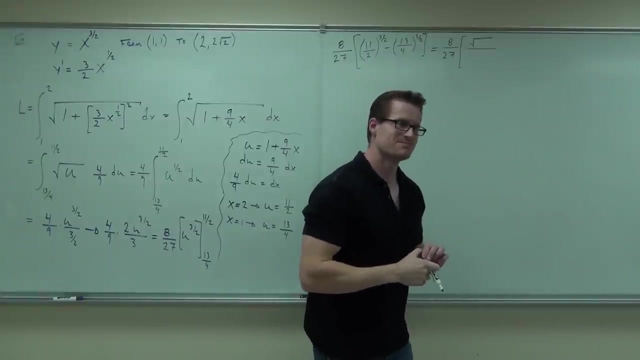 We get to do thirteen to the three-halves over four to the three-halves. Can you give me eleven to the third power please, Because I can't do that in my head. Thirteen to the three-halves. 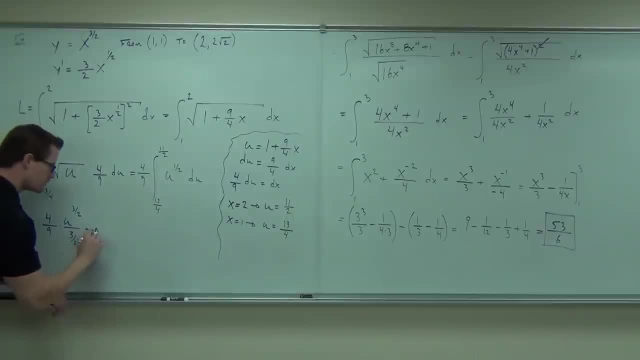 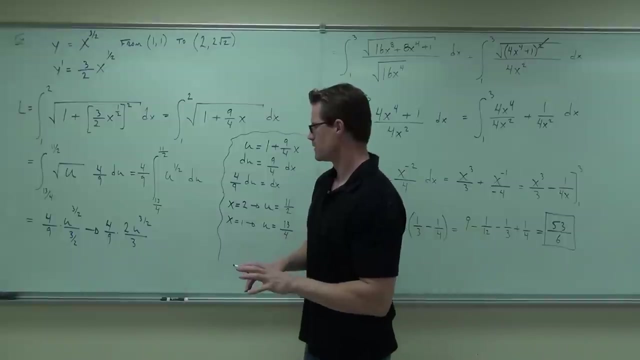 You get three-halves over three-halves. Be careful on making this a little bit prettier. You'll have four-ninths times two? u to the three-halves over three. Still okay, getting that far. Now we're going to have eight over 27.. 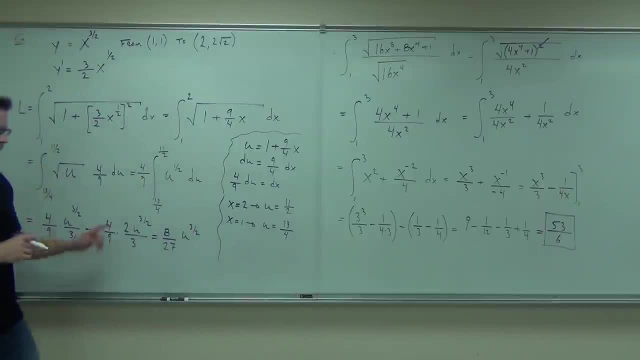 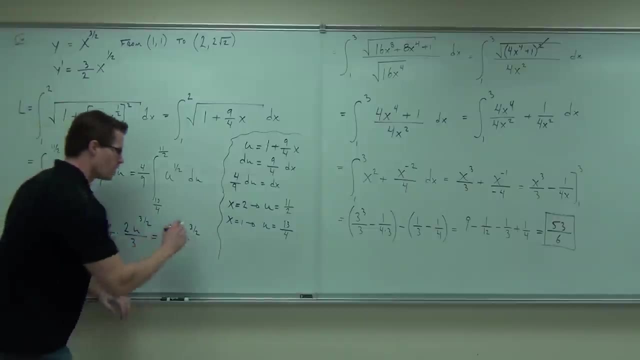 u to the three-halves. Do I need to put this back in To this? No, because I changed the balance. It's great. All I want to do is evaluate from some really nasty numbers, actually Really nasty numbers. 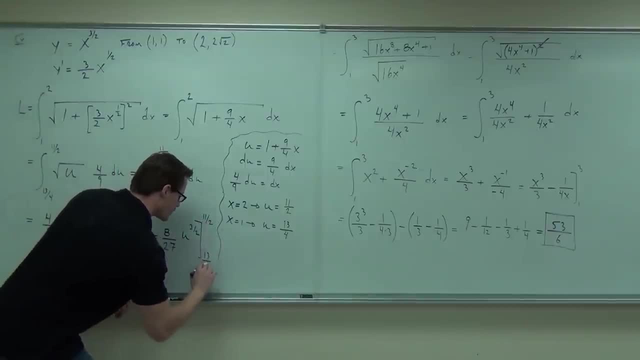 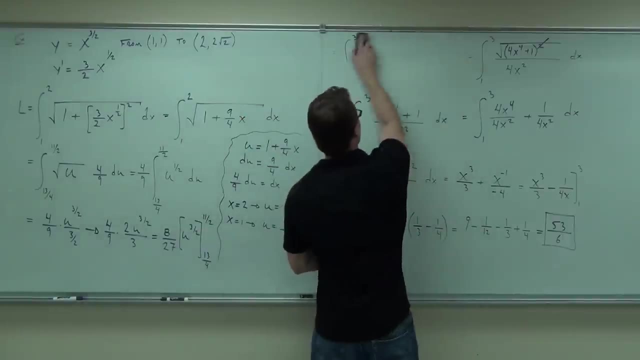 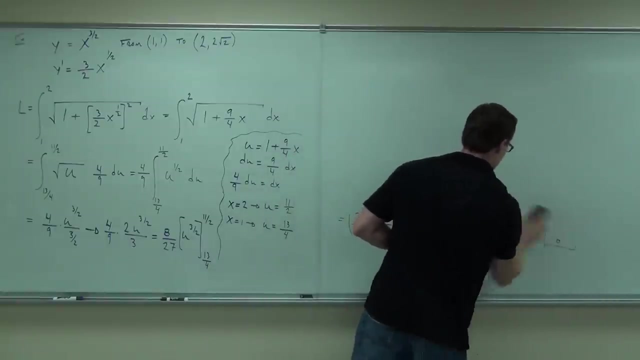 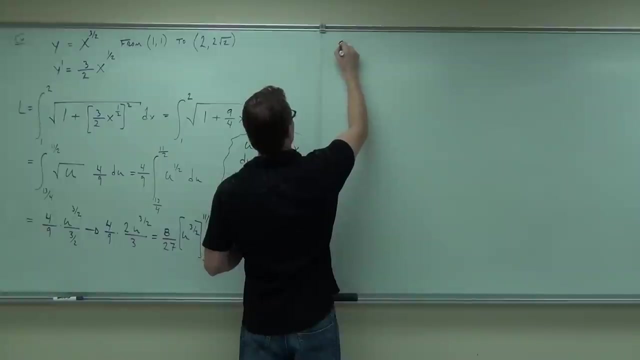 You got 11 over 2.. You got 13 over 4.. Whew, Let's see what that thing works out as So, 8 over 27.. What do you say? we leave that out in front and don't deal with it for right now. 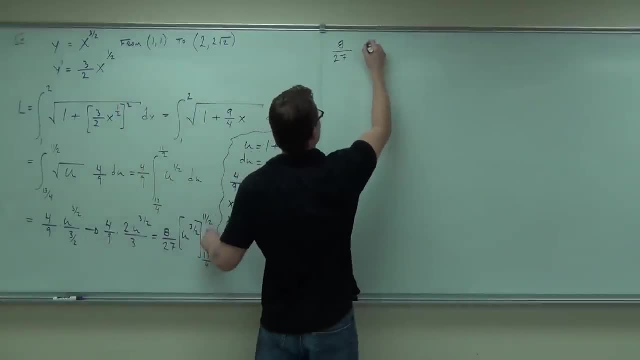 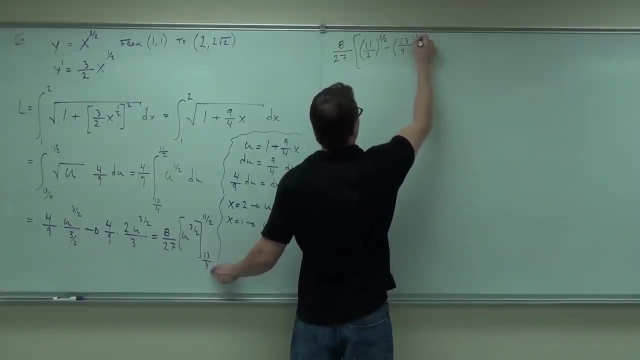 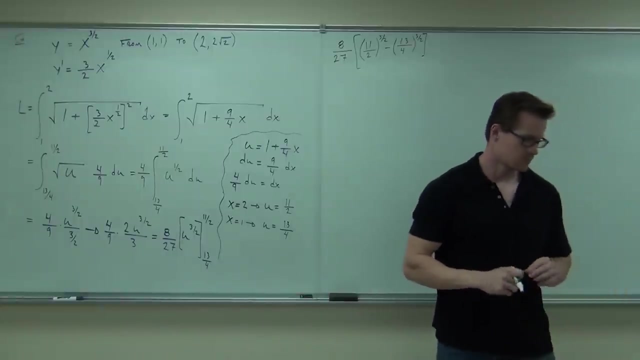 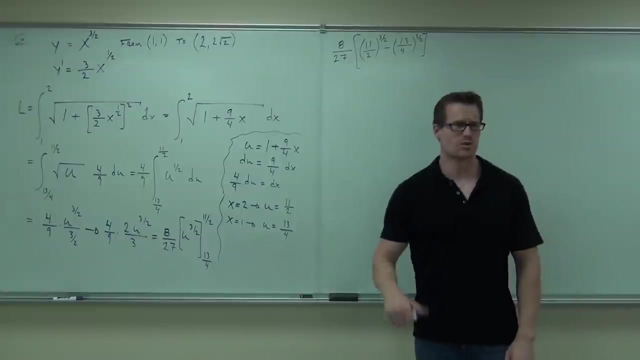 Let's just plug in 11 over 2 to the three-halves and 13 over 4 to the three-halves. Are you still okay with it? I'm not. It's horrible, It's ridiculous, Oh man. 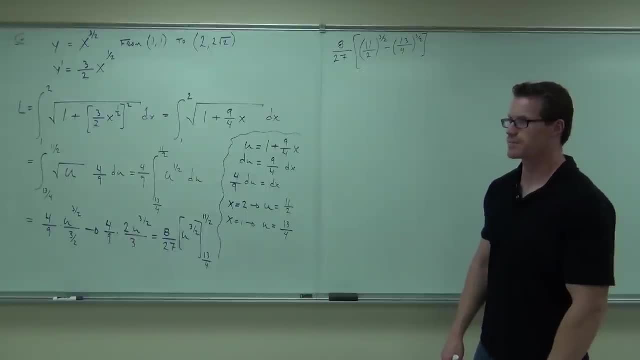 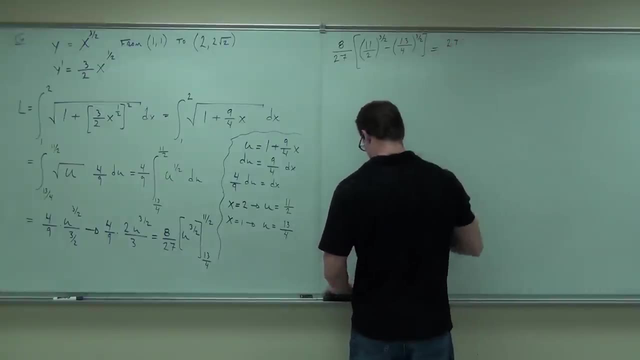 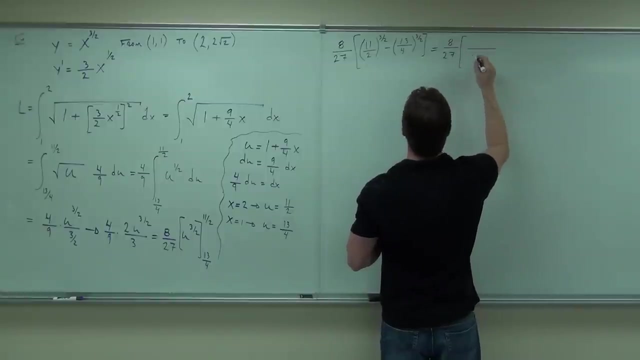 Well, now we get to do 11 to three-halves over 2 to three-halves. We get to do 13 to three-halves over 4 to three-halves. Can you give me 11 to the third power please? 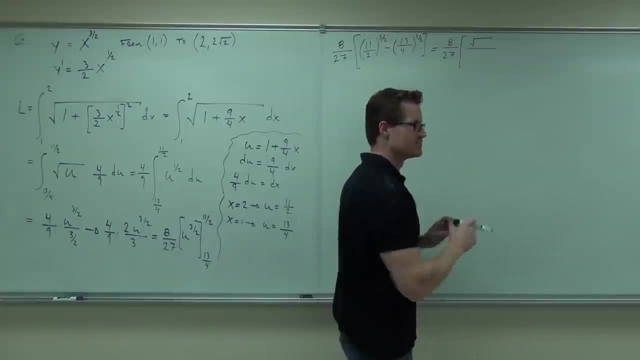 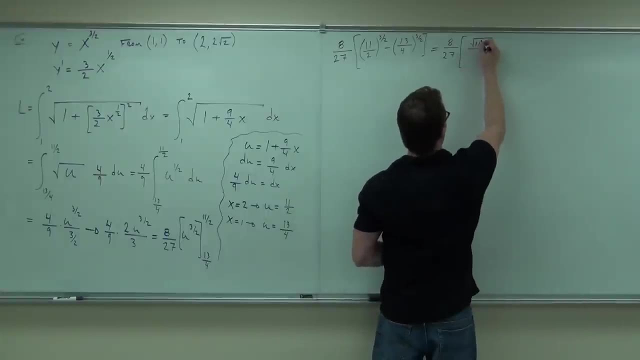 Because I can't do that in my head. 13 to the third power. You know what? Maybe I'll write it like this to keep it a little bit easier. Is it okay if I write it 11 squared times 11 for you? 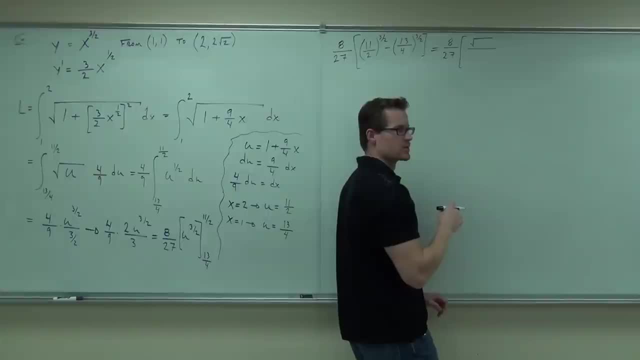 Thirteen to the three-halves. You know what? Maybe I'll write it like this to keep it a little bit easier. Is it okay if I write it? eleven squared times eleven for you? That's still true, isn't it? 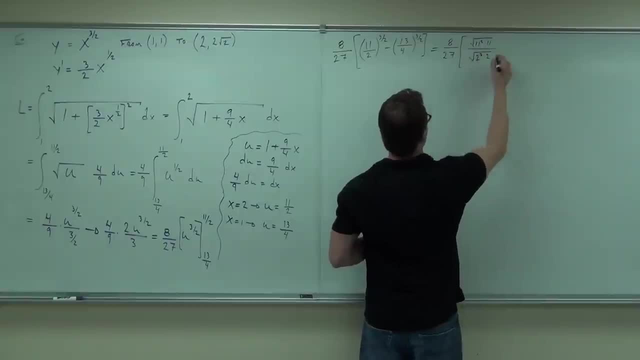 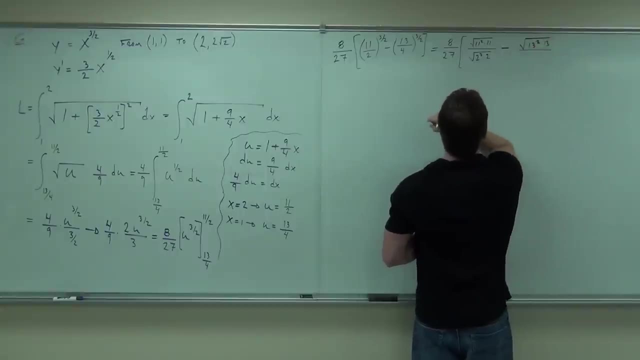 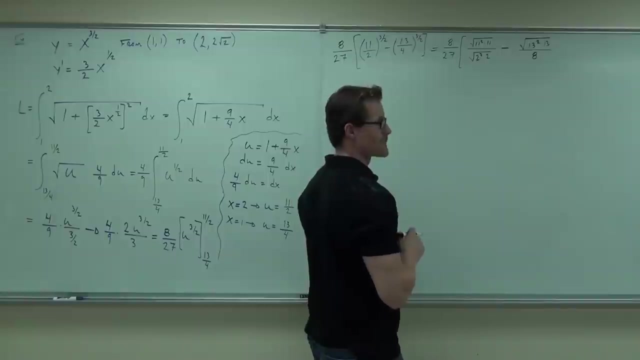 Okay, And I'm going to do the same thing here: Two squared times two minus. I'm going to do thirteen squared times thirteen, And this is just going to be eight. It's like you just pulled that out of your mouth. You can do that if you really want. 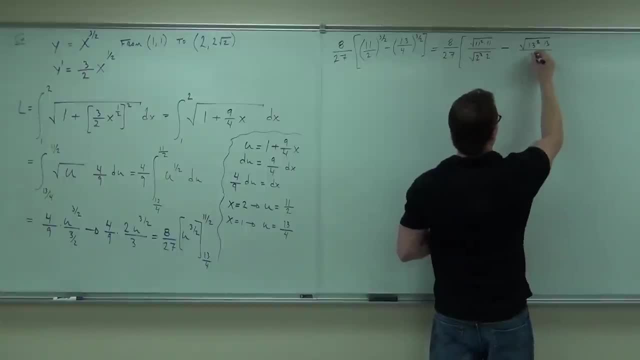 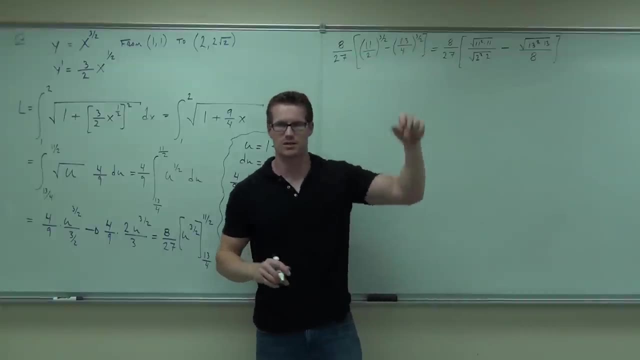 But it's going to be the same thing. It's going to be the same thing. This problem just took a turn for the worse. Isn't that the same thing? Four to the three-halves power squared Four is two. Two to the third power is eight. 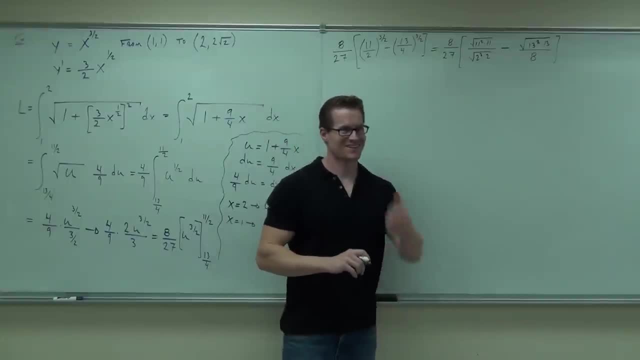 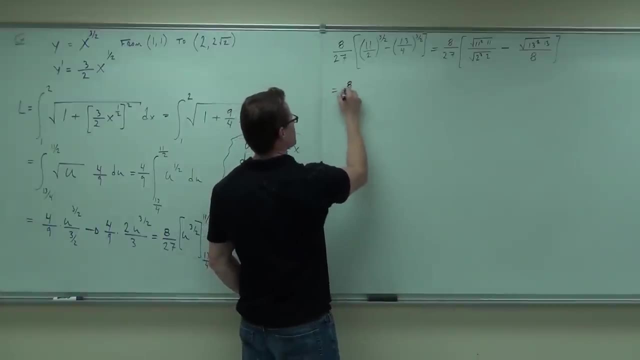 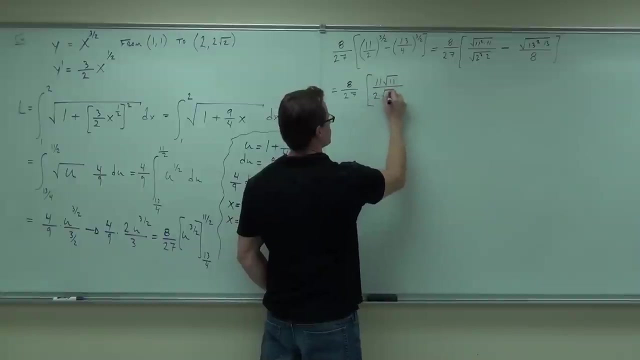 So you get the denominator of eight right there. You still okay. so far. Super duper, All right, Super fun. Okay, Let's see here. So we have eight over 27.. We've got eleven root eleven over two root two. 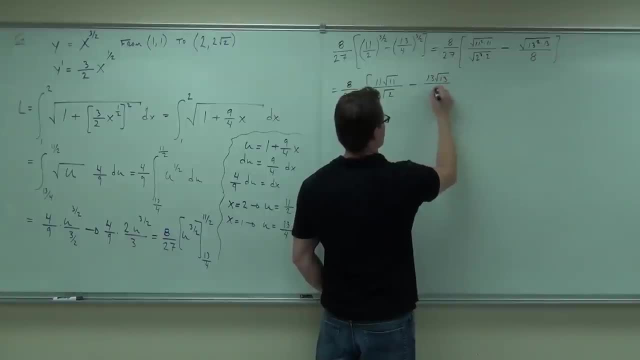 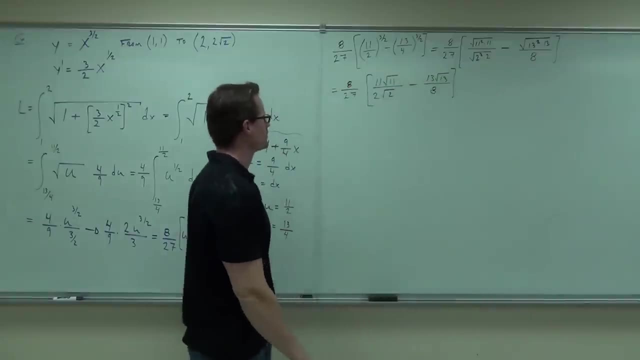 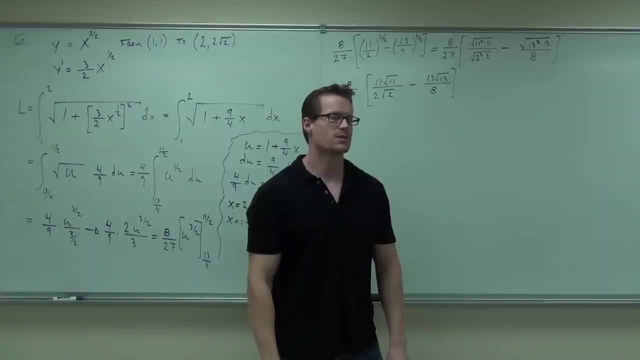 We have thirteen root thirteen, over eight, Awesome, Awesome, Still very cool. How do you get those together? You do Probably the first thing I would do is just deal with this root two. Rationalize that. If I rationalize it, I'll multiply. 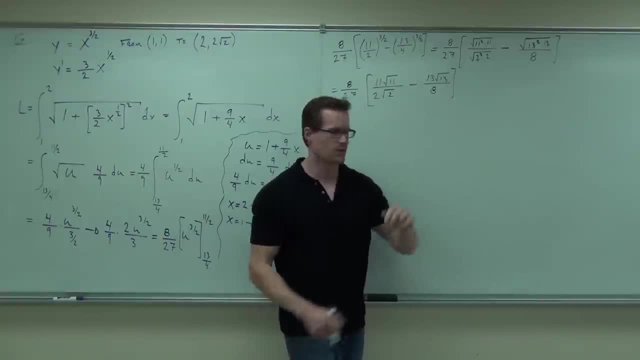 So I'll get the denominator of the root two over the root two, and also four over four to get the common denominator of eight. So I'll show you what I mean by that. Fancy math I suppose, but still basic algebra: Four root two. 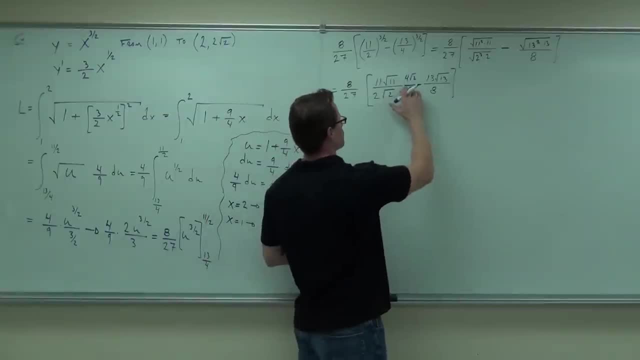 Four root two. Two root five, four, five, four, And it becomes the denominator of eight. I think that will Hang on. Two root two, And don't you always use the same one for your problem? For rationalizing, you don't need to worry about that too. 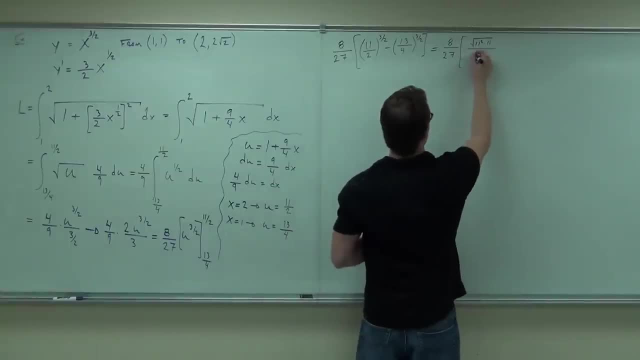 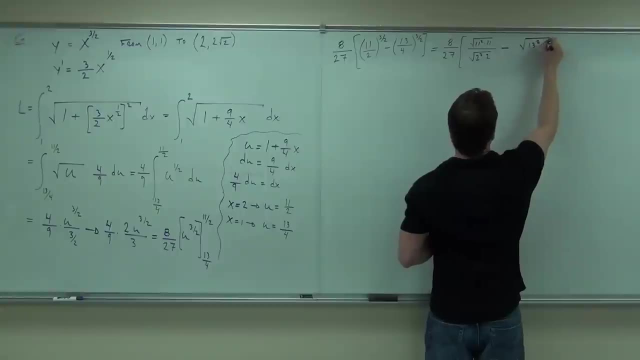 That's still true, isn't it? Okay, I'm going to do the same thing here: 2 squared times 2 minus. I'm going to do 13 squared times 13.. And this is just going to be 8.. 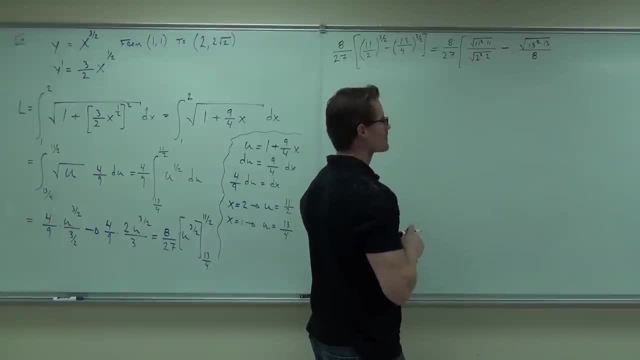 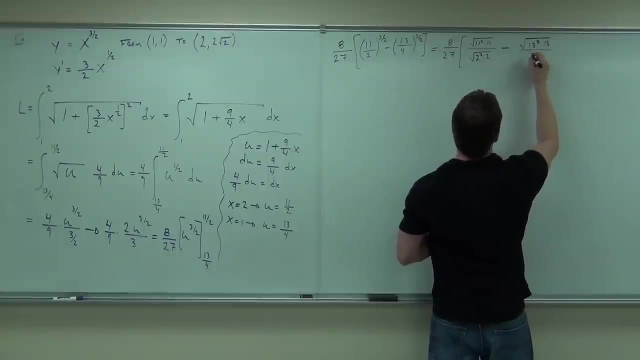 It's like you need to pull that number out of your system. Which one does it belong? You can do that if you really want, All right, But it's going to be the same thing. It's going to be the same thing. 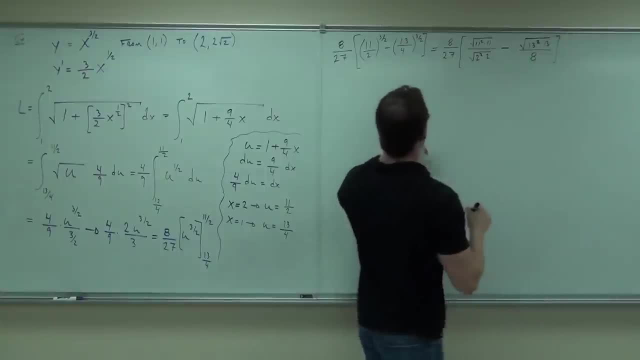 This problem just took a turn for the worse. Isn't that the same thing? 4 to the three-halves power squared, 4 is 2.. 2 to the third power is 8.. So you get the denominator of 8 right there. 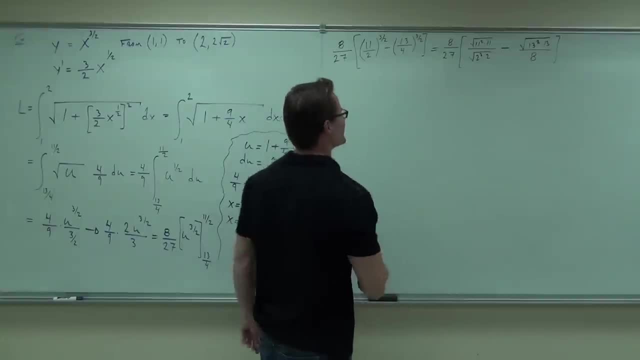 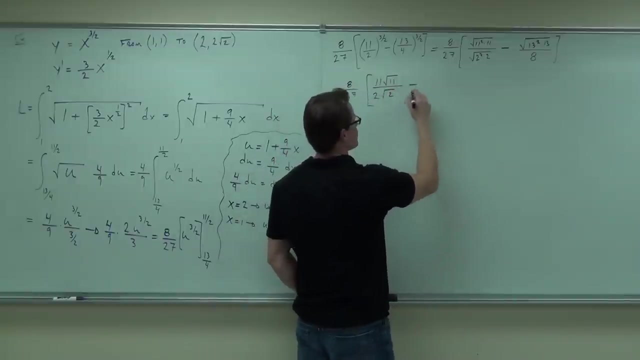 You still okay so far. Super duper, All right, Super fun. Okay, Let's see here. So we have 8 over 27.. We've got 11 root, 11 over 2 root 2. We have 13 root, 13 over 8.. 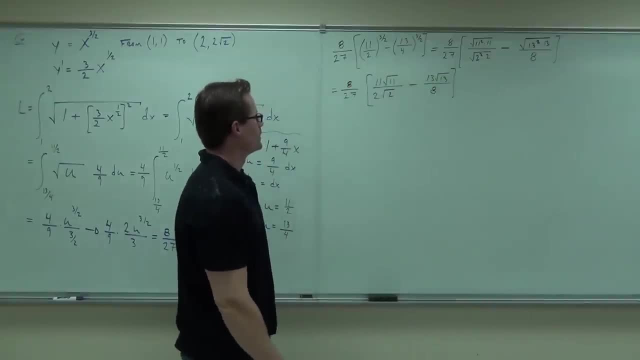 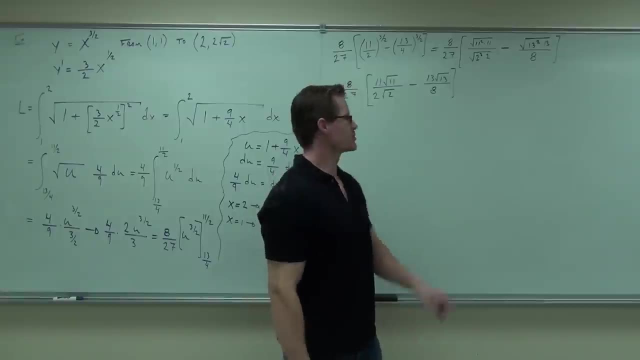 Awesome, Awesome, So very cool. How do you get those together? You do Probably. the first thing I would do is just deal with this root 2.. Rationalize that. If I rationalize, I'll multiply by the root 2 over root 2 and also 4 over 4. 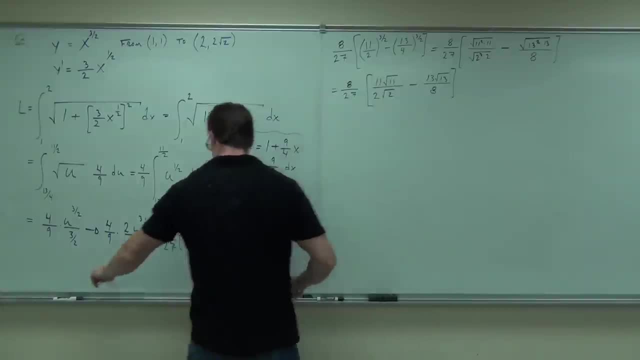 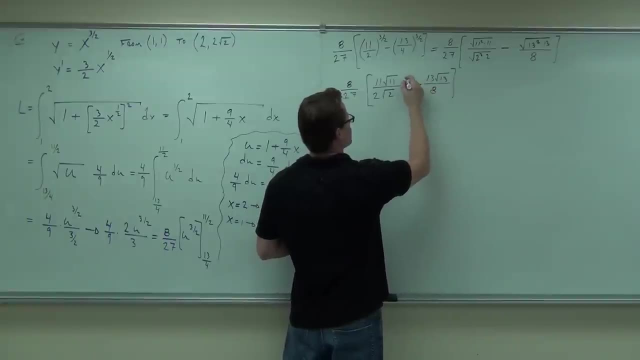 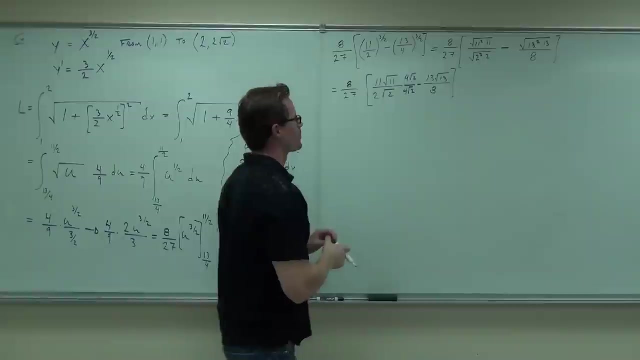 to get a common number of 8.. So I'll show you what I mean by that. Fancy math, I suppose. but still basic algebra: 4 root, 2.. 4 root, 2. 5, 4.. 5, 4.. 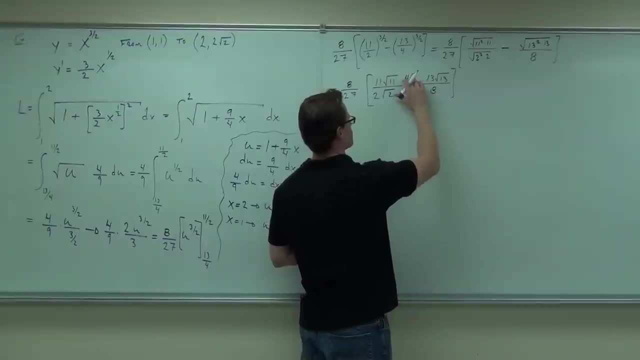 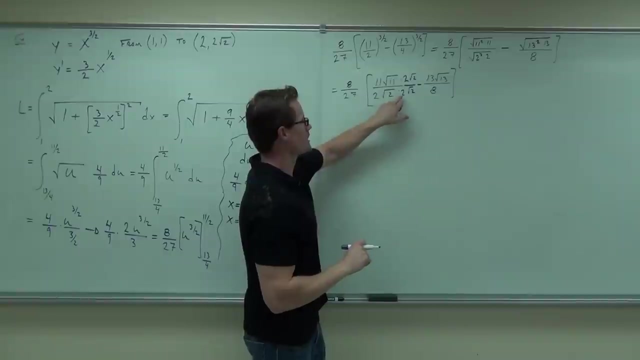 And it comes down to 8.. I think that will Hang on 2 root 2.. All right, Roger, So you're going to use the same one for your problem. You don't For rationalizing, you don't need to worry about that. 2.. 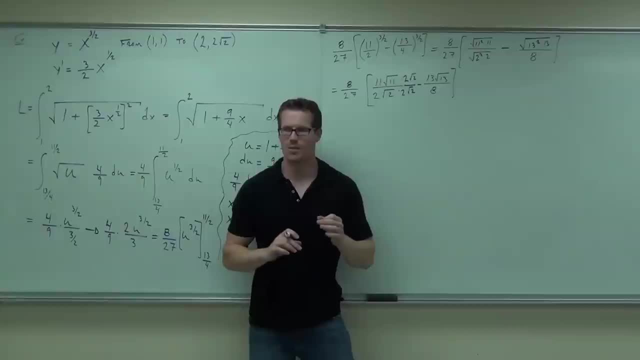 It's just the root two. So rationalizing, it's just the root two. I'm also trying to get a common denominator of eight, though, So I'm going to have two times two, which gives me four times two, which gives me eight. 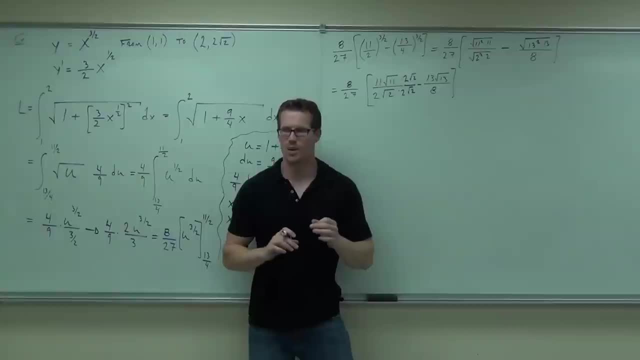 It's just the root 2.. So rationalizing, it's just the root 2.. I'm also trying to get a common denominator of 8, though. So I'm going to have 2 times 2,, which gives me 4, times 2,, which gives me 8.. 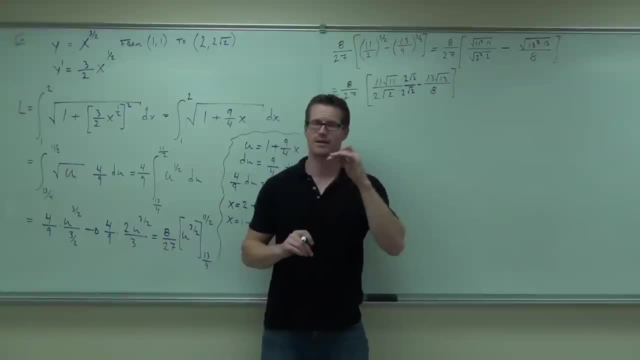 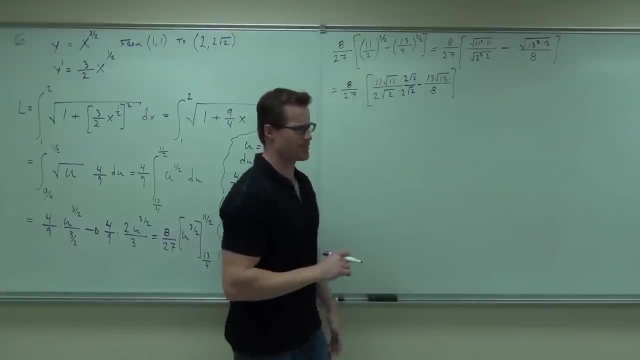 So I'm doing two things at once right here: Getting the common denominator and denominator and rationalizing. Okay, Yes or no? Yes? Well, the problem's easy. It's a cake, It's an integral of the square root of u. 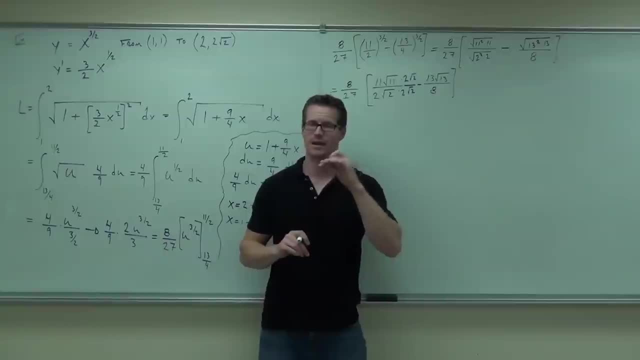 So I'm doing two things at once right here: Getting the common denominator and denominator and rationalizing. Okay, Yes or no? 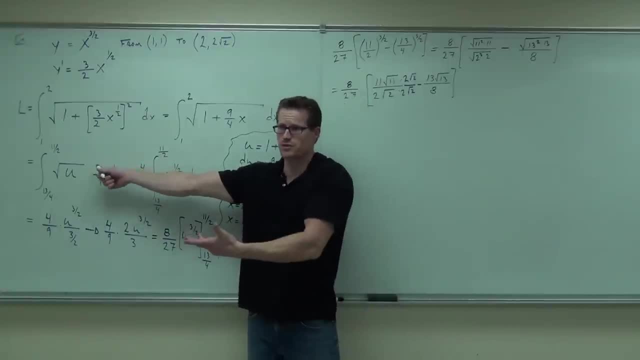 It's a cake. It's an integral square root of u. The evaluation sucks. It's horrible. 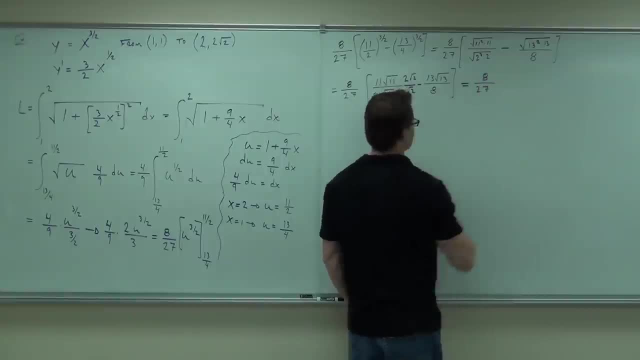 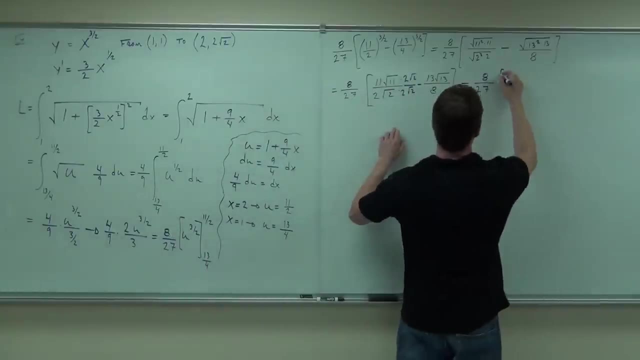 Was that intentional or accidental? You know the numbers just don't work out nice on these. They really don't. I mean, you get some whacked out. You're going to see this. It's crazy, But weird, weird things. 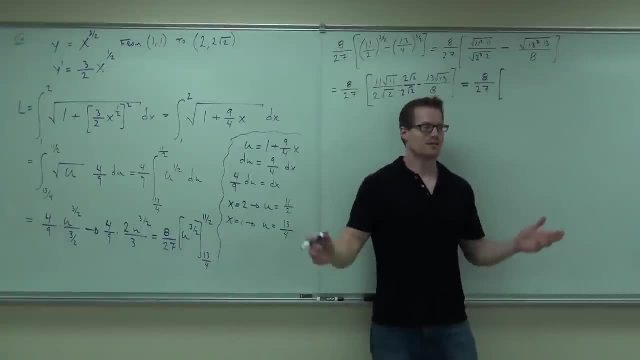 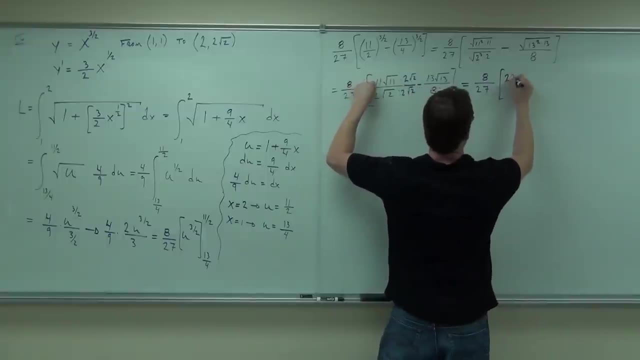 But think about it. I mean, should the length of the line be something like seven? No, Unless it's straight. come on, it's not gonna be that 22 root 22 over eight minus 13 root 13 over eight. 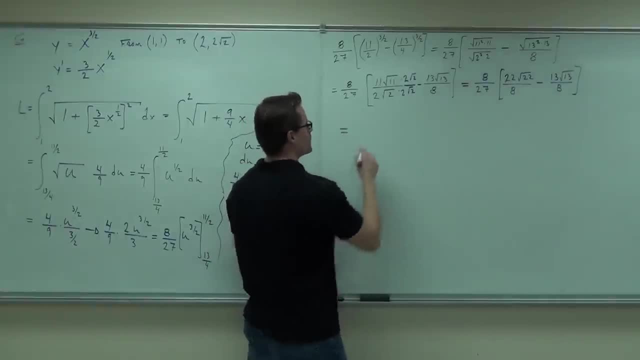 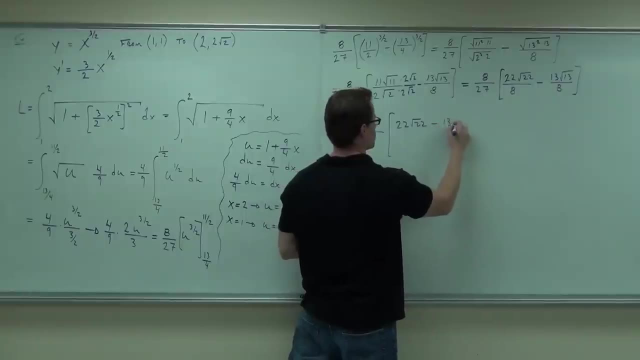 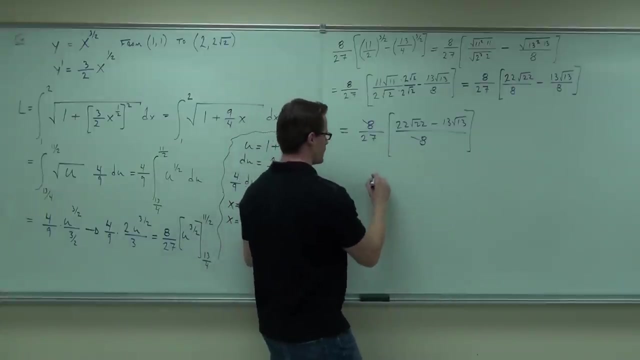 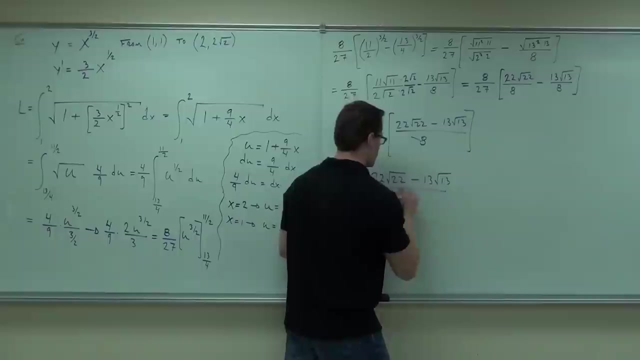 We're almost done, though. just stick with it. You're gonna get 8 27ths, 22 root 22 minus 13 root 13 over eight. Tell me what happens. I like that. Please leave that. just leave it like that. that's it. 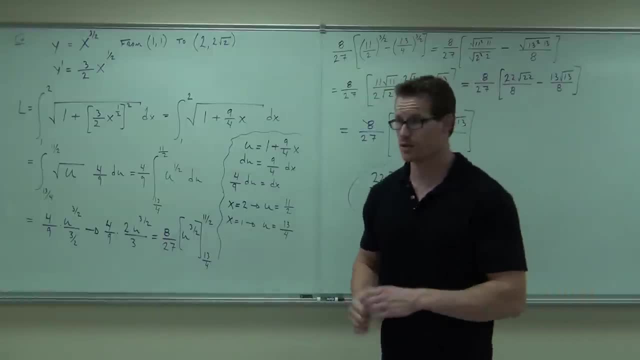 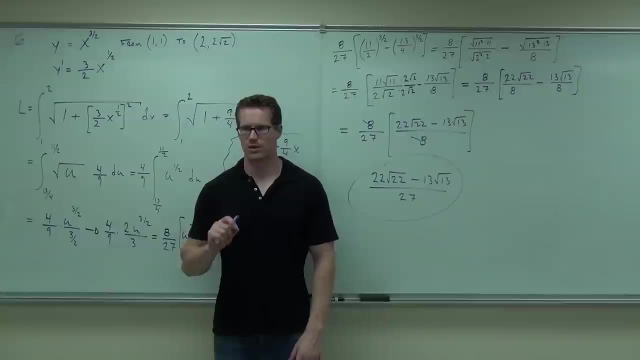 That's close enough. Now, if you want to evaluate, you're gonna get something like you could evaluate, couldn't you? 22 times root 22 minus 13, times root 13,, all over 27, you get 2.09 is the answer. 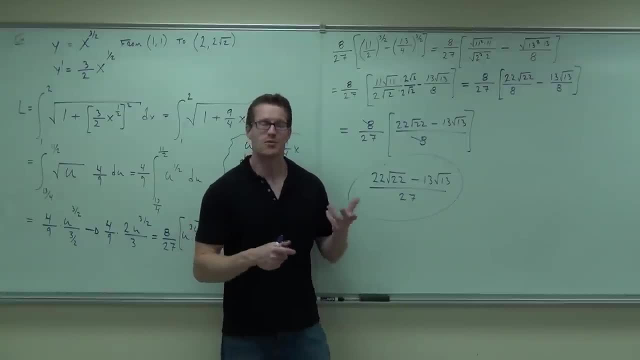 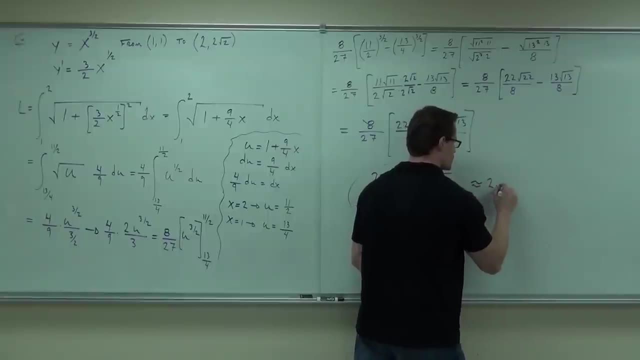 It's about 2.09,. so, all this work, we found the length of a line, though, didn't we? This is the exact, that's exact. It's approximately, if I did it right earlier- 2.09, whatever the units are. 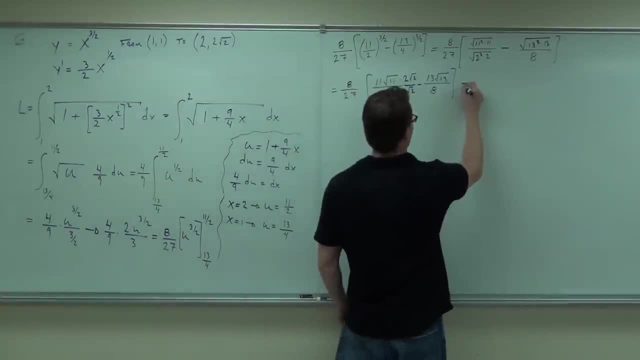 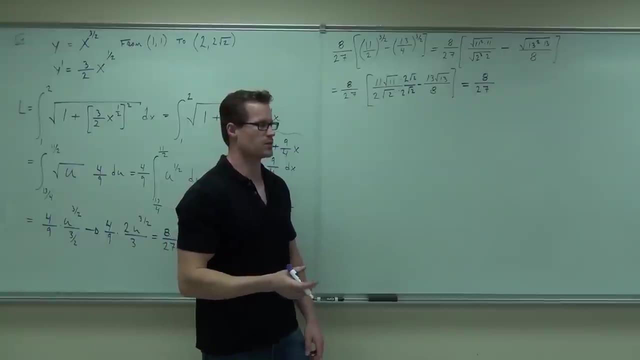 The evaluation sucks. It's horrible. Was that intentional or accidental? You know the numbers just don't work out. nice on these, They really don't. I mean you get some whacked out. You're going to see this. It's crazy. 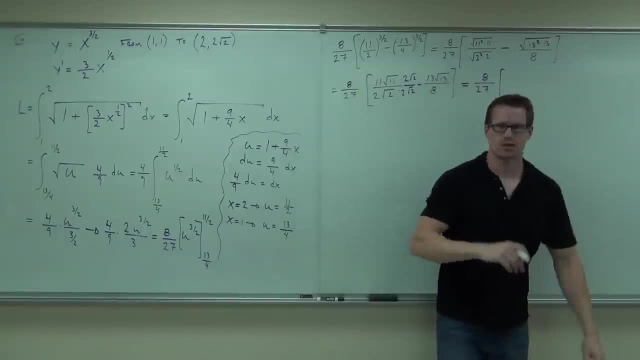 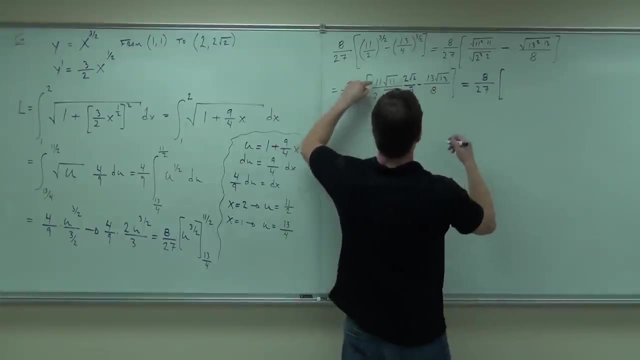 But weird, weird things. But think about it. I mean, should the length of a line be something like 7?? No, Yes, Unless it's straight. I mean, come on, It's not going to be that 22 root 22 over 8.. 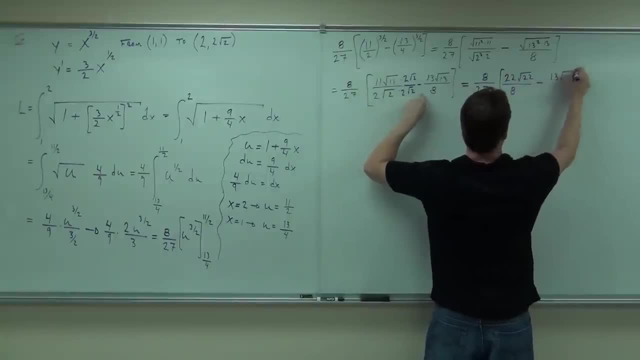 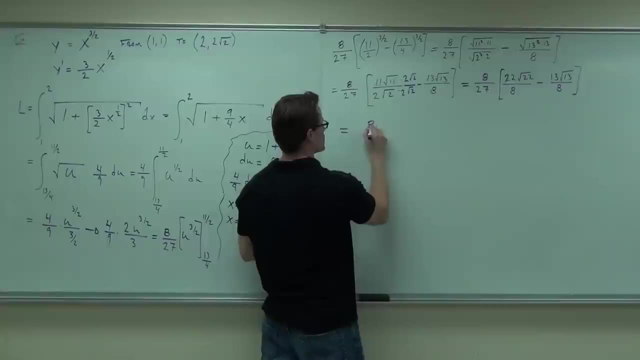 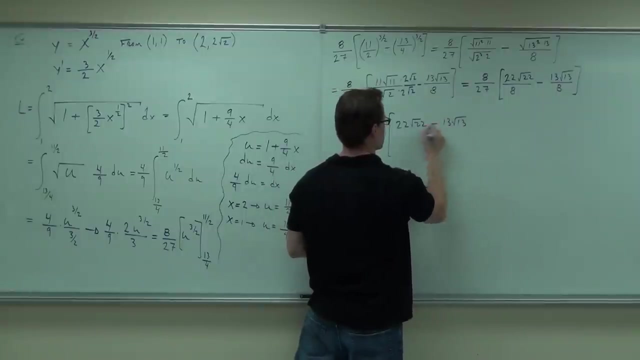 Minus 13, root 13 over 8.. We're almost done, though. Just stick with it. You're going to get 8 27ths 22 root 22 minus 13, root 13 over 8.. Tell me what happens. 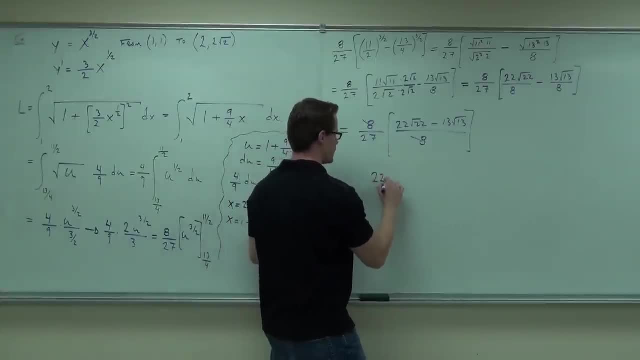 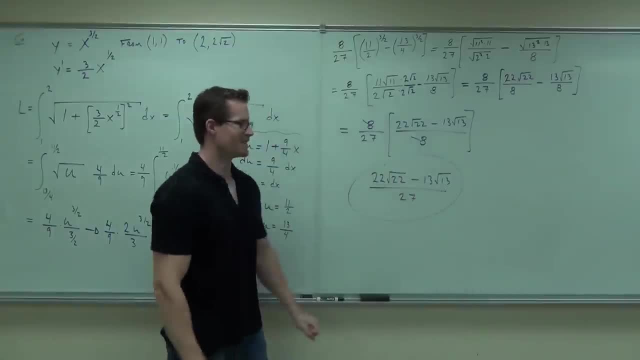 I'm going to do this, I'm going to do this, I'm going to do this. Please leave that. Just leave it like that. That's it. That's close enough. If you want to evaluate, you're going to get something like: 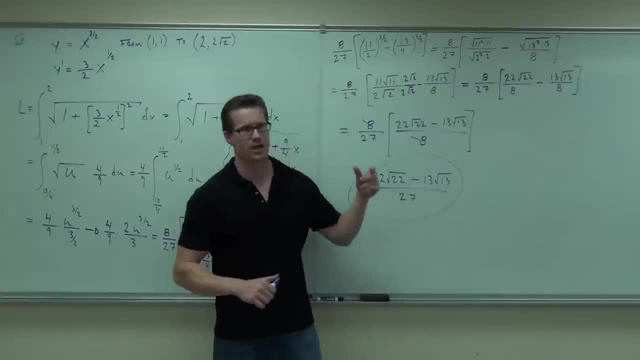 You could evaluate, couldn't you? 22 times root, 22 minus 13 times root, 13, all over 27.. You get 2.09, is the answer. It's about 2.09.. So all this work? We found the length of a line, though, didn't we? 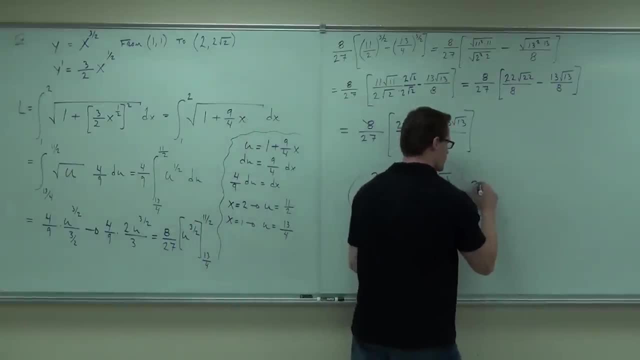 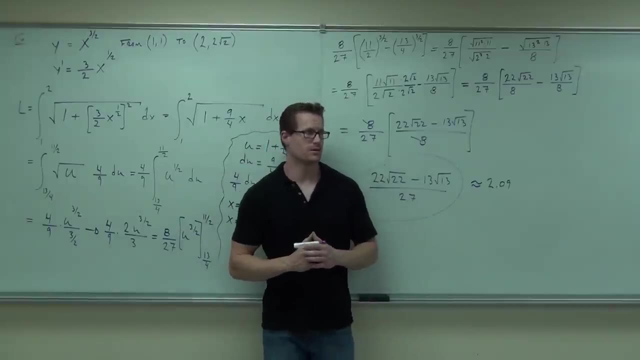 This is the exact. That's exact. It's approximately- if I did it right earlier- 2.09, whatever the units are, But you are finding the length of a line. You've got to start dealing with numbers like this and you want to use decimals. 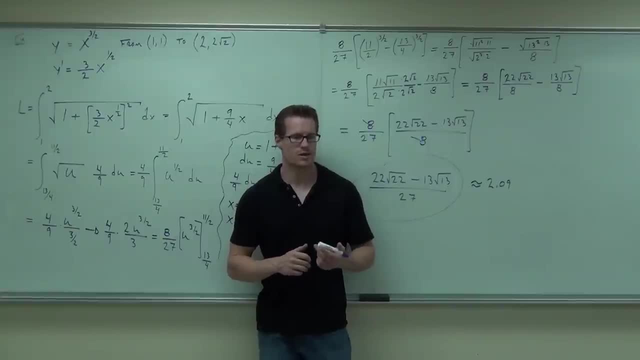 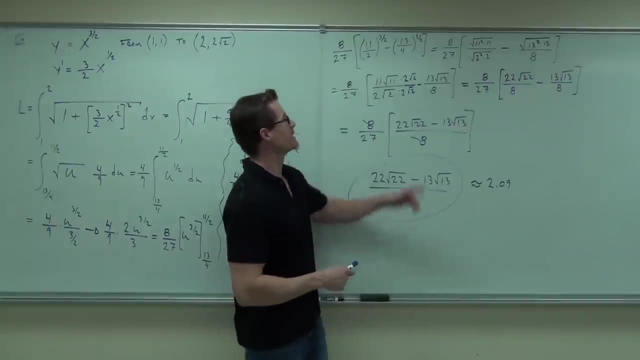 Use the approximation. But as soon as you start using approximations more and more, your problems get more and more off, More and more off. So if I approximated here and then approximated like, well, that would be. 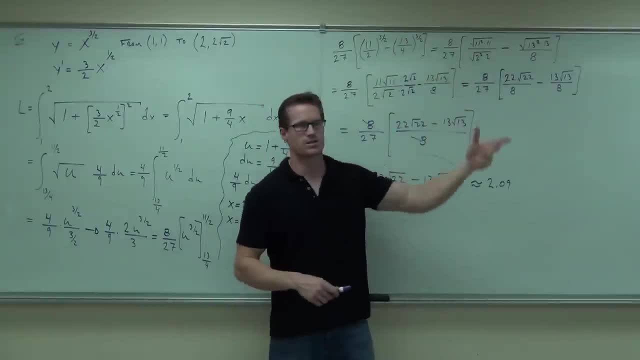 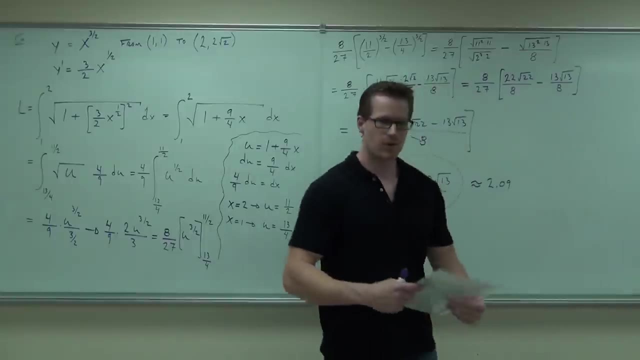 you know, not an approximation, But if I approximated here and then subtract and approximated and approximated and approximated, you're rounding around. it's never a good thing. You're going to be off. How many people feel okay with? 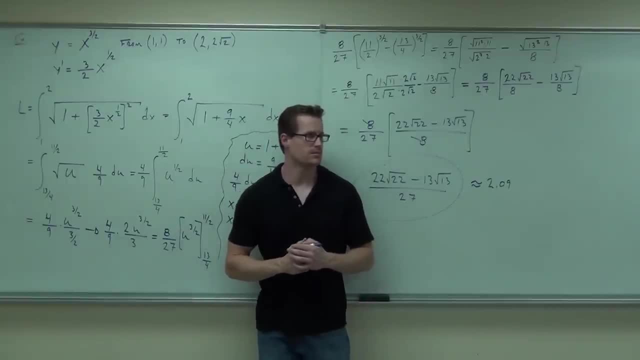 but you are finding the length of a line. You gotta start dealing with numbers like this and you want to use decimals, use the approximation. But as soon as you start using approximations more and more, your problems get more and more off, more and more off. 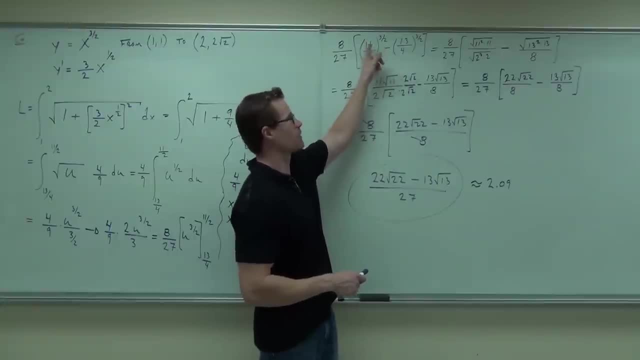 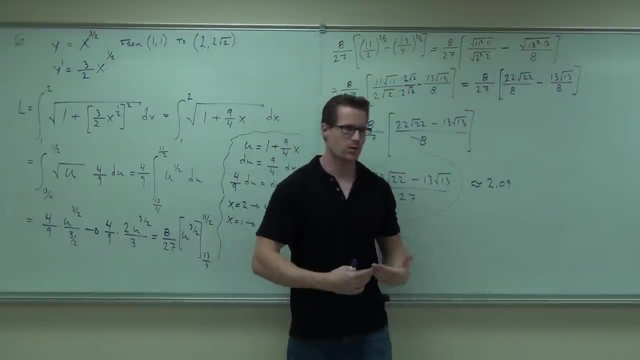 So if I approximated here and then approximated, like well, that would be, you know, not an approximation, but if I approximated here and then subtracting approximated and approximated and approximated, you're rounding around. it's never a good thing. 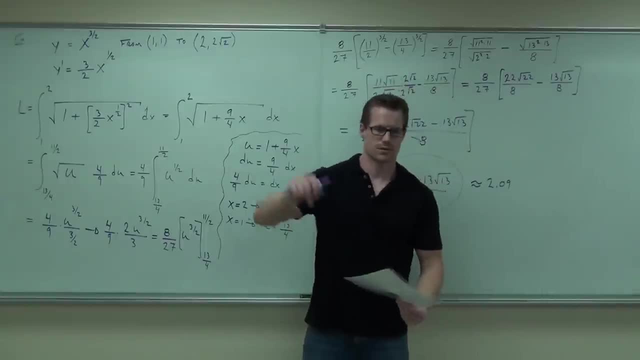 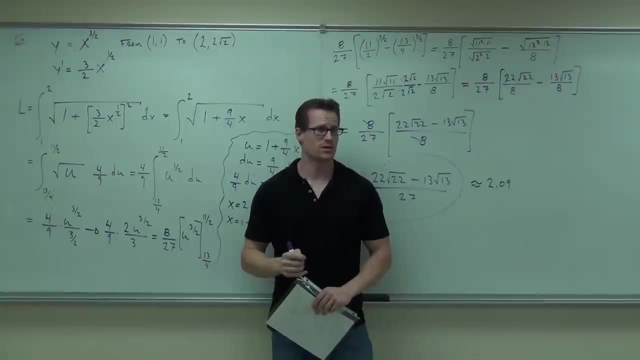 You're gonna be off. How many people feel okay with this so far Now? would you like to do this in terms of why? Just to see how it goes. Yes, Yeah, Yeah. No, not really, I don't either, but I'm going to show you. 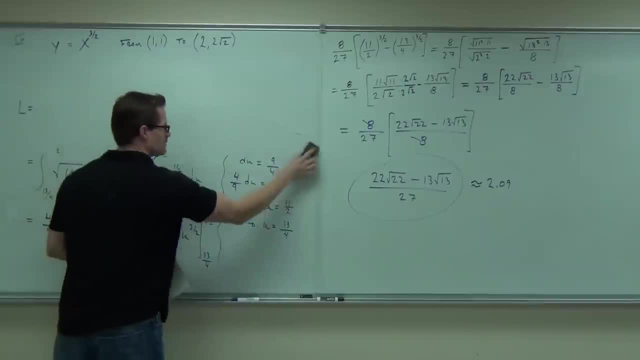 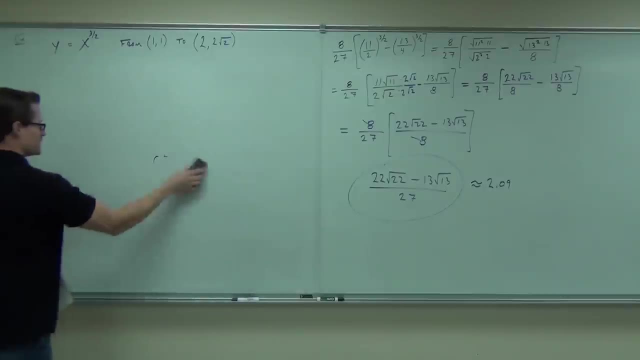 That's a shame. That was so nicely done. Should have taken a picture. It's in my head. I didn't take a picture. Oh, that's right. Yeah, There's one over there. Should have taken a picture Now, if I want to do this. 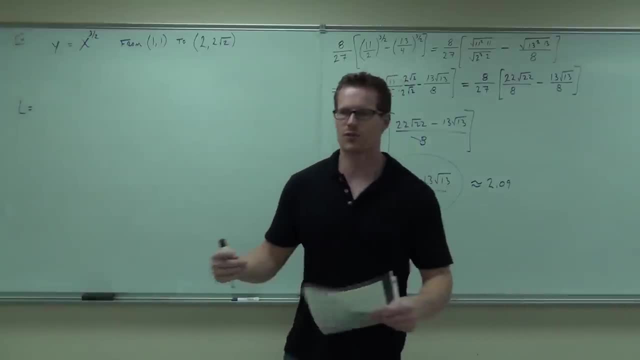 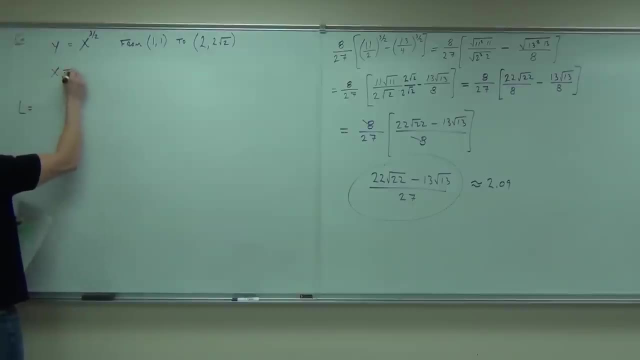 along this, treating this in terms of y, I've gotta solve for the x. So in other words, I would square and take a cube root. So this would mean that x would equal y to the 2 3rds power. 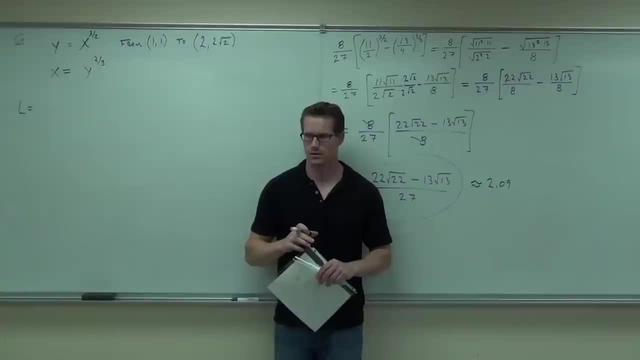 y to the 2 3rds power. Are you okay with that? You sure, So. if x equals three y, sorry. y equals x to the 3 1⁄2,. x equals y to the 2 3rds. 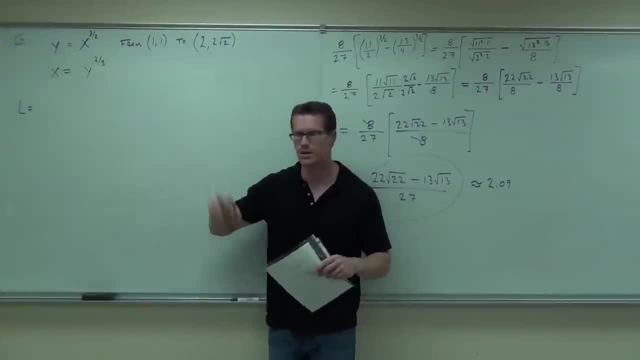 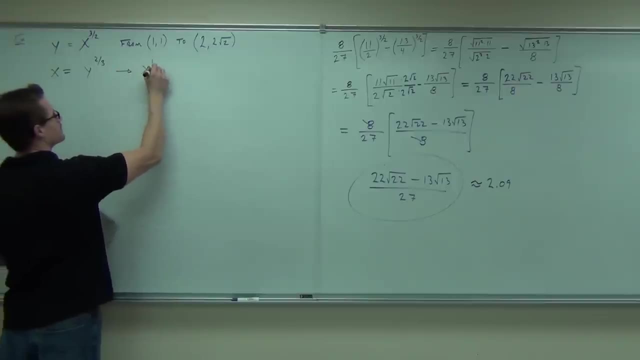 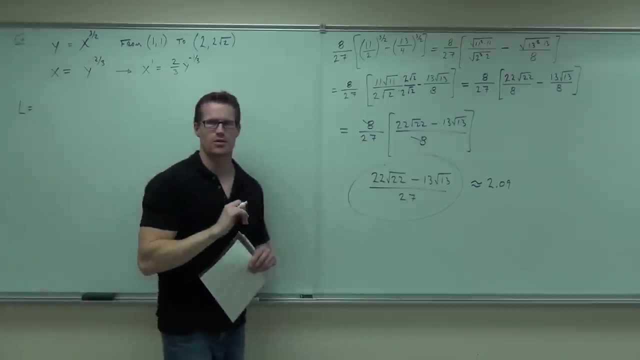 You cube it, cube, root it and you square it. That's what that would be. Now someone tell me the next step: Find your derivative. And that's why it's nasty. The negative 1- 3rd causes you a lot more pain. 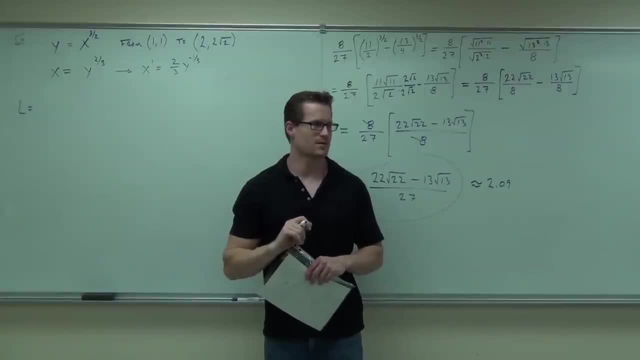 It's suffering. Okay, I was wondering if you were going to be the 2 to the power of the square root of two and the power of the zero to the power of the pain. No, no, not pain, Not there. Maybe a little. 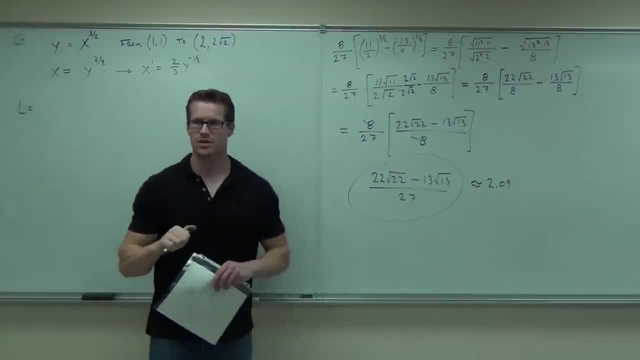 Are you okay with that? I'm okay with the derivative, though. You see where it's coming from. You bring it to 2 3rds. subtract one from it, you make it to 1- 3rd. We can actually set it up right now. 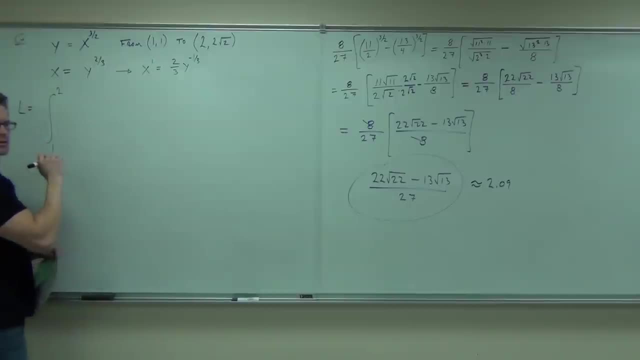 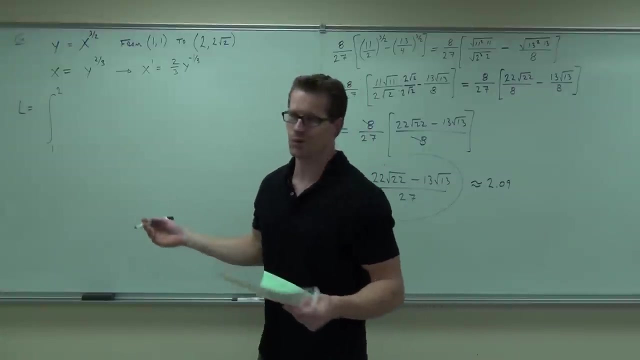 We got one to two. One to two, No one minus two is two. Two over here, Y. That's what you're using in terms of y, In terms of y. now, That's exactly right. So this is really why I wanted to do the problem. 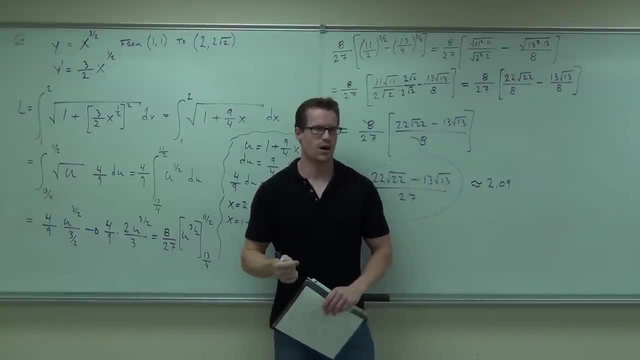 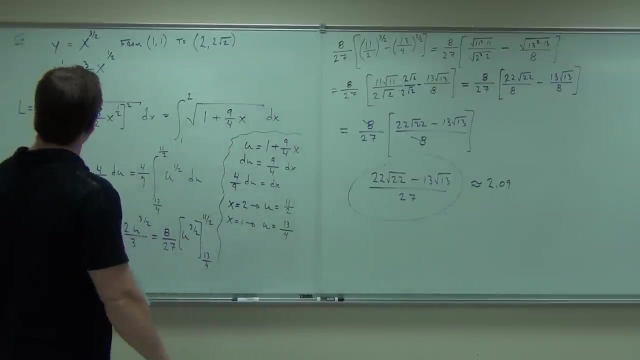 This is so far Now. would you like to do this in terms of why? Just to see how it goes? Yes, Yeah, No, not really, I don't either, but I'm going to show you. That's a shame. 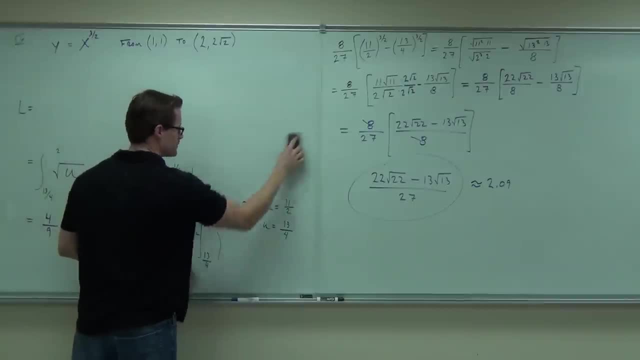 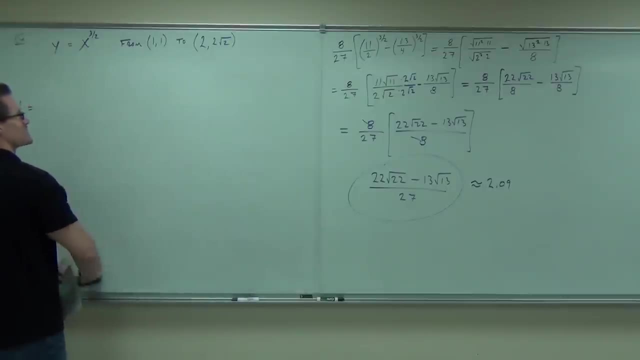 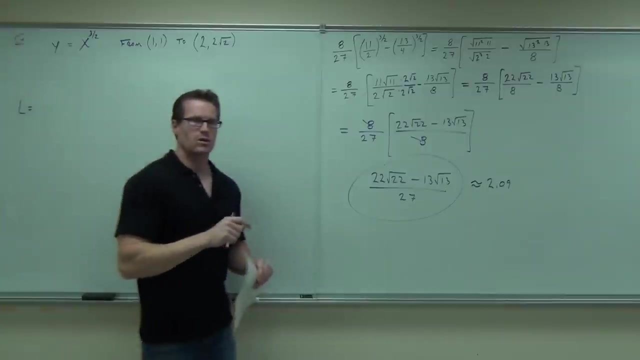 That was so nicely done. It's in my head. I didn't take a picture. Oh, that's all right. Yeah, I should have taken a picture. Now, if I want to do this along, treat this in terms of y. I've got to solve for the x. 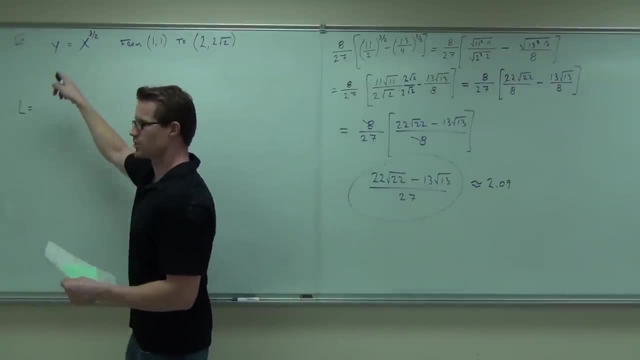 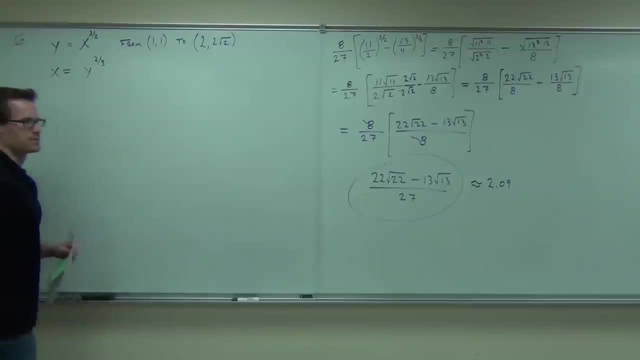 So, in other words, I would square and take a cube root. So this would mean that x would equal y to the two-thirds power, y to the two-thirds power. Are you okay with that? Yeah, Yeah, Are you okay with that? 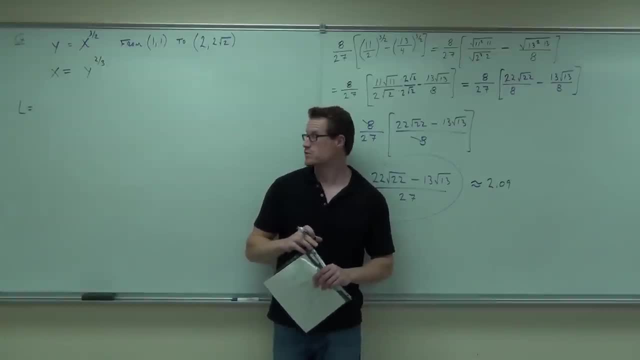 You sure? So if x equals three, sorry, if y equals x to the three-halves, x equals y to the two-thirds. You cube it, cube, root it and you square it. That's what that would be. 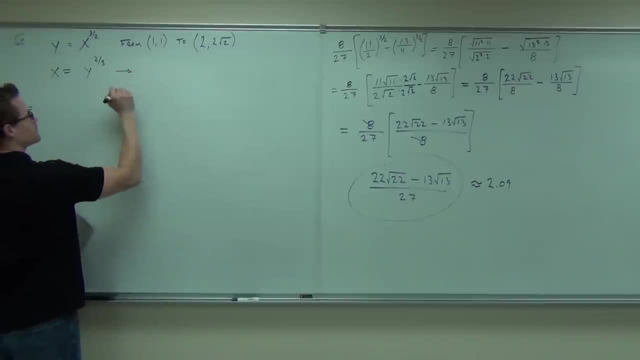 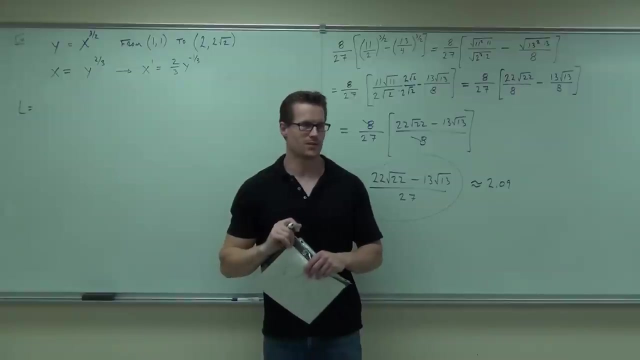 Now someone tell me the next step: Find your derivative. And that's why it's nasty. The negative one-third causes you a lot more pain. It's separate. Okay, I was going to say you're going to be doing two to the power square root of two. 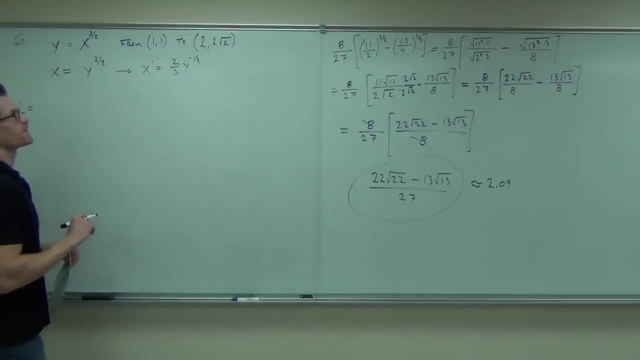 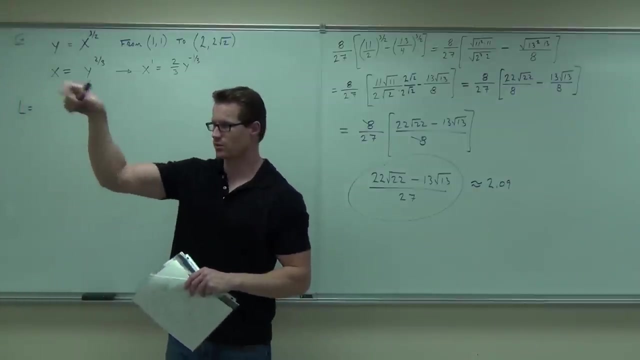 And the power is going to be a lot more pain. No, no, not pain, Not there, Maybe a little. Are you okay with the derivative, though? You see where it's coming from. You bring in a two-thirds subtract, one from it. you make it one-third. 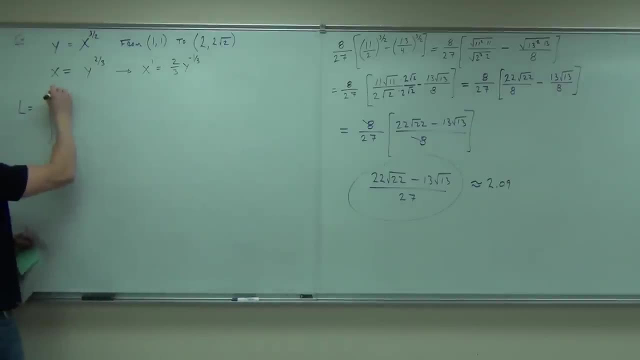 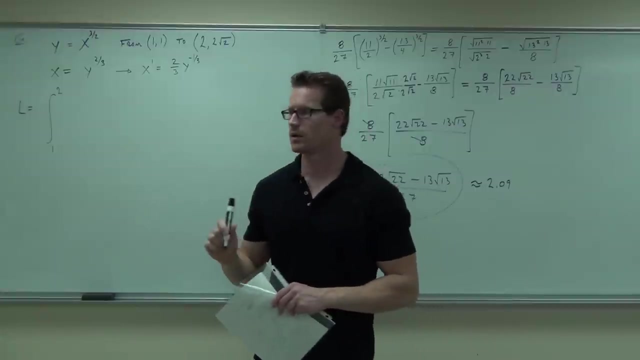 We can actually set it up right now. We got one to two. One to two, No one to two. Two to two. Why? Because we're going to do this in terms of y, In terms of y. Now, that's exactly right. 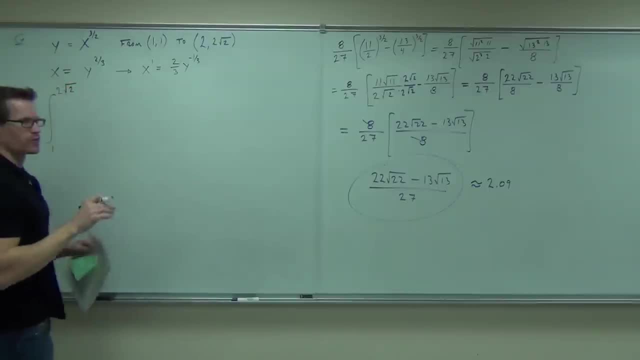 So this is really why I wanted to do the problem. so you see that, Watch out for what you're in terms of. If it's in terms of y, you need y's. If it's in terms of x, you need x's. 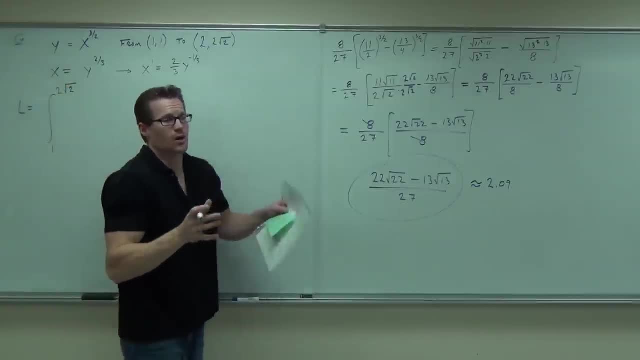 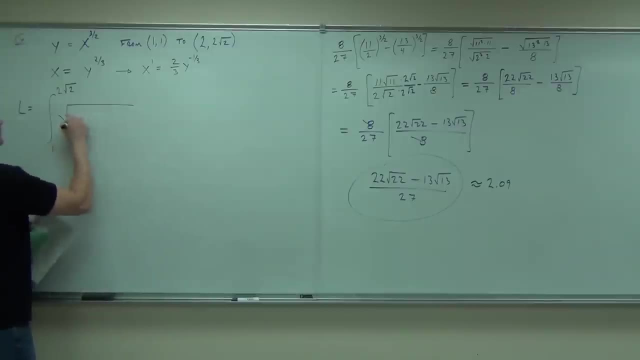 so you see that Watch out for what you're in terms of. If it's in terms of y, you need y's. If it's in terms of x, you need x's One, plus the derivative of x squared 2- 3rds y to the negative: 1, 3rd squared. 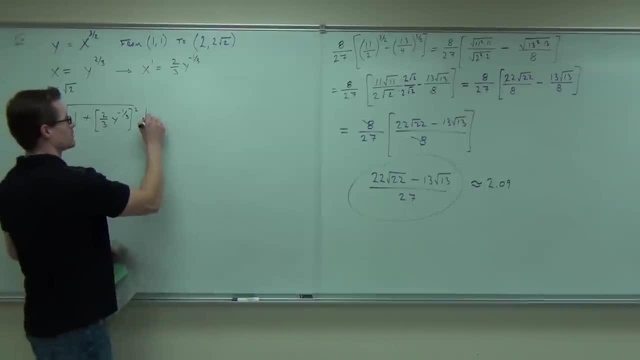 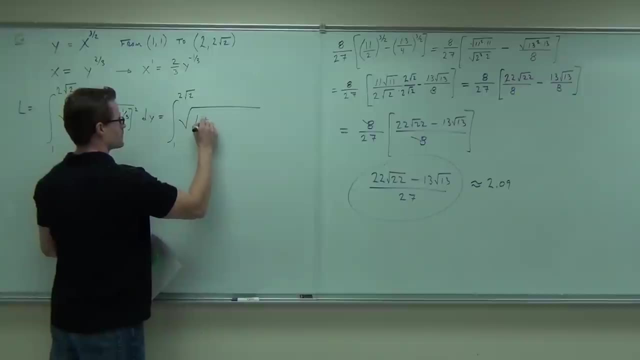 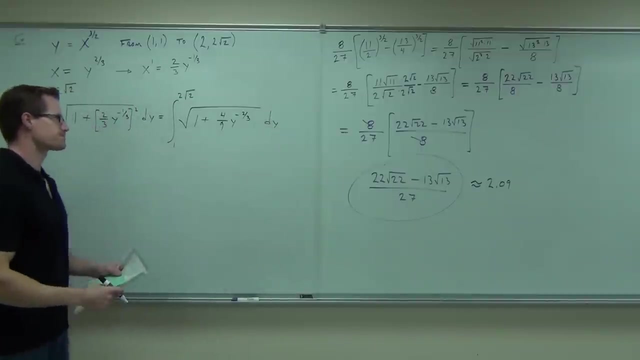 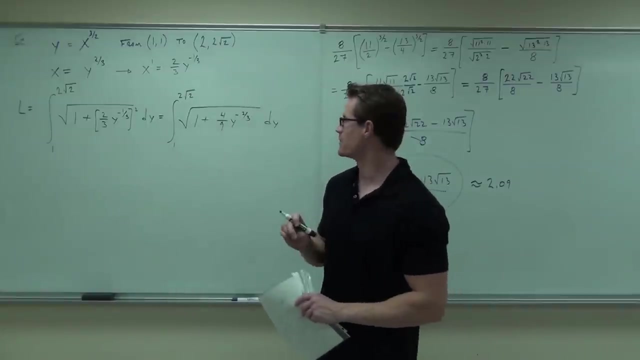 D plus One plus y. Good. Now, unfortunately for us. do you see the problem that we have, that we didn't have previously? The problem before was nice, because it was a one-half and we square one-half, It goes away. 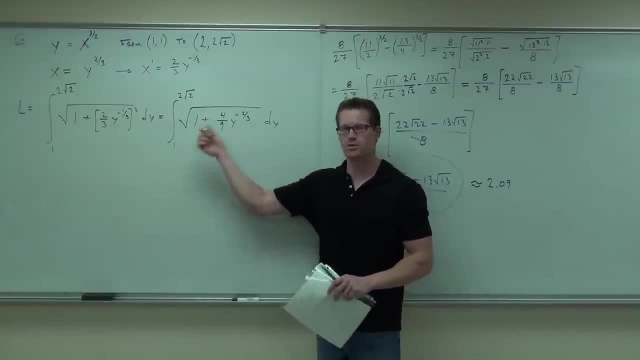 It's just y. This is a problem. Do you see why that's a problem? You cannot do a substitution here. Do you see why, If you do a substitution, you end up still having a y in there? Why? Because there's no y in there and there's no y to get rid of. 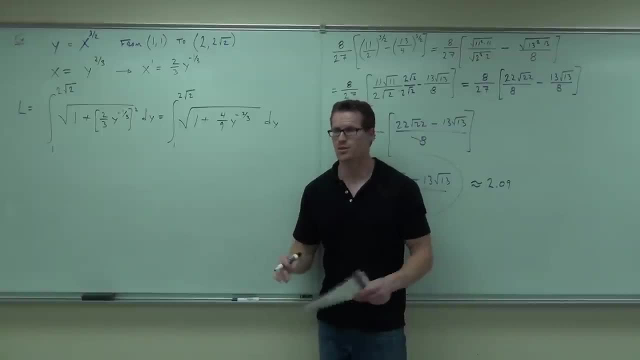 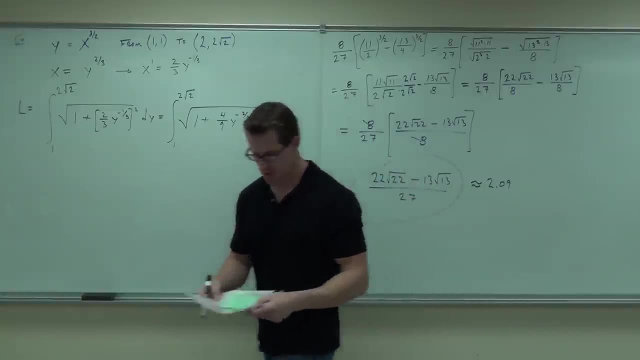 There's nothing, So that's not going to work. What is going to work is very similar to what we did in the first problem. Try to get a common denominator. Try to break that off and then see what you have OK. 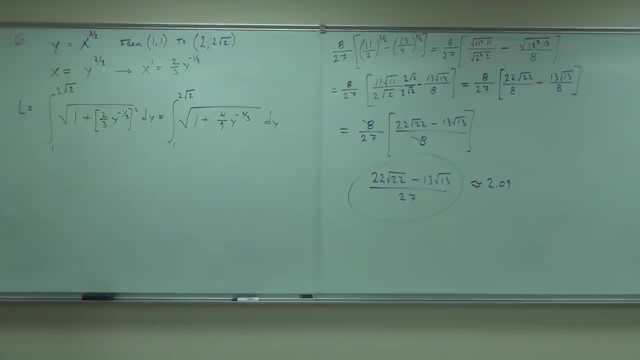 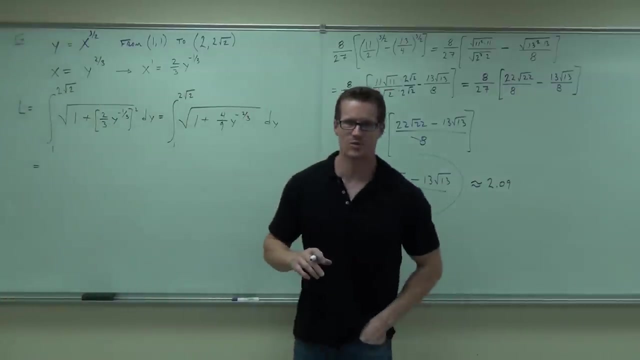 So that's the process, for right now I want to show you- because I know that some of you think I give you some homework problems which are much more brutal than the ones I give you- This is going to be a pretty brutal problem, so at least you're going to get it right now. 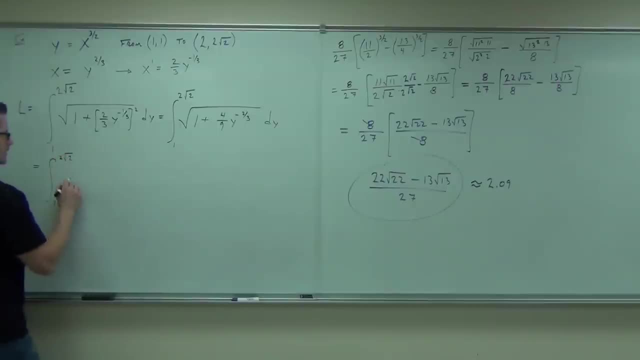 This is 1 to square root of 2, root 2.. What we're going to do- I'm going to kind of go a little quickly through this, just so you're seeing it quickly, I suppose, so we can get done with more things. 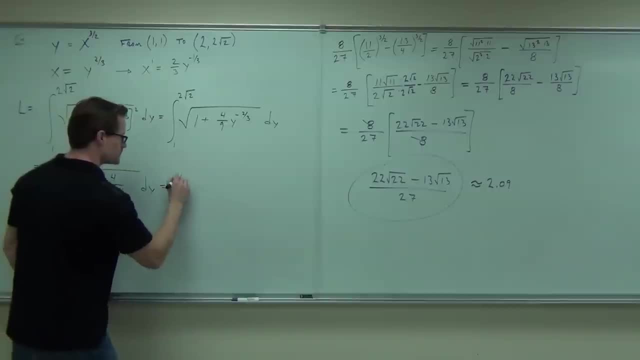 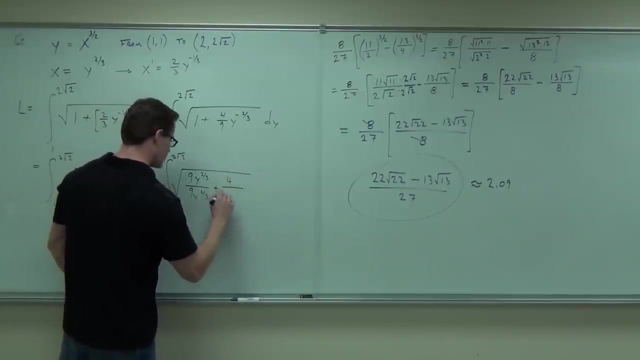 But all of its basic algebra, so you can just go back and do whatever you want to do. It should be all right now. It will be a little bit fine, but this is just going to go a little way down here because I know it does quite a bit. 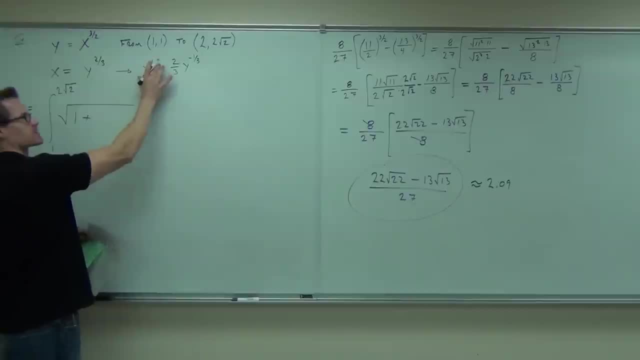 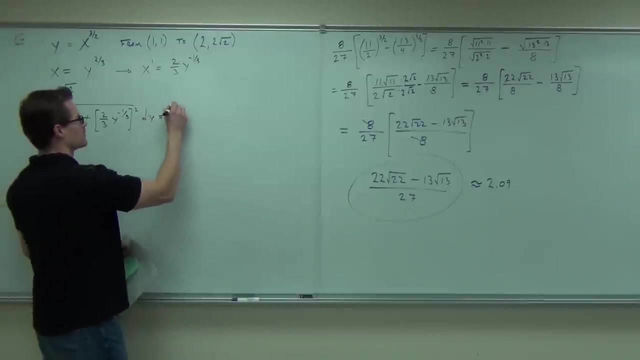 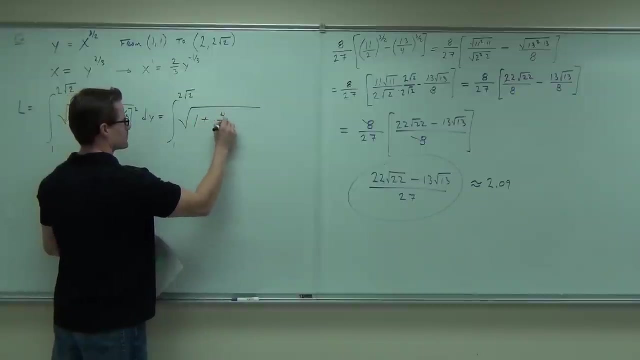 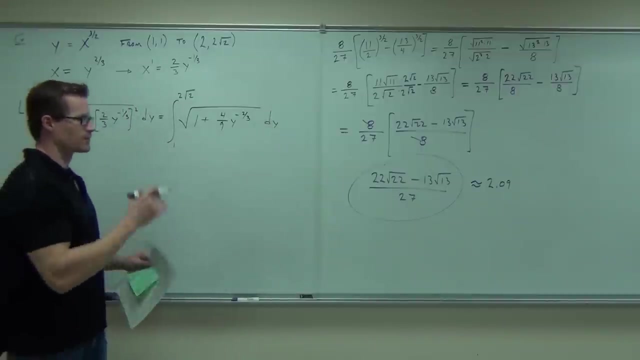 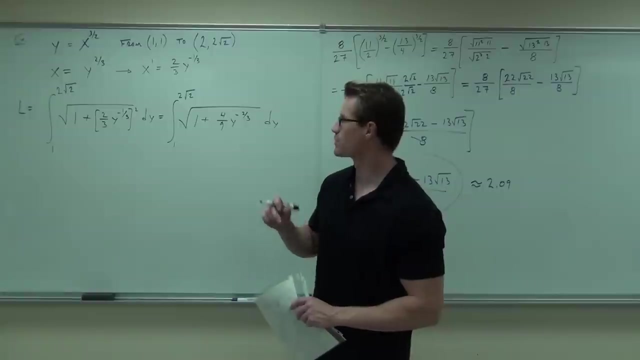 One plus the derivative of x squared Two-thirds y to the negative, one-third squared D plus One to y. Good, Now, unfortunately for us, do you see the problem that we have that we didn't have previously? The problem before was nice. 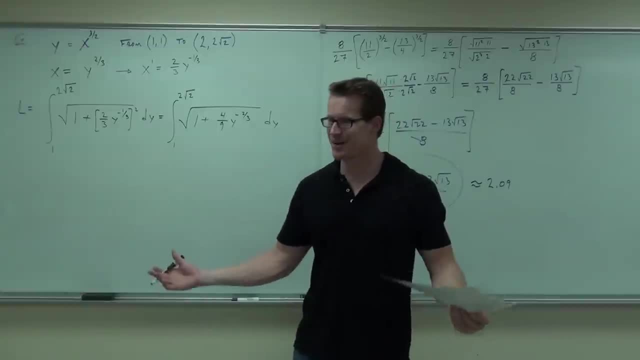 The problem before was nice, Because it was a one-half and we square one-half, It goes away, It's just y. This is a problem. Do you see why? that's a problem? You cannot do a substitution here. Do you see why? 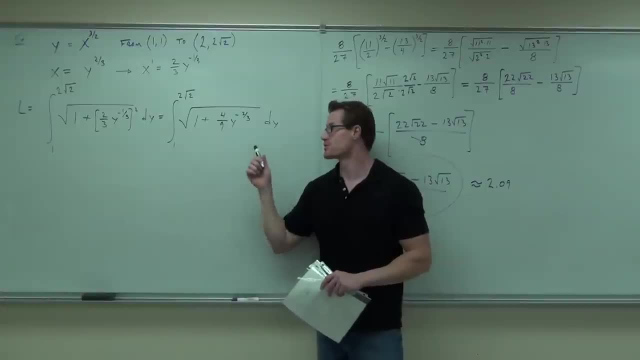 If you do a substitution, you end up still having a y in there And there's no y to get rid of, There's nothing. So that's not going to work. What is going to work is very similar to what we did in the first problem. 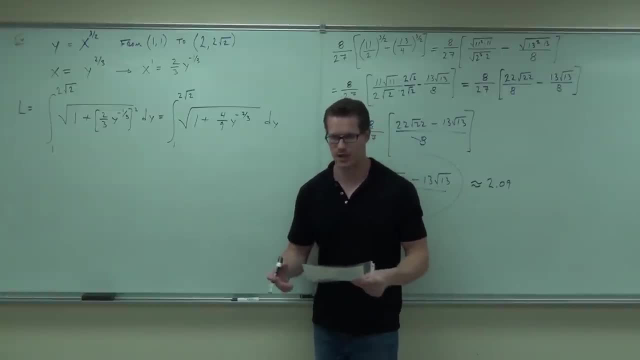 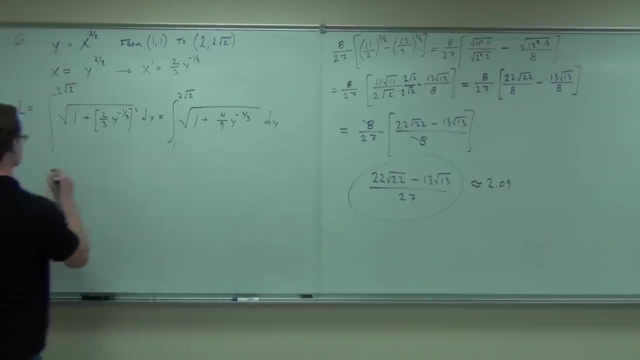 Try to get a common denominator, Try to break that off and then see what you have. okay, So that's the process for right now. Now I want to show you- because I know that some of you think I give you some homework problems- 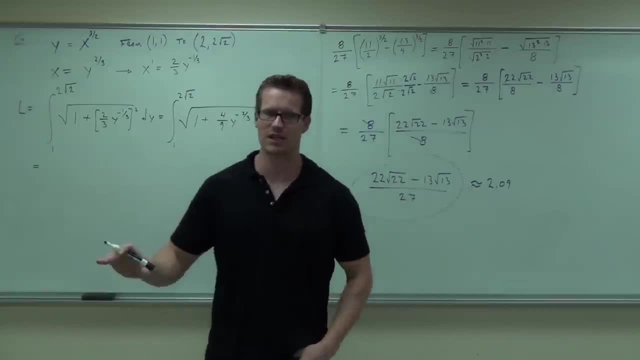 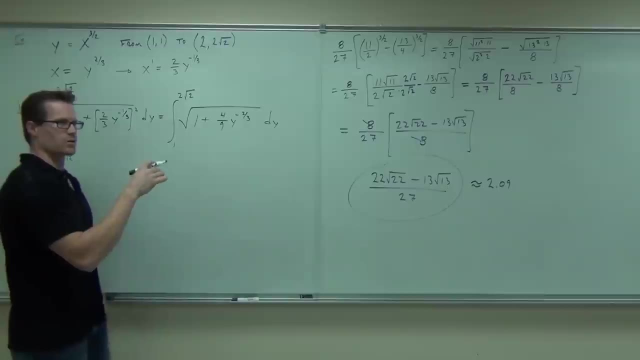 which are much more brutal than the ones I give you. This is going to be a pretty brutal problem, So at least you're going to get it right now. This is 1 to square root, 2 root 2.. What we're going to do. I'm going to kind of go a little quickly through this, just so you're seeing it quickly. 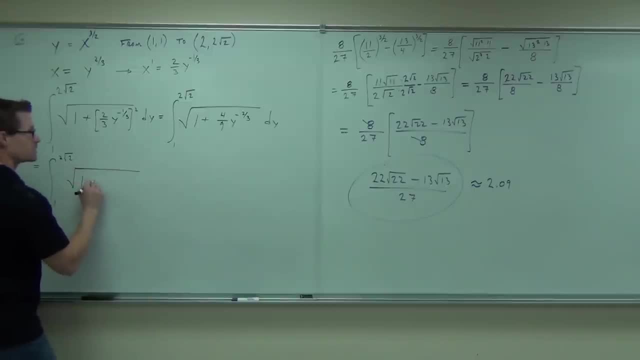 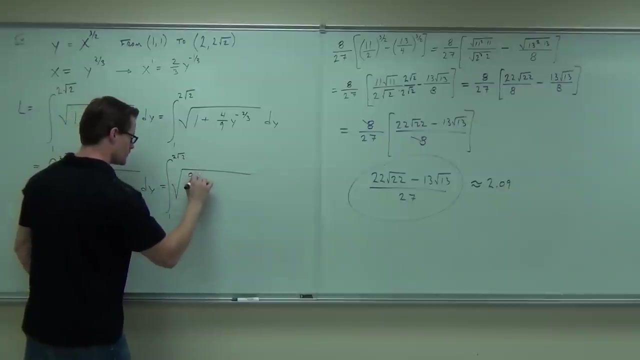 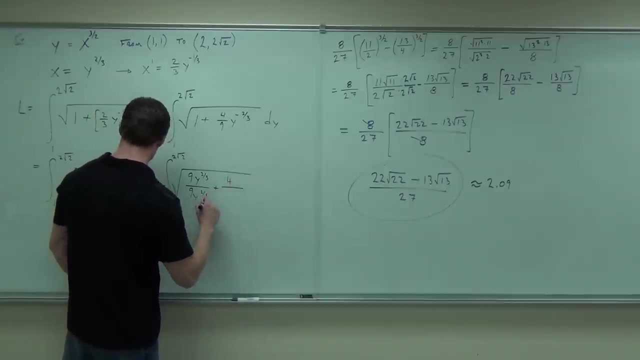 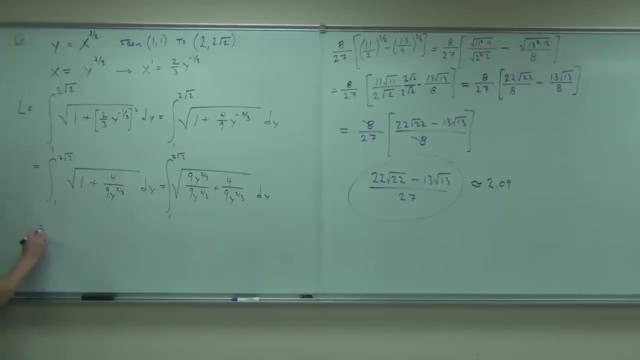 I suppose, so we can get done with more things, But all of this is going to be a problem. All of this is going to be a problem. All of this is going to be a problem. All of this basic algebra. All of this basic algebra. 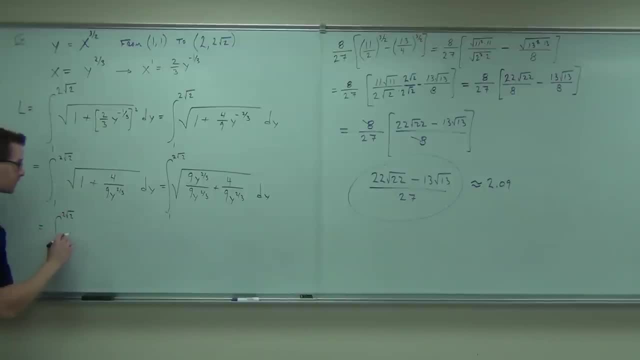 So if I just get rid of some of these points, I should be OK with that. So here's what's going to happen. So I'm going to sort out the numbers and I'm going to take those 2. They're going to the left. 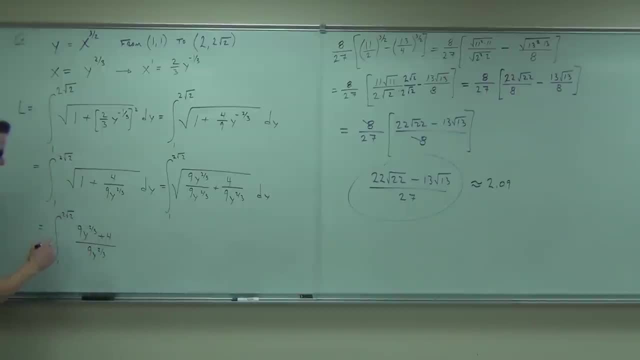 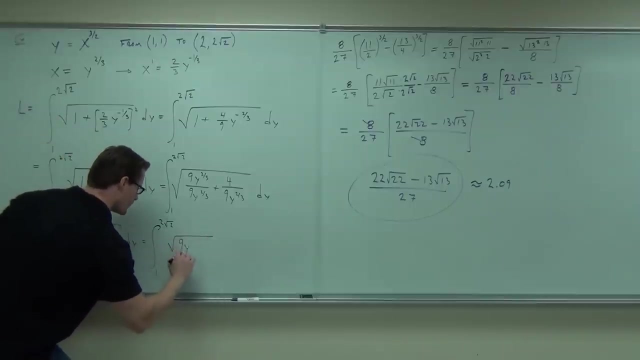 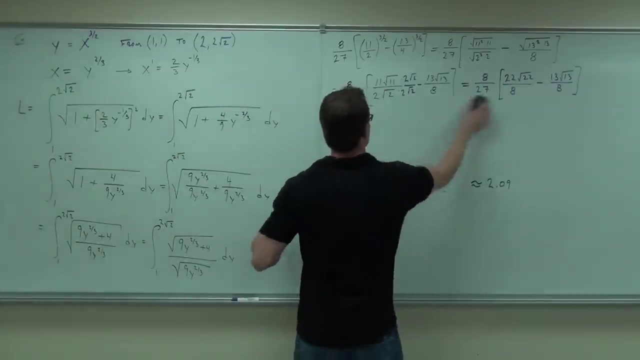 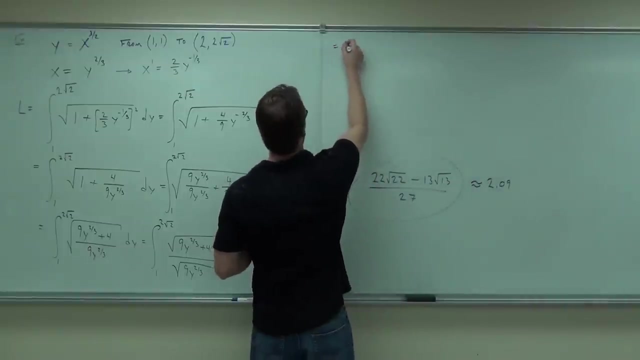 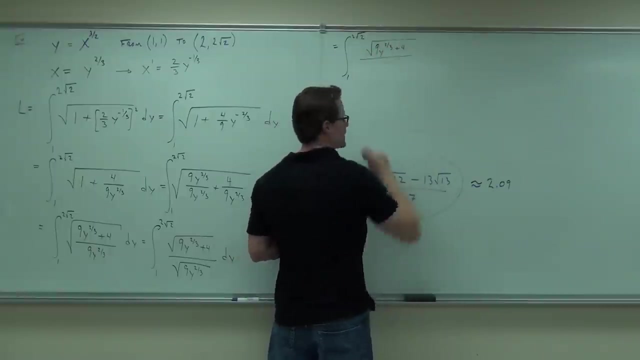 I'm going to sort them out. I'm going to sort them out. So 3 to square root of 2.. So I'm going to sort them out And I'm going to look at the right, All right, And again I'll give you some nice numbers. 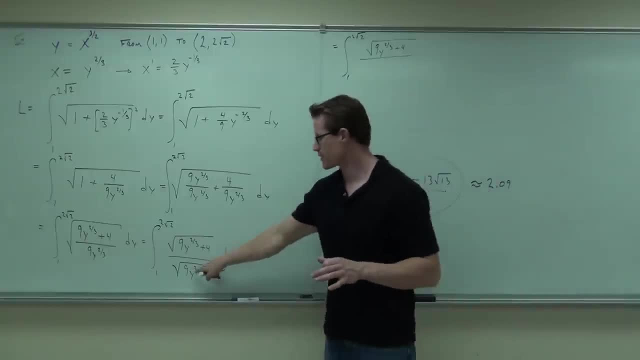 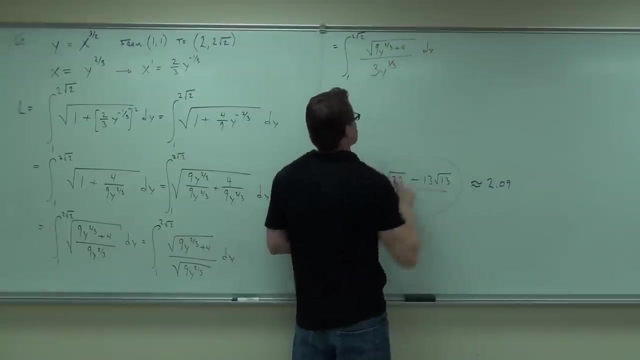 Give them the square root of 9y to the 2 thirds. right here, That's a square root of something that's essentially being squared. What this is is 3y to the 1 third. I'm going to do a couple things here. 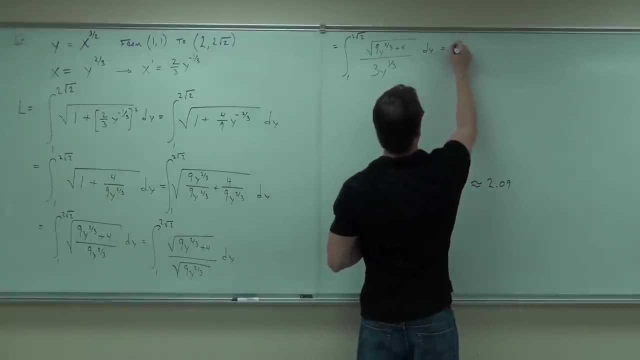 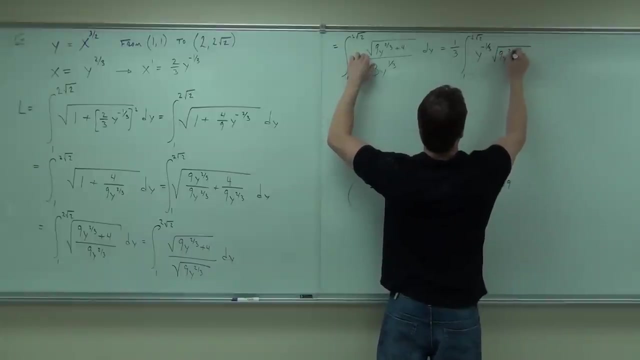 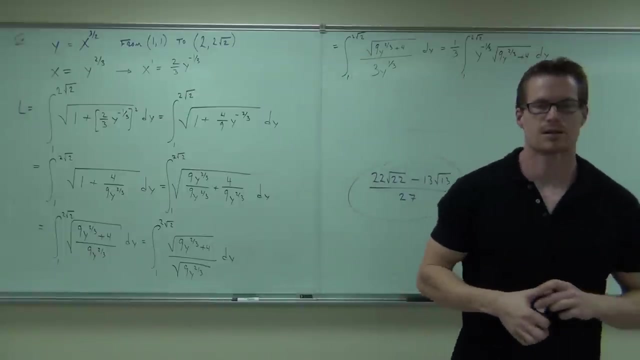 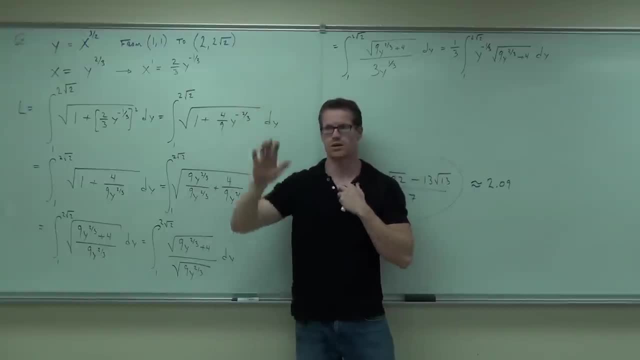 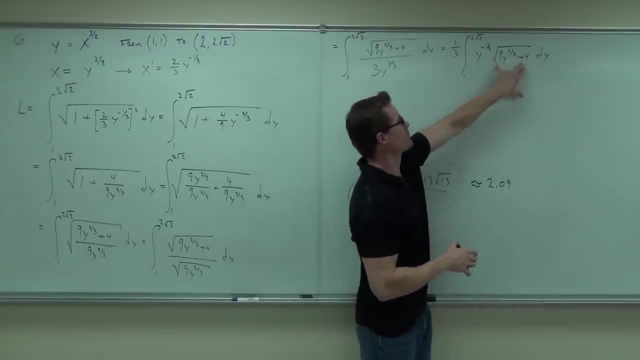 Can you follow the algebra, Would you feel okay with that? so far It's all algebra. Now why is that better? You can do a substitution. Check out the derivative of this. The derivative of that is going to have a y to the negative 1 third, isn't it? 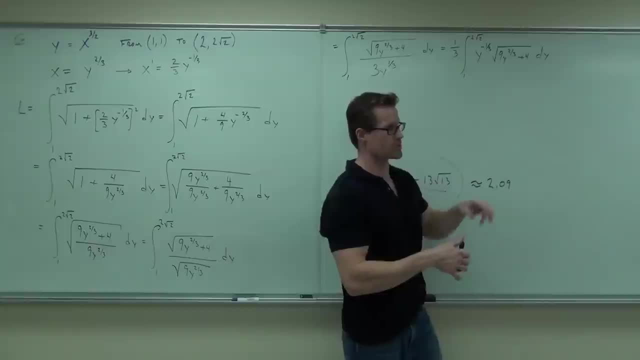 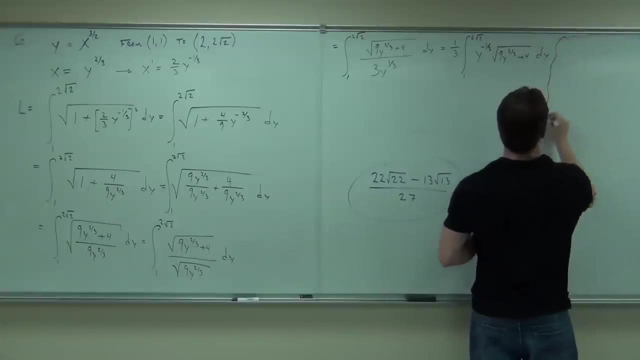 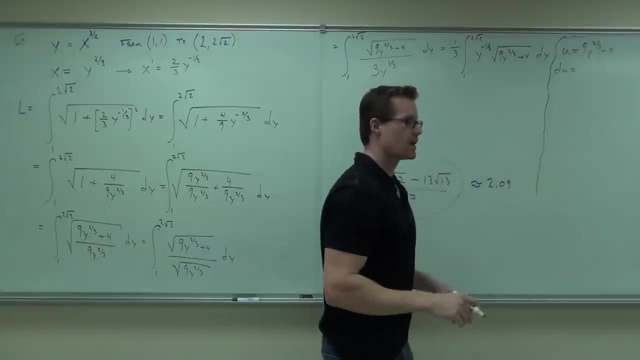 There's a y to the negative 1 third, It's going to work. So now we get to do our substitution and we're going to change the balance. If we do substitution, du equals 2 thirds times 9.. That gives you 6.. 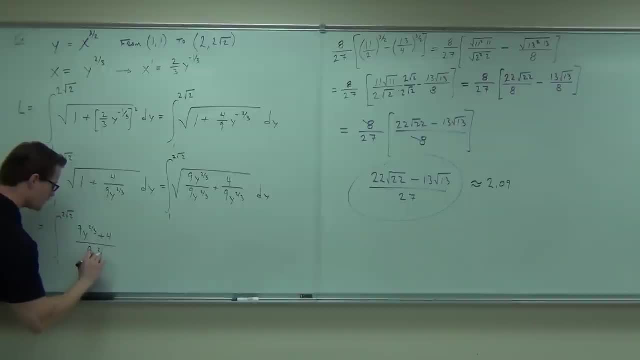 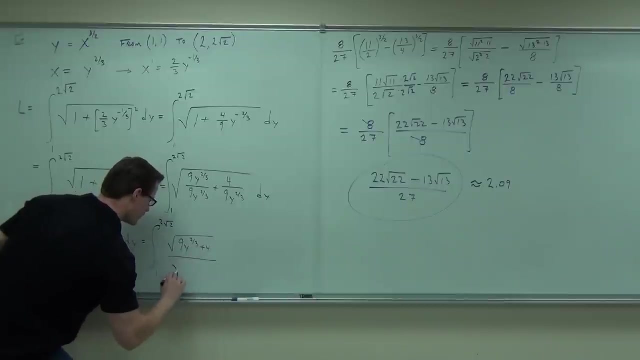 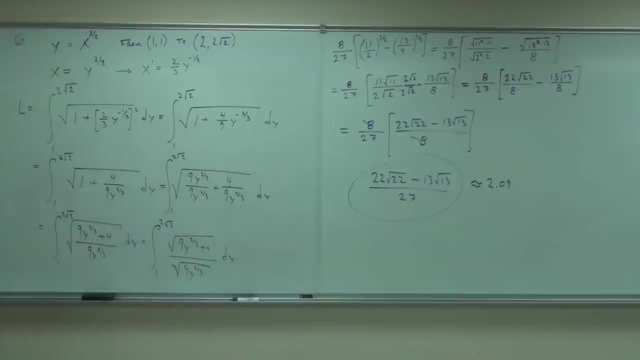 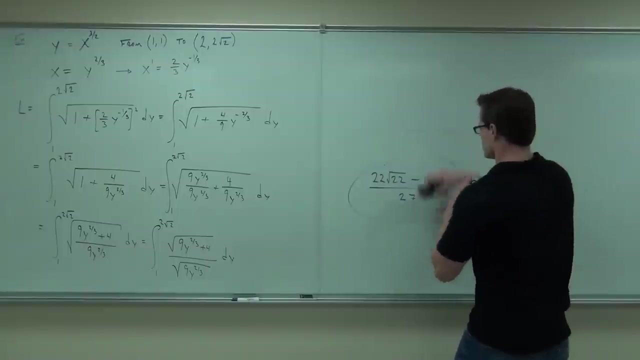 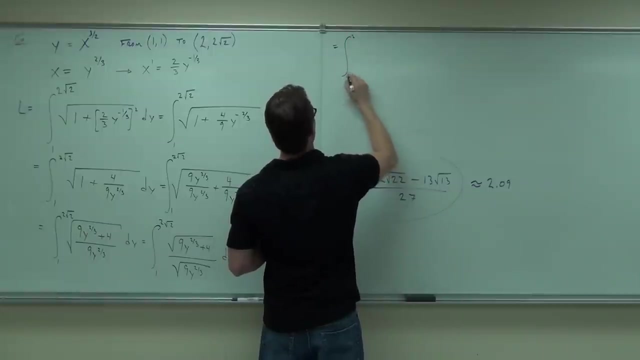 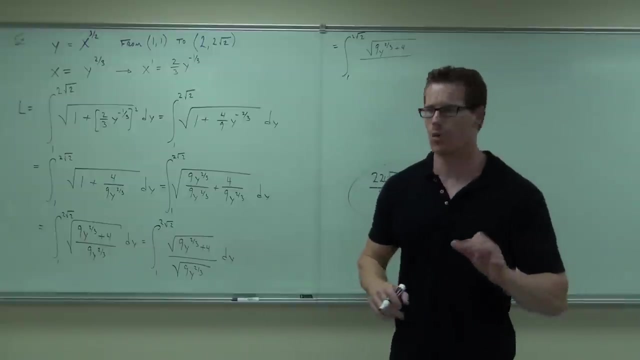 All of this basic algebra, All of this basic algebra, And again I gave you some nice numbers. If you look at the square root of 9y to the 2 thirds right here, that's a square root of something that's essentially being squared. 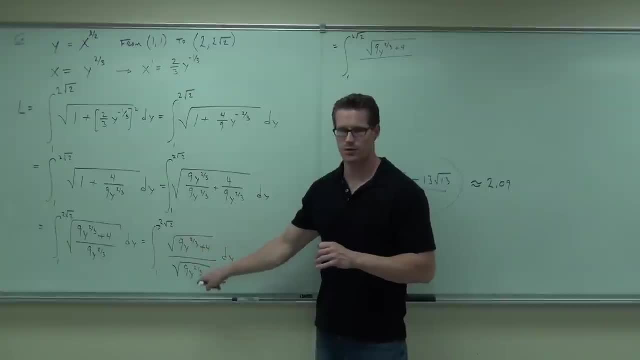 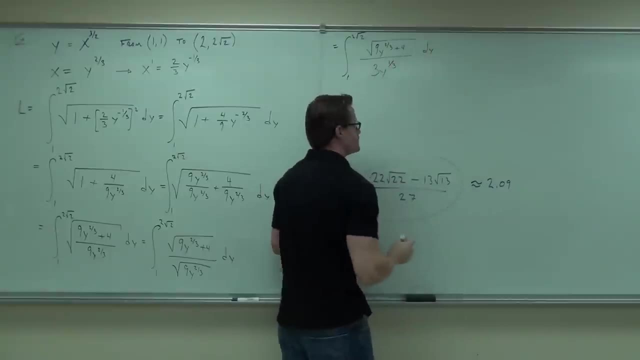 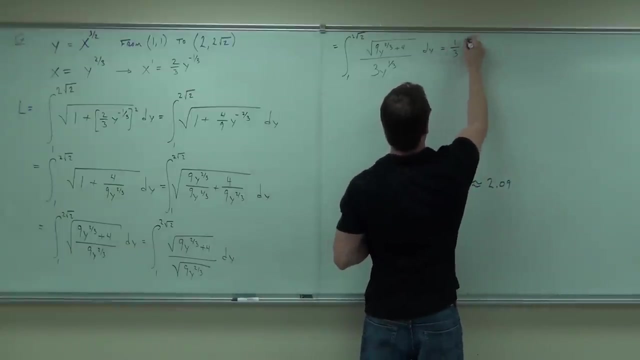 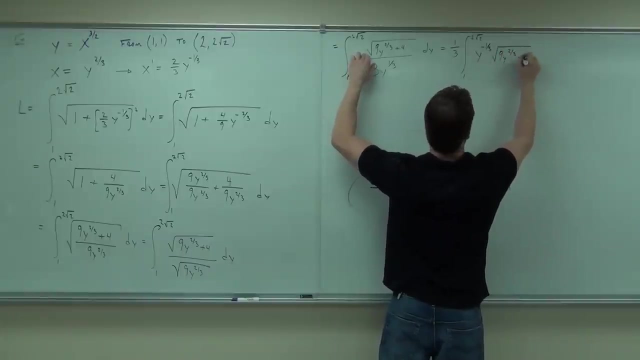 What this is is 3y to the 1 third. I'm going to do a couple things here. I'm going to pull the 1 third out, I'm going to move the y to the 1 third up here And, even though it doesn't look better, it is. 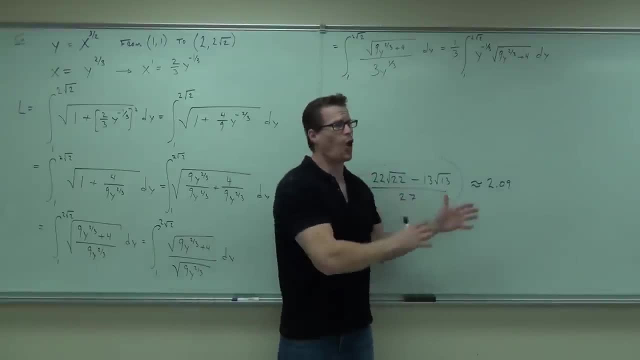 It is. Firstly, it's all algebra. Can you follow the algebra? Does your hand feel okay with that? so far, It's all algebra. Now why is that better? You can do a substitution. Check out the derivative of this. 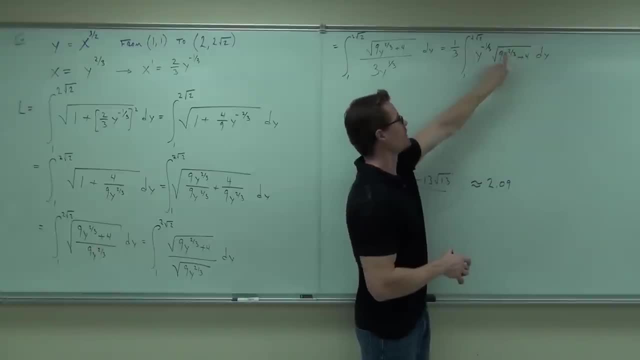 The derivative of that is going to have an y to the negative 1 third, isn't it? There's the y to the negative 1 third. It's going to work. So now we get to do our substitution and we're going to change the balance. 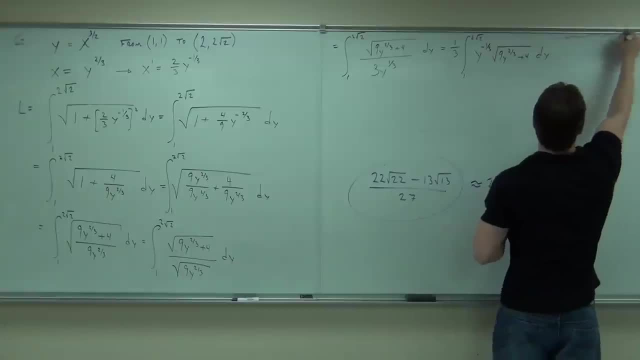 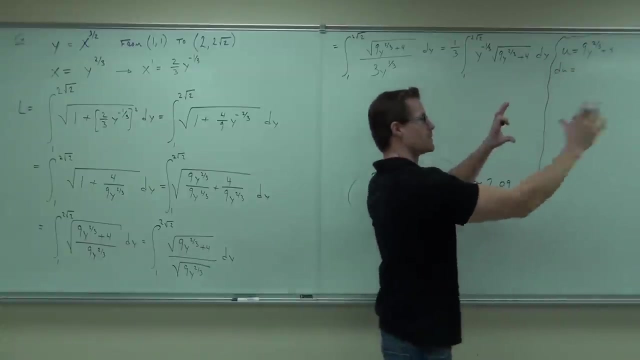 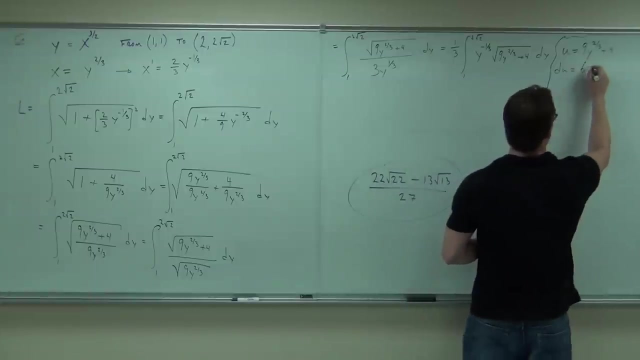 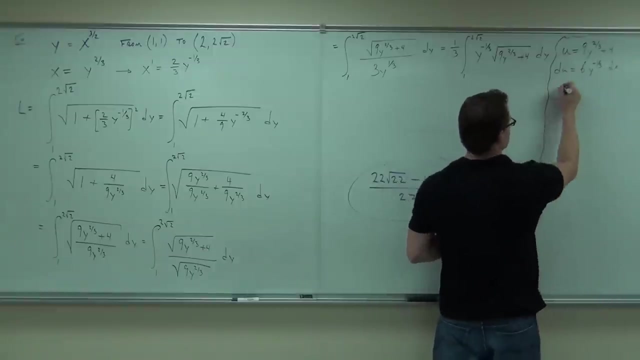 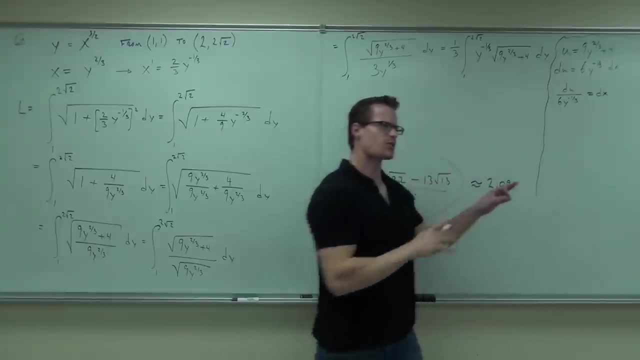 Let's see If we do substitution. du equals 2 thirds times 9.. That gives you. Let's see. So what this means is du over 6y to the negative. 1 third equals dx. Can you guys follow that as well? 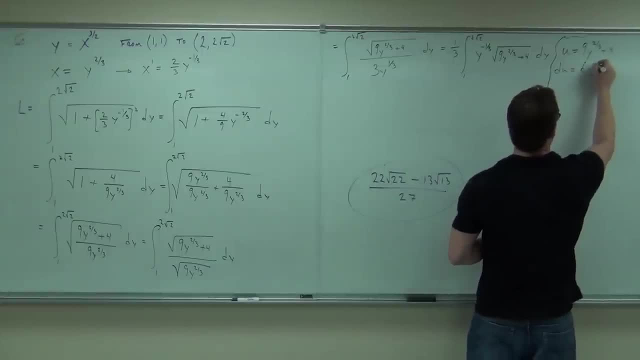 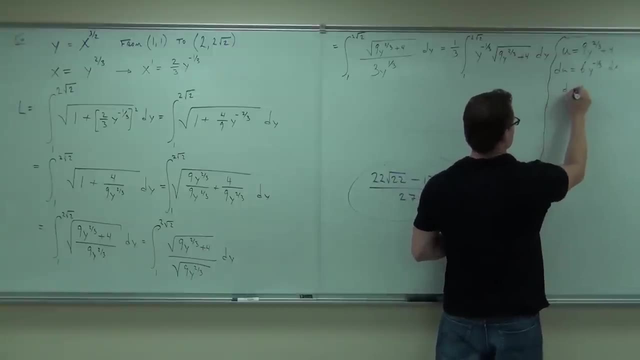 Mm-hmm. So what this means is: du over 6y to the negative. 1 third equals 6y to the negative 1 third. That gives you 6y to the negative. 1 third equals dx. Can you guys follow that as well? 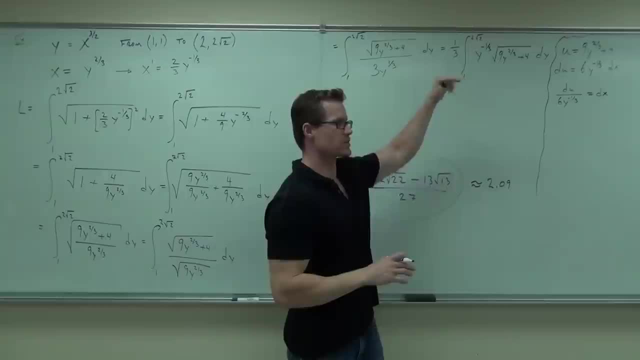 We take our derivative, just like you know how to do. 9 times 2 thirds is 6.. That's 18 over 3, that's 6.. y to the negative 1 third. sure Solve for dx, just divide that. 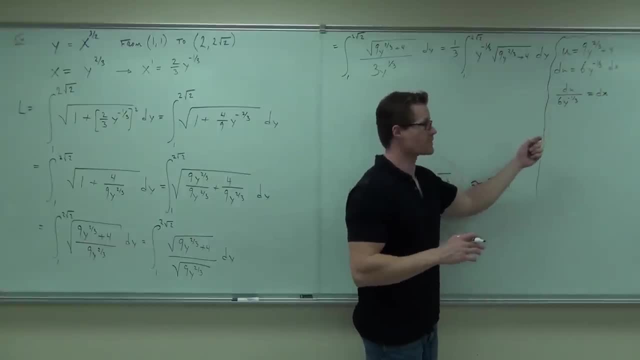 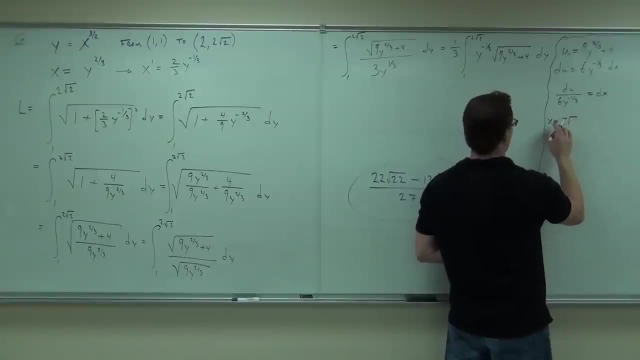 And now we're ready to do our substitution, but we want to change the balance as well, So let's practice doing that. We want x when x equals 2,- I'm sorry, y When y equals 2, root 2, and we want when y equals 1.. 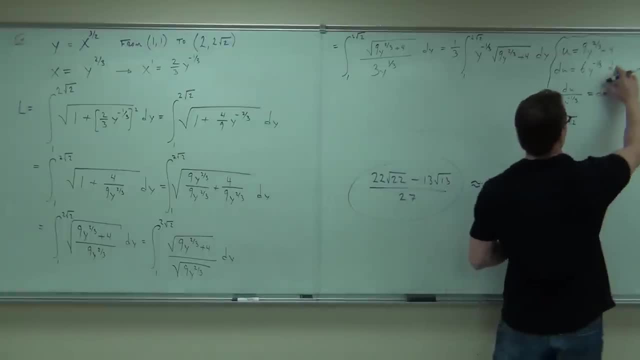 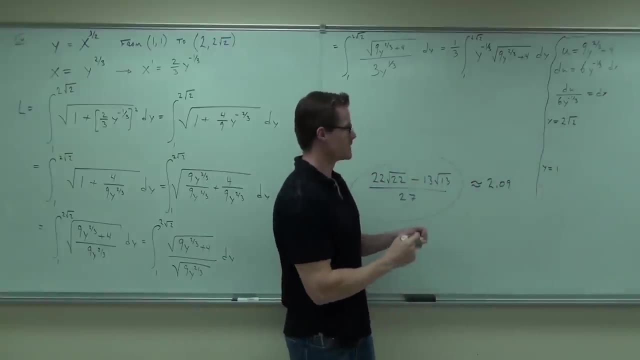 You know what you're right. I'm sorry, dy. very good, I guess we are in terms of y, aren't we? Thank you, sir, Got a little overboard there. So 2 root 2, when y equals 2 root 2, let's plug that in. 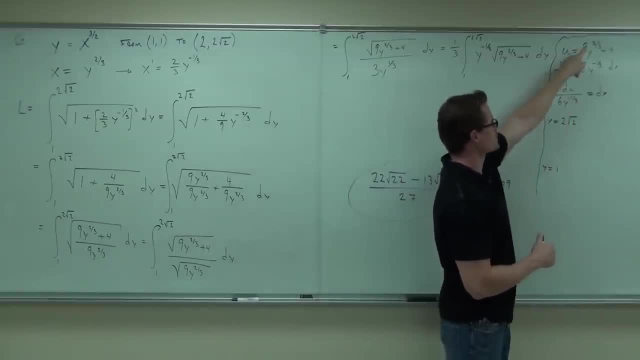 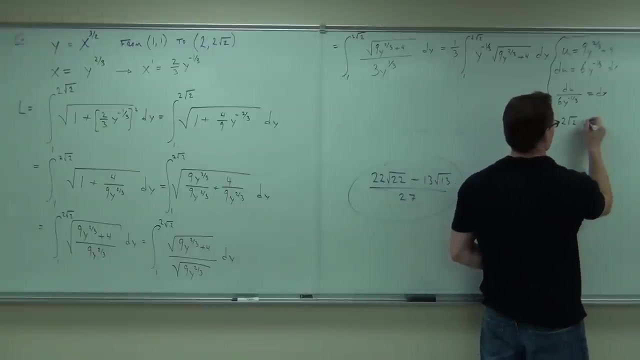 So 2 root 2, you're going to square it and take the cube root of it. Oh my gosh, 22? I'm pretty sure it's square 2.. You don't believe me, do you? I'm trusting you blindly. 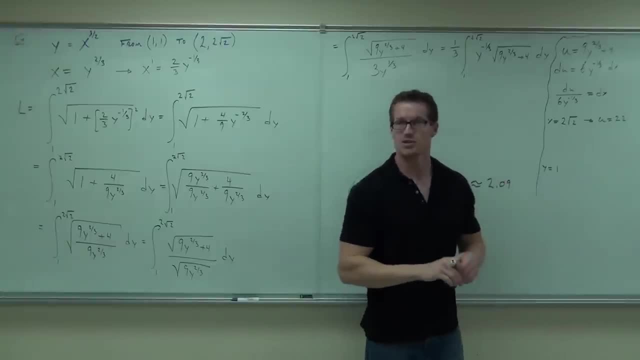 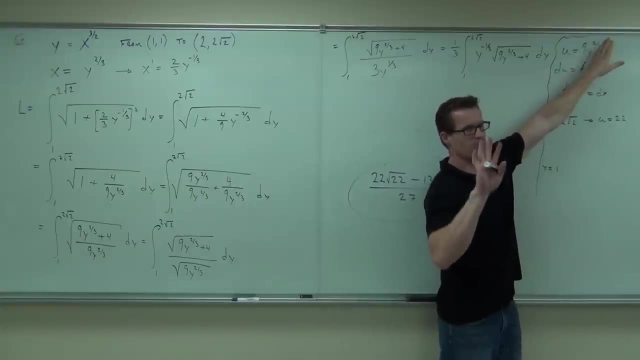 Just try it. Well, let's think about it. Do it in your head. Think about it. 2 root 2, square 2 root 2, you get 4 times 2 is just 8.. Take a cube root of 8,, you get 2 times 9 is. 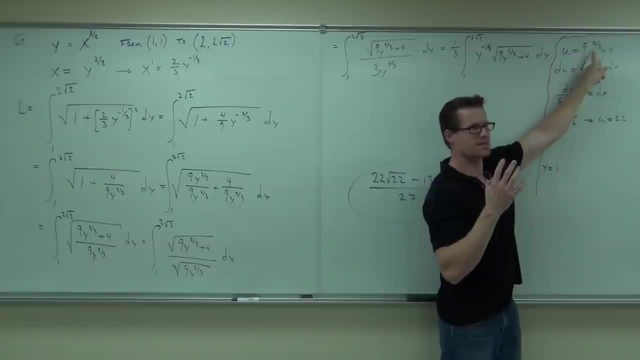 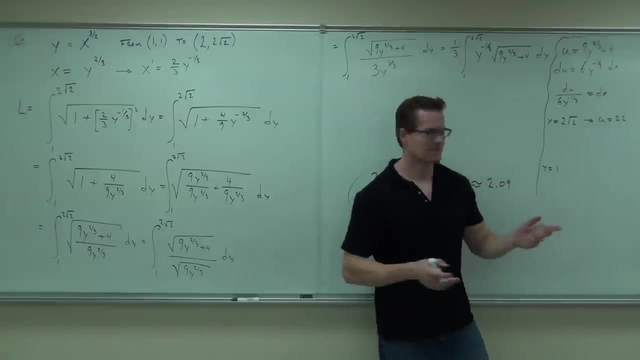 You can't do that on one hand. You can't do that on one hand. thankfully, 18 plus 4 is, You can do that one. 1.. 1's better. What's 1 to the 2 thirds. 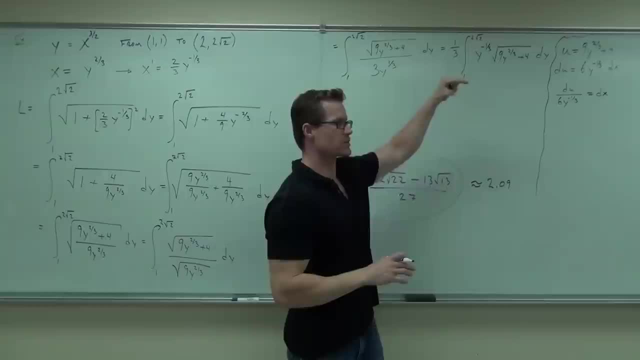 We take our derivative, just like you know how to do. 9 times 2 thirds is 6.. That's 18 over 3, that's 6.. y to the negative 1 third. sure Solve for dx, just divide that. 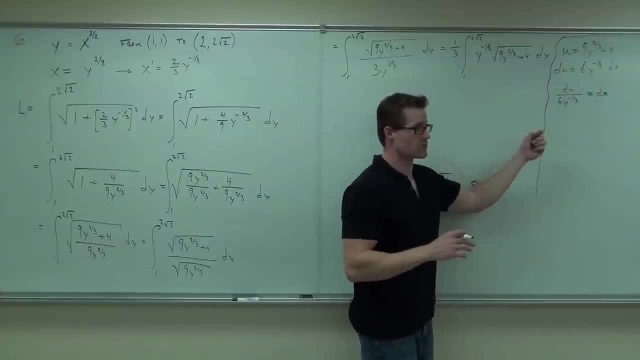 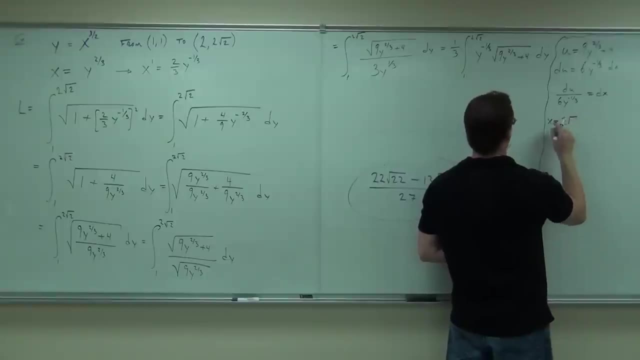 And now we're ready to do our substitution, but we want to change the balance, So let's practice doing that. We want x when x equals 2.. I'm sorry, y When y equals 2 root 2, and we want 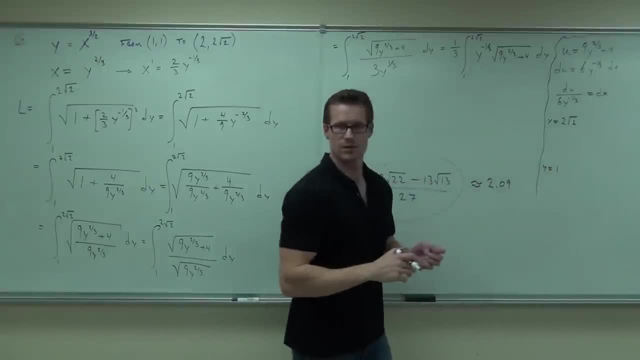 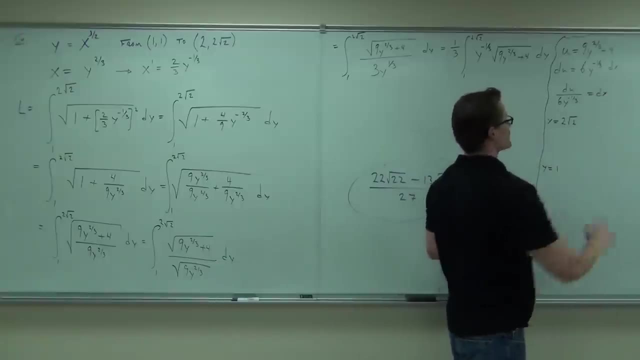 When y equals 1. We want to find out. Say what now You know what? you're right. I'm sorry, du. Very good, I guess we are in terms of y, aren't we? Thank you, sir, Got a little overboard there. 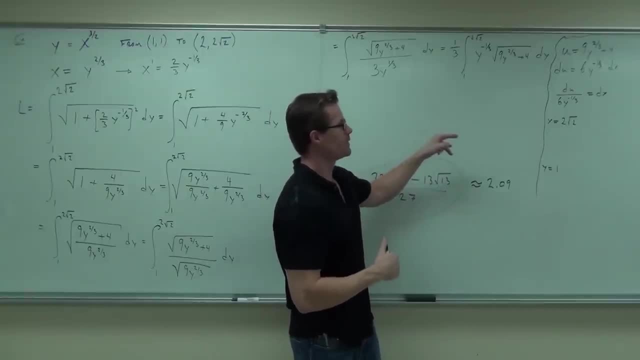 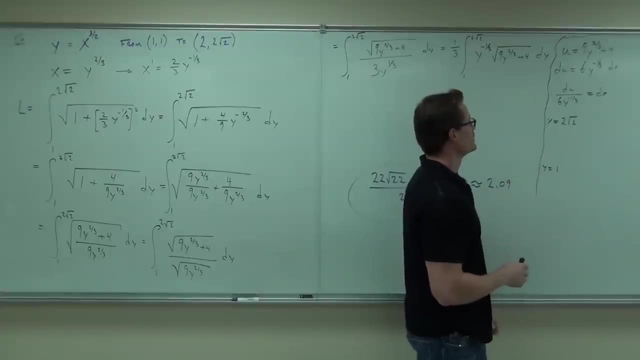 So 2 root 2, when y equals 2 root 2, let's plug that in, So 2 root 2, you're going to square it and take the cube root of it. Oh my gosh, 8,, 2,, 13,, 22?. 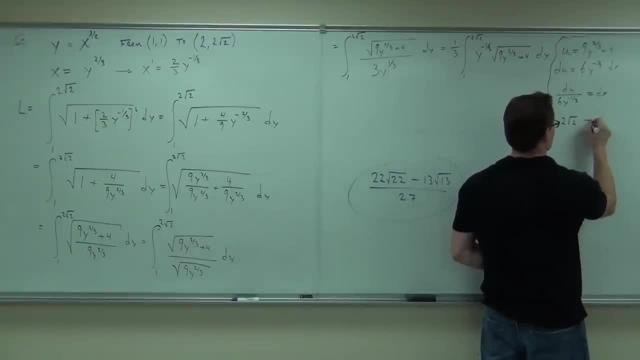 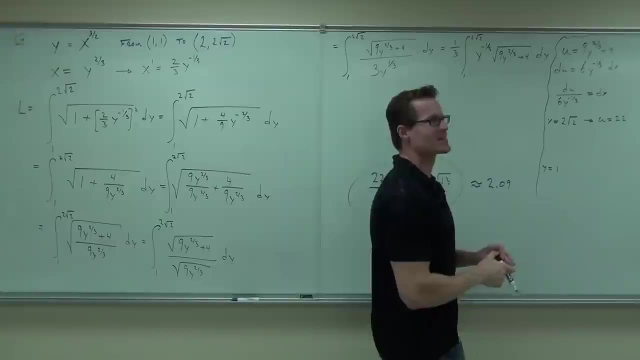 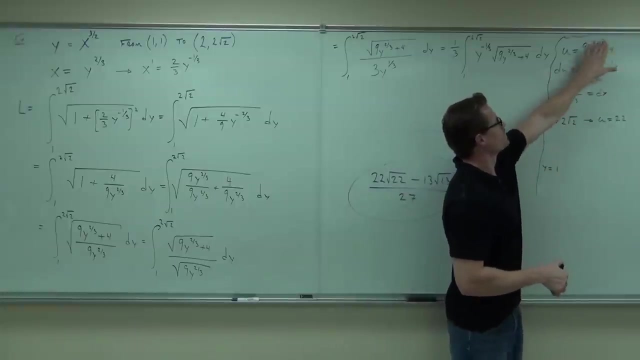 We're sure it's 22.. You don't believe me, do you? I'm trusting you blindly. Just try it. Well, let's think about it, Not just Do it in your head. Think about it: 2 root 2, square 2 root 2, you get 4 times 2, which is 8.. 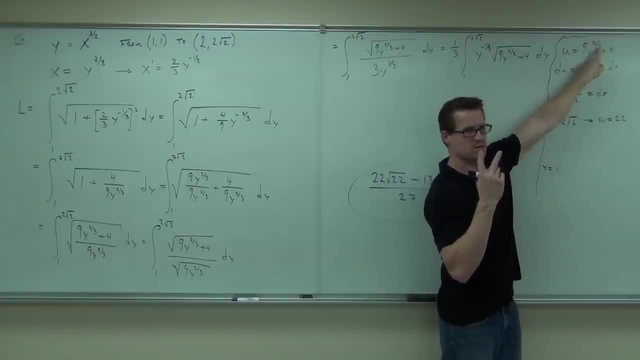 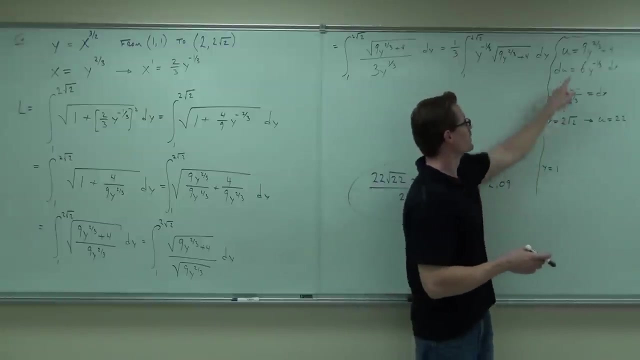 Take a cube root of 8, you get 2 times 9 is You can't do that on one hand. thankfully, 18 plus 4 is You can do that one 1. 1's better. What's 1 to the 2 thirds? 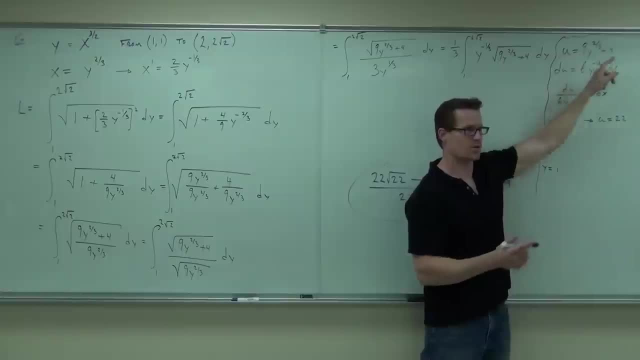 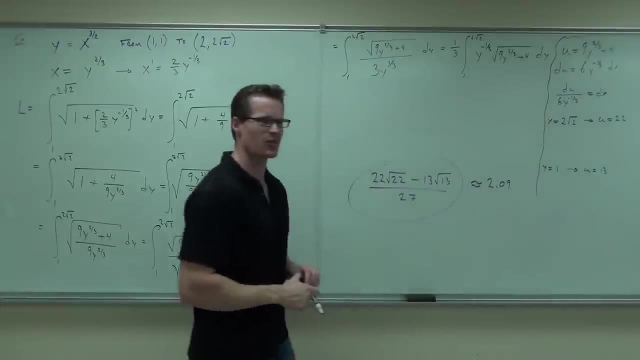 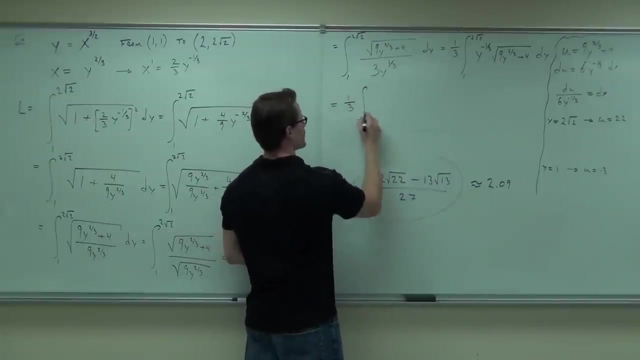 Times 9.. 9 plus 4.. The bounds are actually nicer here. See some numbers that are familiar: 1, third, Not from 1 to 2. root 2 anymore From 13 to 22.. We just changed bounds. 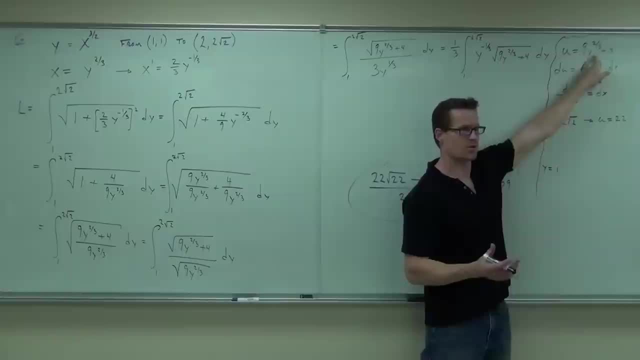 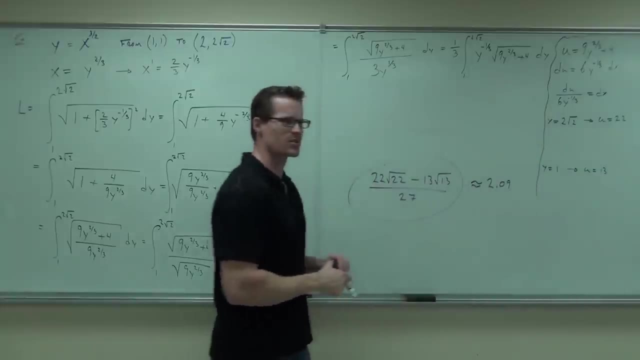 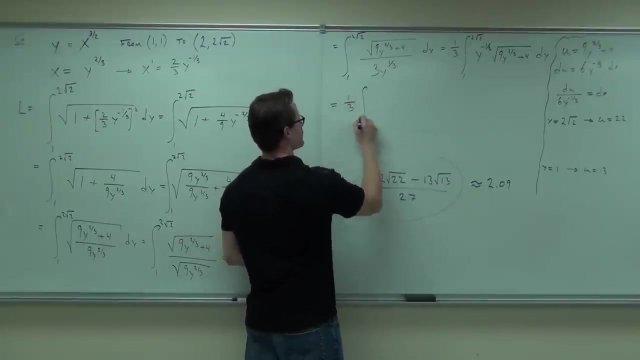 1 times 9 plus 4.. The bounds are actually nicer here. See some numbers that are familiar: Yeah, Mm-hmm. 1. third, Not from 1 to 2, root 2 anymore from 13 to 22.. 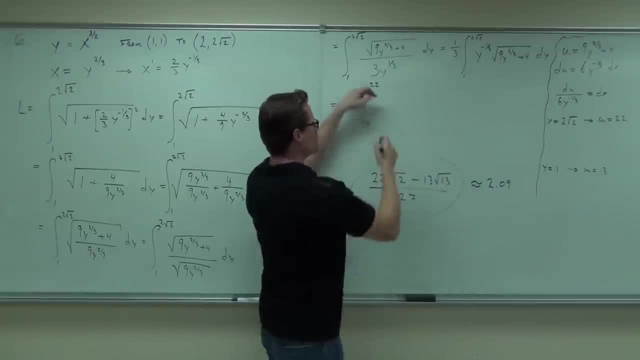 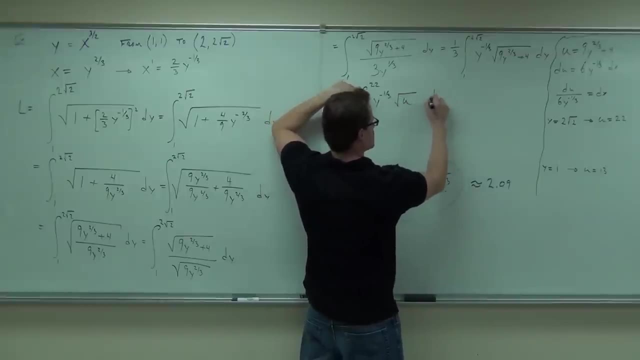 We just changed bounds. We're not in terms of y, we're now in terms of u. This is y to the negative 1 third. This is the square root of. we picked that for our u Instead of dy. we have du over 6y to the negative 1 third. 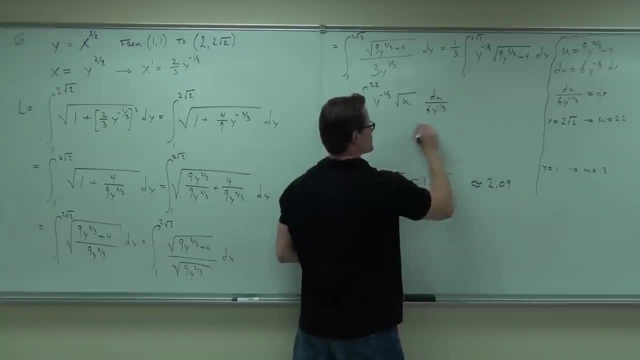 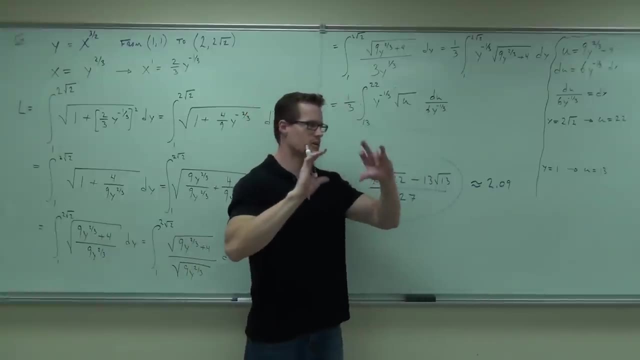 We're almost home free. We're so close. This gone. Pull out the 1 sixth. don't forget about that 1 sixth. We have 1 third. We have 1 sixth. What's it going to become? 1 eighth. 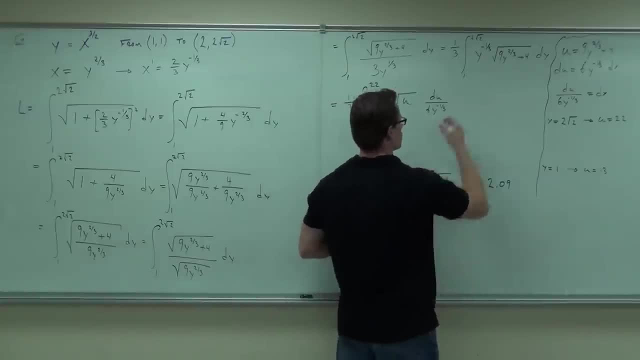 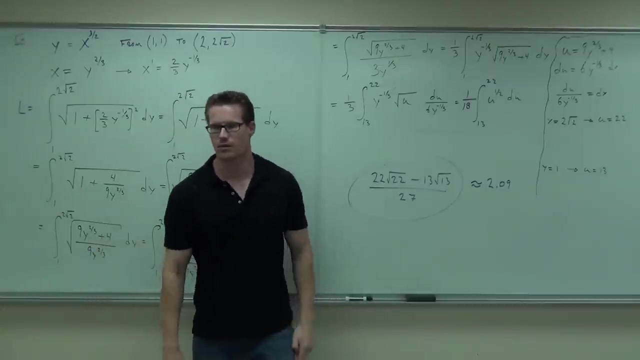 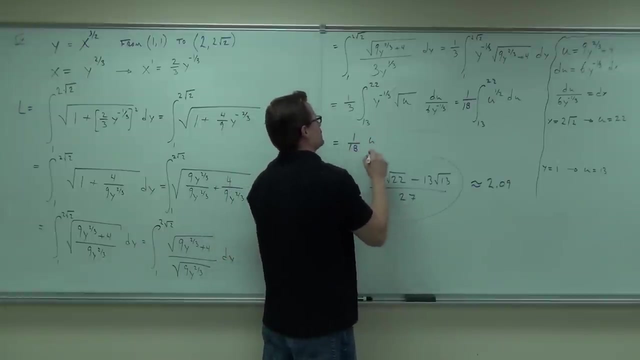 Very good. 13 to 22? u to the 1 half du. Again, the integrals are easy. They are, They're not hard. You get 1 18th? u to the. what is it? 1. 1 half? u to the 3 halves. 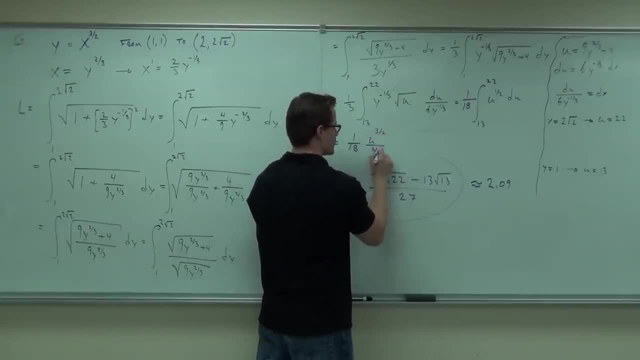 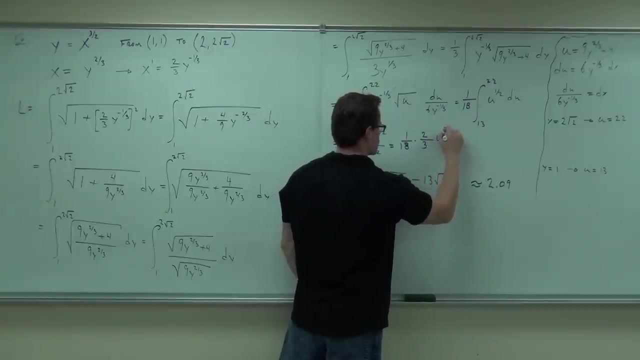 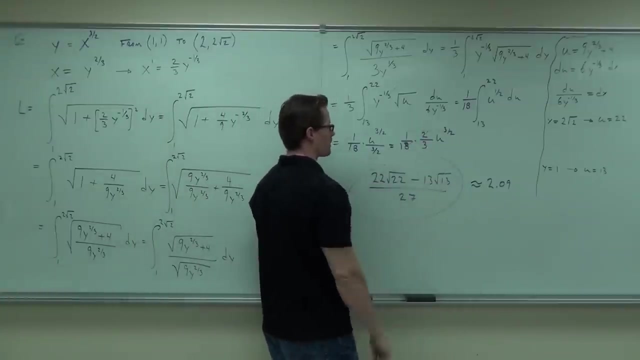 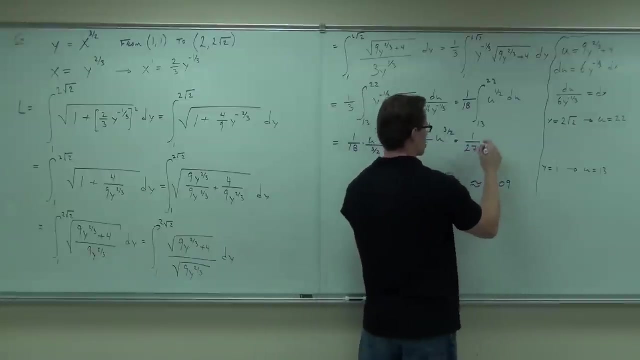 Oh, and u to the 3 halves, Over 3 halves: 1, 2.. 1 18th times 2 thirds. u to the 3 halves, Yes, no, Yes, And we're going to evaluate from 13 to 27.. 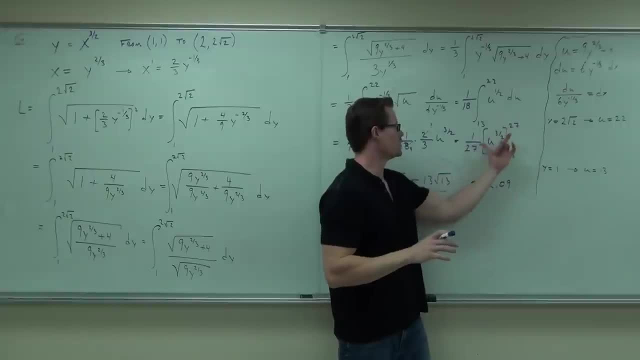 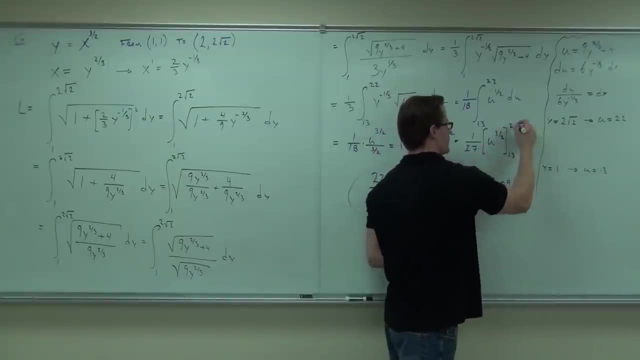 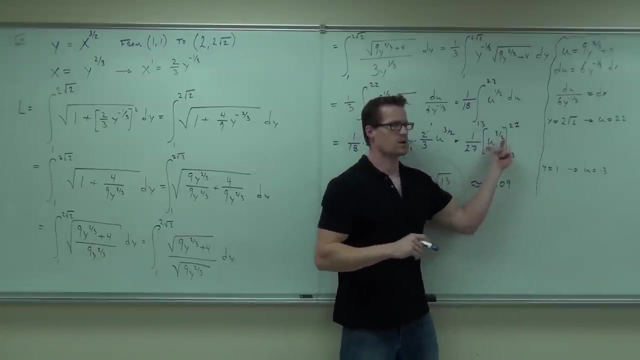 No need to plug our y's back into here. No need at all. What did I do? Oh sorry, I saw that. OK. OK, No need to plug that back in, But check it out. If you plug in the 22,, you have 22 to the 3, halves power. 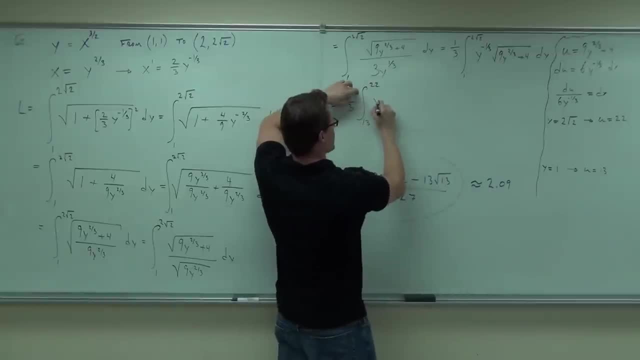 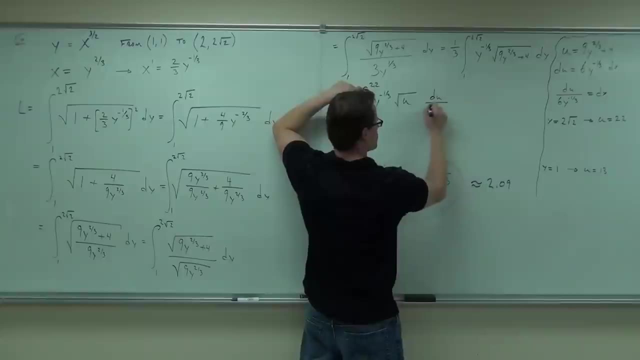 We're not in terms of y, We're now in terms of u. This is y to the negative 1 third. This is the square root of. We picked that for our u Instead of dy. we have du over 6y to the negative 1 third. 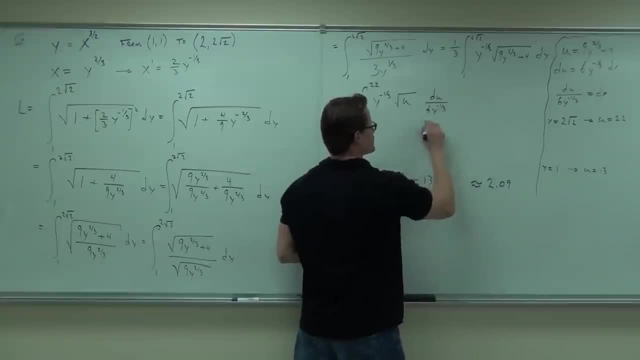 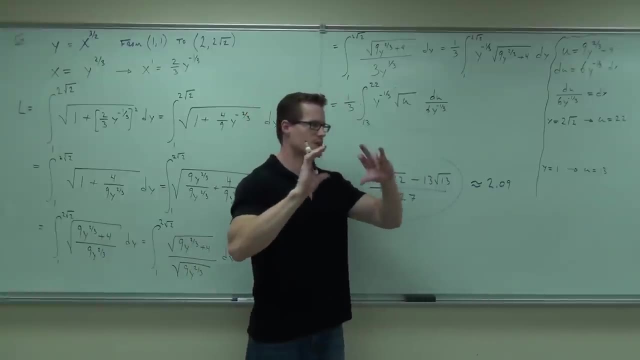 We're almost home free. We're so close. This gone. Pull out the 1 sixth. Don't forget about that 1 sixth. We have 1 third and we have 1 sixth. What's it going to become 20.? 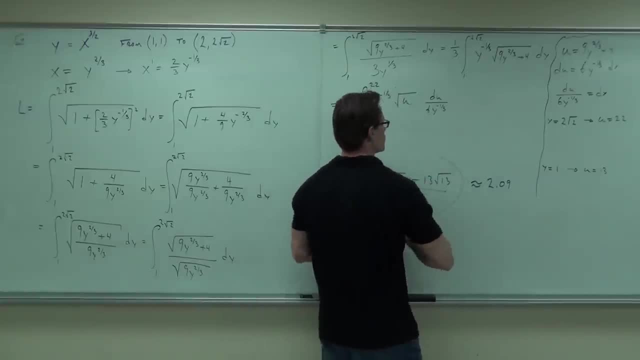 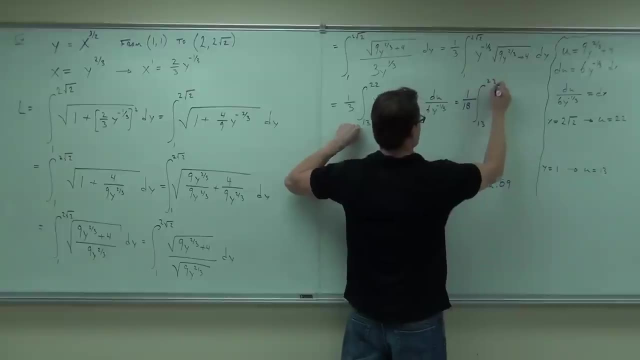 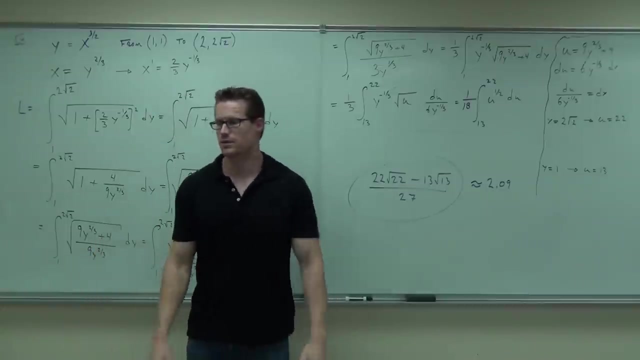 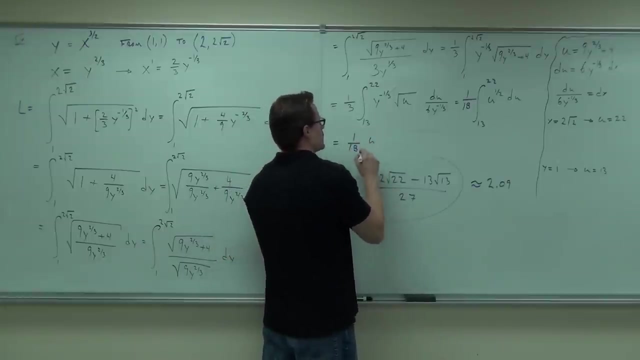 Very good, Very good: 13 to 22.. U to the 1 half. du Again, the integrals are easy, They are, They're not hard. You get 1 18th. u to the. What is it? 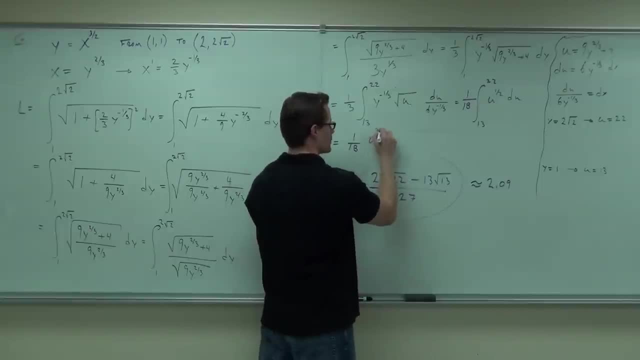 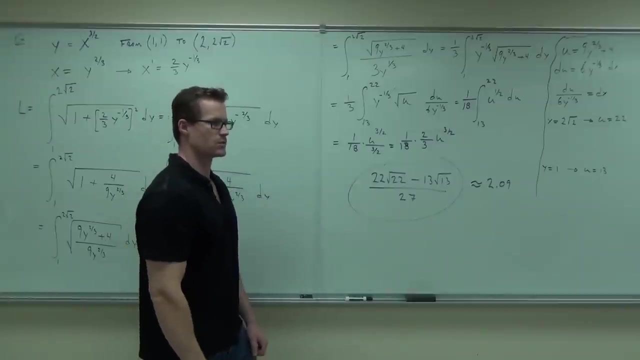 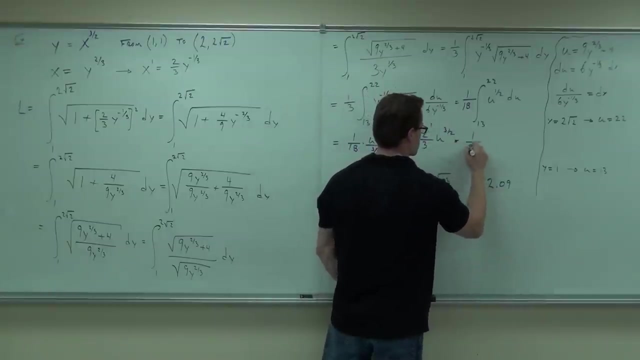 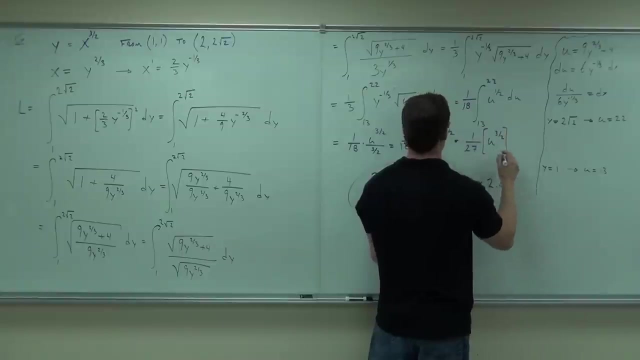 1 half Over 3 halves Over 3 halves: 1: 2.. 1 18th Times, 2 thirds of u. to the 3 halves, Yes, no, 1 27th And we're going to evaluate from 13 to 27.. 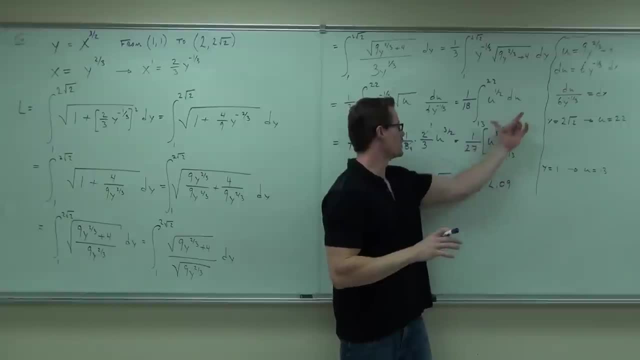 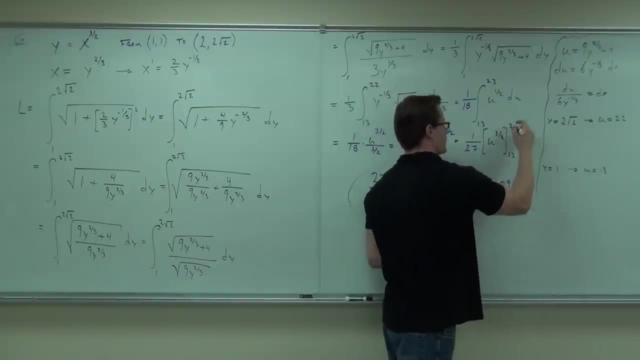 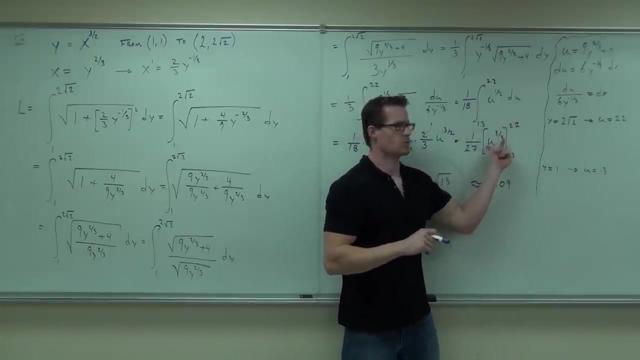 So we have no need to plug our y's back into here. No need at all. What did I do? Oh, sorry, I saw that. Okay, okay, No need to plug that back in, But check it out. If you plug in the 22,, you have 22 to the 3, halves power. 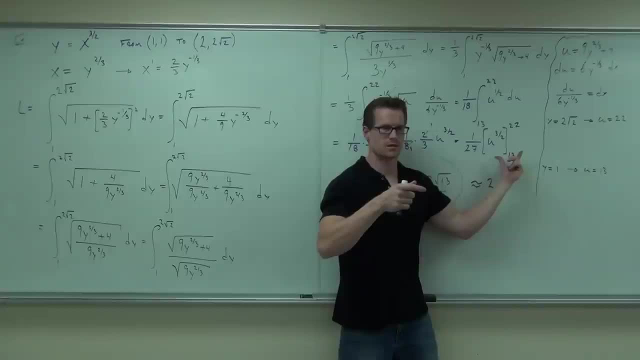 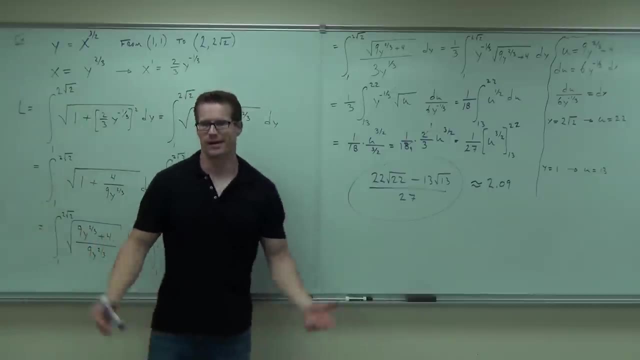 That's 22 root 22.. You plug in the 13,. you have 13, 3 halves powers. 13 root 13, all over 27.. Same answer. Which way is it going to go? Which way is easier? I don't know. 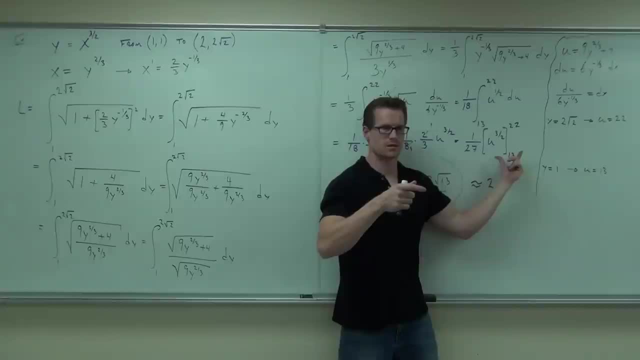 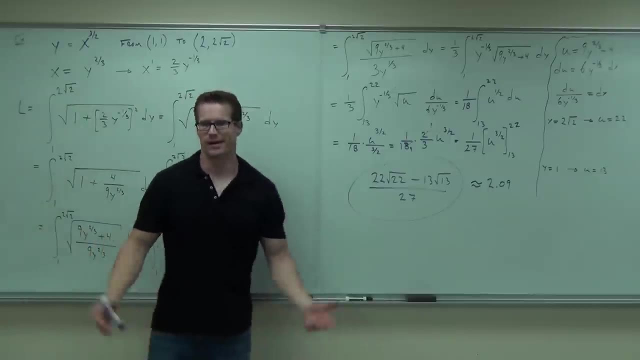 That's 22 root 22.. You plug in the 13,. you have 13, 3 halves powers. 13 root 13 all over 27.. Same answer. Which way is easier? I don't know. I don't care. 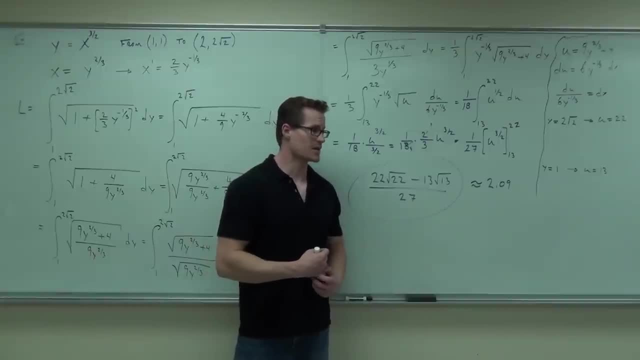 I don't care, They're both about the same. I'd say the first one is probably easier because you can see a substitution very quickly. You don't have to do any algebra ahead of time. This one, you have a lot of algebra to do. 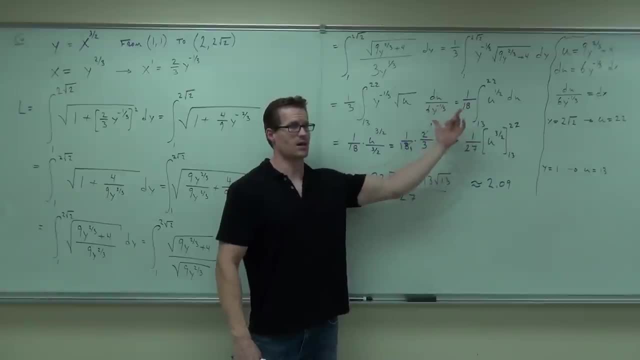 but then your evaluation is a piece of cake. Last one: the evaluation sucked. Oh man, that was really hard. This one evaluation is really easy, but the work on it was hard. So it depends on where you want to do your work, I guess. 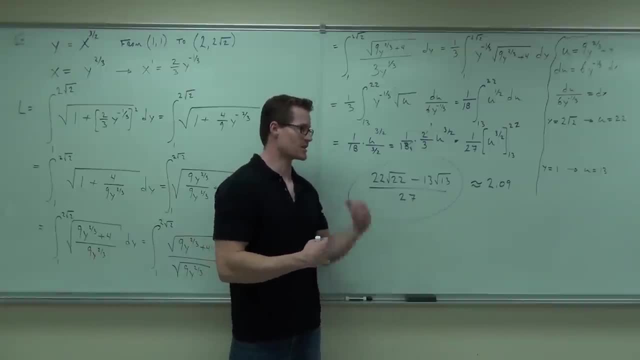 They're both about the same, I'd say the first one's probably easier because you can see a substitution very quickly. You don't have to do any algebra ahead of time. This one, you have a lot of algebra to do, but then your evaluation's a piece of cake. 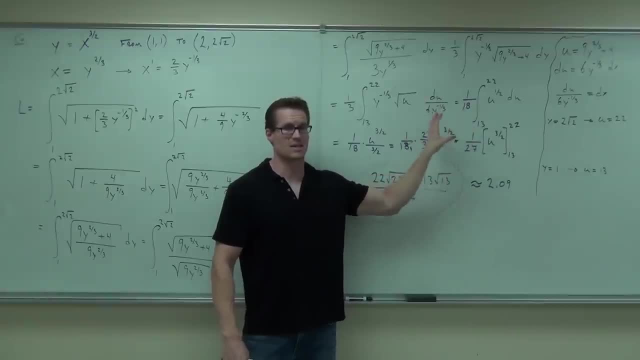 Last one, the evaluation sucked. Oh man, That was really hard. This one evaluation's really easy, But the work on it was hard. So it depends on where you want to do your work. I guess You're going to do the same thing. 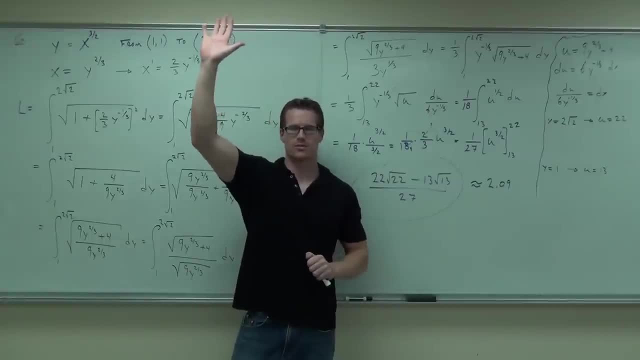 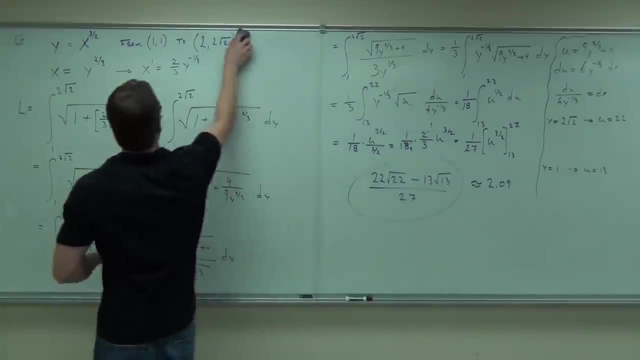 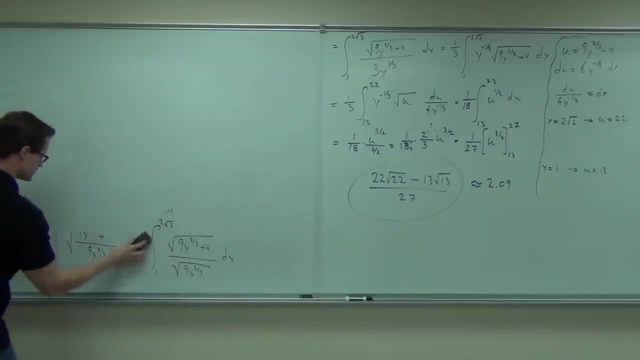 You're going to do the same work. How many of you feel OK with what we talked about so far? I need to introduce to you one more concept today. Here's the concept. I want you to imagine my famous quote. I want you to imagine my famous curve. 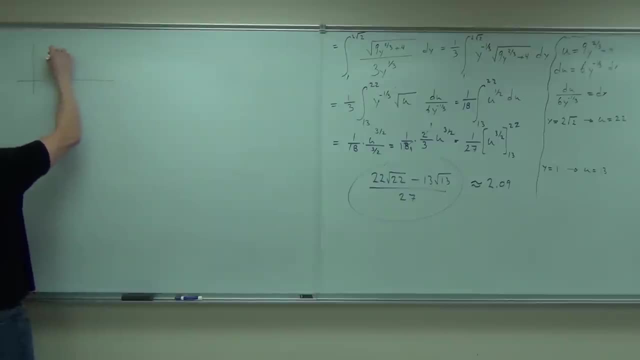 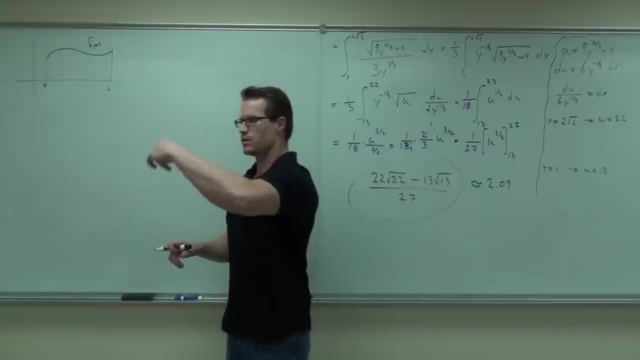 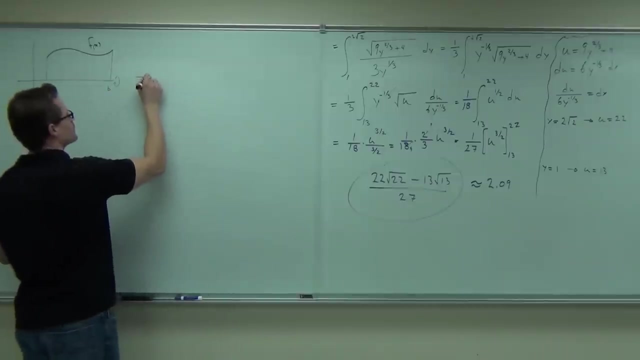 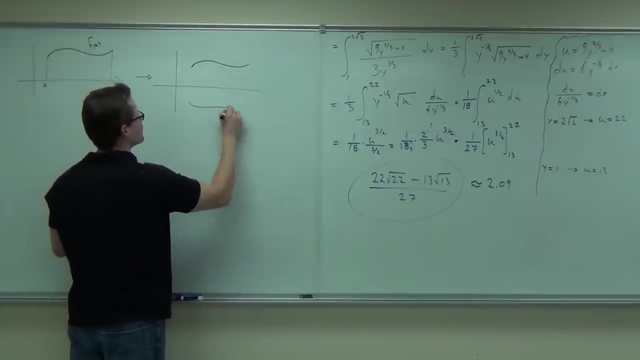 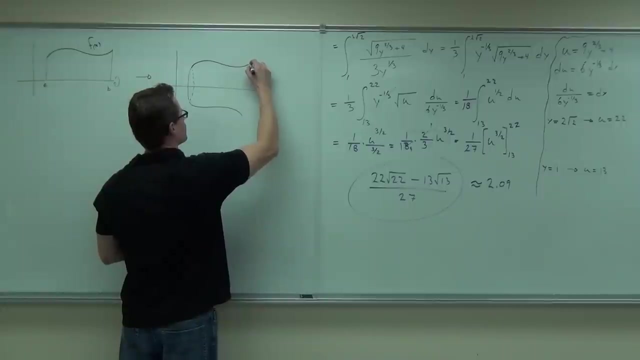 I want you to imagine my famous curve. I want you to revolve it around the x-axis. … …. 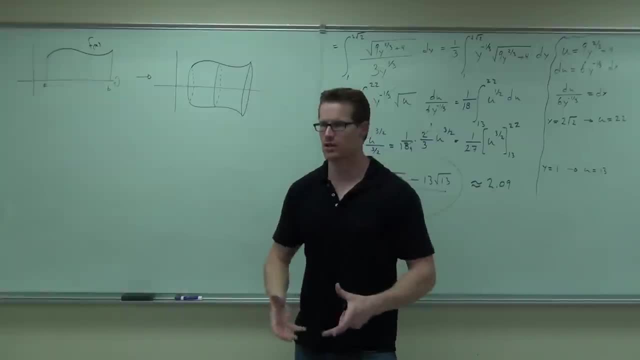 Not volume, not how much it would hold, how the surface area you would need to make it, how much service it has Outside or the inside as well. The outside Of what Covering of the outside, The inside, we are going to consider to be solid? 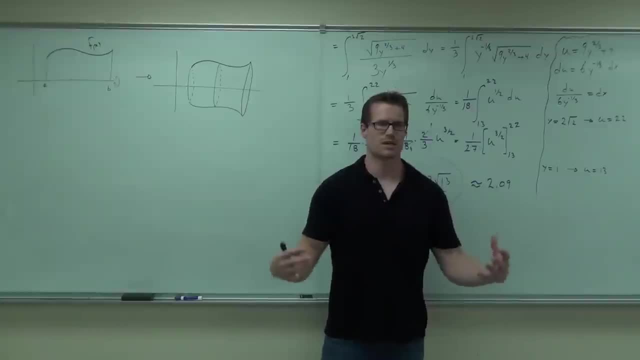 Okay, So it a solid. But we're saying: how much wrapping paper would it take if you were going to give us some as a present, because you didn't have to cover the top and the bottom? Well, tell me something. what's the cross section? 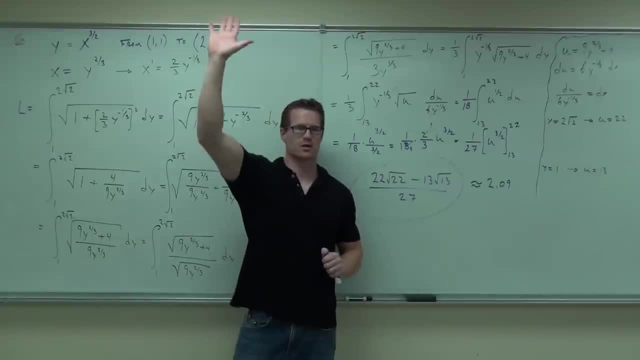 You're going to do the same thing. You're going to do the same work. How many of you feel okay with what we talked about so far? Okay, I need to introduce to you one more concept today. All right, So here's the concept. 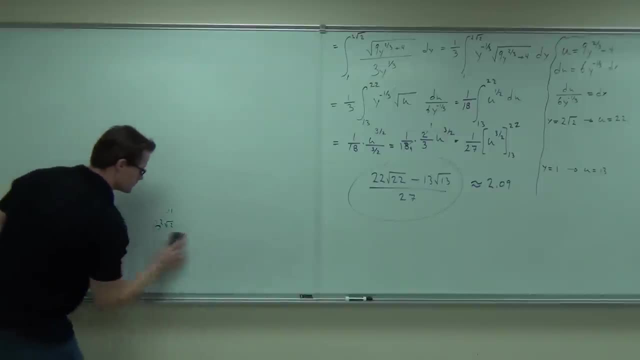 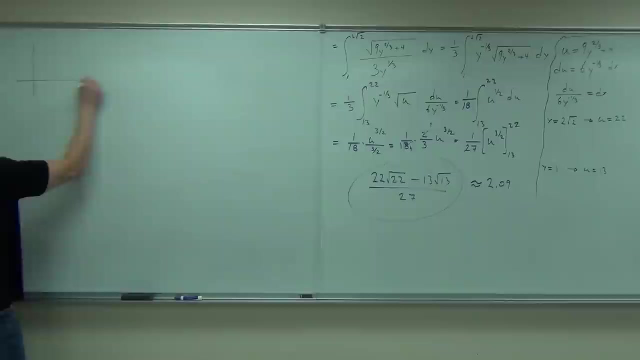 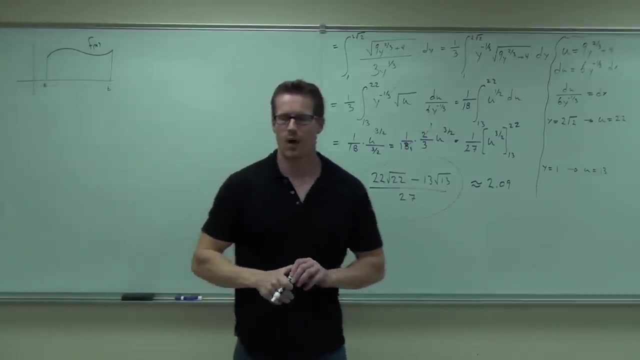 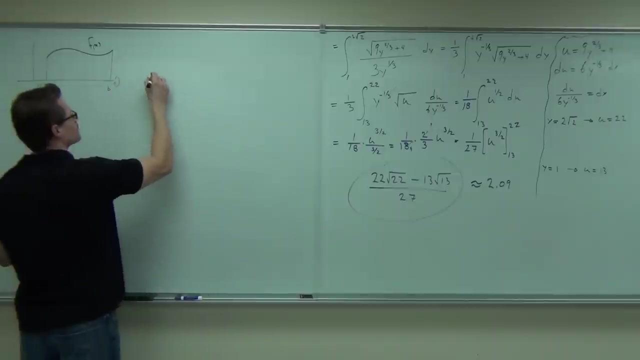 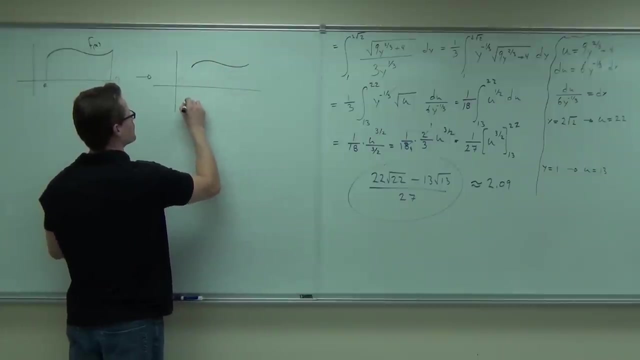 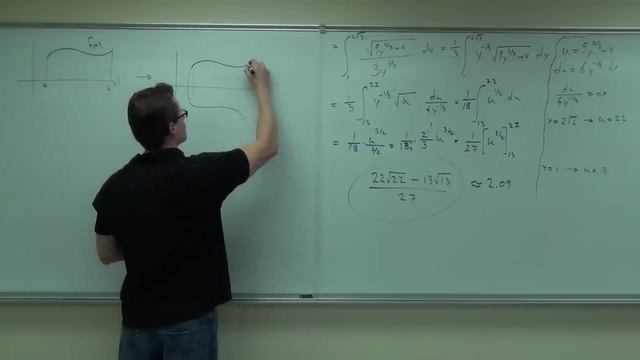 Here's the concept. I want you to imagine my famous curve. Let's see that curve. I want you to imagine What's this word? Imagine my famous curve. I want you to revolve it around the x-axis. Of course we have this before, right. you've seen that. 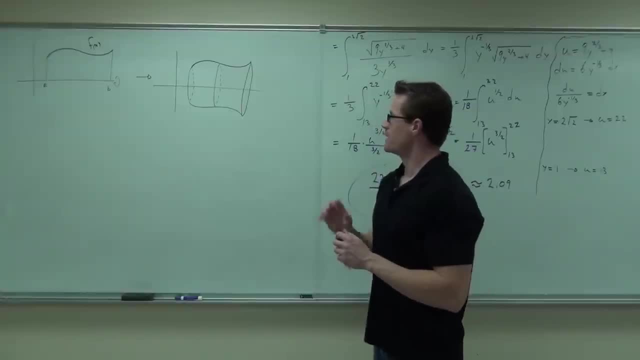 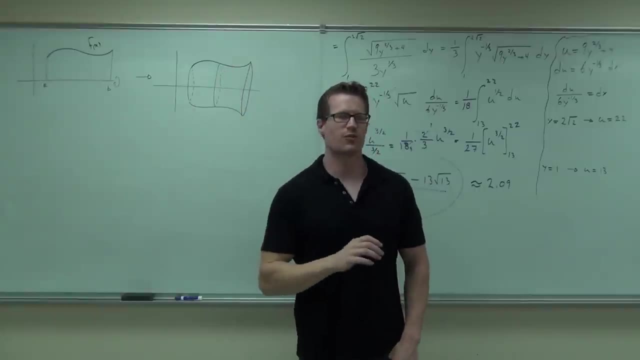 You get this sort of vase-looking thing on its side. Now, we've been able to find the length of the curve. we've been able to find the volume of this figure. What if I ask you not for the volume anymore, but I ask you for the surface area? 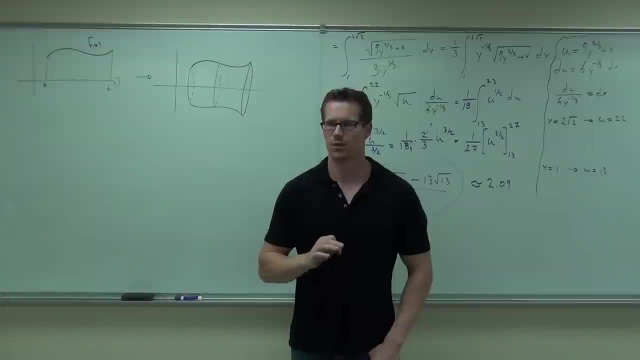 Basically, how much wrapping paper exactly would it take to cover that figure? So not volume, not how much it would hold, how much surface area you would need to have to make it, How much surface it has On the outside or the inside as well. 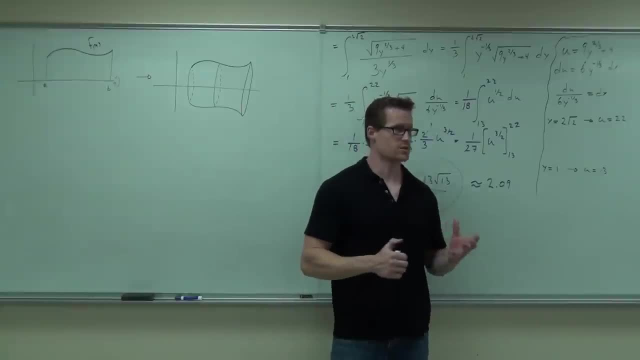 The outside, covering of the outside, The inside we're going to consider to be solid. okay, so it's a solid, But we're saying how much wrapping paper would it take if you were going to give us some as a present so you didn't have to cover the top and the bottom? 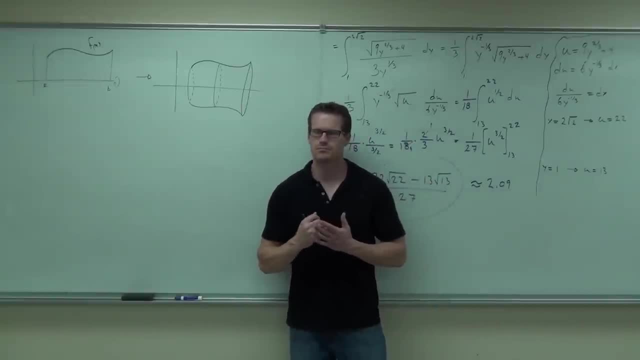 Well, tell me something. what's a cross-section? No, that would be the area. What's the cross-section? The cross-section is a circle, The surface area. Okay, The surface area of the cross-section would be, of course, pi? r squared. 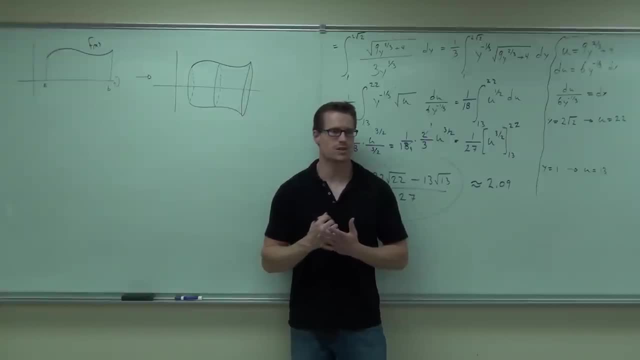 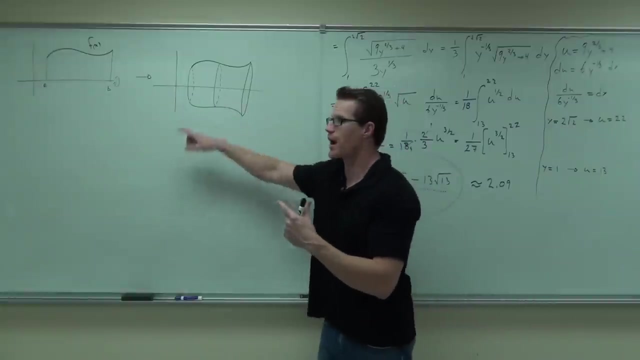 No, that would be the area. What's the cross section? The cross section is a circle. The surface area of the cross section would be, of course, pi r squared. But I'm not asking for the area, am I? I'm asking for what? does it have to do with going around something? 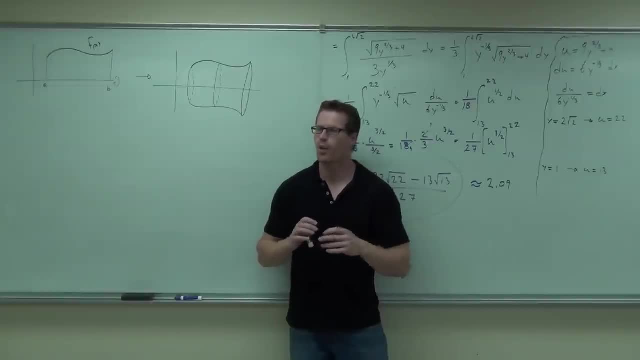 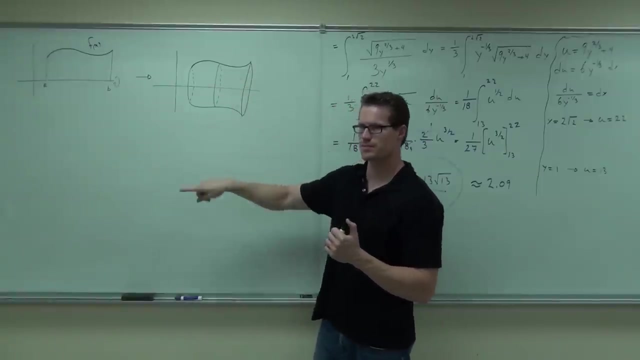 But I'm not asking for the area, am I? I'm asking for what? does it have to do with going around something? The circumference. Can you find the circumference of a circle? What is it? So if I take cross-section and find the circumference- and I do that at every little point and add: 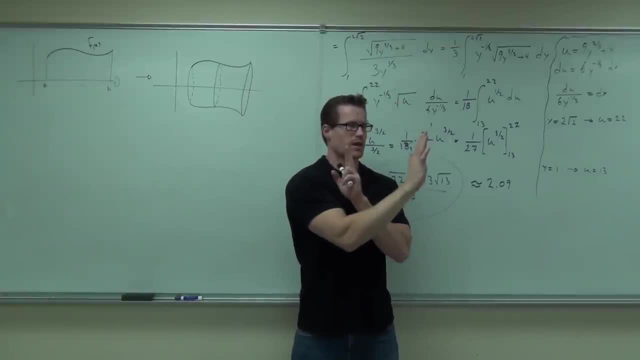 up all those circumferences throughout the whole length. can you see that I'm going to get the surface area, The surface area of this figure. So our idea is here to take the circumference times the length and integrate it. Now we've already found the length, we just need to incorporate what the circumference 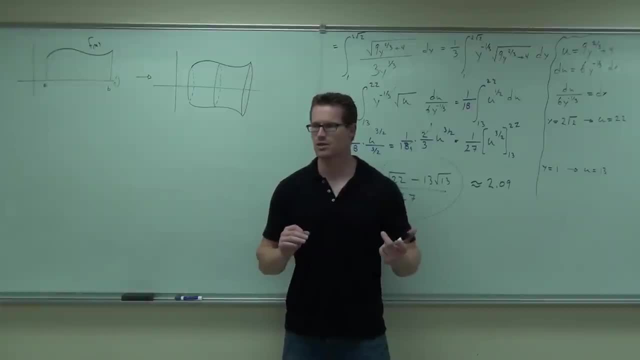 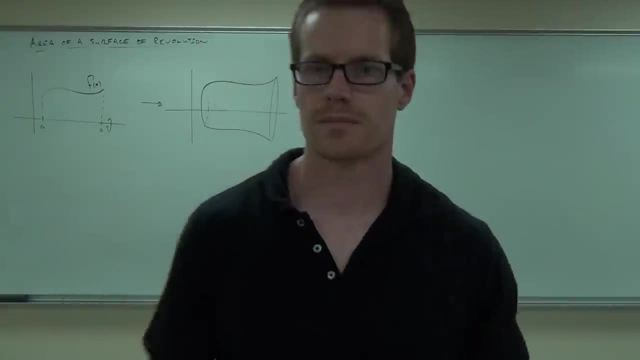 is and very, very quick and easy. next time I'll show you how to do that. I'll give you maybe one or two examples, and that will be it. Okay, so we're all alone. There's no class in here today, but I'm going to give you a pretty thorough explanation. 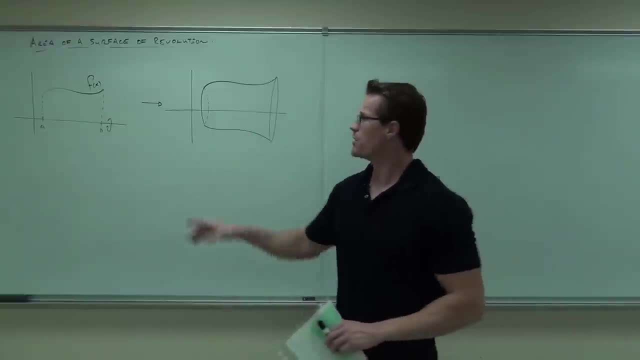 on how to find the surface area of a rectangle. Okay, So what we're going to do is we're going to start with a revolution. The idea is: start with a function, just my famous function, and we're going to revolve that around the x-axis and try to find the surface area of the solid that we create. 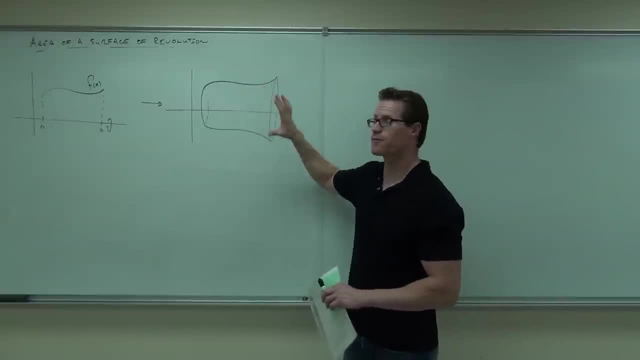 So basically, how much wrapping paper would you need to cover this entire figure on the outside? We're not going to include the ends, so we're going to leave those open, but basically how much wrapping paper around The ends would be just a basic geometry problem. 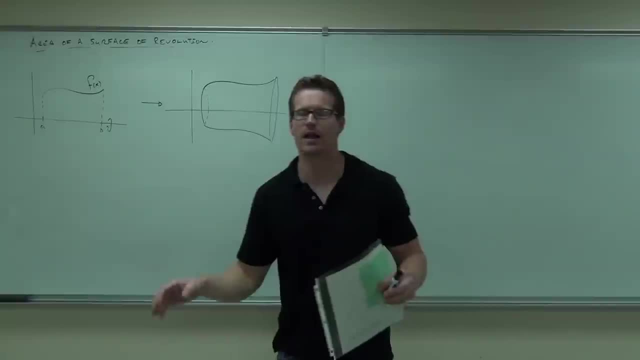 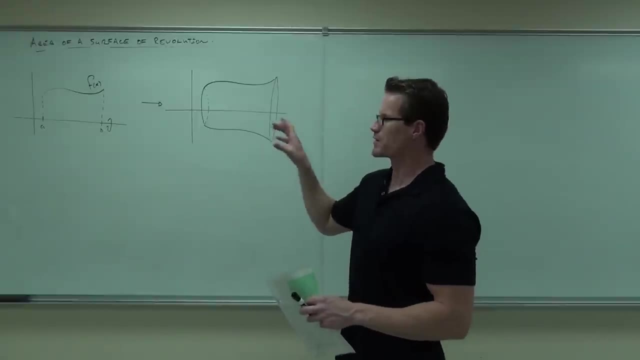 Area of a circle. area of a circle. So we're going to not do that, but we are talking about the surface area of that figure. Now I want to kind of posit this: that the surface area is a combination of the circumference of a circle times its length. 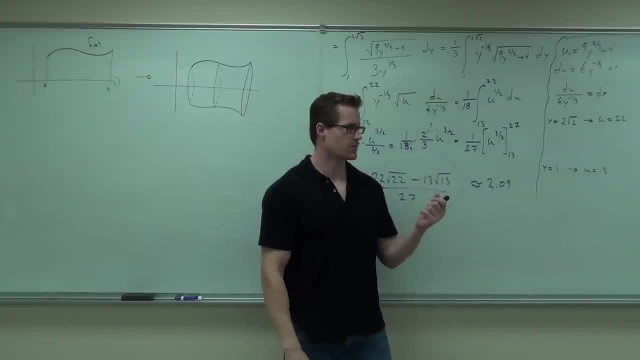 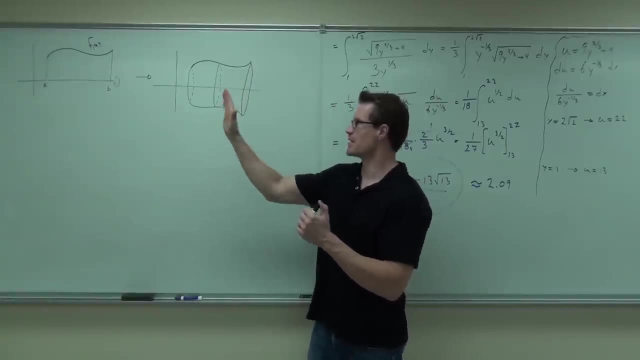 The circumference, The circumference. Can you find the circumference of a circle? What is it? So, if I take cross section and find the circumference- and I do that at every little point- and add up all those circumferences throughout the whole length, can you see that I'm going to? 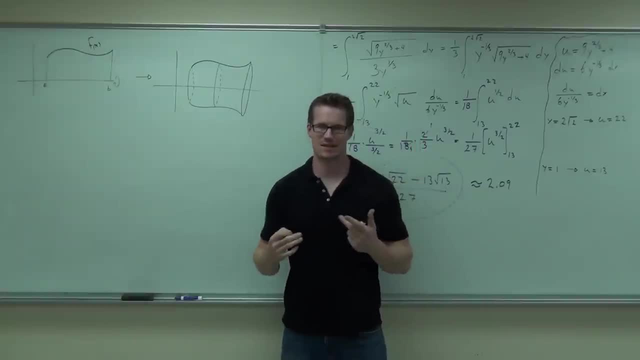 get the surface area of this figure. So our idea is here: to take the circumference times the length And integrate it. Now we've already found the length. We just need to incorporate what the circumference is and it will be very, very quick and easy. 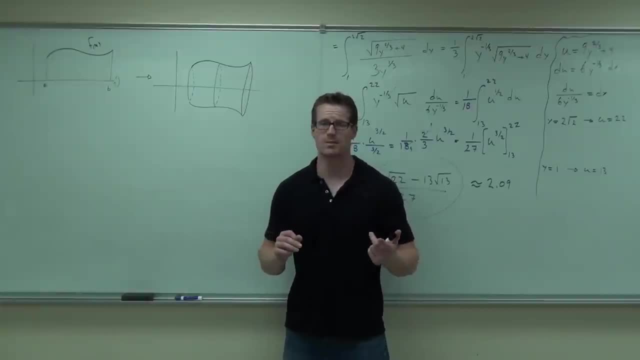 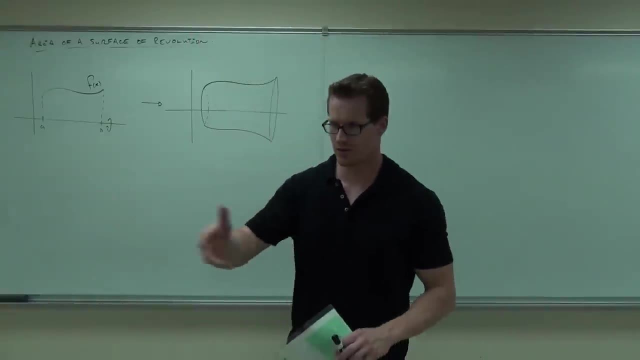 next time. I'll show you how to do that. I'll give you maybe one or two examples, and that will be it. Okay, so we're all alone. There's no class in here today, but I'm going to give you a pretty thorough explanation. 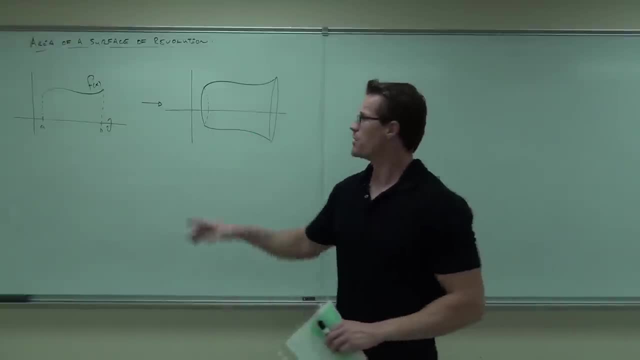 on how to find the surface area of revolution. The idea is, start with a function, just my famous function, and we're going to revolve that around the x-axis And try to find the surface area of the solid that we create. So, basically, how much wrapping paper would you need to cover this entire figure? on the 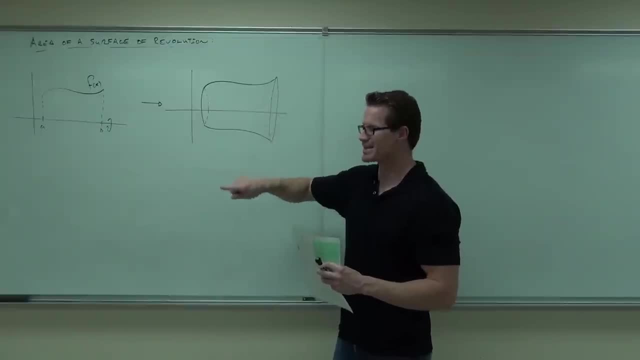 outside. We're not going to include the ends, So we're going to leave those open. but basically, how much wrapping paper around The ends would be just a basic geometry problem. Area of a circle, area of a circle. So we're going to not do that. 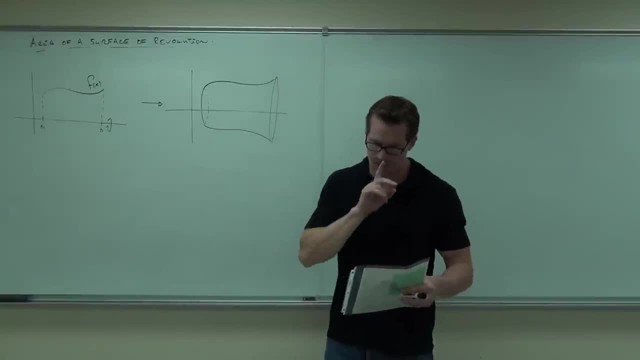 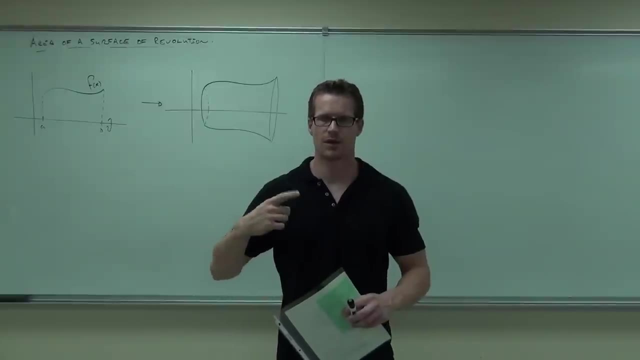 But we are talking about the surface area of that figure. Now I want to kind of posit this: that the surface area is a combination of the circumference. circumference of a circle times its length. So when you think of surface area, it would be, how far around do you have to go at each? 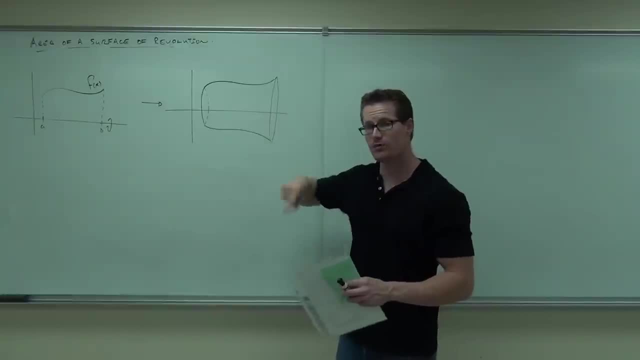 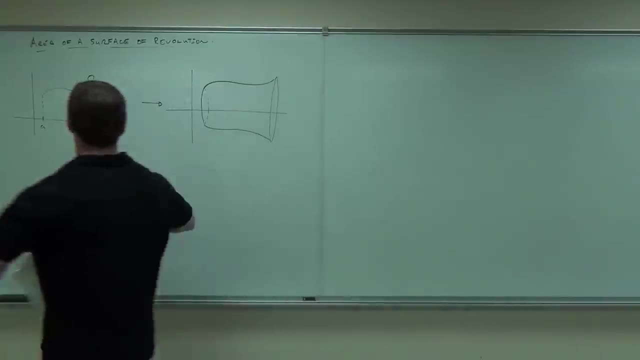 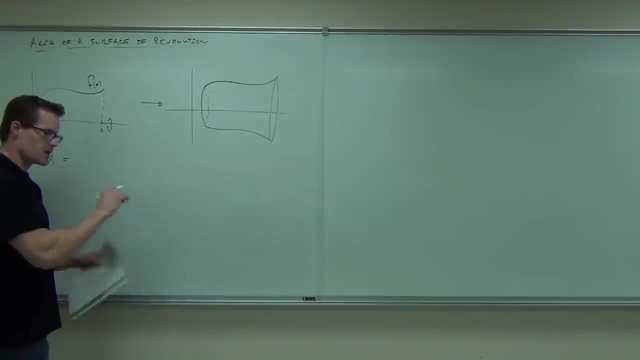 little place on this figure. Then add up all of those surface areas, an infinite number of them, and you're going to get the surface area of the whole entire figure. So the idea is: surface area equals circumference times length. Okay, Okay. 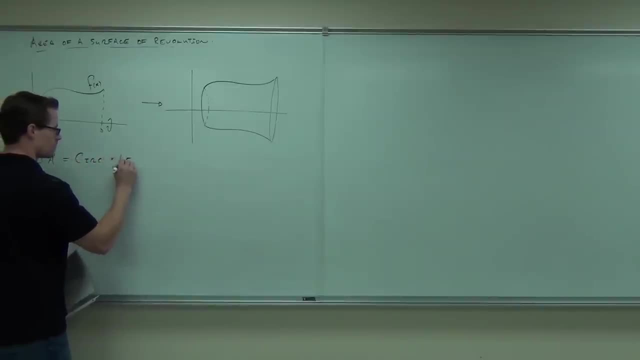 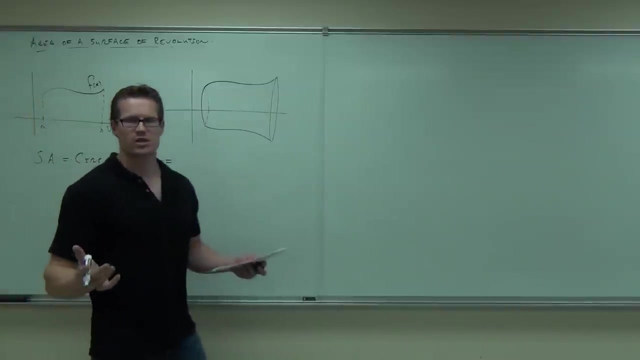 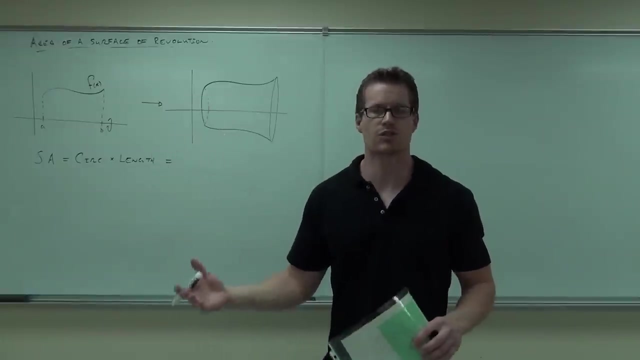 Okay, Okay, Okay. Ore Center per second. Sorry about that Process Prax "-". Well, if you think about it, what shape are we making here? What's the cross section of any of these cuttings? When you think about it, you say yeah, of course. 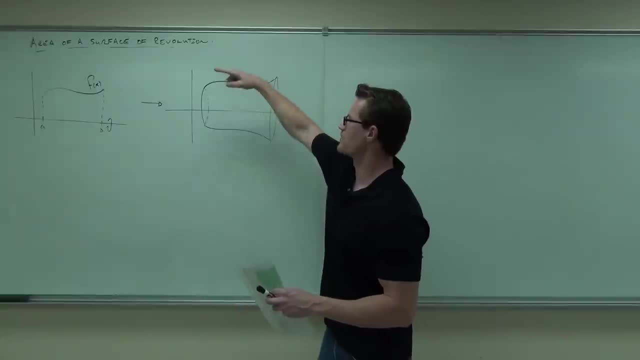 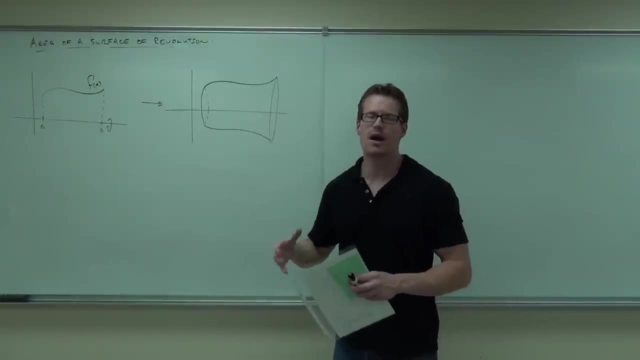 So when you think of surface area it would be: how far around do you have to go at each little place on this figure? then add up all of those surface areas, an infinite number of them, and you're going to get the surface area of the whole entire figure. 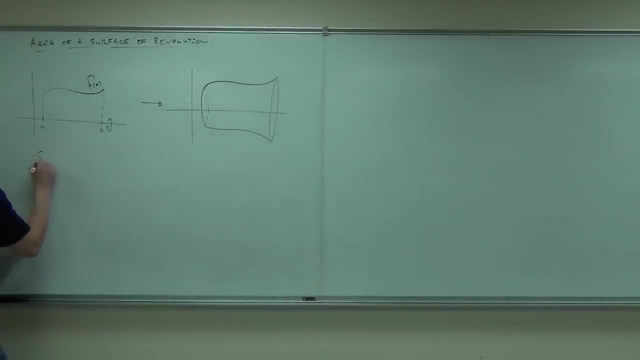 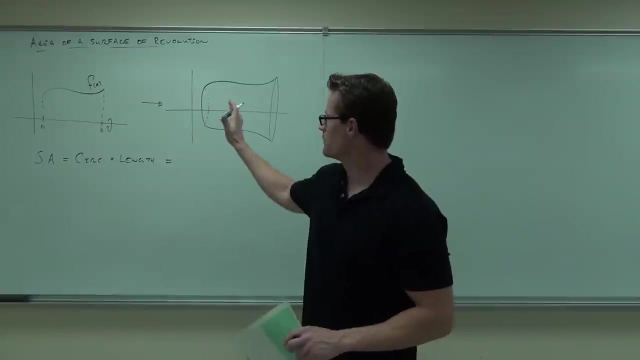 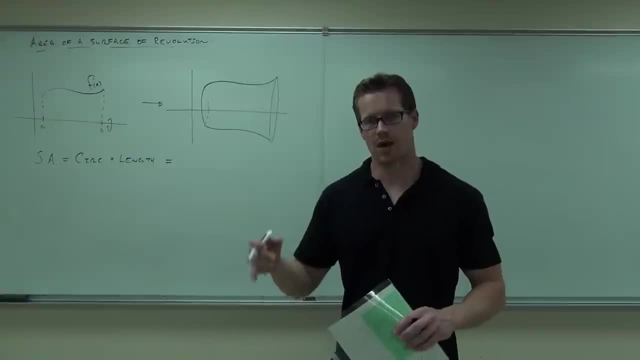 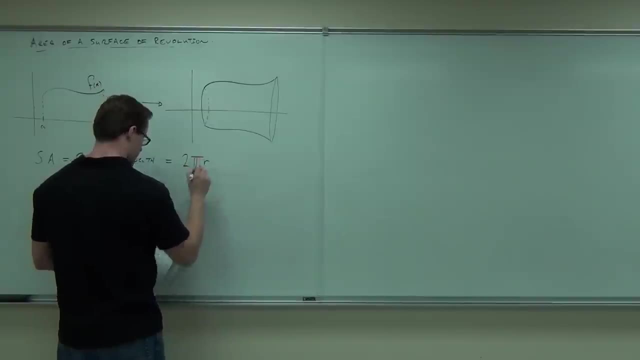 And when you think about it you say, well, yeah, of course it's a circle. What's the circumference of a circle? And we know that as 2 pi r, So we're going to get circumference times, length, 2 pi r times, whatever the length happens. 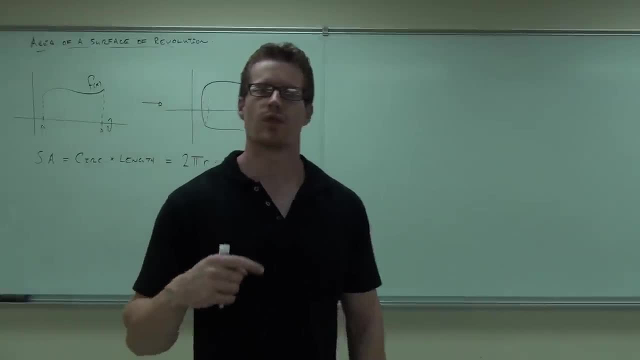 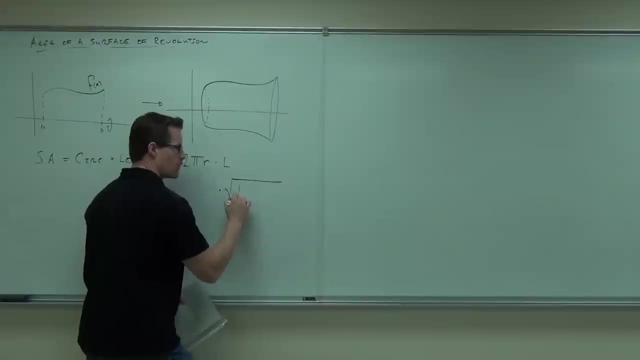 to be Now. if you think back and you watch previous videos, we know that we've already done length. We know that length is actually the square root of 1 f, prime of x, and we'll have a dx of the square root, sorry, and we'll have a dx at the very end. 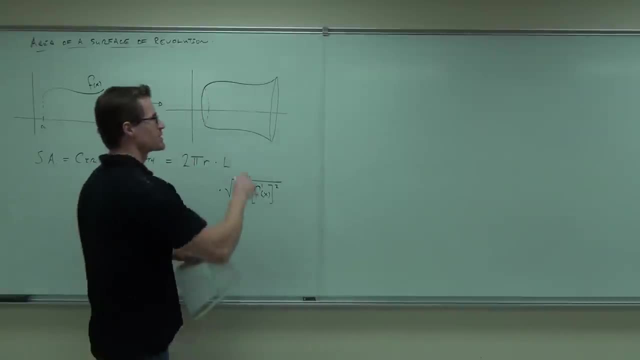 2 pi? r. think about what the radius actually is. The radius is the distance between the two. The radius is the distance between the two. The radius is the distance from here to here at any given point. The distance from the x axis to the function is the function. 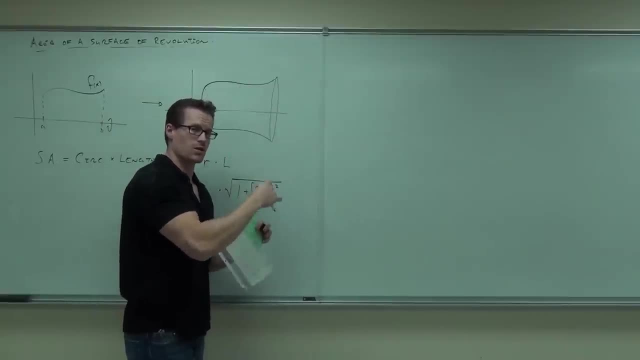 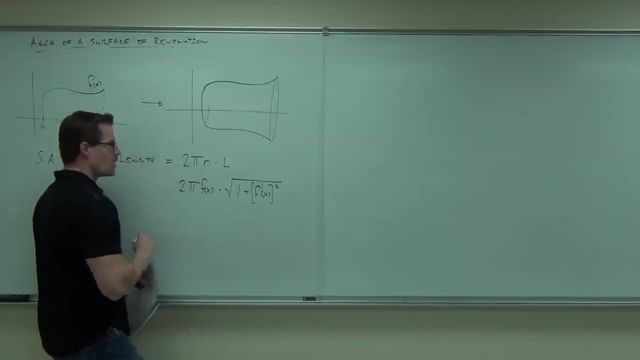 You plug in whatever the x is, it's going to give you the height. So the radius in our case is simply f of x. So we have 2 pi f of x. What that means is that for us to find, and we're going to integrate, of course, at every. 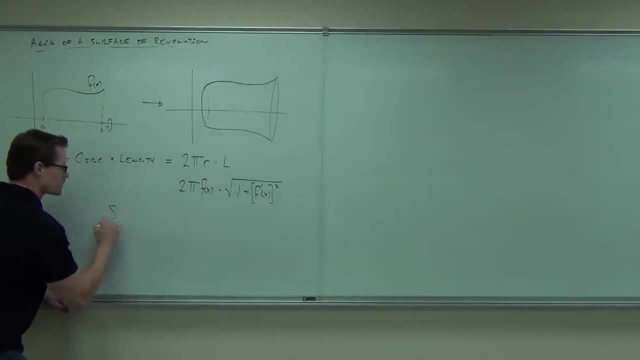 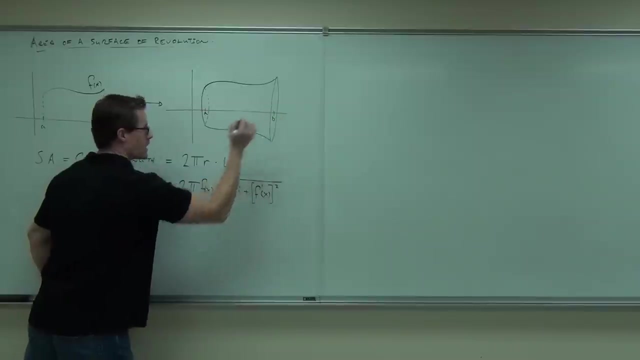 single point. So for us to find the surface area, Surface area is going to equal. Surface area is going to equal An integral, from where we start to where we stop, of 2 pi. that's coming from the circumference F of x times 1 plus f, prime of x squared dx. 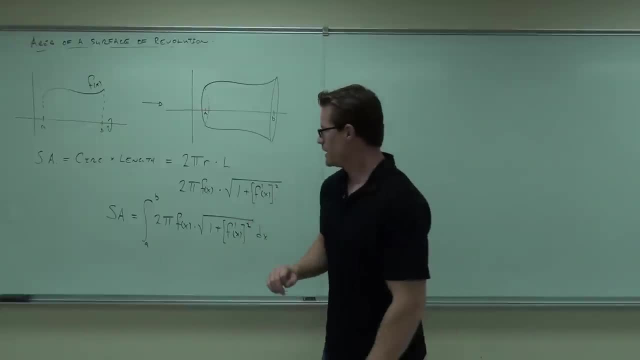 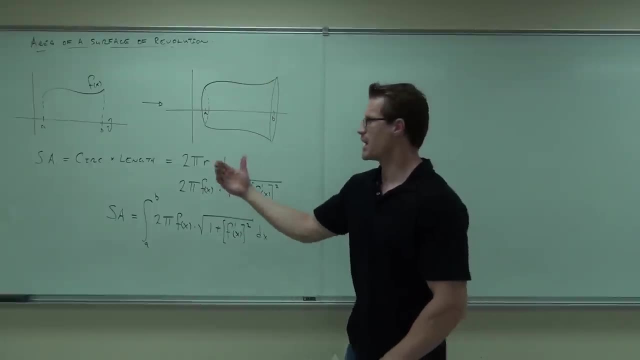 I hope that you can see where the formula is coming from. It is circumference area around- sorry, the distance around a circle. The distance around a circle. Distance around a circle Times the length How many little circles you have to add up. 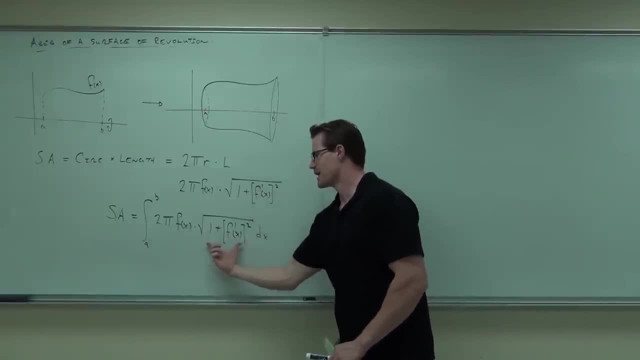 How many surface areas. So here we have circumference, We have length. We've already made this up. That's how we're going to find surface area. Now I'm about to give you a much more in depth explanation. So remember this formula. 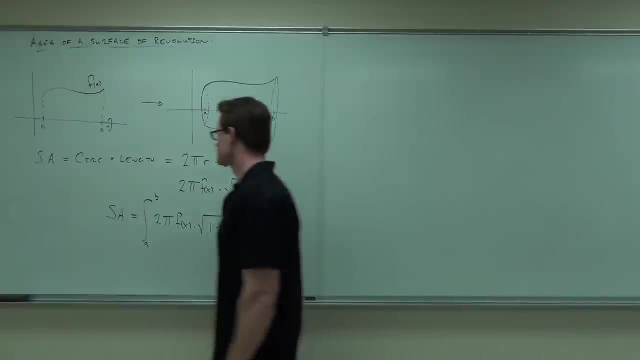 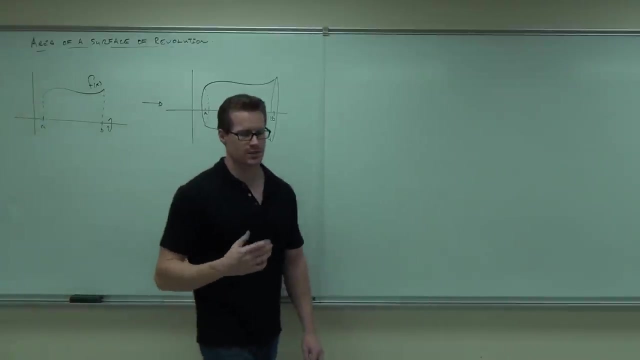 I'm going to give you the calculus behind it all. So here we go. As with anything involving our calculus, the idea is: can you make little cuts and make those cuts cut? Let's go very, very, very small and then add them all together with the limit. 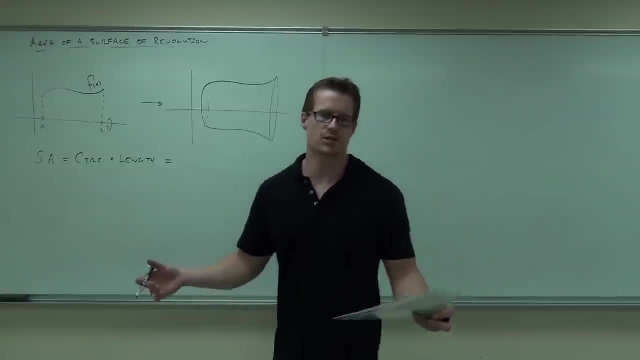 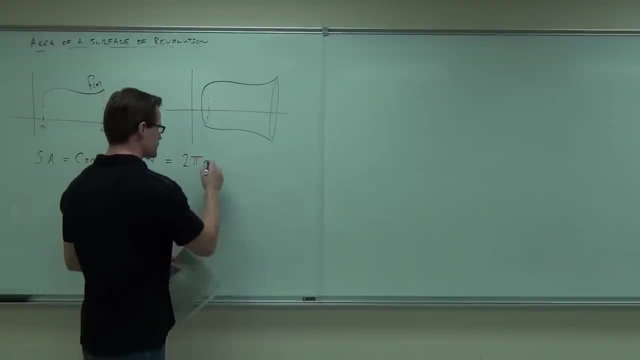 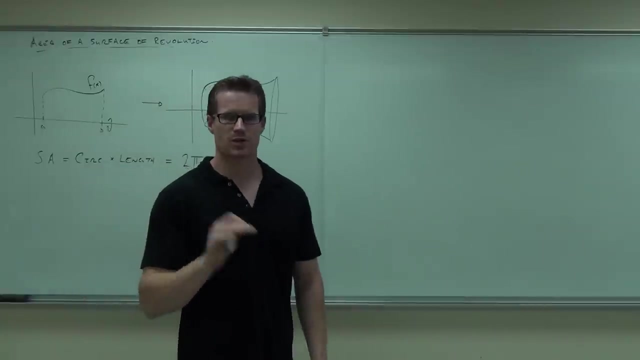 It's a circle. What's the circumference of a circle? And we know that as 2 Pi r, So we're going to get circumference times, length, 2 Pi r times, whatever the length happened happens to be. Now, if you think back and you watch previous videos, we know that we've 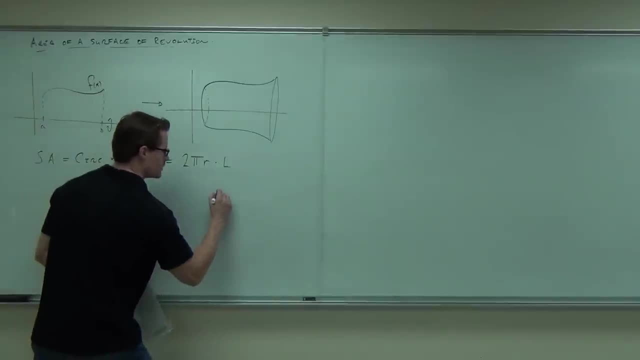 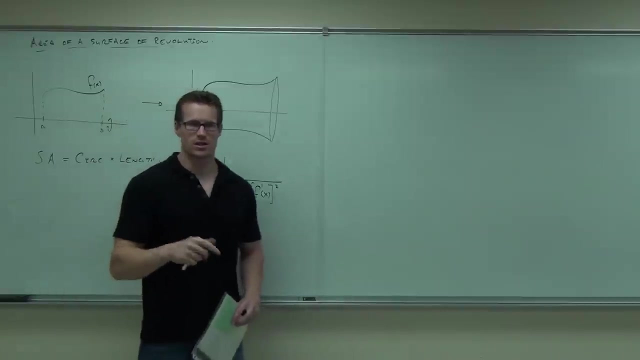 already done, length. We know that length is actually the square root of 1 f, prime of x, and we'll have a dx squared, sorry, and we'll have a dx at the very end, 2 pi r. think what the radius actually is. The radius is the distance from here to here at any given point. 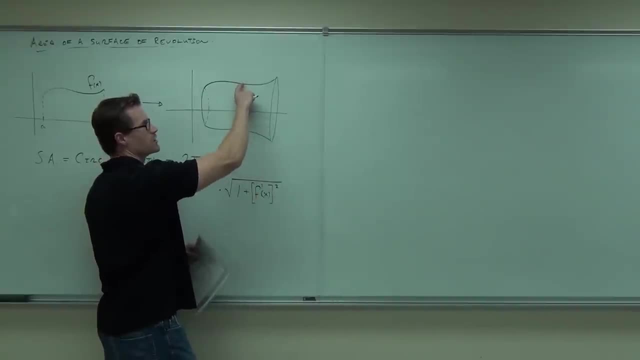 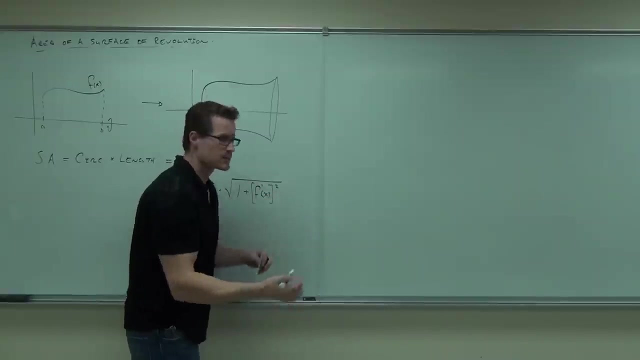 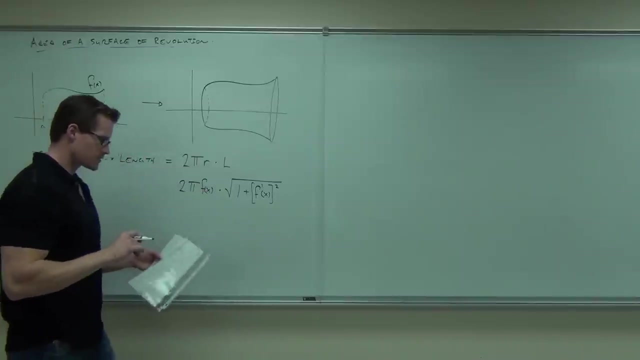 The distance from the x axis to the function is the function You plug in. whatever the x is, it's going to give you the height. So the radius in our case is simply f of x. So we have 2 pi f of x. What that means is that for us to find, and then we're going to integrate. 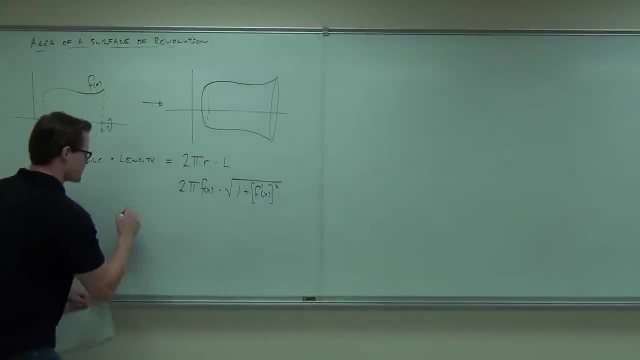 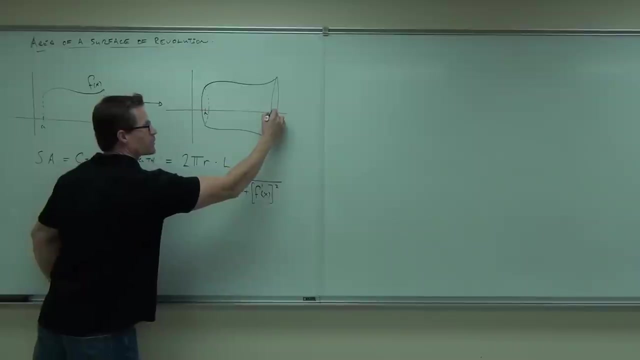 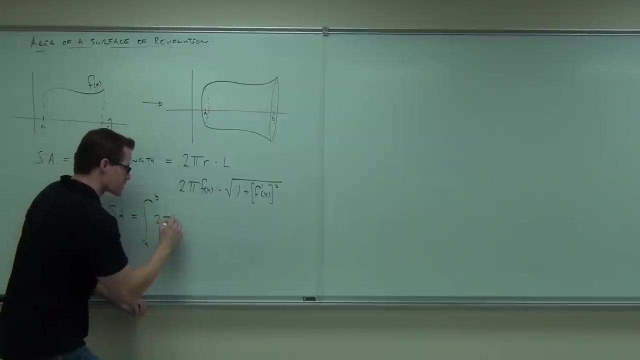 of course, at every single point. So for us to find the surface area, surface area is going to equal an integral from where we start to where we end. Stop of 2 pi. that's coming from the circumference f of x times 1 plus f, prime of x squared. 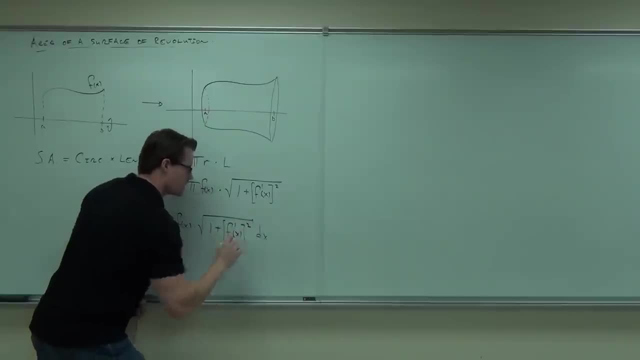 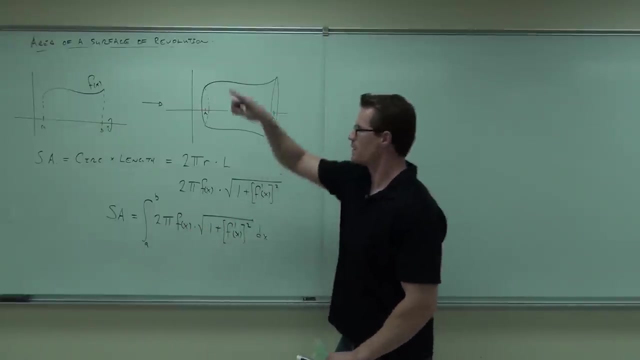 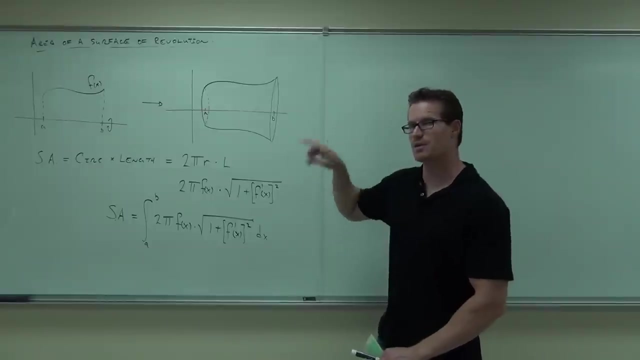 dx. I hope that you can see where the formula's coming from. It is circumference, area around- sorry, the distance around a circle. distance around a circle times the length, how many little circles you have to make, Add up How many surface areas. So here we have circumference, we have length, we've 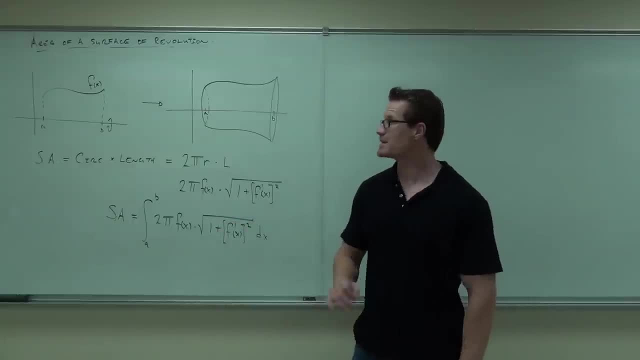 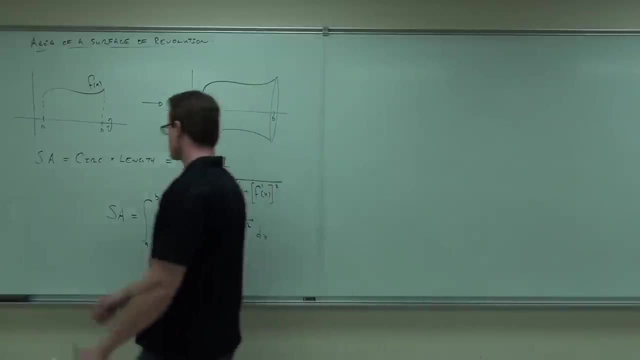 already made this up. That's how we're going to find surface area. Now I'm about to give you a much more in-depth explanation, So remember this formula. I'm going to give you the calculus behind it all. So here we go. 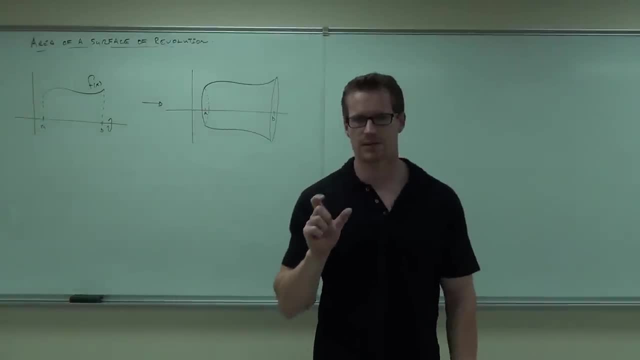 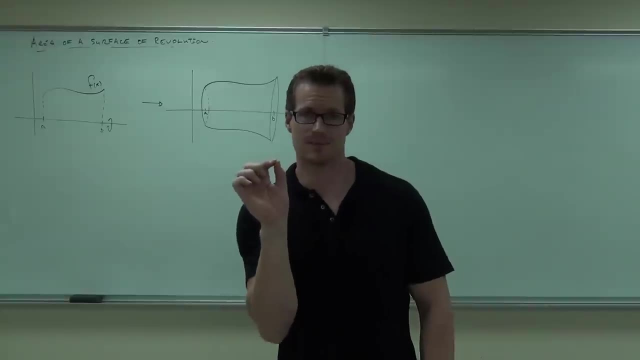 As with anything involving our calculus, the idea is, can you make little cuts and make those cuts go very, very, very small, and then add them all together with a limit? Oh sorry, add them all together with a sum. So now I'm going to take the limit of that sum, saying I'm not going to add, just a few. 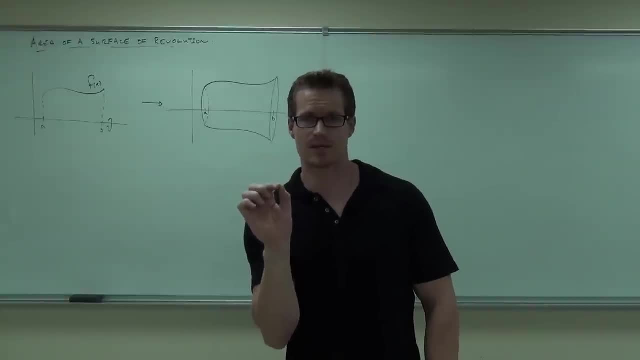 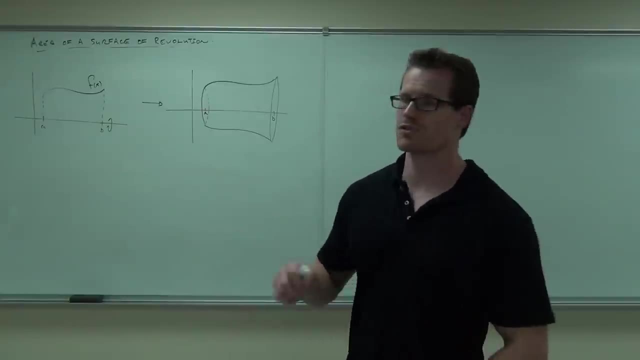 Oh sorry, Add them all together with the sum and take the limit of that sum, saying I'm not going to add just a few of them, I'm going to add an infinite number of them. So basically we start off just like we started the area problem. 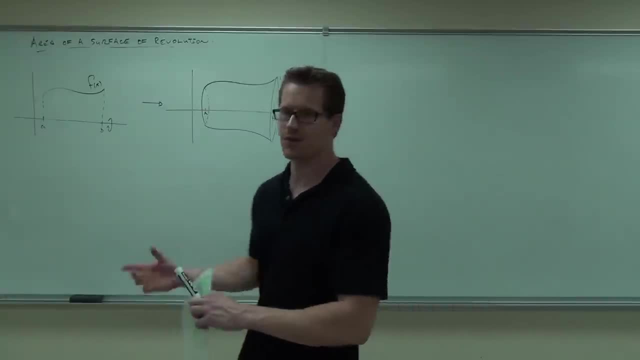 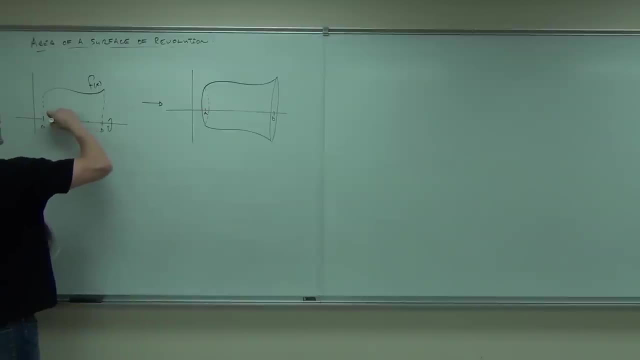 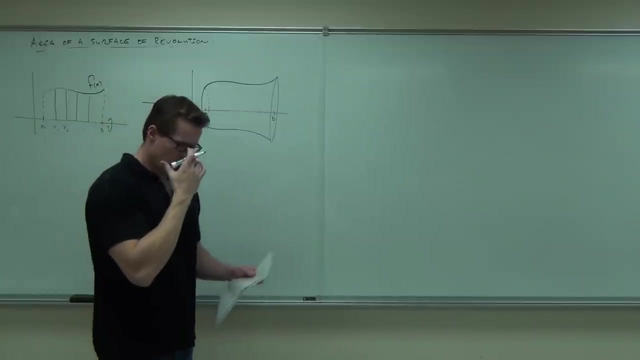 Just like we started the volume problem with discs and washers, Like anything else, we're going to make little cuts. Now we can call them x sub 1, x sub 2, and so on, and so on, and so on. Now, each of those cuts: how we found the length of it? how we found the length of the curve? 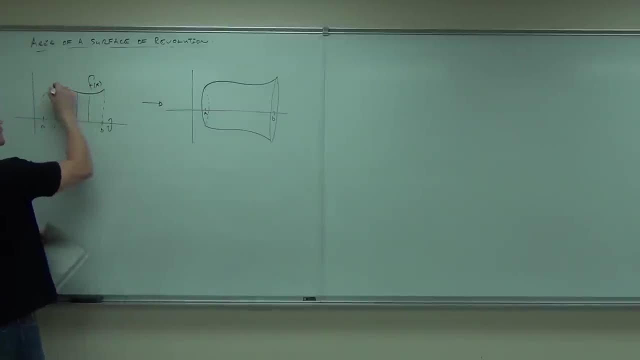 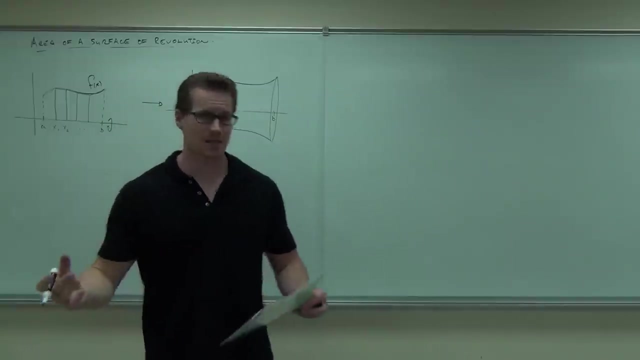 was that we took and we kind of truncated that curve, We cut it off and we found the length of each of these straight lines, because we know how to find the length of the line. What we didn't know how to find was the length of the curve. 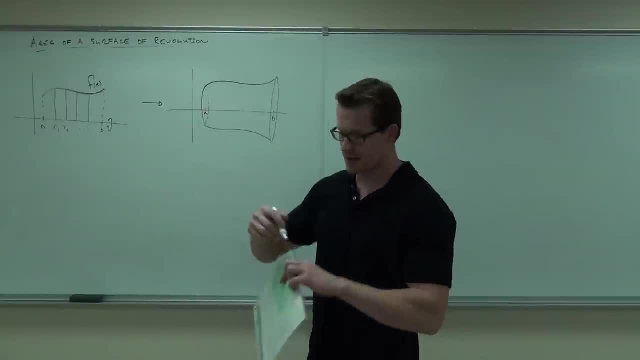 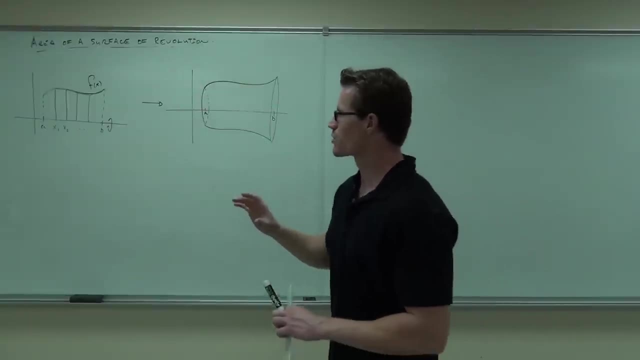 Now that we do. well, we can have that. Now notice, when I take the length of the line, the length of the line, and I revolve it around the x-axis like this: when I revolve that around, what it's going to create are: 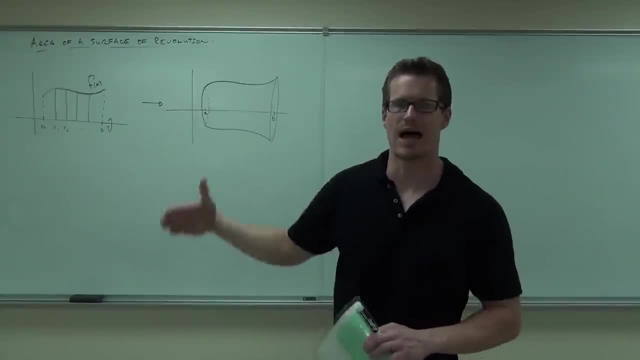 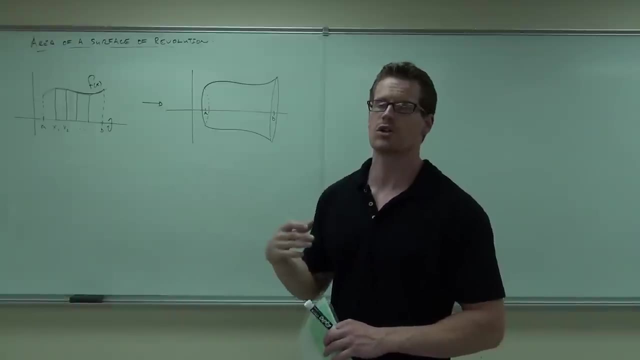 all these figures that have some surface area that's flat. We're going to have a flat surface area. Now we use the length of this line to approximate the length of the curve. What we're going to do now is find the surface area of it's called the frustum. it's the 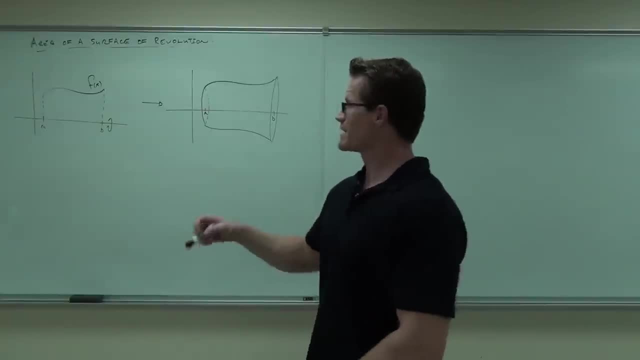 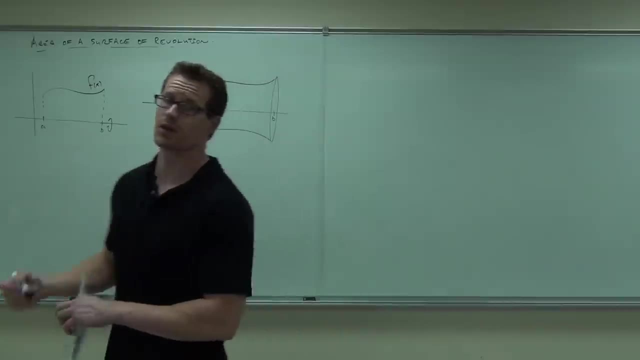 of them. I'm going to add an infinite number of them. So, basically, we start off just like we started the area problem, just like we started the volume problem with disk and washers. Like anything else, we're going to make little cuts. 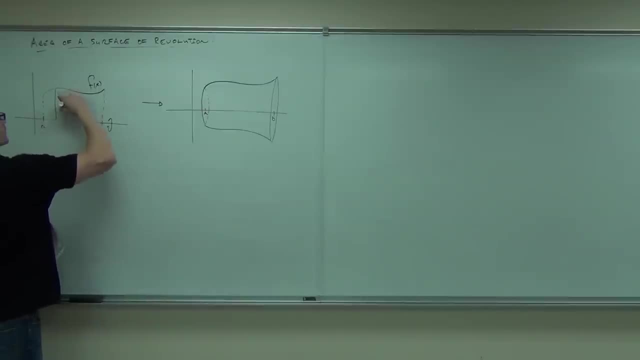 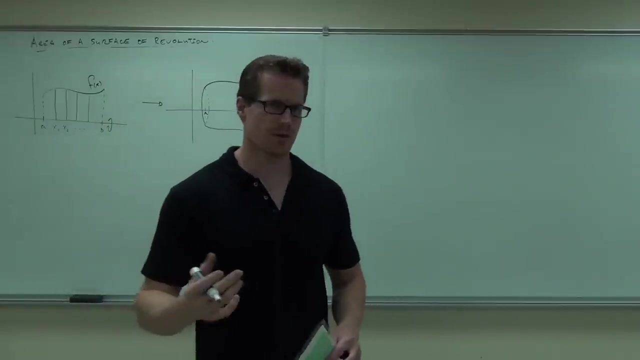 Now we can call them x sub 1, x sub 2, and so on, and so on, and so on. Now, each of those cuts, how we found the length of it, how we found the length of the curve was that we took and we kind of truncated that curve. 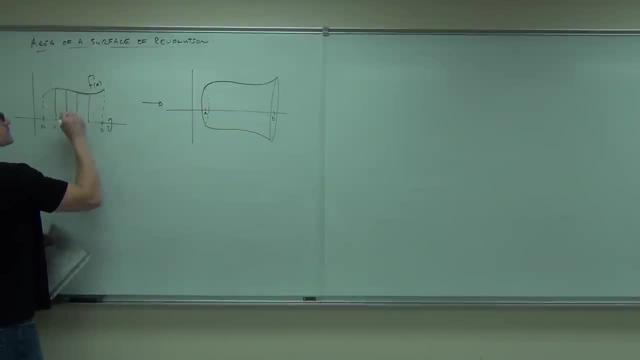 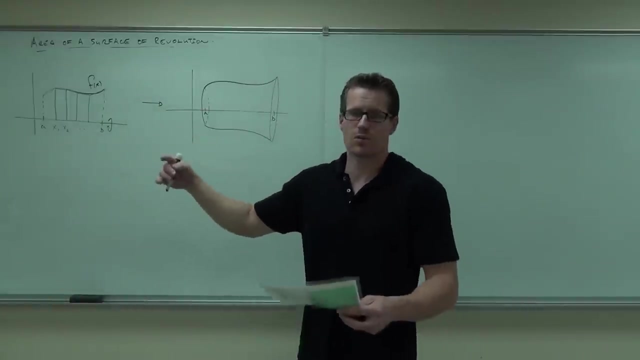 We cut it off and we found the length of each of these straight lines, because we know how to find the length of the line. what we didn't know how to find was the length of the curve. Now that we do, well, we can have that. 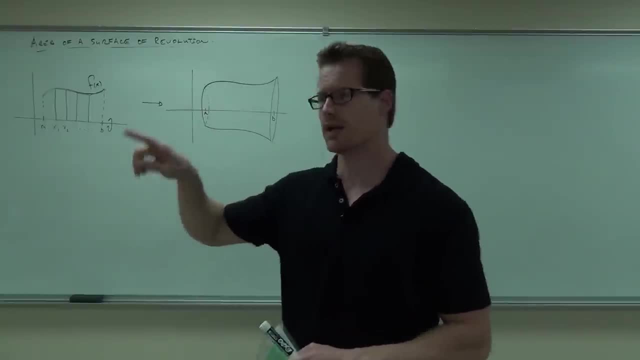 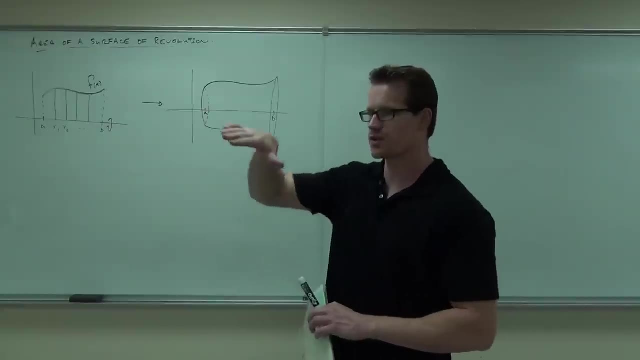 Now notice, when I take the length of the line, the length of the line, and I revolve it around the x-axis like this: when I revolve that around, what it's going to create are all these figures that have some surface area that's flat. 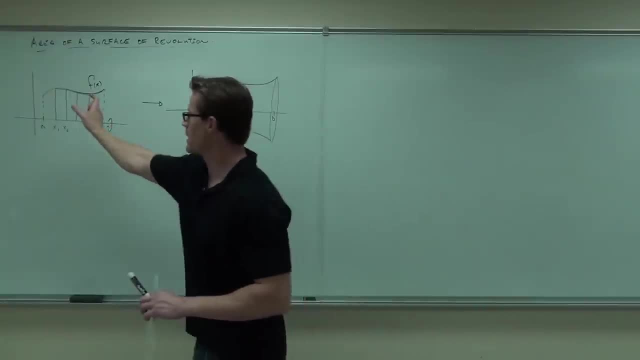 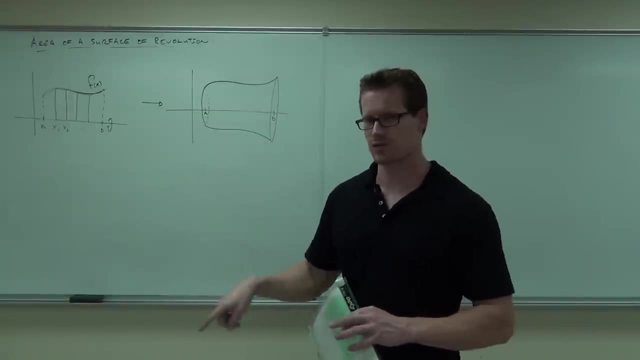 We're going to have a flat surface area. Now we use the length of this line to approximate the length of the curve. what we're going to do now is find the surface area of It's called a fresco, It's called a rostrum. 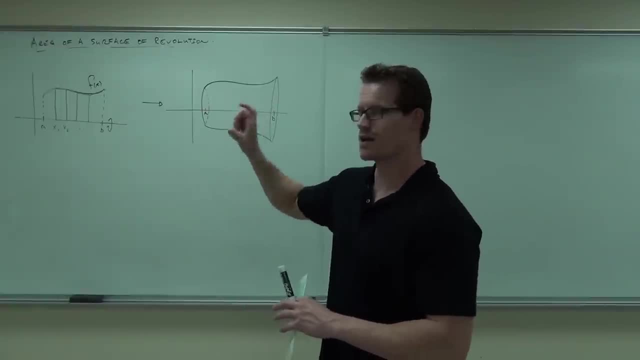 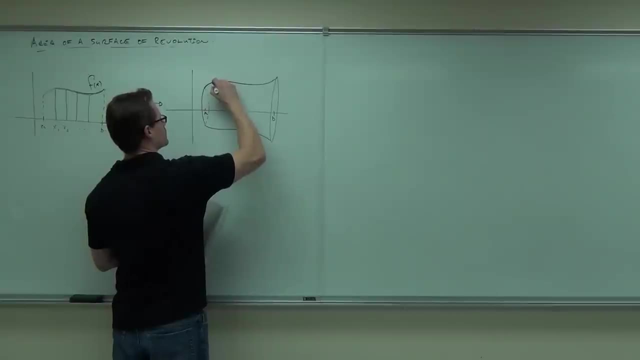 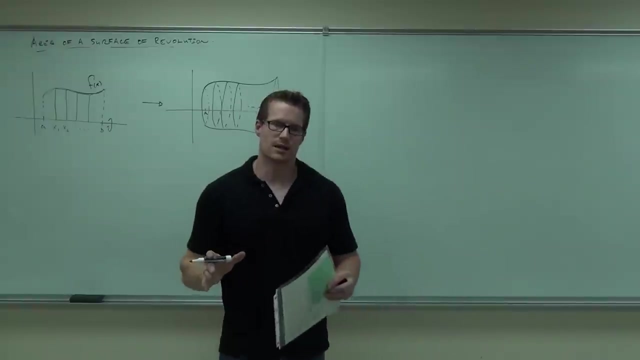 It's the surface area of the flat part, to approximate the surface area of the curved part. So all these cuts make all these cuts over here, And so on and so on, But that's not exactly it, You see, since we truncated these, 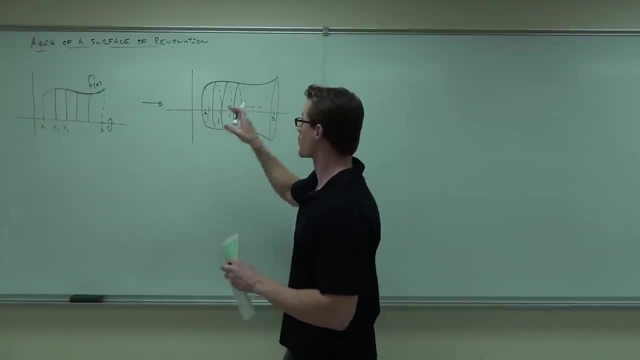 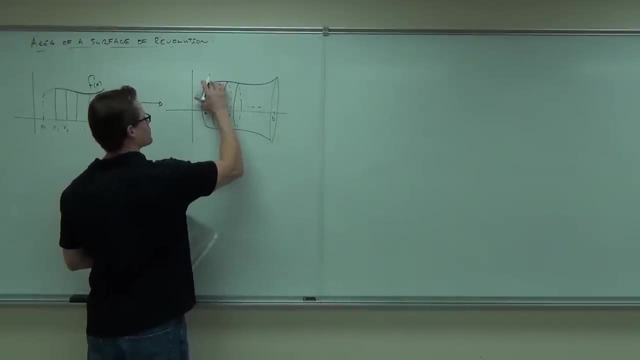 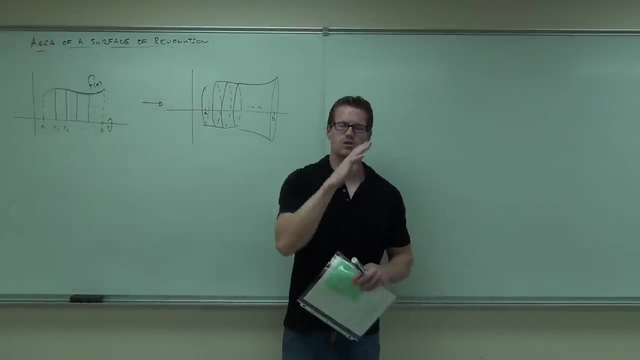 This line. we truncated that function at every single cutting. we're going to do the same thing here, And what we're going to end up with is this figure. That'll be straight, straight, straight. Same thing there. So we basically change a nice curve into a whole bunch of little pieces added together. 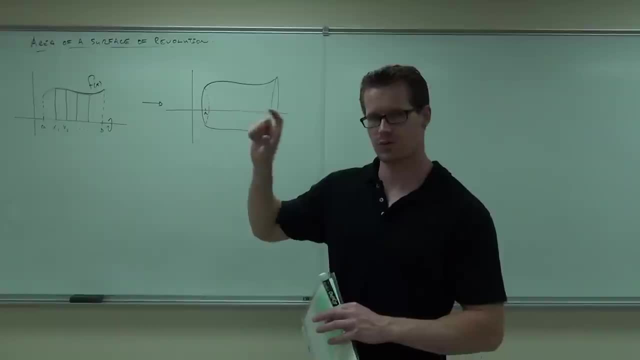 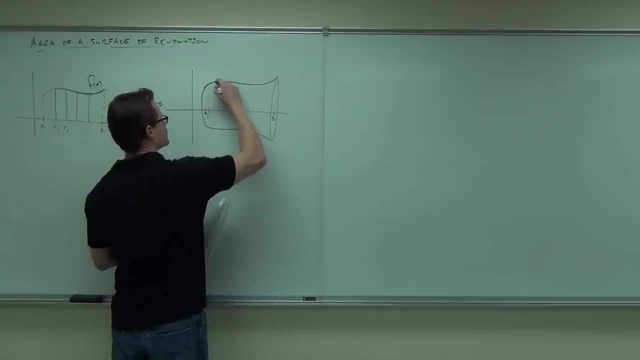 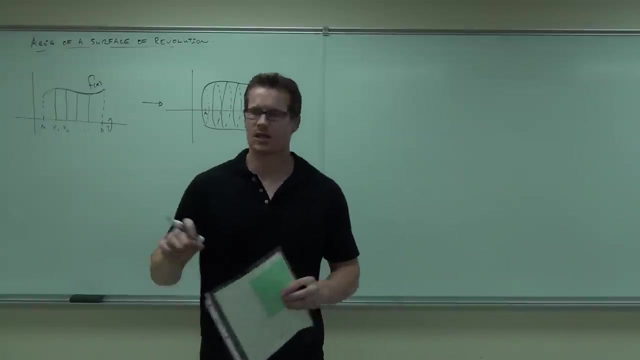 surface area of the flat part To approximate the surface area of the curve, The curved part. So all these cuts make all these cuts over here, And so on and so on, But that's not exactly it. You see, since we truncated these, this line, we truncated that function at every single. 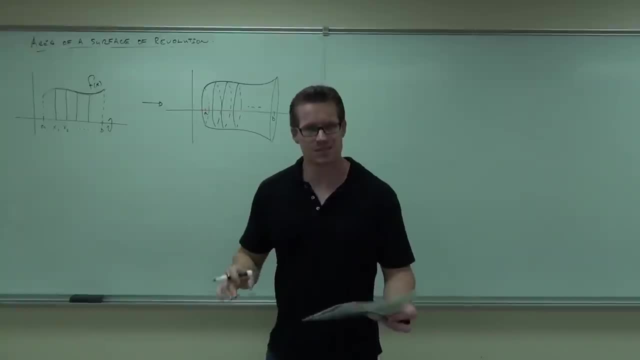 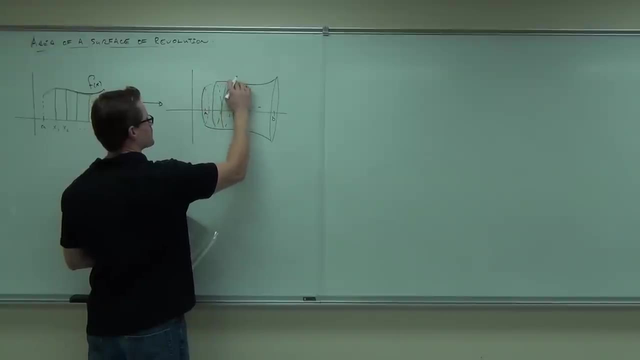 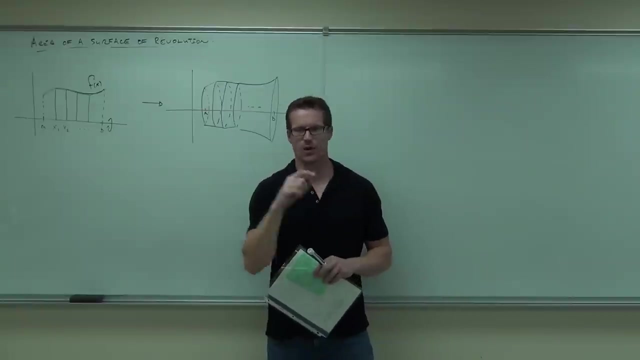 cutting. we're going to do the same thing here. What we're going to end up with is this, This figure, That'll be straight, Straight, Straight, Same thing there. So we basically change a nice curve into a whole bunch of little pieces added together. 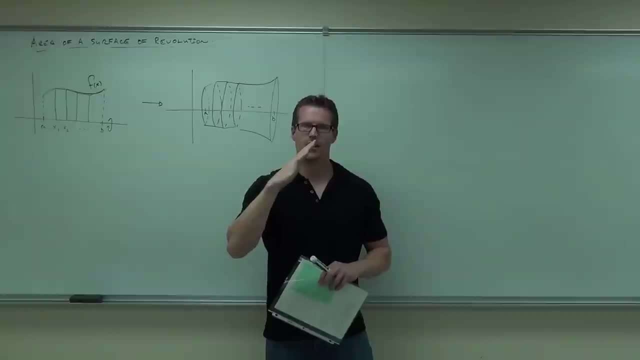 all these frustums added together They're flat-sided, almost like from the side of them kind of look like a trapezoid, almost This perpendicular, perpendicular, and then these angles going up. Now we're going to take a look at one of these frustrums. 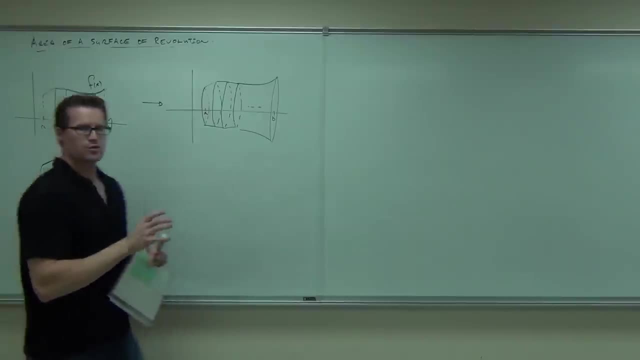 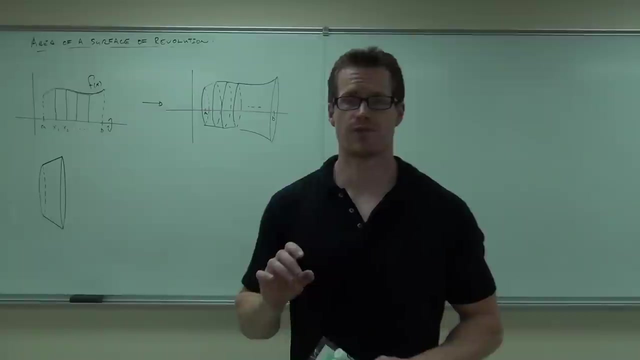 So notice what I've done. I've just taken one of these things, I've pulled it off to the side. Here's our goal. Our goal is to find the surface area of that piece, of this piece, and then add all of. 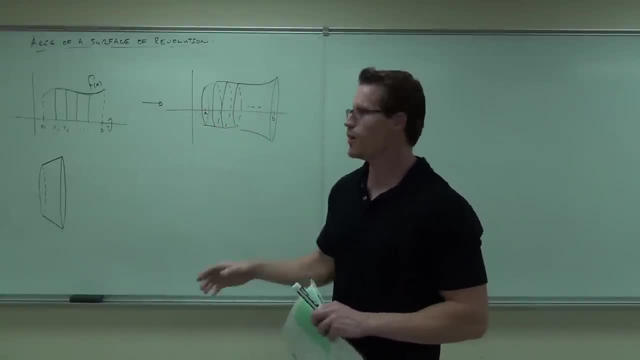 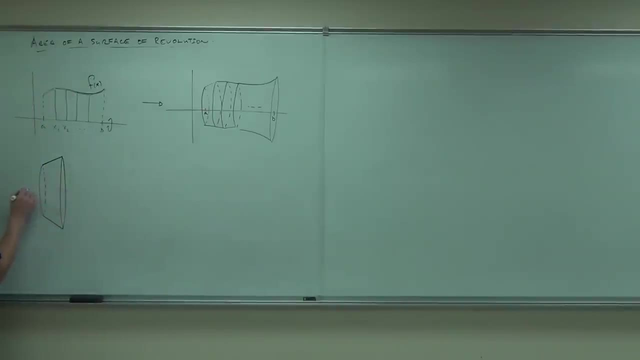 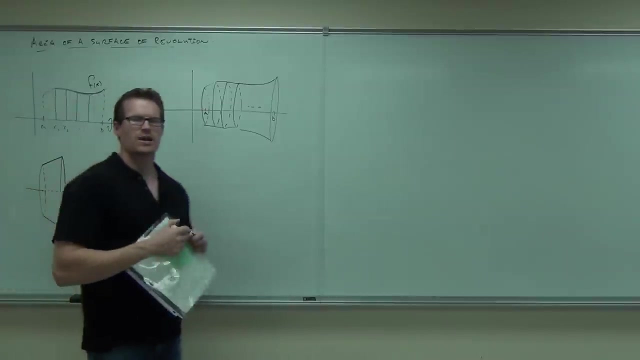 the little frustrums together, all the little pieces together. Well, let's think about that for just a second. First thing: If that's our x-axis, where does our cut start and where does our cut stop? Now, we have to be very general in this. 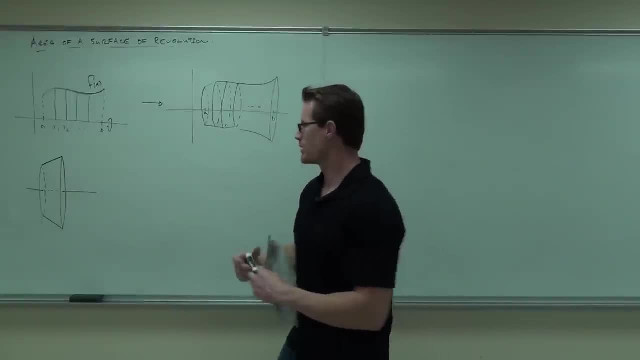 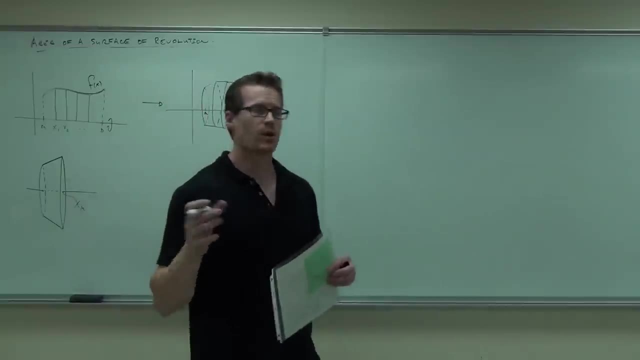 I can't call it a. I can't call it x sub 1, x sub 2.. I need to call it x sub k, and if I do that, what's the one right before x sub k? Well, it's just the previous one, so x sub k minus 1.. 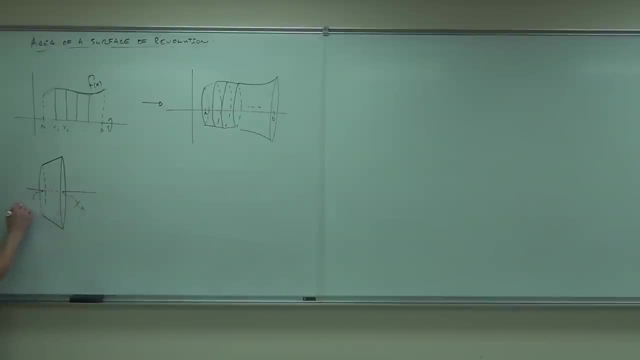 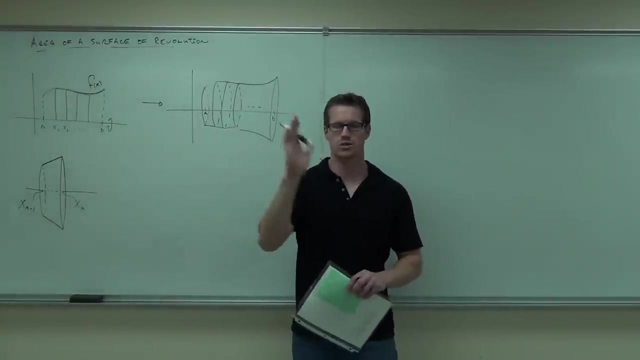 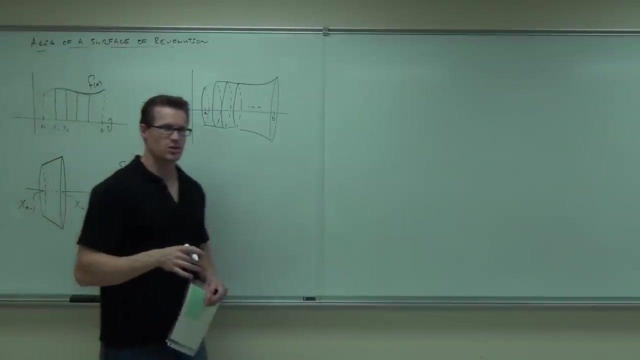 So we now know where the frustrum's going to start and where it's going to stop, where the surface area is going to start and where it's going to stop. Now, in order to find the surface area, I have to just give it to you. but if you look, 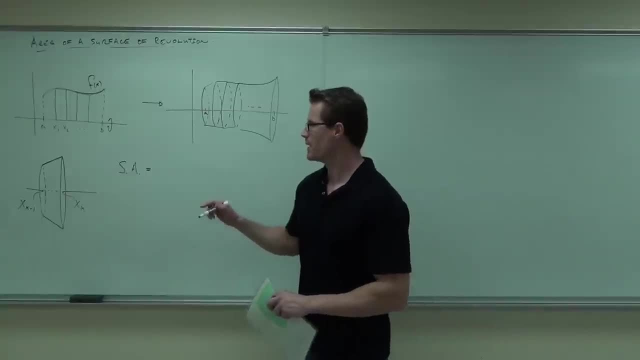 it up in kind of an advanced geometry book. you're going to find out that this is true. If I find the surface area, I'm going to find the x sub 1.. I'm going to find the x sub 2.. If I find the surface area of a frustrum, that's just the outside region. 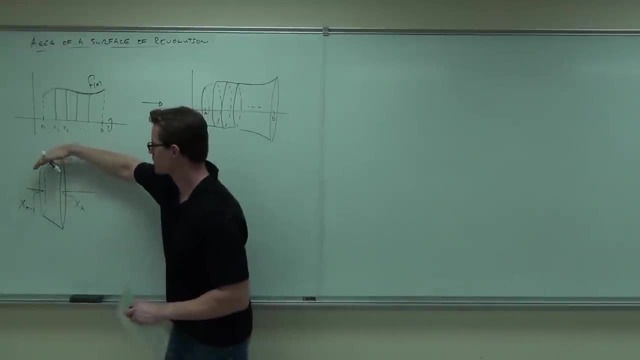 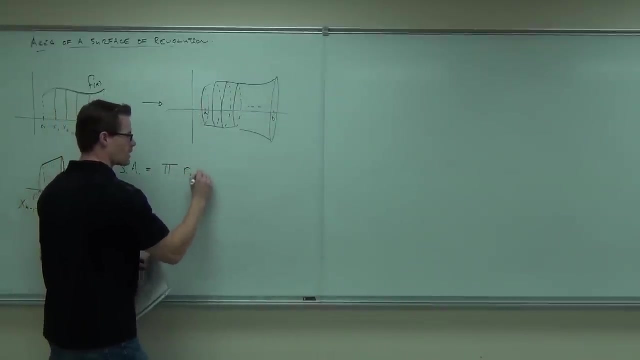 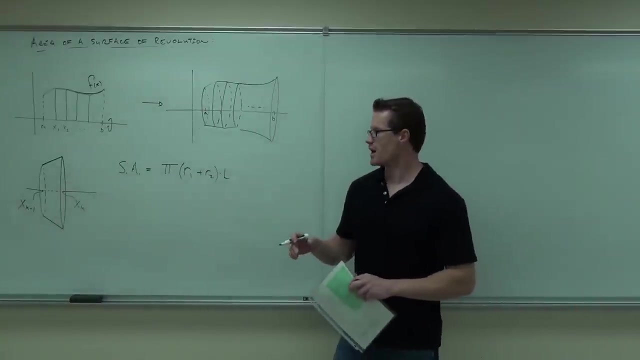 If I find the surface area of that outside region, that means this angled part that's coming out at you. What it is is pi r1 plus r2 times the length. That's the formula for surface area. Now, of course, I'm doing this for each and every frustrum. 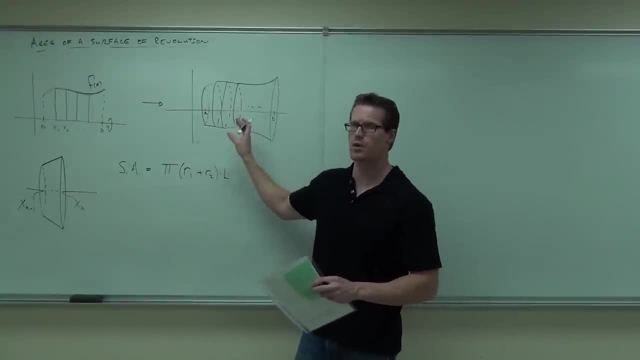 Each and every one of these little frustrums, Each and every one of these pieces. So I'm going to say not just surface area in general, surface area for the kth 1.. Pi is a constant That doesn't change. 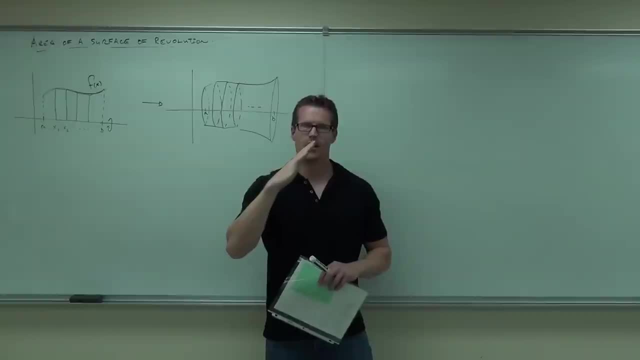 all these frustrums added together, They're flat, They're flat-sided, almost like from the side of them kind of look like a trapezoid, almost. You have this perpendicular, perpendicular and then these angles going up. Now we're going to take a look at one of these frustrums. 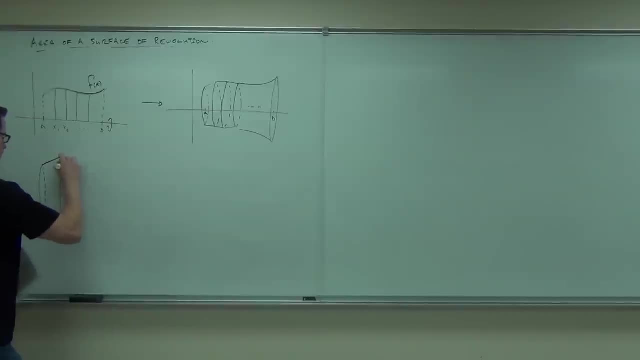 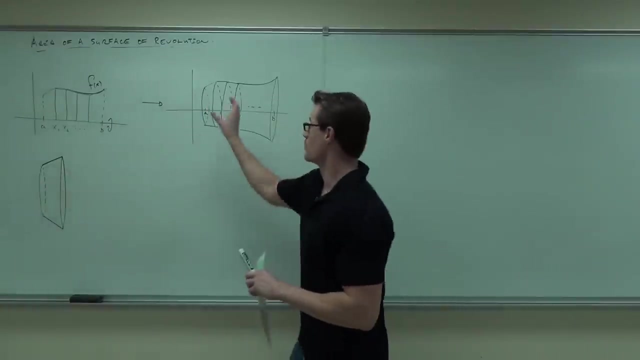 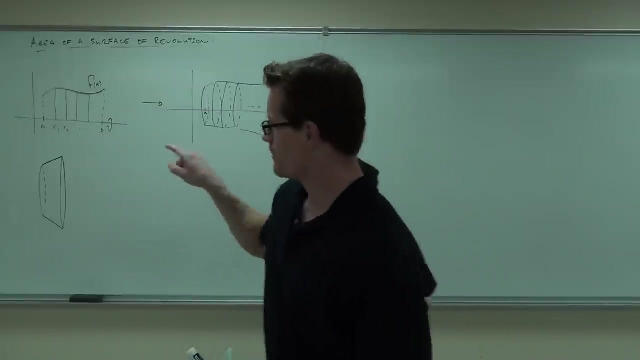 So notice what I've done. I've just taken one of these things, I've pulled it off to the side. Here's our goal. Our goal is to find the surface area of that piece, of this piece, and then add all of. 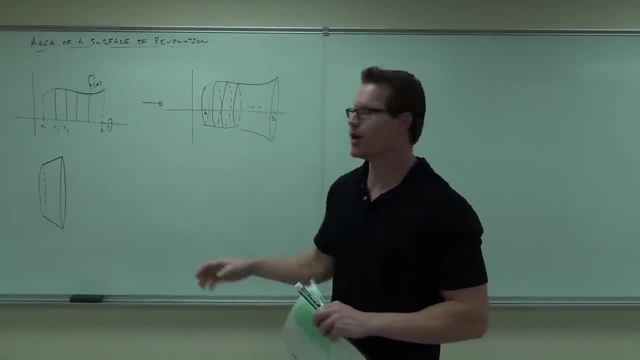 the little frustrums together, all the little pieces together. Well, let's think about that for just a second. First of all, we're going to do this. First of all, we're going to do this. First of all, we're going to do this. 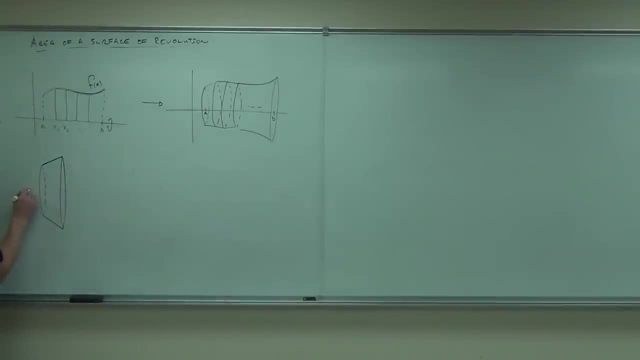 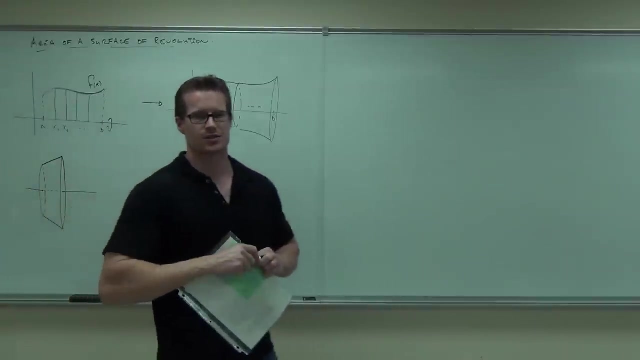 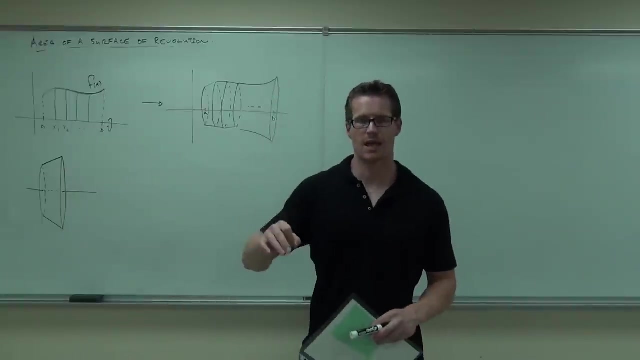 Firstly, if that's our x-axis, where does our cut start and where does our cut stop? Now we have to be very general in this. I can't call it a, I can't call it x sub 1, x sub 2.. 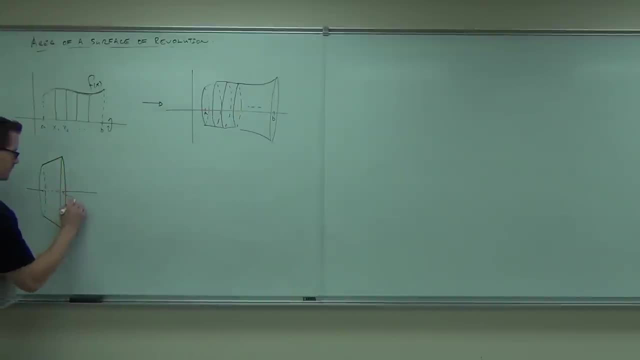 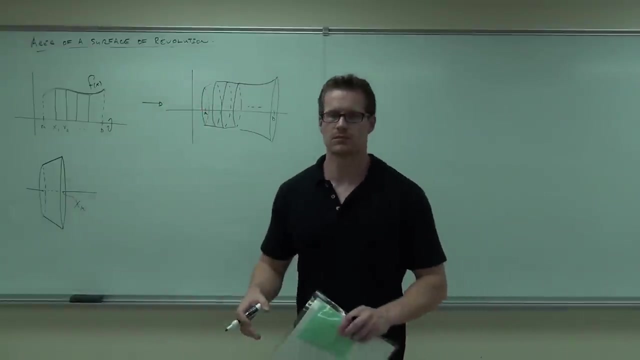 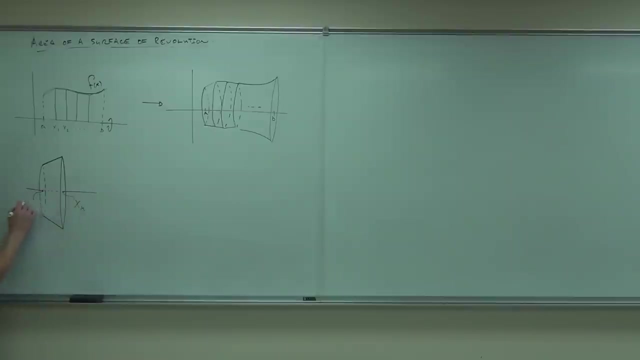 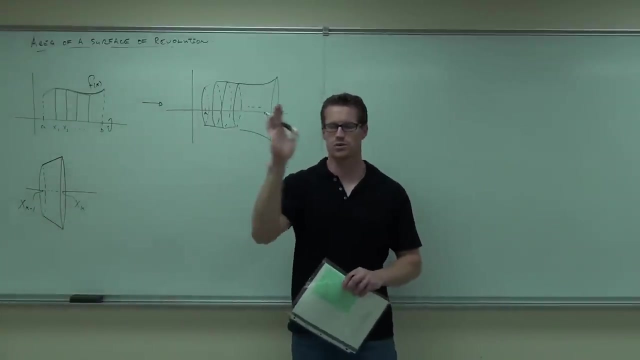 I need to call it x sub k, and if I do that, what's the one right before x sub k? Well, it's just the previous one, so x sub k minus 1.. So we now know where the frustrum's going to start and where it's going to stop where. 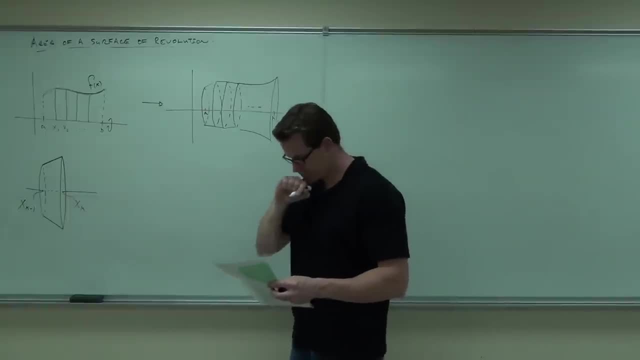 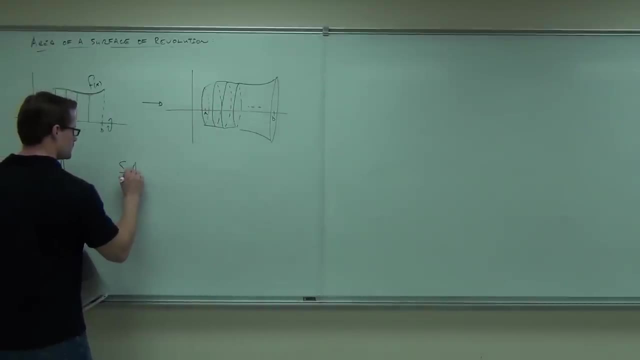 the surface area is going to start and where it's going to stop. Now, in order to find the surface area, I have to just give it to you, but if you look it up in kind of an advanced geometry, you're going to be able to find it. 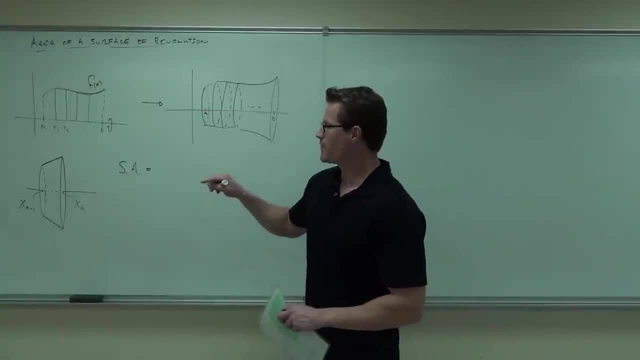 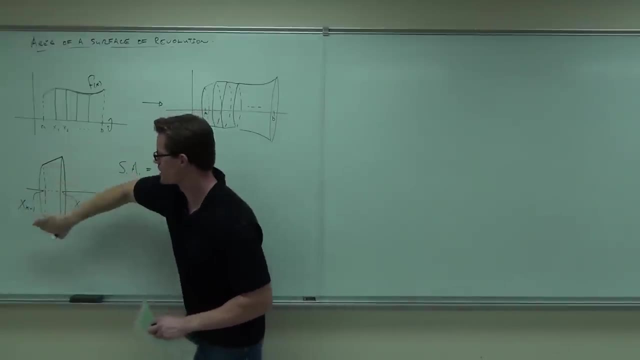 Okay, If you look at the geometry book, you're going to find out that this is true. If I find the surface area of a frustrum, that's just the outside region. if I find the surface area of that outside region, that means this angled part that's coming out at you. what? 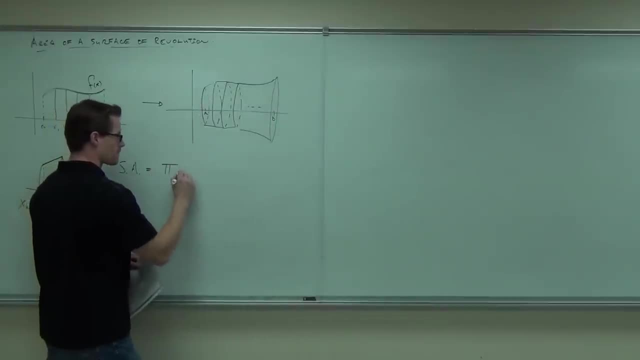 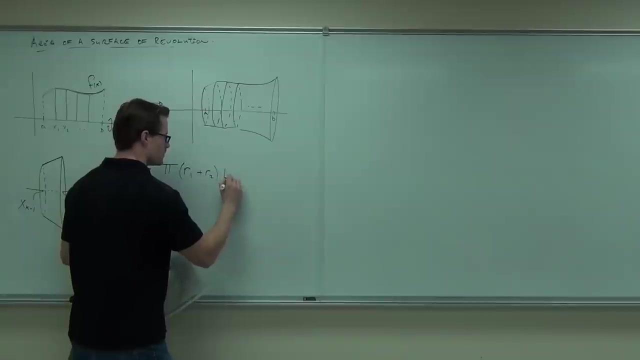 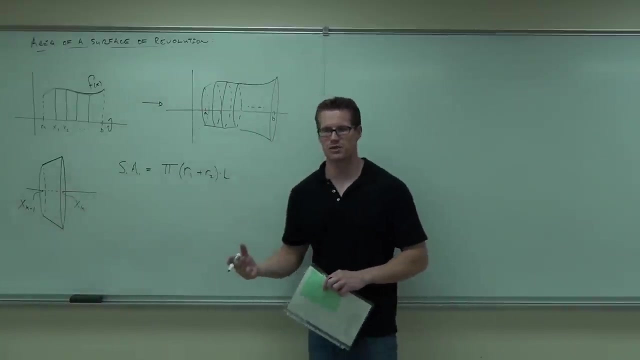 it is is pi r1 plus r2 times the length. That's the formula for surface area. Now, of course, I'm doing this for each and every one of these little frustrums, each and every one of these pieces. So I'm going to say not just surface area in general, surface area for the kth one. 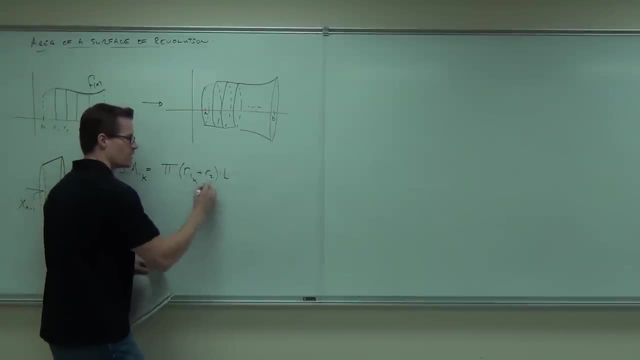 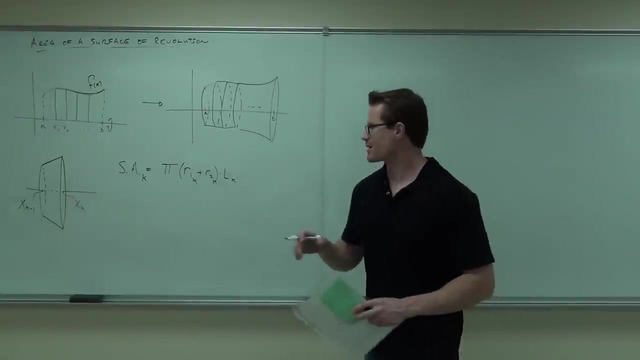 Pi is a constant that doesn't change, but the radius for the kth one, the other radius for the kth one and the length at the kth. frustrum. Now let's talk and try to figure out, if we can figure out, what r sub 1 k is and what. 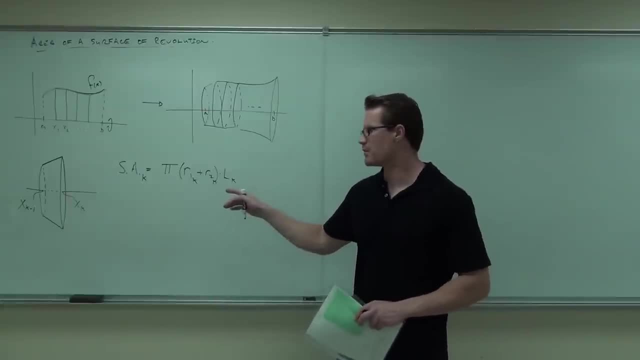 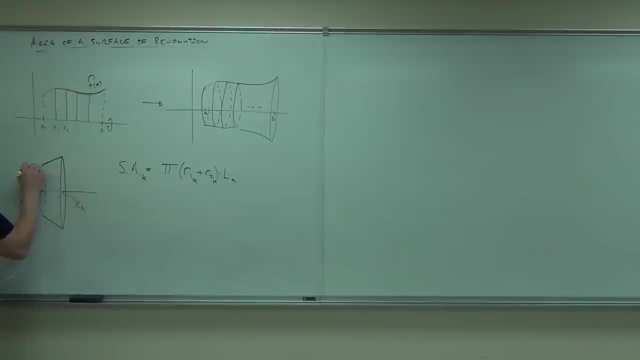 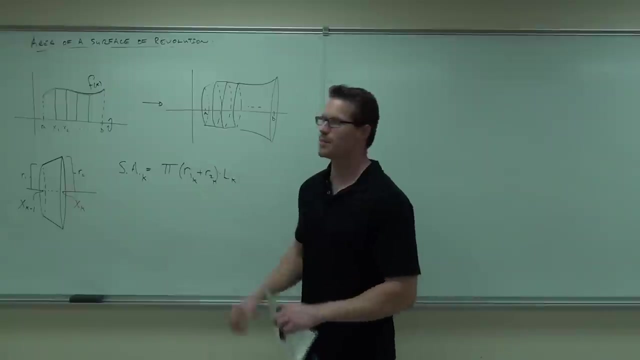 r sub 2 k is l sub k. we already have that one, but we're going to worry about these two things. So if I call this r1, and I call this r2,, can you tell me how much r1 is? 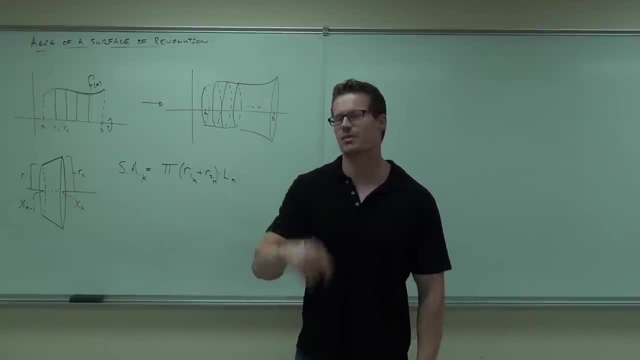 I know you can't because you're on the video, but just think about it for a second. 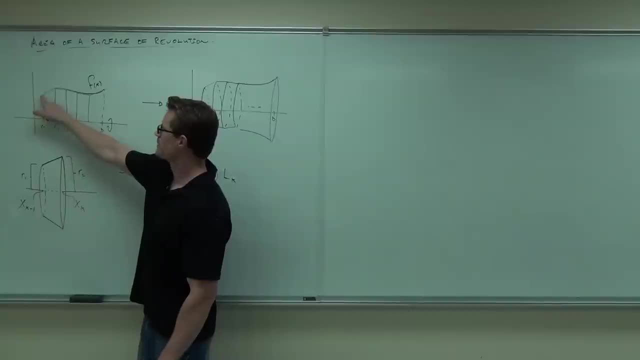 r1, think about what we're doing. We're taking and we're cutting from here to here on the function Notice it's a secant line. So the height at this point is the function height. The height at this point is also the function height. 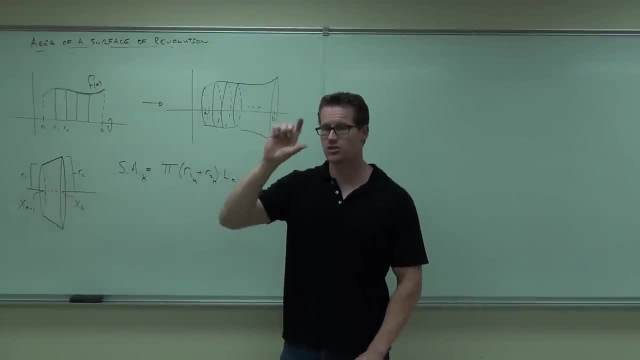 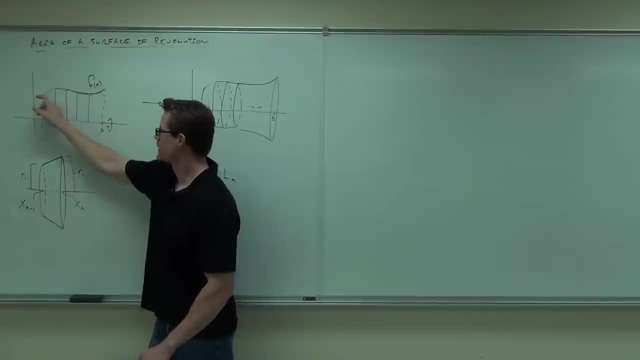 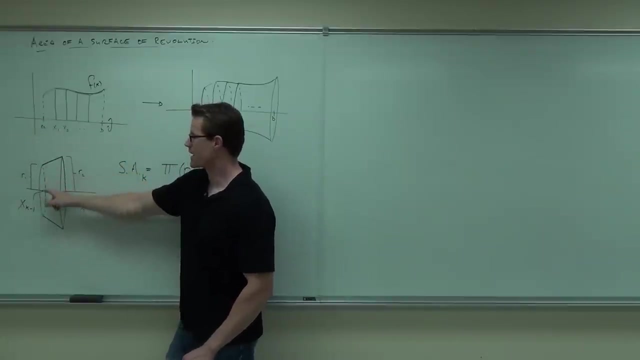 So r1 is actually the function's height at whatever this point is. I'll repeat that The distance from here to here is r1.. The distance from here to here is whatever the function height is at my x coordinate. In this case, my x coordinate is x sub k minus 1.. 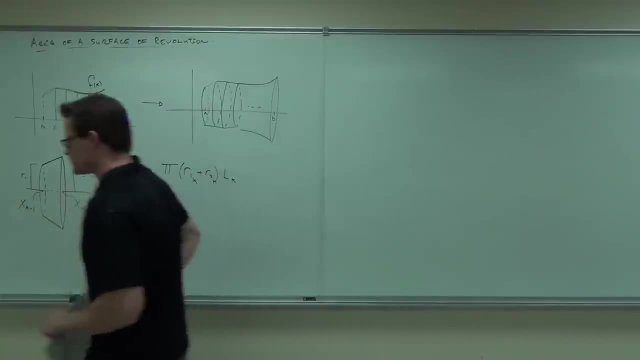 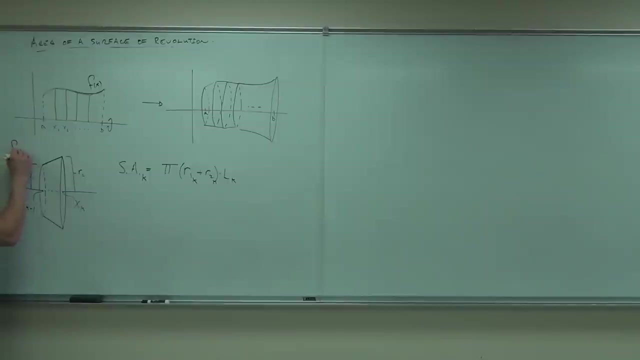 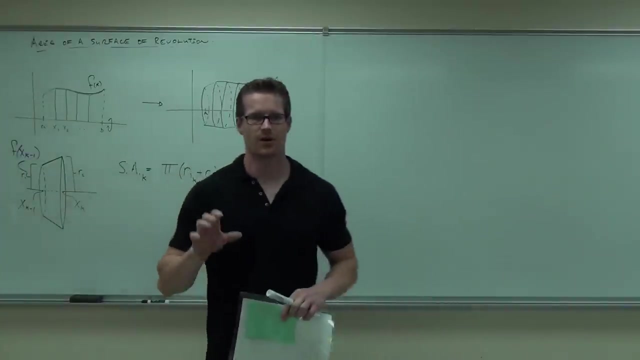 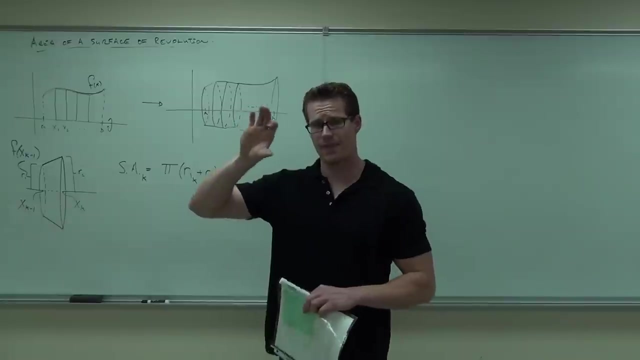 What that means is that my radius is actually f of x sub k minus 1.. You plug in x sub k minus 1 into f. You get the height at that point. That's your radius. How about the height here from here to here? 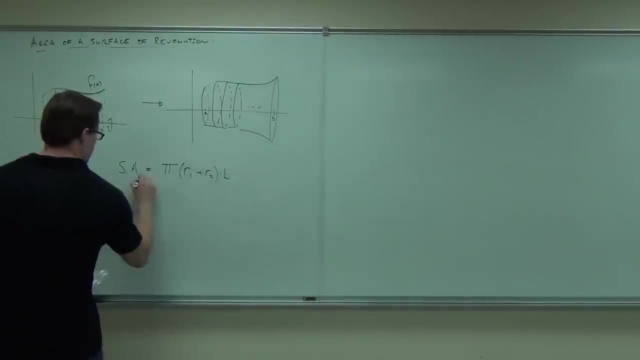 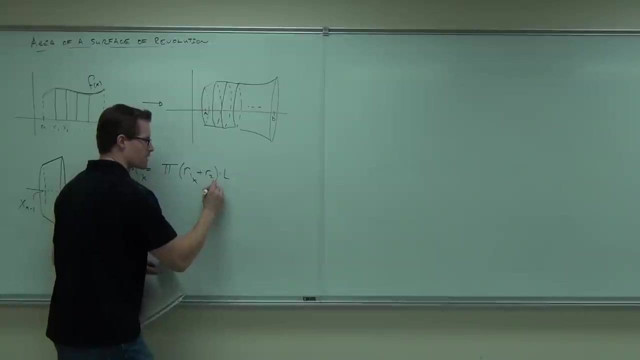 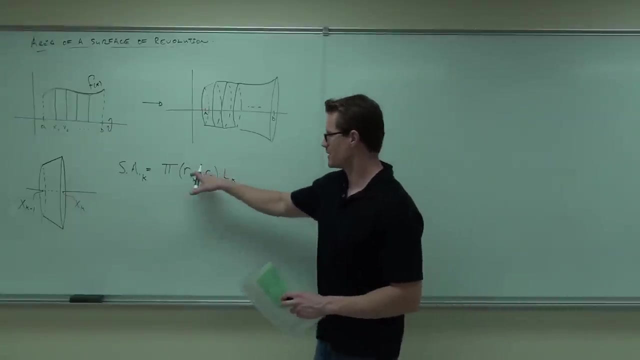 But the radius for the kth 1.. The other radius for the kth 1. And the length at the kth? frustrum. Now let's talk and try to figure out. if we can figure out, what r sub 1 k is and what 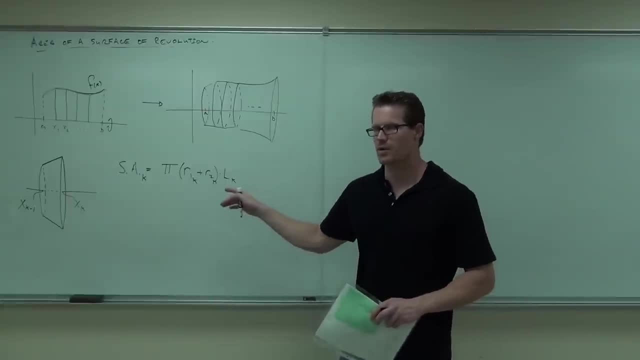 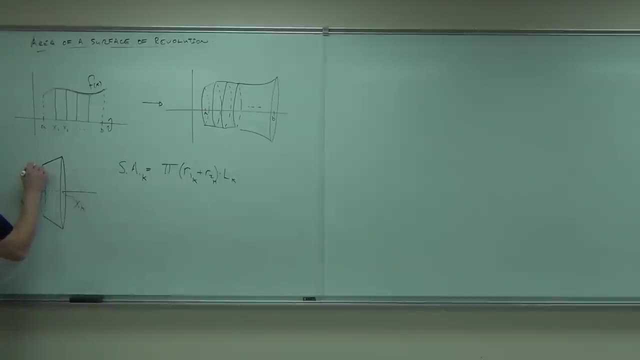 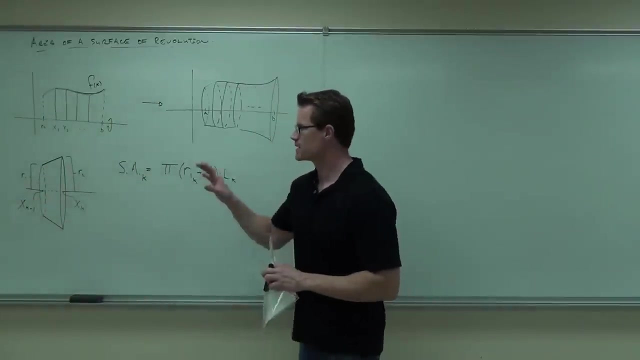 r sub 2 k is L sub k. we already have that one, But we're going to worry about this one. We're going to worry about this one, But we're going to worry about these two things. So if I call this r1, and I call this r2,, can you tell me how much r1 is? 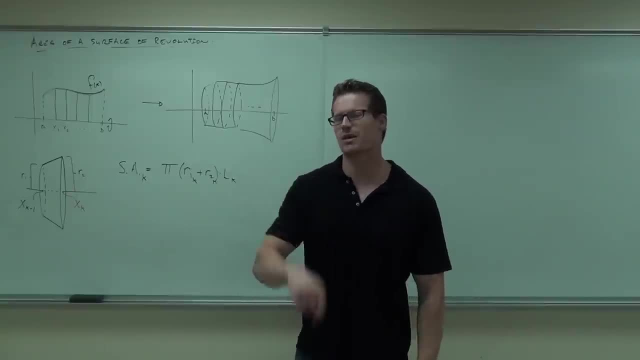 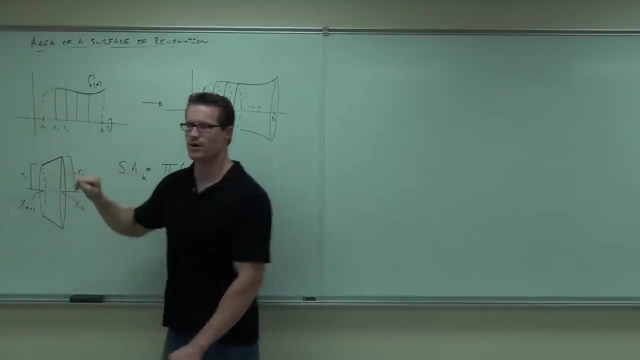 I know you can't because you're on the video, But just think about it for a second. If I'm trying to find r1, think about what we're doing, We're taking and we're cutting from here to here on the function. 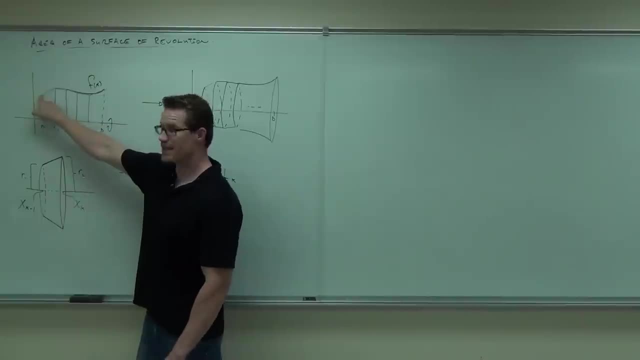 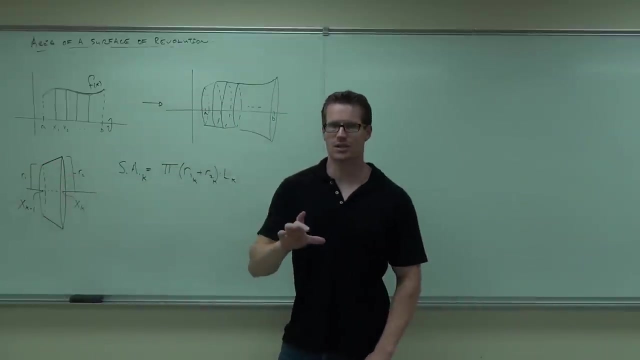 Notice it's a secant line. So the height at this point is the function height. The height at this point is also the function height, So r1 is actually the function's height. at whatever this point is, I'll repeat that. 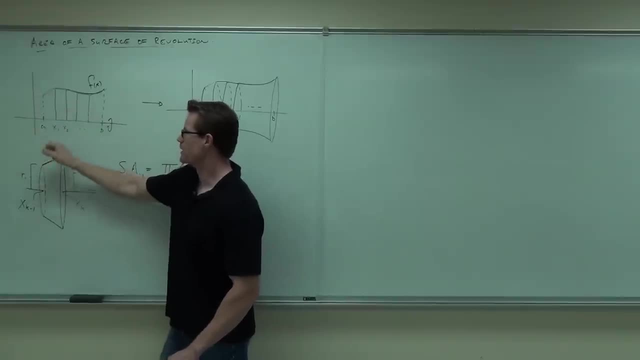 The distance from here to here is r1.. The distance from here to here is whatever the function height is at my x coordinate. In this case, my x coordinate is r1.. So I'm going to call this r1.. My r1 is x sub k minus 1.. 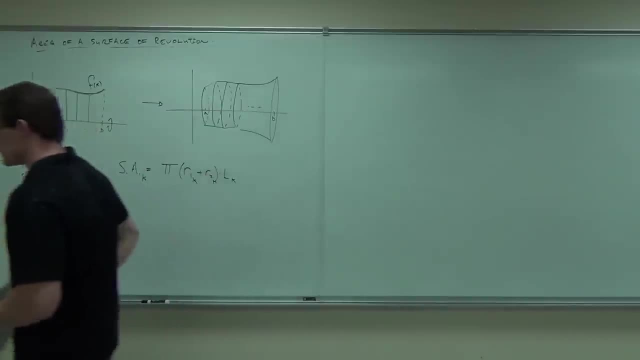 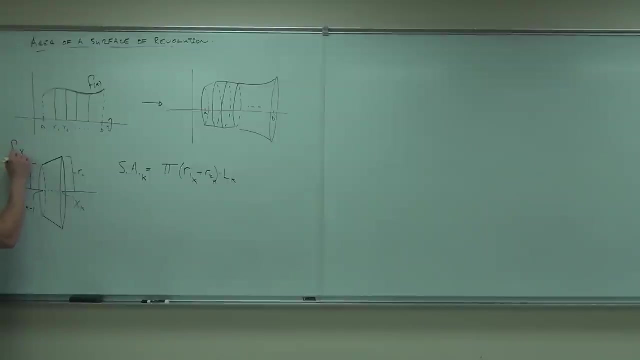 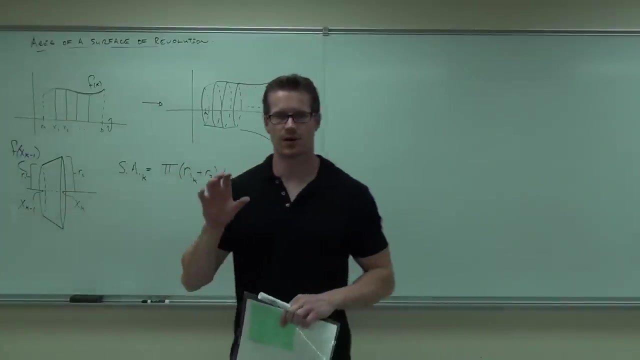 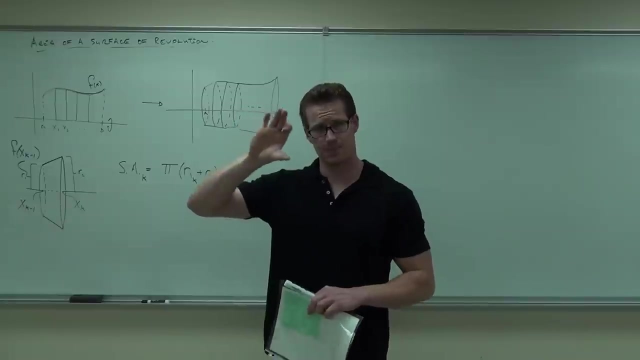 What that means is that my radius is actually f of x sub k minus 1.. You plug in x sub k minus 1 into f. you get the height at that point. That's your radius. How about the height here from here to here? 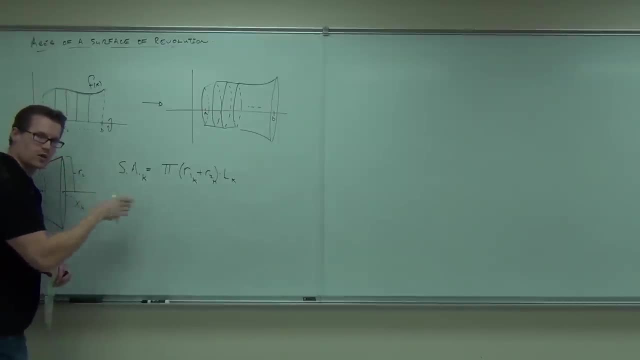 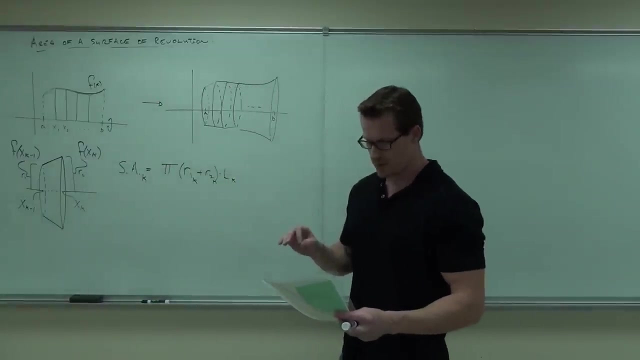 Well look, That's just the height of the function. That's the height of the function at whatever x coordinate I'm plugging in. In this case it's x sub k. So r2 is f of x sub k. 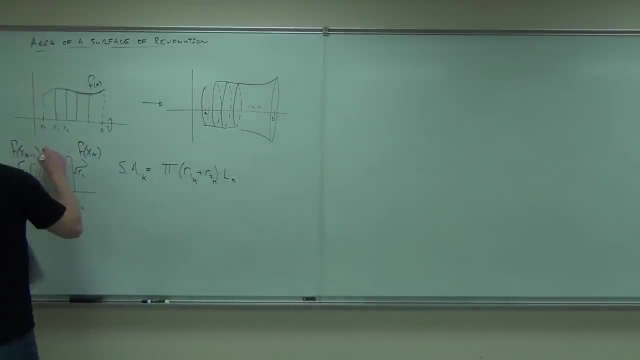 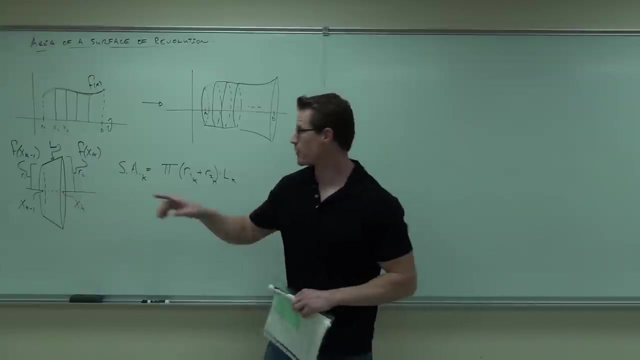 Now, how about l? What we call l is the diagonal distance of our frustum, how far it is from here to here. Now, fortunately for us, we've already found out how to find the length of the curve. We know that l was this. 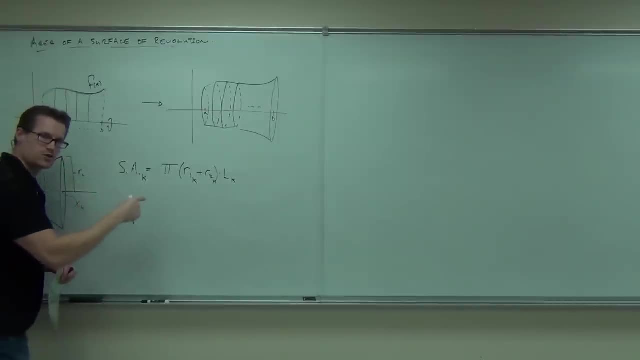 Well look, That's just the height of the function. That's the height of the function of whatever x coordinate I'm plugging in. In this case it's x sub k. So R2 is f of x sub k. 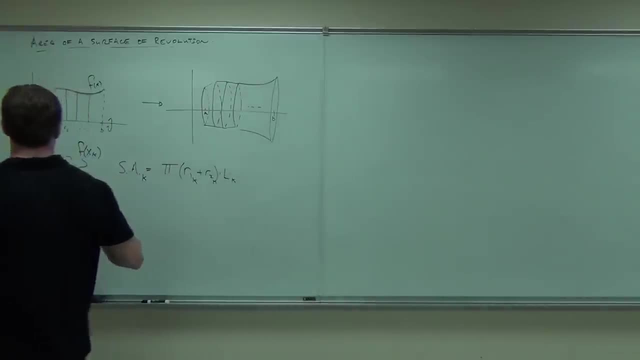 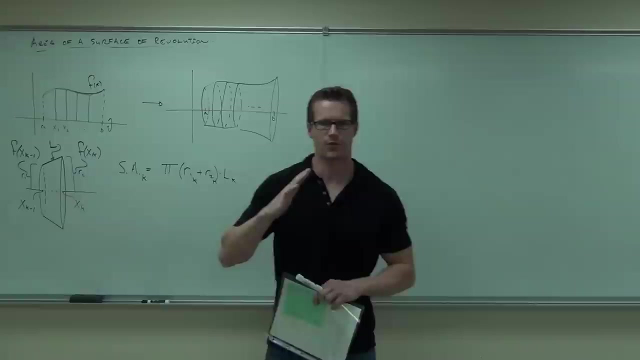 Oh, now how about L? What we call L is the diagonal distance of our frustum, how far it is from here to here. Now, fortunately for us, we've already found out how to find the length of the curve. We know that L was this. 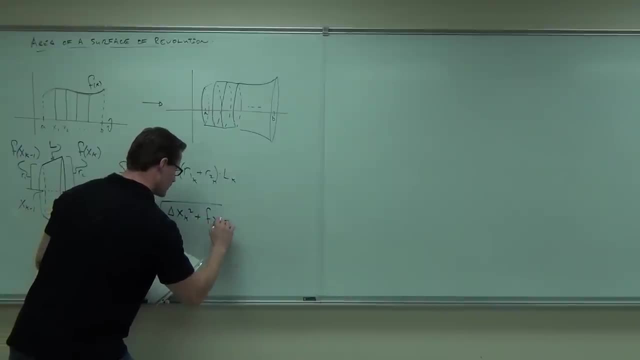 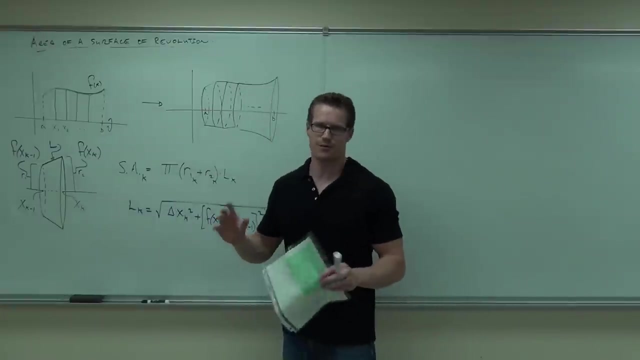 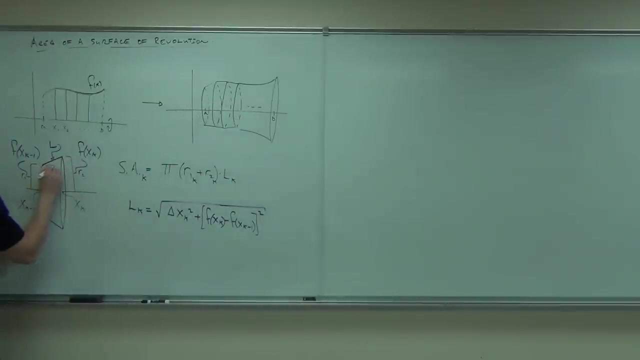 L was this, L was that, And you can get that simply by Pythagorean theorem if you were to think about it. The change in height here, from here to here, remember, if you draw a little triangle, The change in height is simply f of x sub k. 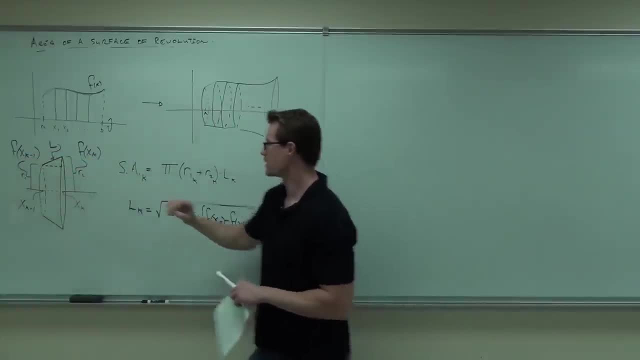 It's just the length of the curve. All right, That's it: k minus f of x sub k minus 1.. So we have this, and then you square it. Pythagorean theorem: square it, Square the height, square the length. 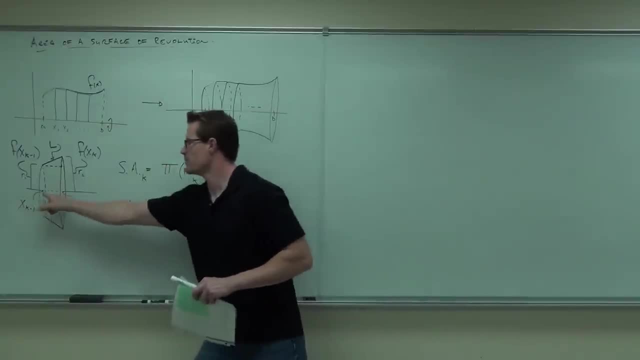 This would be delta x squared, That's the change from x sub k minus 1 to x sub k, And then take a square root of it to find the length. So Pythagorean theorem: leg squared plus leg squared is hypotenuse squared. 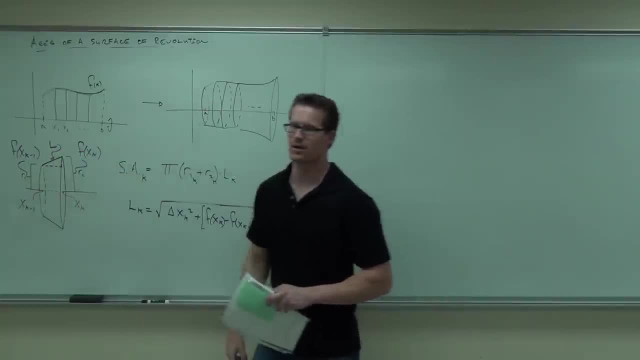 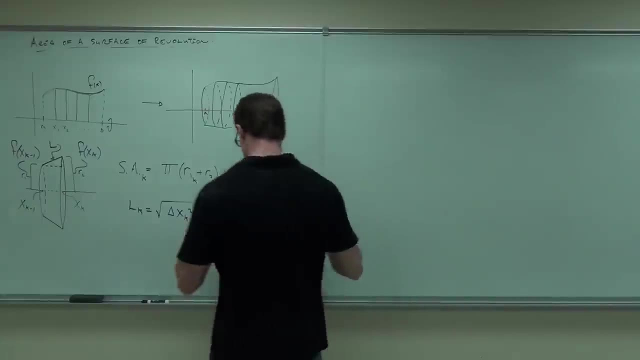 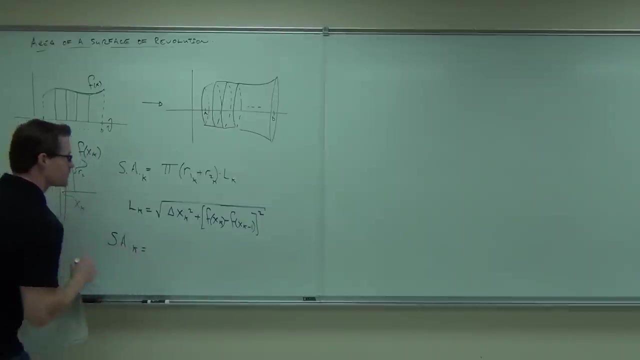 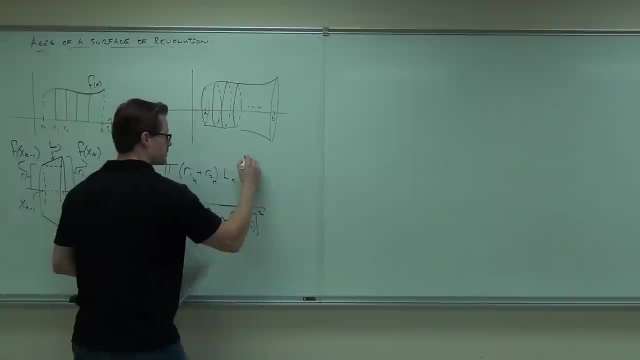 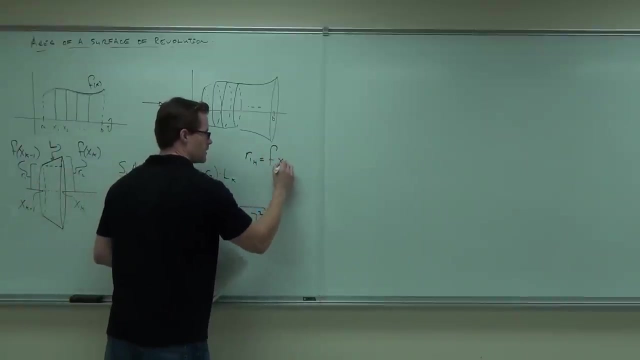 Subtract squared, subtract squared and that's the l. The subtraction here is what's given you delta x. So if we substitute all of this in, we have pi. r1 sub k is the same thing as that And r2 sub k is the same thing as that. 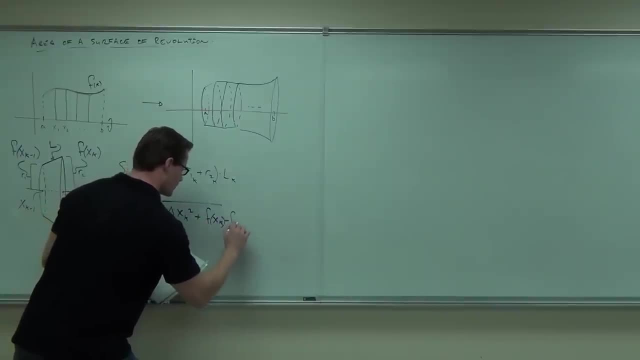 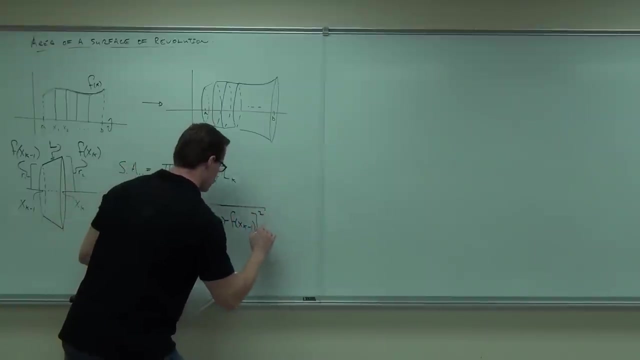 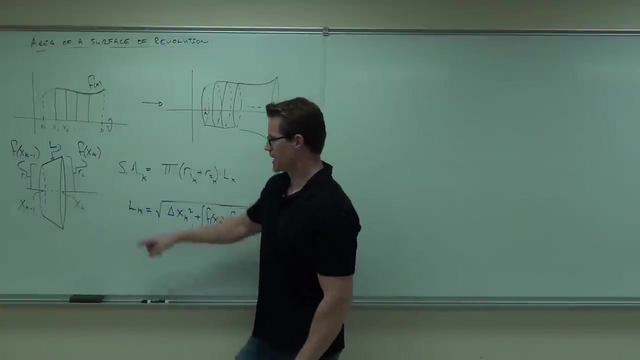 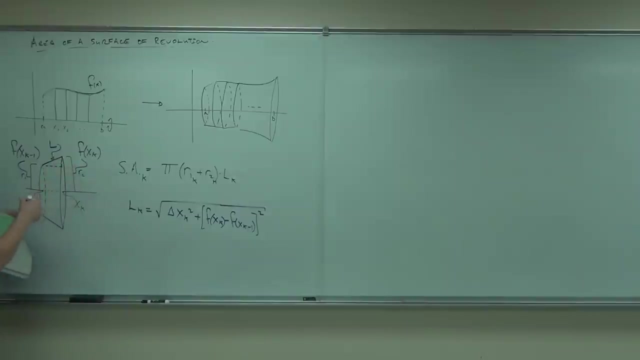 l was that, And you can get that simply by Pythagorean theorem if you really think about it. The change in height here, from here to here- remember, if you draw a little triangle- the change in height is simply f of x sub k minus f of x sub k minus 1.. 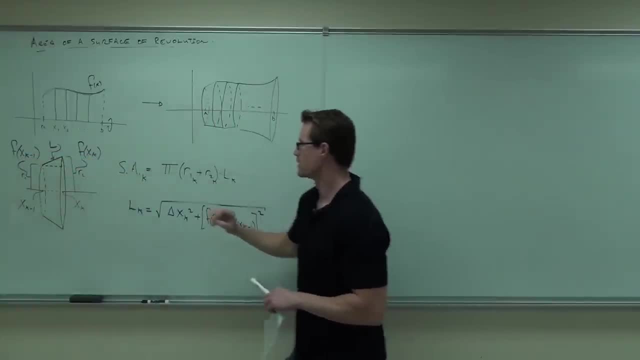 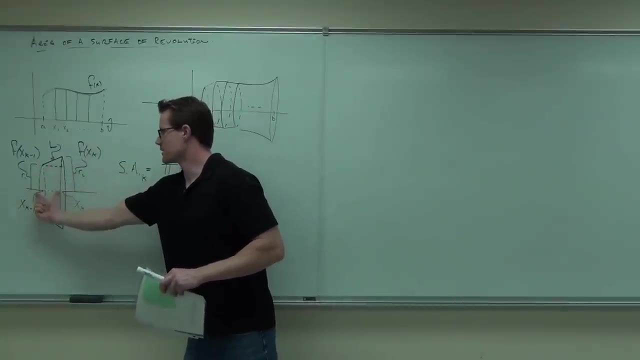 So we have this and then you square it, Pythagorean theorem, square it, Square the height, Square the length. This would be delta x squared, That's the change from x sub k minus 1 to x sub k, And then take a square root of it to find the length. 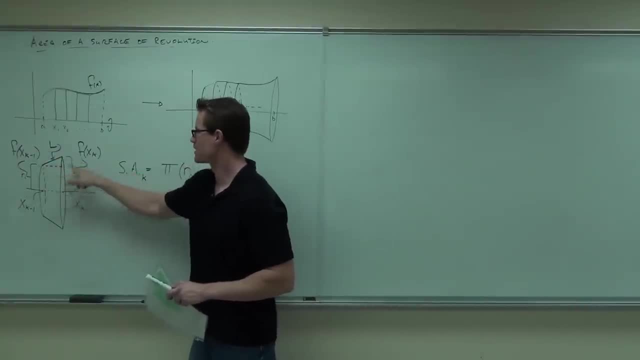 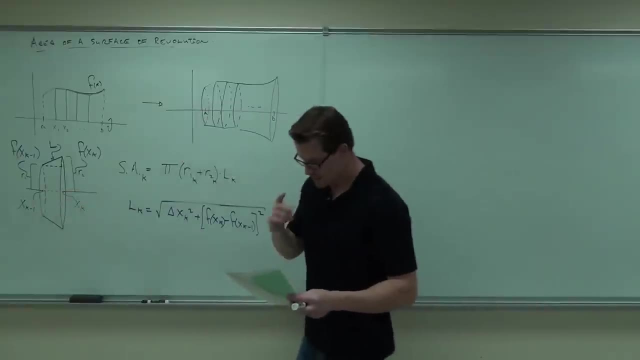 So Pythagorean theorem: leg squared plus leg squared is hypotenuse squared, Subtract squared, Subtract squared, And that's the l. The subtraction here is what's given you delta x. So if we substitute all of this in here, we get delta x. 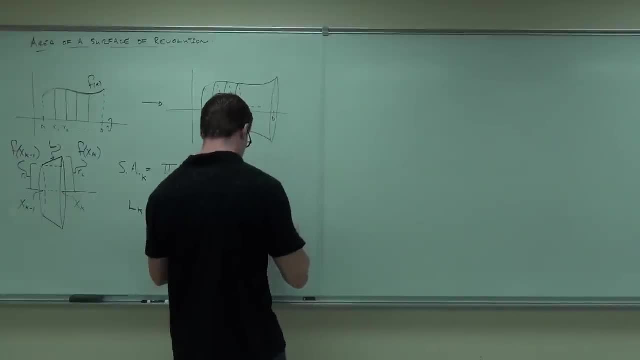 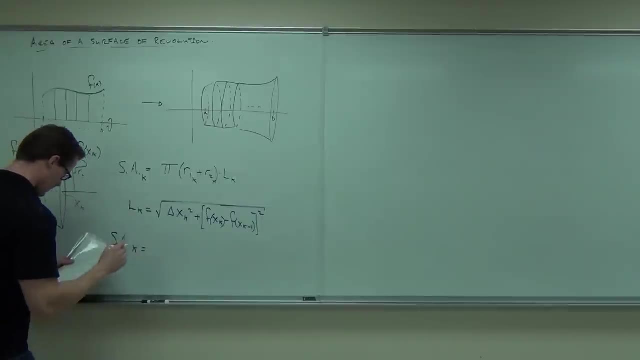 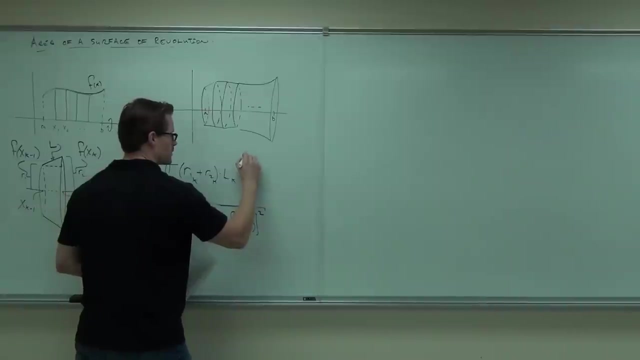 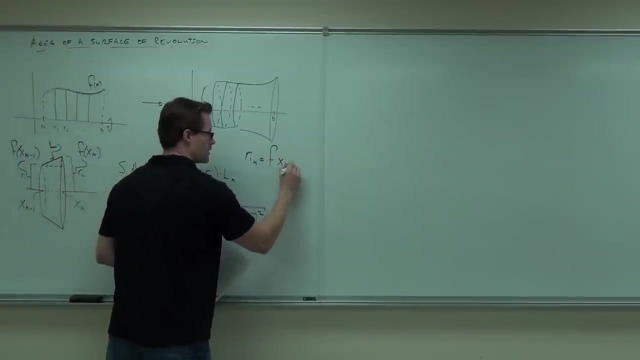 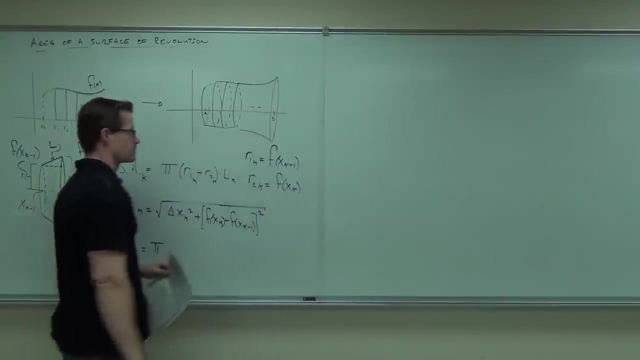 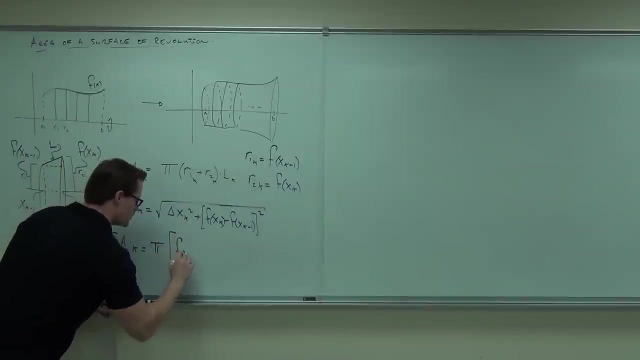 Subtract Subtract, Subtract, Subtract Subtract. We have delta x, So we can substitute all of this in. We have Pi. R1 sub k is the same thing as that And R2 sub k is the same thing as So during our substitution we've got r1 sub k. okay, r1 sub k plus times all of. 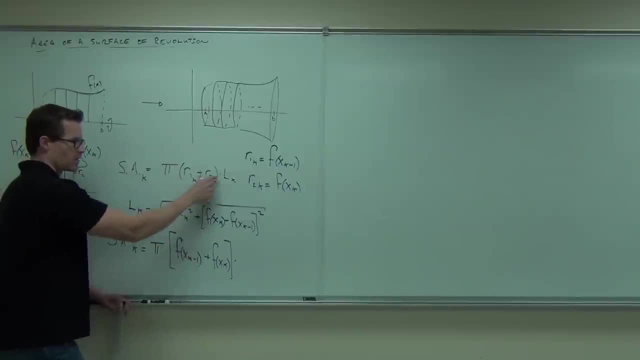 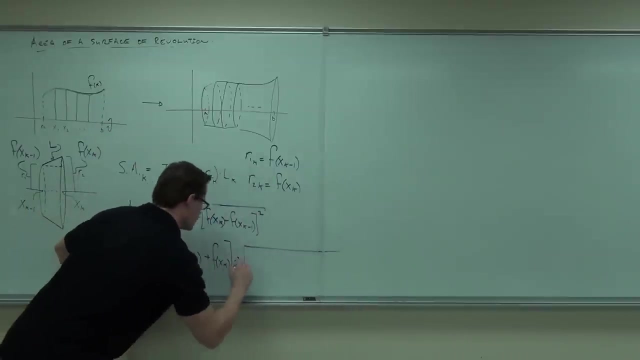 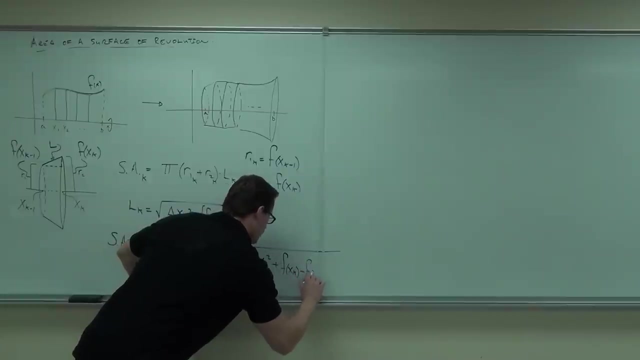 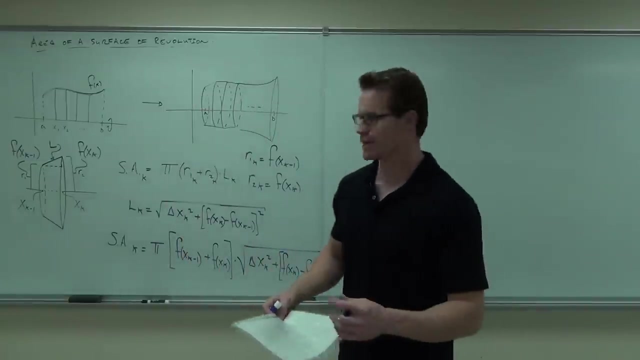 l. sub k, We have pi, pi, r1, r1, r2, r2, l? l Don't forget the square. Now, this is all well and good, but we can't do anything with this unless we deal with. 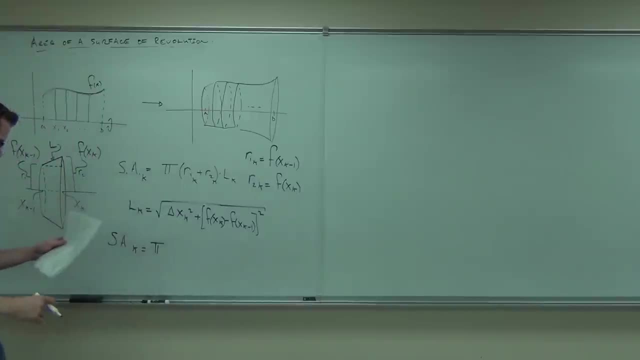 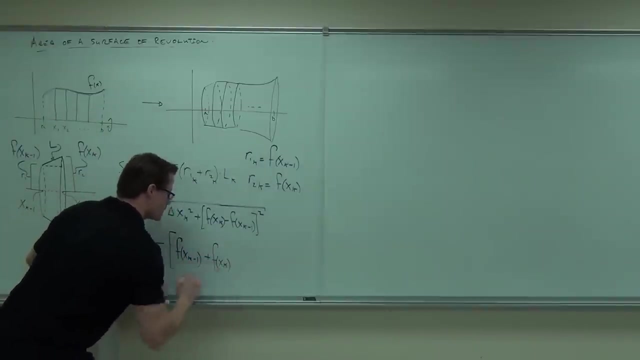 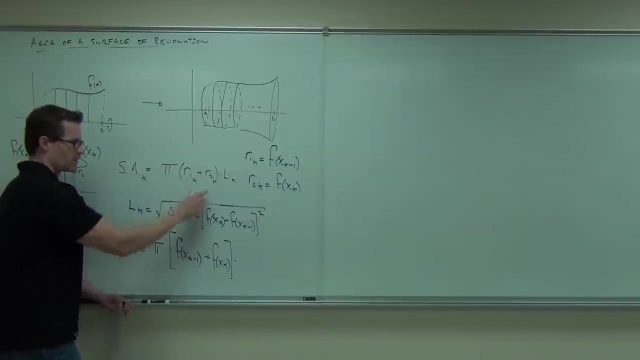 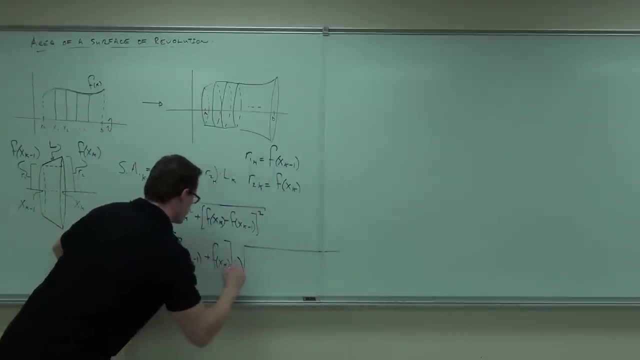 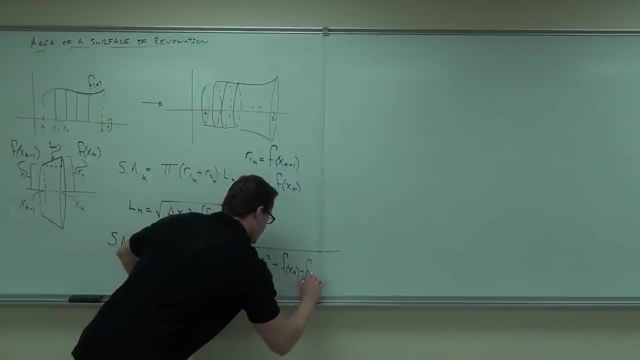 So during our substitution we've got r1 sub k plus times all of l sub k. We have pi, pi, r1, r1, r2, r2, l. l Don't square. Now this is all well and good, but we can't do anything. 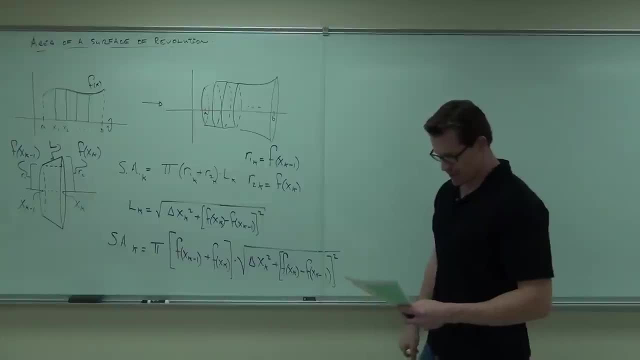 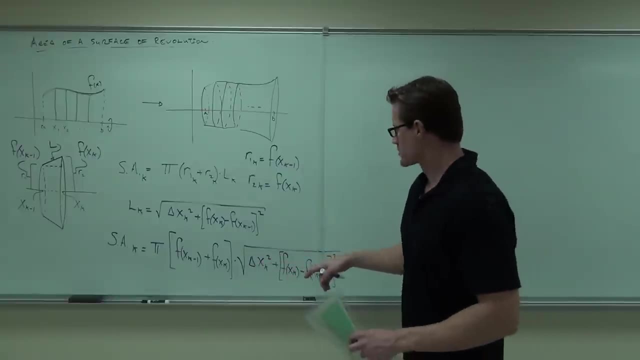 with this, deal with this part unless we deal with this part. So we're going to look at this part right now. This is kind of a reaffirmation that we actually can find length. So basically, what we realize is that this by the intermediate, by the 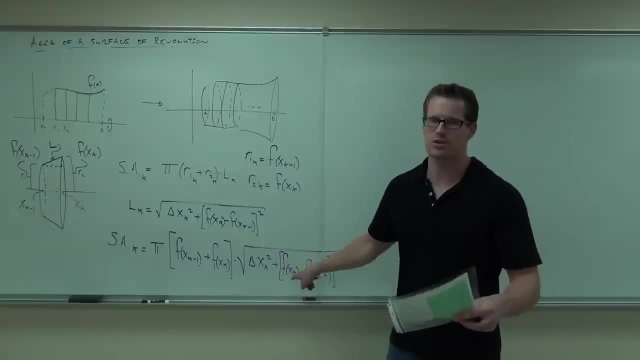 mean value theorem. we can find a point within this. Refresh your last, refresh your memory with the last video. If you weren't able to find the length, if you haven't watched that yet, please watch that. how to find the length of the? 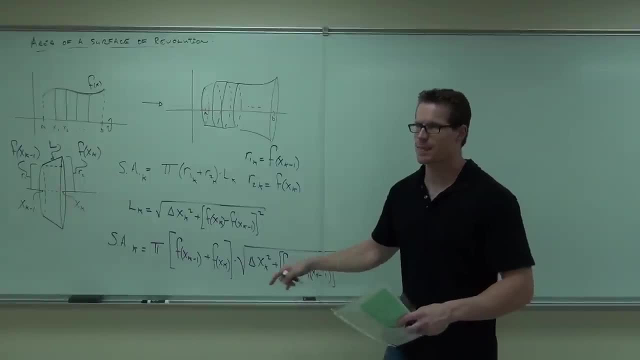 curve, Because what this is by the mean value theorem says: if I manipulate this and have the slope between two points, I can find a certain point, xk dot, which is between x sub k and x sub k minus 1, for which the slope of the function is equal to. 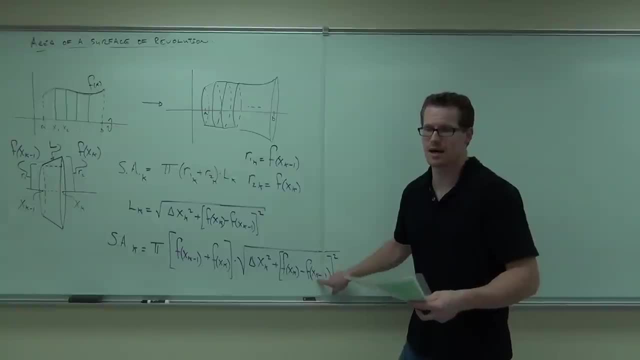 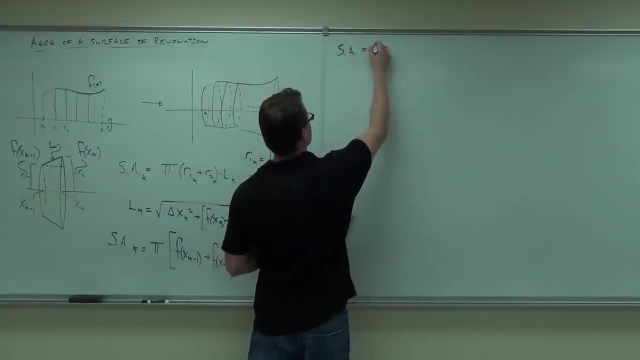 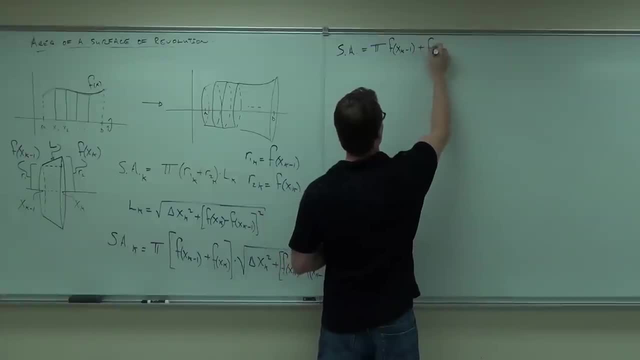 But inside this Pedestrian I have to collect the slope of this speed and whenever it's at x sub k- and it's at x sub k, this curve is going to be equal to the slope of this speed and then we can reframing it for this curve And 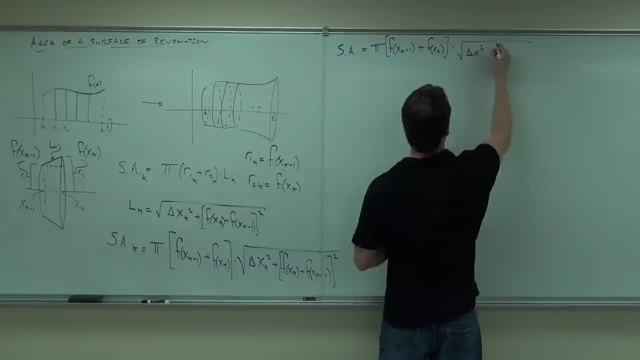 we have a very consistent expression. so we're going to say: if there is a slope between x sub k and x sub k plus 1, that is, let's say, 1 x sub k plus 1, what would that be? So this is the normal deviation between this and this. 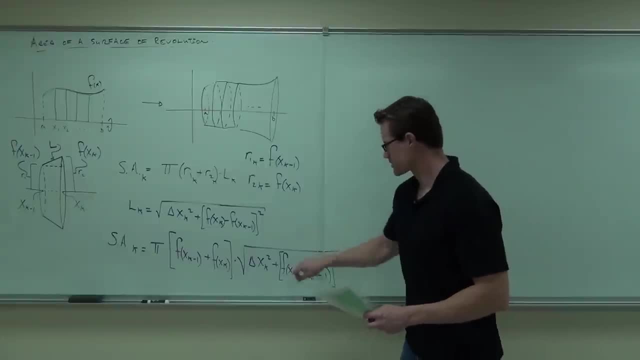 this part unless we deal with this part. So we're going to look at this part right now. This is kind of a reaffirmation that we actually can find life. So basically, what we realize is that this by the intermediate, by the mean value theorem. 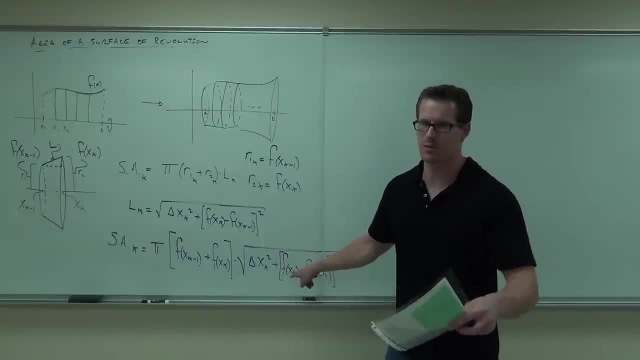 we can find a point within this. refresh your memory with the last video if you weren't able to find the length. If you haven't watched that yet, please watch that. how to find the length of a curve? Because what this is by the mean value theorem says: if I manipulate this and have the slope, 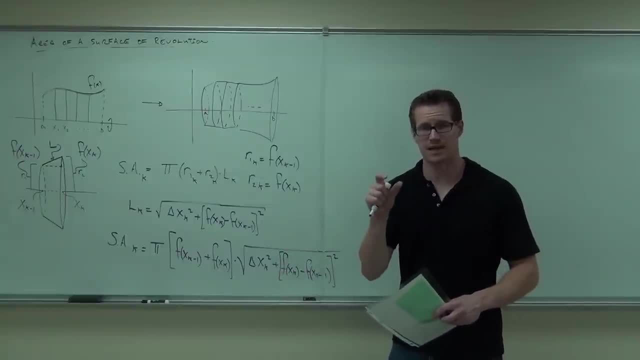 between two points. I can find a certain point, xk dot, which is between x sub k and x sub k minus 1, for which the slope of the function is equal to the slope between the two points. In other words, the derivative at xk dot equals the slope between two points. 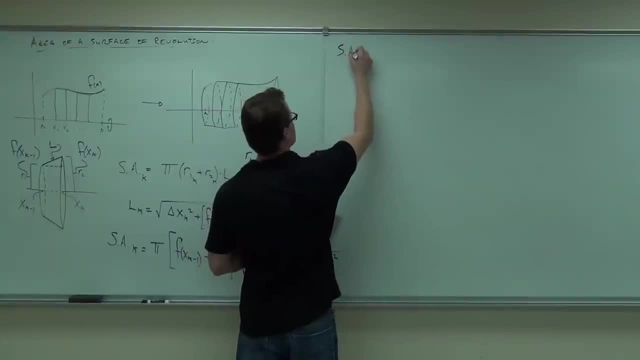 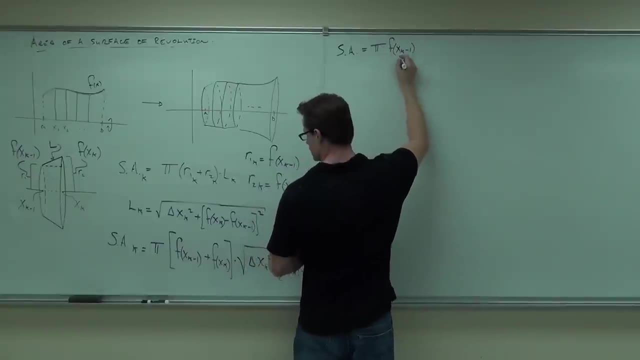 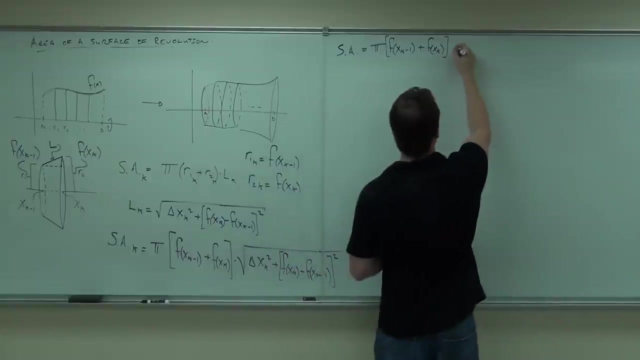 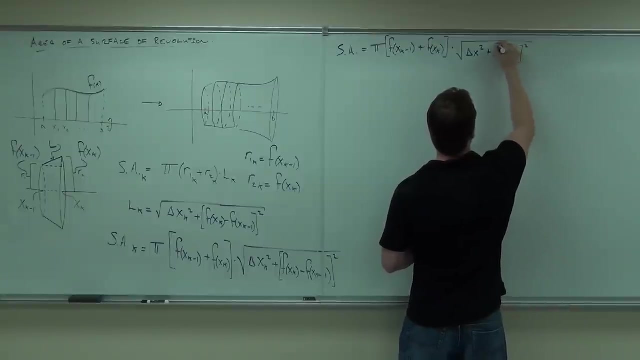 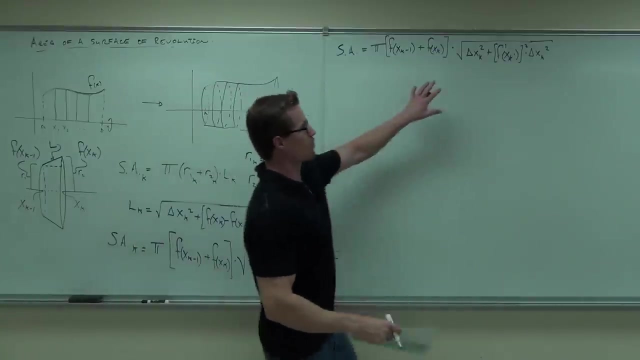 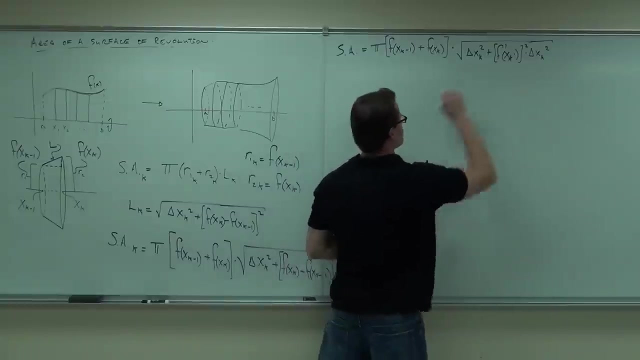 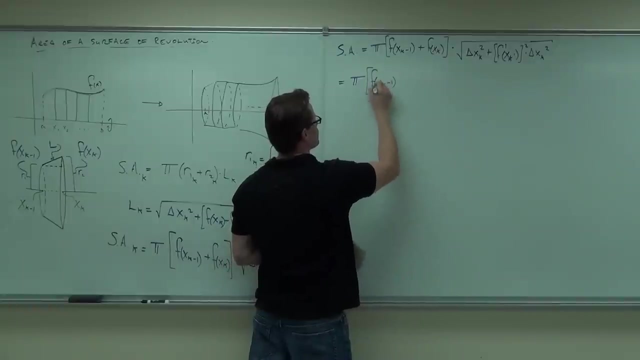 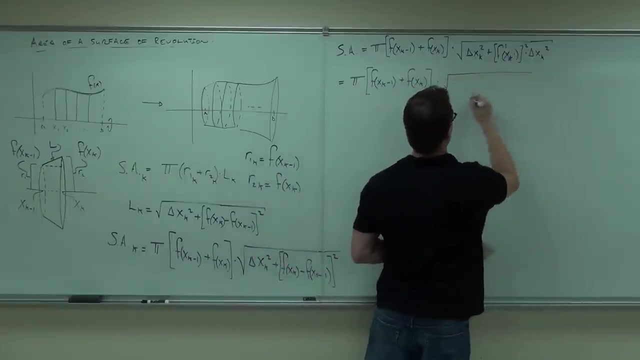 So what this translates to, This translates to, is That's it, and you'll remember this. this is the length from last time, or from section 5.0, earlier in the section, so we'll factor out again. Notice that it has a square root of two things that are being multiplied together. 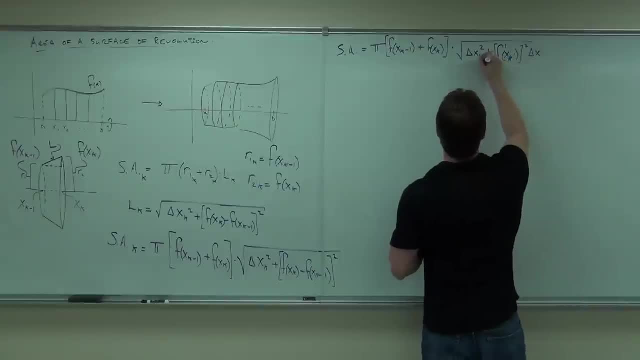 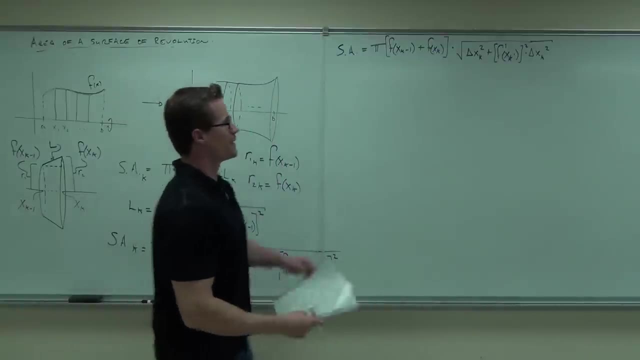 right here. variable- All right. Well, I don't not have time to do that for you Now. we'll take a break and we'll see what we have done. No, that's it, and you'll remember this. this is the length from last time or from section. 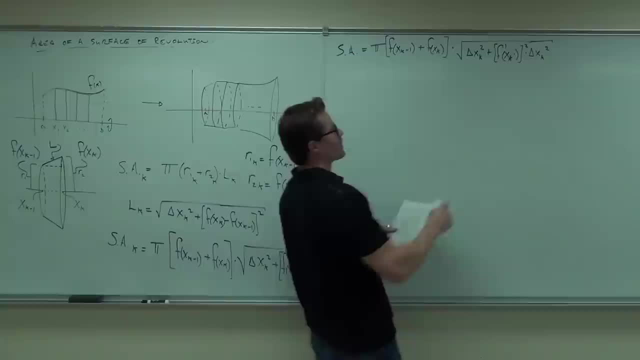 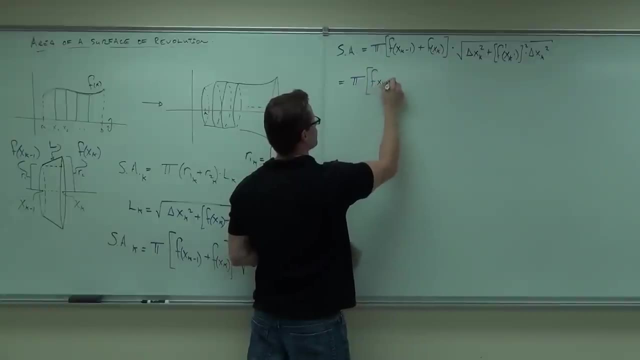 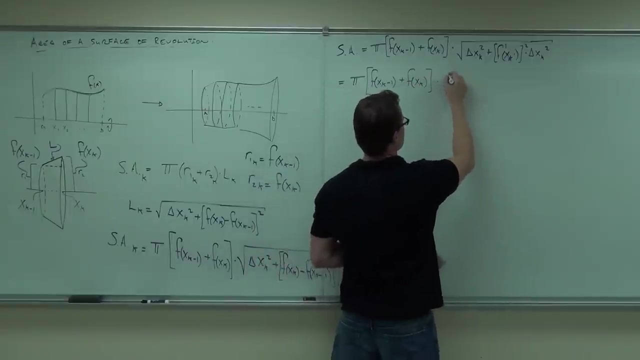 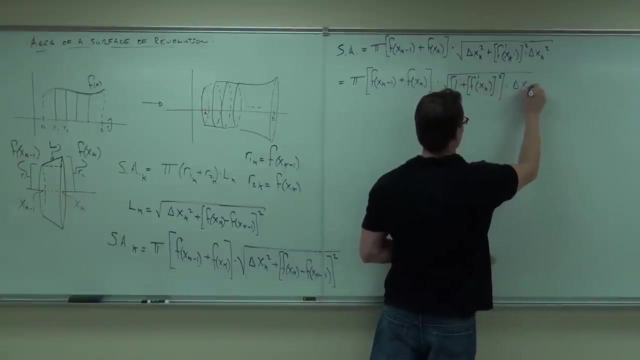 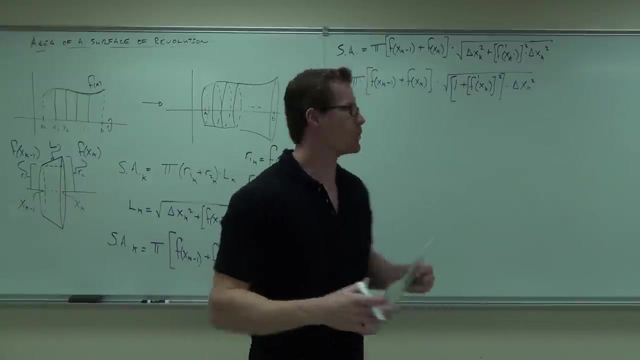 5.0, earlier in the section. So we'll factor out again. Notice that it has a square root of two things that are being multiplied together. We can split up those products, So we'll take the square root of this, leave it. 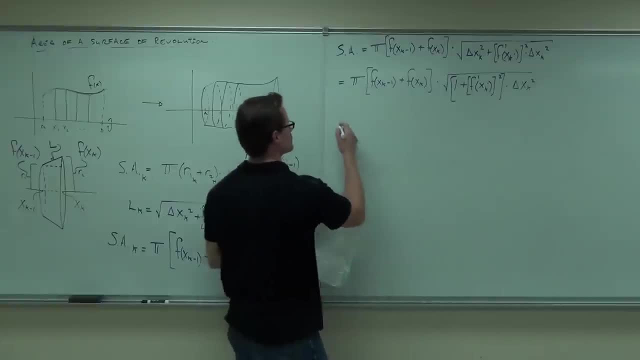 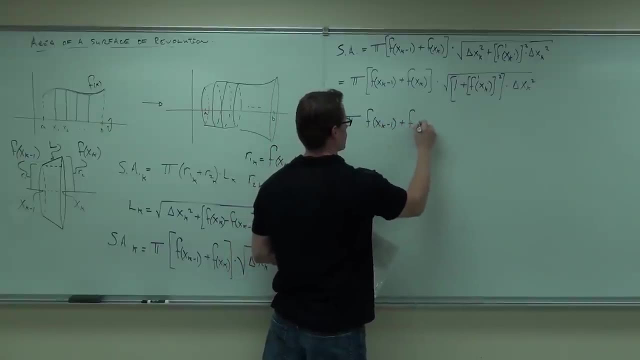 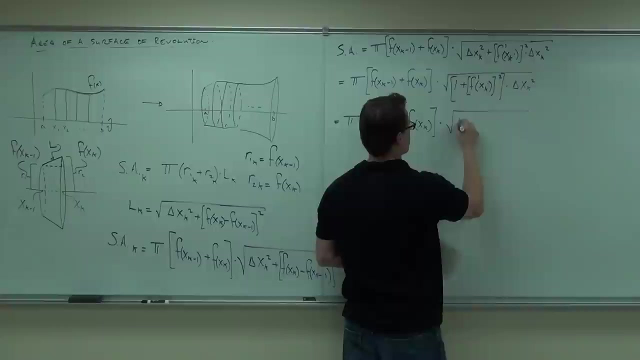 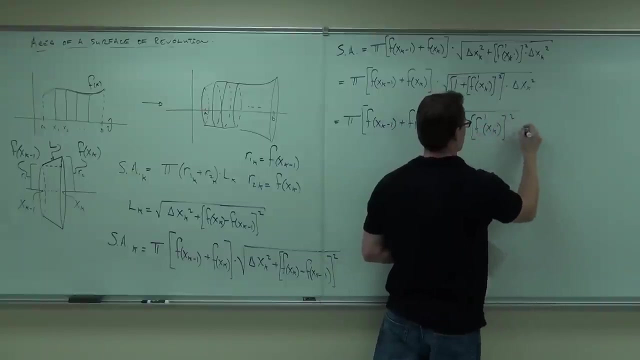 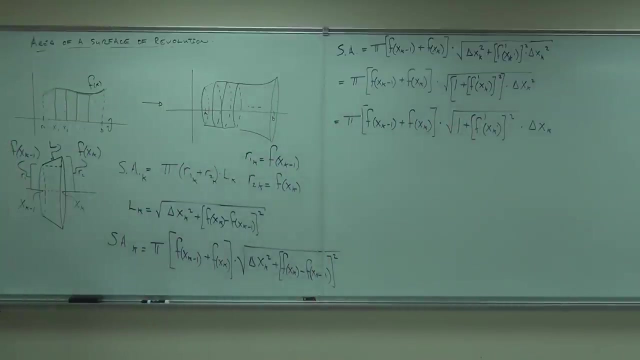 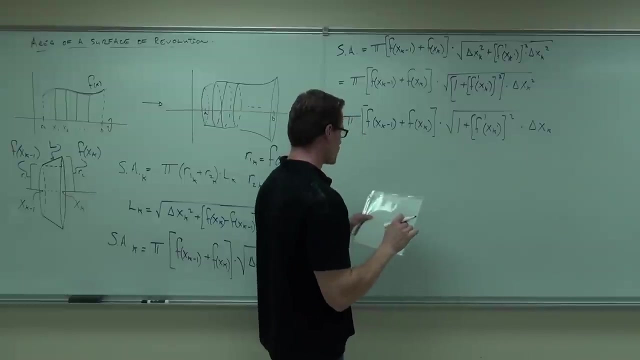 We'll take the square root of this. that'll be delta x sub k. Well, we're almost done. Now I'm going to be a little sneaky here. What I'm going to do is think about just this piece for a second. 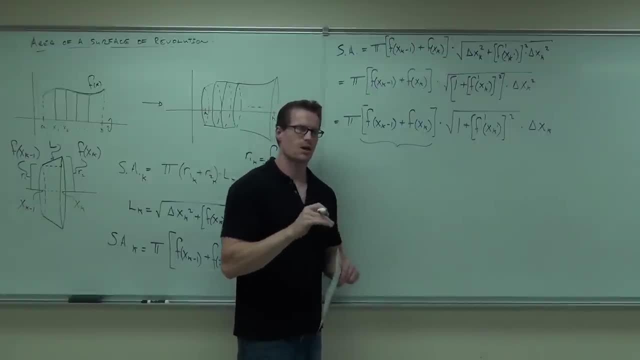 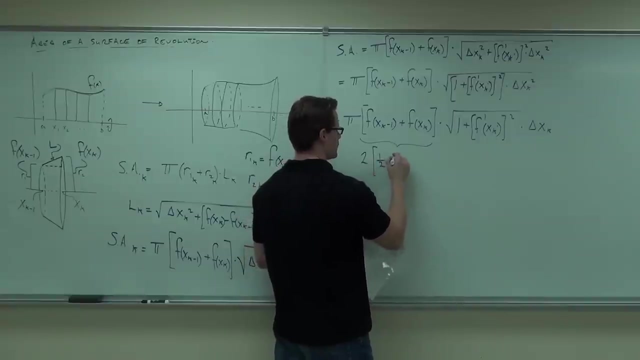 Now just this piece. I'm going to manipulate it. I'm going to multiply by two and by one half. Now, when you think about that, two times one half gives you one. So I'm really only multiplying by one, but I'm doing it in a very special way. 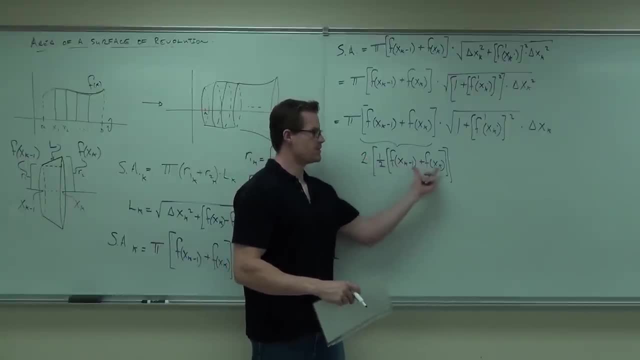 Now what is this? Ignore the two. Look at the one half this. If you add two things together and divide by two, You get the thing that's right in the middle of it. What you get is the average. So, basically, what we're having here is the average of the heights. 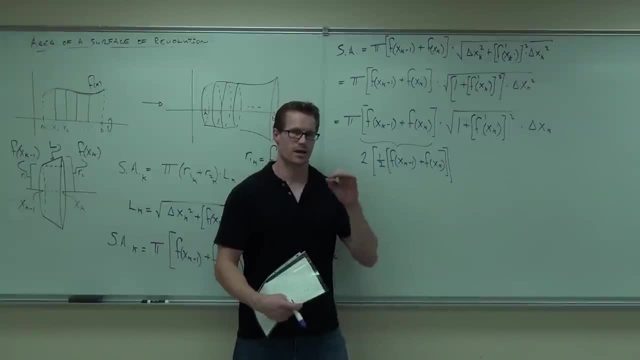 The average of them. Now, what I'm going to do is let another arbitrary point. we have an x k dot already. I'm going to choose x k dot dot to be that. I know it's weird, that other arbitrary point. 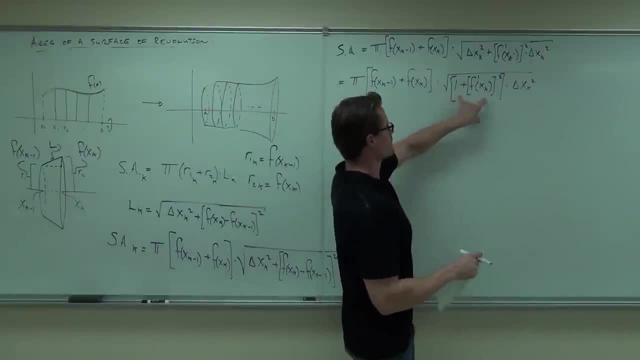 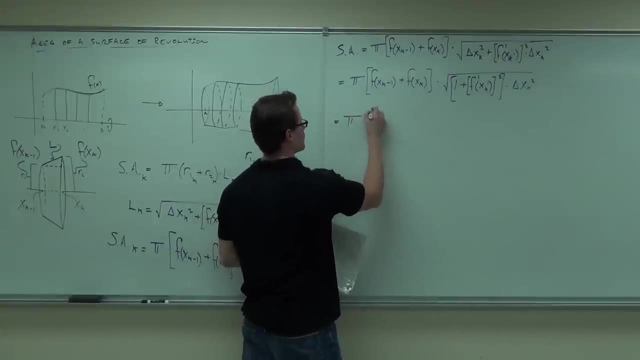 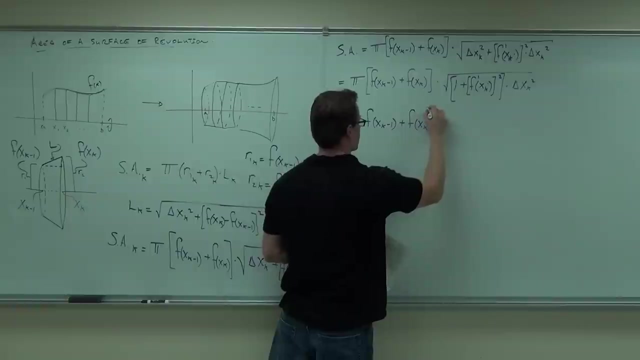 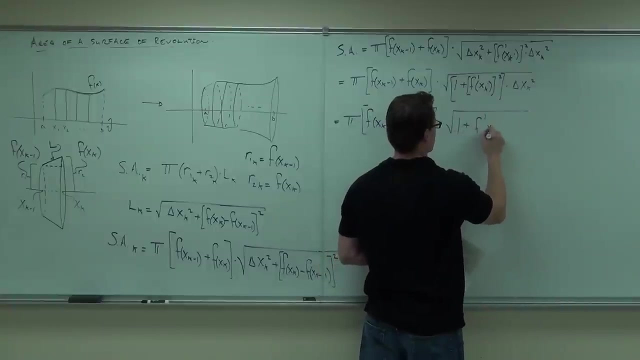 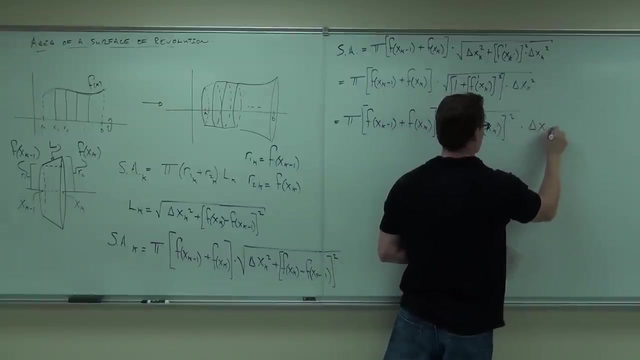 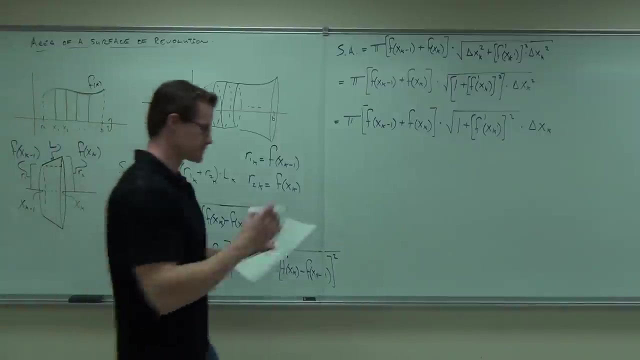 We can split up those products. So we'll take the square root of this. leave it. We'll take the square root of this. that'll be delta x sub k. We're almost done. Now I'm going to be a little sneaky here. 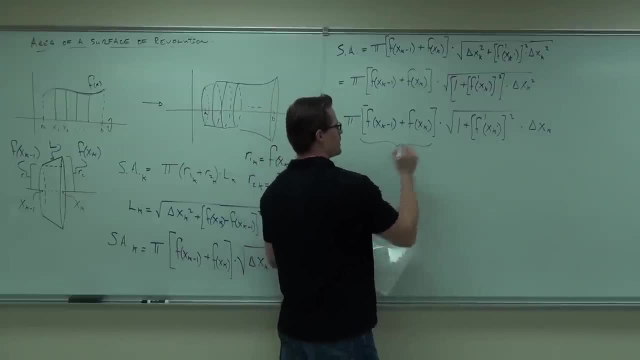 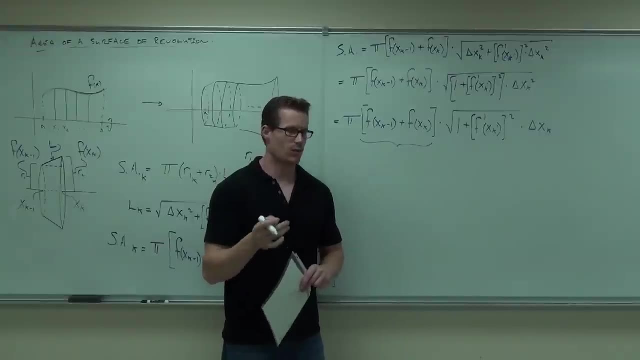 What I'm going to do is think about just this piece for a second. Now, just this piece. I'm going to manipulate it. I'm going to multiply by two and by one-half. Now, just this piece. I'm going to manipulate it. I'm going to multiply by two and by one-half. 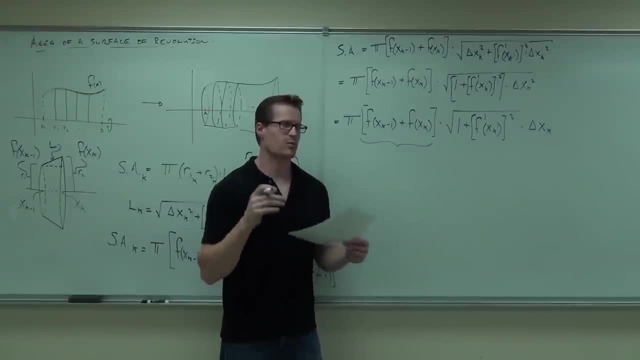 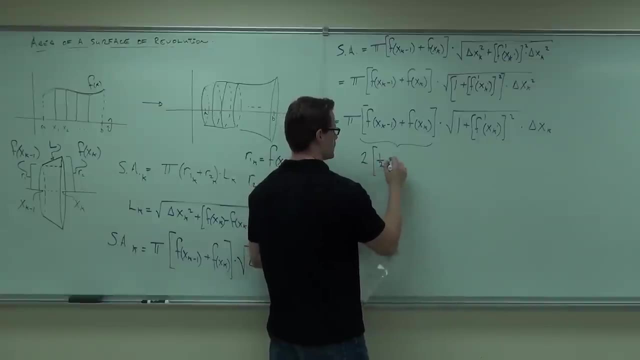 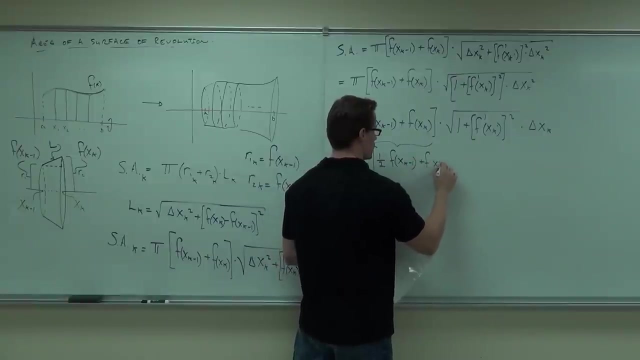 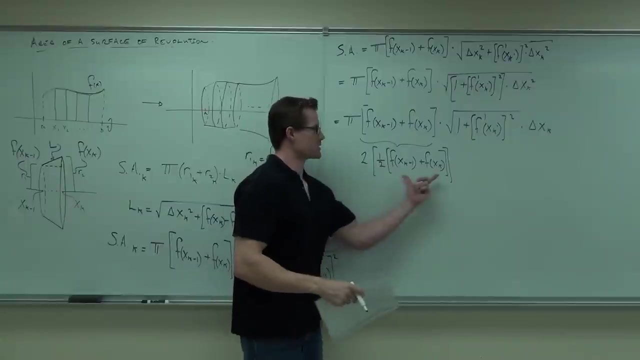 Now, when you think about that, two times one-half gives you one. So I'm really only multiplying by one, but I'm doing it in a very special way. Now, what is this? Ignore the two. Look at the one-half. this: 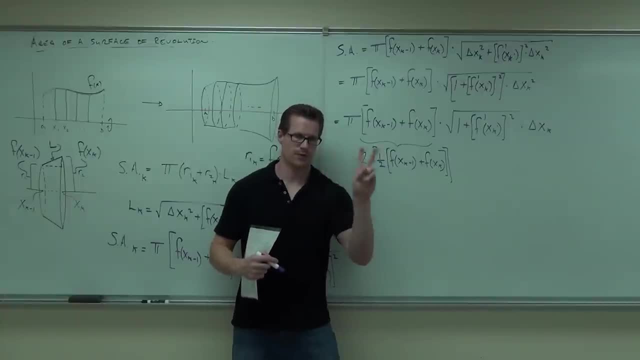 If you add two-thirds, If you put two things together and divide by two, you get the thing that's right in the middle of it. What you get is the average. So, basically, what we're having here is the average of the heights, the average of them. 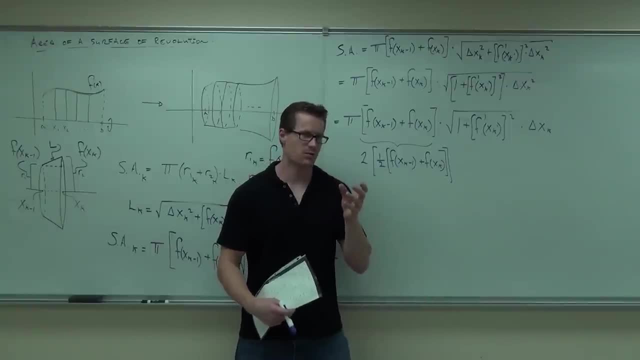 Now what I'm going to do is let another arbitrary point. we have an xk dot already. I'm going to choose xk dot dot to be that. I know it's weird, that other arbitrary point. So I'm going to say there's some point. I'll explain it. 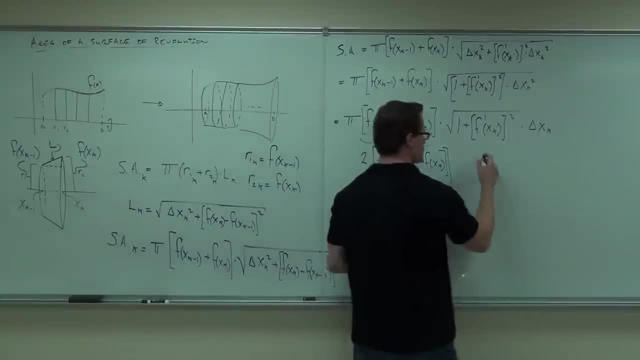 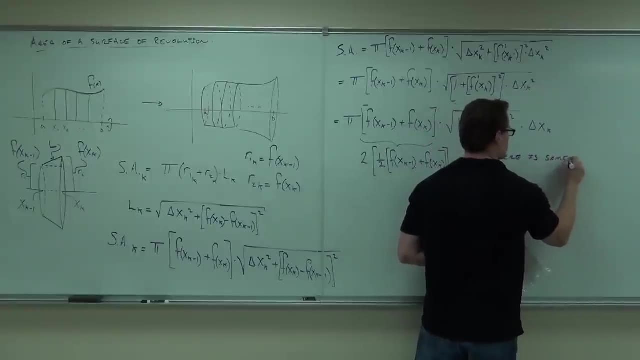 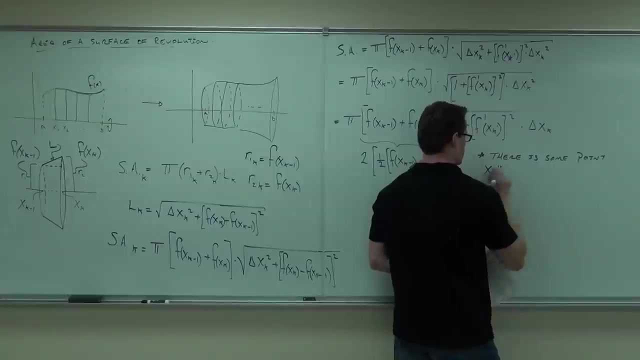 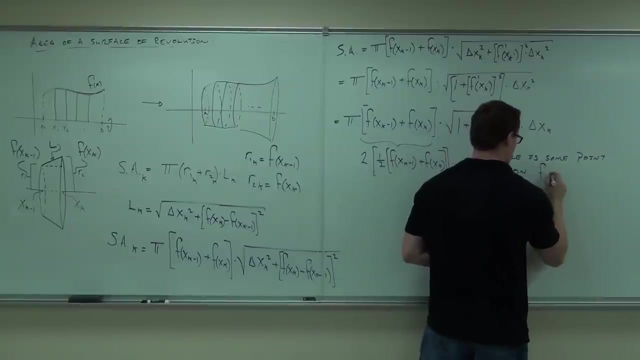 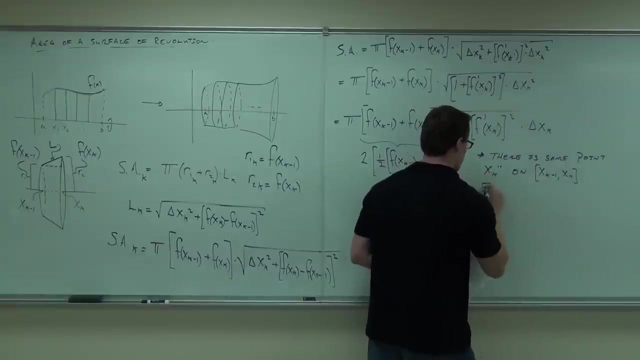 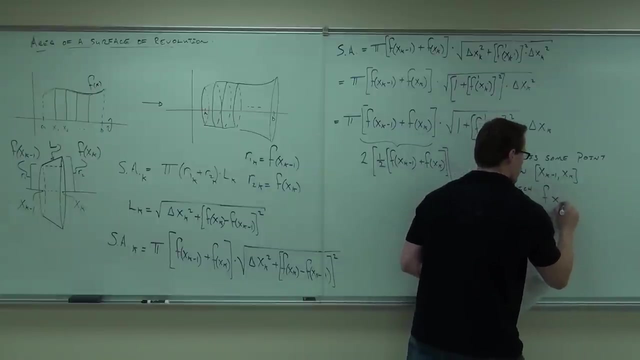 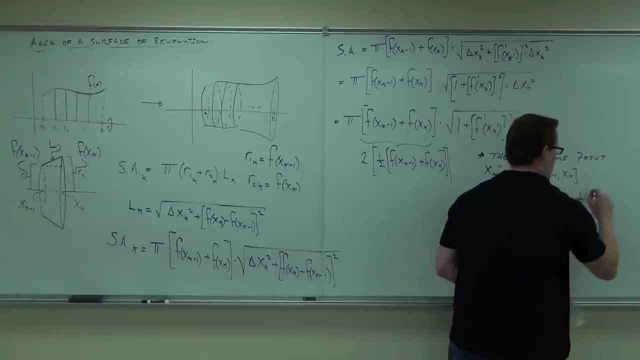 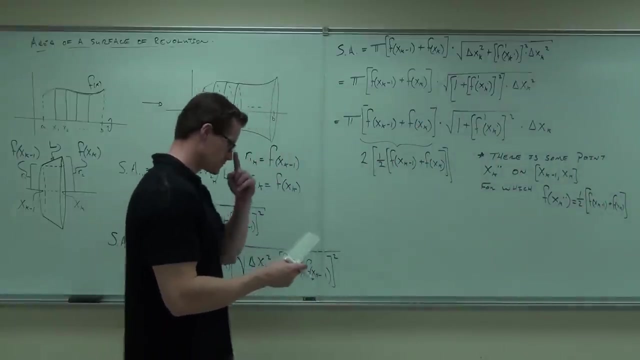 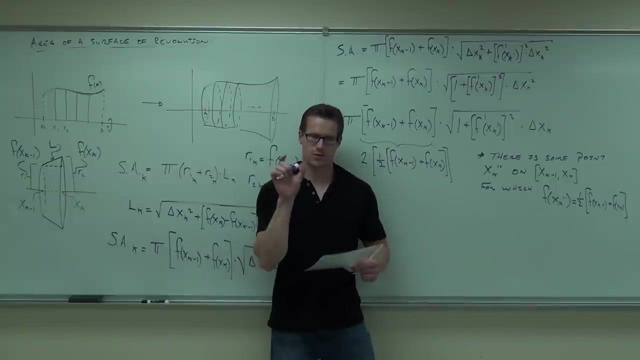 So I'm going to say there's some point. well, I'll explain it. There's some point: xk, dot, dot On this interval, for which f of xk double dot equals one half, equals the average, basically the average height. Here's what it says in English. it says if x is within some interval, 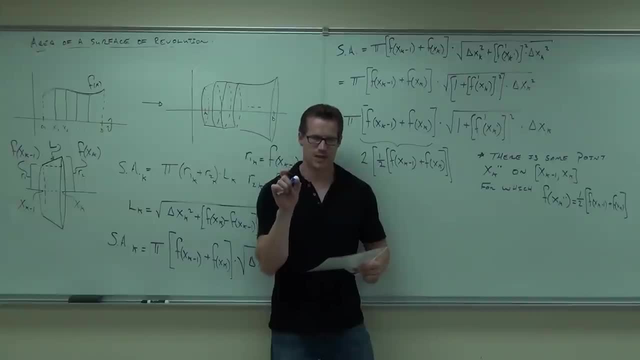 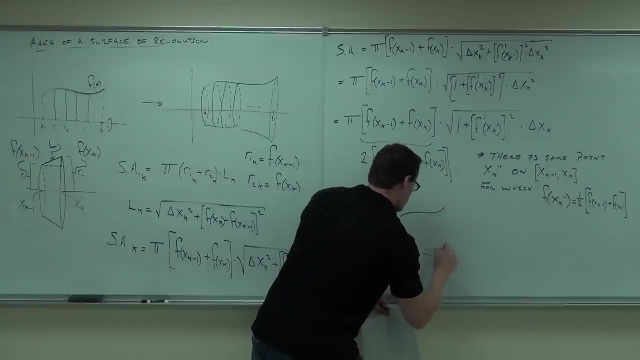 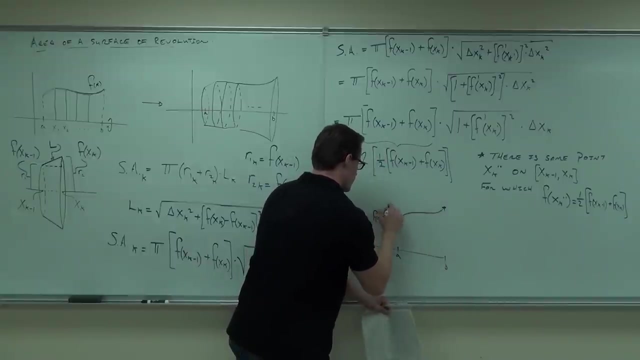 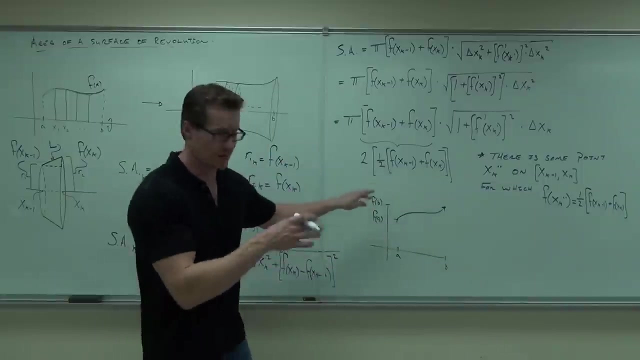 and k is between f of a, b and f of a and f is continuous. f of x has to equal k at some point, x. In other words, it says intermediate value theorem. Basically, it says this thing. this is what I'm using in English. 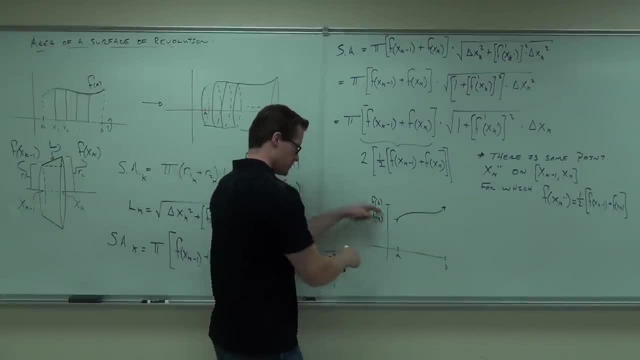 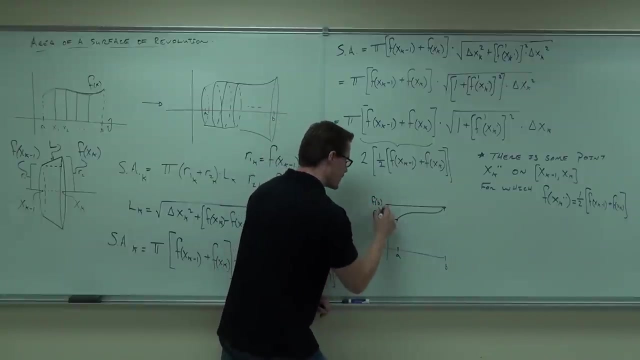 It says: hey, pick a point between here, between here, Pick some point between here. Call it x, We're calling it xk, dot, dot. So maybe we'll put the dot. It says if f is continuous, then there must be some point. 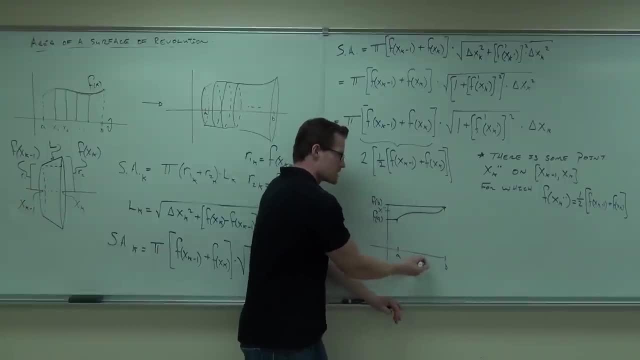 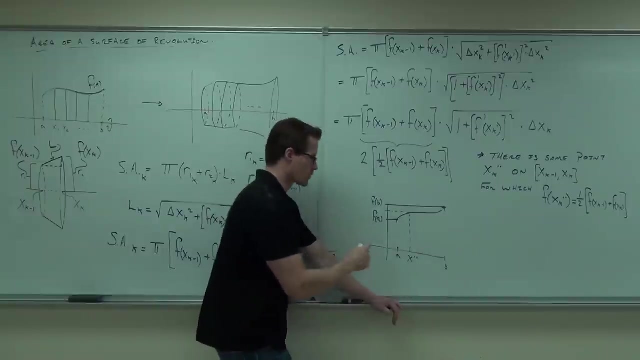 and it must be between here so that when I plug this into my function it gives me exactly this height. Let me show you. It says there's going to be some point. I think I put the x dot in the wrong place. 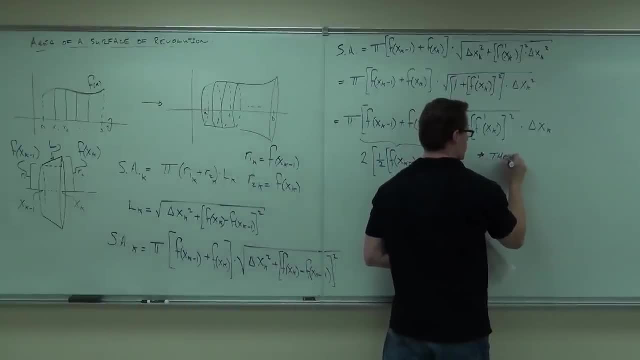 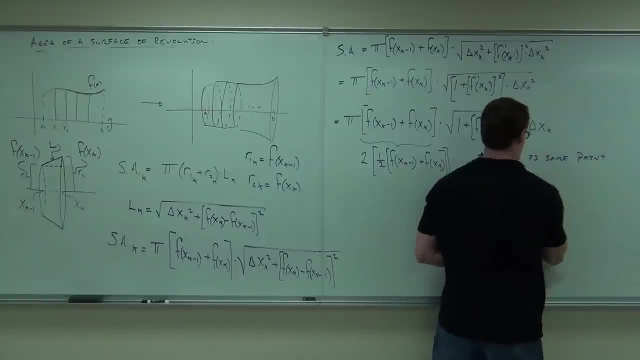 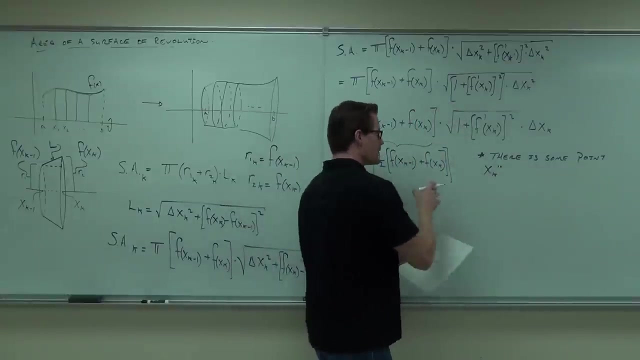 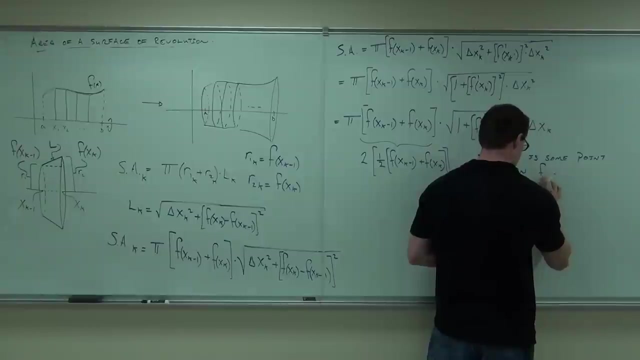 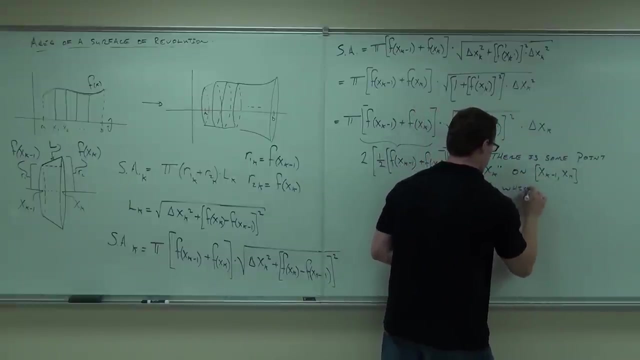 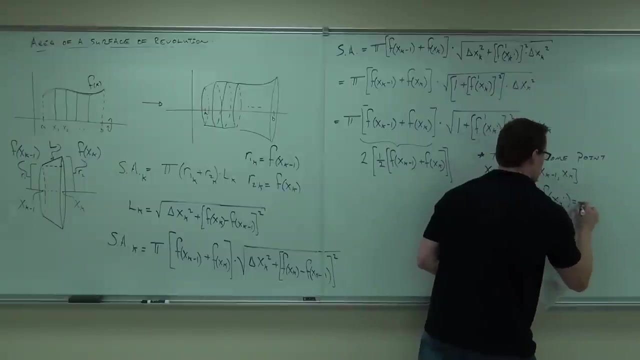 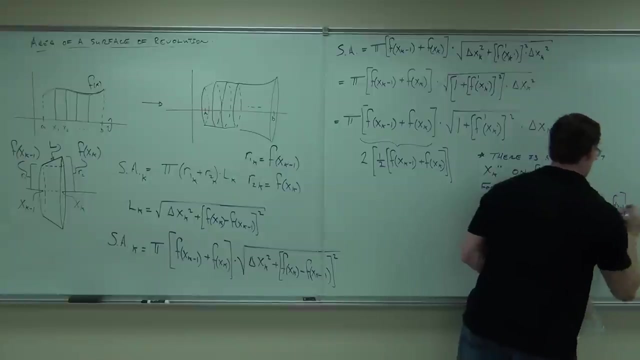 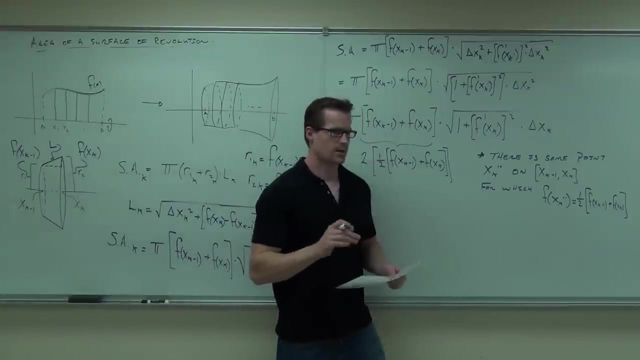 There is some point. There is some point: Xk dot, dot On this interval. This h, For which f of xk double dot equals 1 half, equals the average, basically the average height. Here's what it says in English. it says: if x is within some interval and k is between, 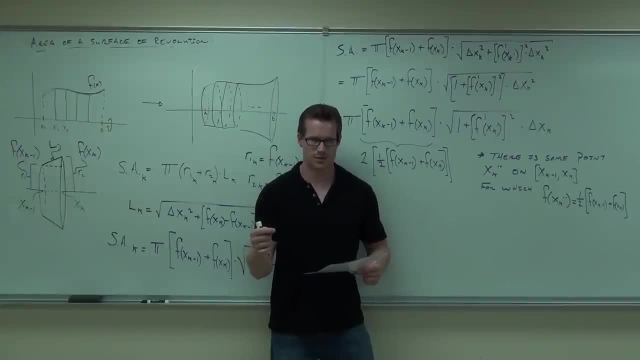 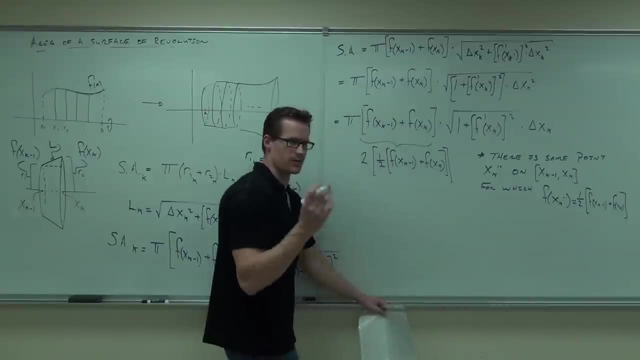 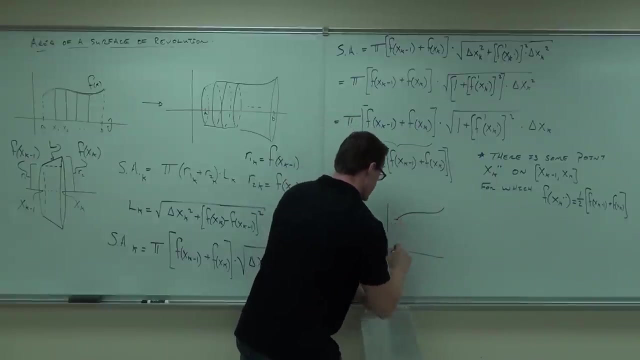 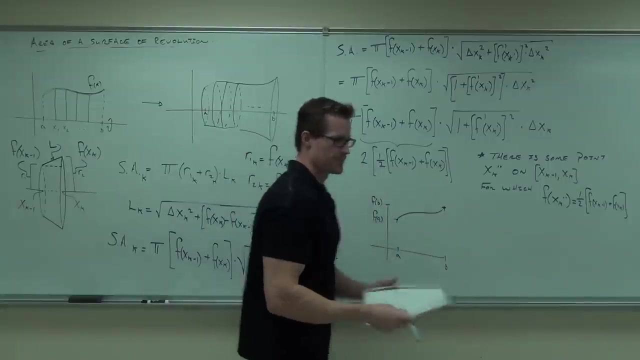 f of a being f of a and f is continuous. f of x has to equal k at some point, k at some point x. In other words, it says intermediate value theorem. basically, it says this thing. this is what I'm using in English. 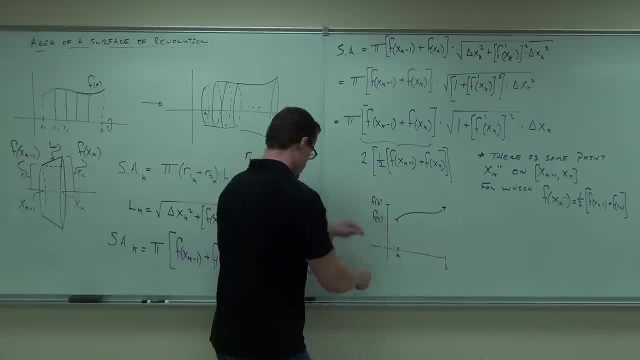 It says: hey, pick a point between here, between here. Pick some point between here. Call it x, We're calling it xk, dot, dot. so maybe we'll put the dot. It says if f is continuous, then there must be some point, and it must be between here. 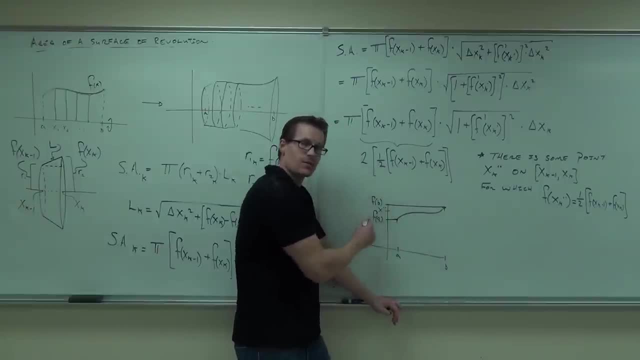 so that when I plug this into my function it gives me exactly this height. Let me show you. It says there's going to be some point. I think I put the x dot in the wrong place. There's going to be some point. x, sub dot dot for which you can find the average. 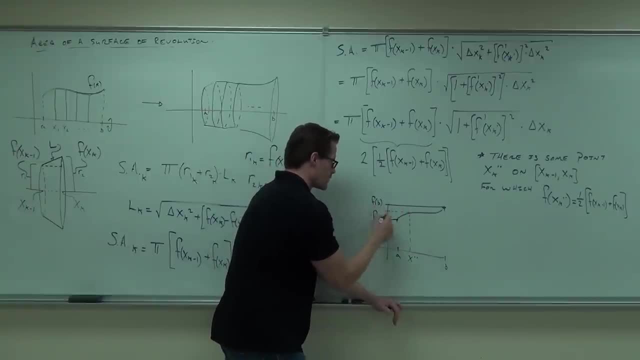 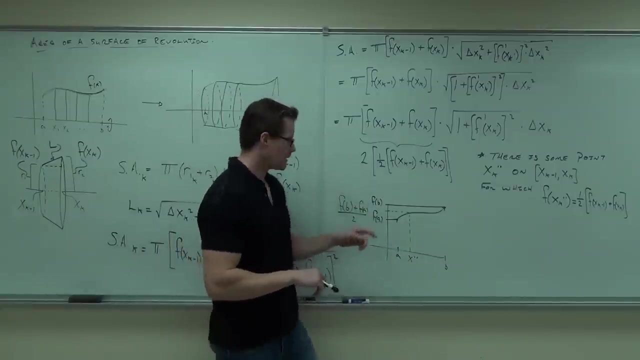 There's going to be some point x, sub dot, dot for which you can find the average. Look what we've done. We've taken the average of f of a and f of b. That's the height right in the middle of it. 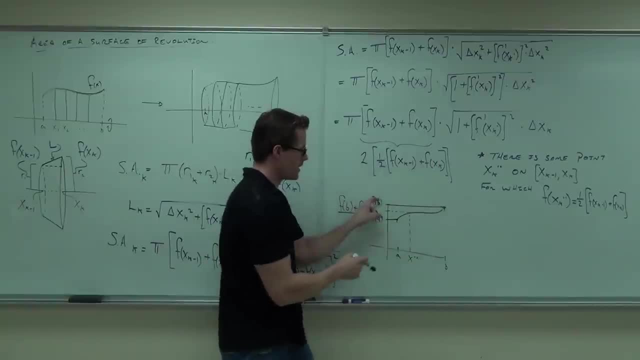 That's actually exactly what this is right here. That's the average height. We're saying that if this is continuous, then there is some point that you can plug in that's going to give you the average height. Let me say that again. 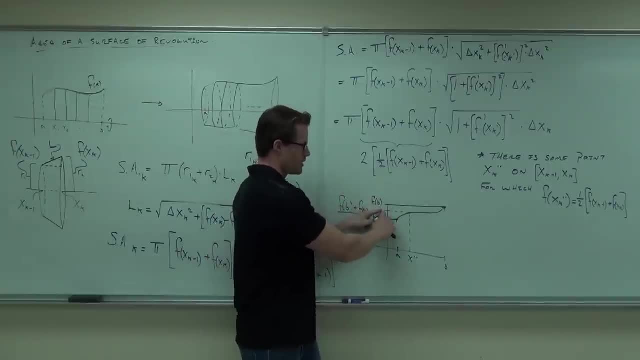 This is the average height. Average height. There must be some point, since f is continuous, so that I plug in that point between a and b and it gives me out the average height. It says: this is going to be there. We're calling it x. dot, dot. 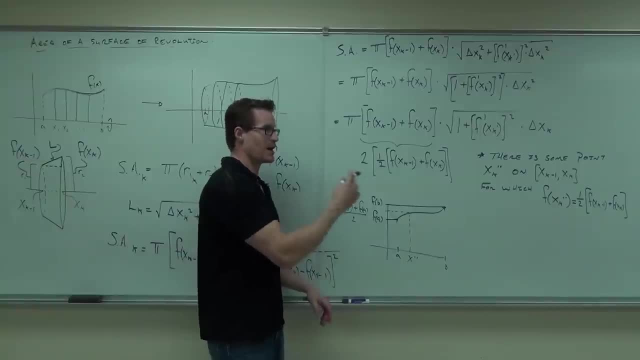 Hopefully you understood that. If you didn't, I'll go back and watch it again. I hope This is just average height, It's continuous. There's got to be a point that I can plug in that gives me average height. There's got to be a point that I can plug in. 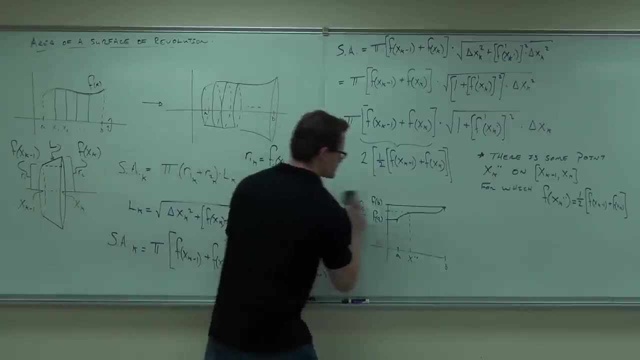 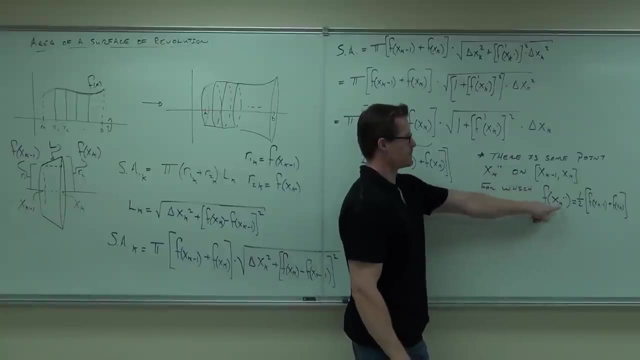 that gives me average height. That's what that says. It says that there's some point that I can plug in. It's between here. When I plug it in, it gives me the average height because f is continuous. It has to happen. 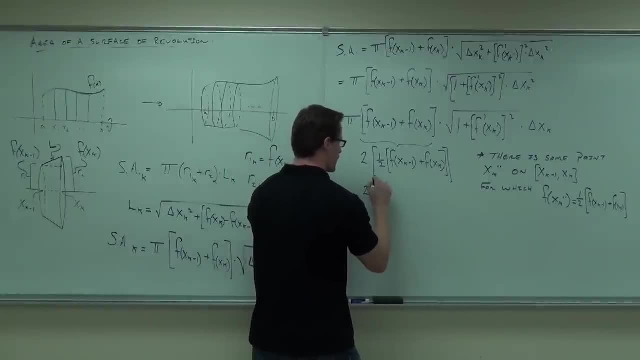 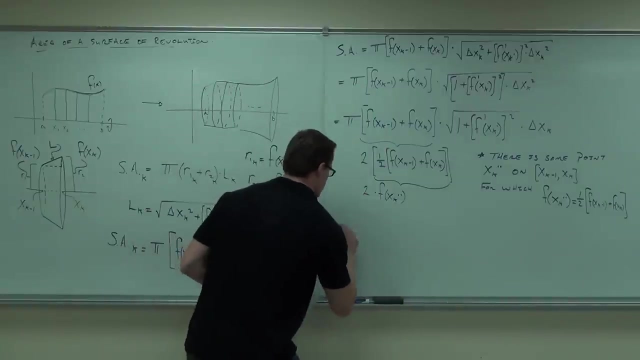 I'm going to let this become 2 times. f of x, k, dot dot. Let's see, We're almost done. We have now a 2, a pi, a 2.. f of x, k, dot dot. That's all this. 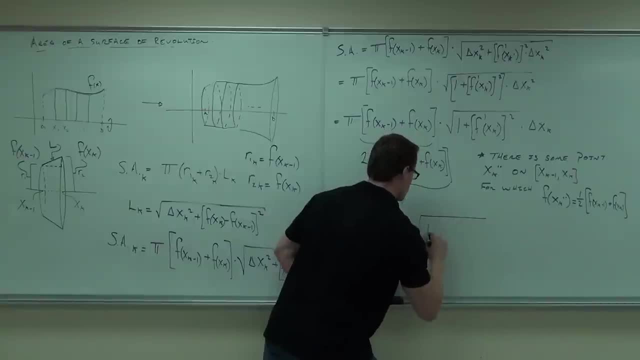 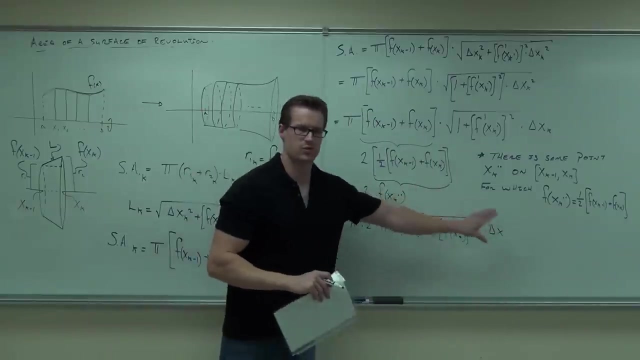 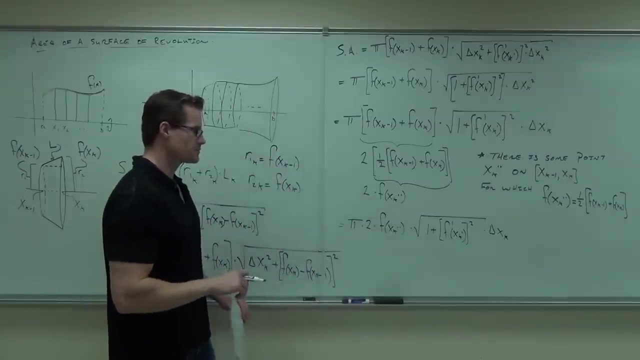 We already had the length Times delta x. Delta x is now outside of our square root. Remember we took the square root of delta x- k dot Times, delta x- k square. Let's try this again, So pretty close to done. 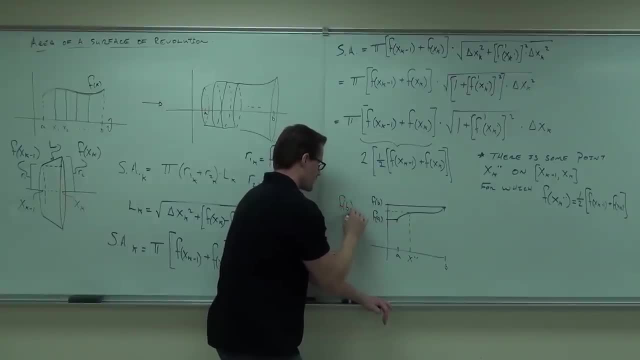 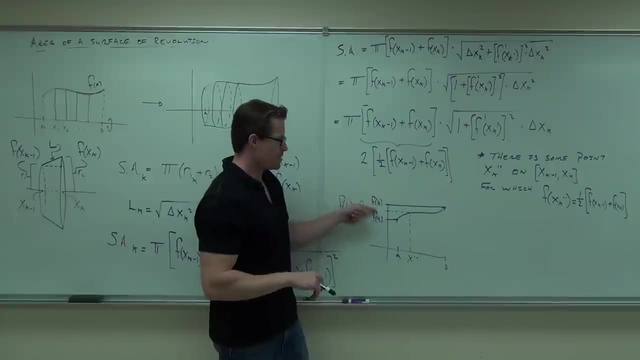 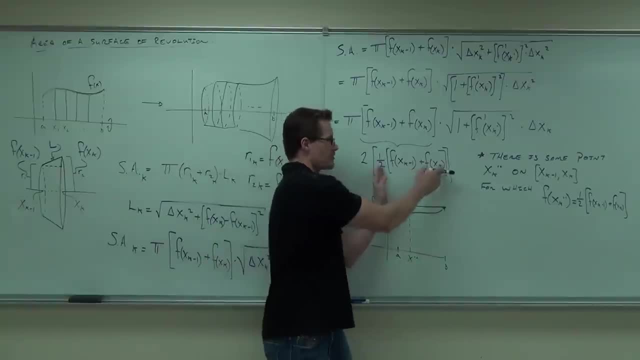 of it. That's actually exactly what this is right here. that's the average height. average height. We're saying that if this is continuous, then there is some point that you can plug in that's going to give you the average height. 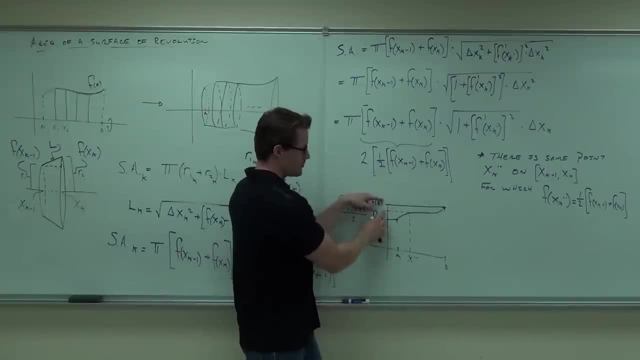 Let me say that again, This is the average height. Average height. There must be some point, since that is continuous. so then I plug in that point between A and B and it gives me out the average height. It says this is going to be there. 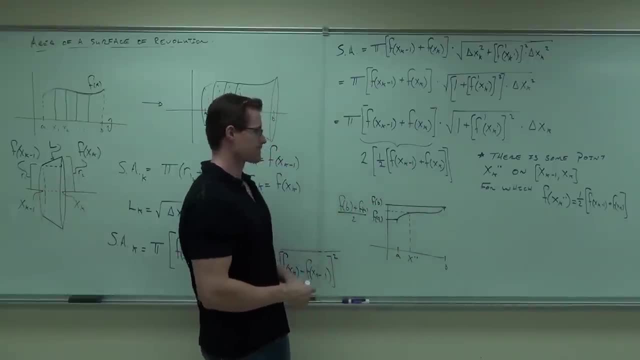 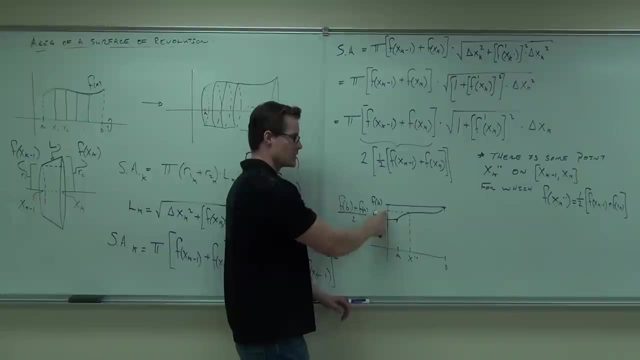 We're calling it X dot dot. Hopefully you understood that. If you didn't, I'll go back and watch it again. I hope This is just average height, It's continuous. There's got to be a point that I can plug. 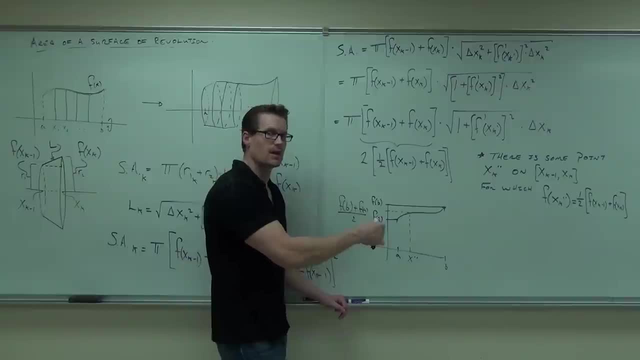 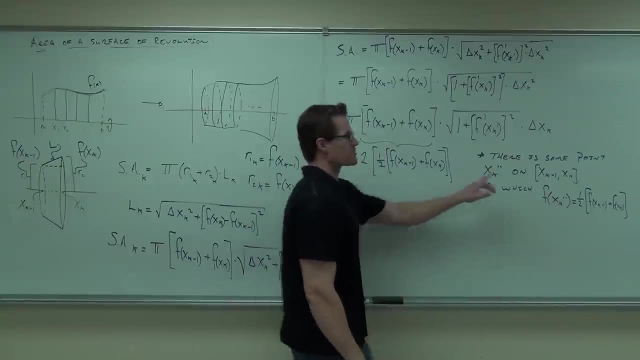 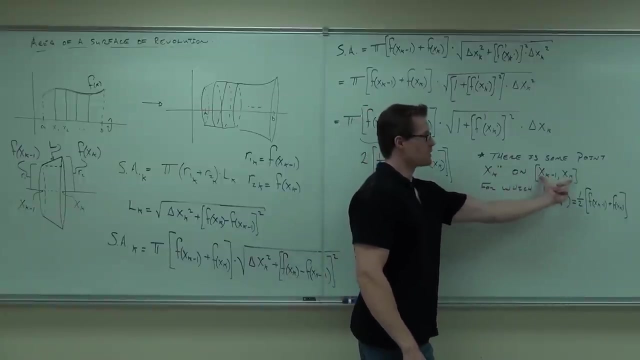 in that gives me average height. There's got to be a point that I can plug in that gives me average height. So that's what that says. It says that there's some point that I can plug in. It's between here and when I plug it in. 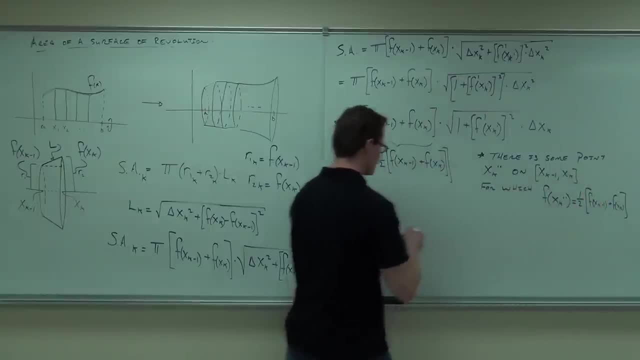 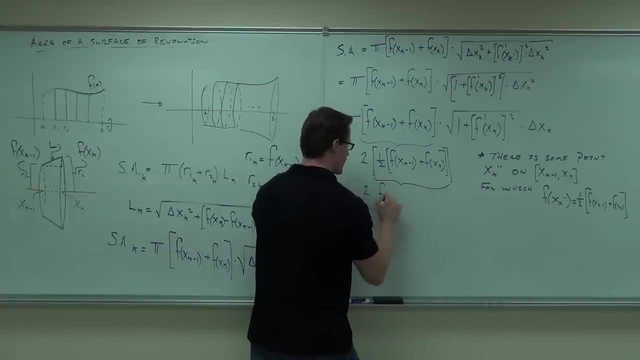 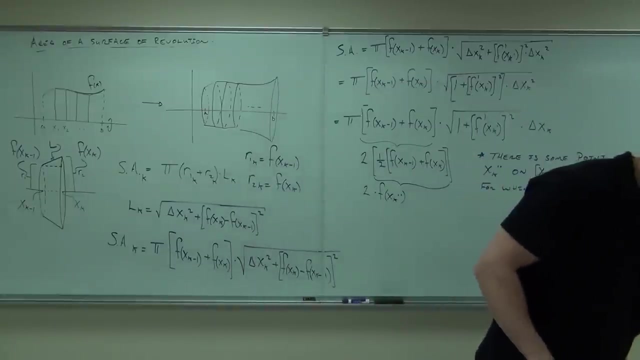 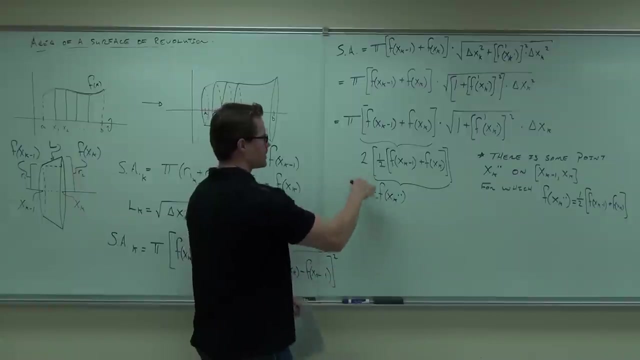 it gives me the average height. because F is continuous, It has to happen, So I'm going to let this become 2 times F of X K dot dot. So let's see, We're almost done. We have now a 2, a pi, a 2, F of X K dot dot. 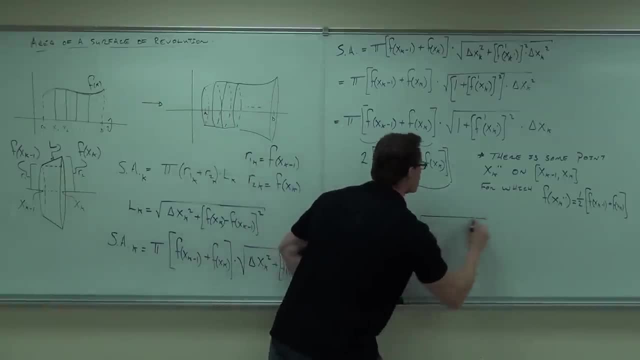 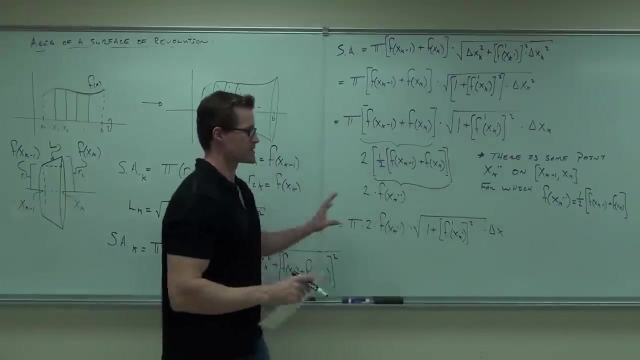 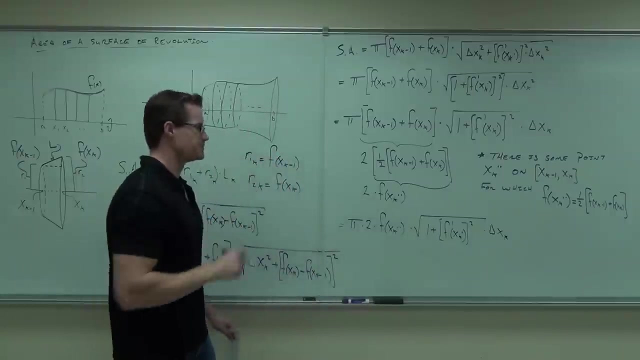 That's all this times. we already had the length. That's all this times. delta X, delta X is now outside of our square root. Remember, we took the square root of the delta X K dot, Delta X K square, So pretty close to done. 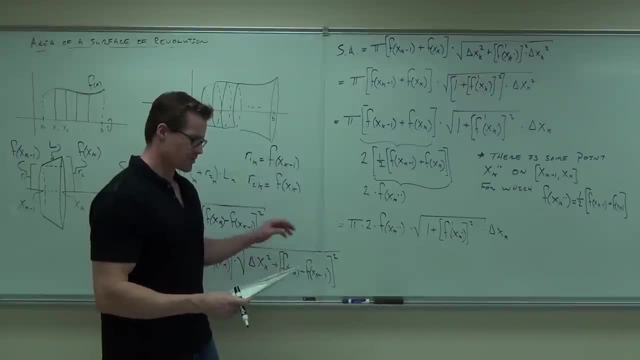 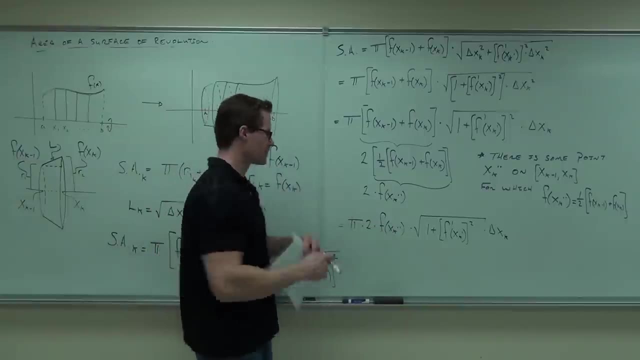 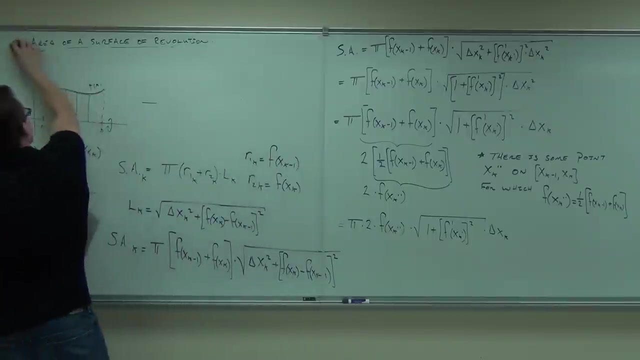 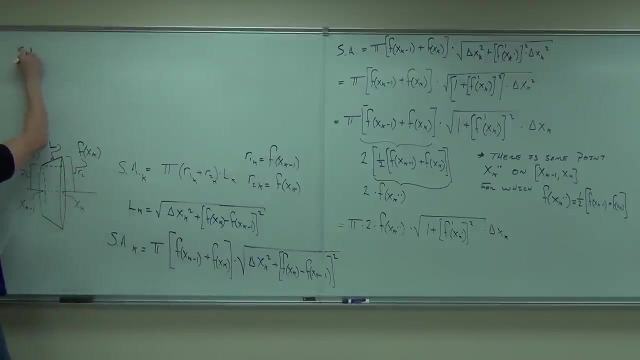 We'll make this a little bit prettier here. Notice that this is just the approximation for one of them, just for the Kth frustum. Now, in order to get all of them, we're going to add them together. So this is one of them. 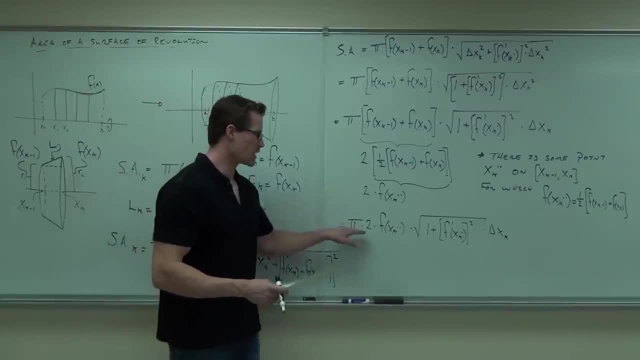 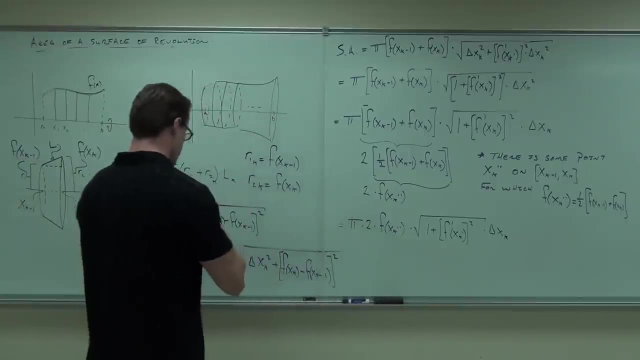 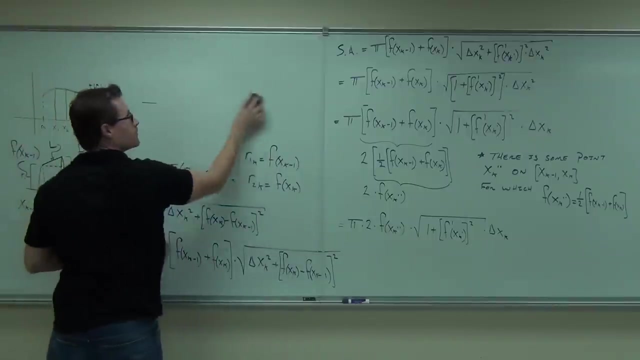 We'll make this a little bit prettier here. Notice that this is just the approximation for one of them, just for the k-th frustrum. Now, in order to get all of them, we're going to add them together. 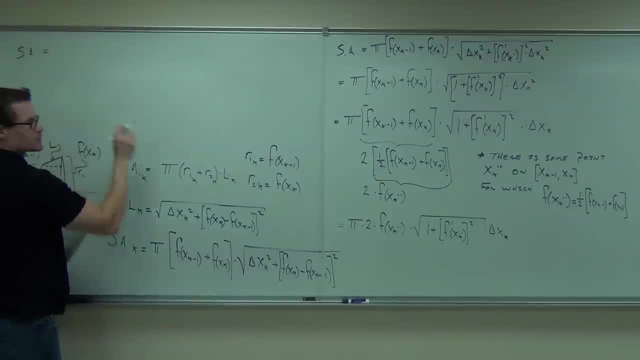 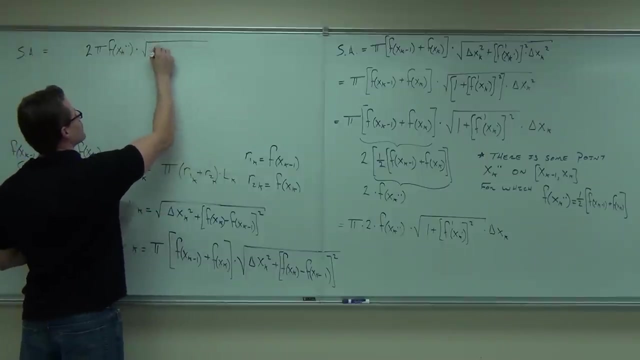 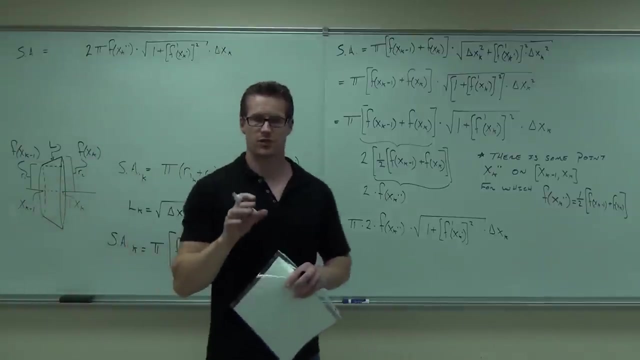 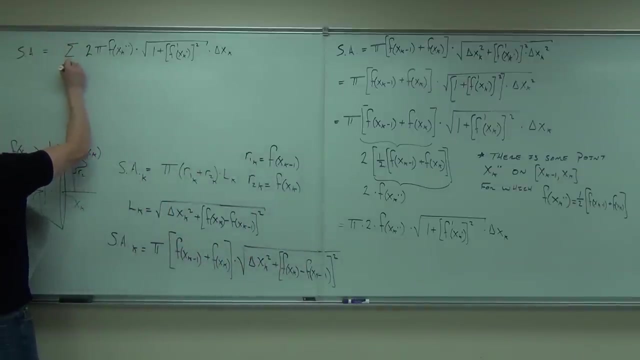 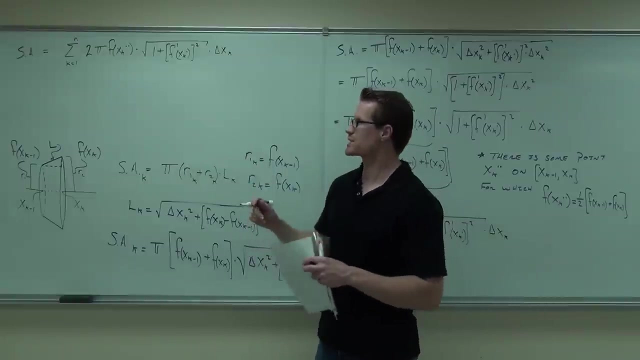 So this was one of them. That's one individual frustum. We're going to find all of them added together. Add them all up Now. that's an approximation. right now, To make it exact, we want to say no, no, no, no. 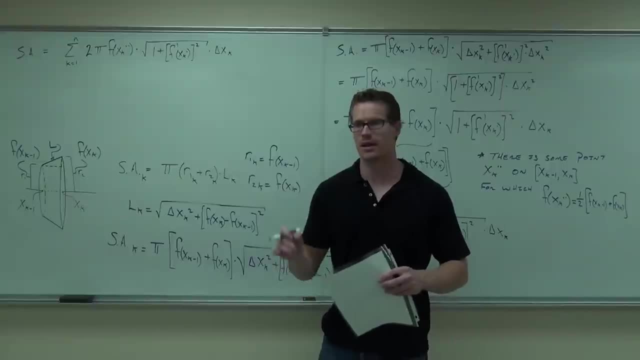 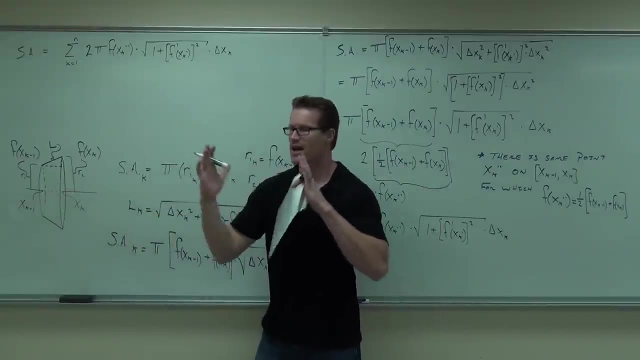 There's not just a finite number n, There's an infinite number, an infinite number of these frustra. That means that all of those xk minus 1xk is going to get smashed together. Everything is going to get super, super, super super close. 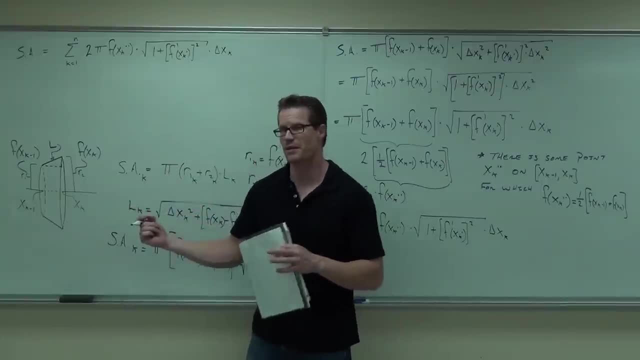 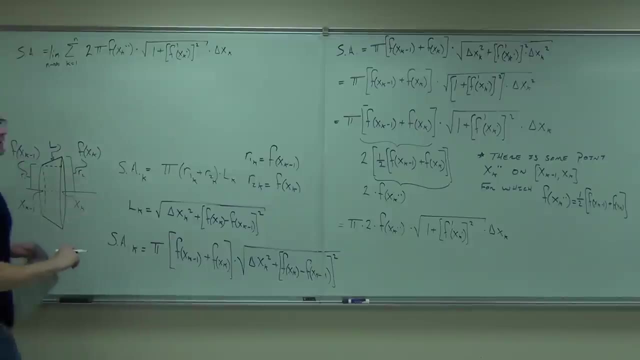 So it's not going to make a difference that we chose arbitrary points within there. It's not If we take a limit, as n goes to infinity. right now we see an integral. We say that a surface area equals. this becomes an integral from where you start to where you stop. 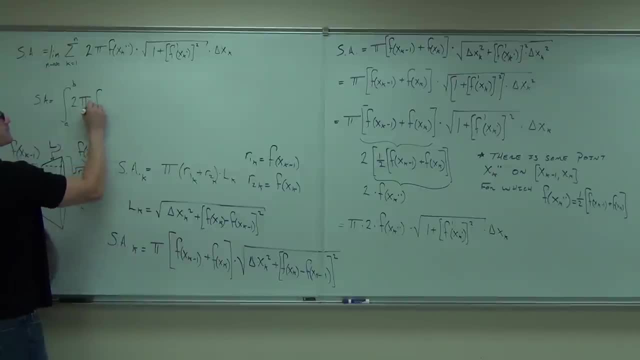 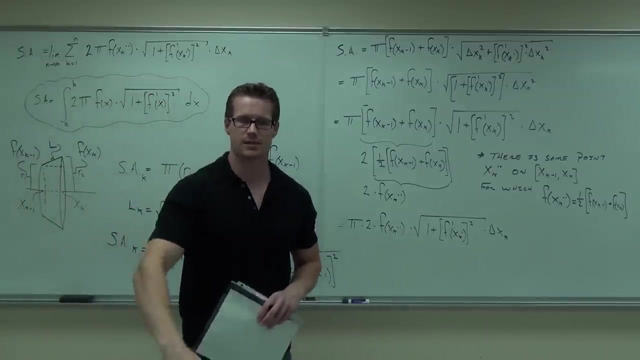 2 pi constant f of xk. double dot f of x times square root, 1 plus f. prime of x, Square Delta, x, dx. This is how you find the surface area of revolution about the x axis. Notice about the x in terms of x. 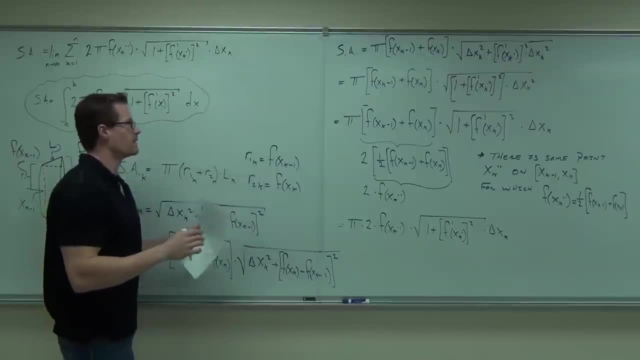 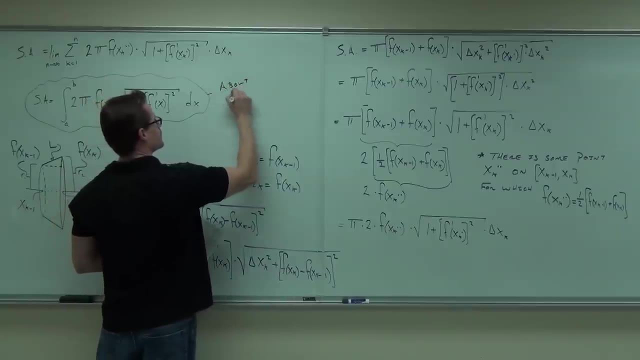 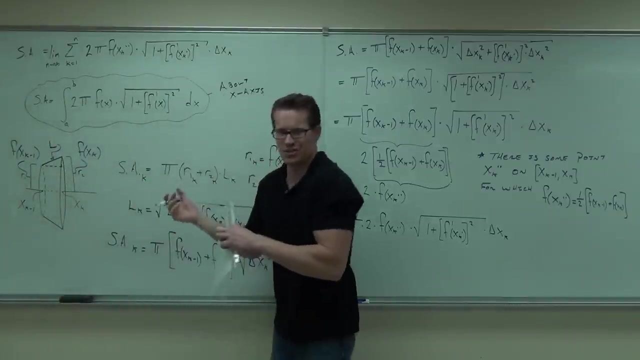 Just like the disk and washer, Just like that, Just like the length of a curve, xx. Notice, it's exactly what we started with, right. It's just. I mean, can you see it? Can you see what it's doing? 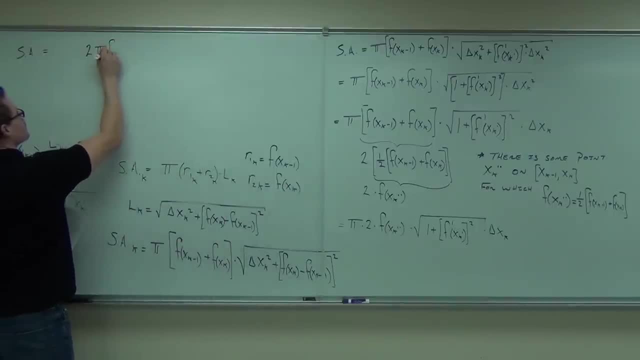 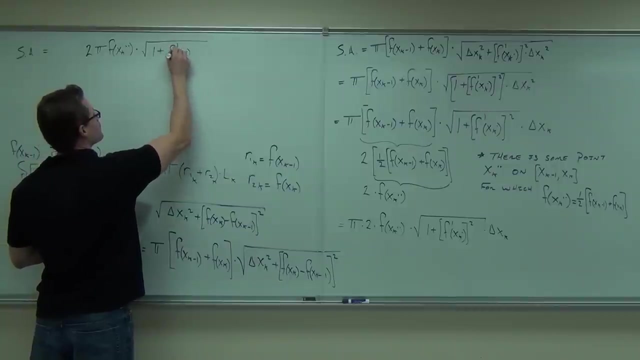 We're going to just divide them together. We are going to be going through the same sequence. So this is our 4, 3, 4, 4, 1, 2, 3, 4, 3, 4, so these are our стало. 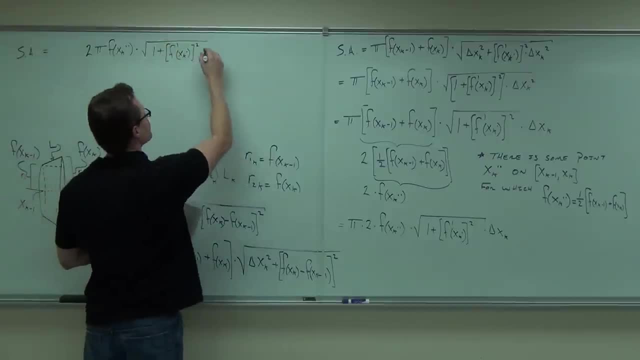 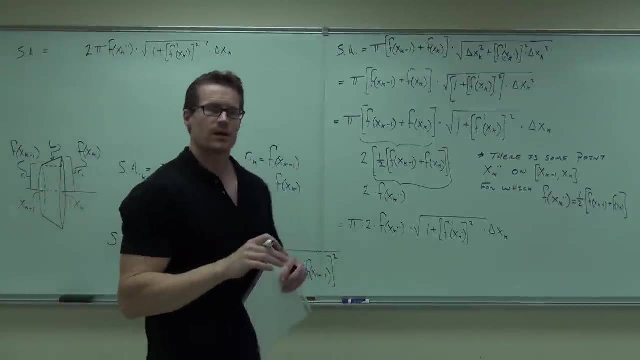 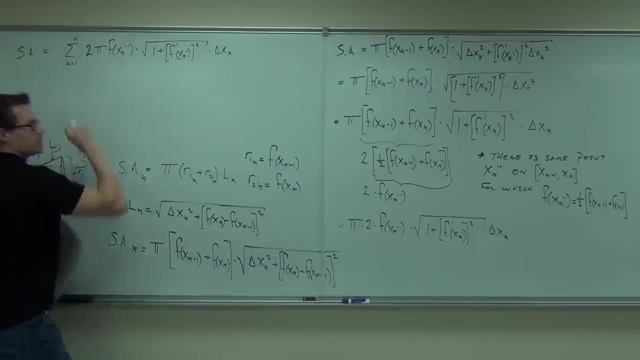 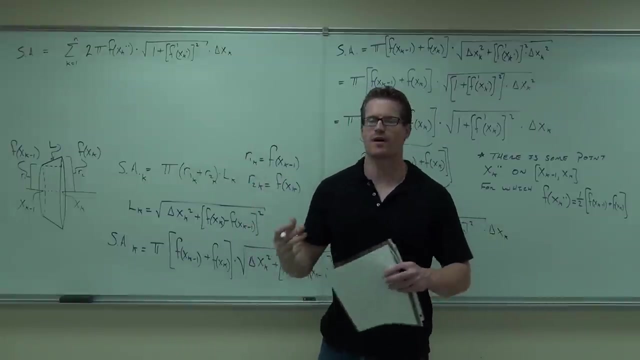 our plus, our minus and our minus. So who are they? OK, That's one individual. frustra To find all of them added together. add them all up. that's an approximation. right now, To make it exact, we want to say no, no, no. there's not just a finite number, n, there's. 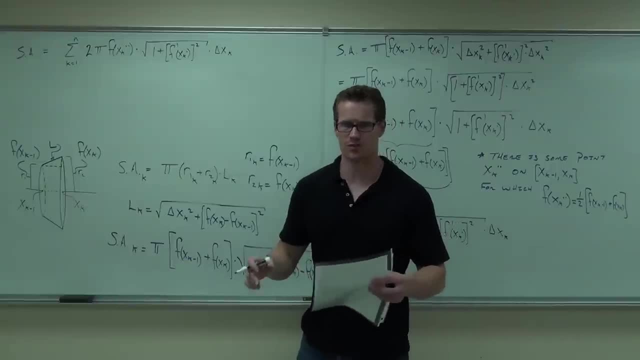 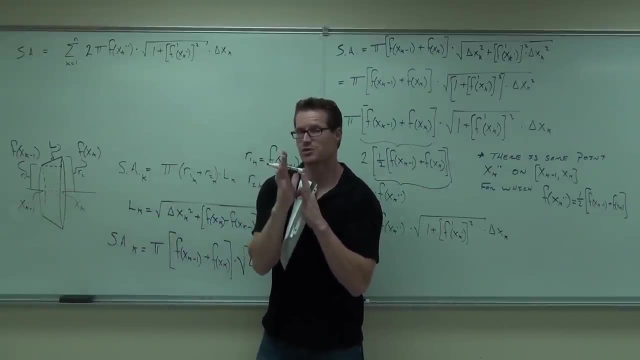 an infinite number, an infinite number of these frustra. That means that all of those xk minus 1xk is going to get smashed together. Everything is going to get super, super, super, super close. So it's not going to make a difference that we chose arbitrary points within there. 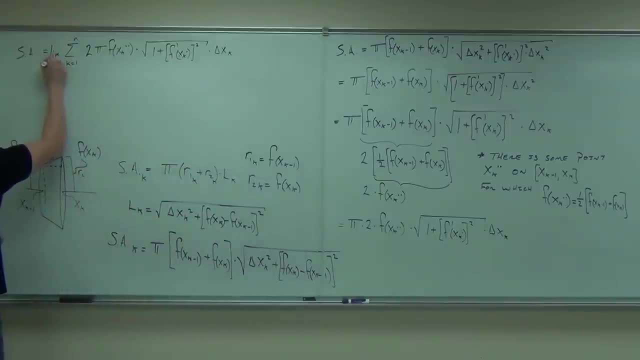 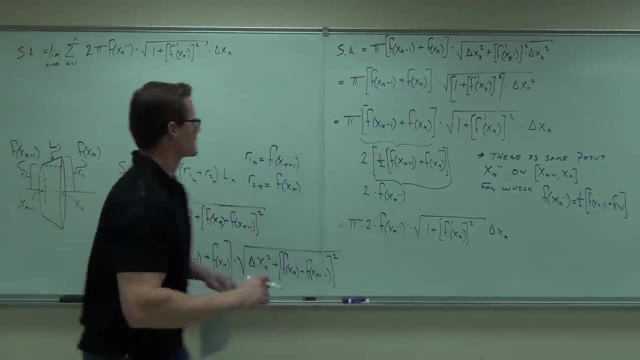 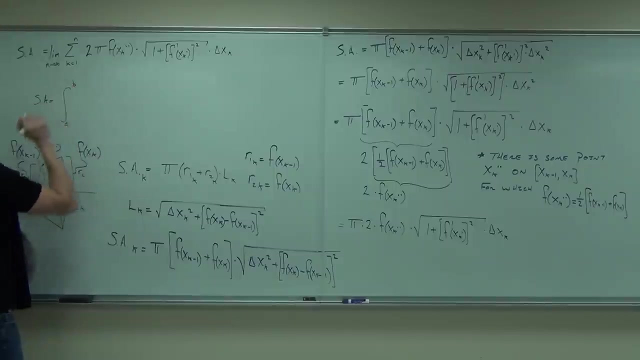 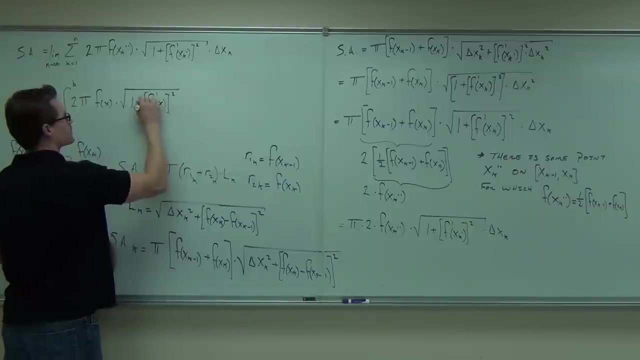 It's not If we take a limit, as n goes to infinity. right now we see an integral. We say that the surface area equals. this becomes an integral from where you start to where you stop. Two pi, Pi constant f of xk, double dot f of x times square root 1 plus f prime of x squared. 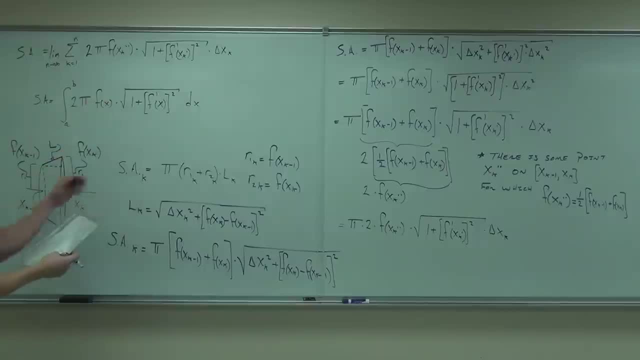 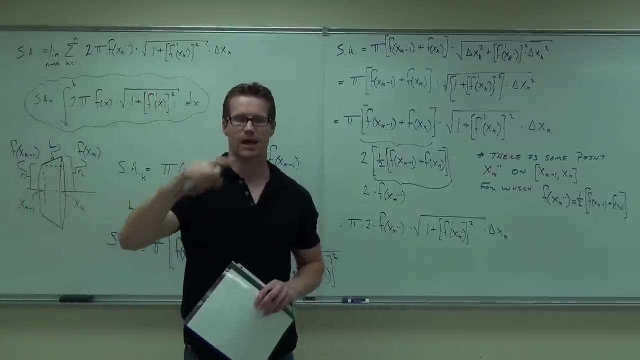 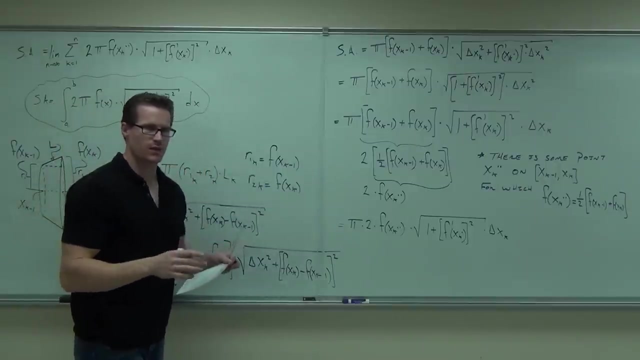 delta, x, dx. This is how you find the surface area of revolution, about the x axis. Notice about the x in terms of x. Just like the disk and washer, Just like that, Just like the length of a curve: x, x. 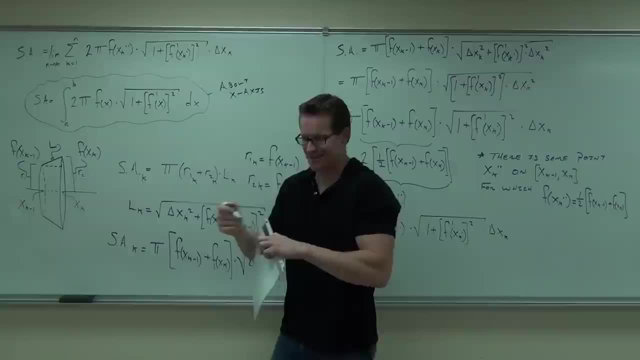 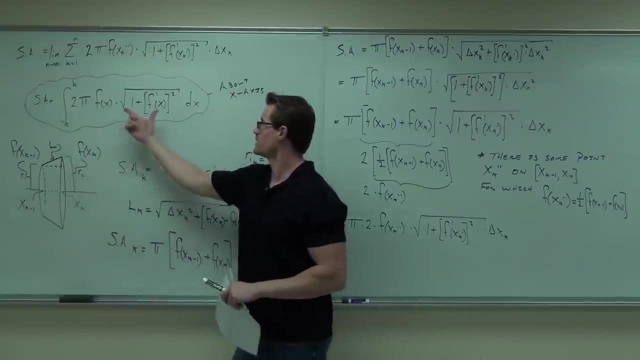 Notice, that's exactly what we started with, right. It's just, I mean, can you see it? Can you see what it's doing? It's saying circumference, just like we started with today, Circumference times the length. We knew this from intuitively, just from before. 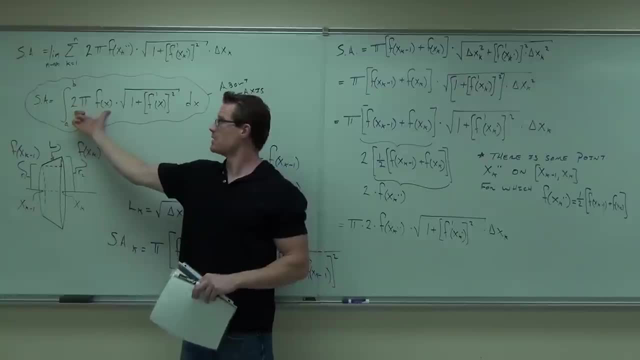 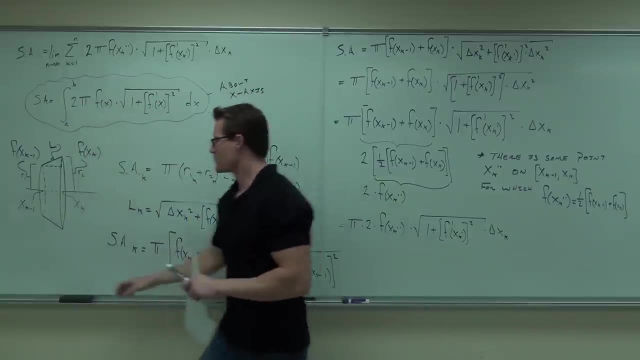 It's saying circumference, Just like we started with today, Circumference times the length. We knew this from intuitively, just from before. That's the length. If we want to do it on the y axis, formulas are going to be very similar. 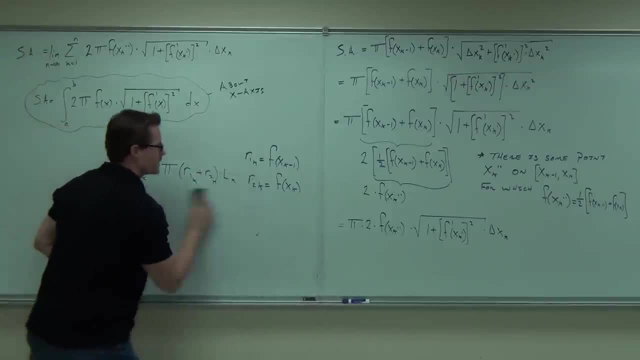 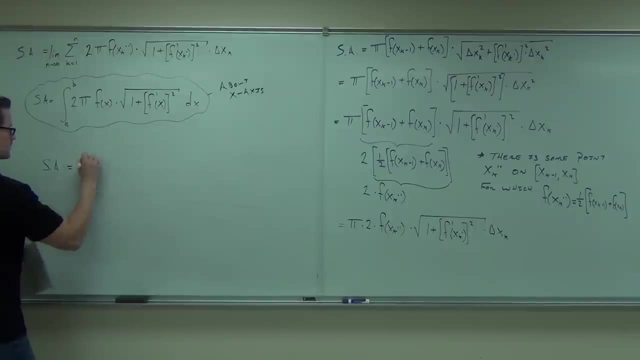 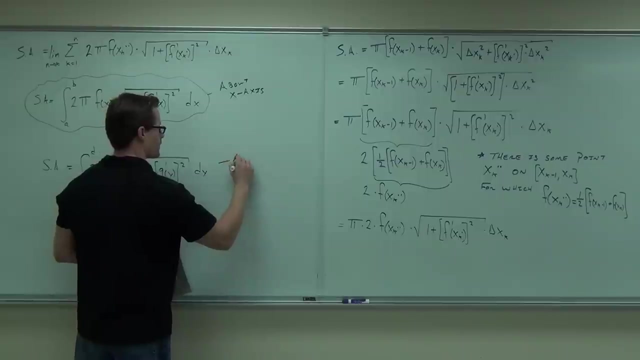 Only it's going to be in terms of y, So let me write that out for you, and then I'll be done. The. 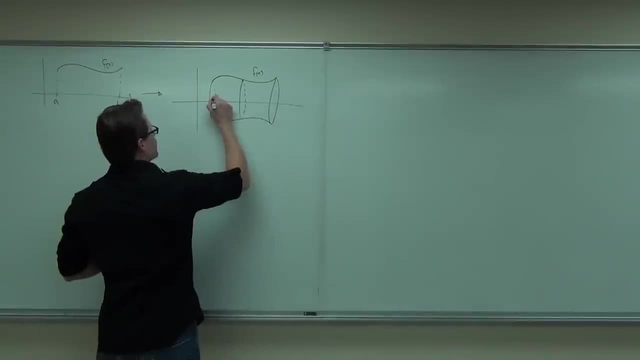 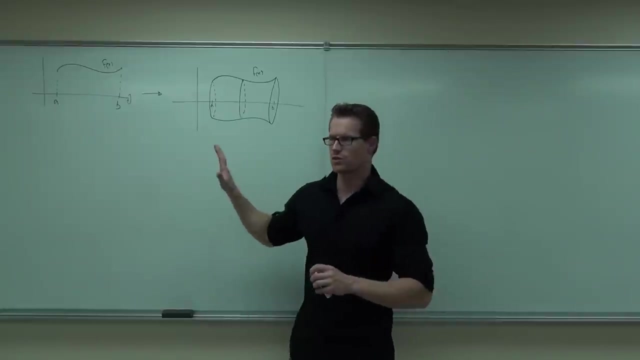 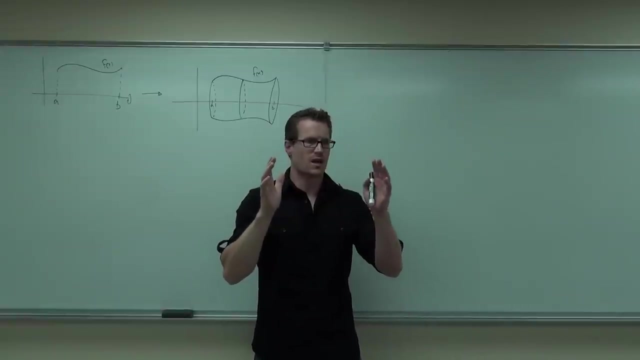 Via, And here's how we're going to think of it. If the cross-section of this figure is a circle and we can find the circumference of a circle, then what the surface area of a three-dimensional object is is basically the circumferences of an infinite number. 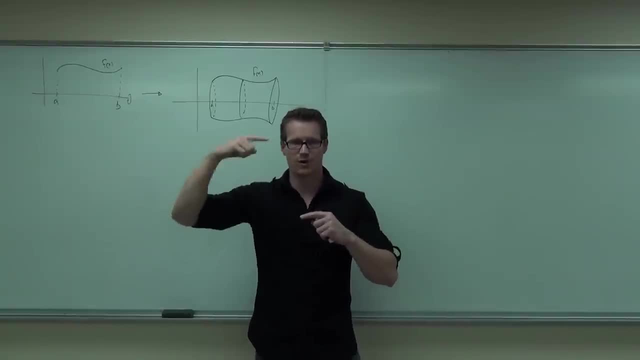 of circles added together, Or in other words the circumference times the length. That basically gives you surface area of like a cylinder. If you took the circumference times the length, would you not get a surface area of a cylinder? without the ends Right, You get the surface area. 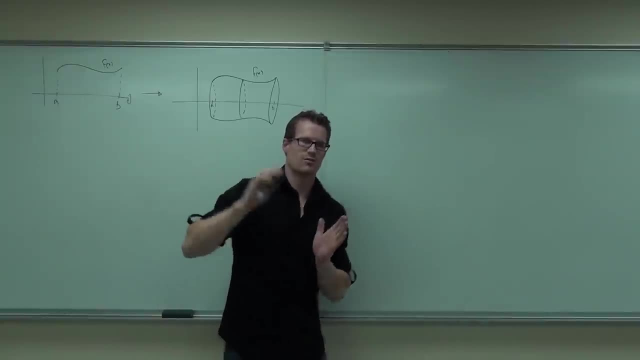 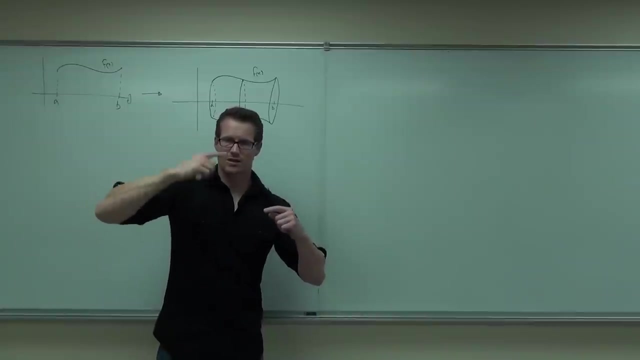 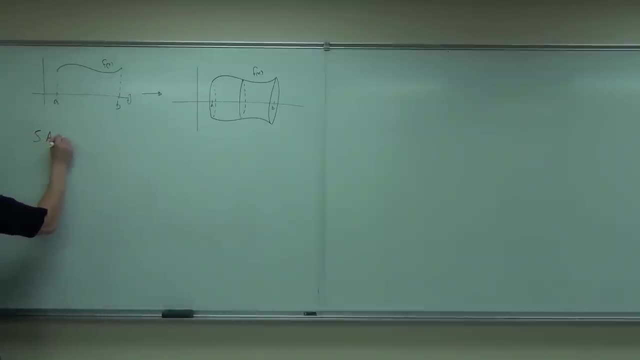 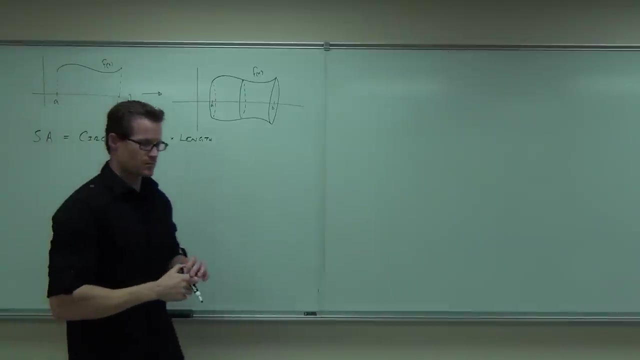 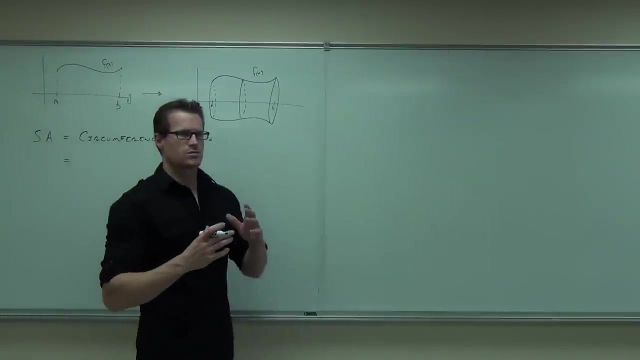 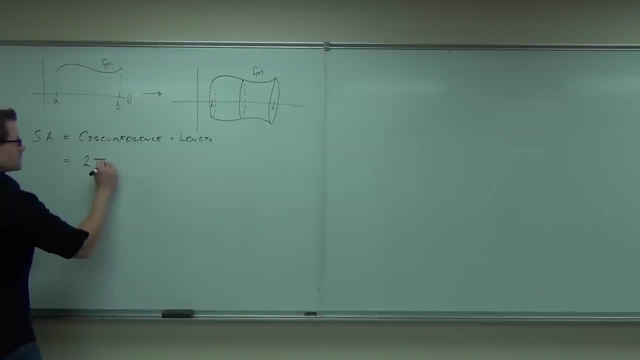 So idea is: surface area is circumference times length. So in other words, circumference of something is 2 pi times whatever the radius happens to be. so circumference, that's pretty easy. That's 2 pi r, The length I'm going to leave. 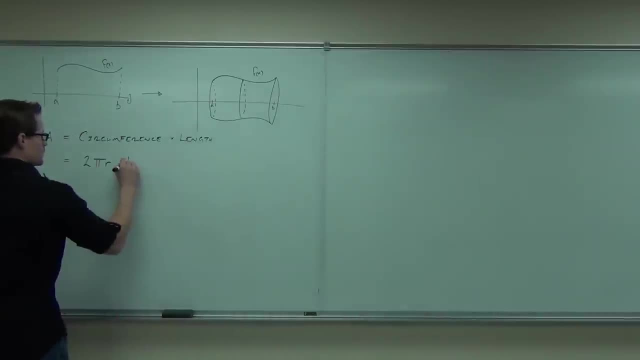 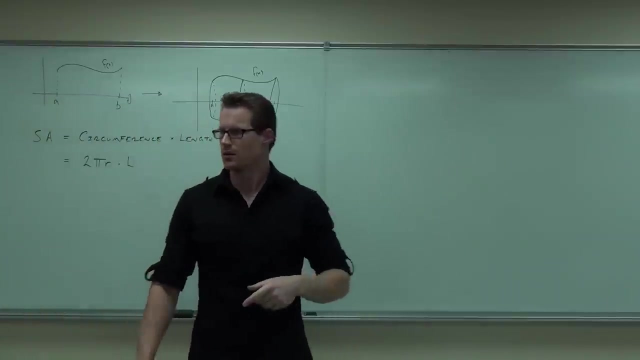 that with a letter l for right now. Now could you tell me what's the r that we have for our figure? What's the radius there? Yeah, we've done this a couple times now. The radius is f of x, So instead of 2 pi r, if I'm dealing. 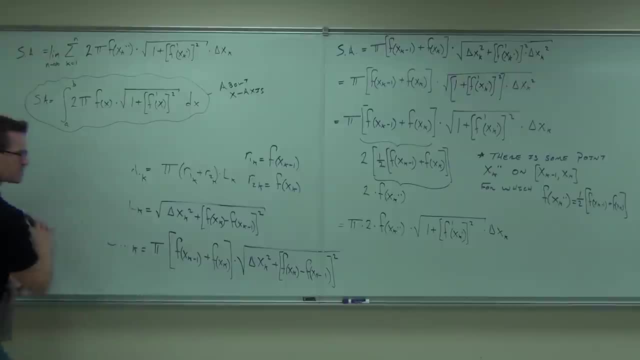 That's the length. If you want to do it on the y-axis, formulas will be very similar, Only it's going to be in terms of y. Let me write that up for you then, and I'll be done. Contact on the souped surface. 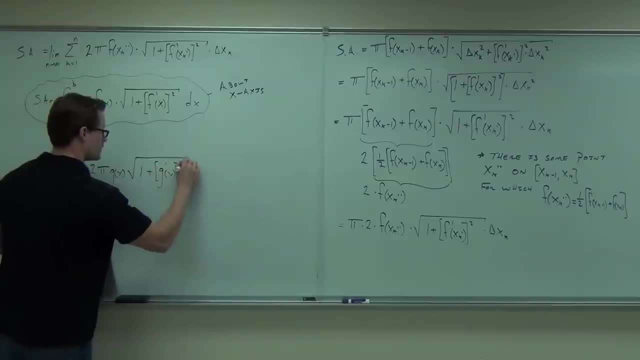 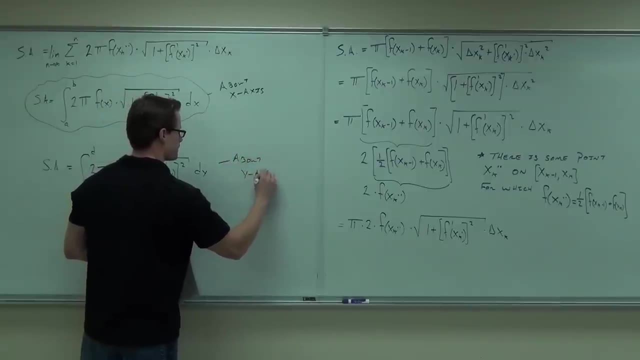 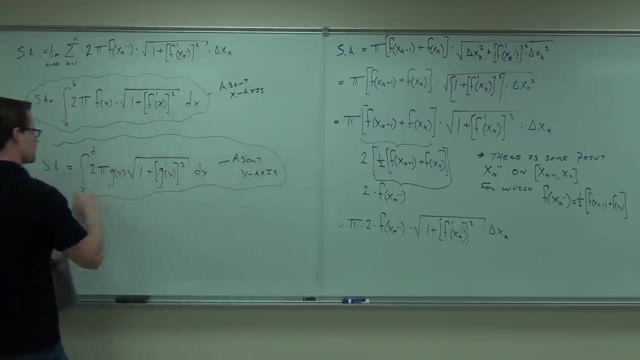 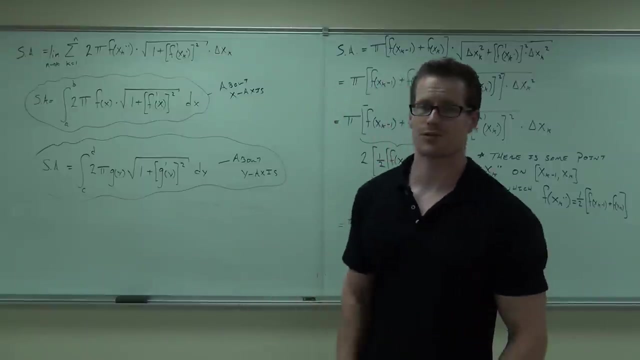 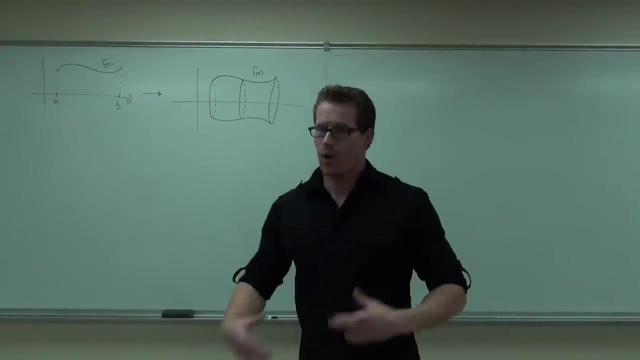 There we are Alright. Alright Out, Drop República. That's the whole idea. hopefully, you got it Alright. so last time we talked about what we're going to do right now. We're going to take this curve and we're going to revolve it around an axis, but we're not. 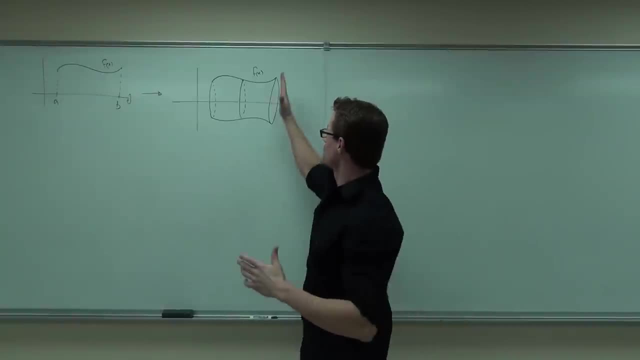 going to look for the volume. we're going to look for the surface area. Again, we're not counting the ends, those are just a basic geometry problem. We're not going to count the surface area of the circle or the circle. you can do that. 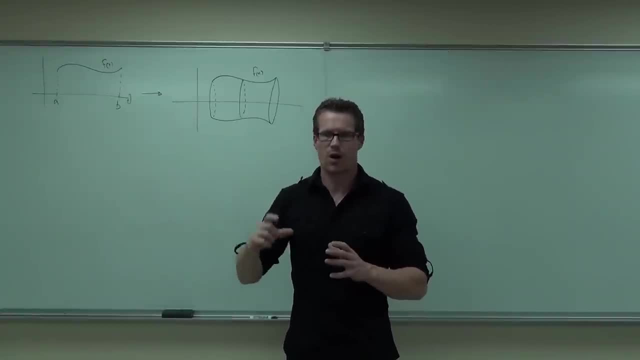 just with the geometry. Take pi r squared, r would be your f of x at that point, at b and at a, and that's pretty much it. So we're really worried about the surface area of the revolving figure. Do you understand the idea here? 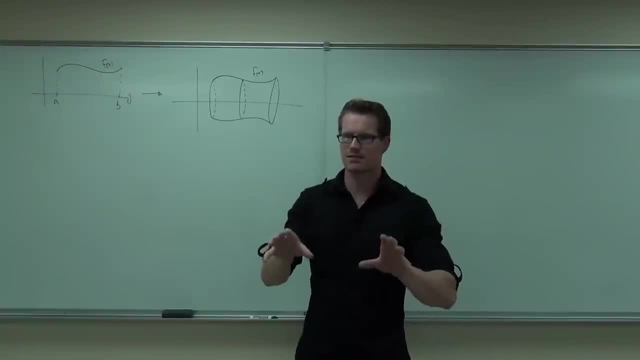 Now again, I'll mention this: the previous sections. you guys have not had that. So if you want the full explanation, rewind the video and go back to the previous section. Okay, Go back to the video. go watch the video. that's the full explanation. 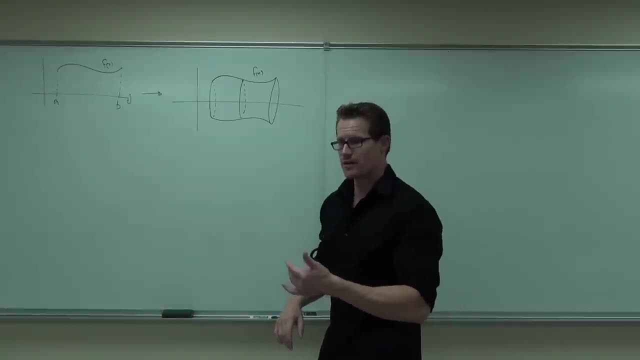 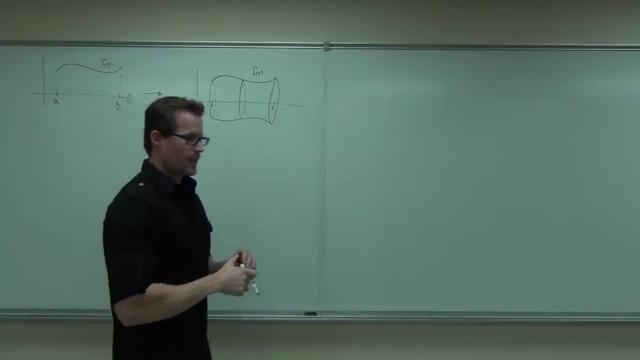 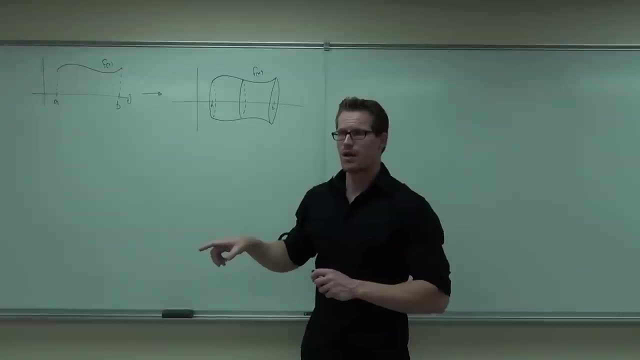 What I'm giving you is a very simplified version of that, And here's how we're going to think of it. If the cross section of this figure is a circle and we can find the circumference of a circle, then what the surface area of a three dimensional object is is basically the circumferences. 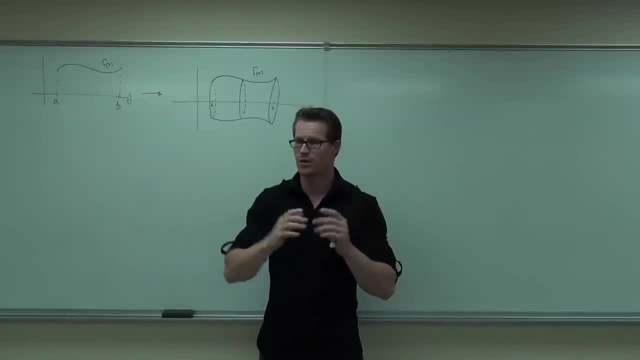 of an infinite number of circles added together, Or in other words the circumference. The circumference times the length, That basically gives you surface area of like a cylinder. If you took the circumference times the length, would you not get a surface area of a cylinder? 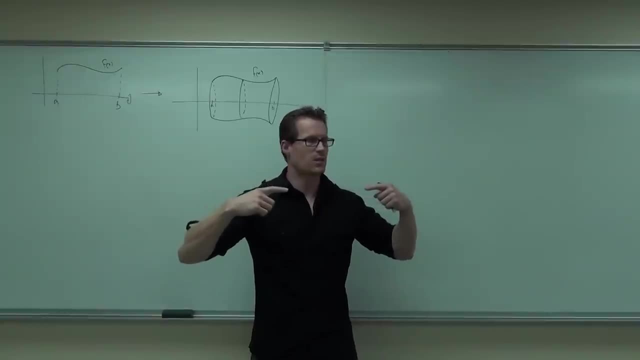 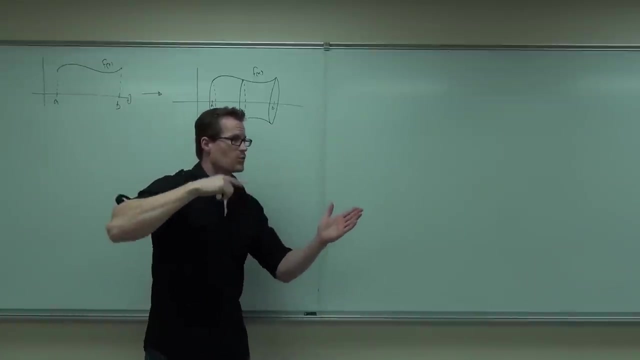 without the ends, You get the surface area. Now we don't have a cylinder, but we have kind of a changing cylinder. We have something that goes like this: So that means, if we can integrate it little by little, take the surface area here and 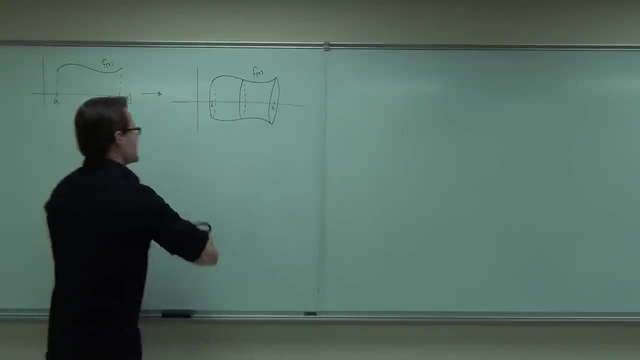 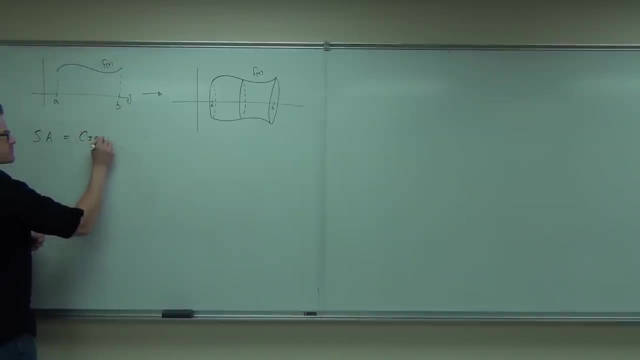 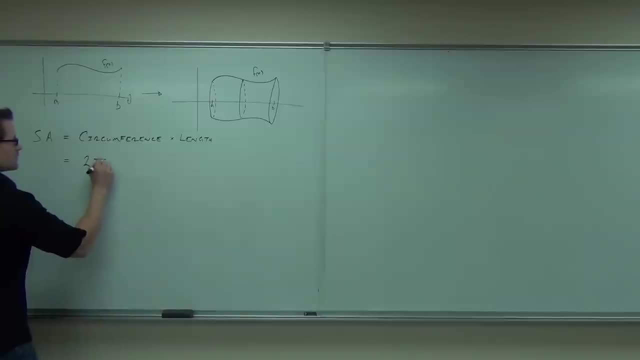 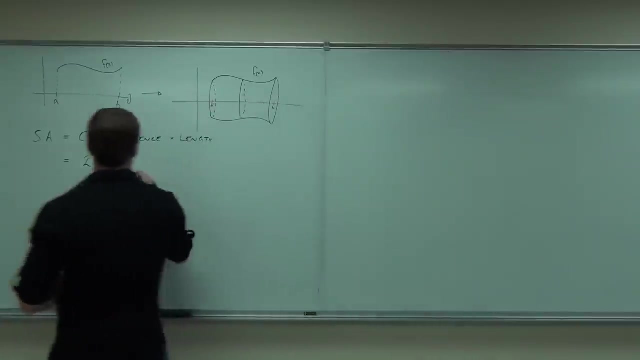 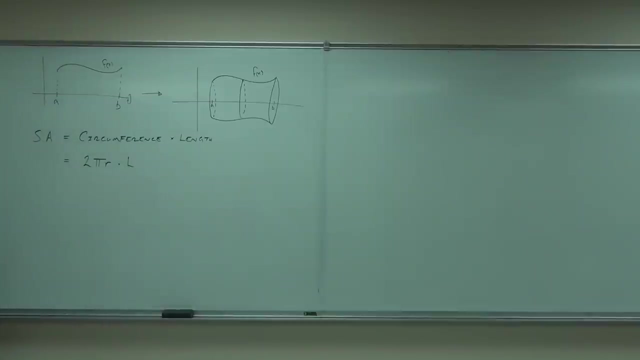 to be So circumference, that's pretty easy. That's 2 pi r, Okay, Okay. Okay, So the length. I'm going to leave that with a letter L for right now. Now, could you tell me what's the r that we have for our figure? 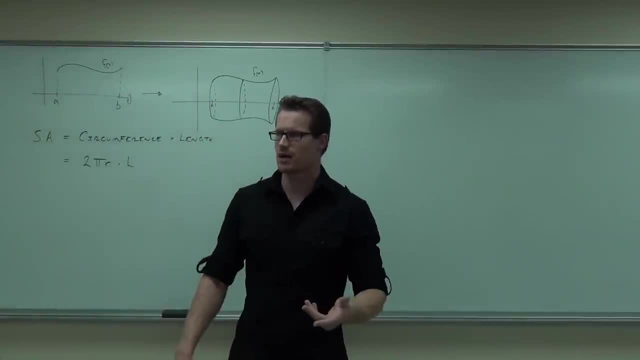 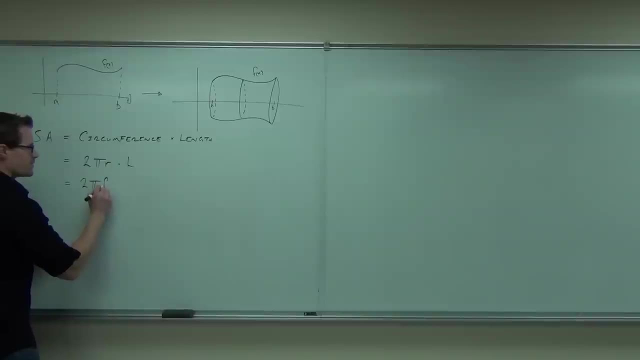 What's the radius there? Yeah, we've done this a couple times now. The radius is f of x. So instead of 2 pi r, if I'm dealing with my function, I'll have 2 pi times f of x. 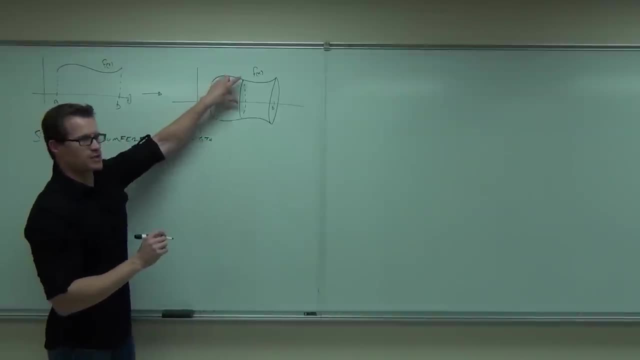 Well, for sure, Because the distance from here to here is 2 pi times f of x. Okay, So the radius from here to here, which is our radius, is also, for any value of x, the function at x. So the radius is the function at x. 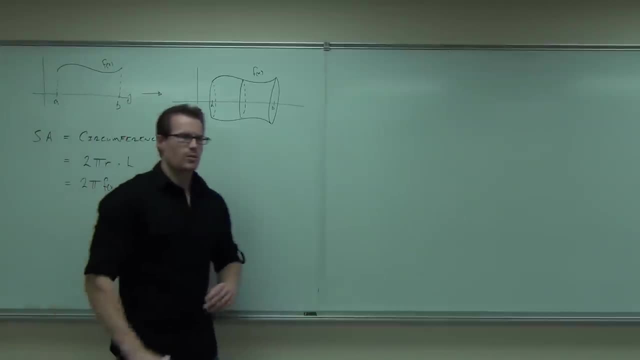 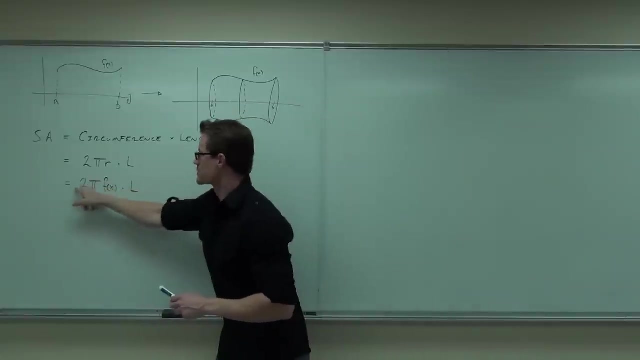 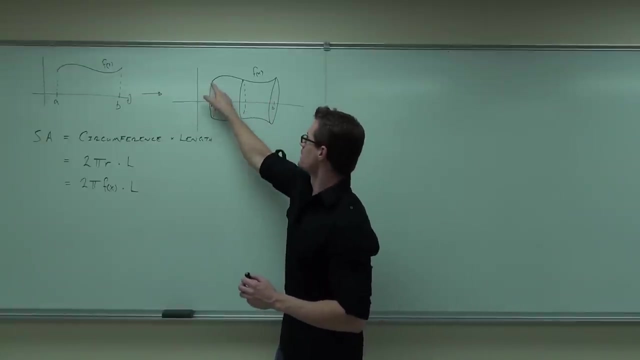 Now L Notice that what we're doing is we're taking the circumference at every point. That happens to be the circumference at every point, x times whatever the length is for the whole thing. Now, the length for the whole thing means what's the length of the function for the whole thing? 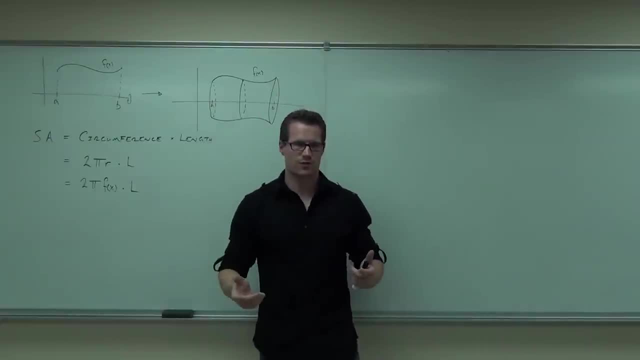 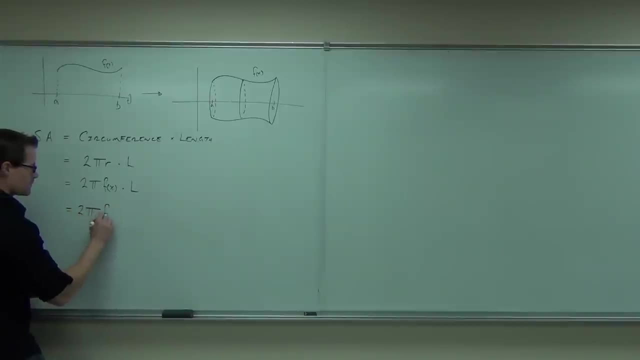 And that's something we just finished doing. In fact, if you looked over your first part of your homework, that's this. That's the square root. Remember the square root thing: One plus f, prime x, squared dx. Well, we're just having an idea right now. 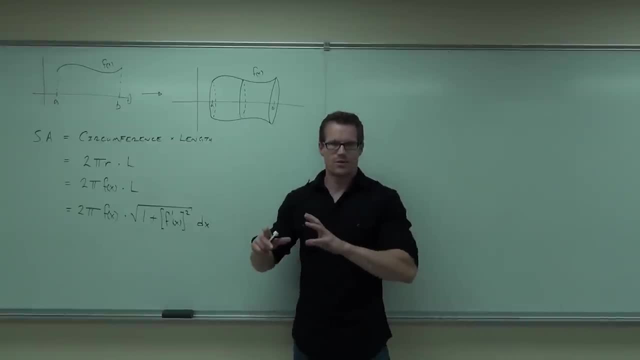 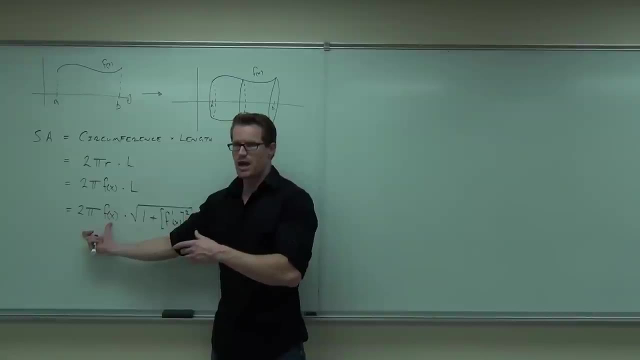 Do you think that's the answer? No, Okay, Do you feel okay with the idea of the circumference here, That is, circumference 2 pi r, where r is f of x. And do you feel okay with times, the length, Where that is the length? 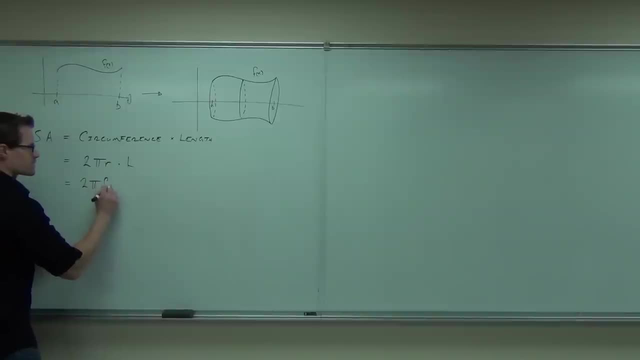 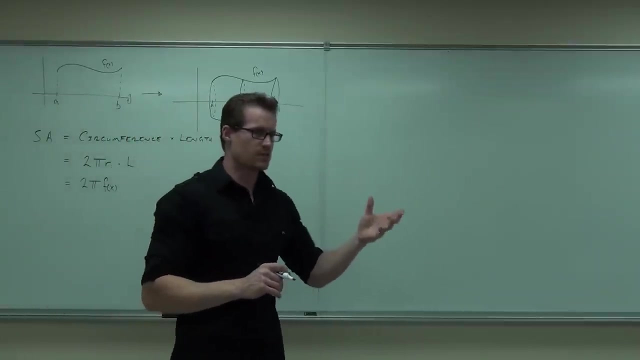 with my function I'll have 2 pi times f of x. Well, for sure, because the distance from here to here, which is our radius, is also, for any value of x, the function at x. So the radius is the function at x. Now l Notice that. 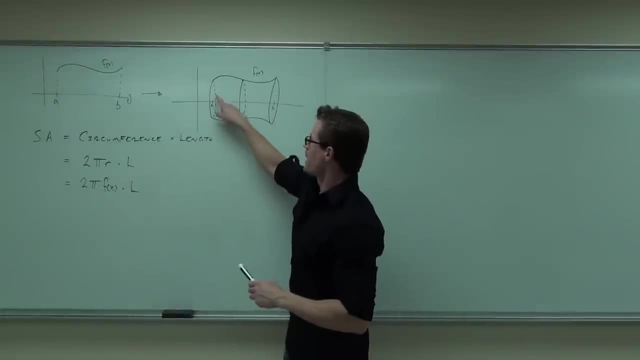 what we're doing is we're taking the circumference at every point. That happens to be the circumference at every point x times whatever the length is for the whole thing. Now, the length for the whole thing means: what's the length of the function for the whole thing? 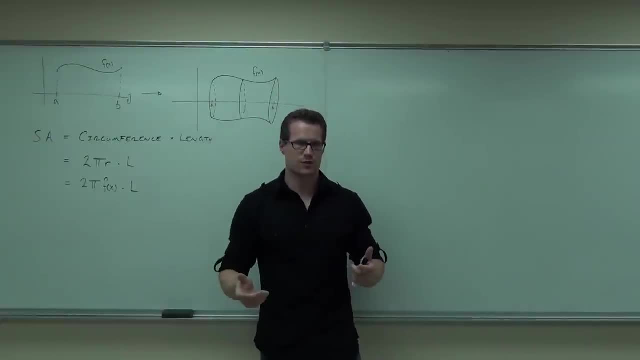 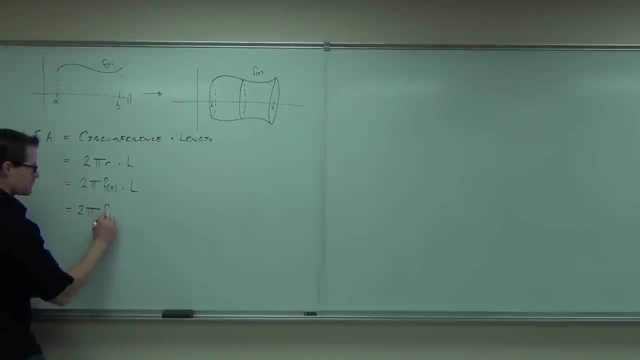 And that's something we just finished doing. In fact, if you looked over your first part of your homework, that's this. That's the square root. remember the square root thing: 1 plus f, prime x squared dx. Well, we're just having an idea right now. 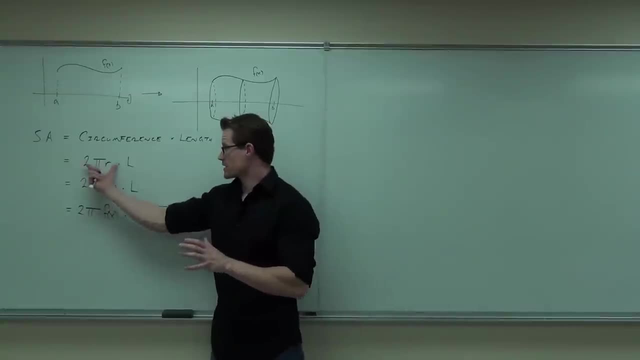 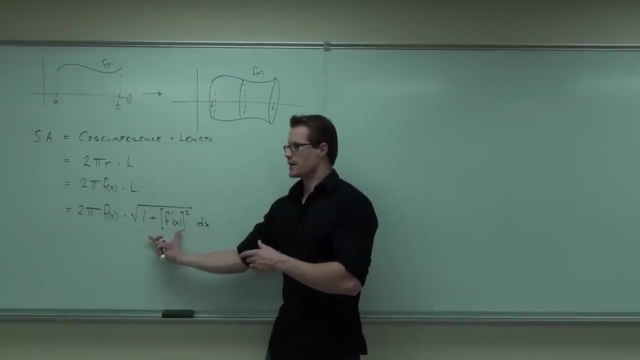 Do you feel okay with the idea of the circumference here, That is, circumference 2 pi r, where r is f of x. And do you feel okay with times, the length, where that is the length? Why can't you just use the bounds to find the length? 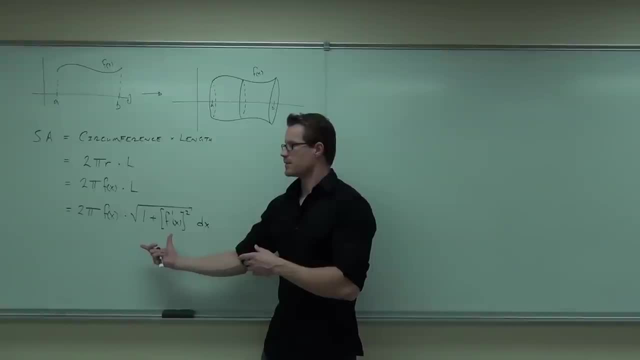 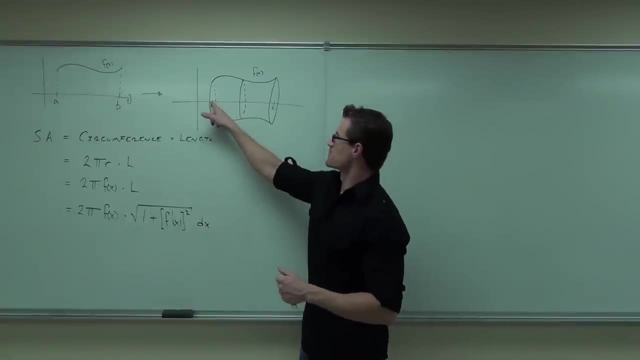 It's like I'm not sure if I see why you need the the length formula, Because that's a great question. His question, as I understand it, is: why can't you use just the difference or the distance from a to b? 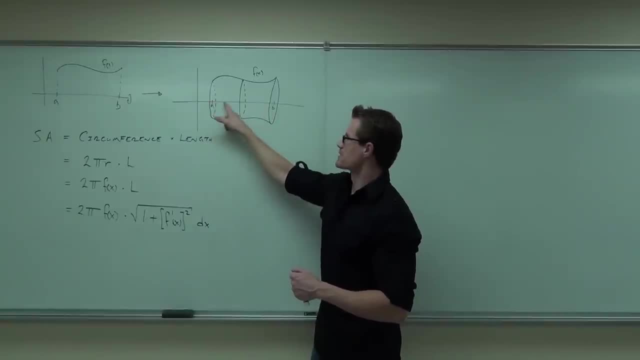 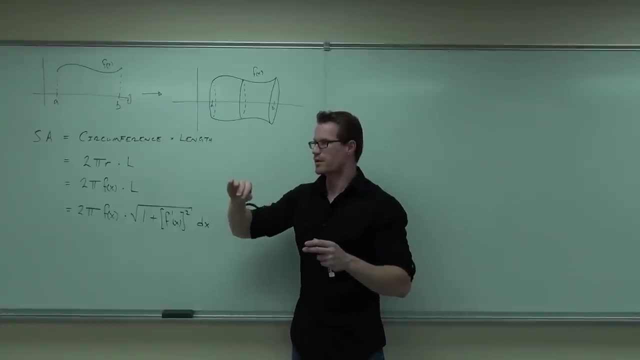 Why can't you just use that? Well, a straight line is the smallest distance between two points. Two points, correct? Is that a straight line? So this distance is not just b minus a. It's not that easy. This goes up, it goes down. it's longer than that. 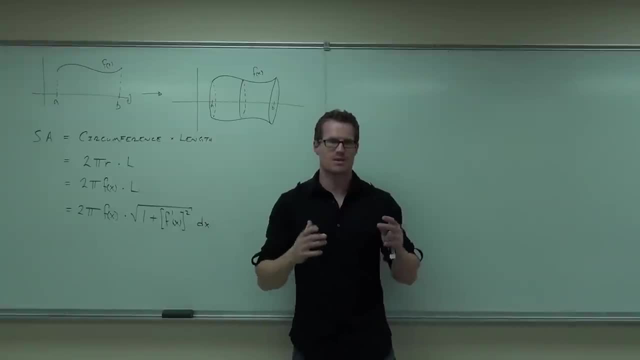 Does that make sense? So I can't use b minus a, because that would imply that I actually have a cylinder. I do not. I don't have a cylinder. Okay, what we have is a thing: It's longer than the cylinder would be. 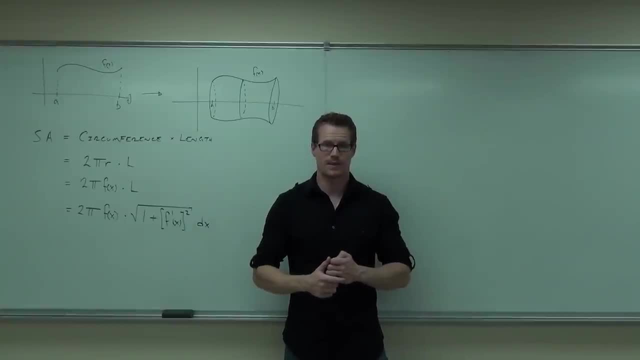 Yes, When we're adding to the circumference or multiplying the circumference, does that mean we're looking at the circumference, We're looking at the line of three-dimensional space? no, The circumference, Yeah. Yeah, this is definitely three-dimensional. 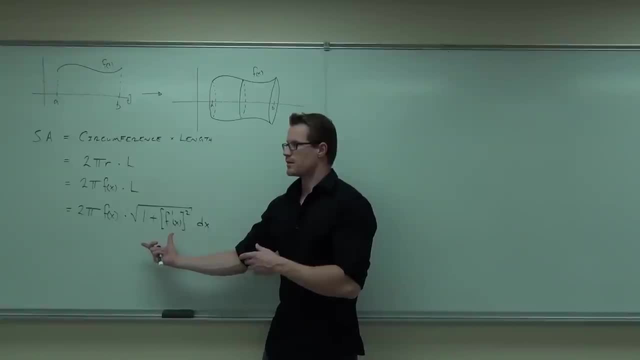 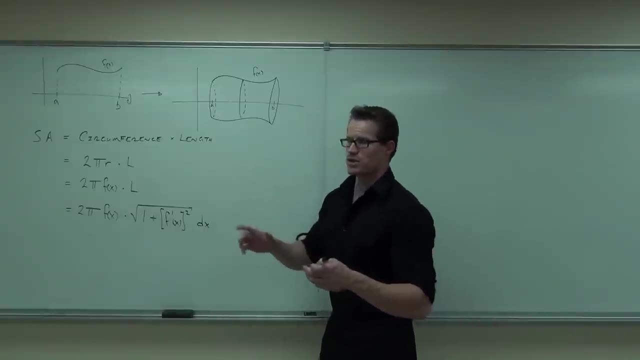 Why can't you just use the bounds to find the length? I'm not sure if I see why you need the length formula, Because that's a great question. His question, as I understand it, is: why can't you use just the distance from a to b? 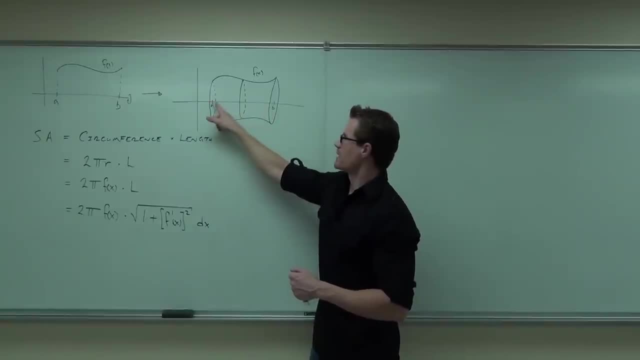 Why can't you just use that? Well, a straight line is the smallest distance between two points, correct, Is that a straight line? So this distance is not just b minus a. It's not that easy. This goes up, it goes down. it's longer than that. 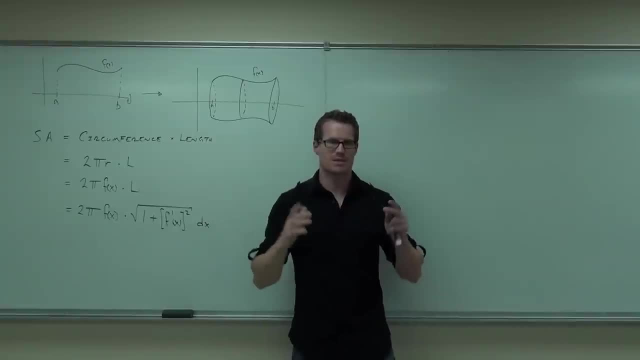 Does that make sense? So I can't use b minus a, because that would imply that I actually have a cylinder. I do not. I don't have a cylinder. Okay, What we have is a thing: It's longer than the cylinder would be. 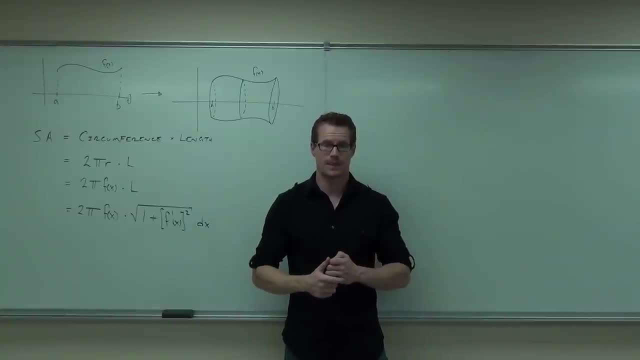 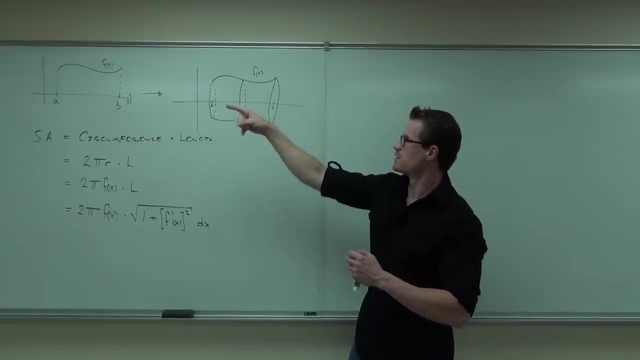 Yes, So if we're writing the circumference or multiplying the circumference, does that mean we're looking at the line in a three-dimensional space? now The circumference, Yeah Yeah, this is definitely three-dimensional. This is a three-dimensional figure. So the circumference is taking this, taking every cross-section and find the circumference. 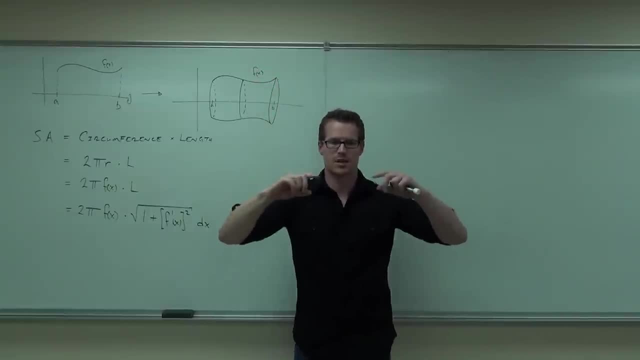 of that. Okay, So we're revolving around the x-axis. So it's saying: take a cross-section, okay, The cross-section is going to be a circle. It's very similar to volume, only we're not talking about the surface area. 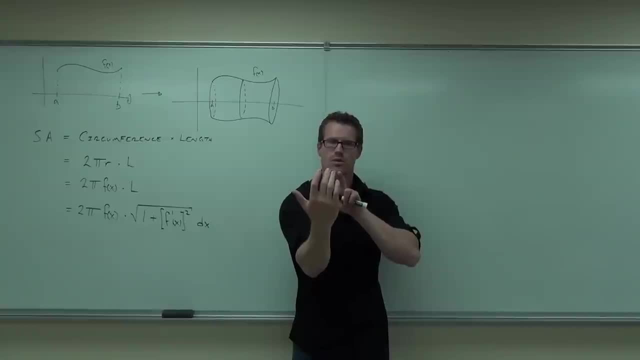 We're talking about the surface area of the cross-section, We're talking about the circumference of the cross-section right now. So you take the cross-section, find the circumference. It's 2 pi r, Integrate that across the length. So basically multiply by length and add them all up. 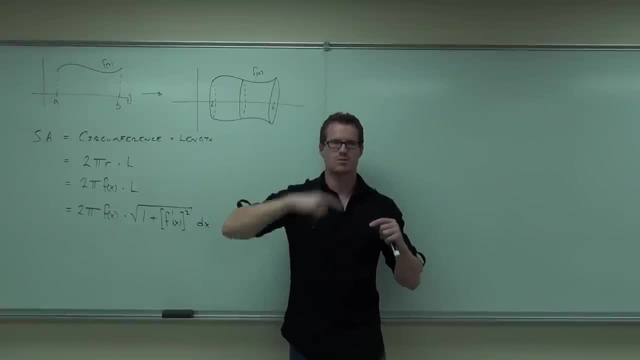 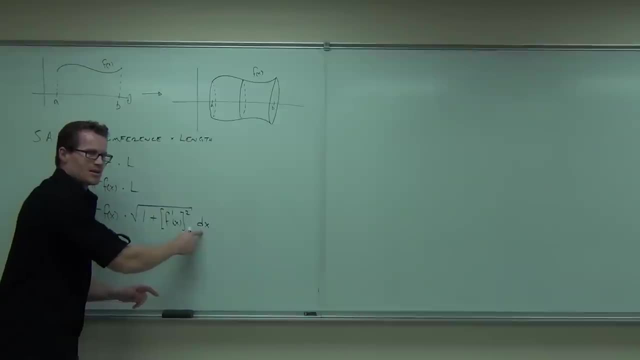 In order to get the dx, though reasonably, I can't just say dx. okay, Joe was right, I need to have an integral, So surface area, when I get it all said and done, is an integral from a to b of this. 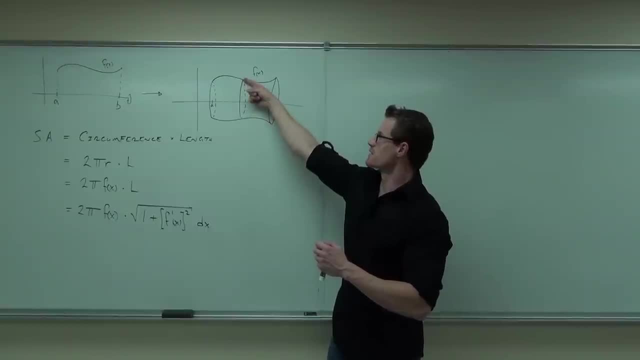 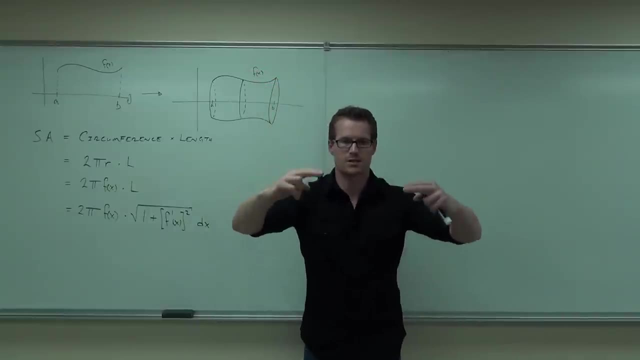 This is a three-dimensional figure. So the circumference is: taking this, taking every cross-section, and find the circumference of that, Okay, So we're revolving around the x-axis. So it's saying: take a cross-section, okay. 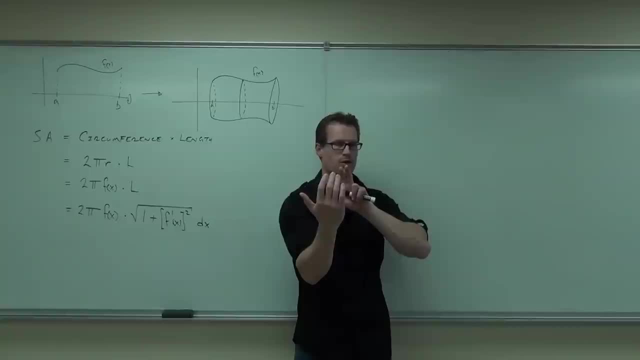 Find this. the cross-section is going to be a circle. It's very similar to volume, only we're not talking about the surface area. We're talking about the surface area of the cross-section, We're talking about the circumference. So we're talking about the circumference of the cross-section right now. 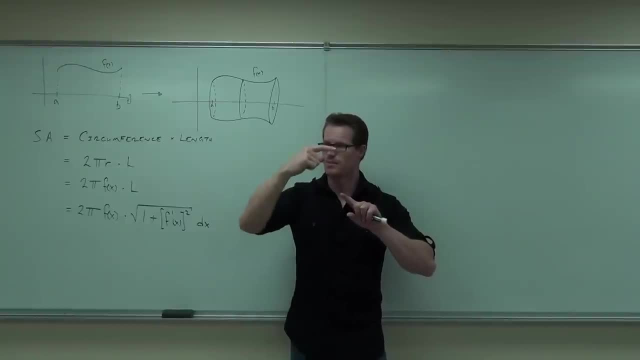 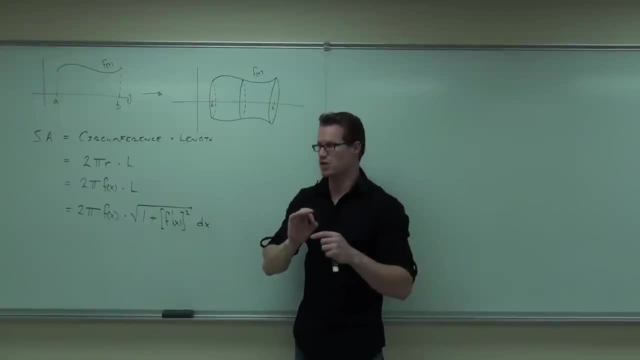 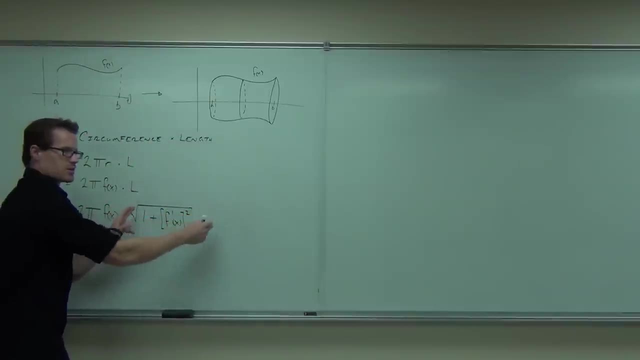 plus circumference, Again and again, repeated addition of circumferences that are actually changing. That requires an integral and a limit. So here's circumference times length, Here's circumference, Here's length, In order to get the dx though reasonably. 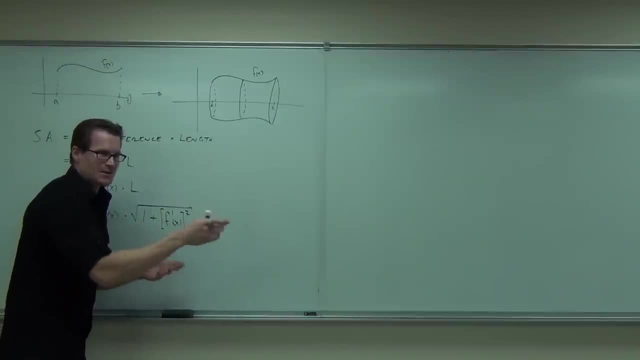 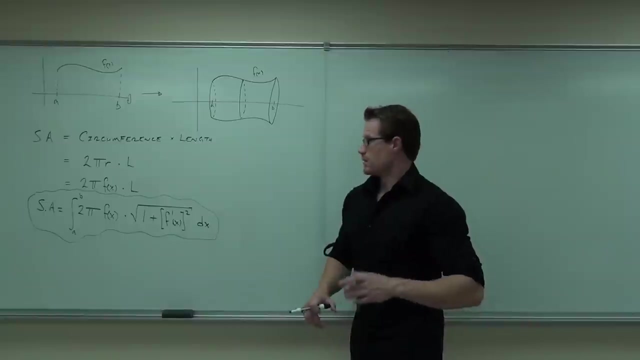 I can't just say dx, okay, He, Joe was right. I need to have an integral. So surface area, when I get it all said and done, is an integral from a to b of this. Now a question. 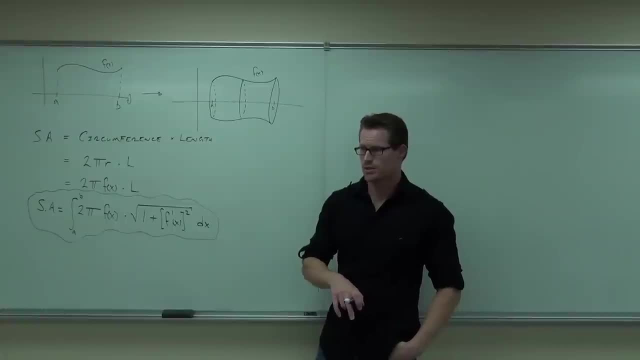 What axis did we just go around? 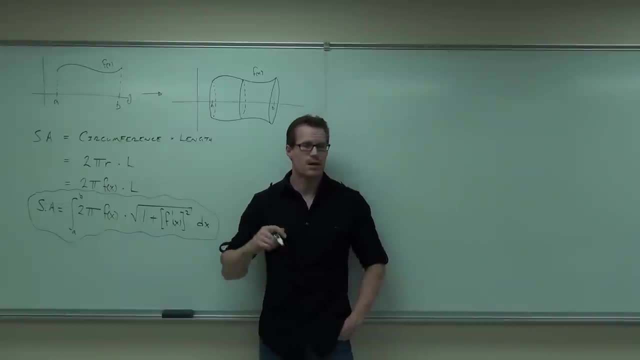 Most of our formulas are like that: If you go around x, you have it in terms of x. If you go around y, you have it in terms of y. 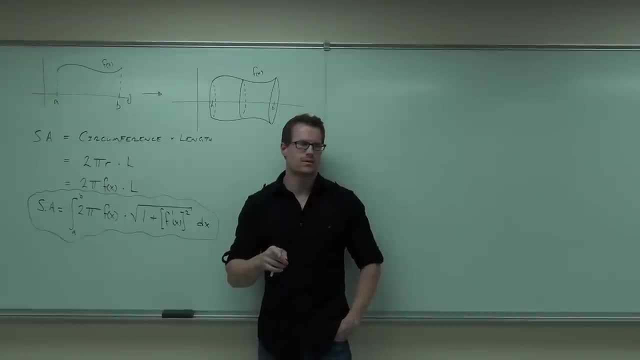 What's the only one that's not like that? The shells, the cylindrical shells, is the only one that's not like that, So that's the one to watch out for. So if I say, buy cylindrical shells, if you're going around the x, it's in terms of y. 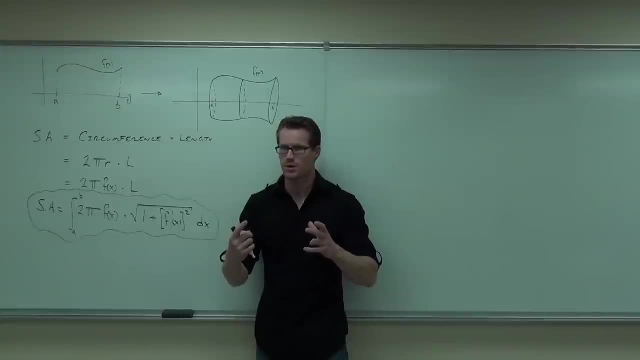 If you're going around the y, it's in terms of x. Those are the different ones, okay. Everything else is basically: you're going around the x, you want x's. You're going around the y, you want y's. 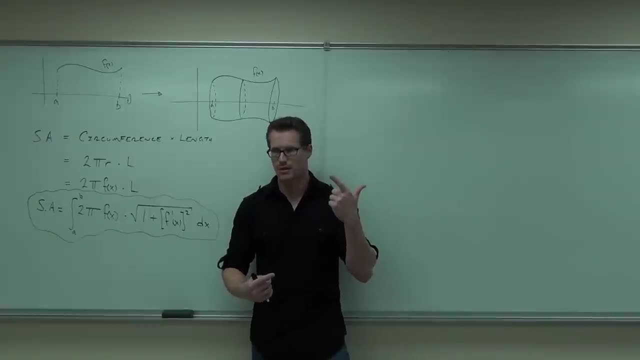 Discs and washer works like that. Area between two curves works like that. This length of a curve- that doesn't matter, But this works like that. The surface area revolution works like that. The only one that doesn't is the cylindrical shells. 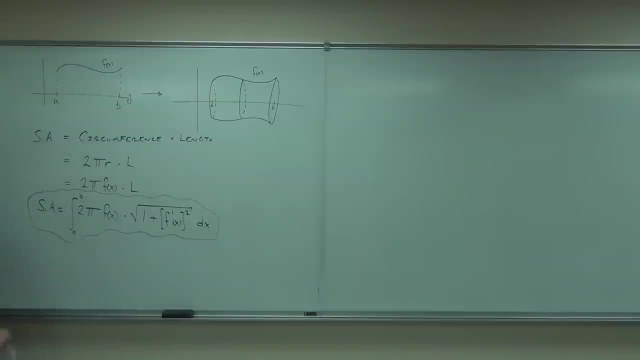 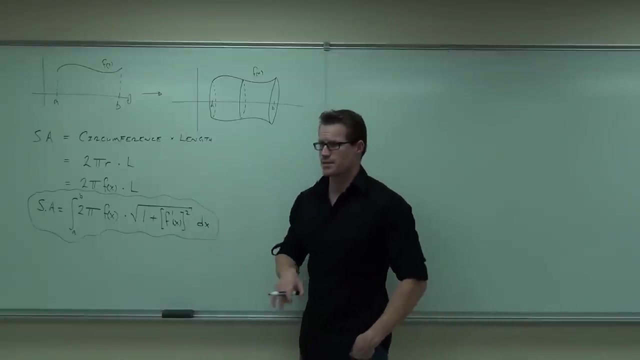 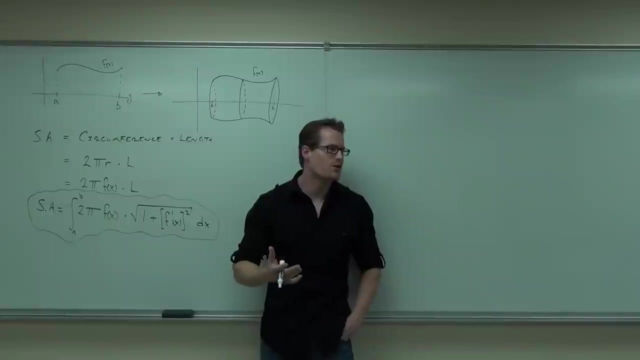 Now a question, Okay, Okay, Question. What axis did we just go around? Notice how it's in terms of x. So most of our formulas are like that: If you go around x, you have it in terms of x. 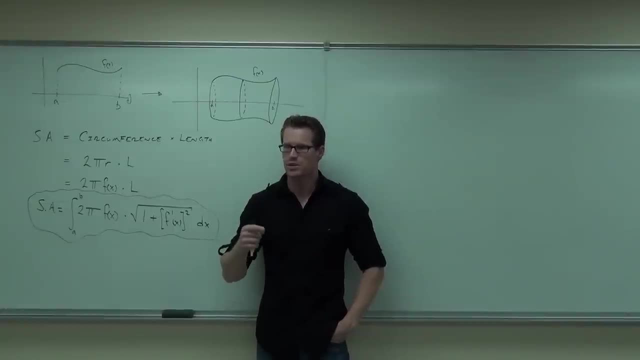 If you go around y, you have it in terms of y. What's the only one that's not like that? The shells, The cylindrical shells- is the only one that's not like that. So that's the one to watch out for. 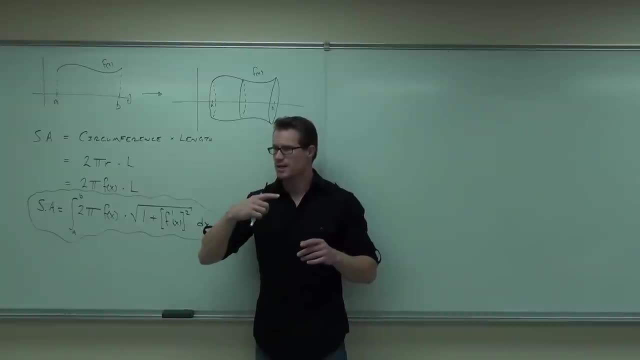 So if I say bi-cylindrical shells, If you're going around the x, It's in terms of y. If you're going around the y, it's in terms of x. Those are the different ones. okay. Everything else is basically: you're going around the x. 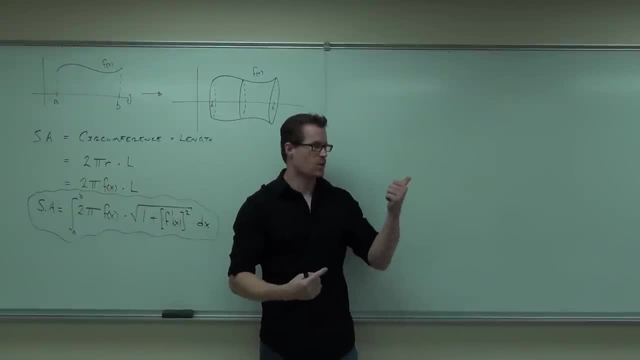 You want x's, You're going around the y, You want y's. Discs and washer works like that. Area between two curves works like that. This length of a curve, that doesn't matter, But this works like that. The surface area of revolution works like that. 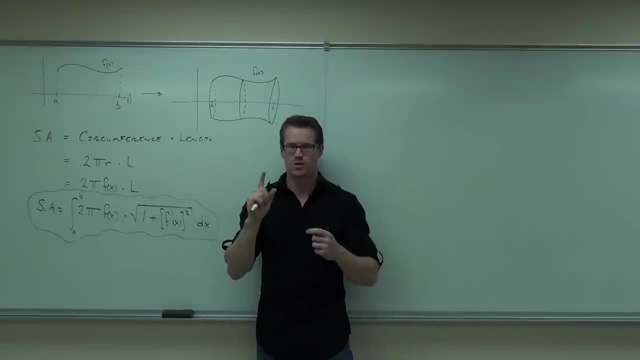 The only one that doesn't is the cylindrical shells. That one is reversed. You're going around the y You want in terms of x. You're going around the x You want in terms of y. I'm not sure if you're okay with that so far. 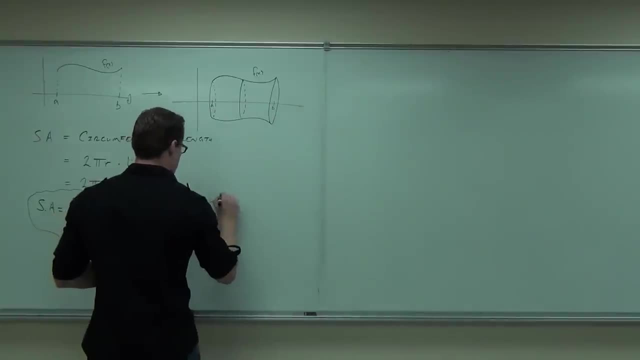 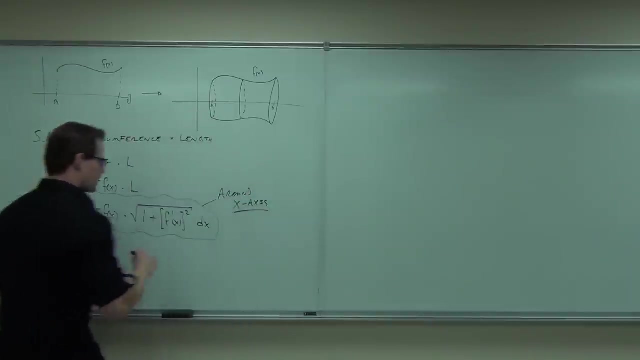 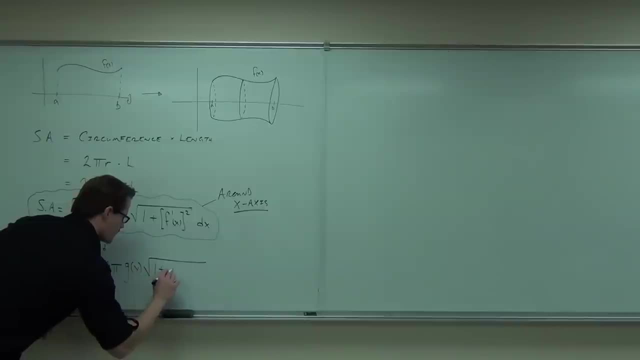 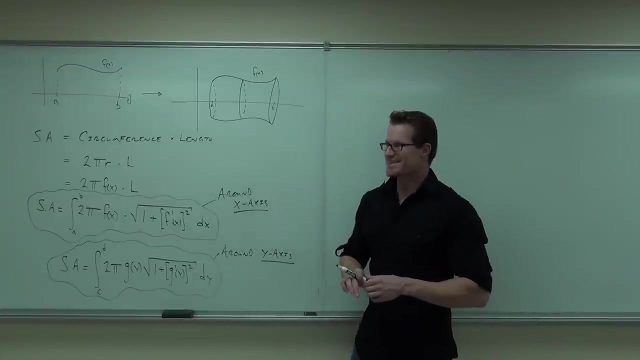 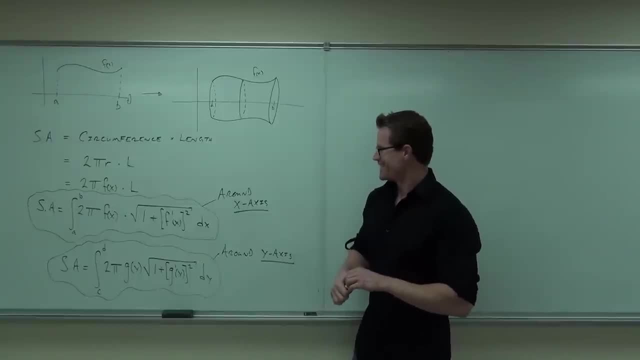 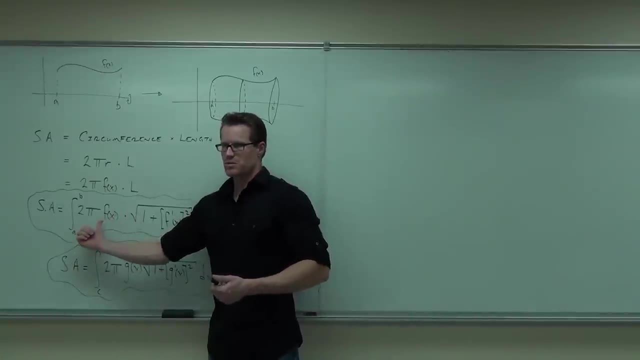 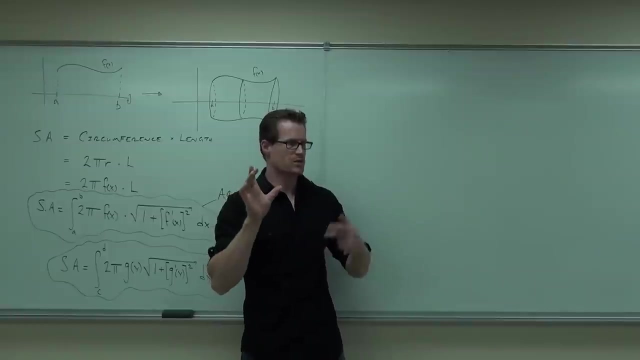 Nice. Can you see what the parts are? Can you see that this is actually circumference of every little circle at x? No problem, That's circumference. This is the length of the entire curve and in order to find surface area, you multiply the circumference times the length. 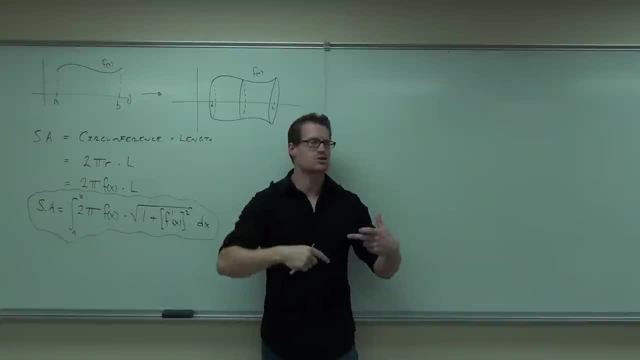 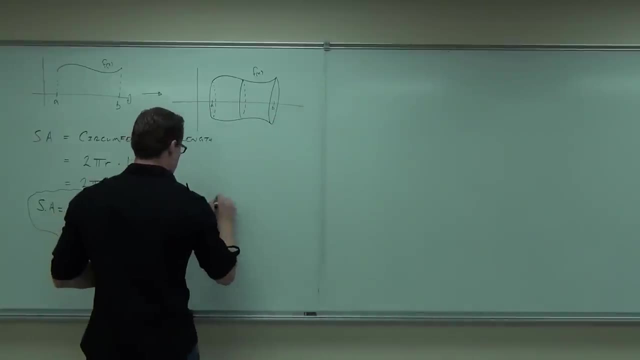 That one is reversed. You're going around the y you want in terms of x. You're going around the x you want in terms of y. I'm not sure if you're okay with that so far, Alright. so this make a note. this is around the x axis. 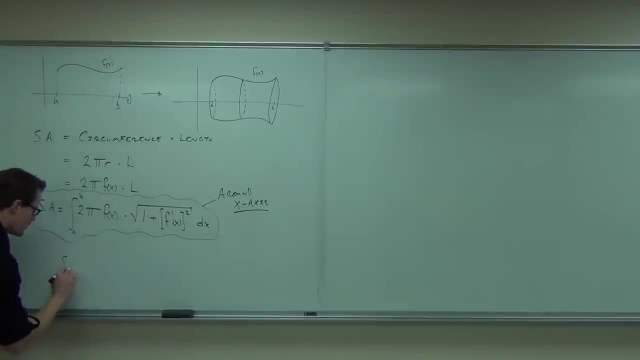 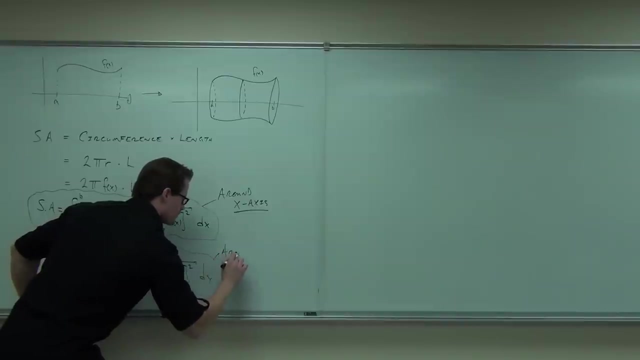 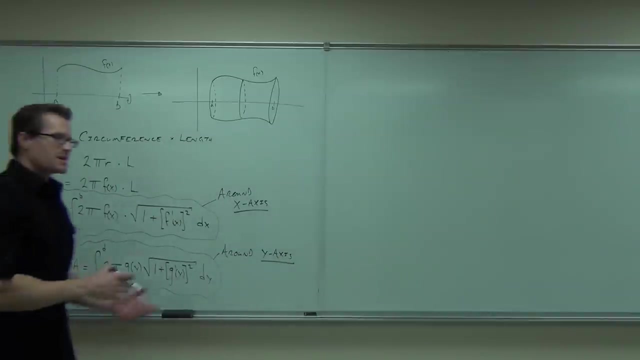 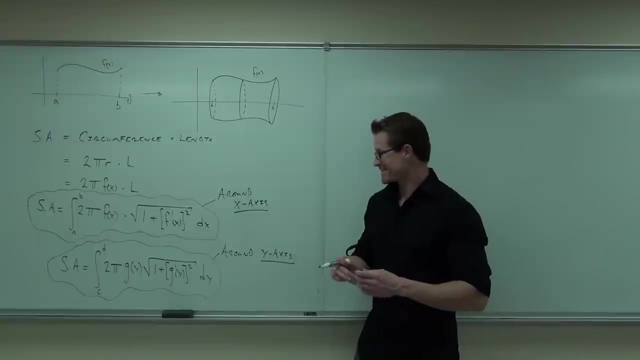 I can go around the y axis. just gotta switch my variables. This one would be for around the y axis. That's basically it. That's the last formula you have to deal with in this particular class. Nice, Nice, Yay. 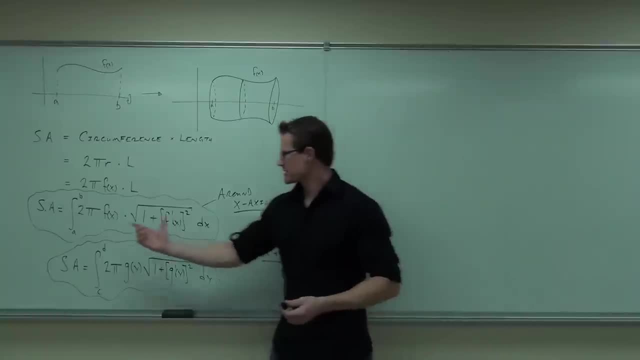 Can you see what the parts are? Can you see that this is actually circumference Of every little circle at x? No problem, that's circumference. This is the length of the entire curve and in order to find surface area, you multiply the circumference times the length. 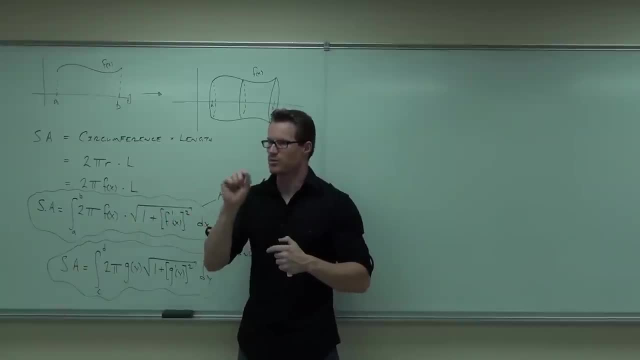 We have to integrate because it's changing. That's what the integration does for us. It breaks it up little by little, adds every single little piece, But that's basically the idea. circumference, times, length, Again, if you want a more explicit definition of this, 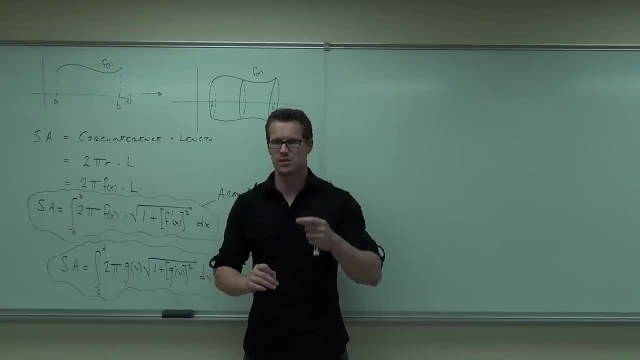 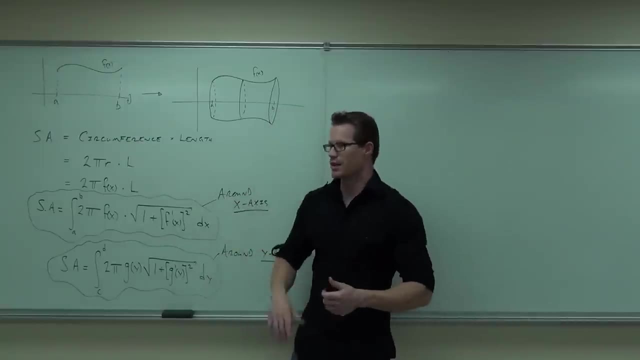 I break it down piece by piece. You can go online, Watch the previous section and then hopefully you'll be able to follow the actual calculus behind it. This was kind of a logical explanation, not a very serious explanation. Could you follow the not very serious explanation? 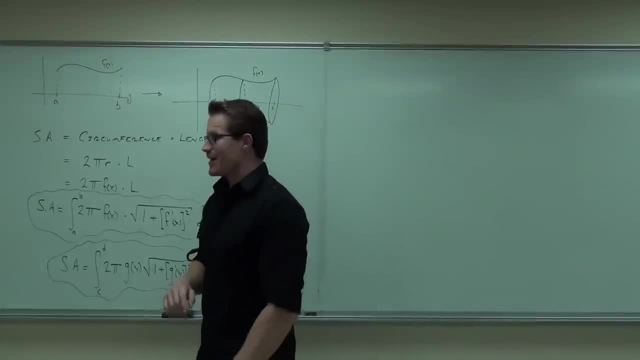 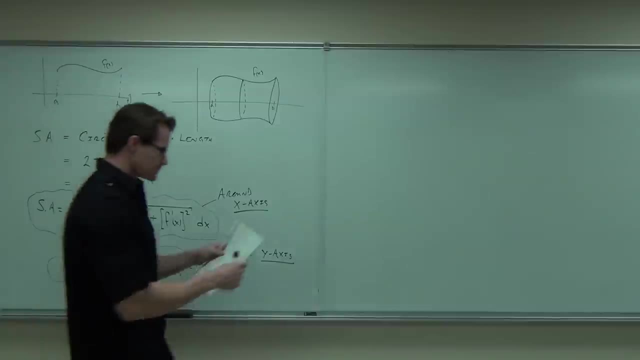 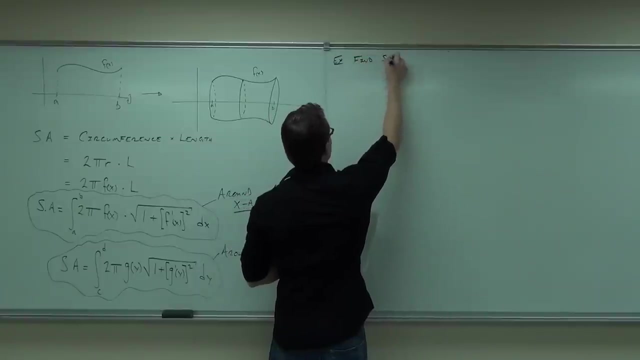 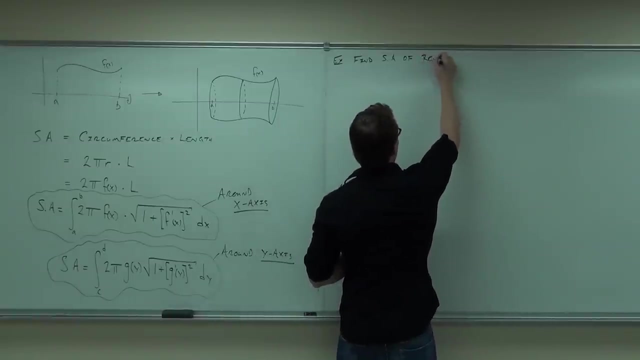 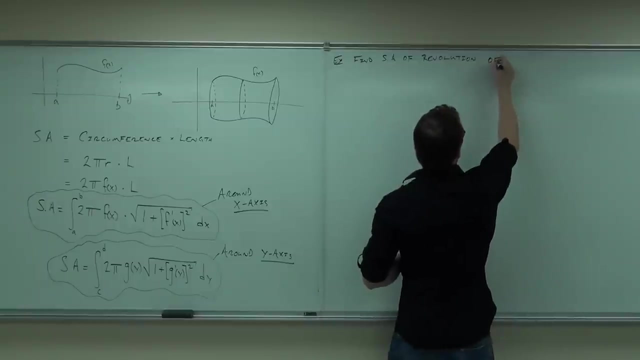 OK, go watch the serious one now. Now, I'm guessing that you're going to want a couple examples. Would you like some? Oh yeah, Let's find the surface area of revolution of y equals x. cubed between x equals 0.. 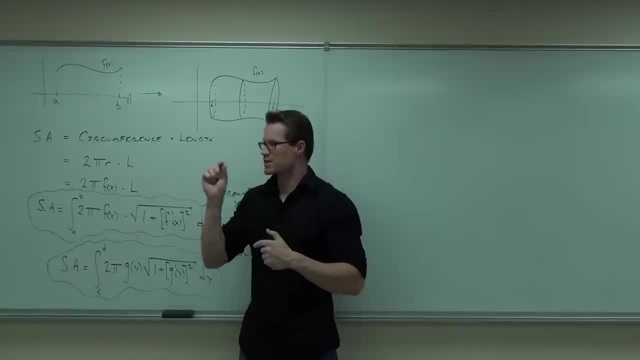 We have to integrate because it's changing. That's what the integration does for us. It breaks it up little by little, adds every single little piece, but that's basically the idea. Circumference, times, length. If you want a more explicit definition of this, I break it down piece by piece. 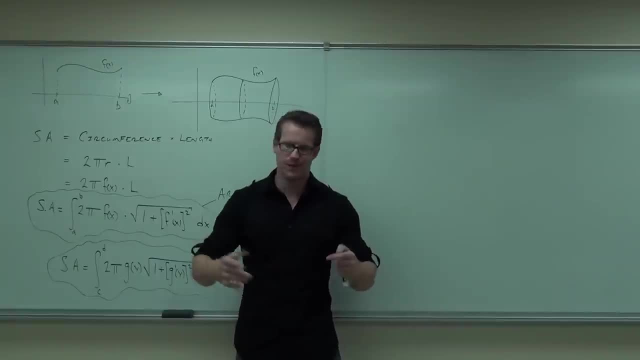 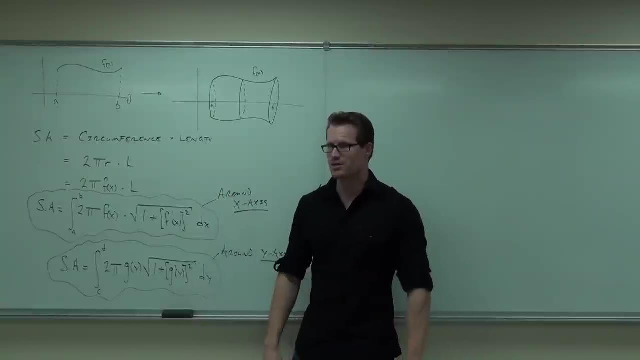 You can go online watch the previous section and then hopefully you'll be able to follow the actual calculus behind it. This was kind of a logical explanation, not a very serious explanation. Could you follow the not very serious explanation? Okay, Go watch the serious one now. 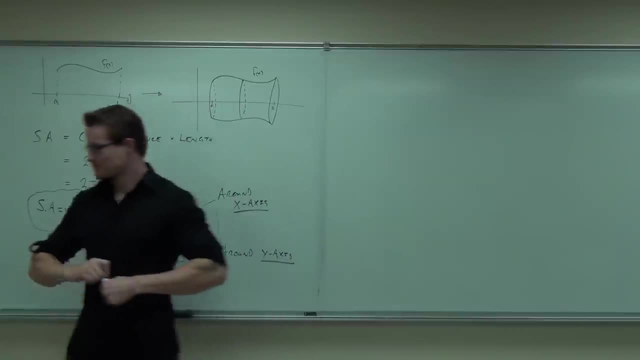 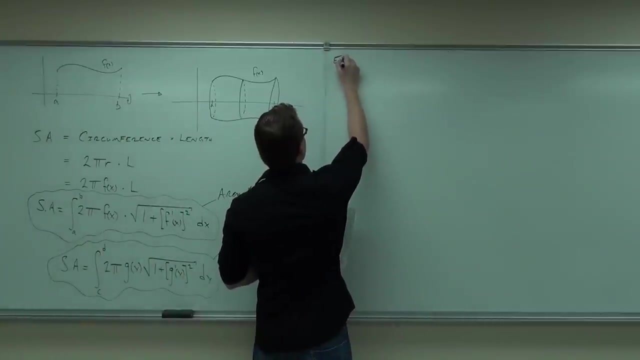 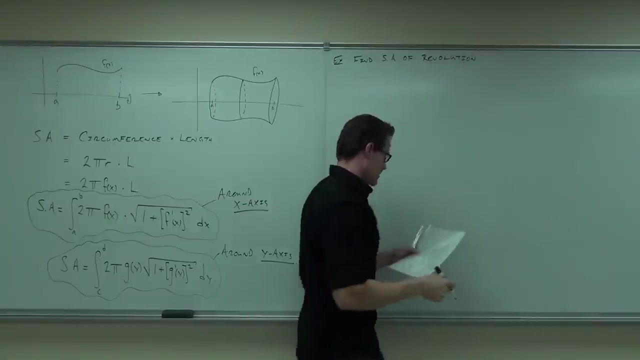 Now I'm guessing that you're going to want a couple of examples. Would you like some? Yeah, Okay, Okay, Okay, All right, Let's find the surface area of revolution. That's my thing. music Of Y equals X cubed. 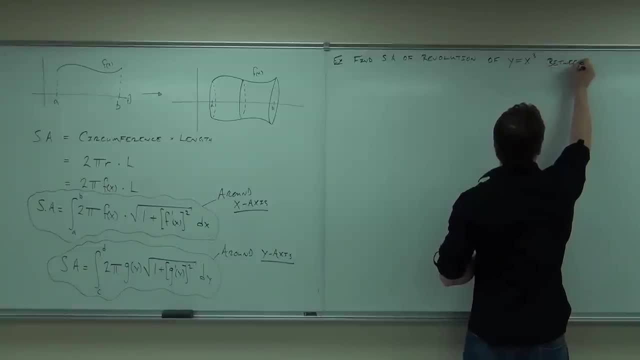 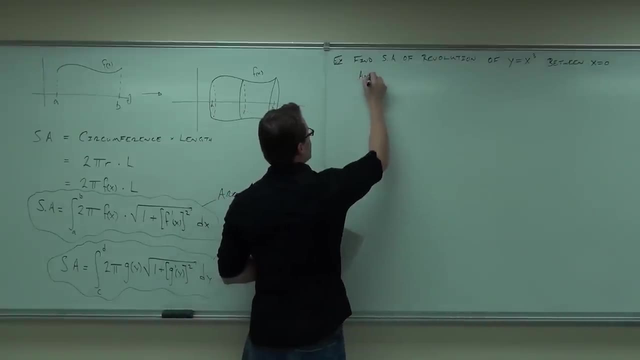 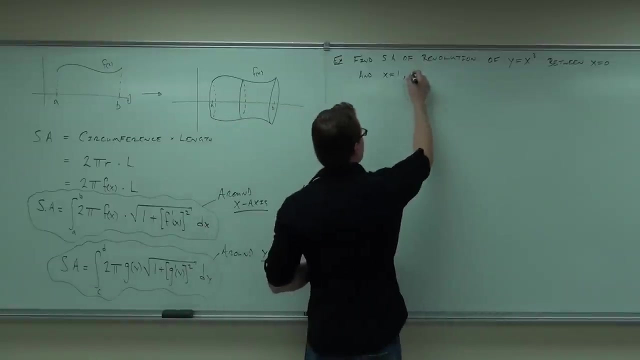 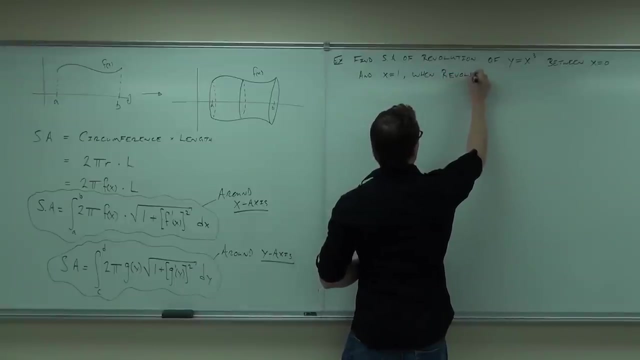 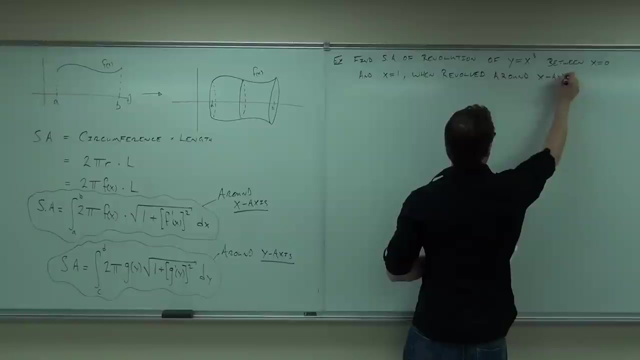 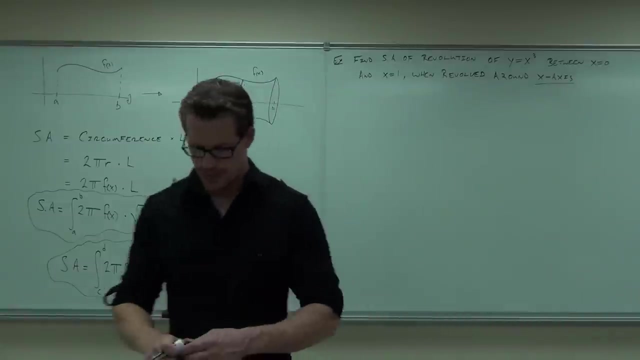 All right between x equals 0 and x equals 1 when we revolve it around the x-axis. Oh, tell me something before we begin. the problem is my function. okay, if we're going around the x-axis for surface area, is it okay? 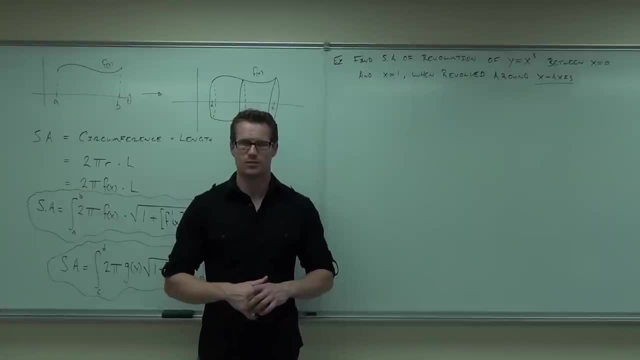 Yes, Cool. Would it be okay for disks and washers finding volume? Yeah, Would it be okay for cylindrical shells? No, Okay, good, So you're getting the hang of it. Cylindrical shells is the one where you have to have it in terms of y, everything else. 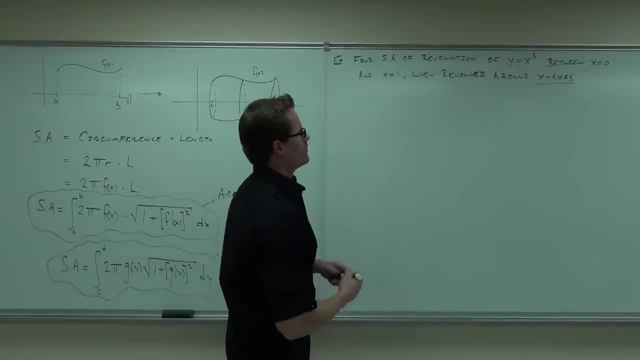 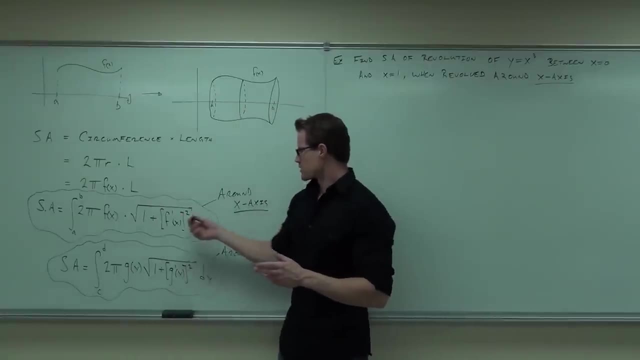 matches up with the axis. You're good to go. Now can you set up the integral. Before you set up the integral, let's look at the formula. We're using this one because we're around the x-axis. What might you want to do first before you start just plugging random things in? 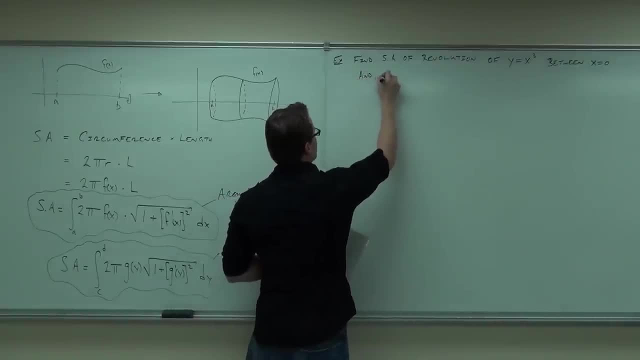 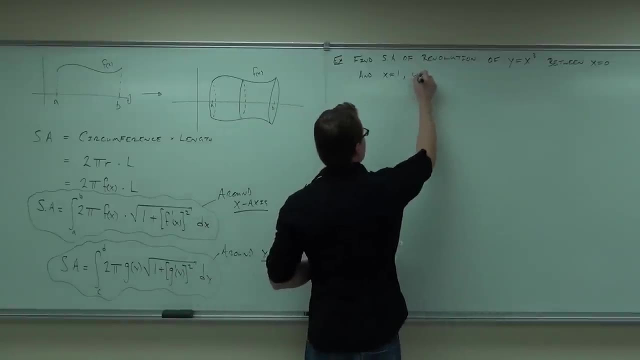 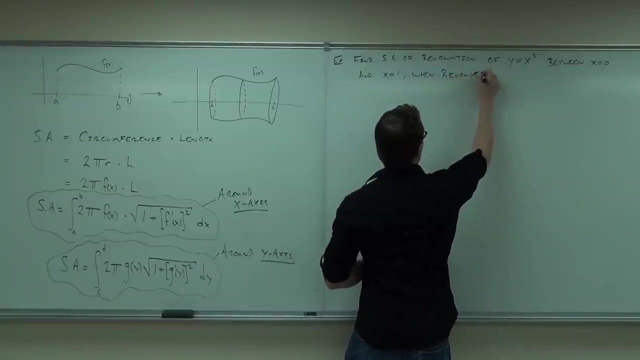 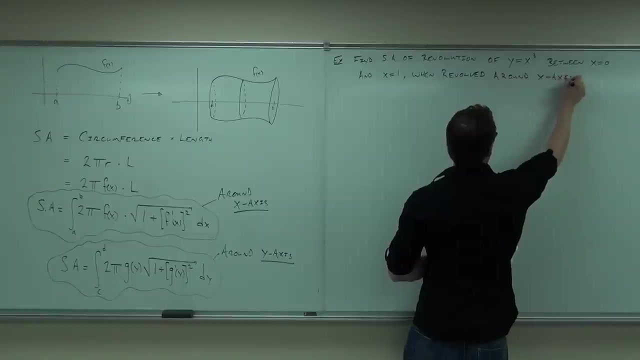 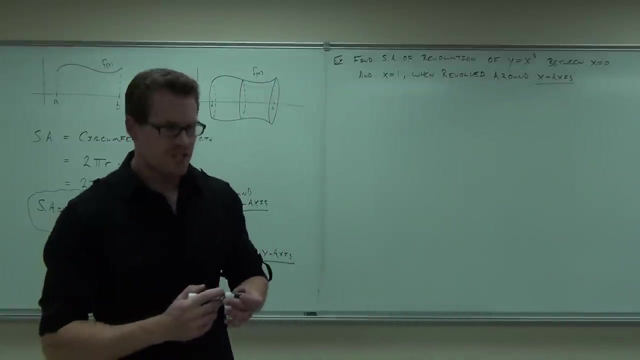 OK, And x equals 1 when we revolve it around the x-axis. Oh, tell me something Before we begin the problem: Is my function OK if we're going around the x-axis for surface area? Is it OK, Cool? 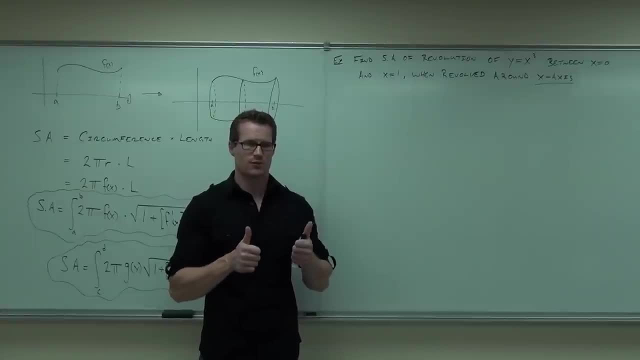 Would it be OK for disks and washers finding volume? Would it be OK for cylindrical shells? OK, good, So you're getting the hang of it. Cylindrical shells is the one where you have to have it in terms of y. 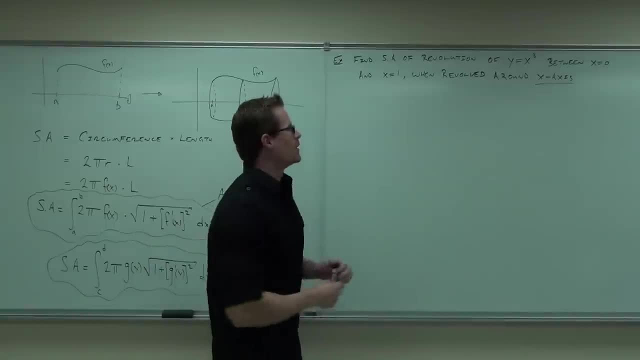 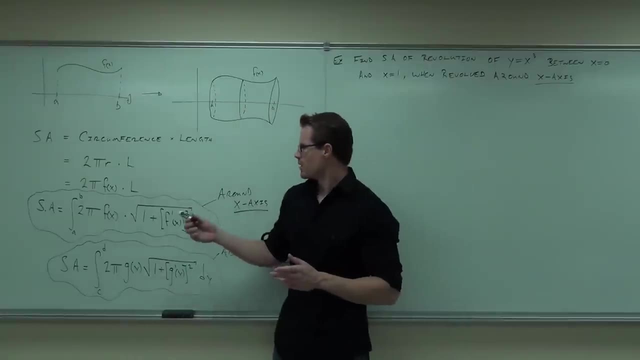 Everything else matches up with the axis. You're good to go. Now can you set up the integral? Before you set up the integral, let's look at the formula. We're using this one because we're around the x-axis. What might you want to do first? 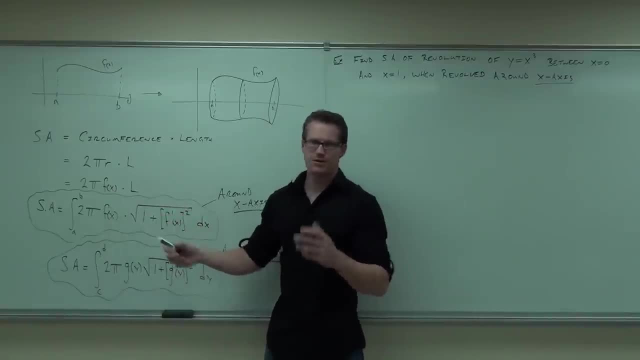 Before you start just plugging random things in The derivative. The derivative's a must, So you've got to be able to take that derivative. So let's go ahead and find We know that y equals x cubed. Let's find the derivative y prime equals what? 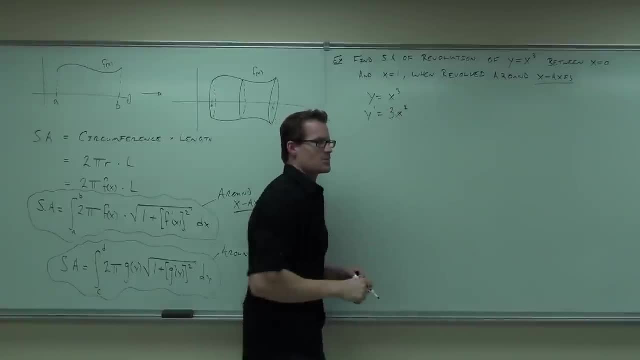 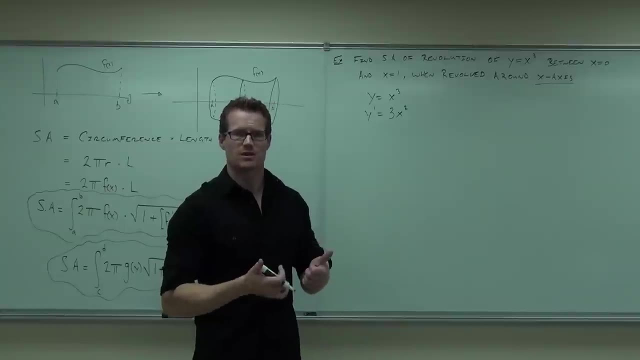 Square- Yeah, don't forget about the square. I know that some of you go very fast And you forget some of these constants. Those constants are going to be huge in these problems, So basic derivatives are a must for you. There's not going to be anything ridiculous like chain rule. 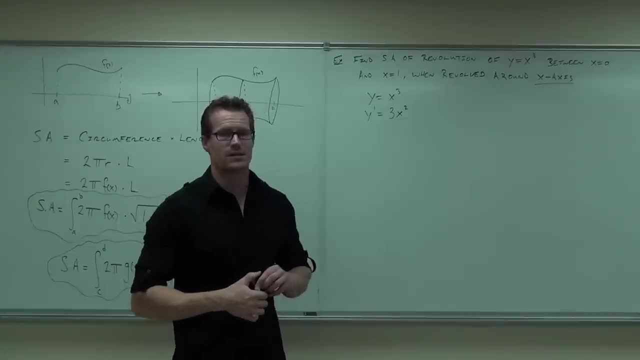 quotient rule, things like that within this And what. That must be pretty tasking. I mean it would be very hard, But be able to take a simple derivative. Now let's continue to set this thing up. Surface area. 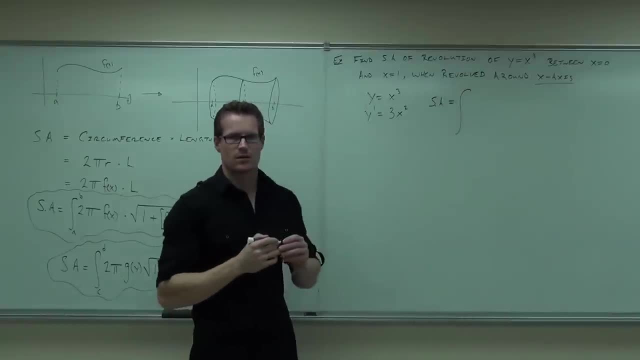 Start me out, folks. What am I going to have from where to where? 0.. Yeah, notice, it's in terms of x, correct, And that's what we wanted for going around the x-axis. So that's perfect for us. 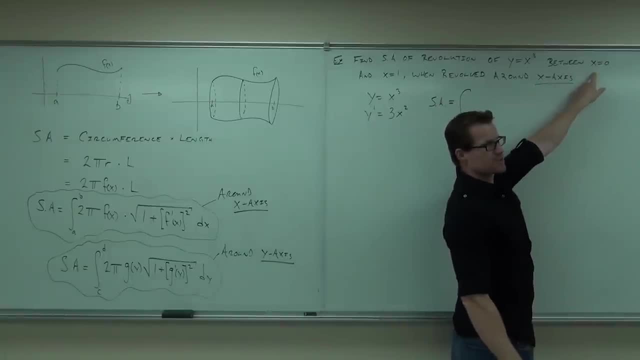 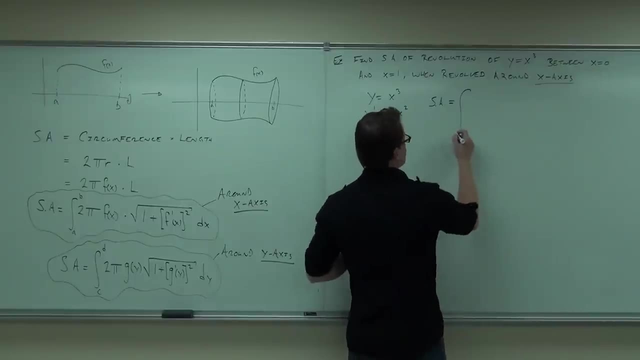 If this wasn't- or look it- If this was going around the y-axis, I would have to change x's into y's for this. So here I have 0 to 1. Not too bad, Continue. What else are we going to have? 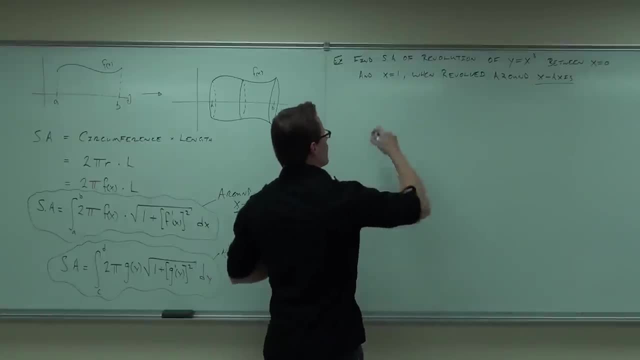 The derivative. The derivative is a must, So you've got to be able to take that derivative. So let's go ahead and find. we know that y equals x cubed. let's find the derivative y prime equals what Square? Don't forget about the square. 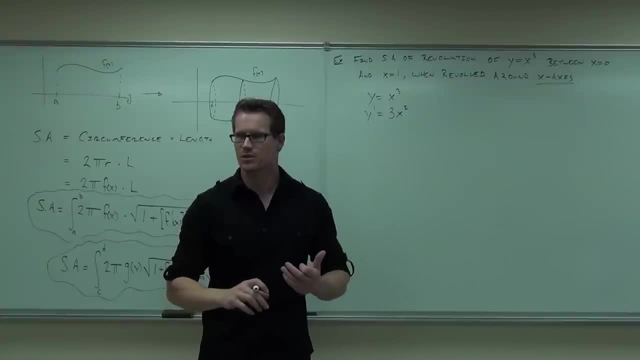 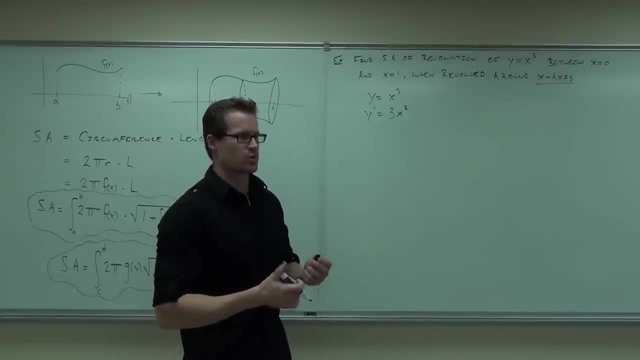 I know that some of you go very fast and you forget some of these constants. Those constants are going to be huge in these problems, So basic derivatives are a must for you. There's not going to be anything ridiculous like chain rule, quotient rule, things like. 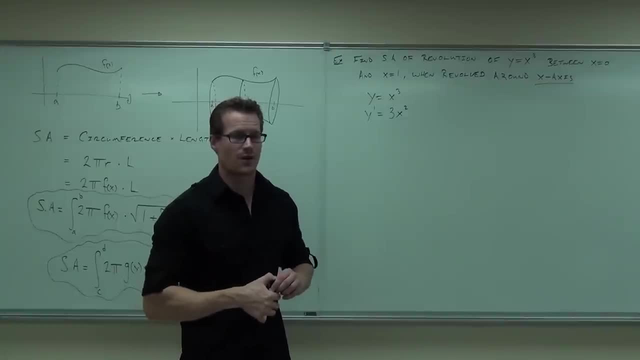 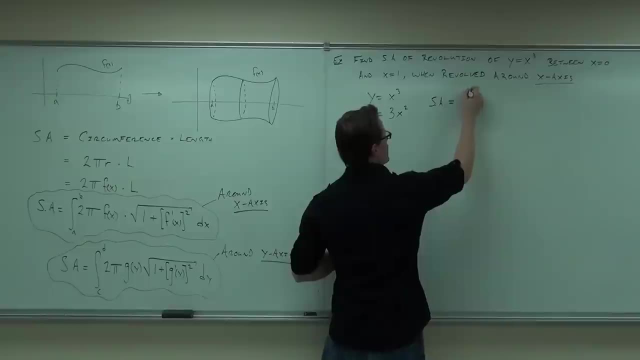 that within this, It'll be pretty tasking, I mean, it'll be very hard- But be able to take a simple derivative. Now let's continue to set this thing up: Surface area. Start me out, folks. What am I going to have? 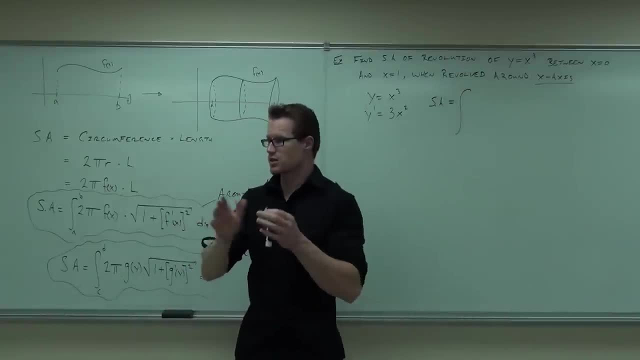 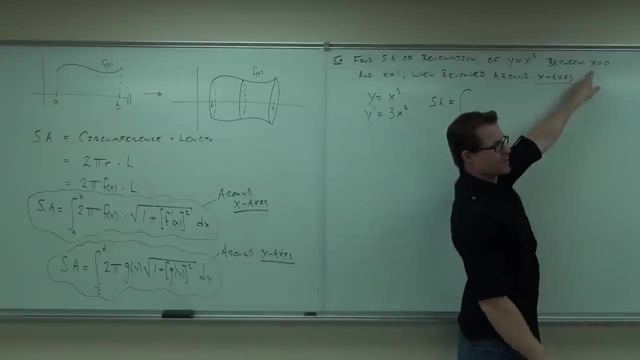 From where to where? Zero? Yeah, notice, it's in terms of x, correct? And that's what we wanted for going around the x-axis. So that's perfect for us If this wasn't- or, look it, If this was- going around the y-axis. 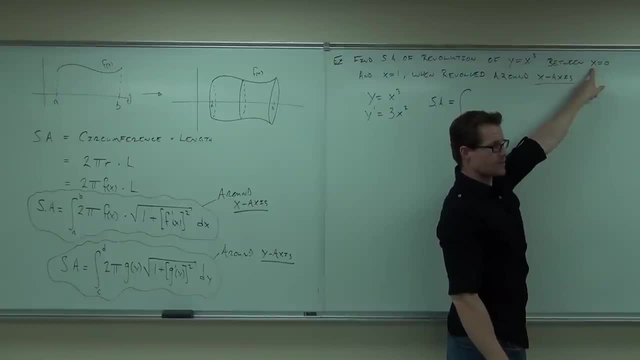 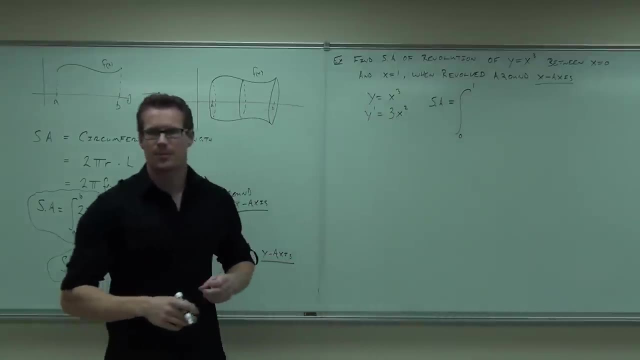 I would have to change x's into y's for this. So here I have zero to one. Not too bad. Continue. What else are we going to have? Two pi, Two pi is going to be there. Two pi comes from the fact that we're taking circumferences. 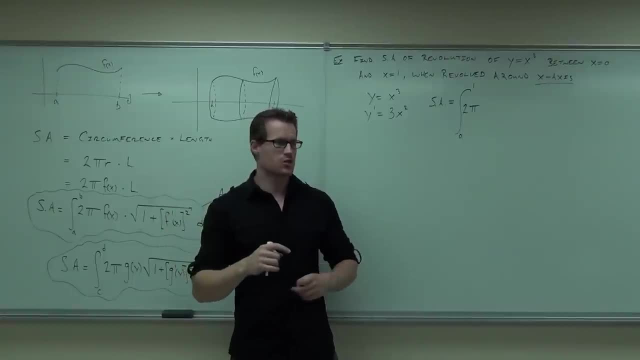 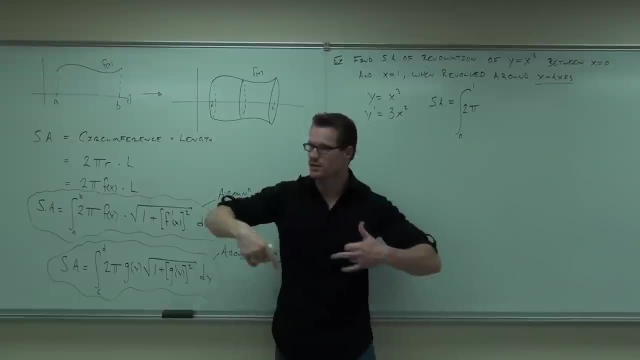 That's where that's coming about. What now? Where are you getting x cubed? Yeah, that's what that says. Take your function, whatever it happens to be in terms of x, because we're going around the x. Okay. 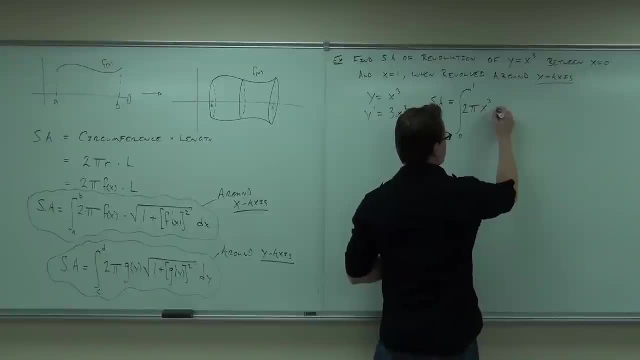 Okay, Okay, Then what? Square root, Square root. What's inside my square root? One plus 3x squared. Where's the 3x squared come from The derivative. That's the derivative We already found. that's why you find it first. 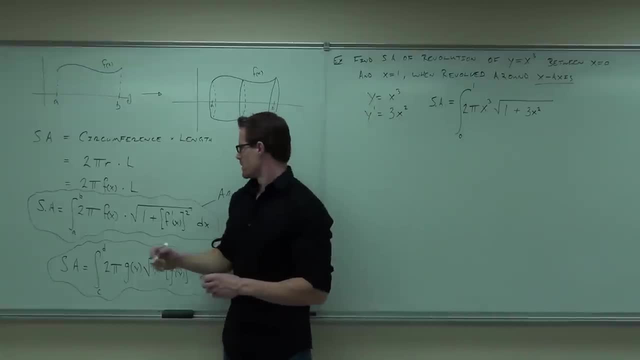 And then what Square root? Oh yeah, don't forget the square root. If you forget the square root, you pretty much can't do that integral in this class. So don't forget that. Dx Again around the x Dx. 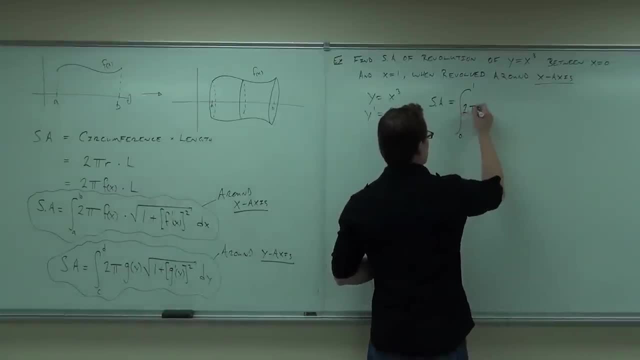 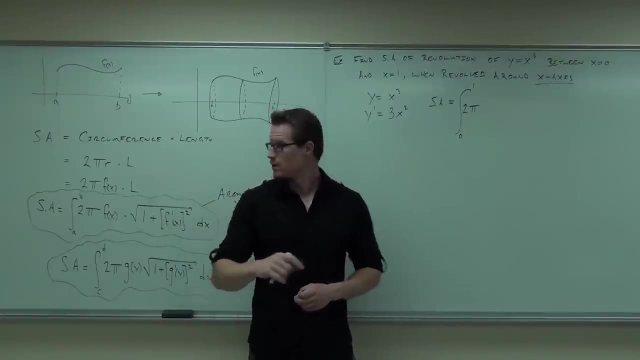 2 pi. 2 pi is going to be there. 2 pi comes from the fact that we're taking circumferences. That's where that's coming about. What now? x cubed? Where are you getting x cubed The function? 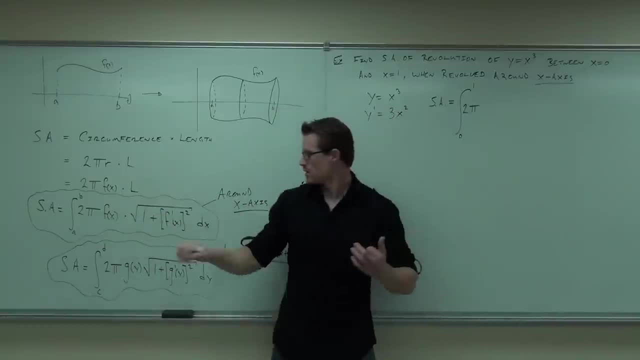 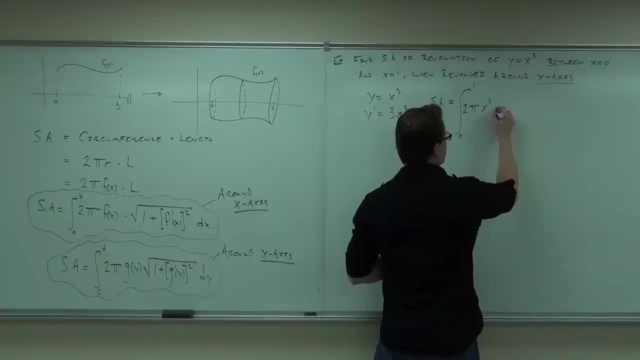 Yeah, that's what that says. Take your function, whatever it happens to be in terms of x, Because we're going around the x, Then what Square root? Square root, What's inside my square root? 1 plus. 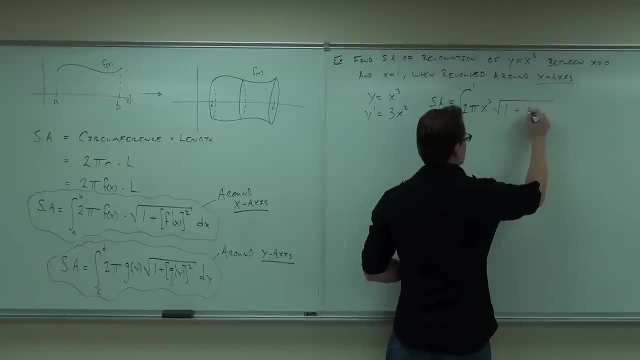 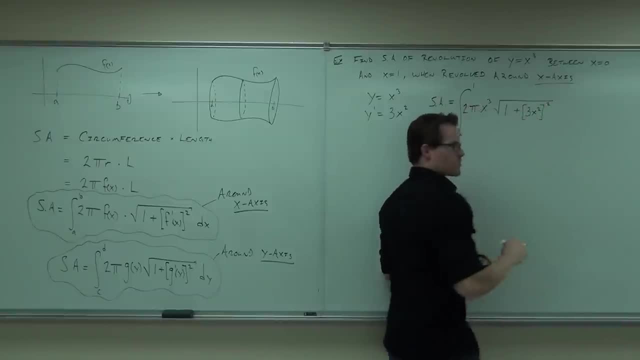 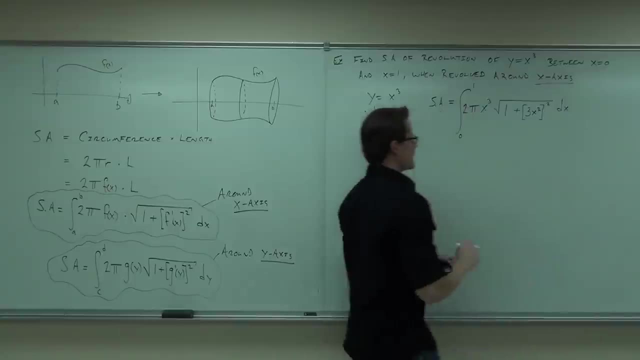 And then what Square root? Oh yeah, Don't forget the square root. If you forget the square root, you pretty much can't do that integral in this class. so don't forget that dx begins around the x. Do y'all feel OK with the setup? 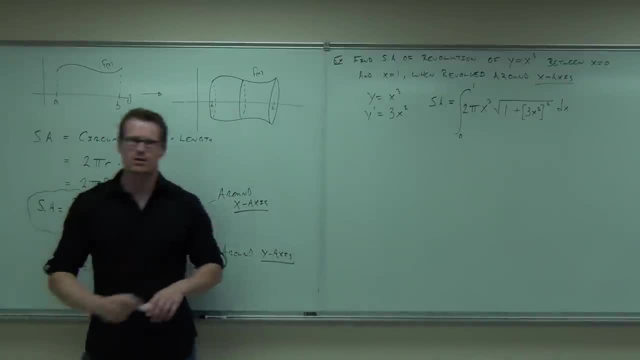 Yeah, Let's go piece by piece, step by step, and figure out this thing. What are you going to do first? do you think Pull out the 2 pi out? OK, we can pull the 2 pi out. I like that idea. 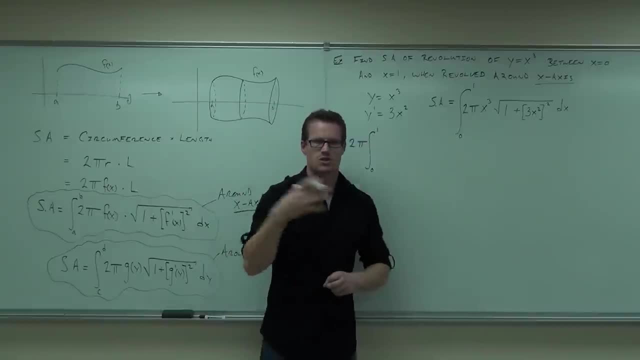 Go from 0 to 1.. In fact, I think the formula in some books actually gives a 2 pi in front of it, which is appropriate. That's just fine. I like to show it here because you see where the part is. 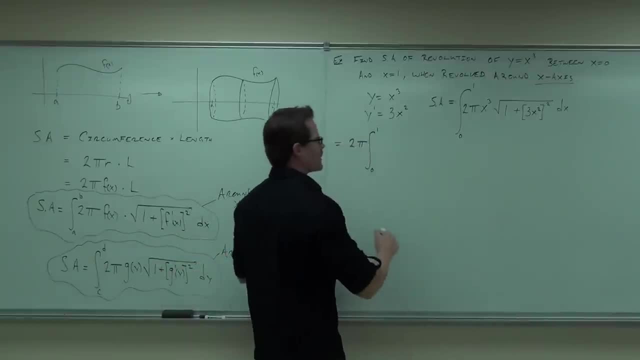 But you can always pull that 2 pi out. It's a constant. It's being multiplied, No problem. What now? I would do x to the cube and I would also do substitution. Well, before we even look at that, 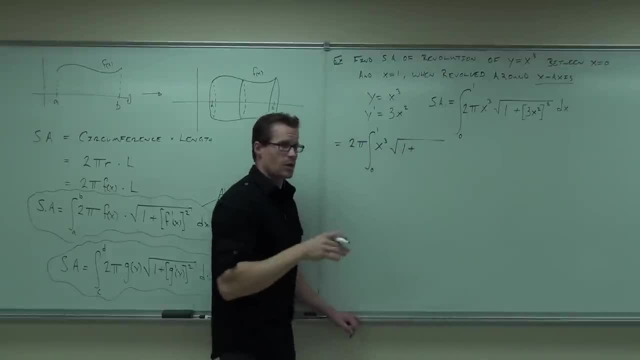 I'd do: square root of 3x squared. What am I going to get when I square the 3x squared, 3x squared, 9x, 9x, 9x. Good, Then you do the substitution. 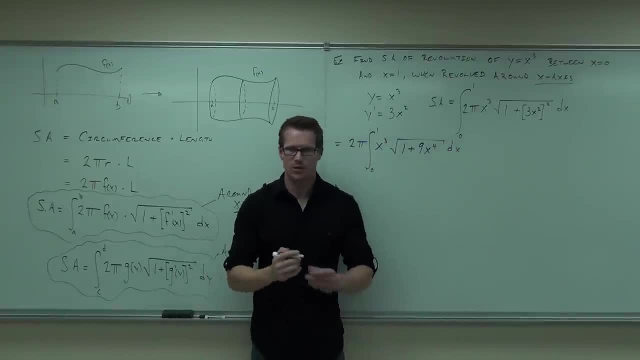 Cool. Now we look at it as an integral, because that's what it is. We say: how in the world can we do this integral? We've mastered that stuff already. What type of problem is this for you? Substitution, An easy one, because it's really smacking in the face, right? 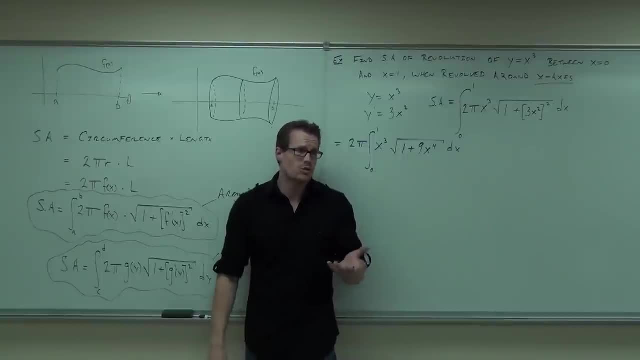 It's got to work out. It's something we've done in this class or we can't do it. There's no more integration techniques for first semester calculus. You have them, So you either have to maneuver, You have to manipulate it somehow, which? 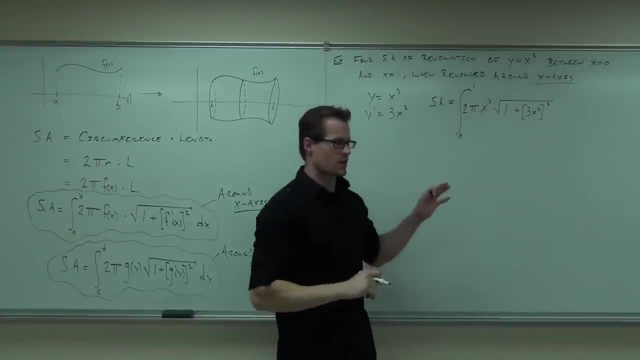 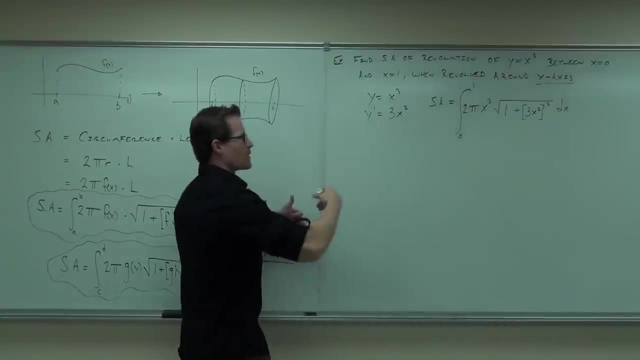 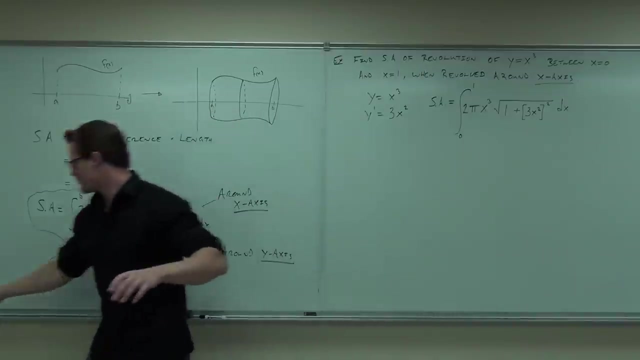 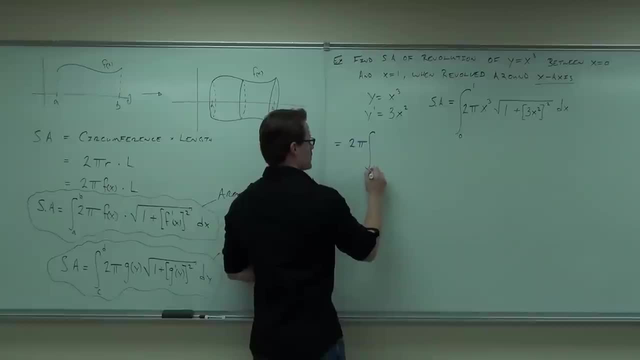 Okay, we can pull the 2pi out. I like that idea: Go from 0 to 1.. In fact, you know what? I think the formula in some books actually gives a 2pi in front of it, which is appropriate. 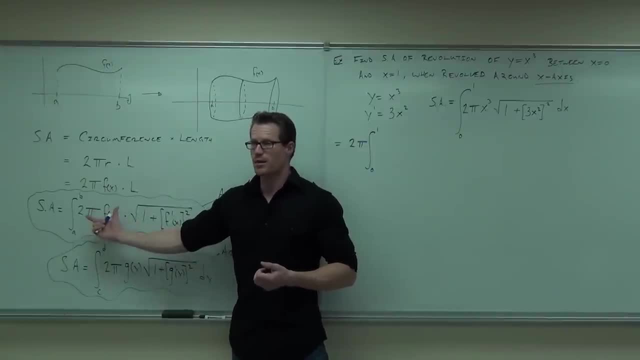 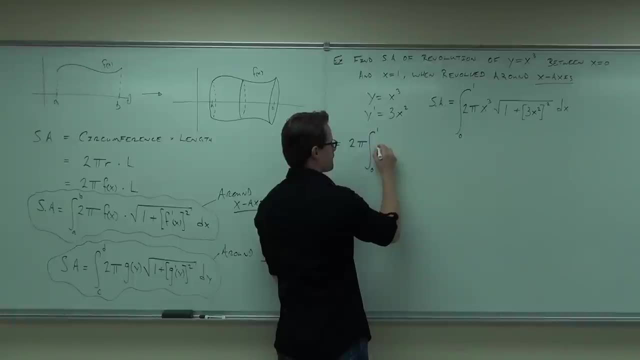 That's just fine. I like to show it here because you see where the part is. But you can always pull the 2pi out. it's a constant. it's being multiplied, No problem. What now? I would do x to the cube. 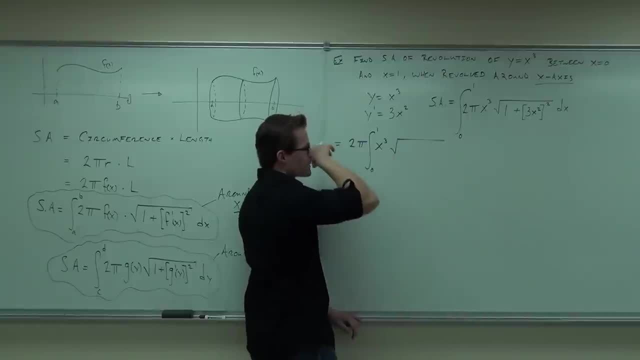 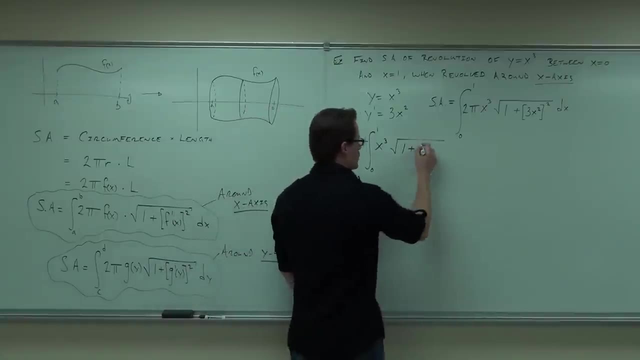 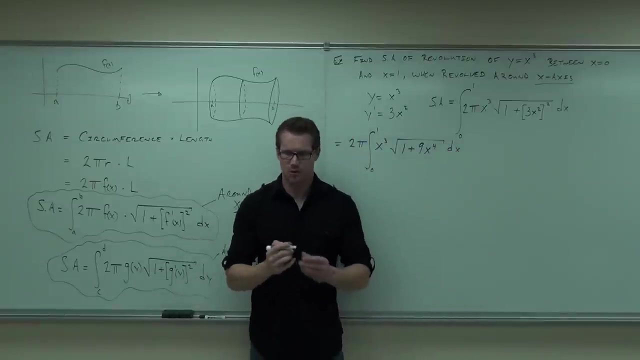 I would also do something else. Well, before we even look at that, what am I going to get when I square the 3x squared? Good, Cool. Now we look at it as an integral, because that's what it is. We say: how in the world can we do this integral? 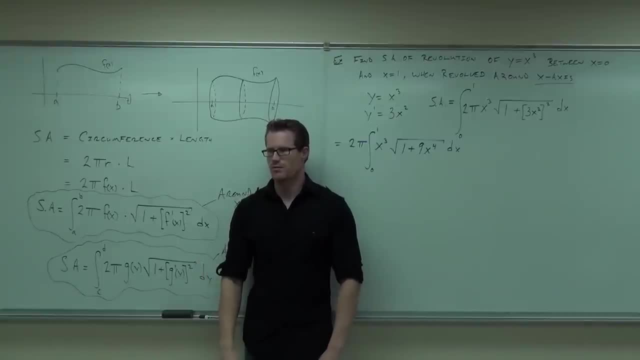 We've mastered that stuff already. What type of problem is this for you? An easy one, because it's really smacking the face right. It's got to work out. It's something we've done in this class or we can't do it. 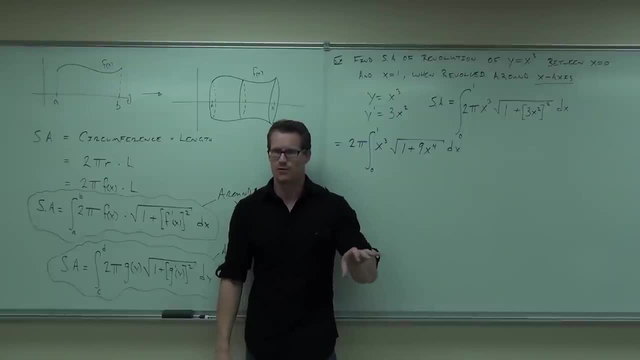 There's no more integration techniques for first semester calculus. You have them. So you either have to manipulate it somehow, which I've shown you a couple ways now, especially with the length of the curve. Oh my gosh, those are pretty heavy duty. 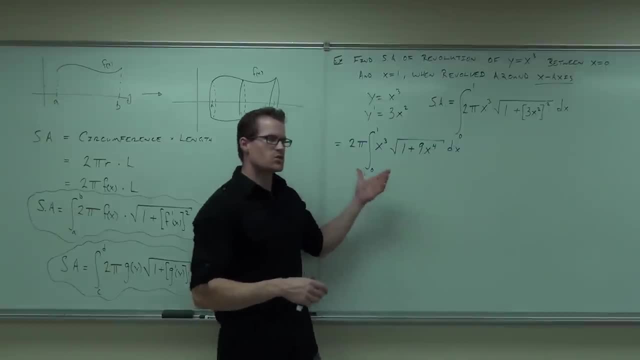 Or use some sort of a substitution. Do you see, the substitution is in fact going to work. here We have an x to the fourth and an x to the fifth. It's going to work. It's going to work just fine. 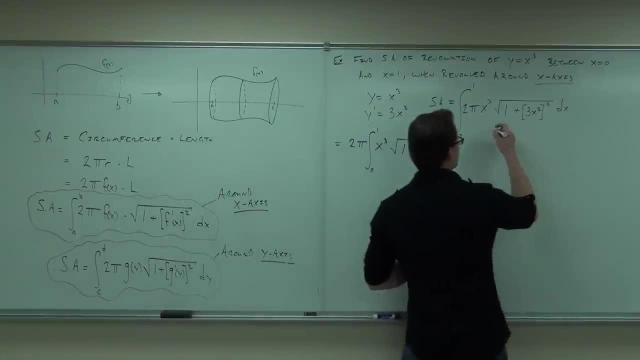 So let's use our substitution. What is your u for this? 1 plus 1.. Yeah, you pick the whole thing inside that square root. If that's the case, du equals 36x to the third dx And we have du over 36x to the third equals dx. 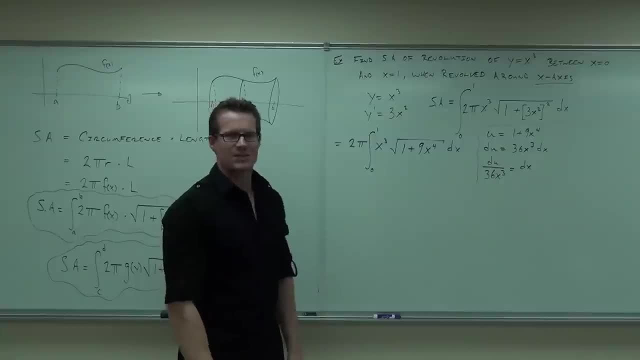 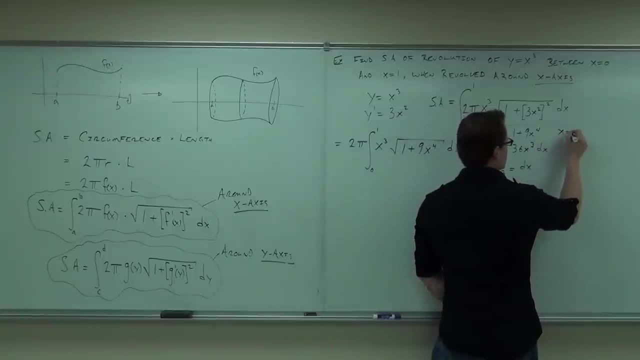 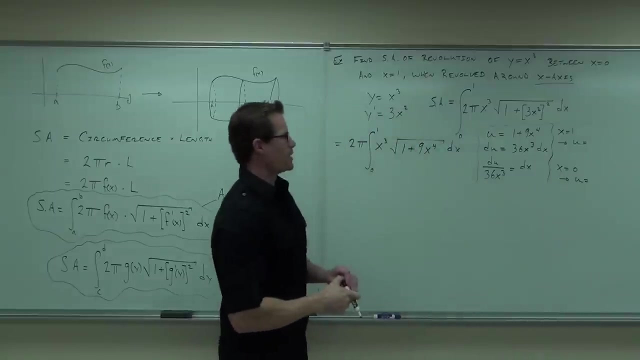 What else might you want to do? Do you guys like changing bounds? I like changing bounds too. It makes it easier later on. So let's take our x equals 1 and our x equals 0. Let's change those bounds. If x equals 1 and u is 1 plus 9x to the fourth, how much are you going to be? 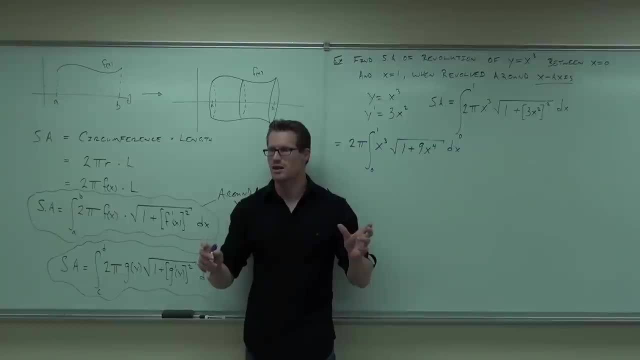 I've shown you a couple ways now, especially with the length of the curve- Oh my gosh, Those are pretty heavy duty- Or use some sort of a substitution. Do you see, the substitution is in fact going to work here. 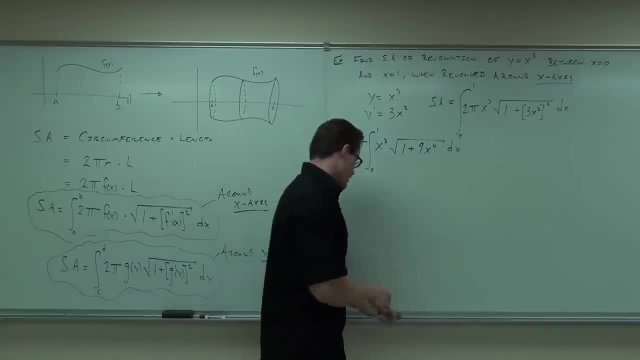 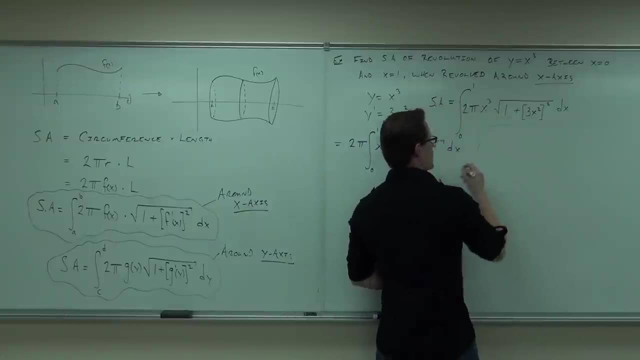 We have an x to the fourth and an x to the fifth. It's going to work. It's going to work just fine, So let's use our substitution. What is your u for this? 1 plus 1.. 9x to the fourth. 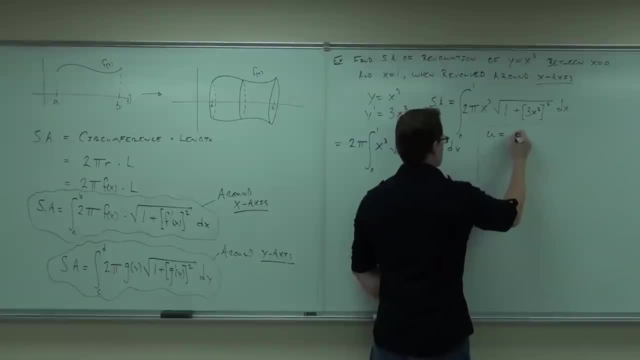 Yeah, You pick the whole thing inside that square root. If that's the case, du equals 1. 36x to the third dx And we have du over 36x to the third equals dx. What else might you want to do? 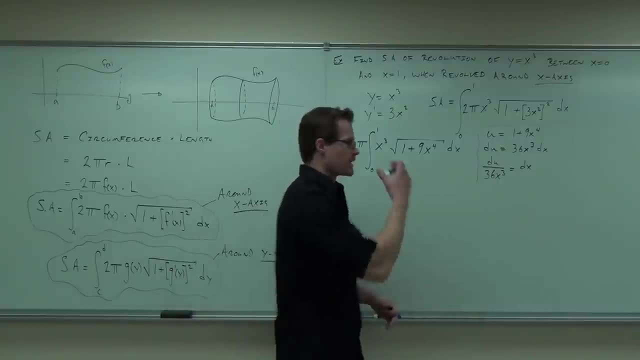 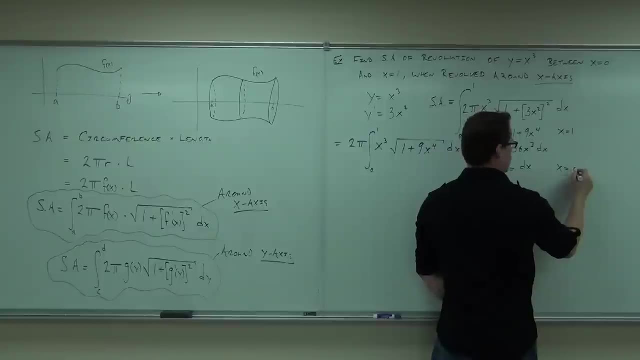 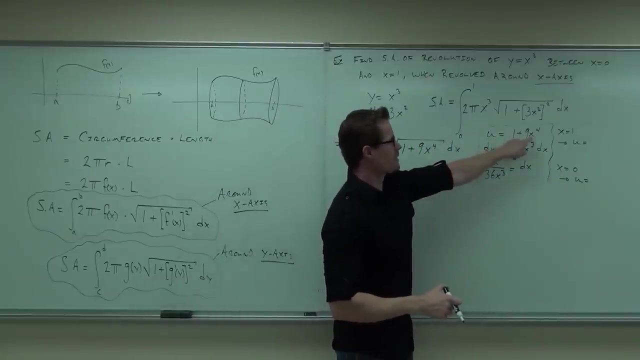 Do you guys like changing bounds? I like changing bounds too. It makes it easier later on. So let's take our x equals 1 and our x equals 0. Let's change those bounds. If x equals 1 and u is 1 plus 9x to the fourth, how much are you going to be? 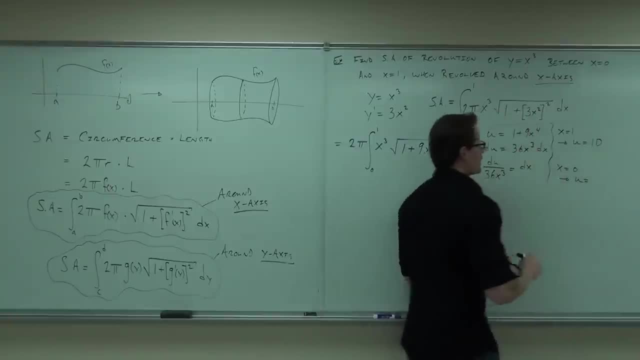 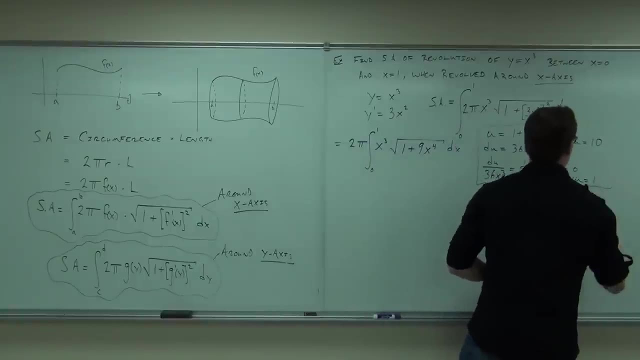 10x to the fourth. Perfect, Not too bad. If x equals 0,, how much are you going to be 1.. Not bad either. Hey, we're about ready to go on this thing. We've got our 2 pi. 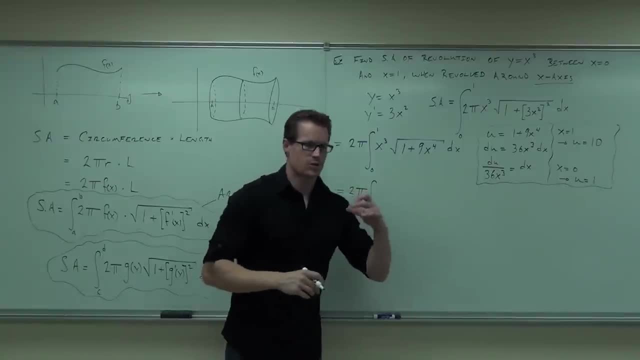 We're not going from 0 to 1 anymore. Those were in terms of x. Those are our bounds in terms of x. We want to change to u, So let's change our bounds as well. We're going to go not from 0 to 1, but from 1 to 10.. 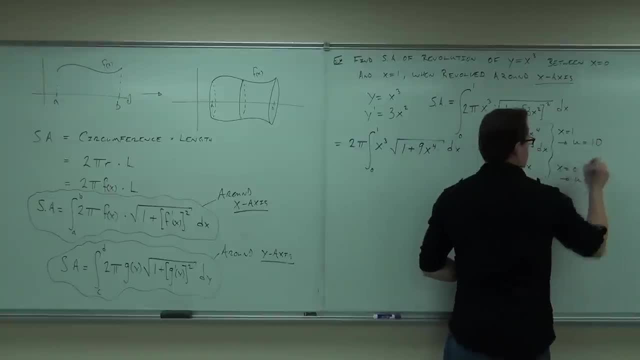 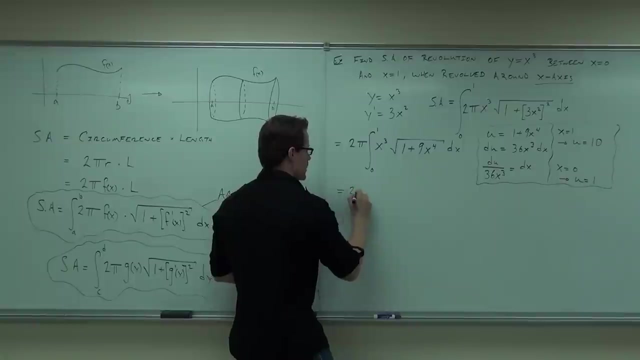 10. Perfect, Not too bad. If x equals 0, how much are you going to be? 1. Not bad either. Hey, we're about ready to go on this thing. We've got our 2 pi. We're not going from 0 to 1 anymore. 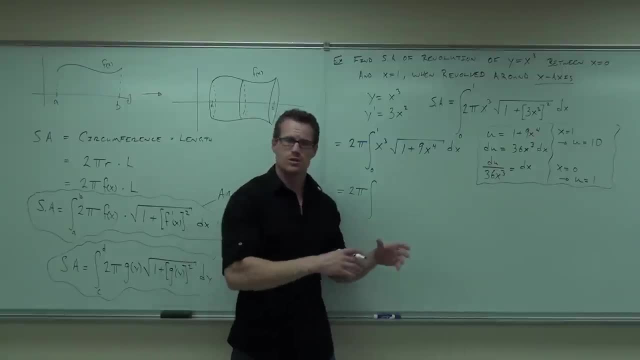 Those were in terms of x, Those were our bounds in terms of x. We want to change to u, So let's change our bounds as well. We're going to go not from 0 to 1, but from 1 to 10.. 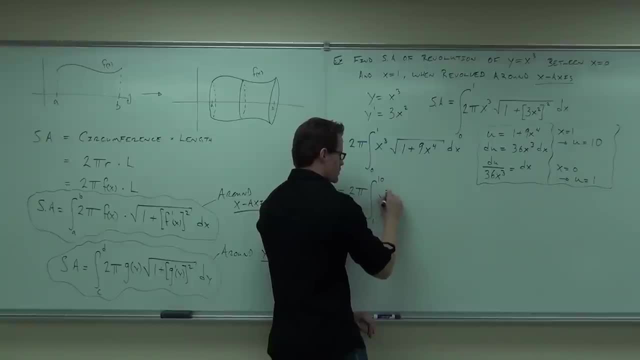 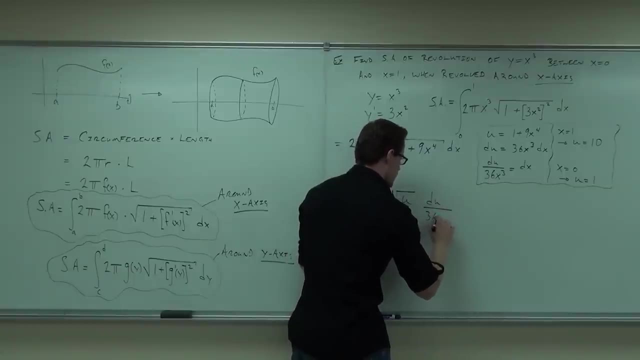 Do I still have an x cubed? Yes, Do I still have a square root? No, What's inside the square root? U? Yes, I am du over 36x to the third. That's where we make our substitution: dx equals du over 36x to the third. 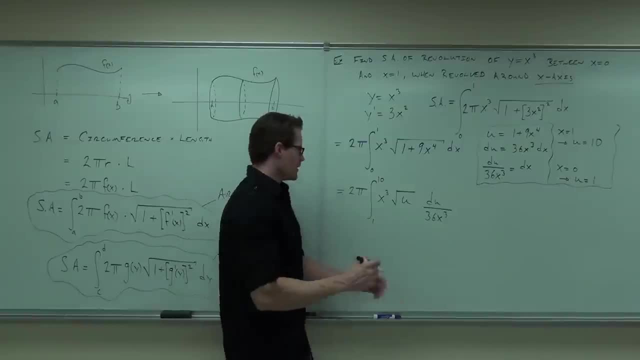 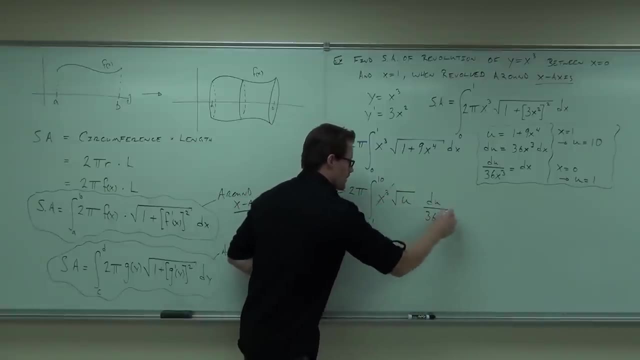 Tell me some cool things that happen here, folks. What's happening? That's what we had to have happen, right, If we couldn't get rid of those x cubed. we're basically stuck, So done and done. What else are you going to do? 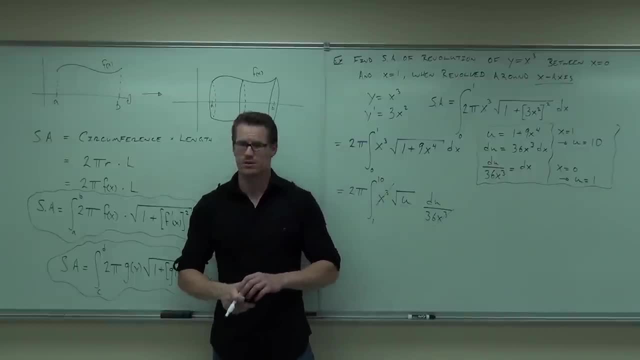 What about the 36?? Don't forget about the 36.. That's important. So if we lose that, What about the 36?? Yeah Well, the 36 is going to be 136.. Yes, But don't forget about it. 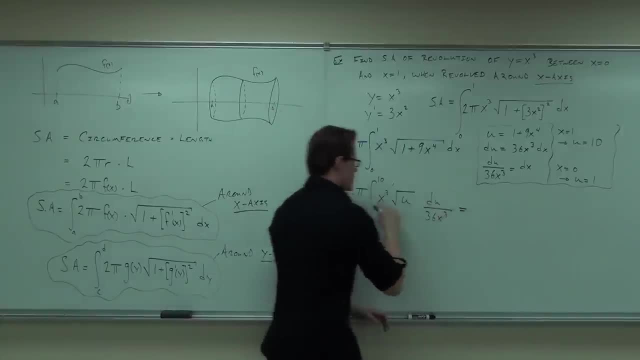 So we pull out the 136.. You have a 2 over 36.. What you're going to have up front is pi over 18.. You okay on the pi over 18?? So combine those two fractions: Still an integral 0 to 1.. 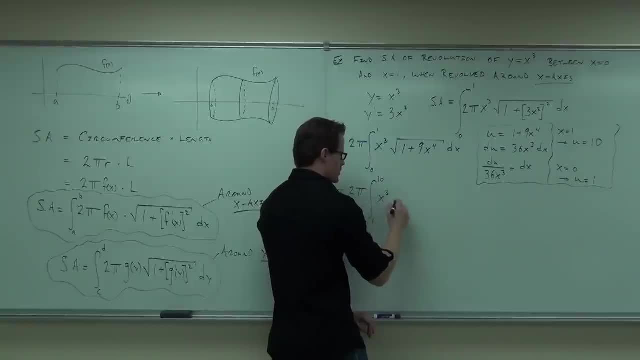 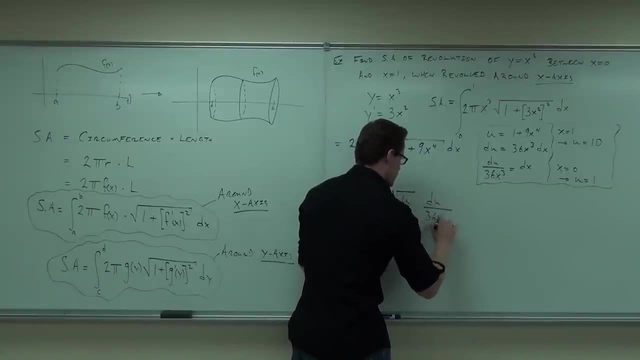 Do I still have an x cubed? Do I still have the square root? What's inside the square root? Yes, I am du over 36x to the third. That's where we make our substitution: dx equals du over 36x to the third. 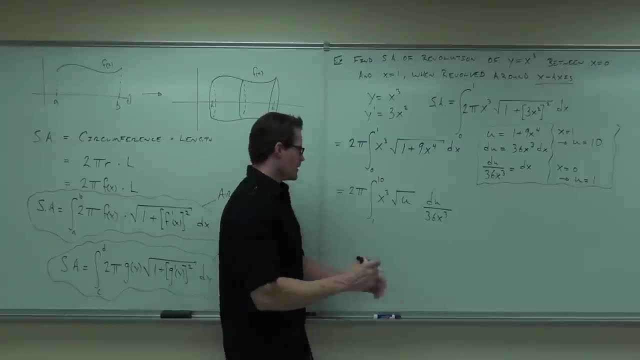 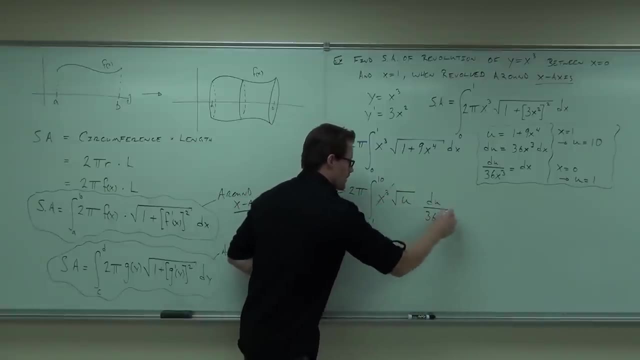 Tell me some cool things that happen here, folks. What's happening? That's what we had to have happen, right, If we couldn't get rid of those x cubed. we're basically stuck, So done and done. What else are you going to do? 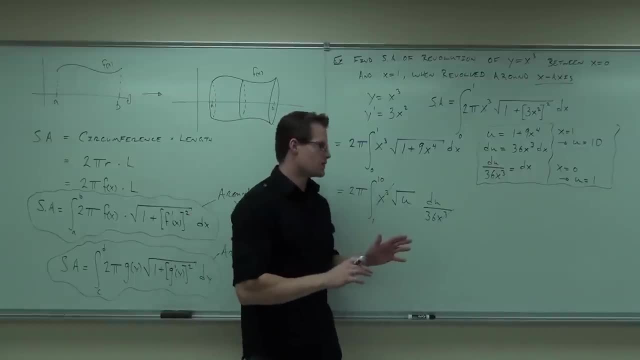 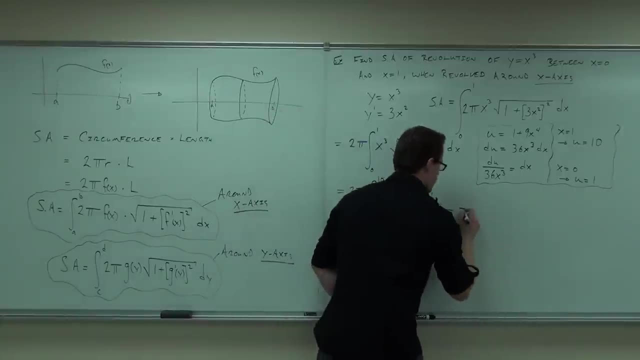 Don't forget about the 36.. That's important. So if we lose that, yeah, well, the 36, and it's going to be 136.. Yes, but don't forget about it. So we pull out the 136.. 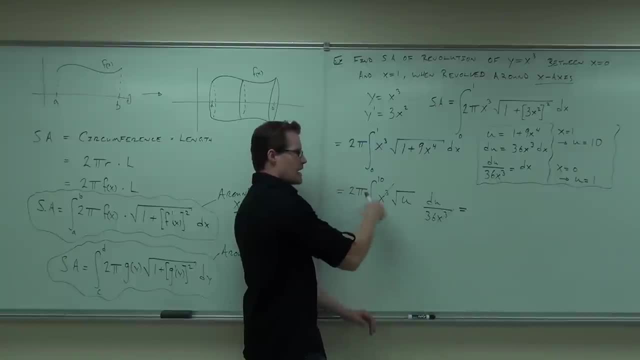 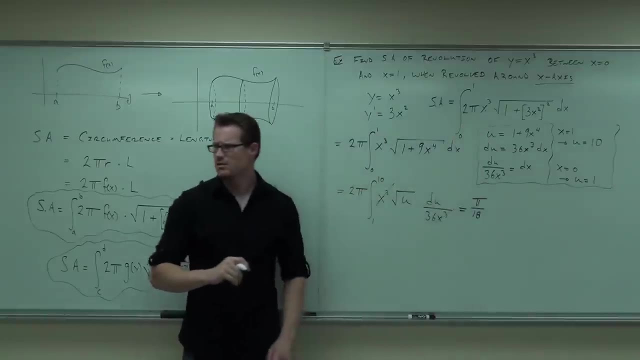 You have a 2 over 36.. What you're going to have up front is pi over 18.. You're going to have pi over 18.. So combine those two fractions: Still an integral 0 to 1.. Not 2 to 1, 1 to 10.. 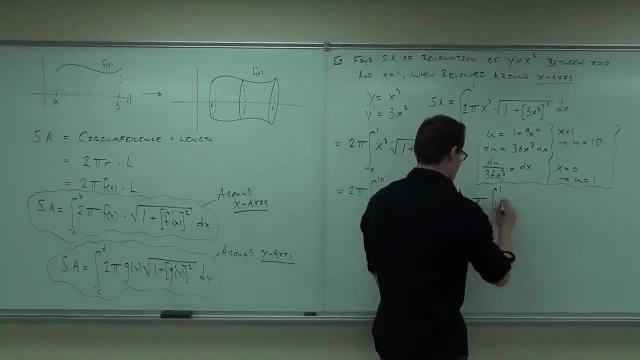 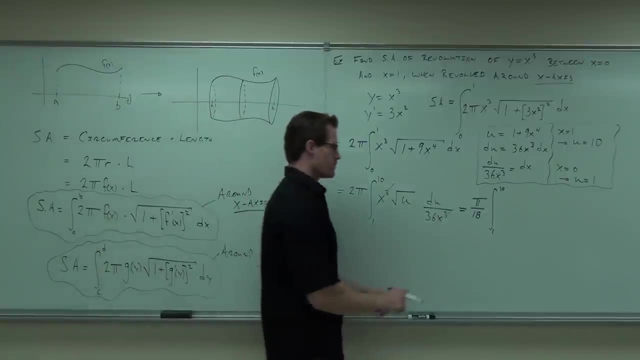 Oh, what's that? So it's actually testing you. Good job Turn. You'll never know. 1 to 10.. What's on the inside of our integral 1 and 1 half? Good, OK, So we've got to make sure it fits our integration table. 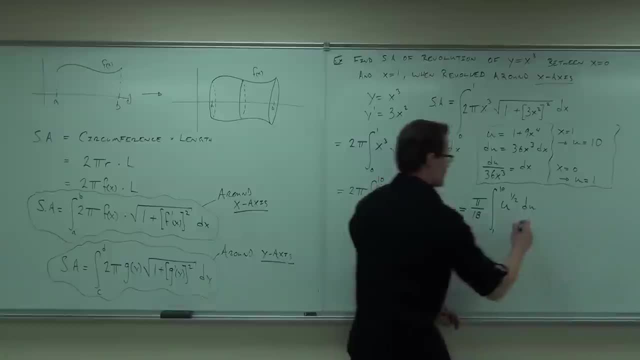 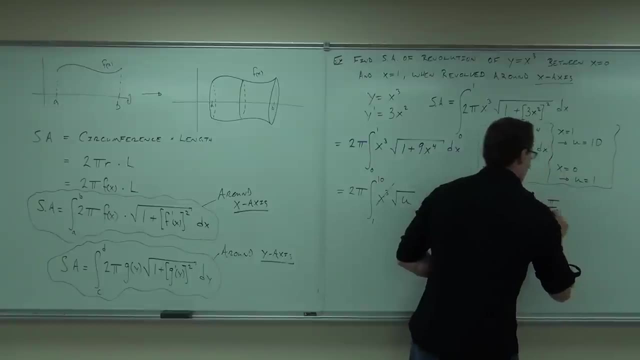 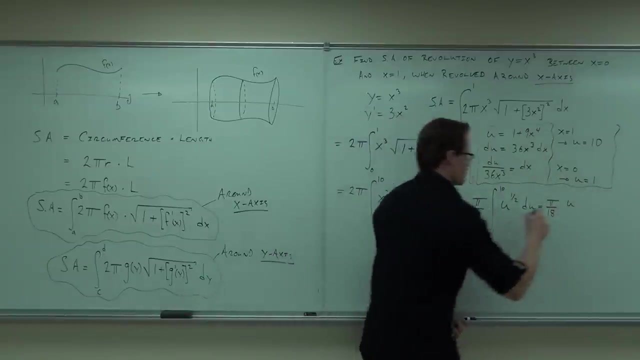 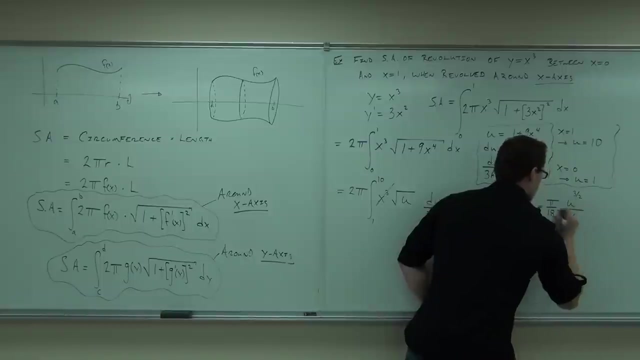 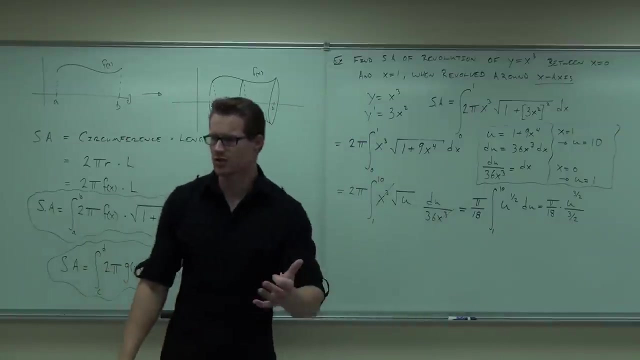 And we're in du, which is great for us. So pi over 18, u to the? u to the over. so pi over 18 times u to the, 3 halfs over 3 halfs. Of course, we're going to make that fraction look better. 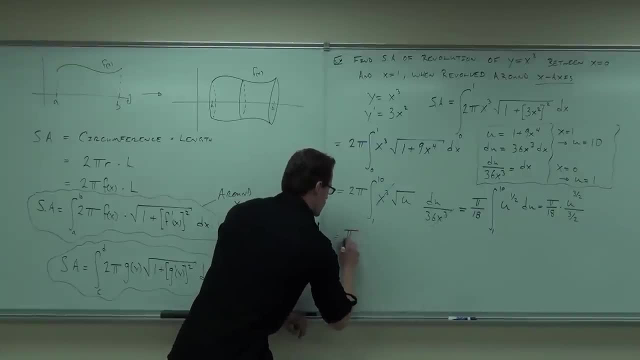 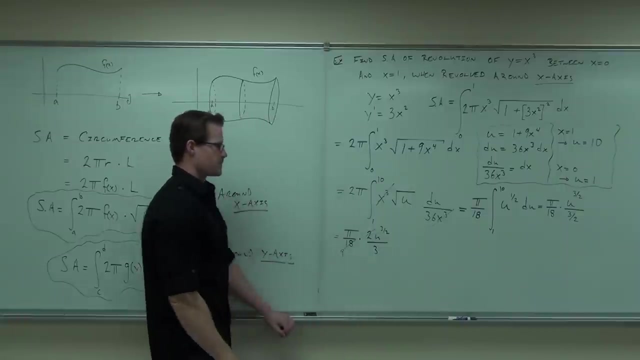 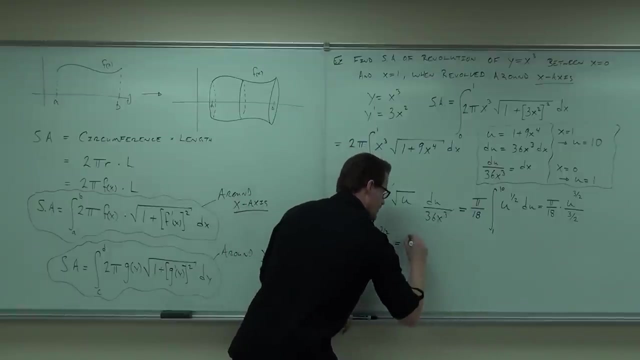 We're going to make this, So I'll do it in two steps: Pi over 18,. 2u to the 3 halfs over 3.. Just fine, We can simplify the 2 with the 18.. We'll end up getting pi over 27,. u to the 3 halfs. 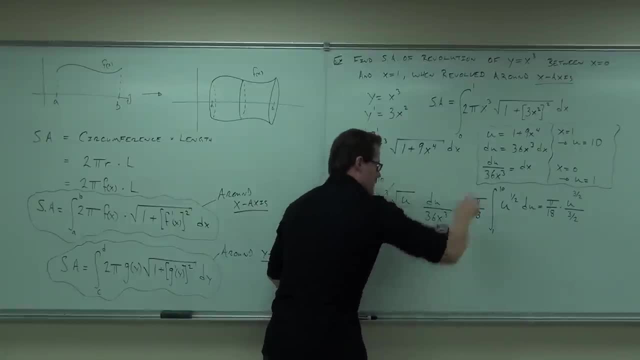 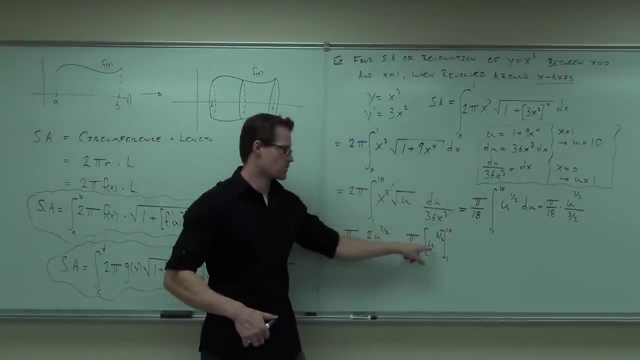 And we'll be going. We'll be going from 1 to 10, as our integral said we would. Can you please explain to me why I am not plugging this back into here before I'm evaluating, Because you changed bounds. I did change bounds. 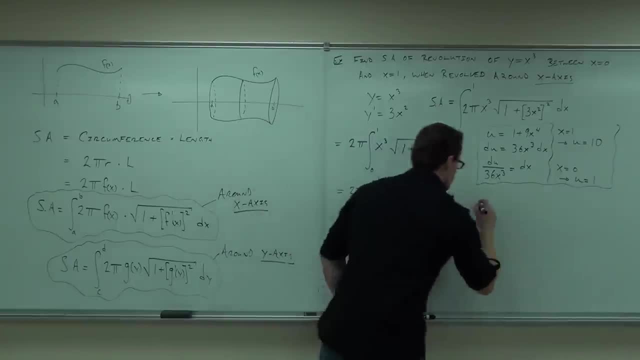 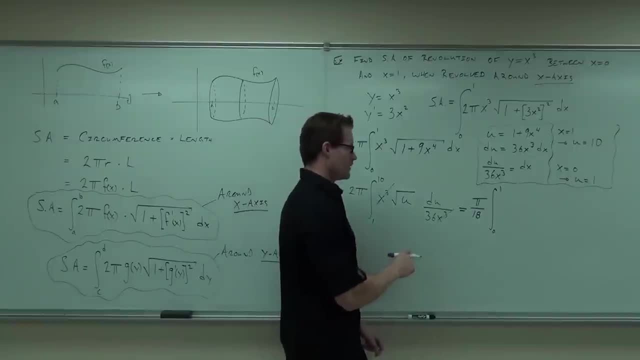 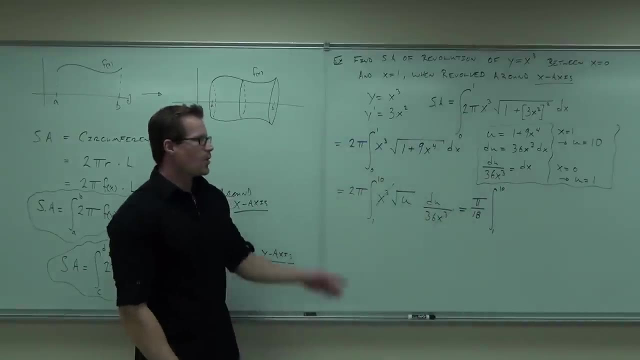 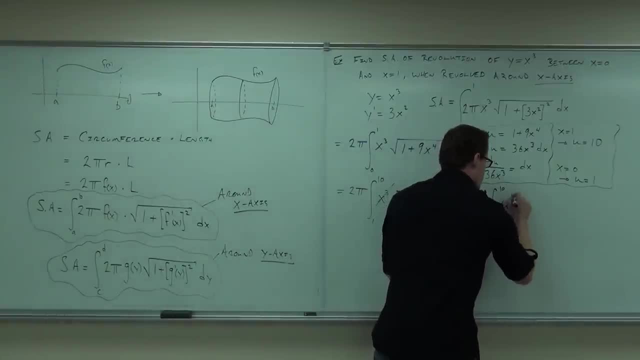 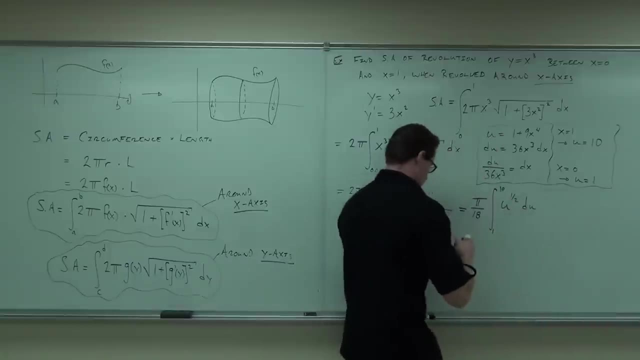 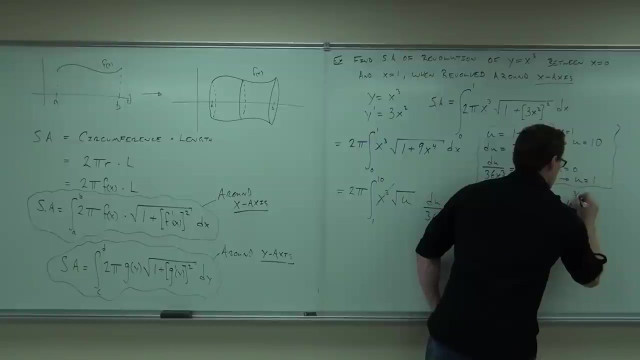 Good, Okay. So we've got to make sure it fits our integration table And we're in du, which is great for us. So pi over 18.. U to the? U to the Two, over two-thirds, over four-thirds. 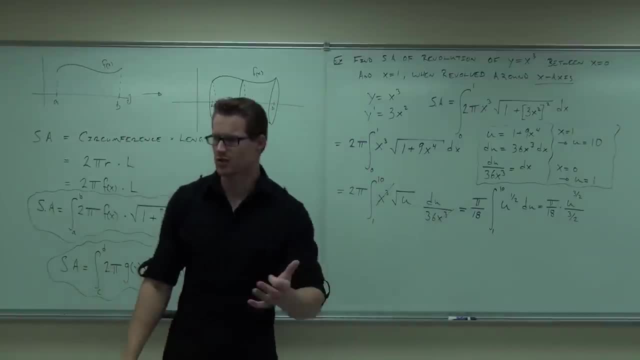 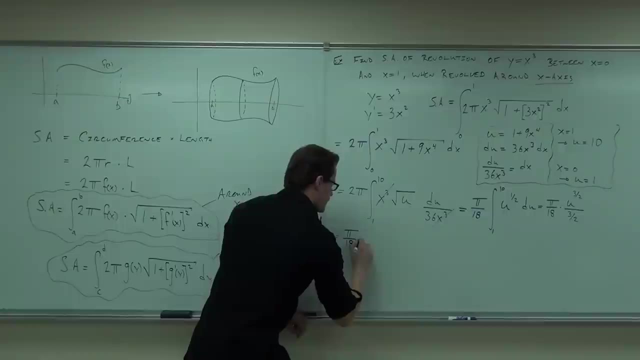 So pi over 18 times u to the three-halves over three-halves. of course we're gonna make that fraction look better. We're gonna make this. I'll do it in two steps: Pi over 18, two: u to the three-halves over three. 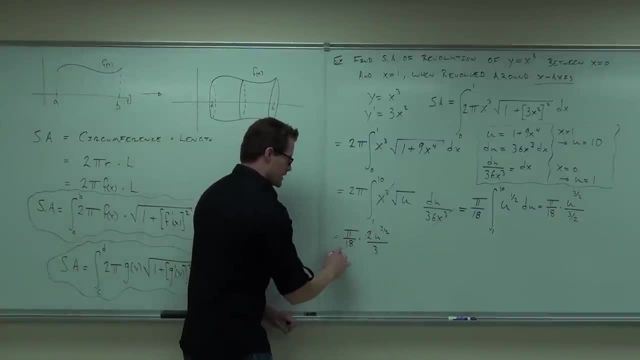 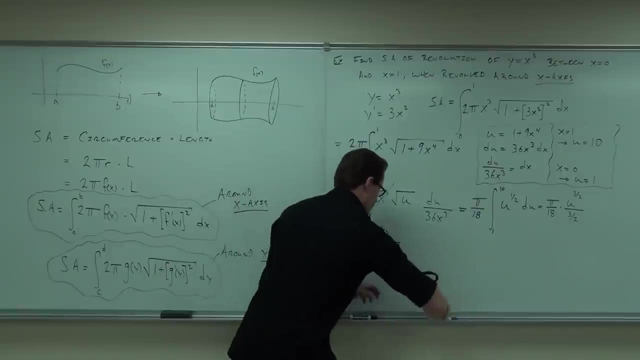 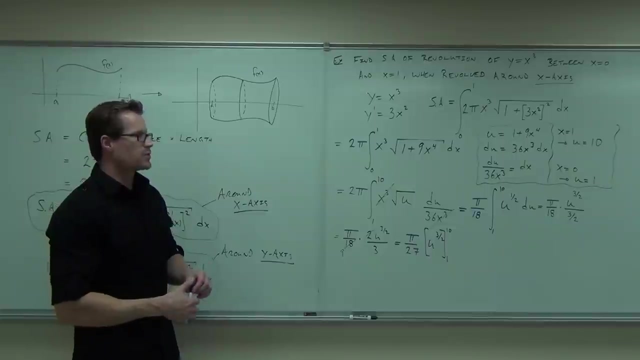 just fine, We can simplify the two with the 18. We'll end up getting pi over 27, u to the three-halves and we'll be going from one to 10, as our integral said we would. Can you please explain to me why I am not plugging this? 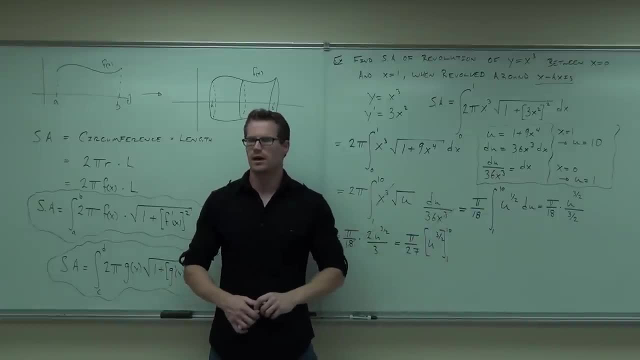 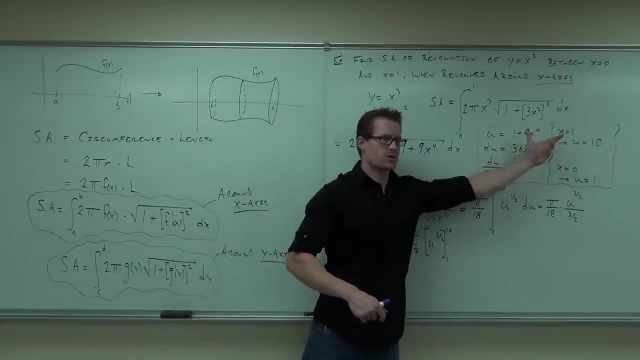 back into here before I'm evaluating. I did change bounds. If I hadn't changed bounds, that is what I would be doing right now. You gotta take care of this operation somewhere. It's either before you do the integral or after, but somewhere it's going to happen. 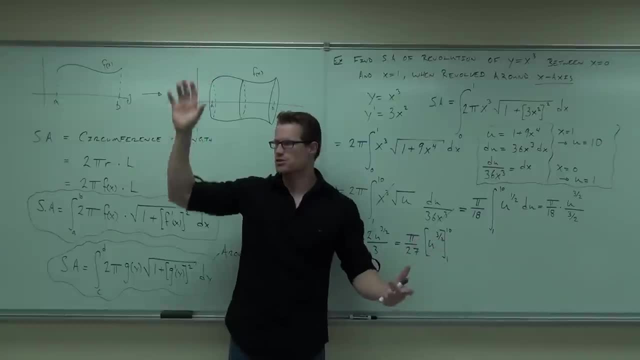 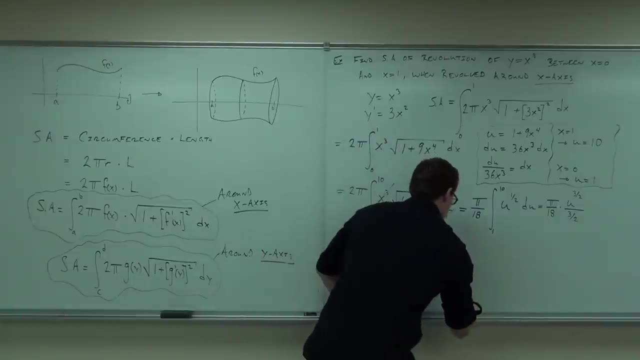 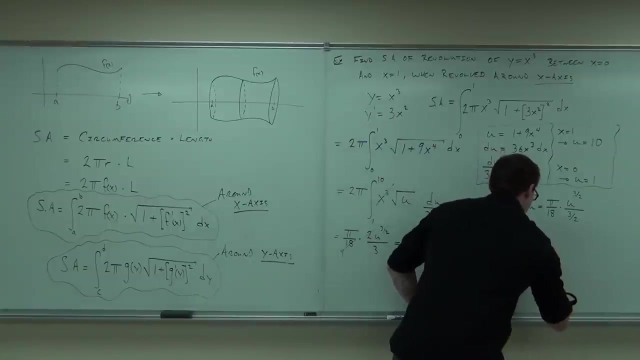 Let's show hands how people feel okay with the calculus. Basically done with the calculus, Now just evaluate. We're gonna take 10 to the three-halves minus one to the three-halves. 10 to the three-halves is going to be 10 to the 10.. 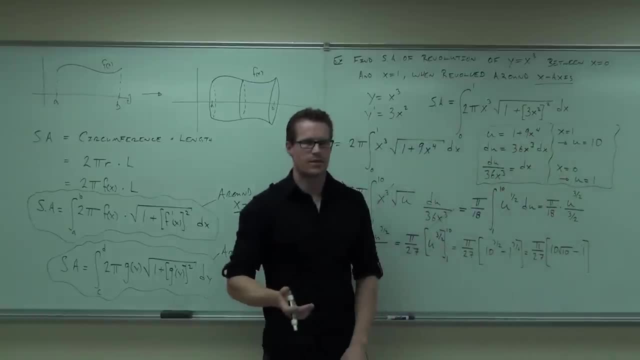 Minus one. There's a variety of ways you can write that. You can write that 10 pi root 10 over 27 minus pi over 27. for right now it's just a tree For right now. can you just verify that? this is okay. 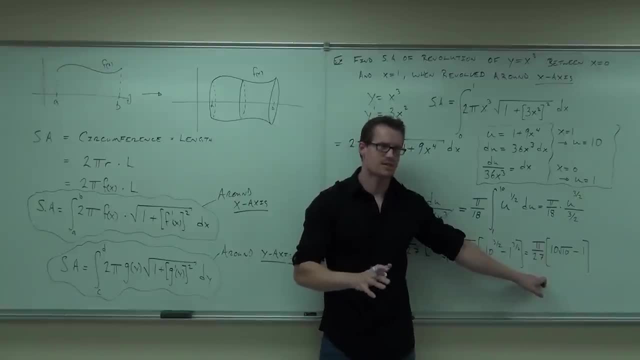 and leave it like that for me. Do you feel okay with leaving it like that? It's just as valid. it's as simple as we can make. the radical 10 root 10 minus one. You can't take anything away from that. 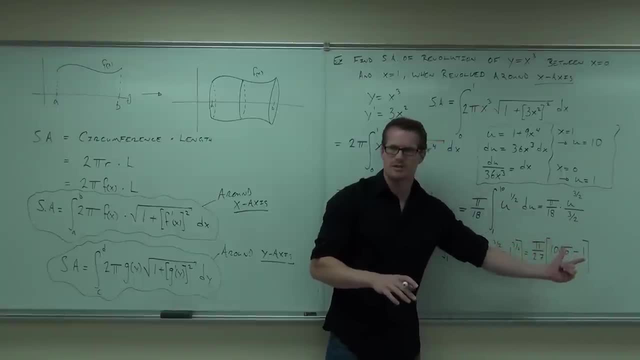 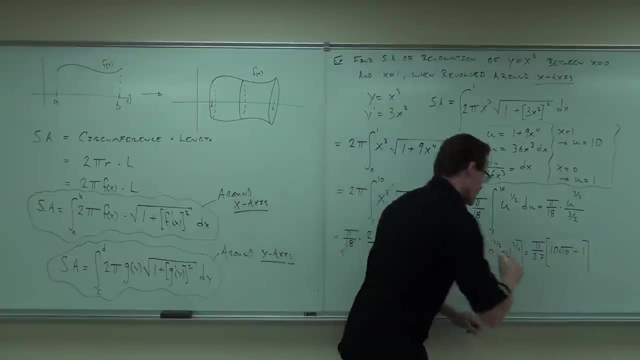 What you could do is just distribute in that pi over 27, and that's about as good as you could get. You get 10 pi root, 10 minus pi all over 27.. So the other way would be: for some reason this looks prettier than that to me. 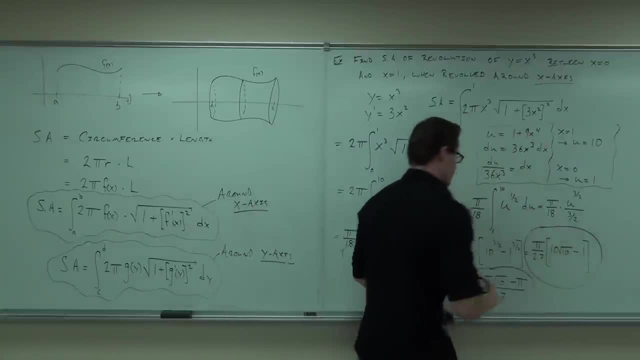 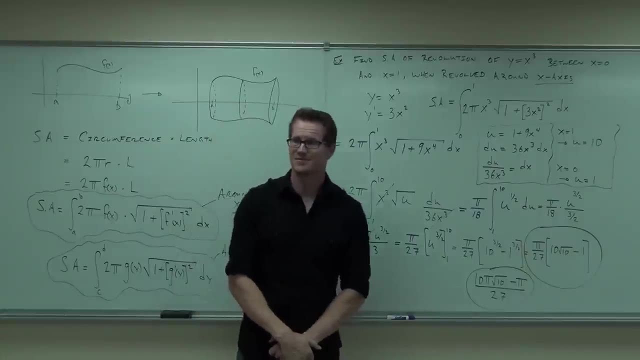 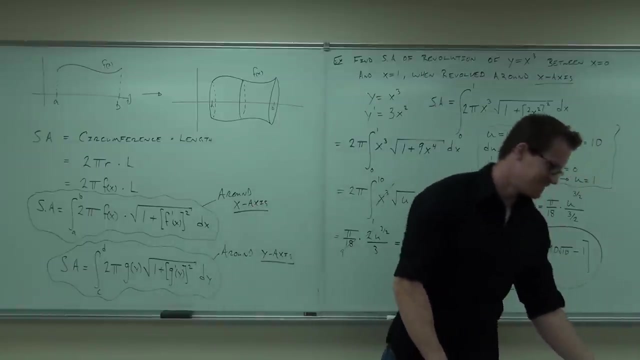 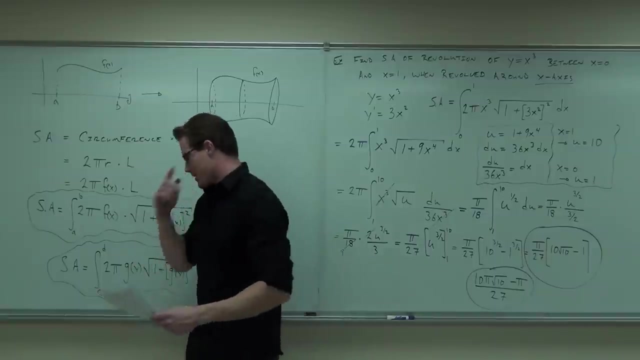 So either way, Yes or no, Feel okay with it. Would you like to try one more? You guys like it? No, Not too bad though, is it Not too bad? Not too bad. at least The integrals have to work out, which is nice. 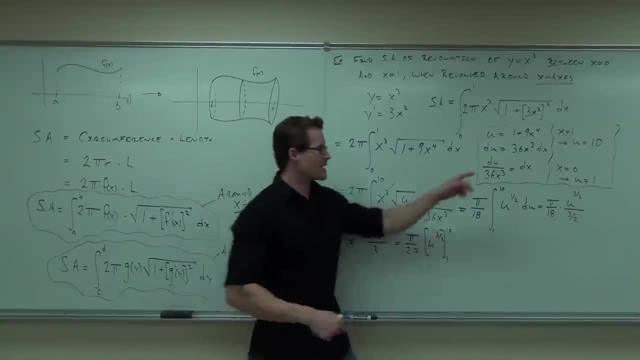 If I hadn't changed bounds, that is what I would be doing right now. You've got to take care of this operation somewhere. It's either before you do the integral or after, But somewhere it's going to happen. Let's show hands. 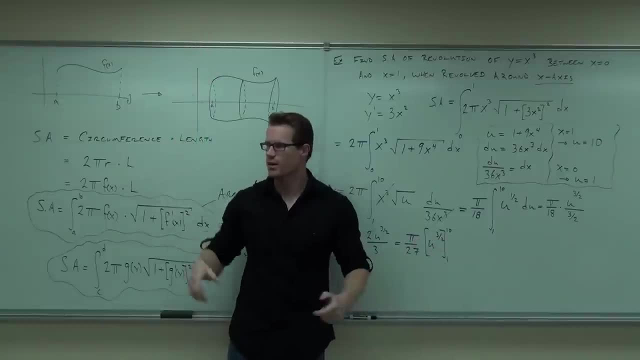 How many of you will be OK with the calculus? Basically done with the calculus, Now just evaluate. We're going to take 10 to the 3 halfs, 2. Minus 1 to the 3 halfs. Minus 1 to the 3 halfs. 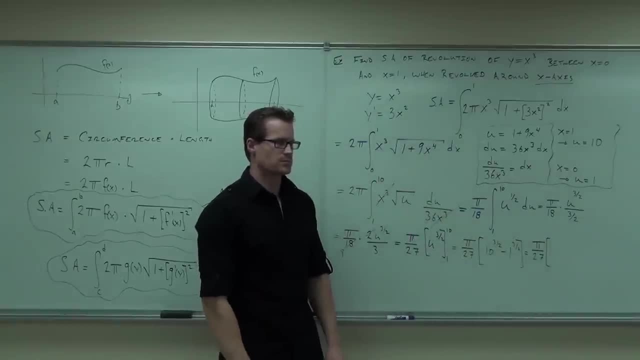 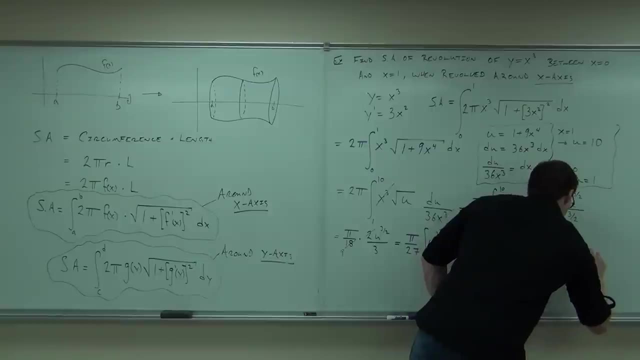 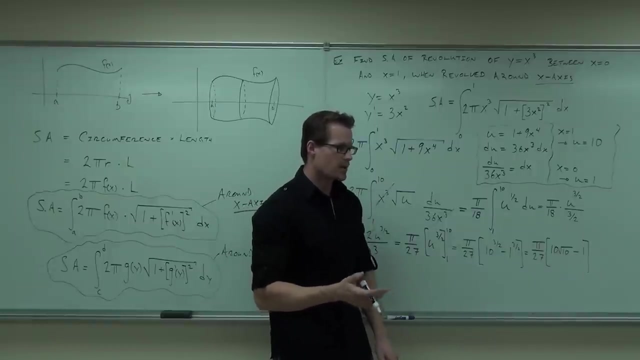 10 to the 3 halfs is going to be 10 to the 10. Minus 1.. There's a variety of ways you can write that. You can write that 10 pi root 10 over 27 minus pi over 27.. 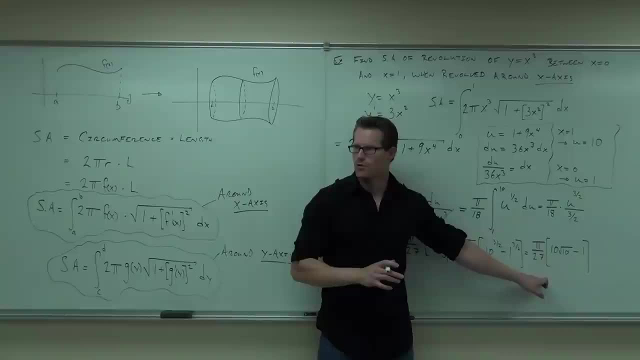 For right now. can you just verify that this is OK and leave it like that for me? Do you feel OK with leaving it like that? It's just as valid. It's as simple as we can make. the radical 10 root 10 minus 1.. 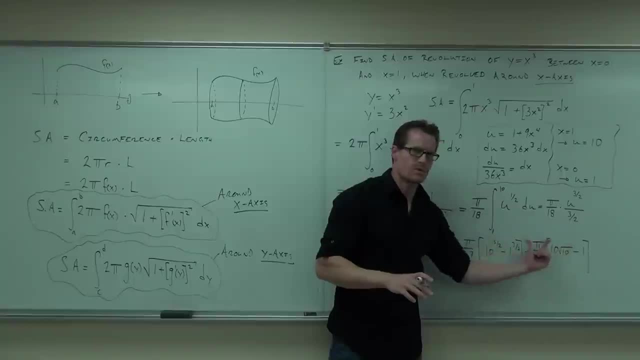 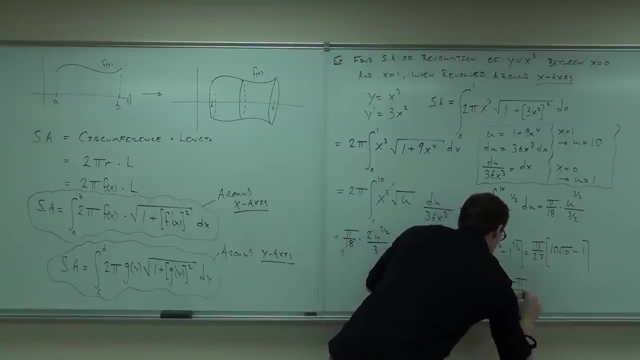 You can't take anything away from that. What you could do is just distribute in that pi over 27,. and that's about as good as you could get. You get 10 pi root, 10 minus pi all over 27.. So the other way would be: for some reason this looks prettier than that to me. 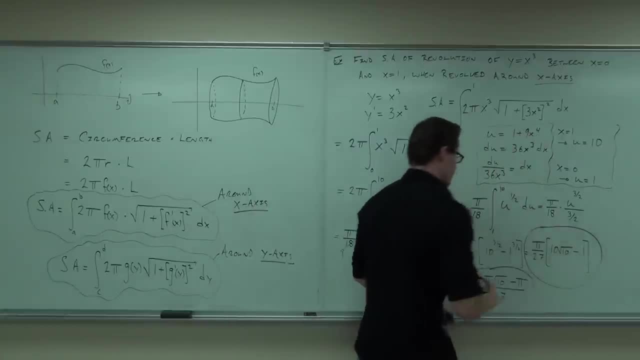 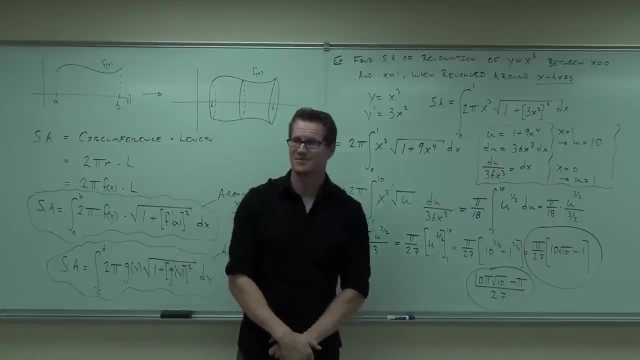 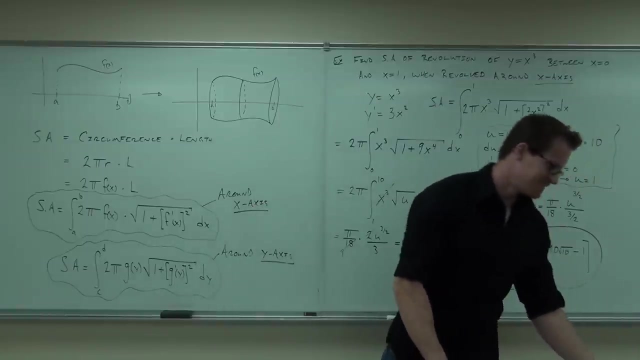 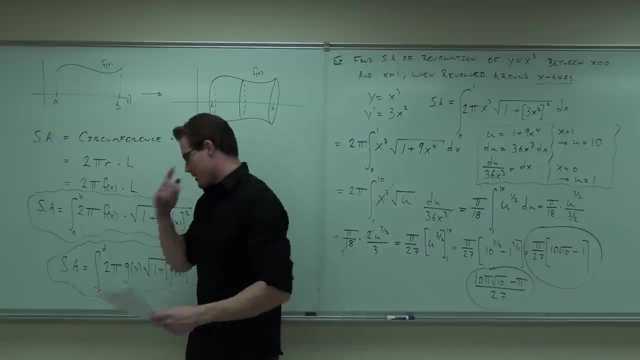 So, either way, Yes, no, Feel OK with it. No, Would you like to try one more? You guys are allowed to do it. Not too bad though, is it Not too bad? Not too bad at least. 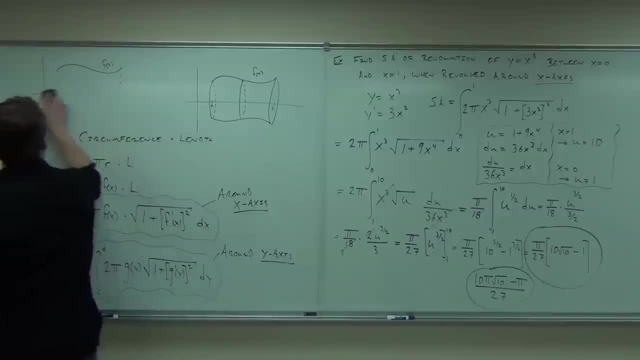 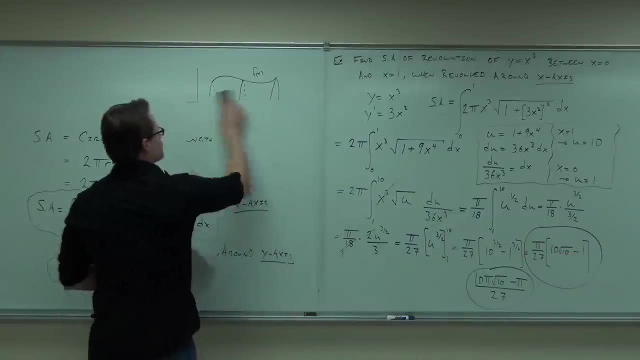 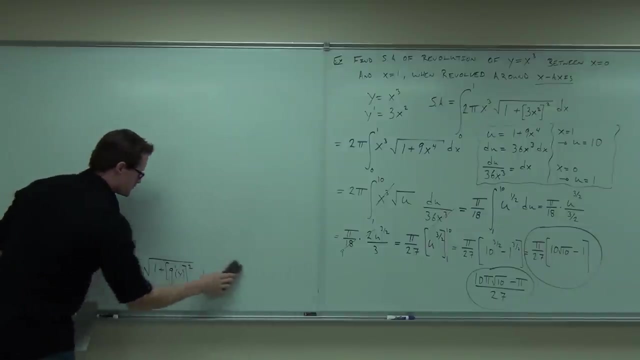 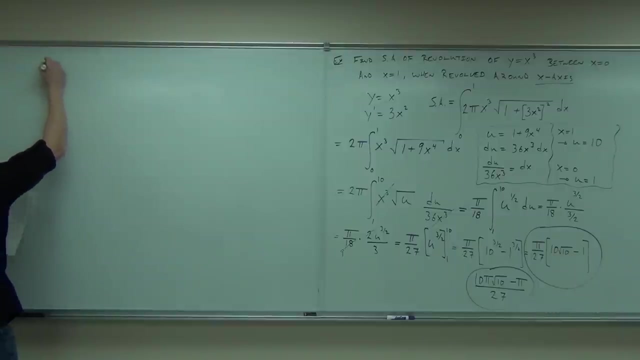 The integrals have to work out, which is nice. Are there any more questions on the exclamation before I erase it? No, no, OK, one more, Let's do the same thing. Find the surface area of revolution of Y equals X squared. 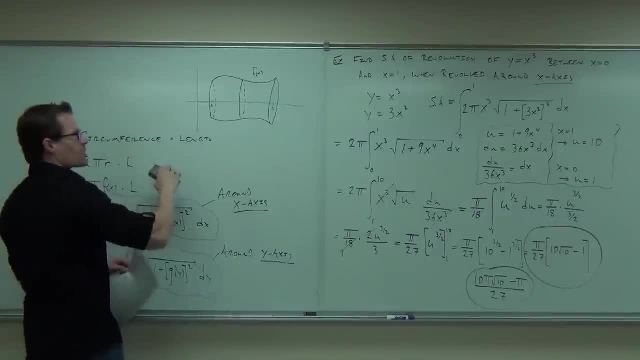 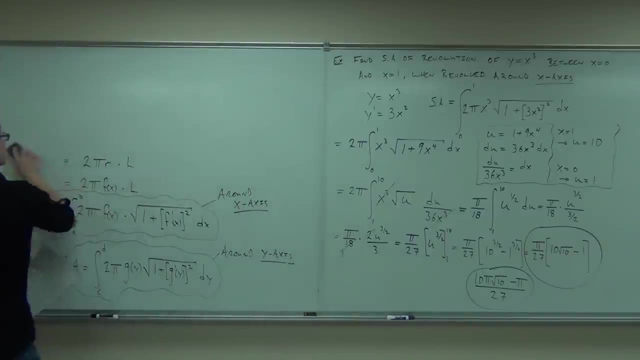 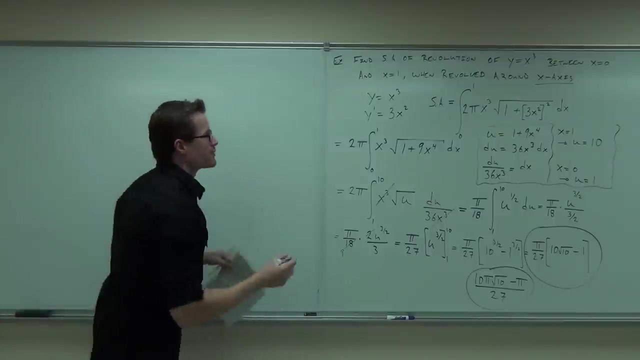 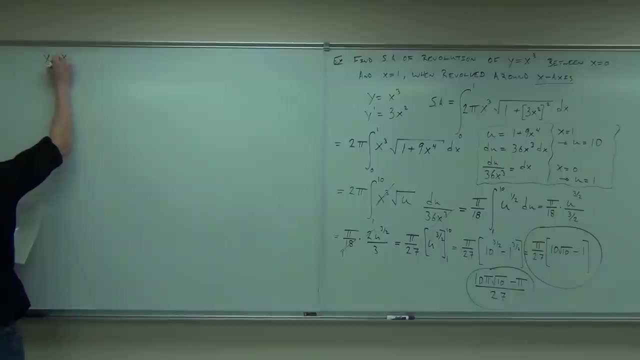 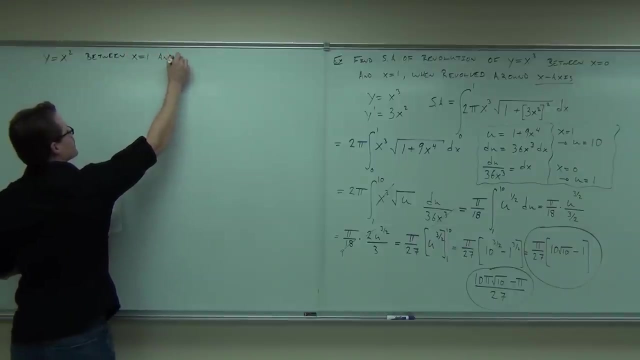 I realize Are there any more questions on the exclamation before I erase it. Okay, one more. Let's do the same thing. Find the surface area of revolution of Y equals X squared between X equals one And x equals 2 around the y-axis. 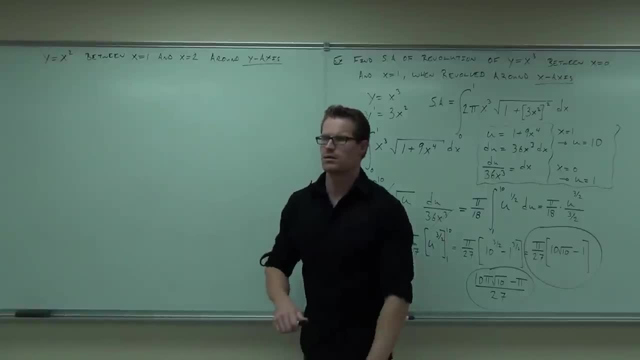 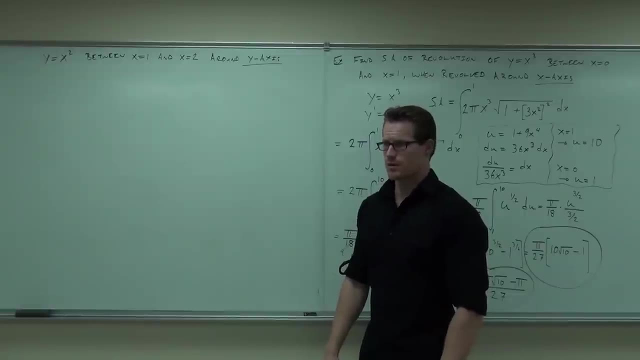 Is someone on the right-hand side, my right-hand side, tell me what's wrong? What's wrong right now? It's in terms of x, And what do we need it to be in terms of? For the surface area of revolution? that's exactly correct. 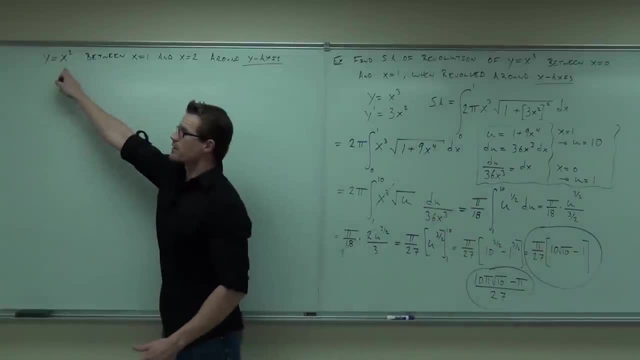 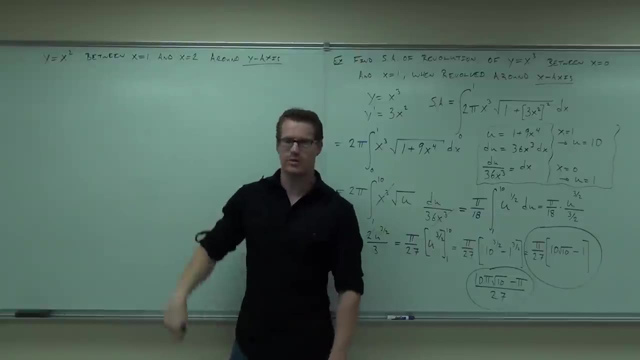 So right now we have some problems up here. We have in terms of x, we have O, x and x and y. those things don't match up. So you're going to have to do a little translation. Notice that area between two curves. it's whatever axis you're relating it to. that's what your variables have to be in. 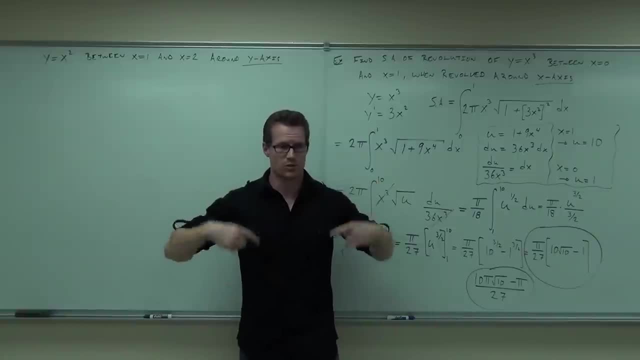 Same thing with disk and washer. Same thing with surface area of revolution. Only one's not like that. This is a numerical shell, so be careful on this. This is not set up for around the y-axis. How do we set it up for around the y-axis? 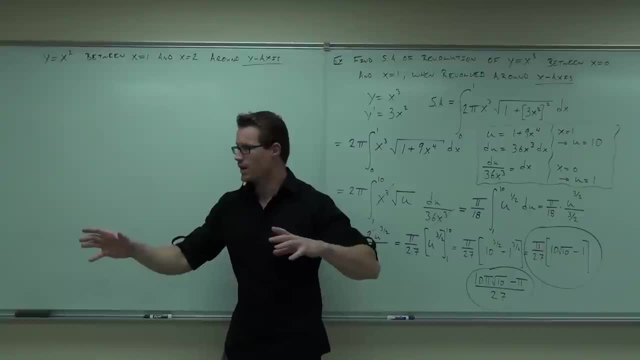 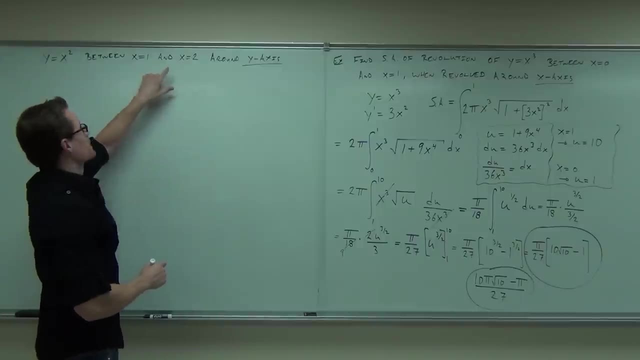 Solve for x, put it in terms of y. that's the same thing. So the first step: you know what I'm going to deal with these before I get too crazy on this stuff. How can I change x's into y's? 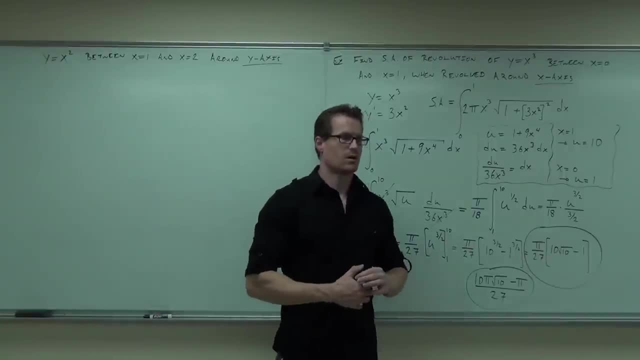 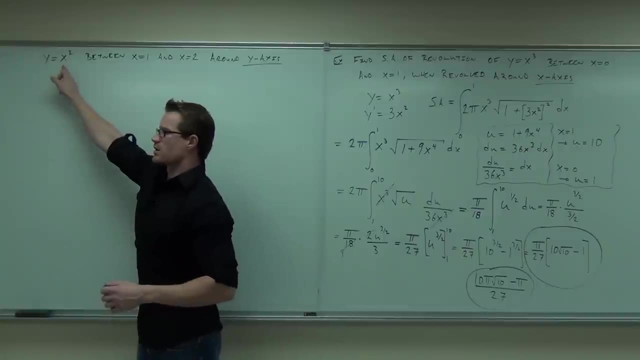 Say what? Y-square them. Okay, great, So square them, because when I plug them into my function, that's what I'm going to get. Notice it says y equals x-squared. It's giving you x's, Just plug them in. 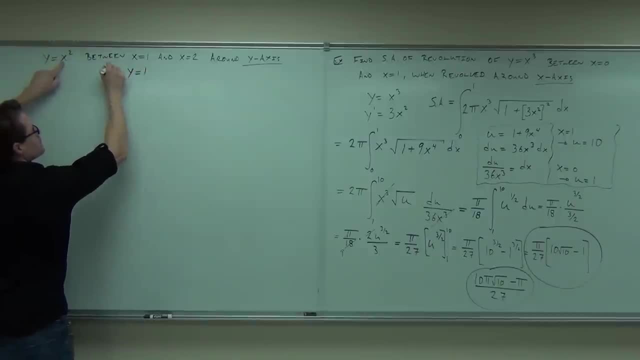 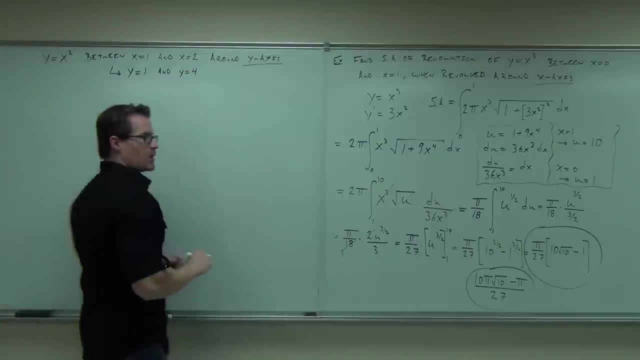 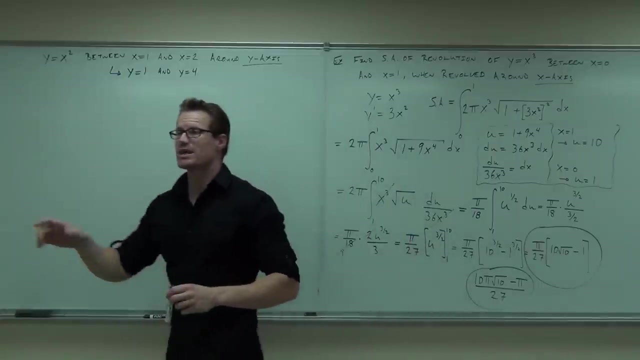 If x equals 1,, then y equals 4.. And if x equals 2,, then y equals 4.. Perfect, Now we have bounds in terms of y. Still, okay, Alright, let's continue. How do we get in terms of y? 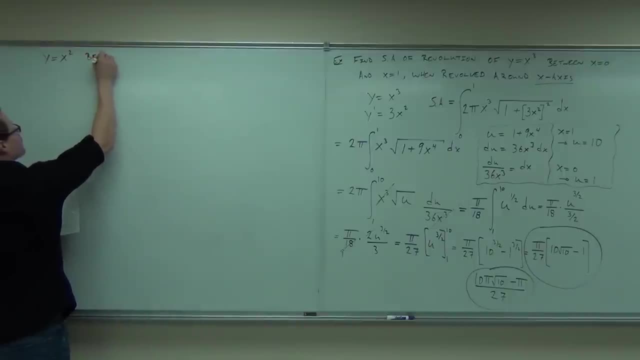 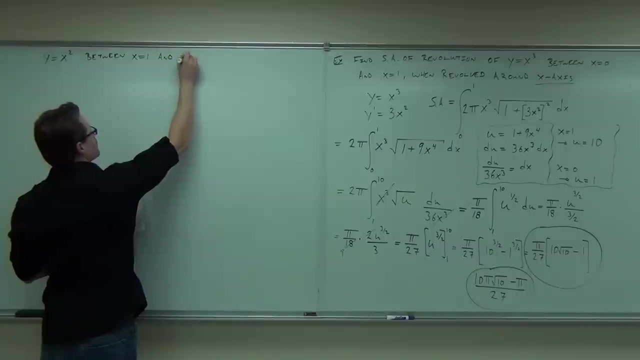 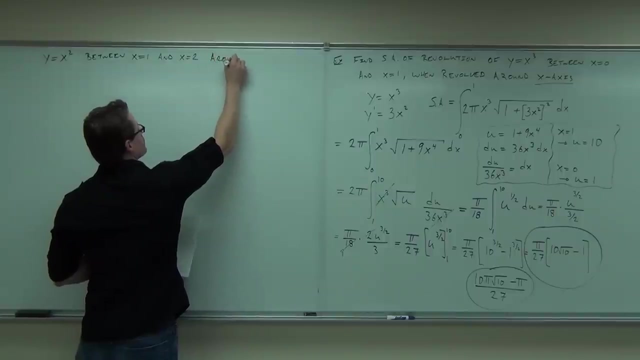 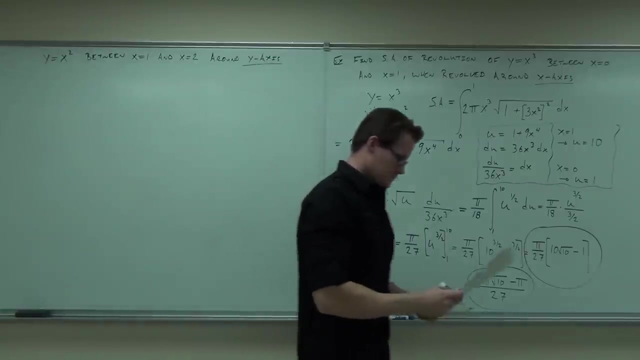 I'm sorry. I should have written that first. I made a mistake Between x equals 1 and x equals 2 around the y-axis. Is someone on the right-hand side- my right-hand side- tell me what's wrong? What's wrong right now. 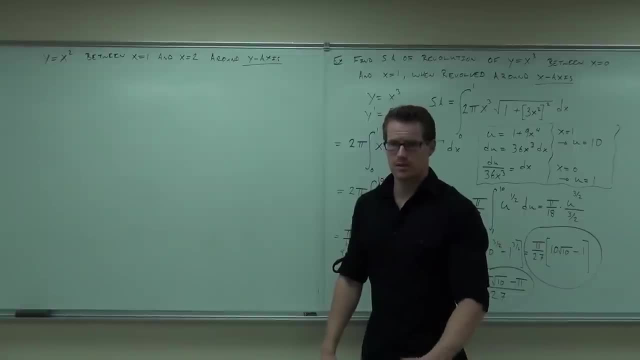 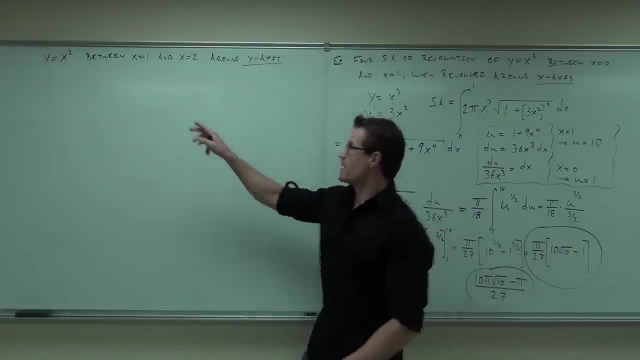 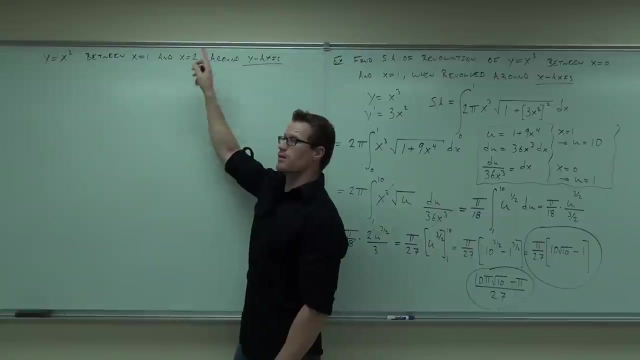 It's in terms of x, and what do we need it to be in terms of Y For the surface area of revolution. that's exactly correct. So right now we have some problems up here. We have in terms of x, we have O, x and x and y. 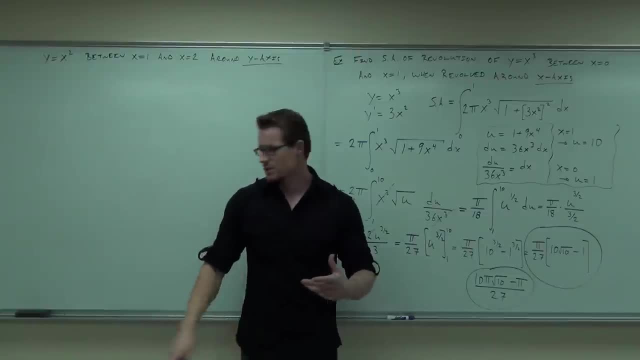 Those things don't match up, So you're going to have to do a little translation. Notice that area between two curves. it's whatever axis you're relating it to. that's what your variables have to be. in Same thing with disk and washer. 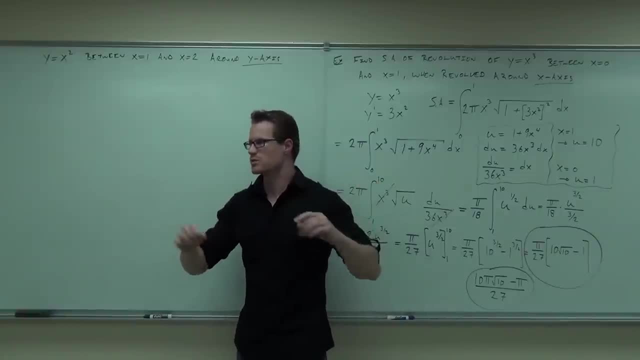 Same thing with surface area of revolution. The only one that's not like that again is cylindrical shells. Be careful on this. This is not set up for around the y-axis. How do we set it up for around the y-axis? 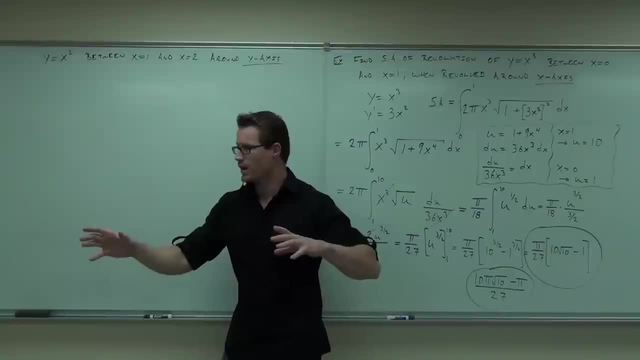 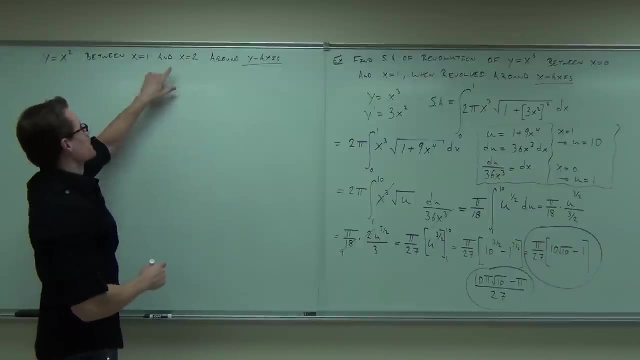 Solve for x. put it in terms of y. that's the same thing, okay, So the first step: you know what I'm going to deal with these before I get too crazy on this stuff. How can I change x's into y's? 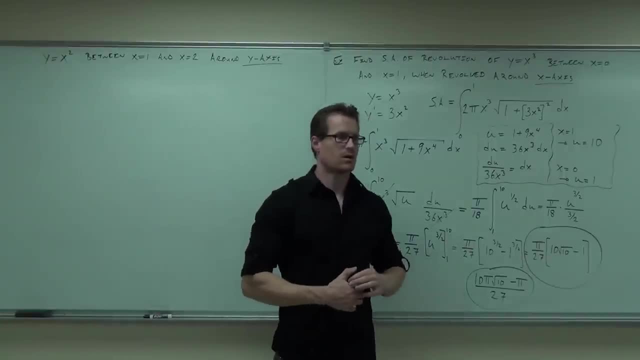 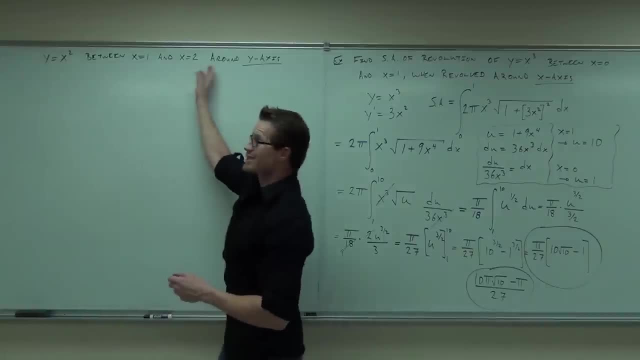 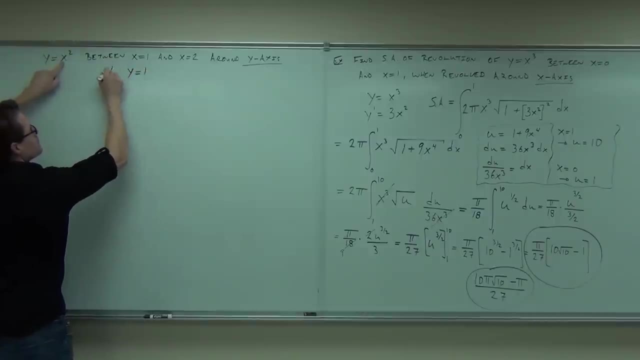 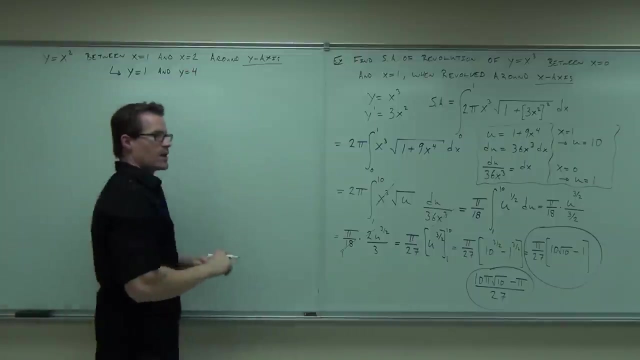 Notice: it says y equals x squared. It's giving you x's, Just plug them in. If x equals 1, then y equals, and if x equals 2, then y equals 4.. Perfect, Now we have bounds in terms of y. 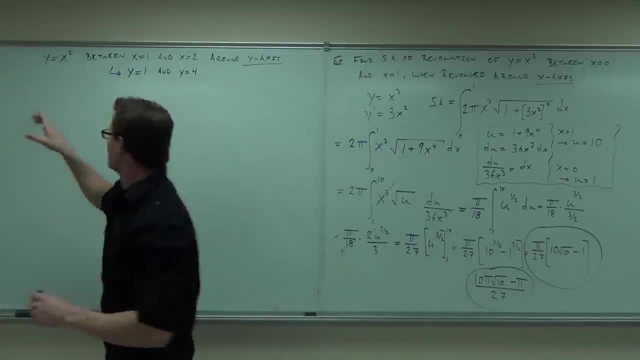 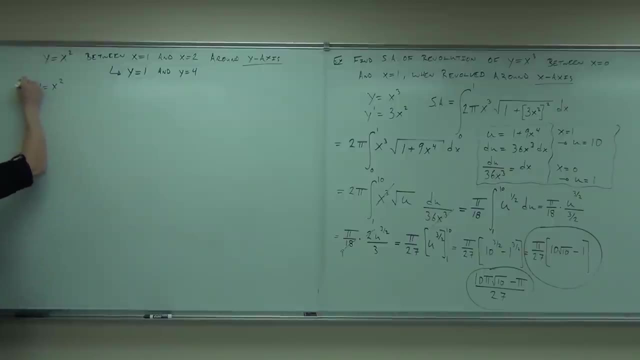 Still okay. Yeah, All right, let's continue. How did we get? in terms of y, if we do square root, we have y equals x squared. take a square root of both sides with a plus and minus and you get x equals the square root. 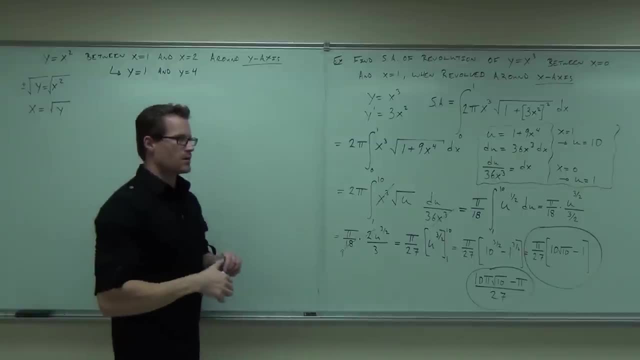 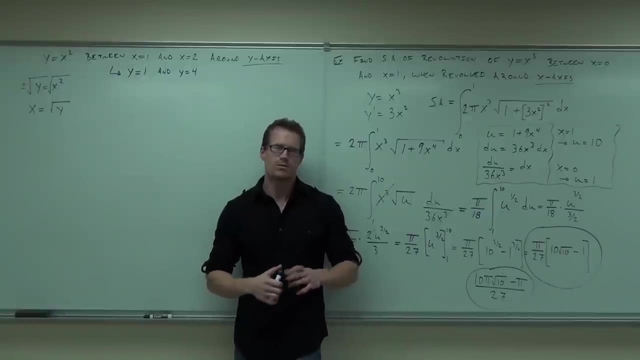 of y plus and minus, Don't forget. Well, explain to me why I can forget the minus here. Surface area: You can't make it a surface area, Not quite that. That's where you're talking about. 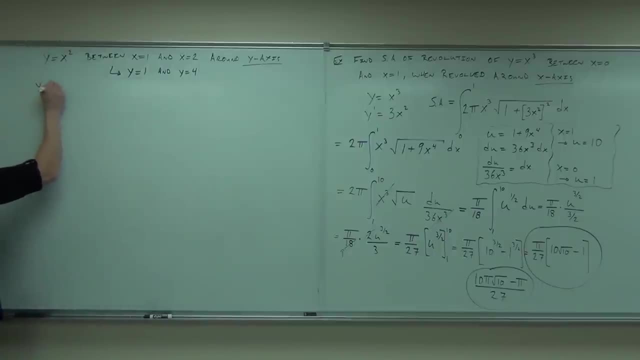 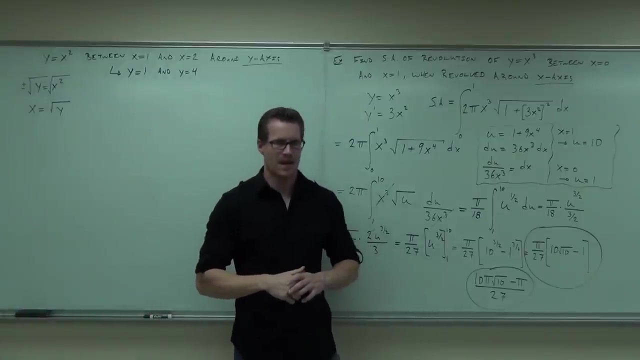 If we do square root, we have y equals x-squared. Take a square root of both sides with a plus and minus and you get x equals the square root of y, plus and minus. Well, explain to me why I can forget the minus here. 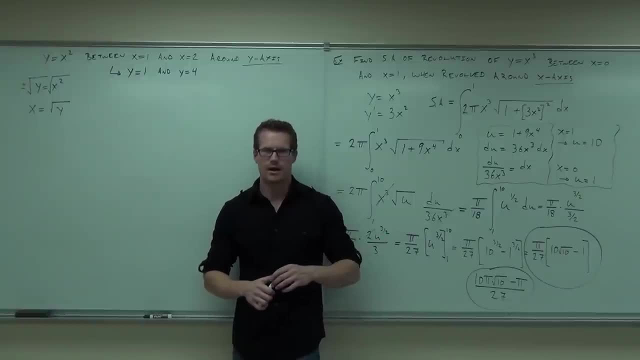 Surface area? Not quite that. That's where you're talking about, where the functions, where the things that carry that. Okay, Well, firstly, because, firstly, it's this: If I'm revolving x-squared around the y-axis, I only need half of it. 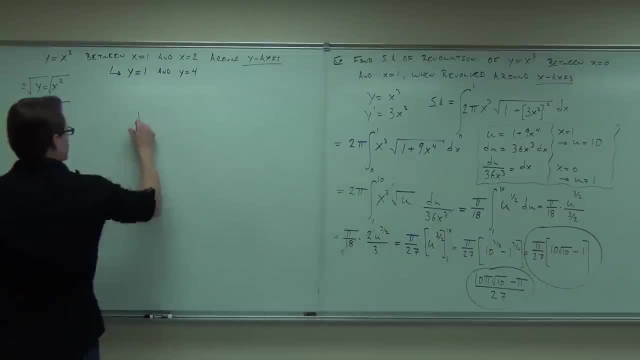 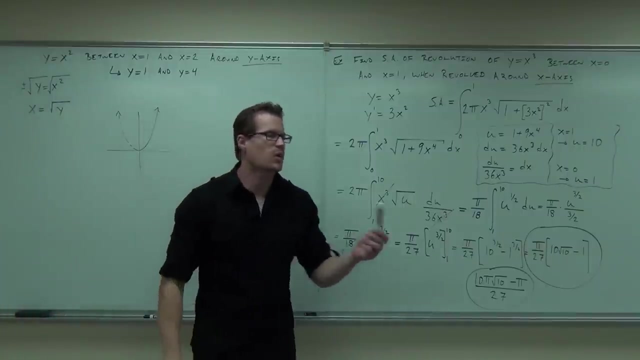 So if I'm revolving a whole, You realize that's my picture, right? I'm taking this thing and spinning it this way. Won't half of it make the same shape as the whole thing? Plus, think about my- yeah, think about my- bounds, my original bounds. 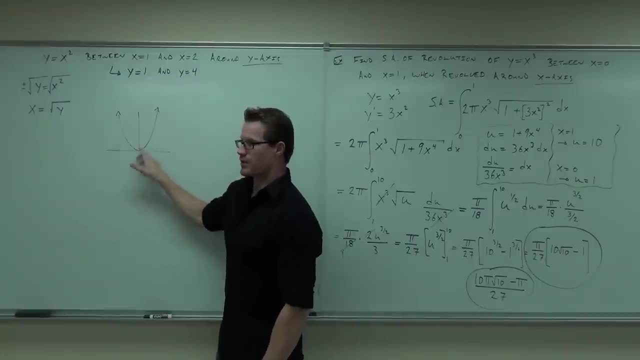 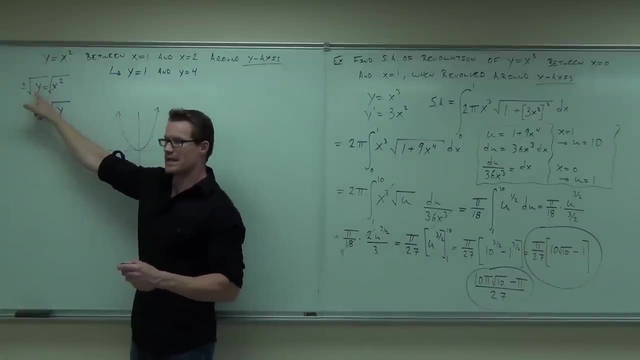 I'm talking between x equals 1 and 2. That doesn't have this part of it. That's just this part of it, not this over here. So it's saying: yes, this would be mathematically correct. However, it's out of the bounds of my integration. 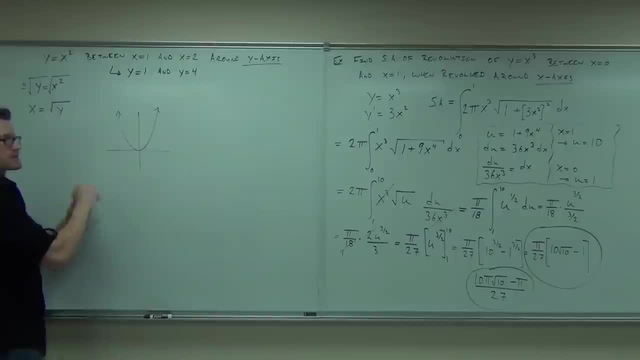 My function's not even defined right there for this integral, so I don't need this half. I don't need the negative part of that. Did you understand that logic? Okay, So we don't need that, just to answer a question you might not have even had. 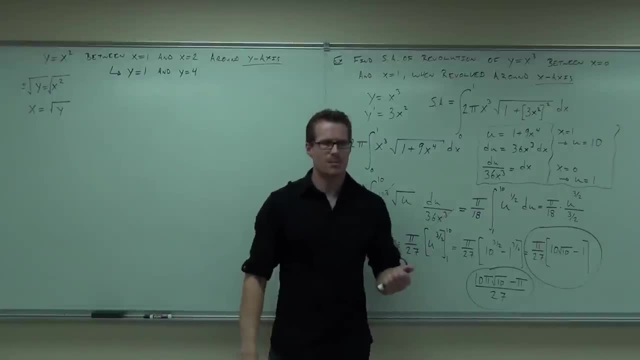 But there it is. Are we set up? We're going around the y-axis. It's now in terms of y, that's great. We have our bounds. in terms of y, We should be about ready to set up our integral. Just tell me one more thing we gotta do before we get to our integral. 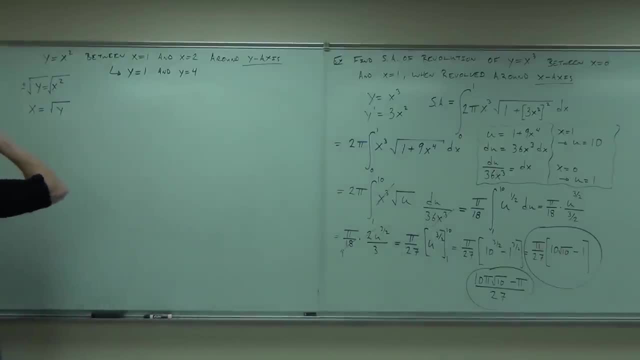 Let's take the derivative. What is my derivative? 1 times the y, times the negative of that. Perfect Yeah, exactly right, Excuse me. So since we're looking for surface area revolution, we know it's around the y-axis- let's put everything in terms of y. 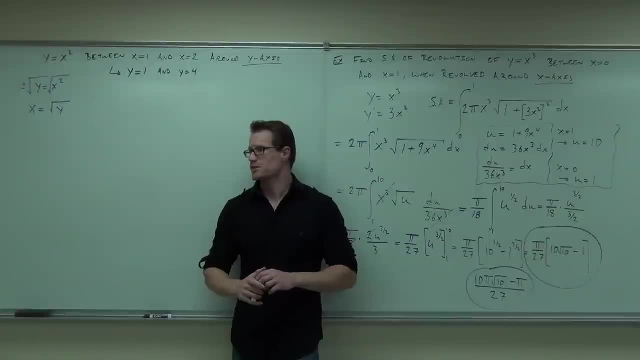 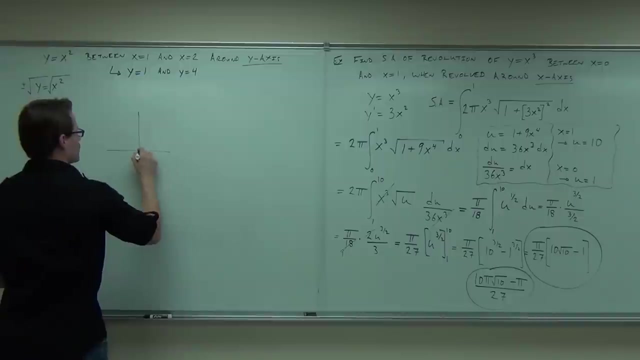 Okay, Well, firstly, because? first is this: If I'm revolving x squared around the y axis, I only have a bit, So I'm going to hold. You realize that's my picture, right? I'm taking this thing and spinning it this way. 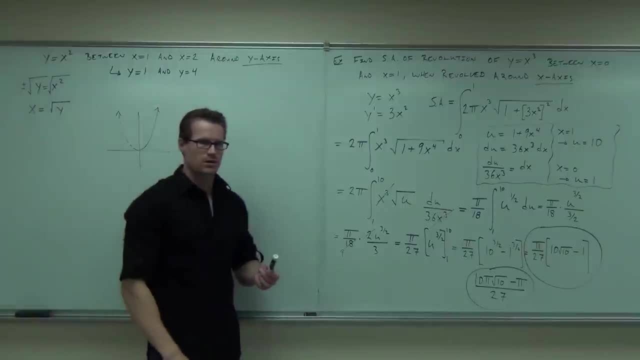 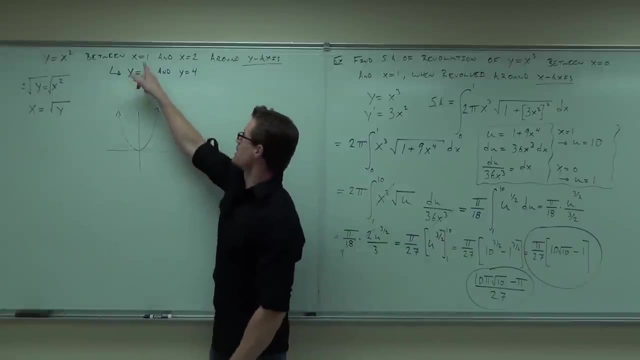 Won half of it, make the same shape as the whole thing. Plus, think about my- yeah, think about my bounds, my original bounds. I'm talking between x equals 1 and 2.. That doesn't have this part of it. 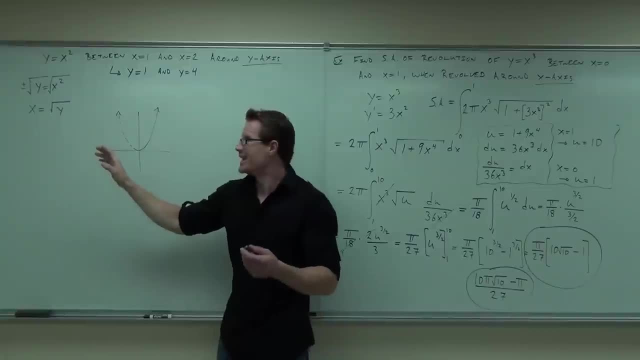 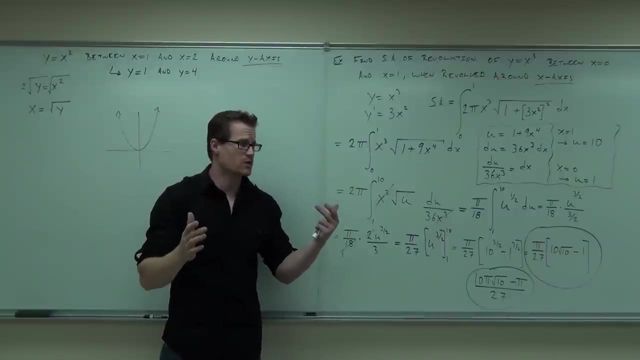 That's just this part of it, not this over here. So it's saying: yes, this would be mathematically correct. However, it's out of the bounds of my integration. My function's not even defined right there for this integral. 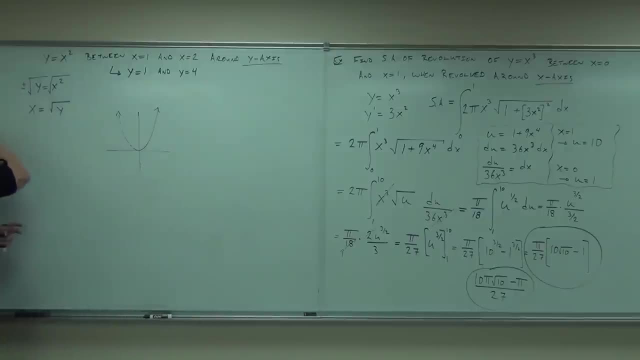 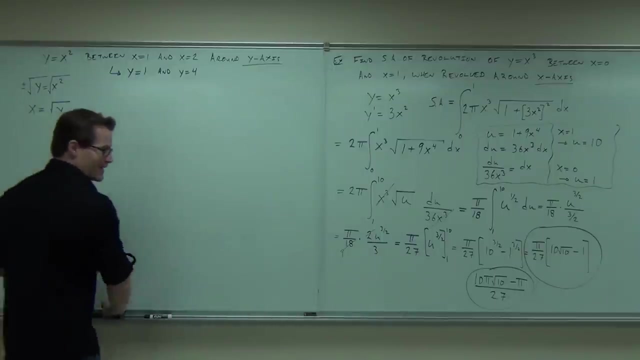 So I don't need this half. I don't need the negative part of that. Did you understand that logic? Okay, So we don't need that. That's just to answer a question you might not have even had, But there it is. 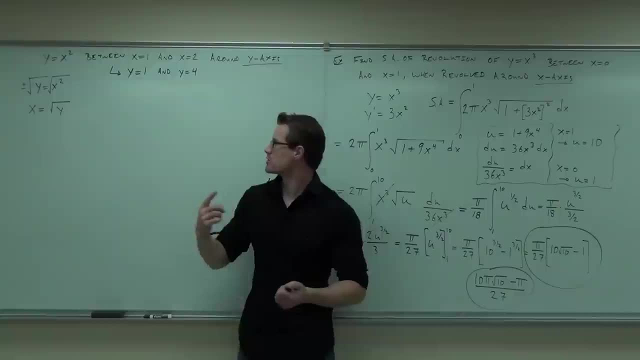 Are we set up? We're going around the y axis. It's now in terms of y. That's great. We have our bounds in terms of y. We should be about ready to set up our integral. Just tell me one more thing we got to do before we get to our integral. 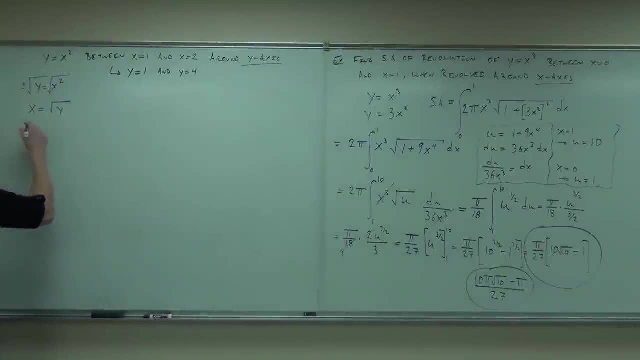 Let's take the derivative. What is my derivative? e 1.. 1 has the y in it. Perfect Yeah, exactly right. Excuse me So, since we're looking for surface area revolution, we know it's around the y axis. 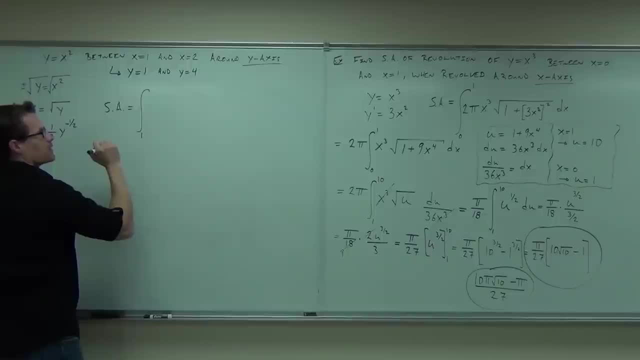 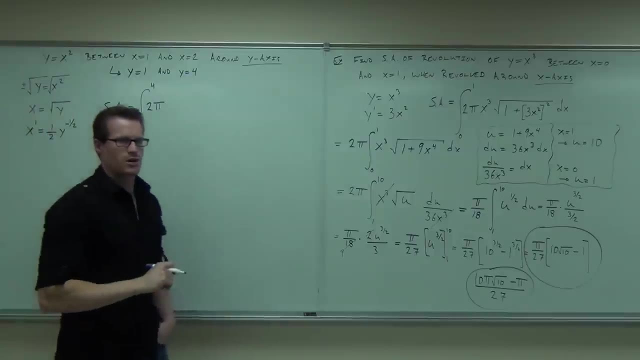 Let's put everything in terms of y. It goes from 1 to where 1.. Good, because we're going around the y, It has to be in terms of y. 2 pi has got to be there. What's the next thing I'm going to write next to the 2 pi? 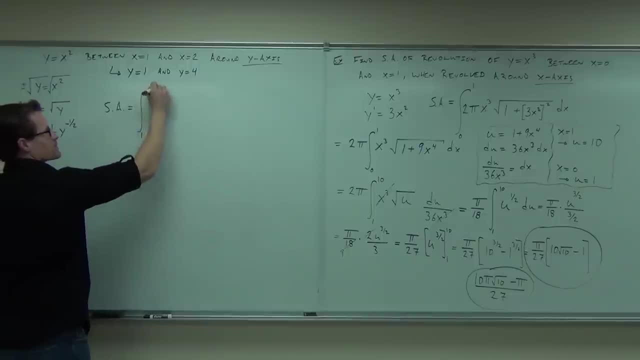 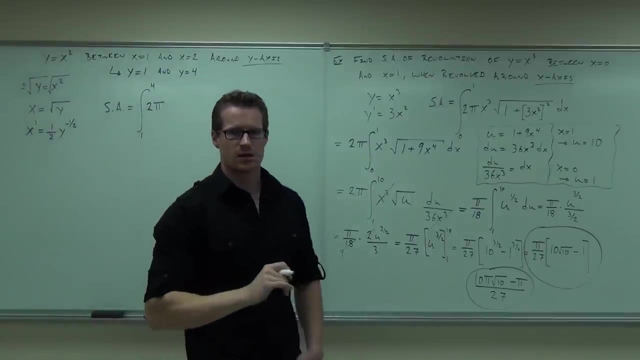 It goes from 1 to where 1.. Good, because we're going around the y, It has to be in terms of y. What's the next thing I'm going to write next to the 2 pi? Say what Square root of y. 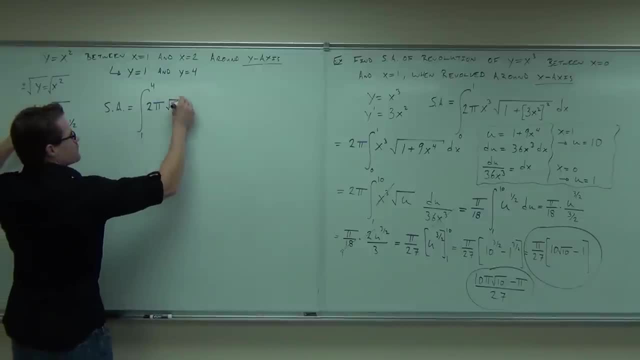 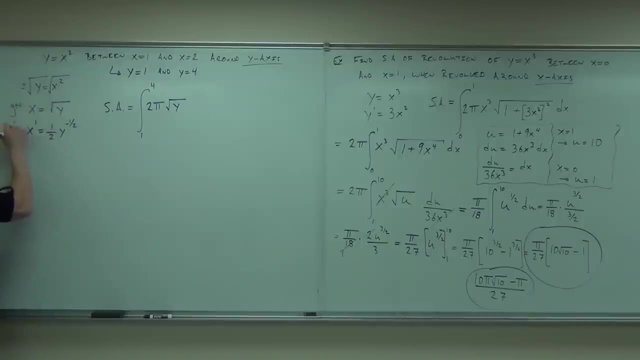 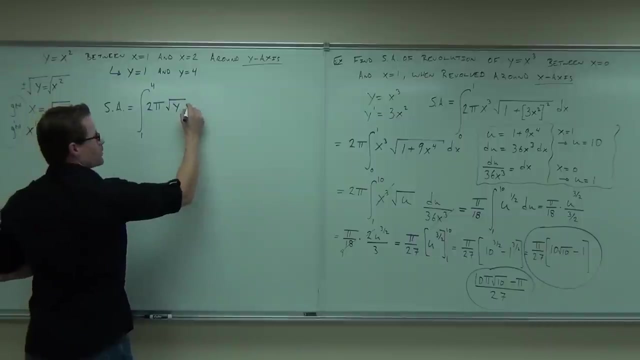 Square root of y because it's in terms of. It says: take the function in terms of y Before you take the derivative. this would be like g of y. This would be like g prime of y Function itself. Then we go ahead and we multiply by what? 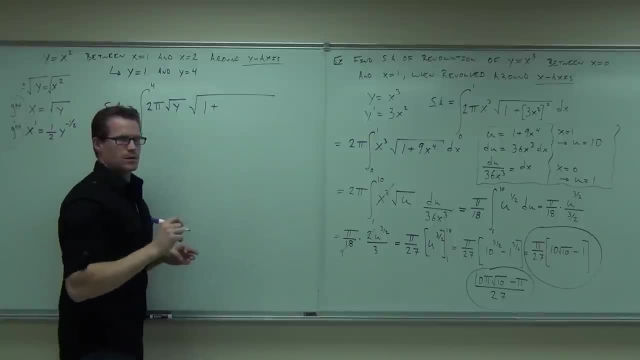 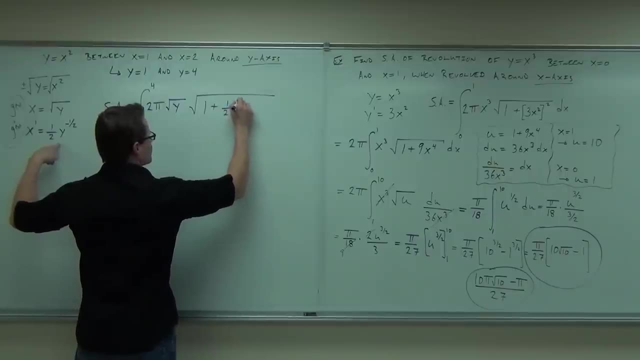 Square root of 1 plus 1 over 2.. 1 over 2. root of y. Okay, This thing right. Don't forget to square it, Man. I think it's nasty if you forget to square it. It's wrong and it's nasty. 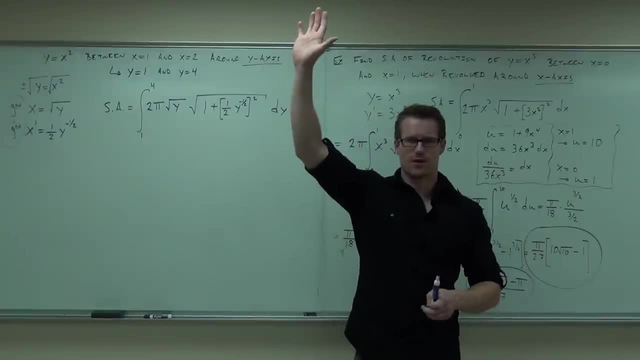 That's the worst kind of wrong to be Show of hands. how many of you feel alright with getting that far? Yeah, You can make something nasty and it's fine if it's right. But getting something wrong and being nasty and working on it. 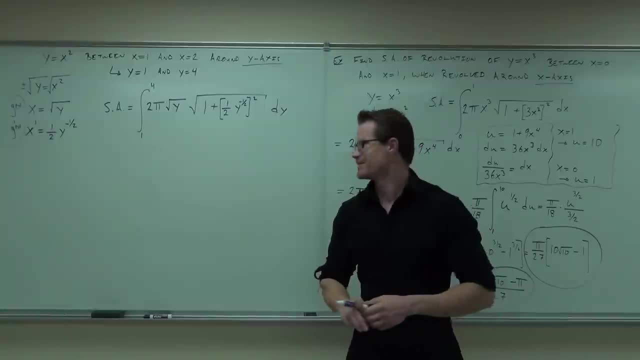 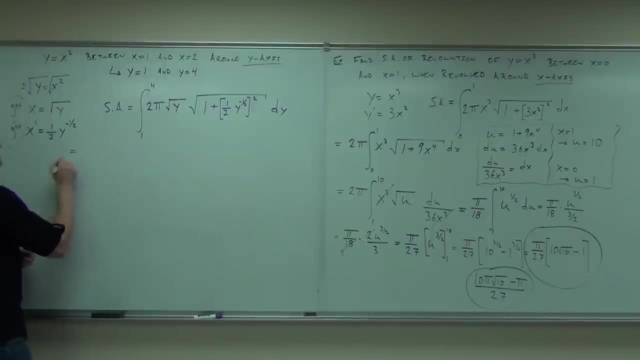 Oh man, You don't want to do that, do you? No, You don't want to do that. At least, I hope not. Well, let's work on this thing. It's going to take a lot of algebra, but not a lot of calculus, honestly. 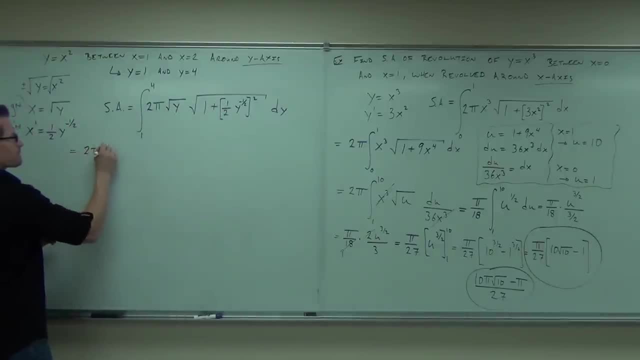 A lot of algebra. Let's pull the 2 pi out, Let's go from 1 to 4.. Let's have a square root of y. Let's have the 1 plus Square that thing. What do you get? 1 plus y. 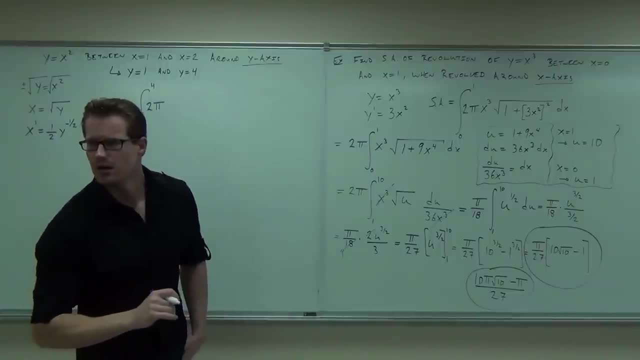 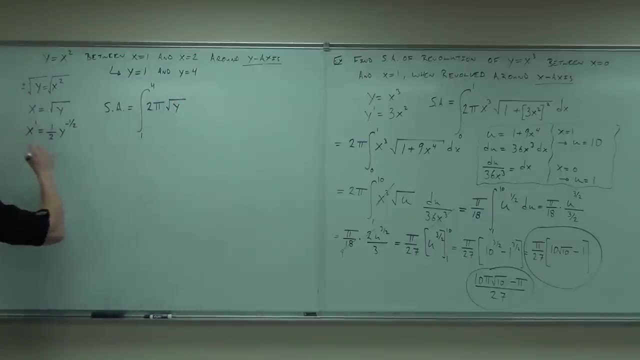 The 2 pi over the y Say what Square root of y? Square root of y because it's in terms of y. It says: take the function in terms of y Before you take the derivative. this would be like g of y. 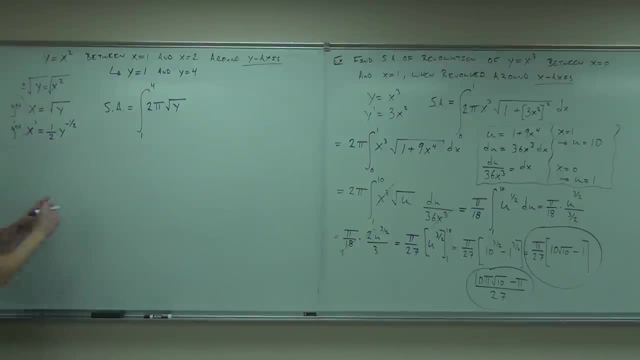 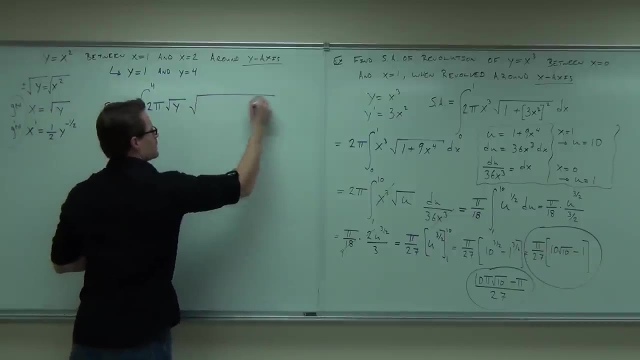 This would be like g prime of y Function itself. Then we go ahead and we multiply by what? Square root of 1 plus 1 over 2 root of y. OK, This thing right. We first have to unstable square root. 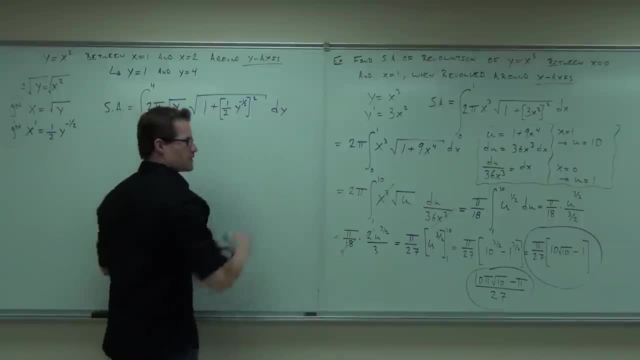 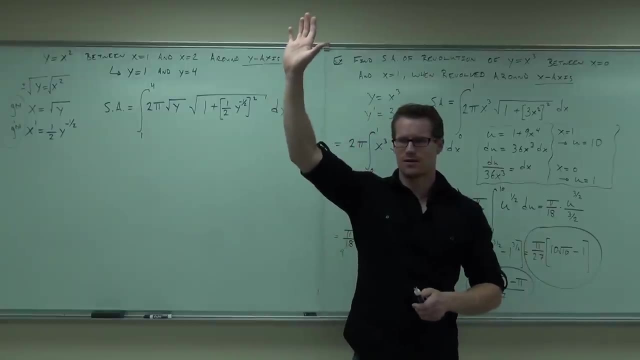 Don't forget to square. I think it's nasty to forget to square. It's wrong and it's nasty- That's the worst kind of wrong to be. Show of hands- how many people are all right with getting that far? Yeah. 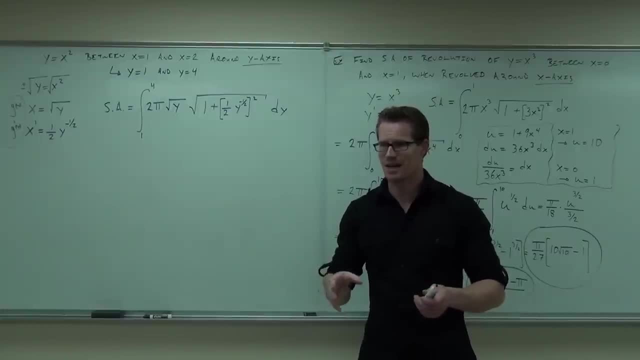 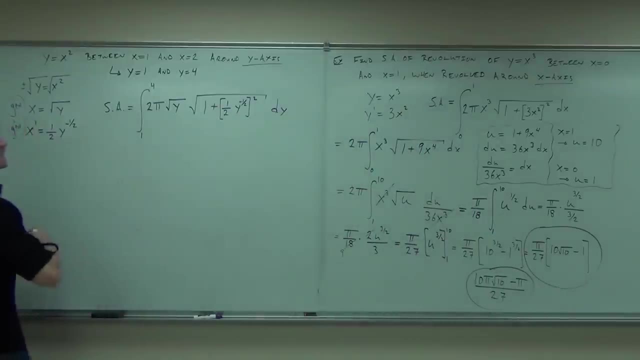 You can make something nasty, and it's fine if it's right, But getting something wrong and being nasty and working on it, Oh man, you don't want to do that, do you? No, No one wants that. At least, I hope not. 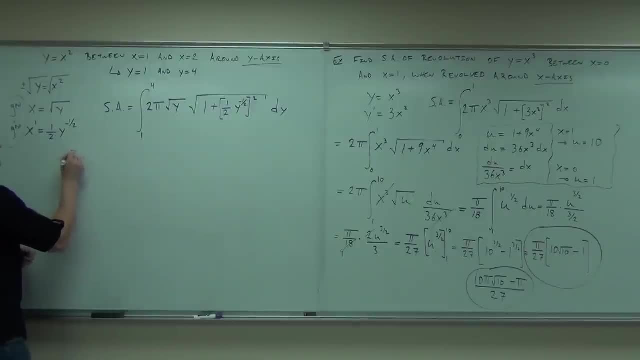 Well, Well, let's work on this thing. It's going to take a lot of algebra, but not a lot of calculus. honestly, A lot of algebra. Let's pull the 2 pi out. Let's go from 1 to 4.. 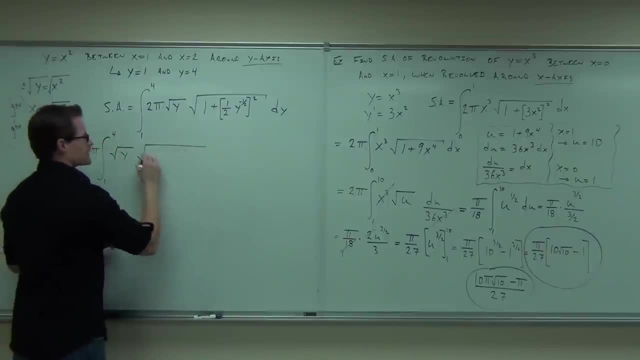 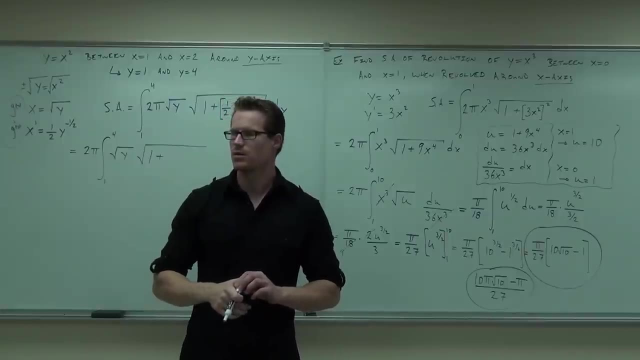 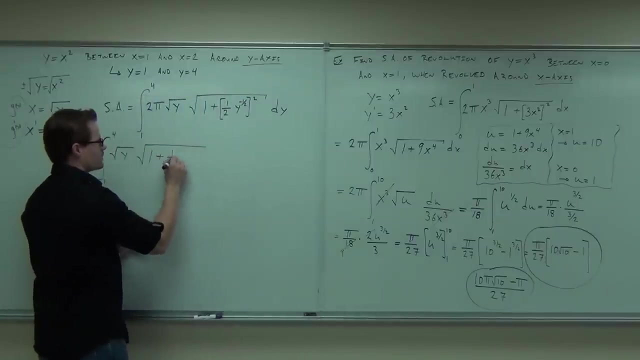 Let's have a square root of y. Let's have the 1 plus square, that thing. What do you get? Be very careful, Be very careful. The 1 fourth, very good. The y negative 1 half times 2, not adding times. 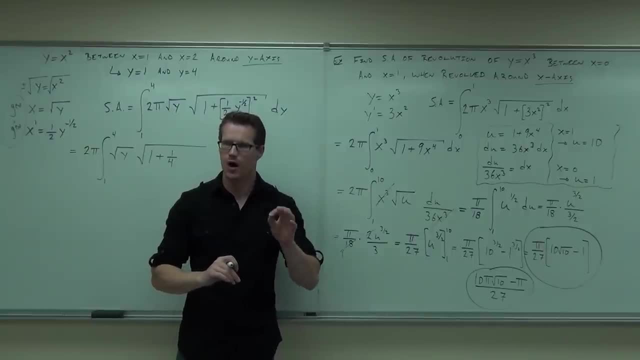 Negative 1 half times 2 is negative 1.. So you're not going to get 1 fourth y, You're going to get 1 over 4y, Do you see it? Or you can do y to the negative 1 over 4, but you're going to change that. 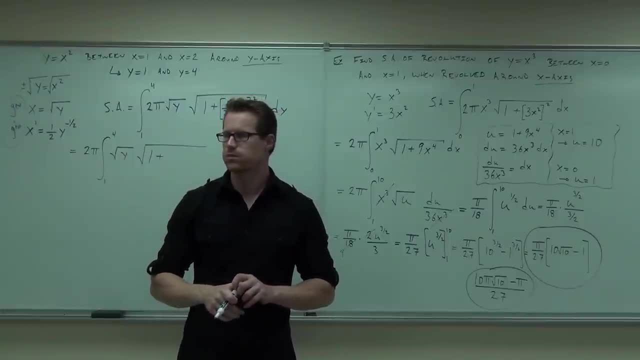 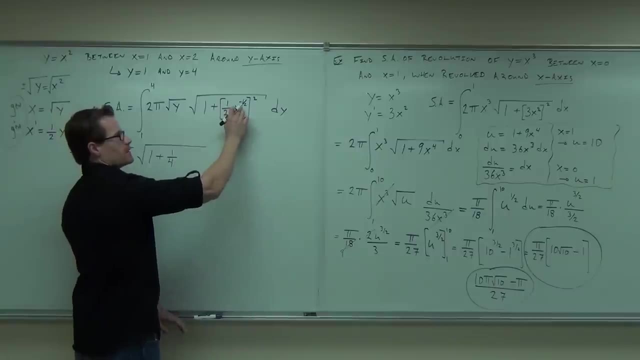 What? 1 plus y. 1 plus y. 1 plus y. Be very careful, Be very careful. The 1 fourth very good. The y negative 1 half times 2, not adding times Negative: 1 half times 2 is negative 1.. 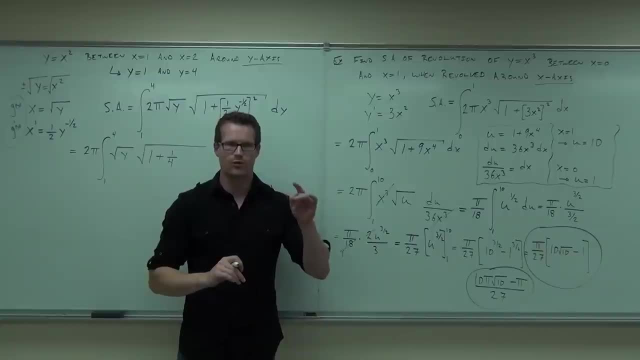 So you're not going to get 1 fourth y, You're going to get 1 over 4y, Do you see it? Or you can do y to the negative 1 over 4, but you're going to change that. 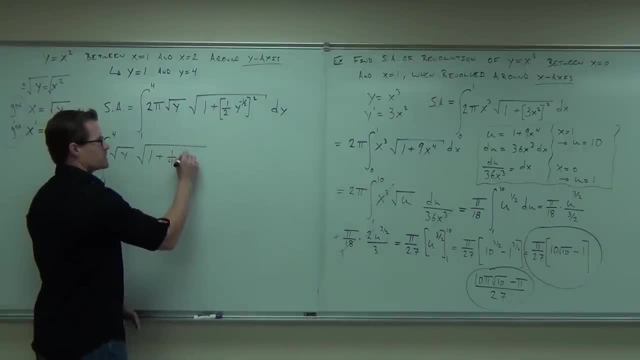 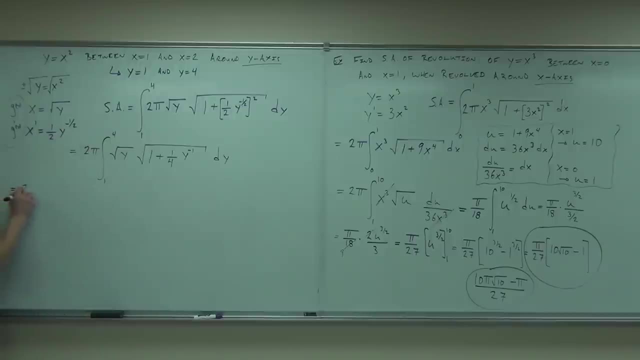 So, one-fourth, I'll say y to the negative 1, just to follow the steps down. What that becomes is 2 pi 1 to 4, square root of y, square root of 1 plus 1 over 4y dy. 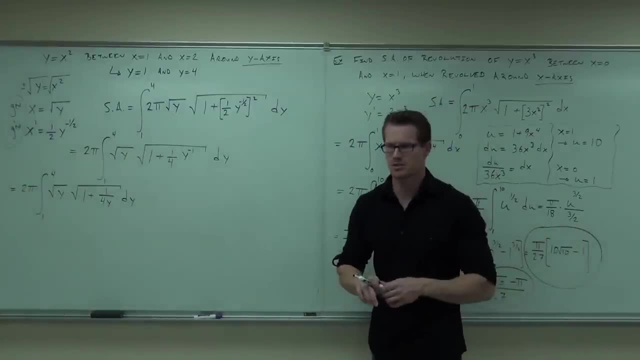 Take a look at it, see if you can follow it down. It's a lot of algebra with those negative exponents. I know they can catch you sometimes. You'll see. you'll see just a second. you okay with it so far. 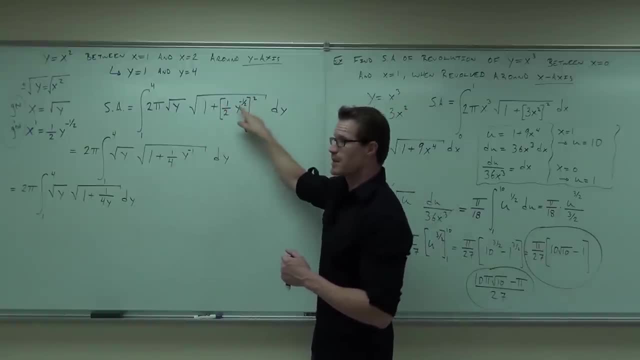 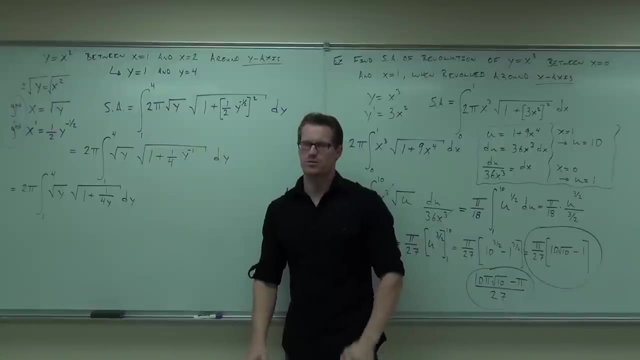 So this square root, one-fourth square root, negative 1, y to the negative 1, denominator, You okay with all of it. Okay, now I'm about to do some fancy math, fancy-pants math. 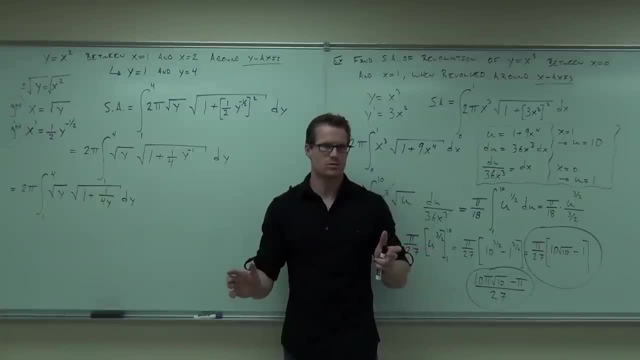 There's a few ways to do this. I will be showing you one way. Okay, Maybe I'll show you both ways. we've got some time, maybe I'll show you both ways. Here's fancy math way, and then I'll show you non-fancy math way. 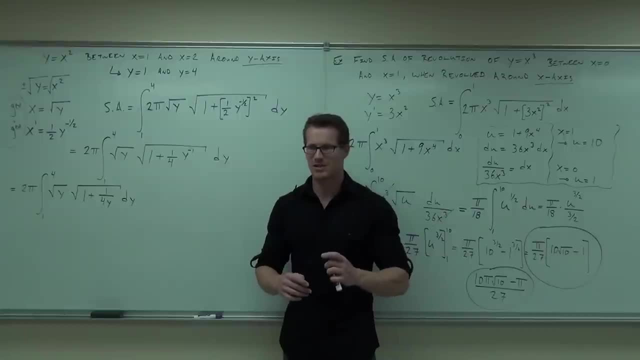 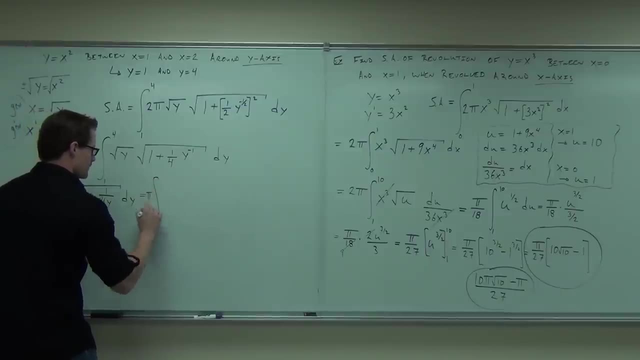 Either way works just fine. okay, So two options. fancy math. you ready to see fancy math? Here's fancy math. Fancy math way says: take the 2 back in there, but call it the square root of 4.. One to 4, one to 4.. 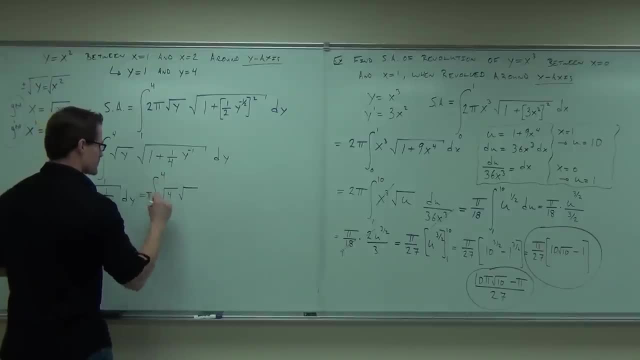 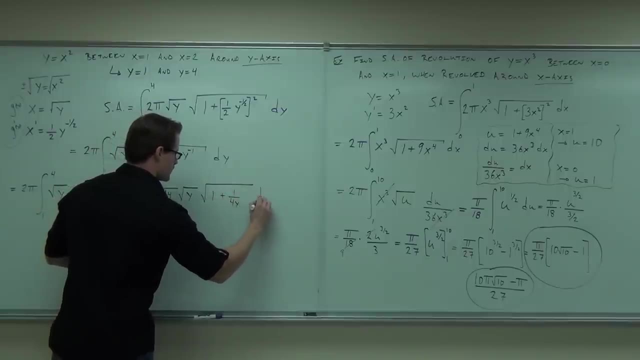 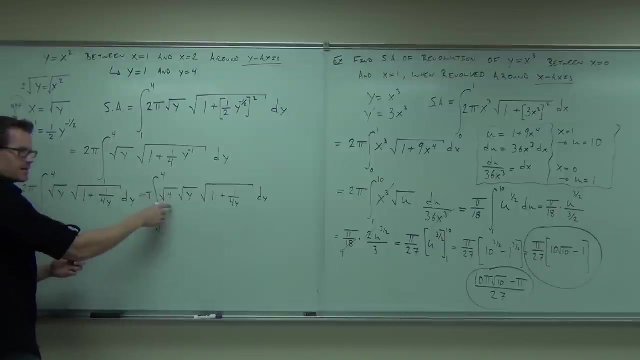 Oh shoot, I'm on the last row. I'm still here. Good, catch, Here's fancy math. take the 2 back inside, but call it the square root of 4.. You, okay with that? so far Is it still 2?? 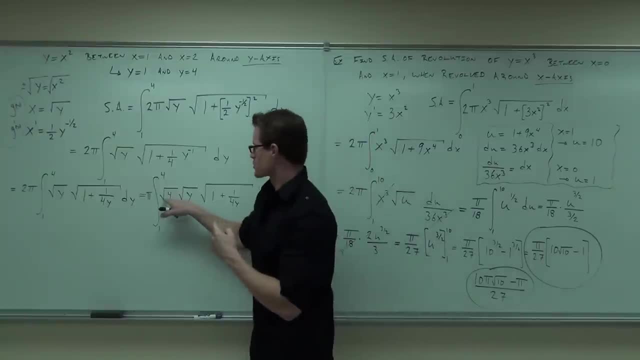 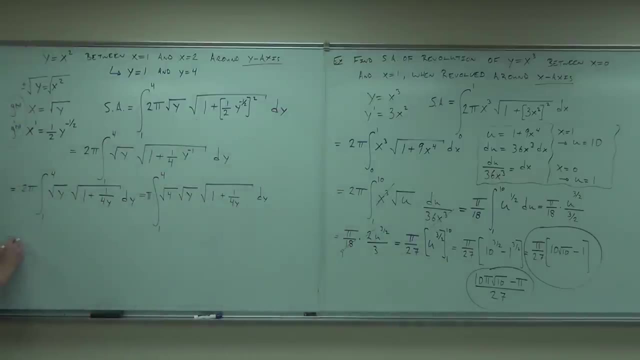 Why am I doing that? I'm doing that because I know that the square root of 4 and the square root of y can be multiplied together to give me the square root of 4y. Okay, Okay, Okay, Shoot, Shoot. 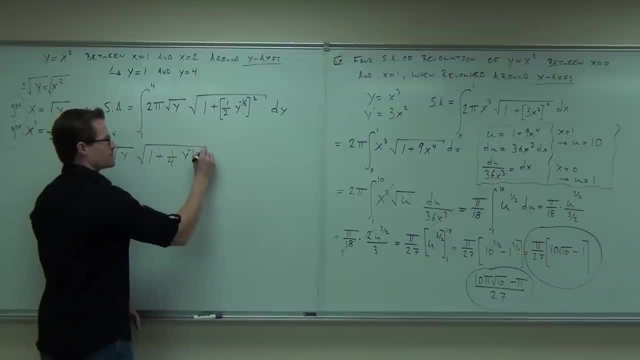 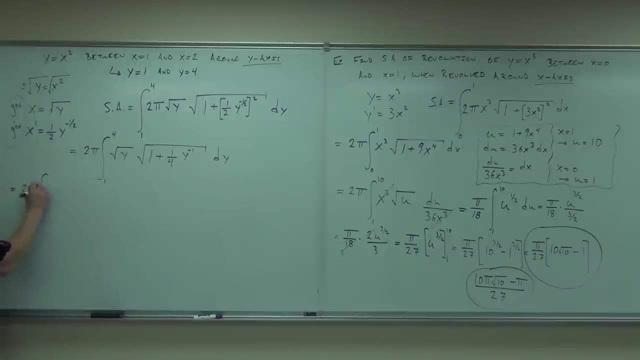 So 1. fourth, I'll say y to the negative 1, just to follow the steps down. What that becomes is 2 pi 1 to 4.. Square root of y, square root of 1 plus 1 over 4y dy. 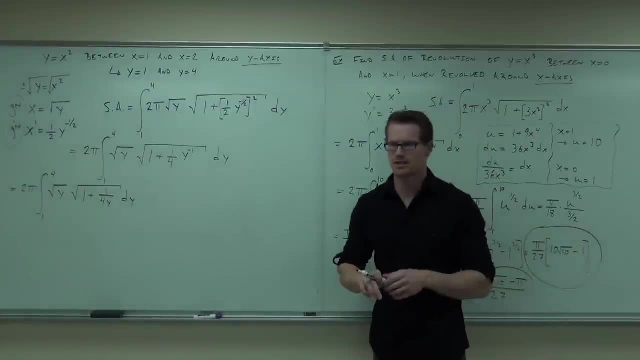 Take a look at it, See if you can follow it down. It's a lot of algebra with those negative exponents. I know they can catch you sometimes. Why don't you just go over it now? You'll see, You'll see. 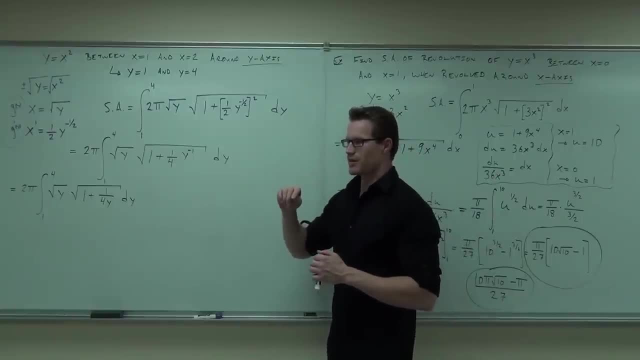 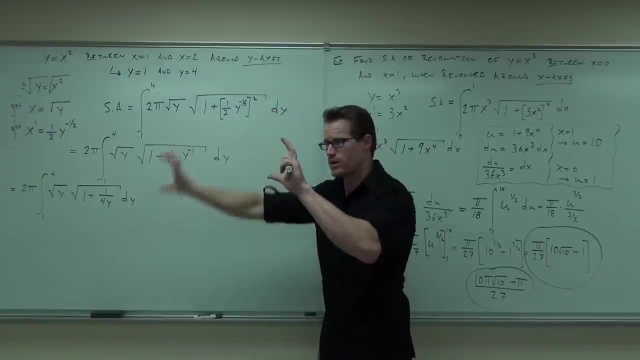 Just a second. You okay with it so far. So this square root 1, fourth square root, negative 1.. Y to the negative 1, denominator. You okay with all of it. Okay, now I'm going to do some fancy math. 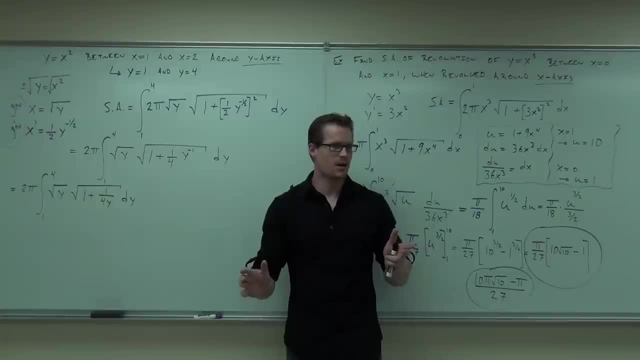 Fancy, fancy math. There's a few ways to do this. I will be showing you one way. Maybe I'll show you both ways. We've got some time. Maybe I'll show you both ways. Here's fancy math way, and then I'll show you non-fancy math way. 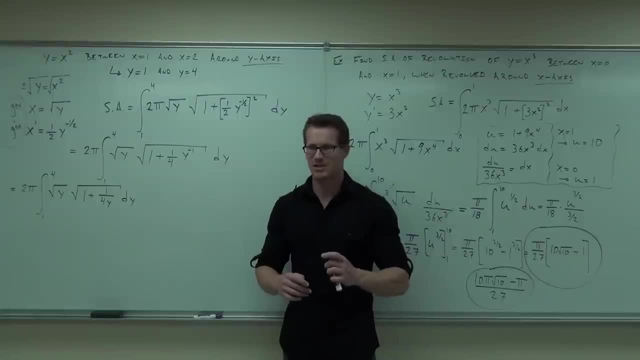 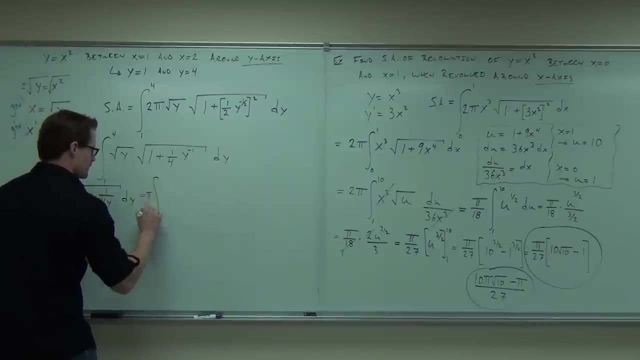 Either way works just fine. okay, So two options. Fancy math. You ready to see fancy math? Here's fancy math. Fancy math way. Fancy math way says: take the 2 back in there, but call it the square root of 4.. 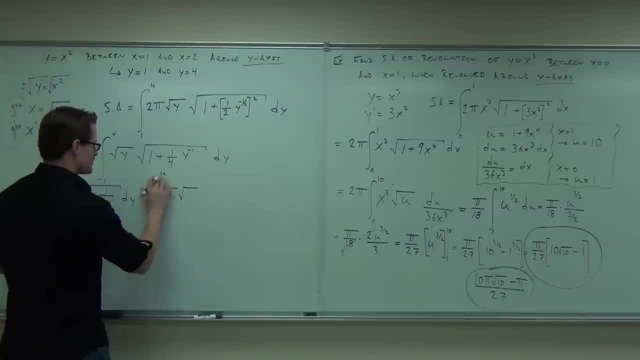 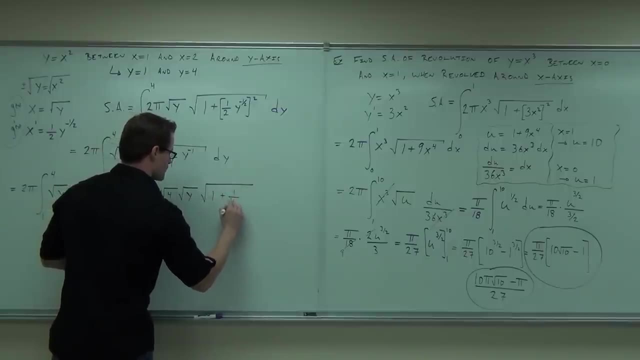 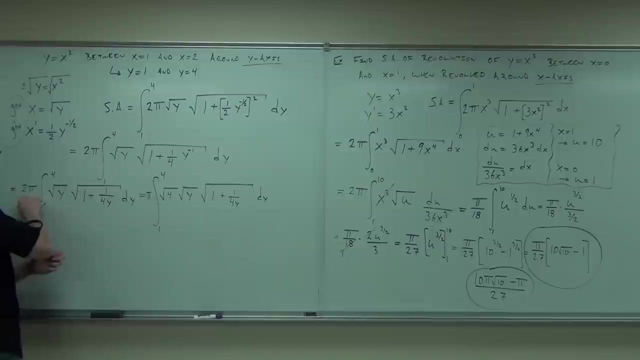 1 to 4.. Oh shoot, I'm on the last row. I'm still here. Good catch, Here's fancy math. Take the 2 back inside, but call it the square root of 4.. Are you okay with that? so far. 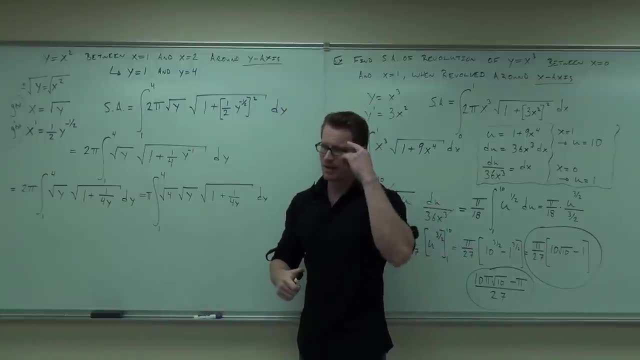 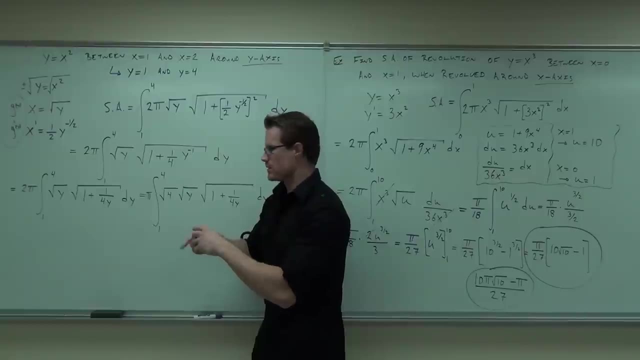 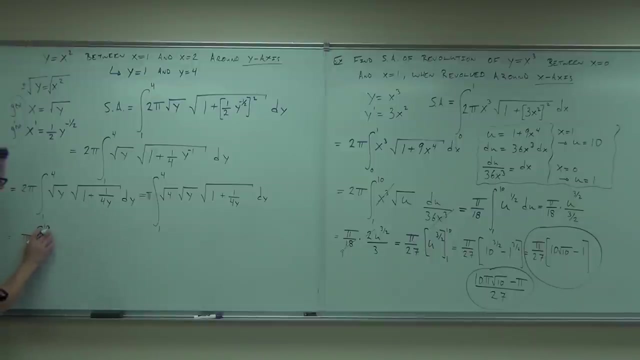 Is it still 2?? Why am I doing that? I'm doing that because I know that the square root of 4 and the square root of y can be multiplied together to give me the square root of 4y Shoot. Why did I pick 4y? 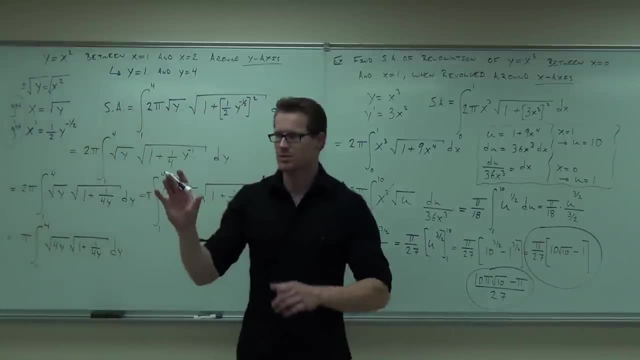 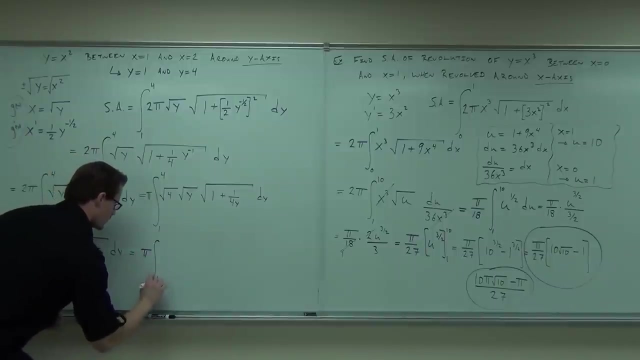 Well, look at that. I have a square root, times a square root, and what I know about that is that I can multiply square roots, times square roots and the radicands that's inside the square roots can multiply together. So if I do this, hopefully you can see this: 1 to 4, big square root, look it 4y- and 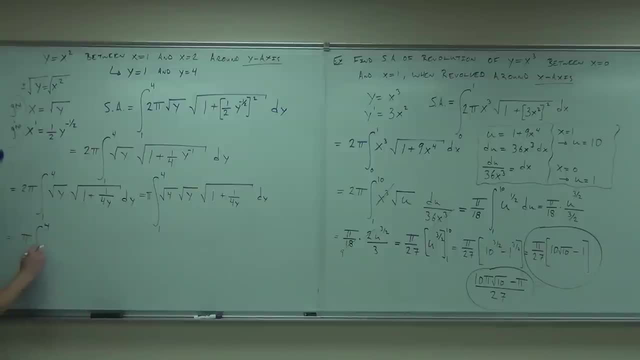 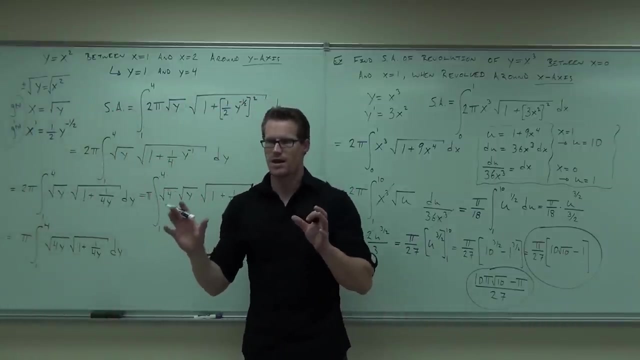 Why did I pick 4?? Well, look at that. I have a square root times a square root, and what I know about that is that I can multiply square roots, times square roots and then radicands- that's inside square roots- can multiply. 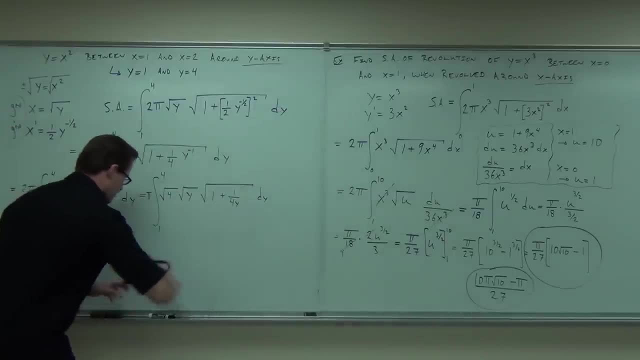 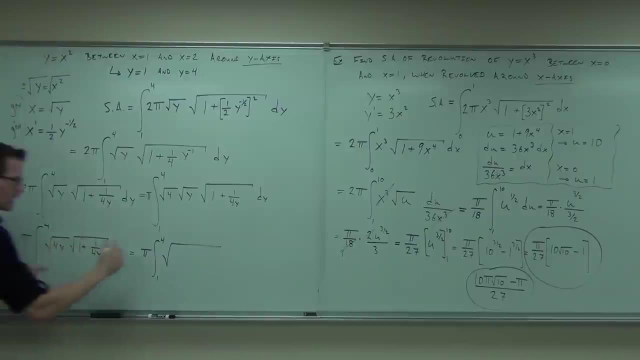 together. So if I do this, hopefully you can see this Okay. 1 to 4, big square root. look at it: 4y, and what's going to happen here? 4y times 1 gives you 4y. 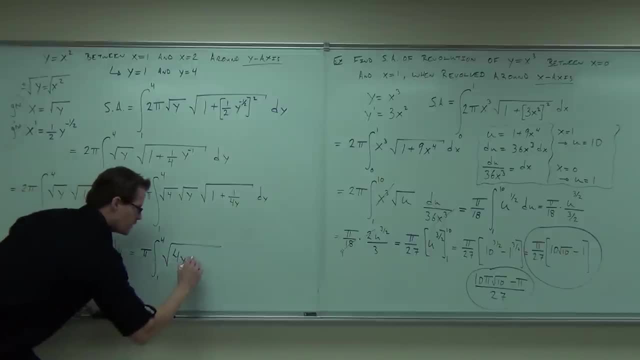 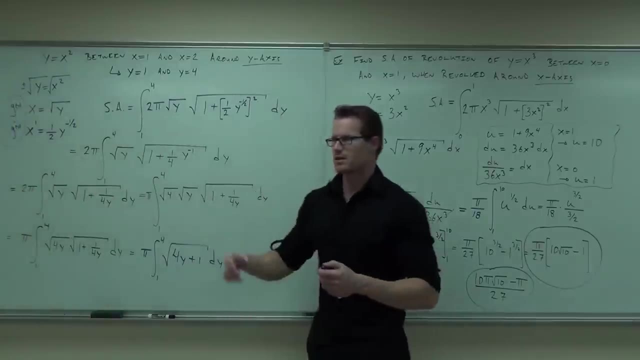 4y times 1 over 4y gives you 1. Done, Practically, Practically done. That's a fancy way to do it. Take the number inside of there, make it up. make it instead of 2, square root of 4,. 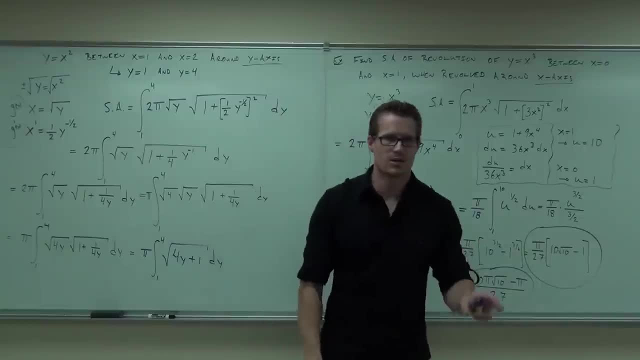 see if it simplifies something. In this case it did. That was kind of a nice easy way to do it. Were you able to follow it? Let's say you didn't see it, because chances are you're probably like. 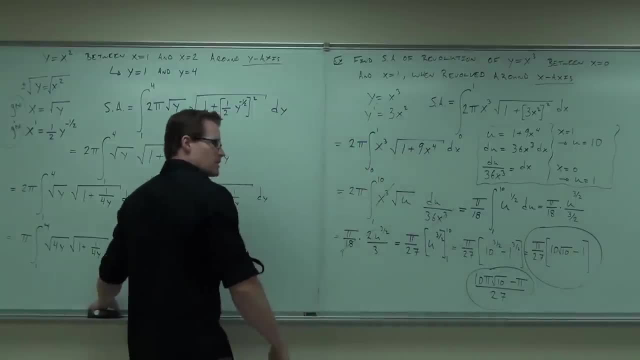 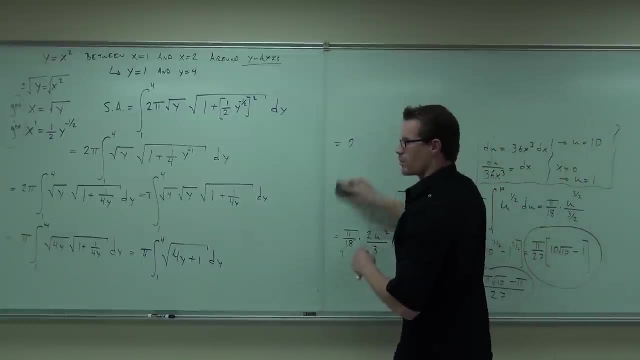 oh my gosh, I wouldn't be able to see that on my own. Can you do it differently? Yeah, I believe. so We're distributing right here 4y times 1 plus 4y times 1, over 4y. 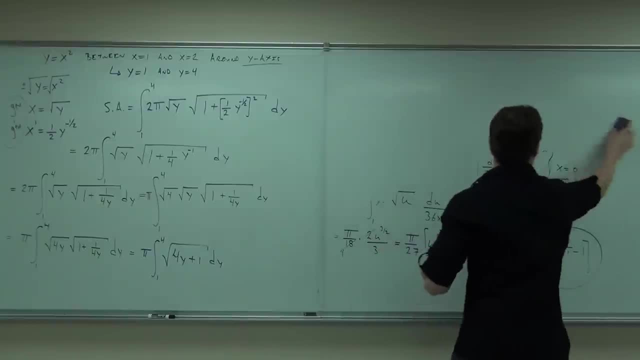 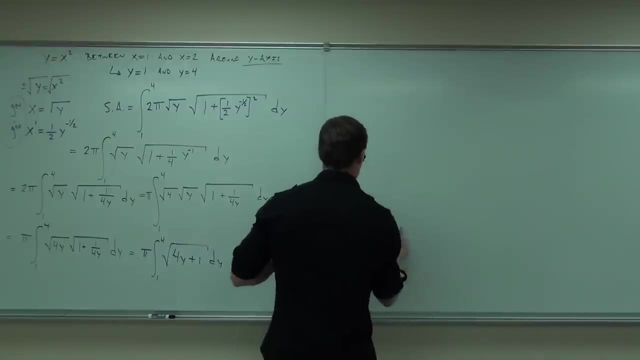 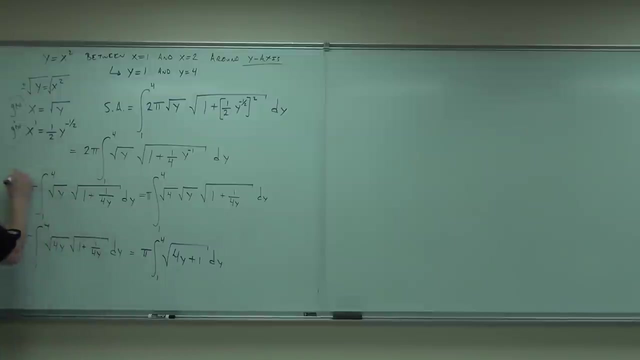 4y's are going to simplify, Let's try again: 4y times 1 plus 4y is 5y times 2.. I'm going to try and find out if I can do it that way. Anyway, here's what I'm going to be doing. 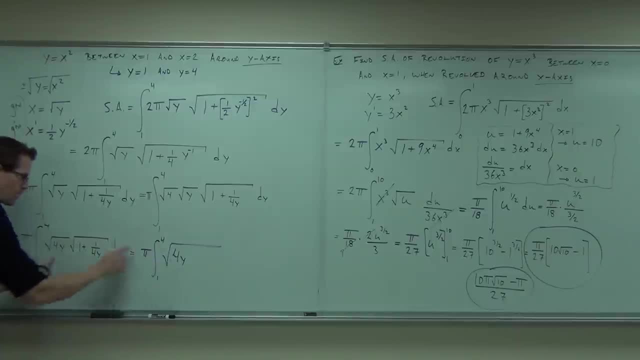 what's going to happen here? 4y times 1 gives you 4y. 4y times 1 over 4y gives you a 4y. 4y times 1 over 4y gives you a 4y. 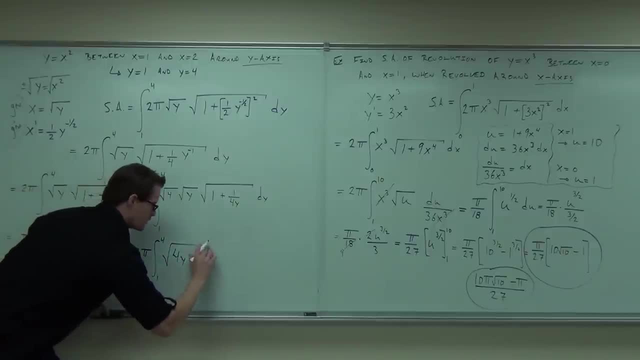 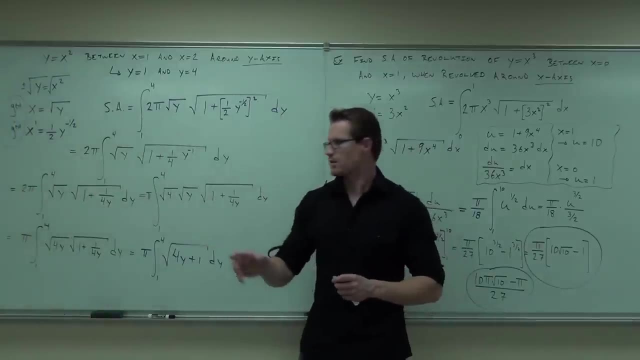 4y gives you a 4y Done, Practically, Practically done. That's a fancy way to do it. Take the number inside of there, make it up. make it instead of 2, square root of 4,. 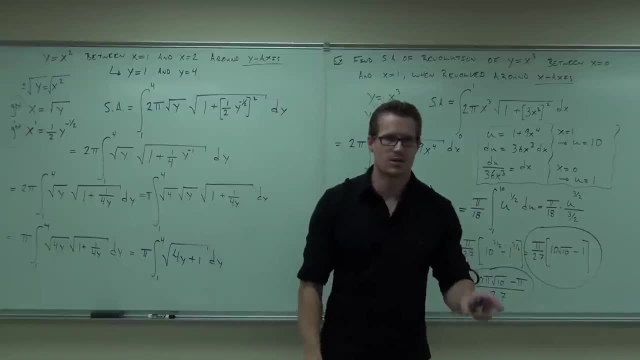 see if it simplifies something. In this case it did. That was kind of a nice easy way to do it. Were you able to follow it? Let's say you didn't see it, because chances are you're probably. oh my gosh. 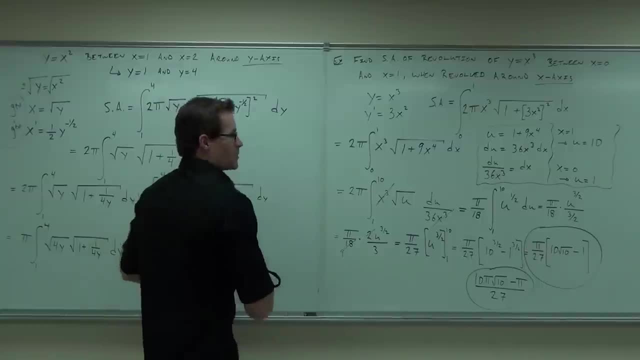 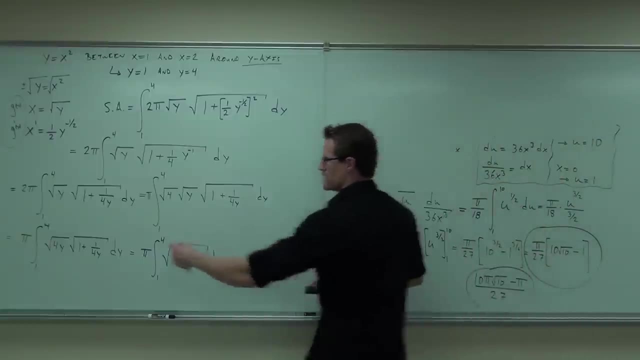 I wouldn't be able to see that on my own. Can you do it differently? Yeah, I believe so. We're distributing right here 4y times 1 plus 4y times 1 over 4y. The 4ys are going to simplify. 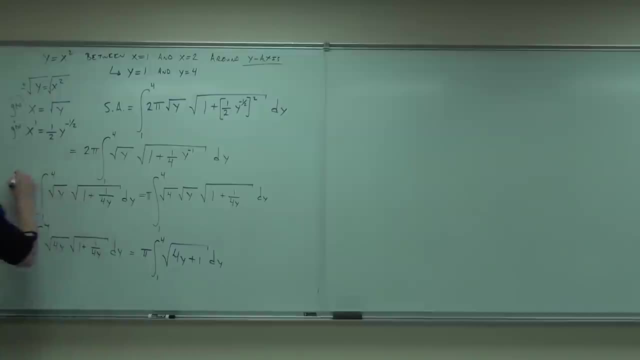 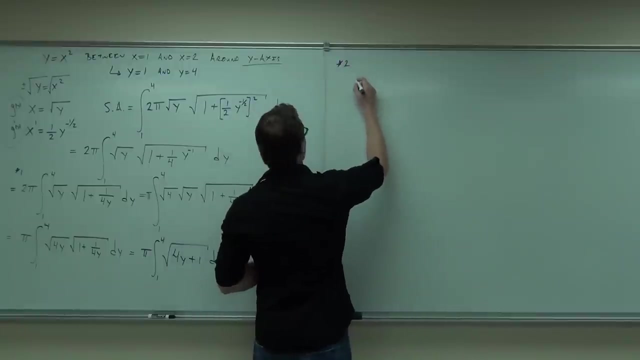 Okay, so this was, like I'll call this Here's star 2.. So, from this point, if you don't do what I just did, what you end up with is square root. 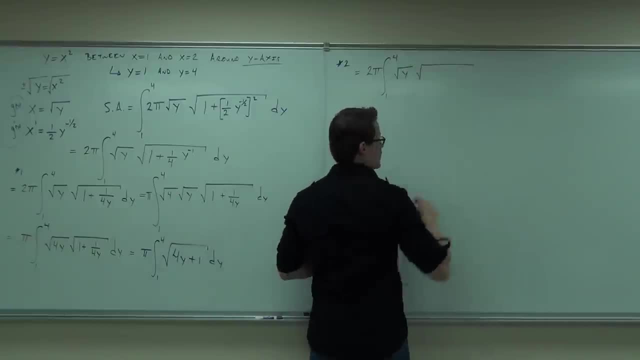 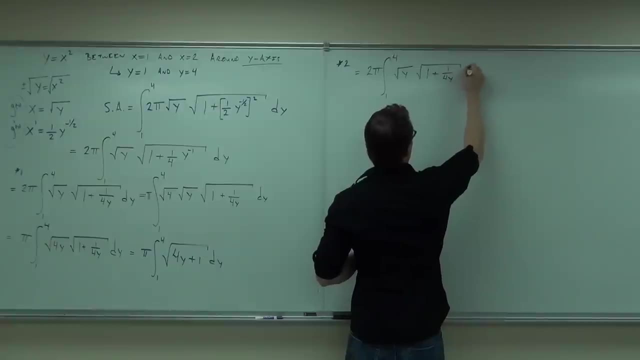 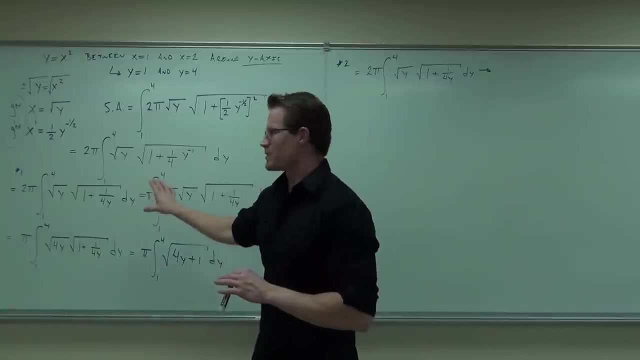 of y, 1 plus 4y. I'll rewrite it: 1 plus 1 over 4y dy. What you have to do is what we've done. similarly, I just showed you a nice step that didn't require you to do this, but you can do it in a way. 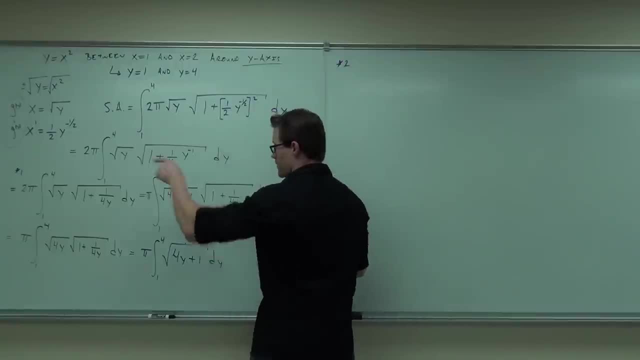 I'm going to be drawing on all this. Alright, I'm going to start this out, I'm going to just write it down. Okay, so this was like I'll call this Here's star 2.. So, from this point, If you don't do what I just did, what you end up with is: how much do you have to do? You're going to have a lot of information. If you don't do what I just did, what you end up with is: 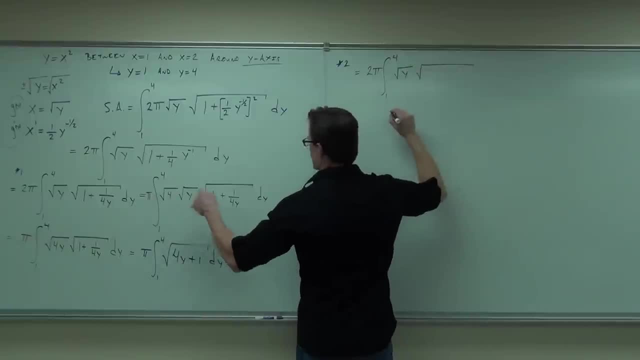 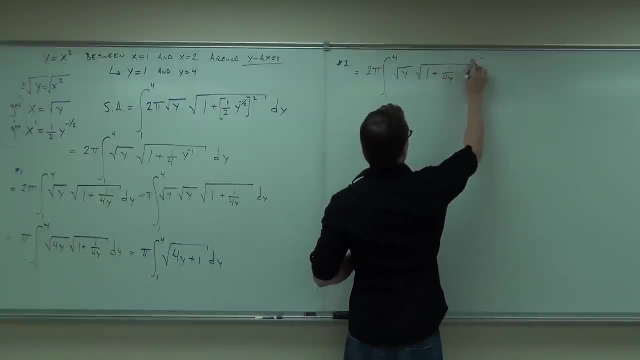 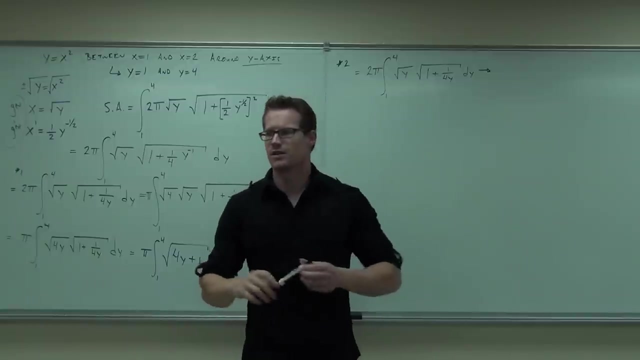 I'm going to write down what I just did: Square root of y, 1 plus 4y. I'll rewrite it: 1 plus 1 over 4y dy. What you have to do is what we've done, similarly. 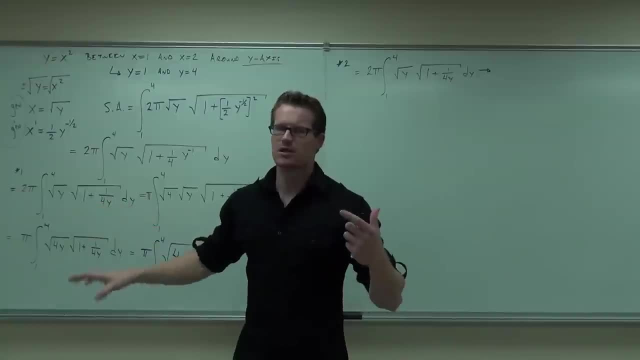 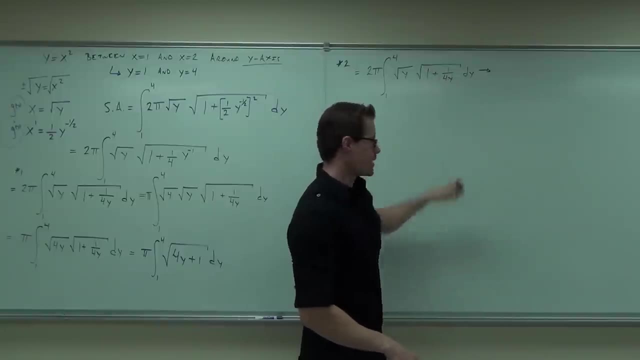 I just showed you a nice step that didn't require you to do this, but you can do it in a way that I think, hopefully, should be familiar to you. Find the common denominator over here: 4y over 4y plus 1 over 4y. 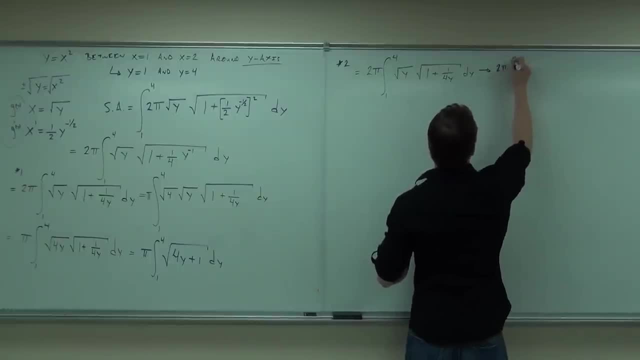 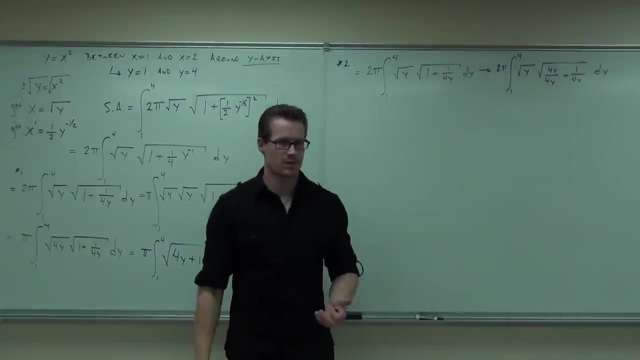 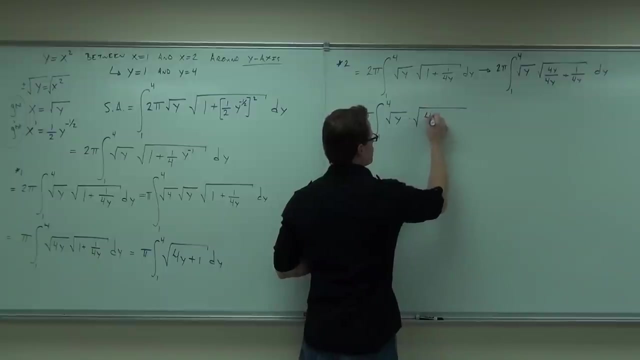 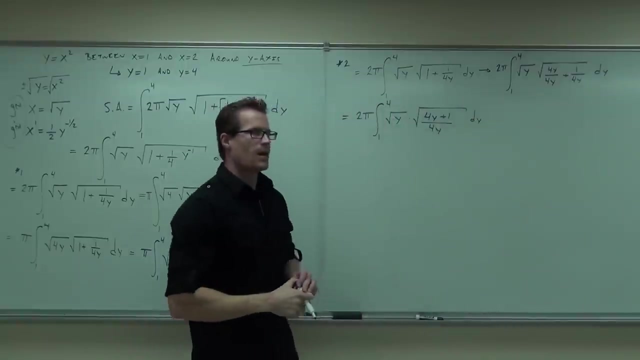 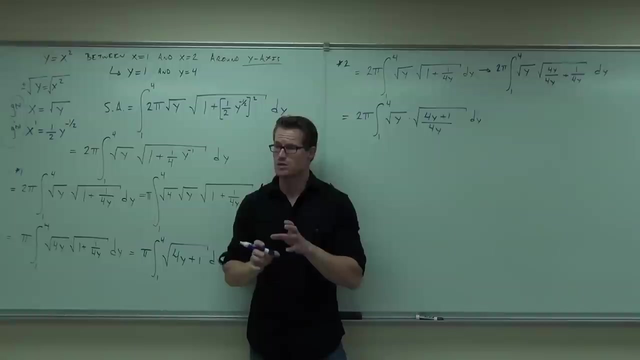 Like that. Find that common denominator. You got me still Put the fractions together. Do you remember doing this? It's very similar to something we've done before, where we had to break up that square root by a quotient. Can we do that now? 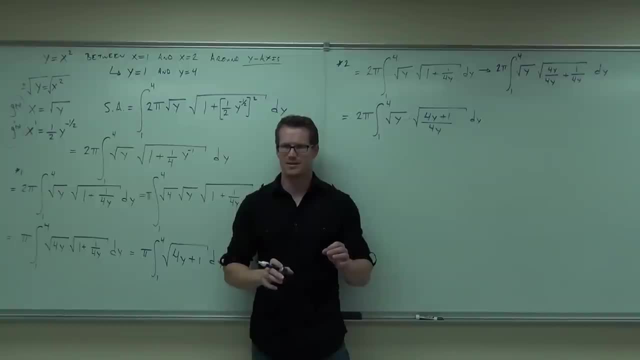 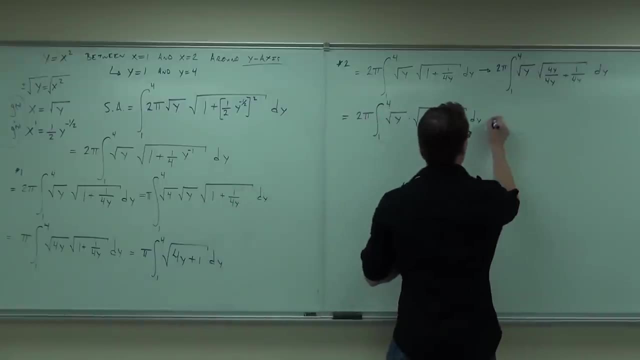 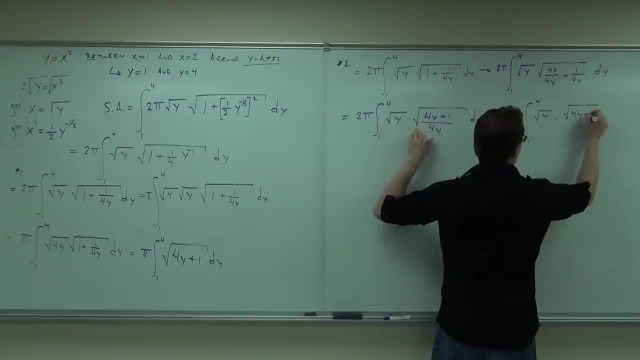 Have I lost you? Are you with it? Do you see what we've done so far? Found the common denominator, put the fractions together. That way we can separate them. So 2pi still square root of y times square root of 4y plus 1.. 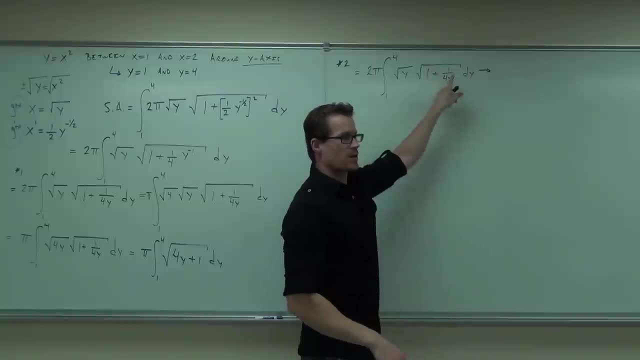 that I think hopefully should be familiar to you. Find the common denominator over here: 4y over 4y plus 1 over 4y. 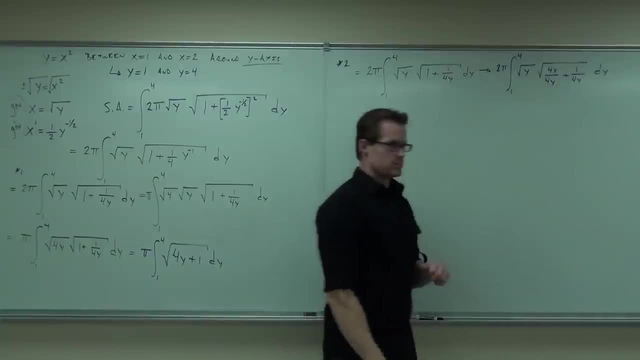 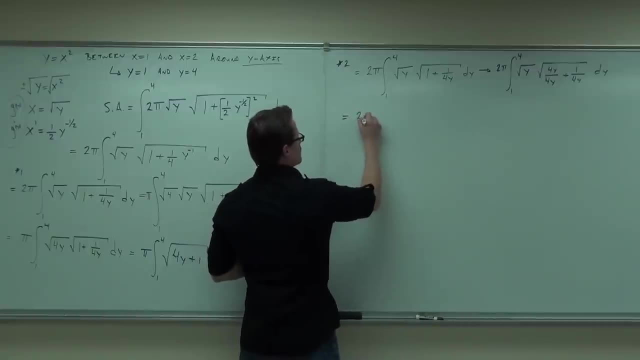 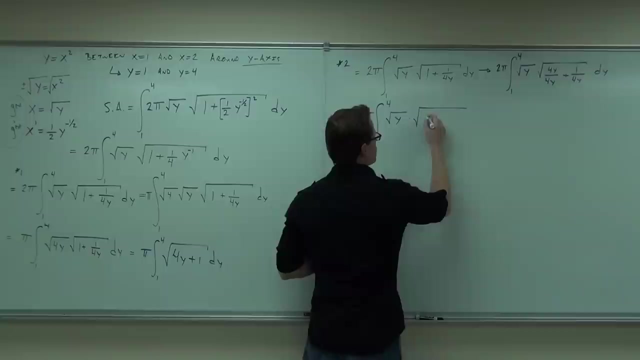 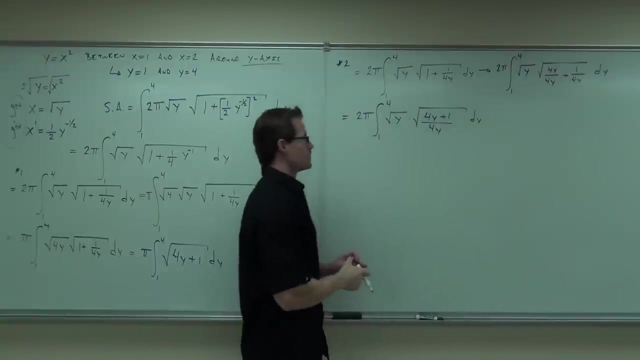 Do you got me still Put the fractions together. 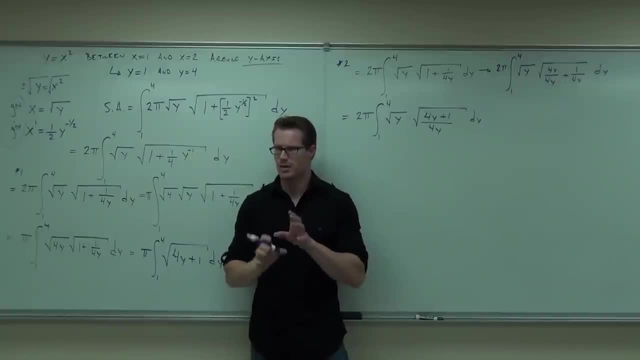 It's very similar to something we've done before where we had to practice the to break up that square root by a quotient. Can we do that now? Have I lost you? 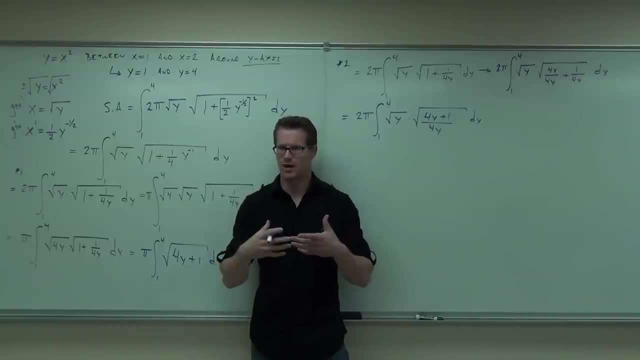 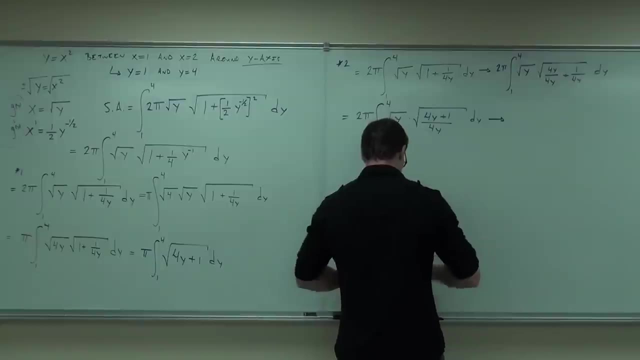 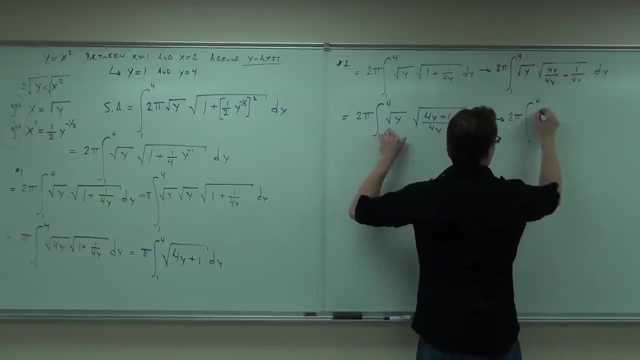 Are you with it? Do you see what we've done so far? Found a common denominator, put the fractions together. That way we can separate them. So two pi still Square root of y times, square root of four y plus one, Four y plus one. there's nothing you can do. 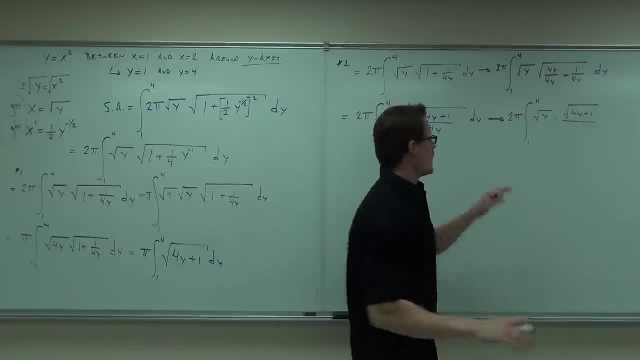 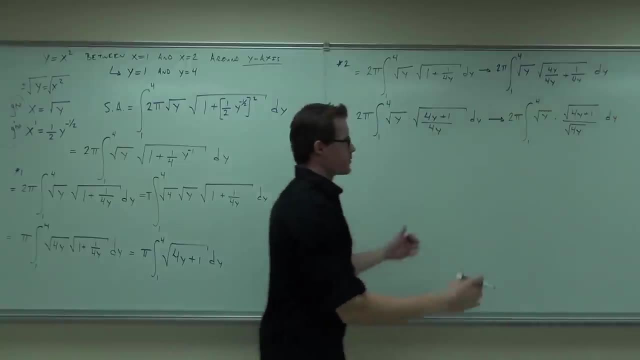 with the square root of four y plus one. right now, Nothing. you can't split that up. However, this is the square root of four y on the denominator as well. Now, when you think about the square root of four y, what that is. 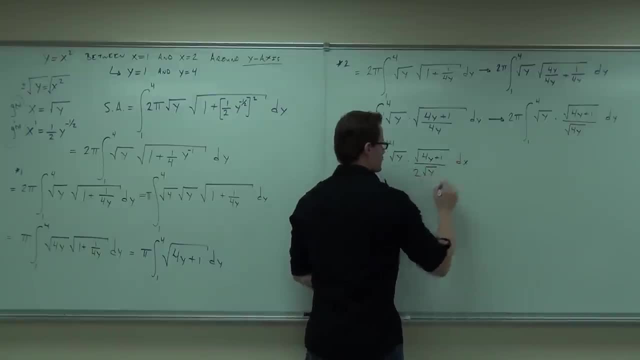 is two square root y. See how to get the two square root of y. Yeah, you see, we're gonna get the same thing. It's kinda cool. either way you do it, This has a few more steps. I mean really. 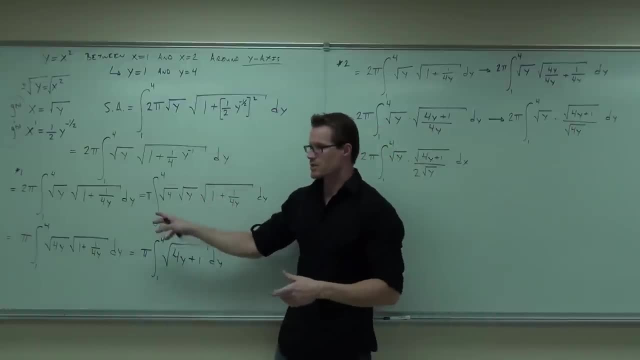 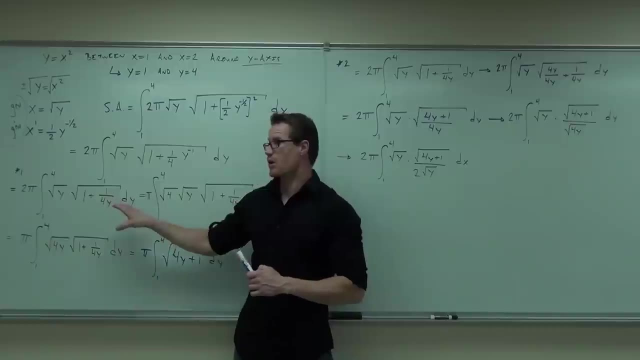 it's just like three steps, five steps, But you're gonna get the same thing. Whatever way seems easier, I don't care, But I just gave you another option over here. This is kind of the fancy pants type of math. Ooh, I wanna be fancy, do the fancy. 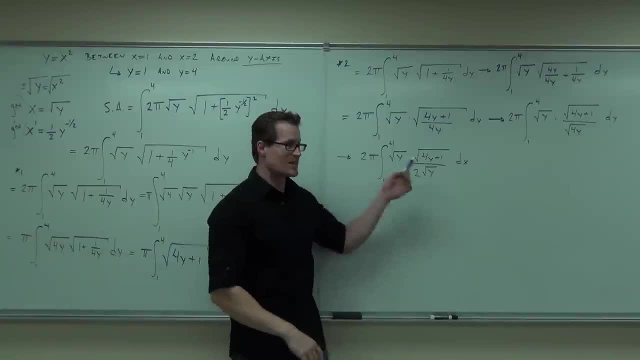 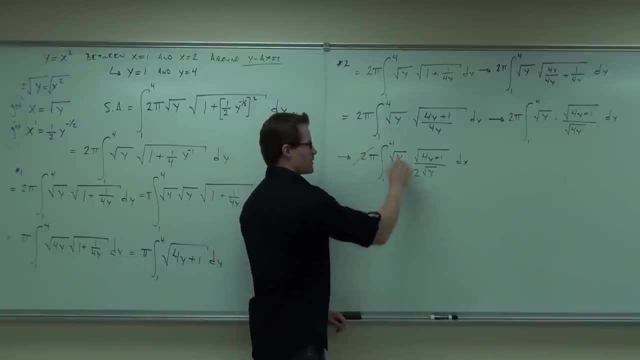 Two's are gone. Yeah, constant, constant, very good. What else Square root of y? That helps you a lot, doesn't it? Because if you don't get rid of that square root of y, somehow you're smoked. 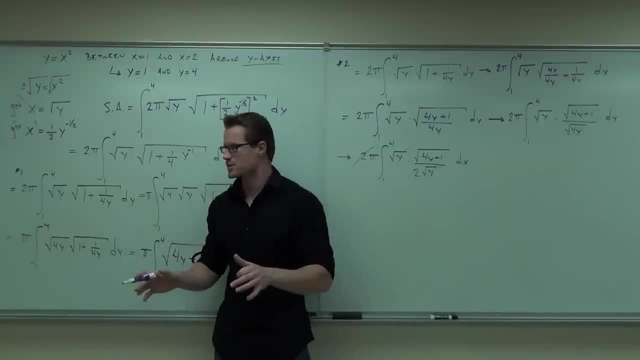 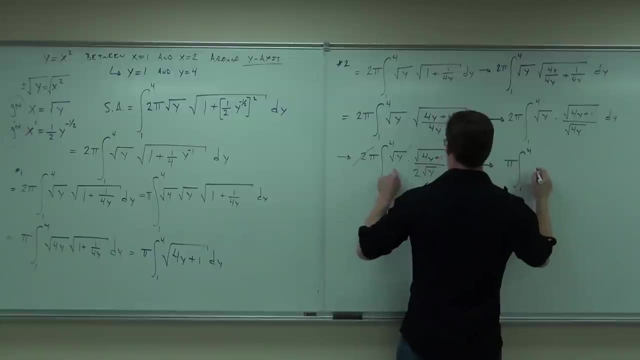 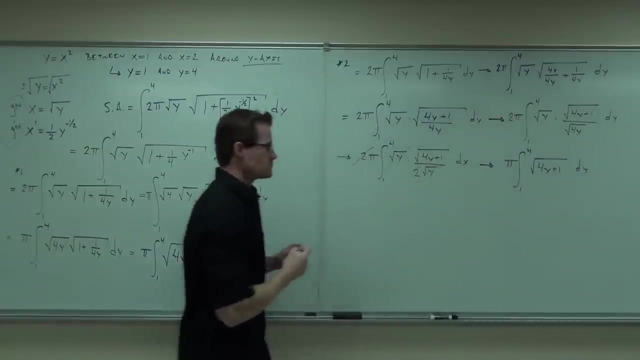 Otherwise you'd have to look for some substitution, and that's just not gonna happen with this example. So now we're left with pi one to four, square root of four y plus one dy. Now will a substitution even work? 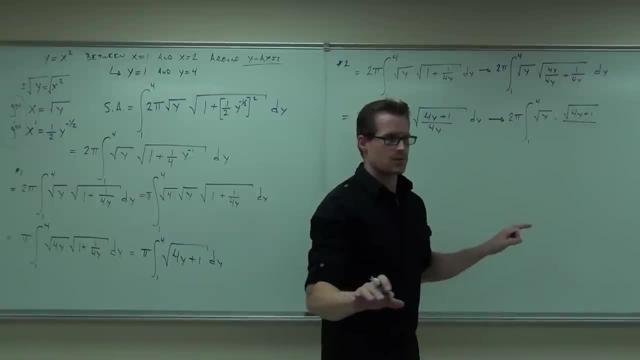 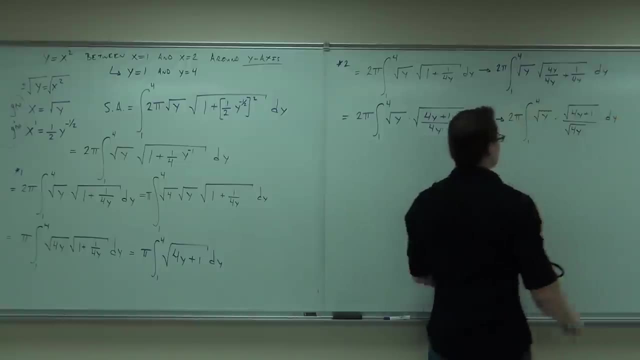 There's nothing you can do with the square root of 4y plus 1 right now, Nothing. You can't split that up. However, this is the square root of 4y on the denominator as well. Now, when you think about the square root of 4y, what that is. 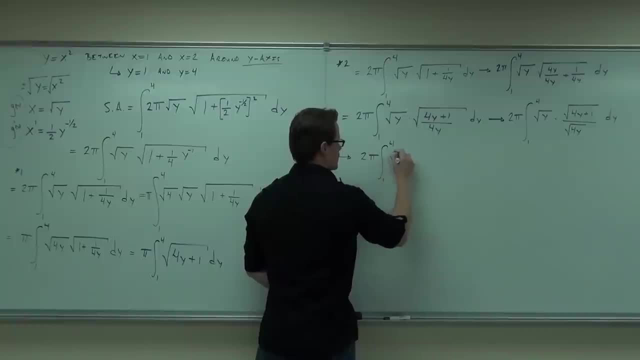 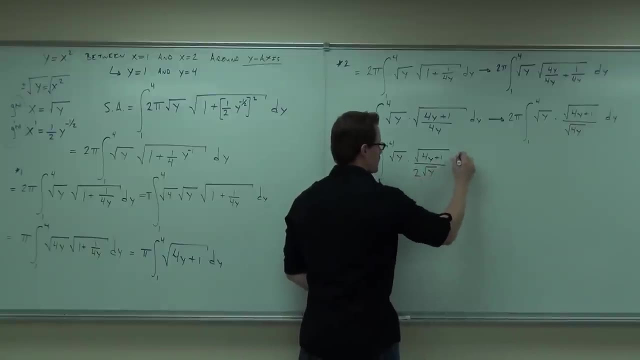 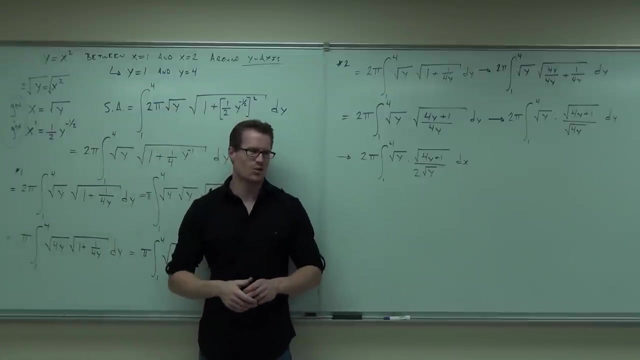 this is the square root of 4y, So the square root of 4y is 2 square root of y. See how to get the 2 square root of y. Did you see we're going to get the same thing. It's kind of cool. 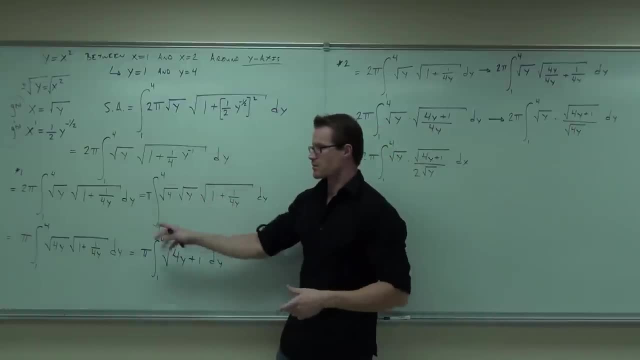 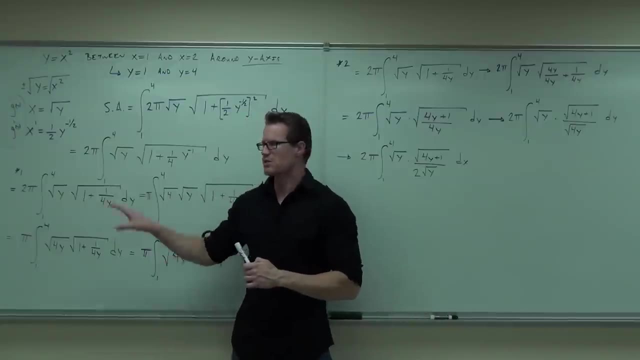 Either way you do it, This has a few more steps. I mean, really it's just like three steps, five steps, But you're going to get the same thing. Whatever way seems easier, I don't care, But I just gave you another option over here. 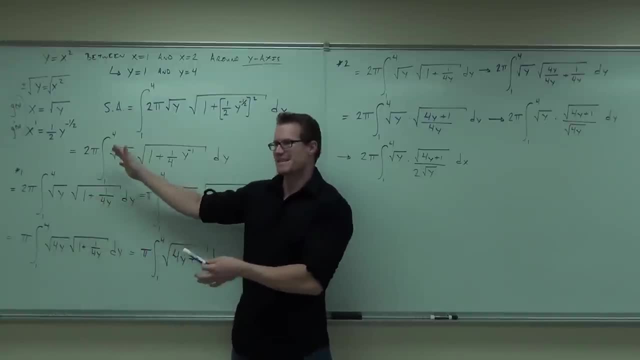 This is kind of the fancy pants type of math. Ooh, I want to be fancy, Do the fancy pants. If you don't want to be fancy and you get this, do this. I really don't care as long as you get the right answer. 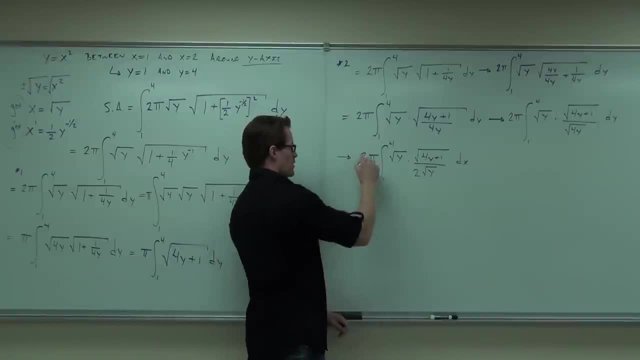 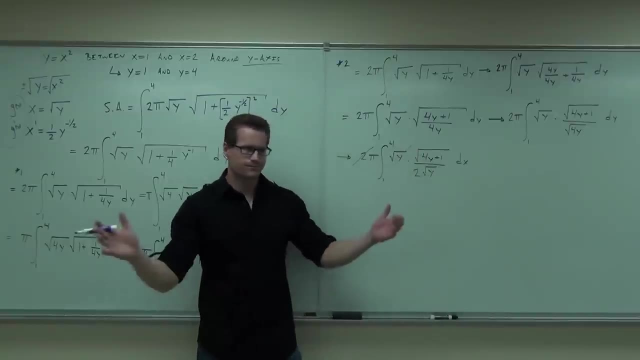 Tell me what happens here, please. The 2's are gone. The 2's are gone. Yeah, Constant, constant, Very good, What else? Square root of y? That helps you a lot, doesn't it? Because if you don't get rid of that square root of y, somehow you're smoked. 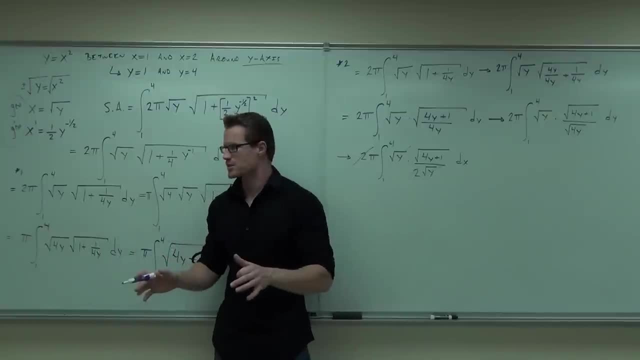 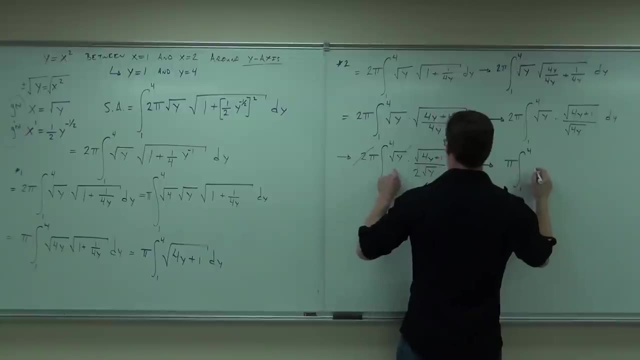 Otherwise you'd have to look for some substitution, and that's just not going to happen with this example. So now we're left with pi 1 to 4, square root of 4y plus 1.. Now what's the derivative of 4y plus 1?? 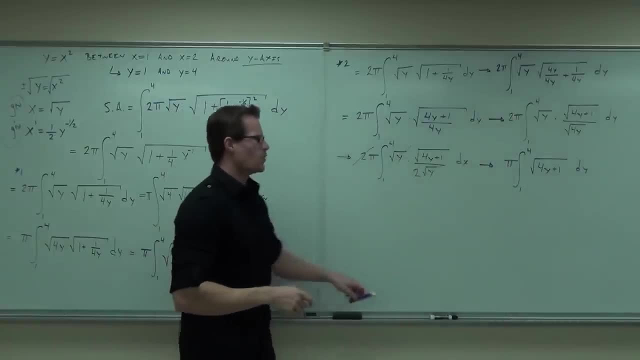 4y 4y. Now will a substitution even work? What's the derivative of 4y plus 1? 4. Does it have a y in it? Then of course it'll work. You always neglect constants with your substitutions. 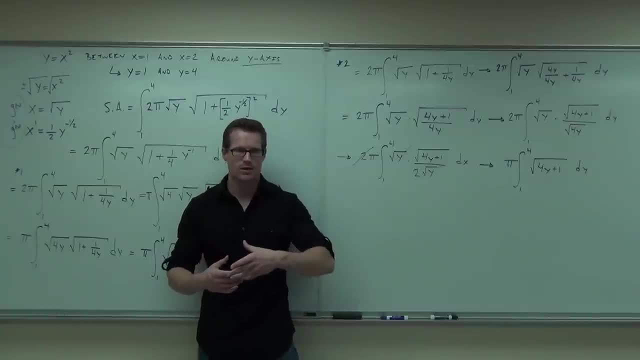 Constants don't matter, because you're just going to pull them out front anyway, right, So will a substitution work here? Yes, Absolutely. What's the derivative of 4y plus 1? It's 4.. There's nothing that you need to simplify out. 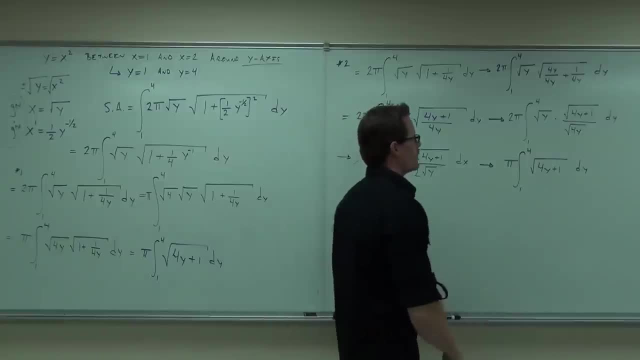 You're going to pull the 1- fourth out of your integral anyway, So let's do that here. U equals 4y plus 1.. You generally pick the thing that's inside your problem, And right now our problem's the square root. 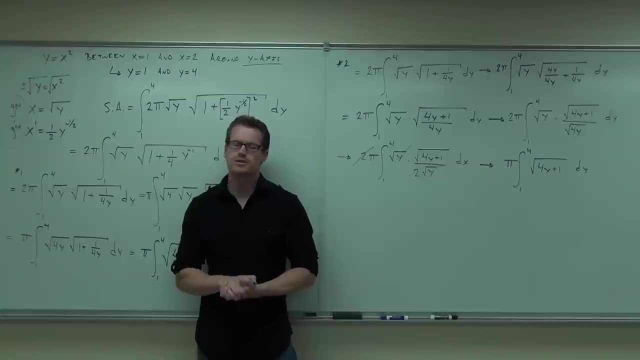 What's the derivative of four y plus one Four? Does it have a y in it? Then of course it'll work. You always neglect constants with your substitutions. Constants don't matter, because you're just gonna pull them out front anyway, right? 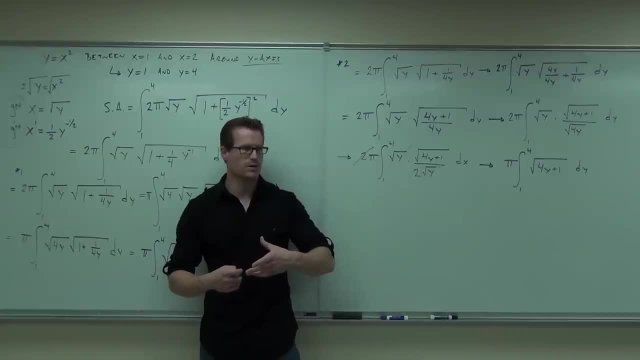 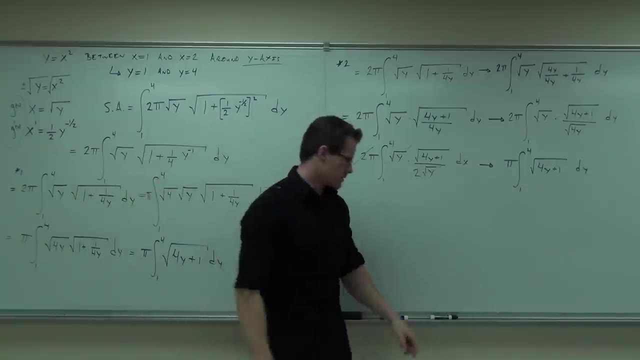 So will a substitution work here? Yes, Absolutely. What's the derivative of four y plus one? It's four. There's nothing that you need to simplify out. You're gonna pull the one-fourth out of your integral anyway, So let's do that here. 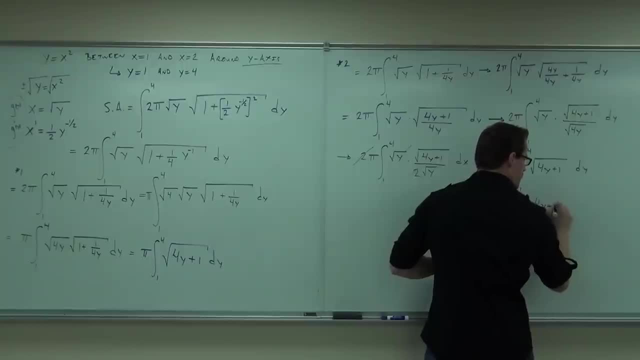 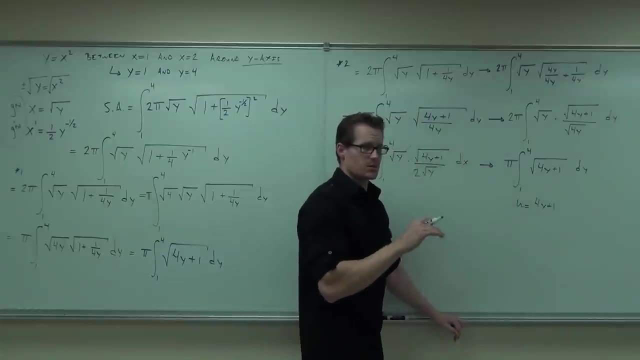 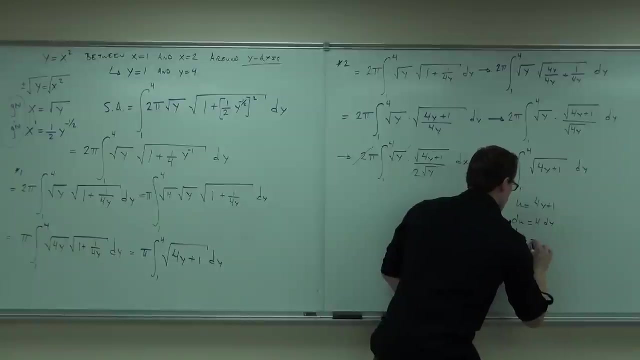 u equals four y plus one. You generally pick the thing that's inside your problem. Right now, our problem's the square root. Don't forget that you do need a substitution, though You absolutely must. du equals four dy. du over four equals dy. 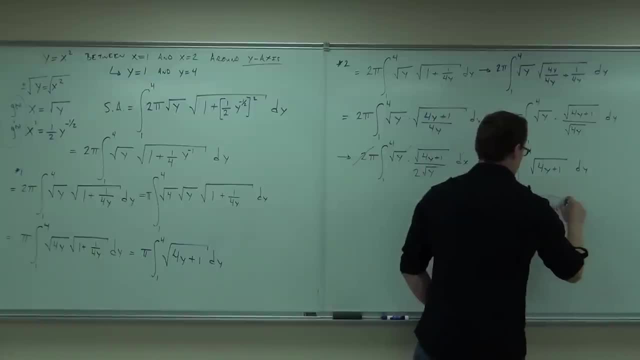 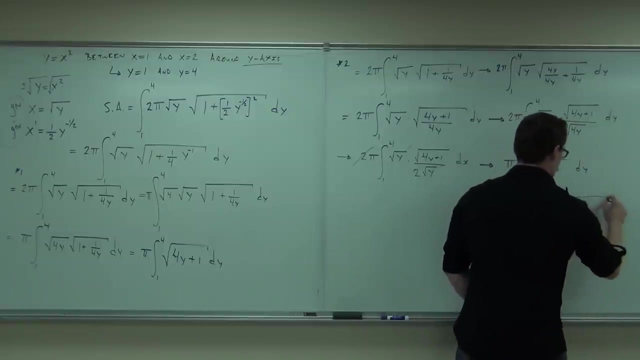 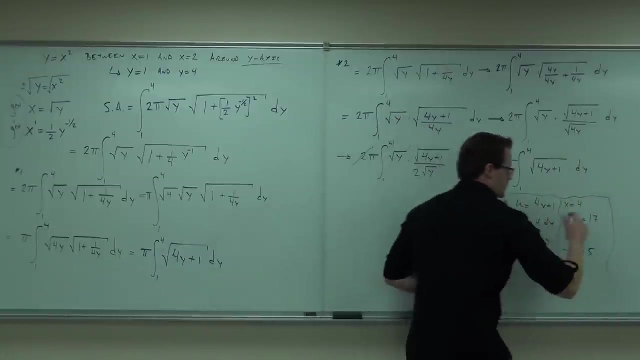 What else do you wanna do right now? Let's do that. I'm sorry, when u is four you get how much? And u is one sure five. So those right there, those are our new bounds of integration. 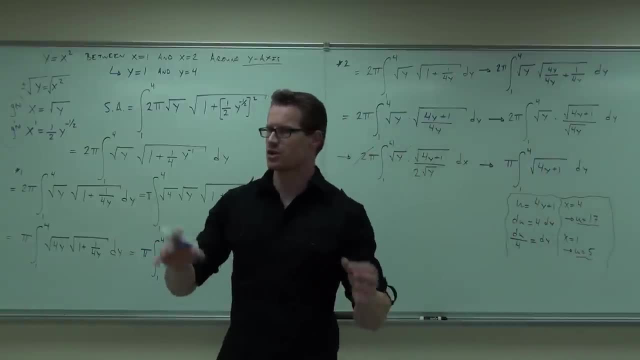 We're not gonna have to substitute back in for x's later. We have these in terms of u. We're good to go, So let's rewrite our integral real quick. before we do it, We'll have a pi. We'll have this integral from one to- I'm sorry, five to seventeen. 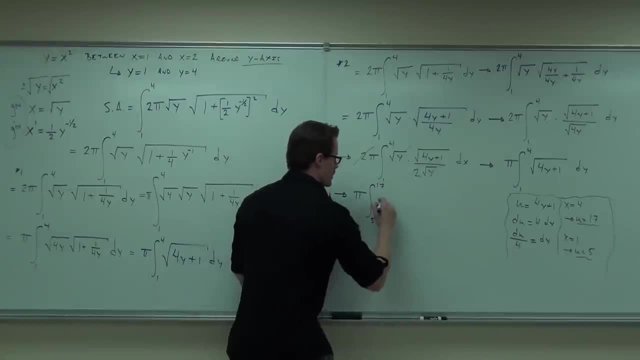 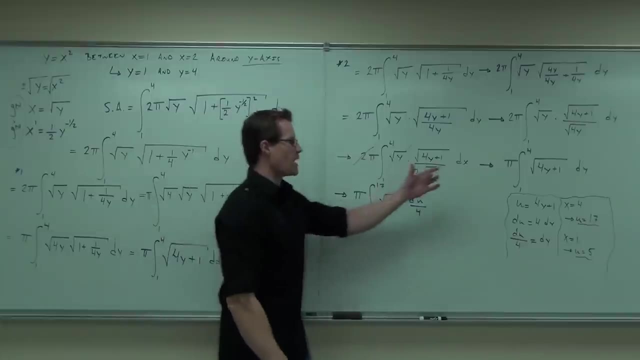 Because we just changed bounds Square root of u, du over four. Don't forget that the dy becomes a du over four. So four y plus one u Seventeen from the four when we plugged it in, Five from the one after we plugged it in. 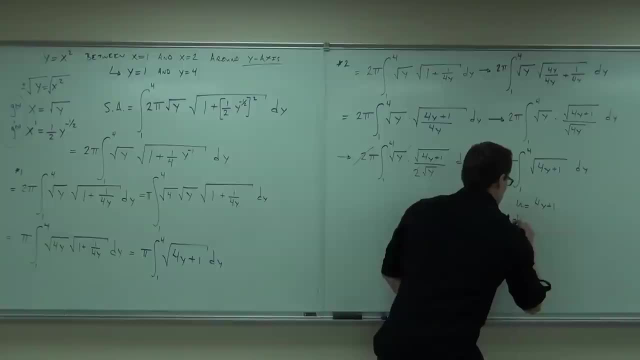 Don't forget that you do need a substitution, though You absolutely must. Du equals 4dy. Du over 4 equals dy. That's the derivative of 4y plus 1.. That's the derivative of 4y plus 1.. 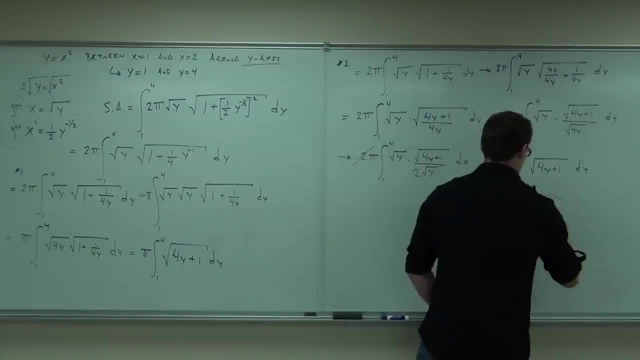 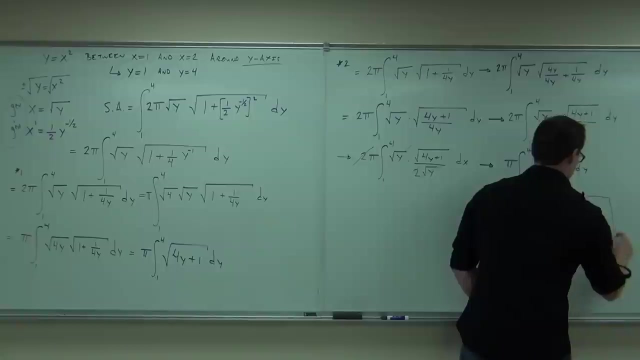 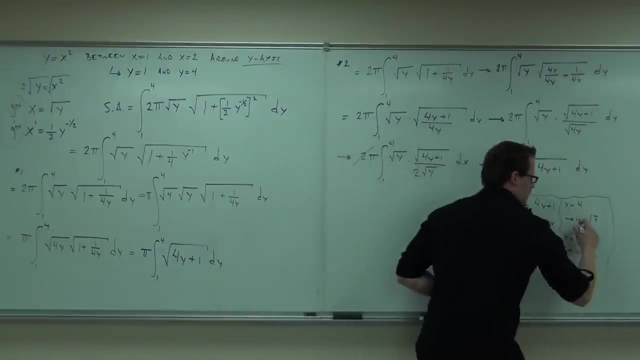 What else do you want to do right now? Let's do that. I'm sorry, When u is 4, you get how much? And u is 1., Sure, 5.. So those right there, those are our new bounds of integration. 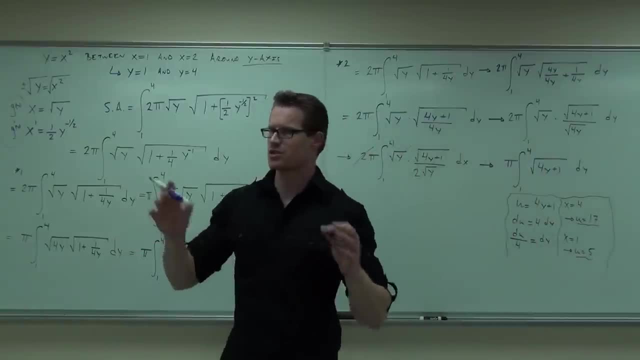 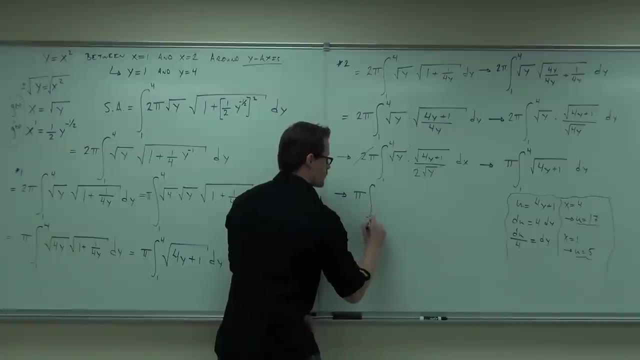 We're not going to have to substitute back in for x's later. We have these in terms of u. We're good to go, So let's rewrite our integral real quick. before we do it. We'll have a pi. We'll have this integral from 1 to- I'm sorry- 5 to 17.. 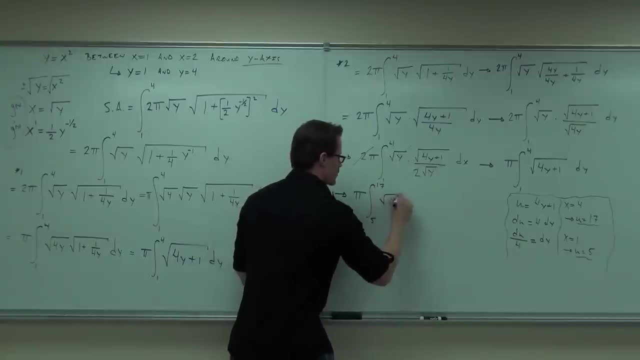 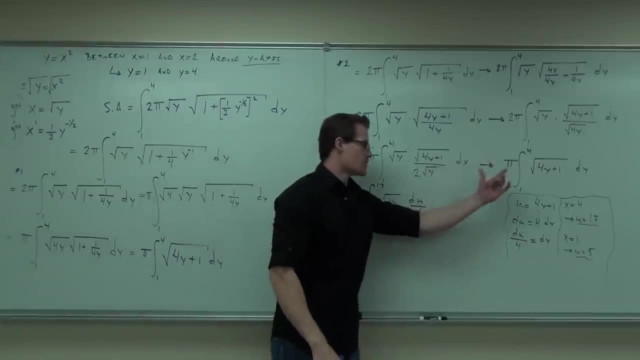 Because we just changed bounds Square root of u Du over 4.. Don't forget that the dy becomes a du over 4.. That's the derivative of 4y plus 1.. So 4y plus 1, u. 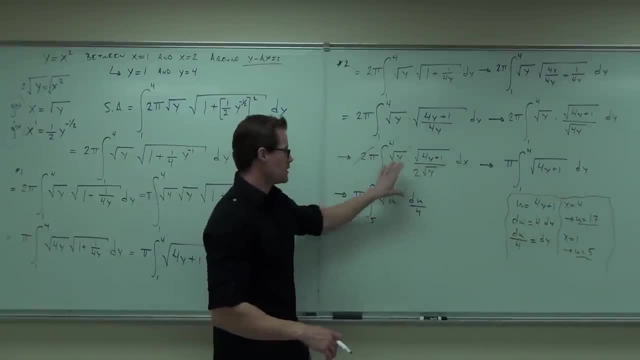 17 from the 4 when we plugged it in, 5 from the 1. after we plugged it in Du over 4, that's equivalent to dy. So we have the appropriate integral right now. Quick head nod if you're okay getting that far with the calculus. 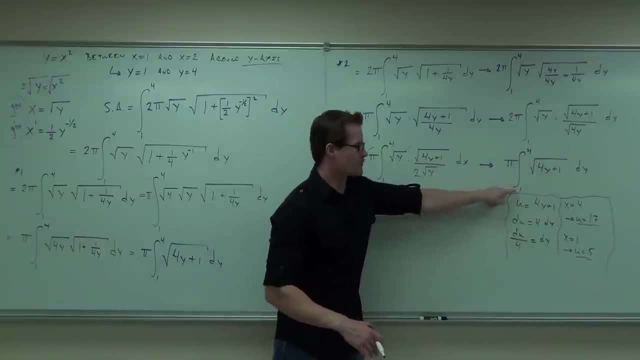 Yes, yes, okay, cool, Are you ready to do the integral? Yeah, it basically fits our integration table. Maybe I'll write it one little different way here. What's the integral? You have to do the integral, right? I don't know if this is the right way to do this. 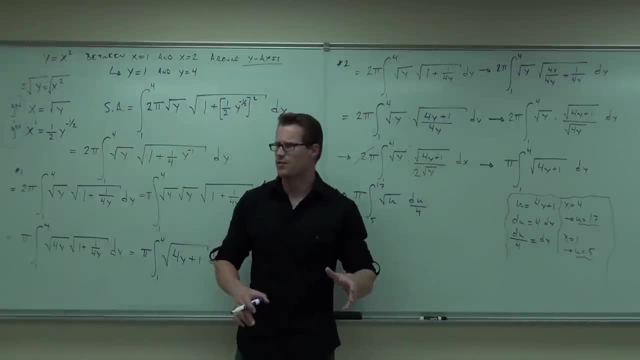 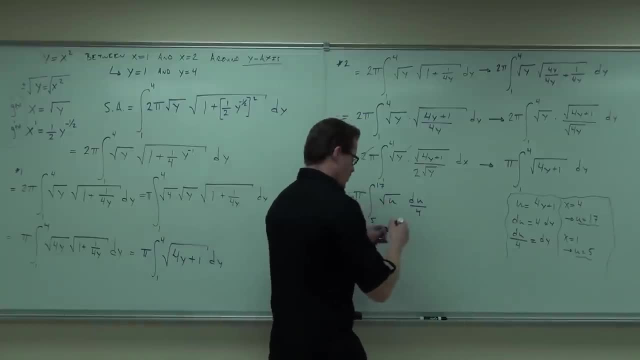 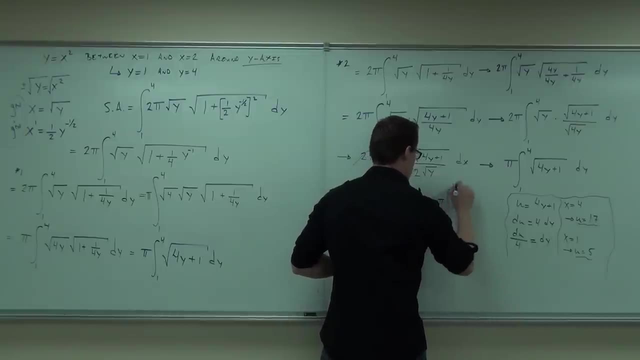 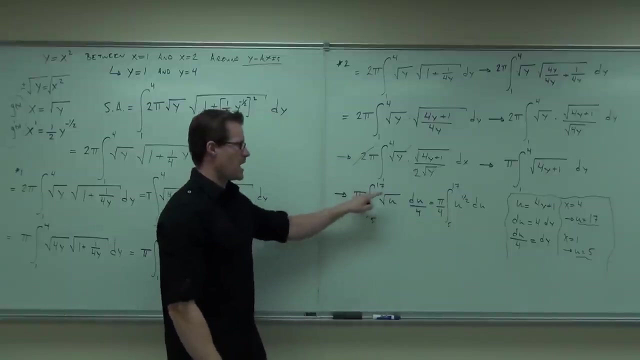 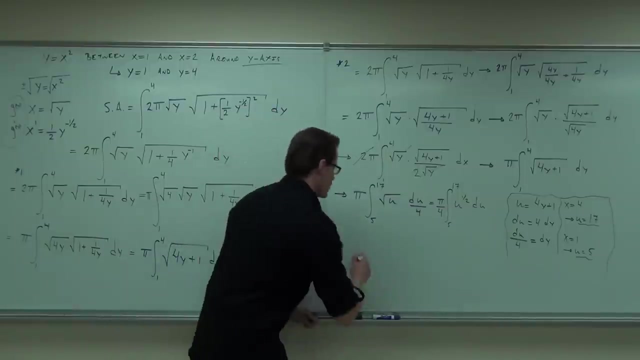 integral. Yeah, it basically fits our integration table. Maybe I'll write it one little different way here. Pull that 4 out in front. We have pi over 4, so pi over 4, u to the 1 half going from 5 to 17, basic integral. Now we all know that the integral of u to the 1 half is u. 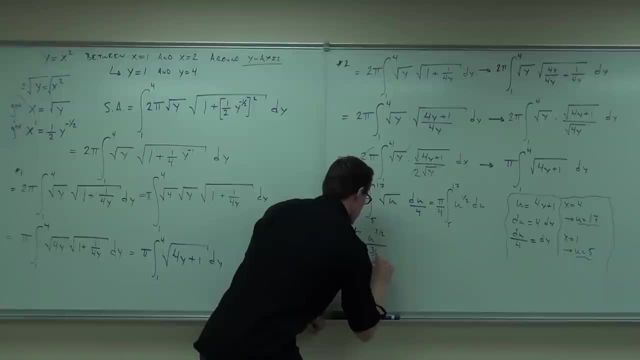 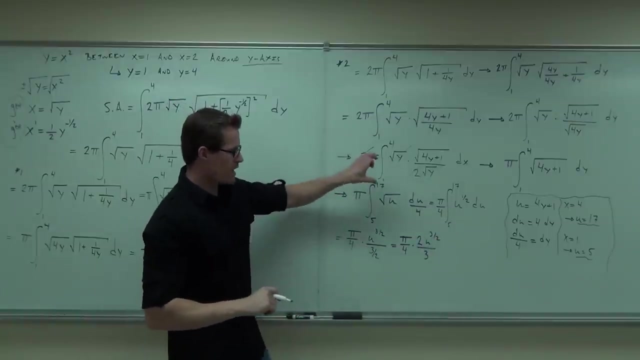 to 3 halves over 3 halves, That is pi over 4 times 2. u to the 3 halves over 3 multiplied by 4.. Hey, we've got to simplify that plug. in some numbers we'll be good to go. 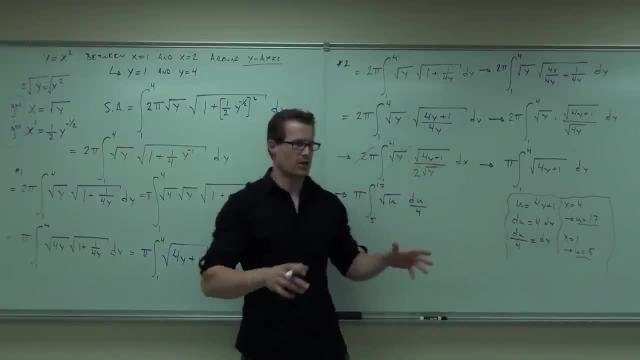 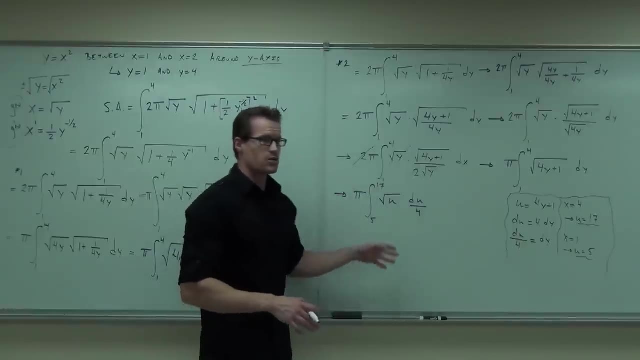 du over four, that's equivalent to dy. So we have the appropriate integral right now. Quick head nod if you're okay getting that far with the calculus. Yes, yes, Okay, cool, Are you ready to do the integral? Yeah, it basically fits our integration table. 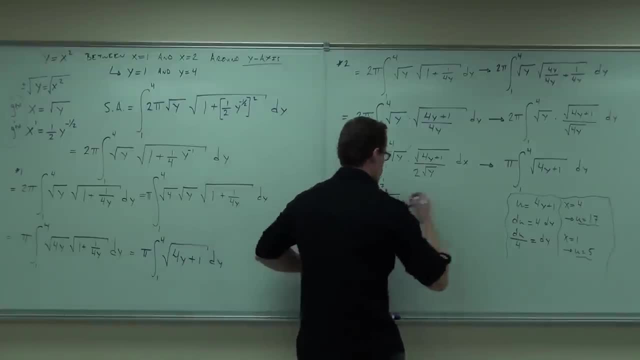 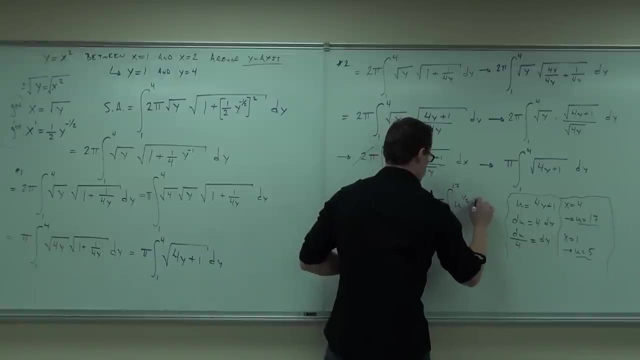 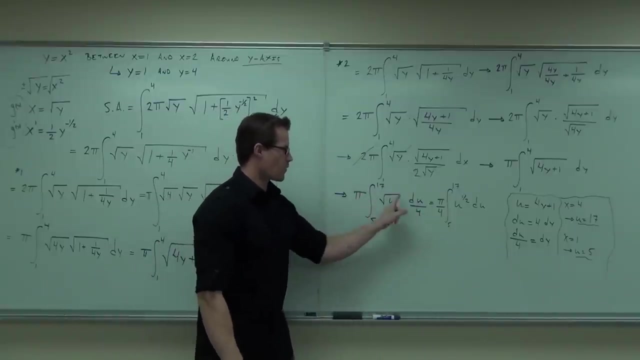 Maybe I'll write it one little different way here. Pull that four out in front. We have pi over four, So pi over four. u to the one half, going from five to seventeen Basic integral. Now we all know the integral of u to the one half is u to three halves over three halves. 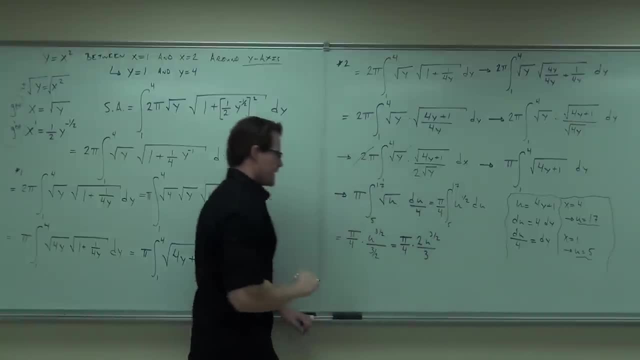 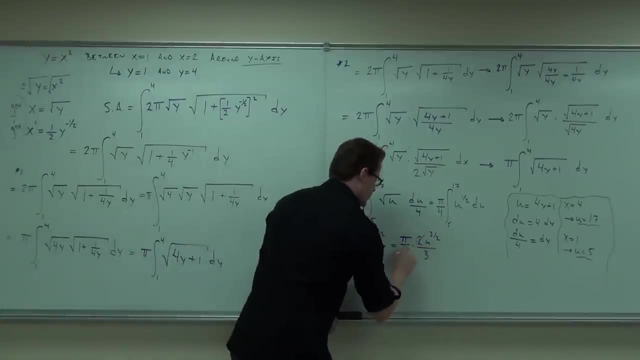 That is pi over four times two? u to the three, halves over three. Hey, we got to simplify that. Plug in some numbers We'll be good to go. So, two with the four, We're going to get pi over six. 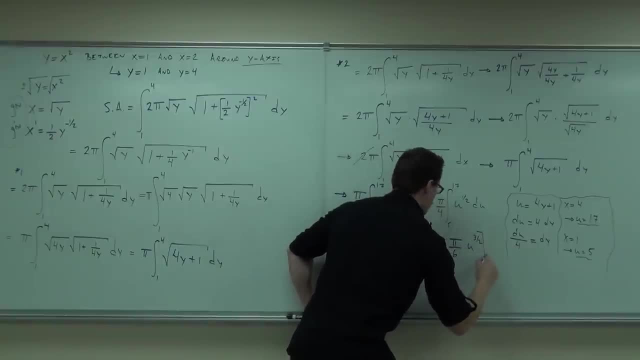 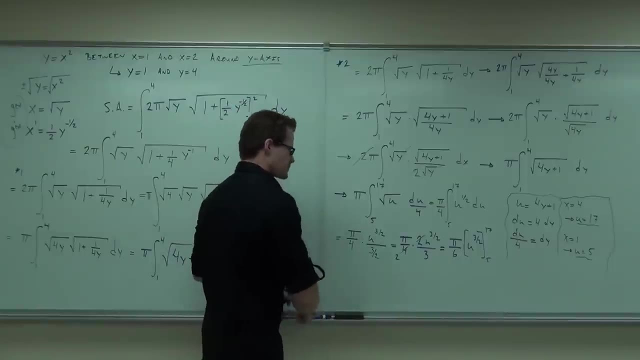 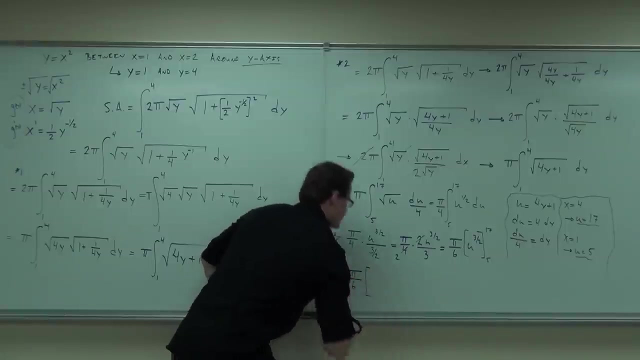 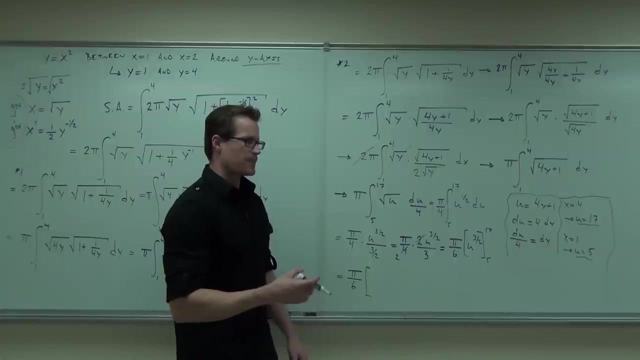 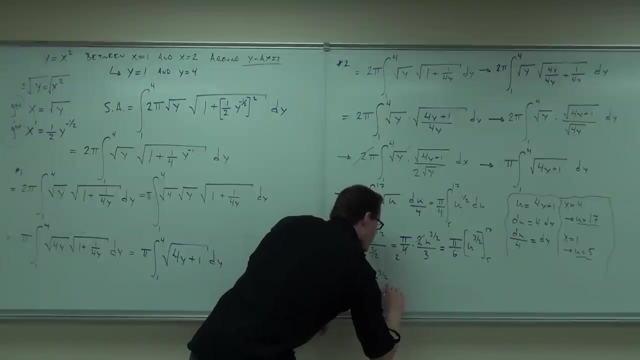 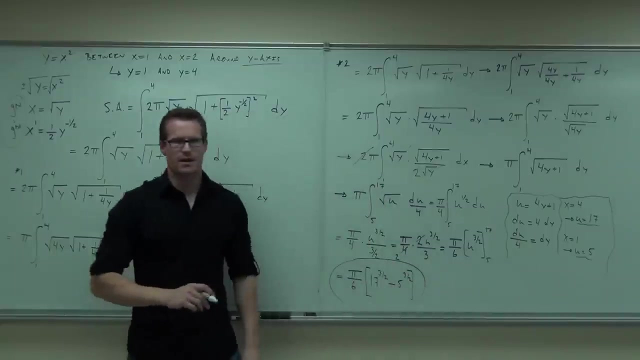 U to the three halves. Oh, we're going from five to seventeen. Now we're going to plug in seventeen to the three halves power. Seventeen to the three halves power. That's right. In fact, some books, some books, leave it just like that because they're like seriously. 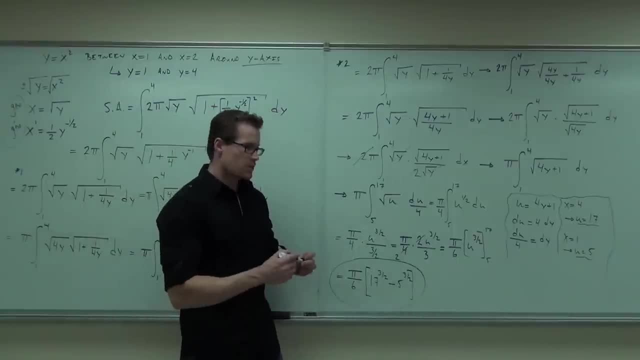 are you going to go any further than that? You know what are you going to do. Well, it doesn't really matter If you can make it down that far. I know you know what you're doing. okay, These numbers generally are not very nice. 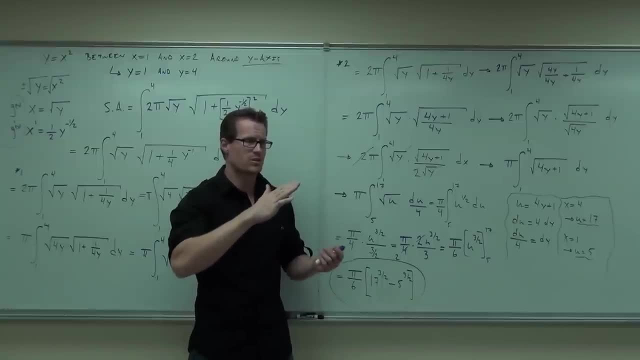 You're dealing with a length right, Which is why you get the weird seventeen root seventeen thing And five. remember those From the length of the curve. you get a lot of those. You get those a lot with that. So with this you're going to get those a lot as well. 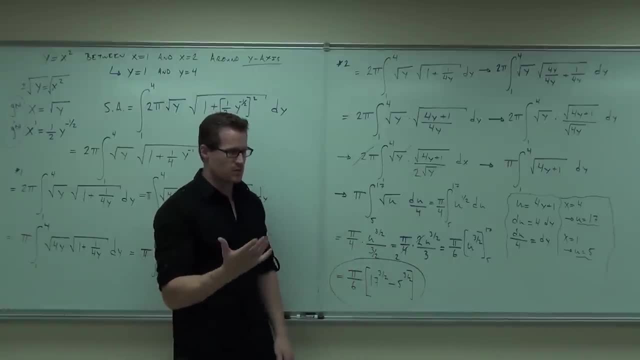 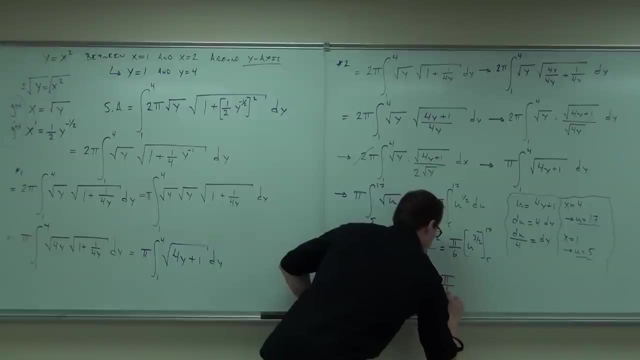 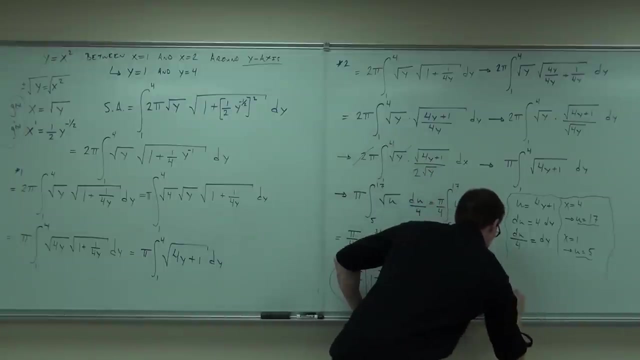 You're just multiplying by circumference right now, Length times circumference basically. So you get a lot of this, So leave it like that or go one step further And we leave our length problems in the same form there- Exponents- instead of breaking it down further. 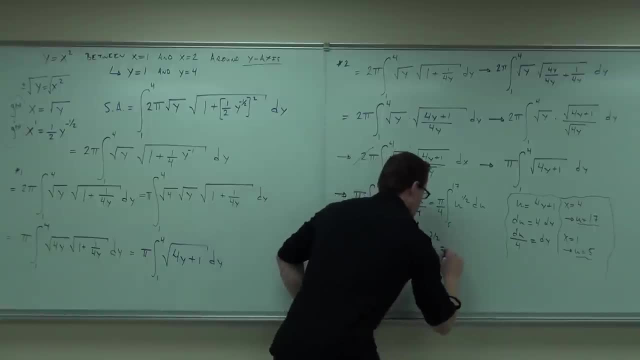 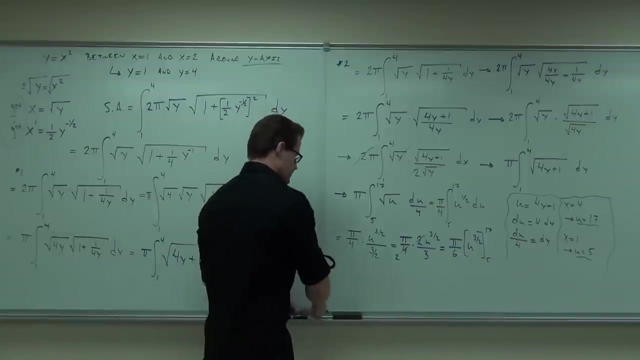 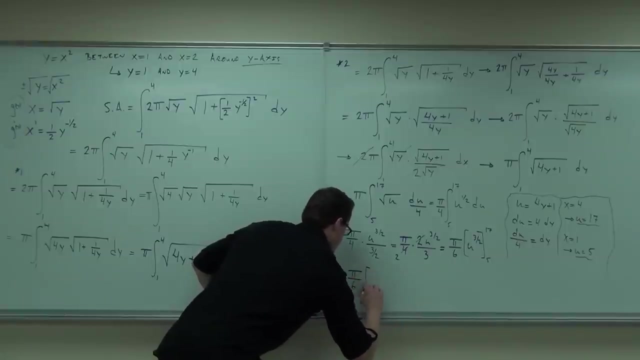 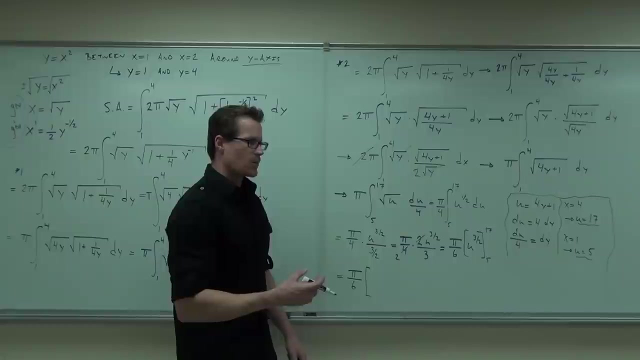 So two with the four, we're going to get pi over six. u to the three halves. oh wait, I'm going from five to 17.. Now we're going to plug in: 17 to the three halves power. 17 to the three halves power. 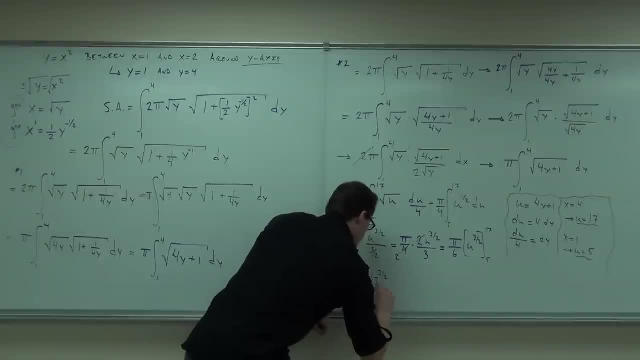 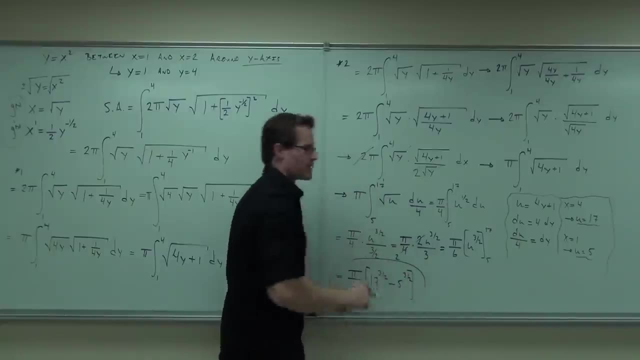 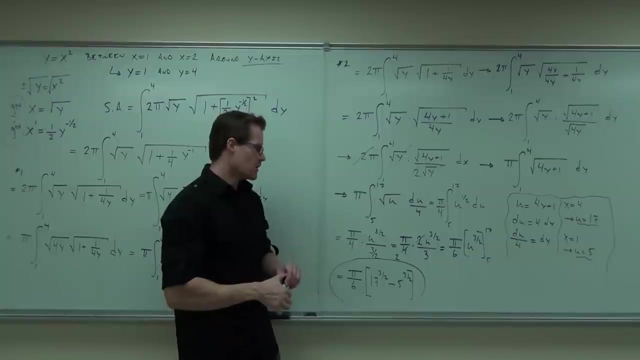 Yeah, that's right. In fact, some books, some books, leave it just like that because they're like: seriously, you're going to go any further than that. You know what are you going to do. Well, it doesn't really matter. 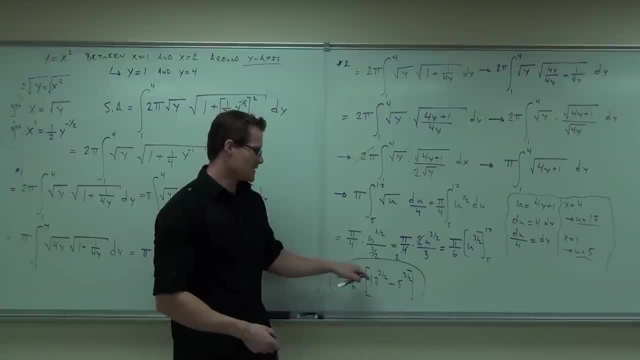 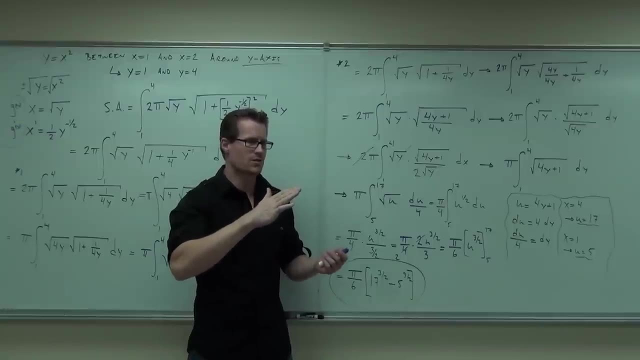 If you can make it down that far. I know you know what you're doing, okay, But these numbers generally are not very nice. You're dealing with a length, right, Which is why you get the weird 17 root 17 thing. 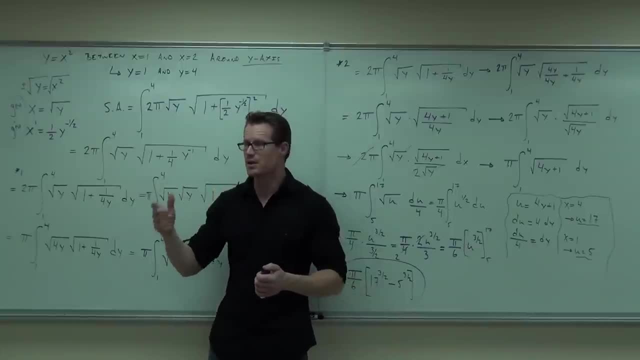 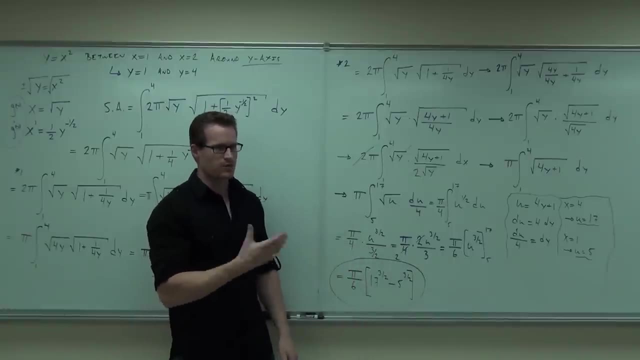 and the five. remember those From the length of the curve. you get a lot of those. You get those a lot with that. So with this you're going to get those a lot as well. You're just multiplying by circumference right now. 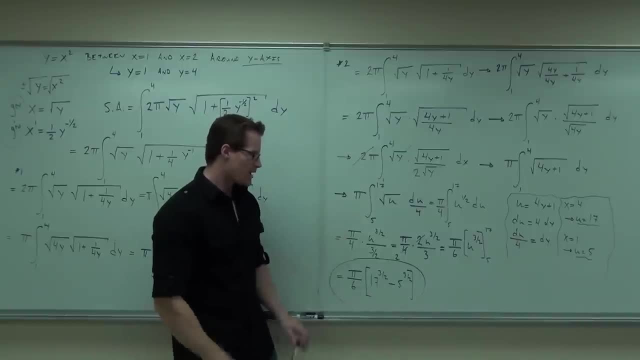 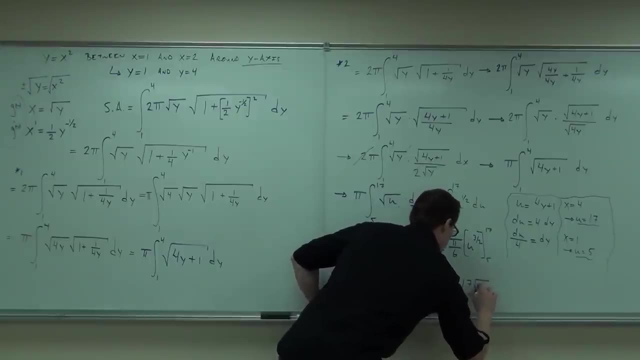 length times, circumference, basically. so you get a lot of this, So leave it like that or go one step further. Can we leave our length problems in the same format, the exponents instead of? I'm going to keep breaking it down for a bit. 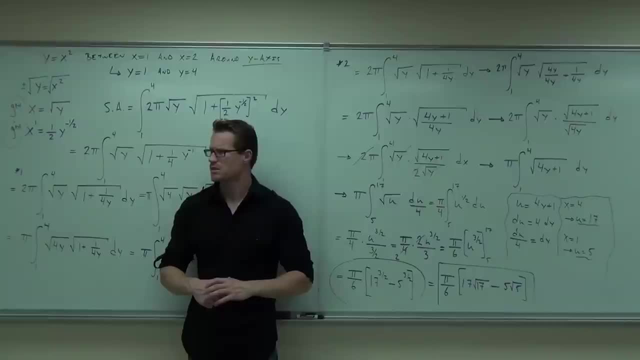 By the way, do you know why 17 to 3 1⁄2 power gives you 17 root 17?? Yeah, it's the square root of 17.. OK, it's because you have 17 squared times 17,. 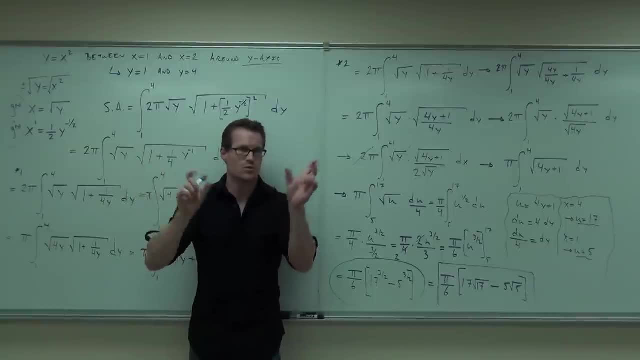 square root of 17,. square root of 17.. But you can't take out the next one, so you have 17 root 17.. That's the answer. Would you raise your hand if you feel OK with what we talked about so far today? 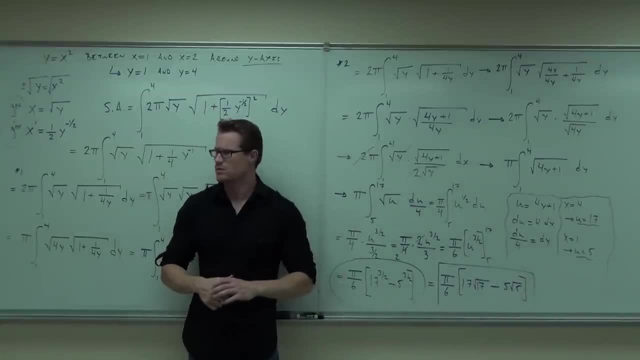 By the way, do you know why seventeen to three-halves power gives you seventeen root seventeen? It's because you have seventeen squared times seventeen, square root of seventeen, square root of seventeen, but you can't take out the next one, so you have seventeen root seventeen. 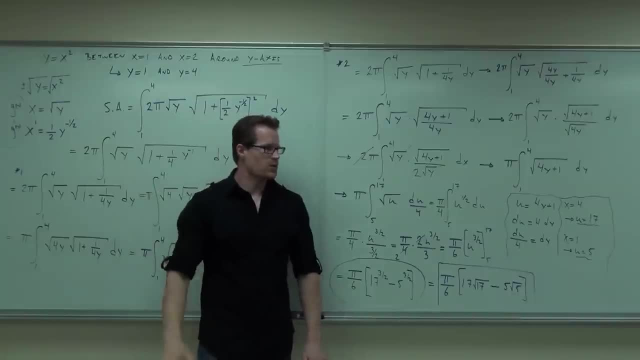 That's the answer. Would you raise your hand if you feel okay with what we talked about so far today? Alright, Well, are there any questions? I hope you enjoyed calculus.